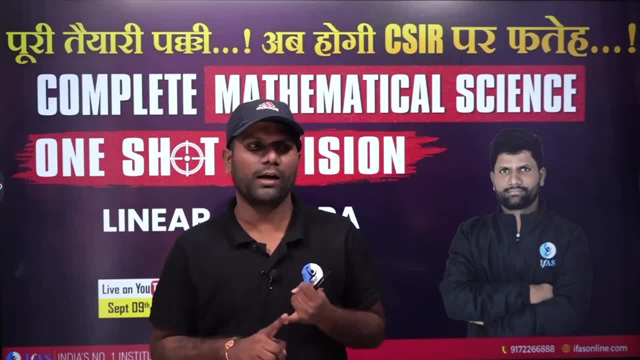 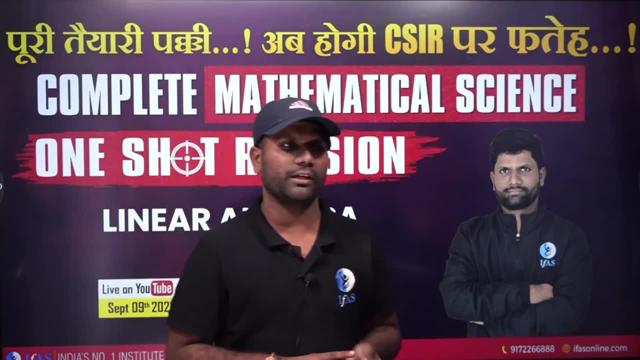 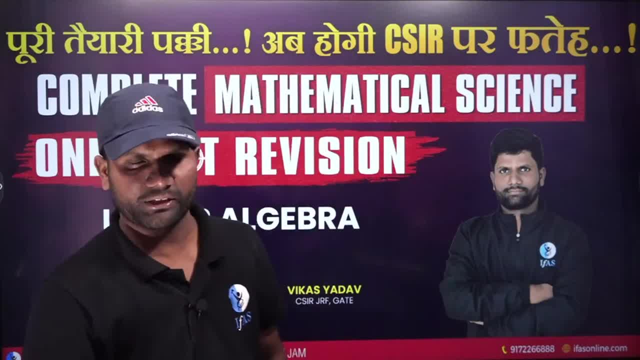 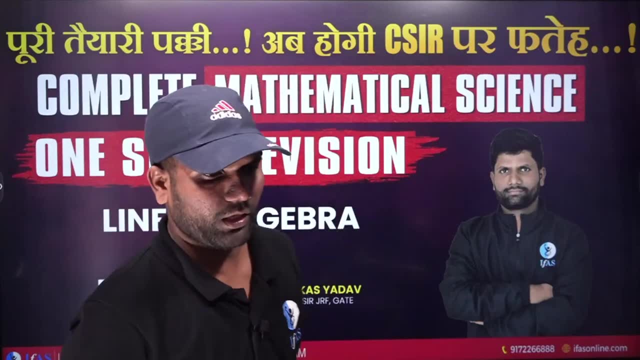 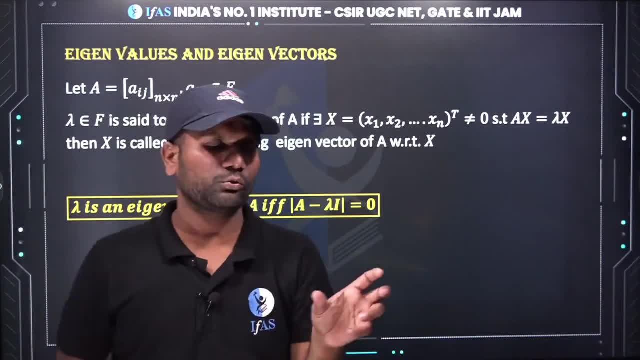 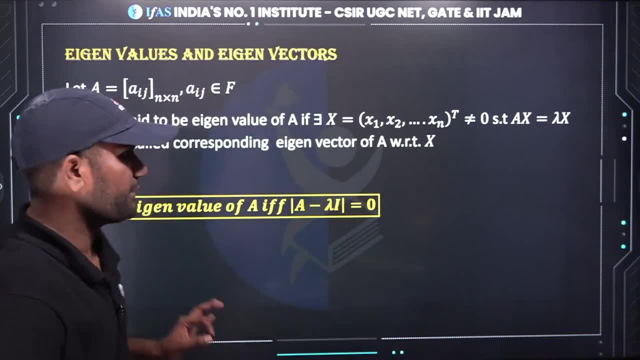 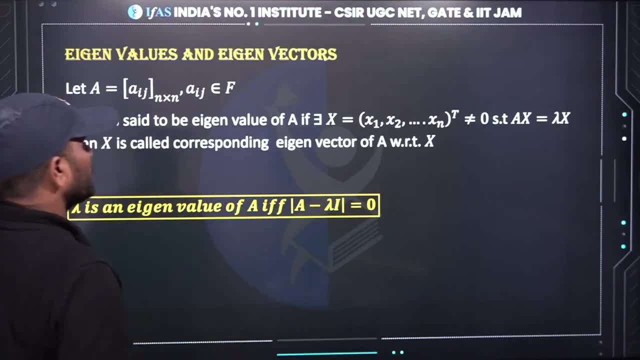 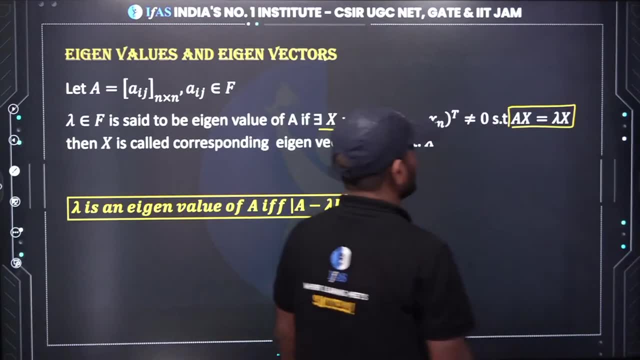 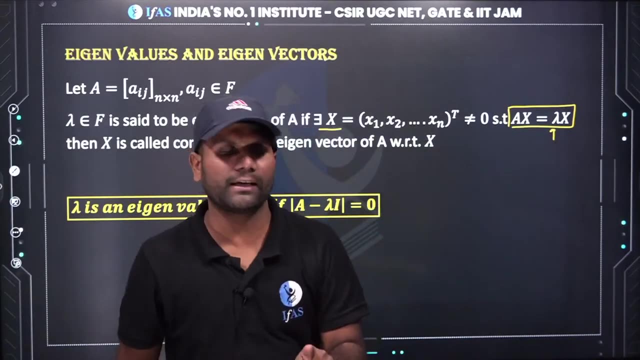 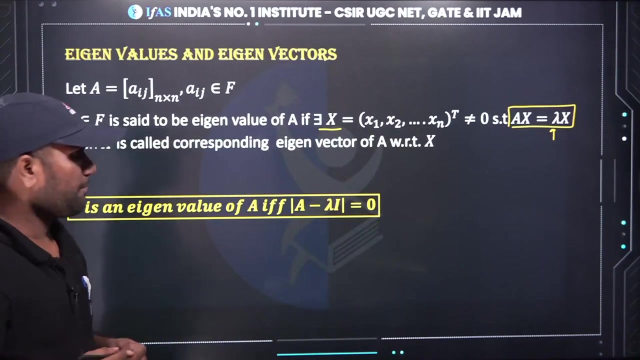 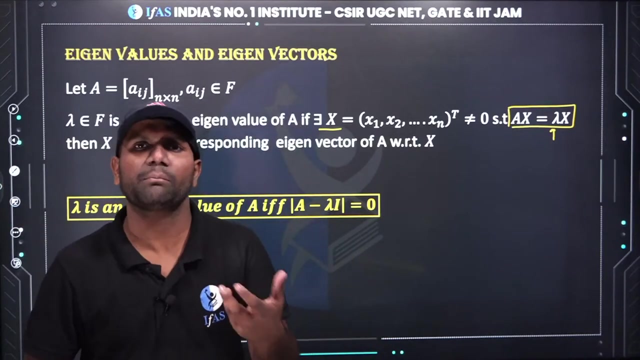 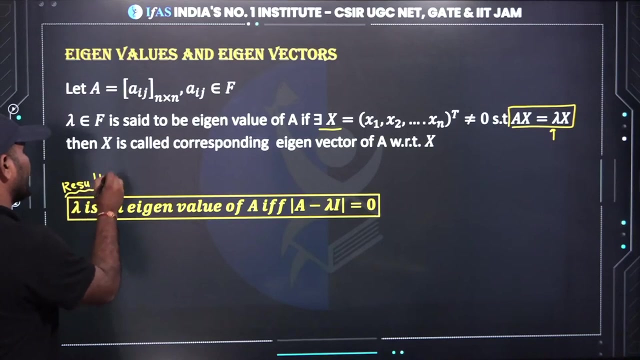 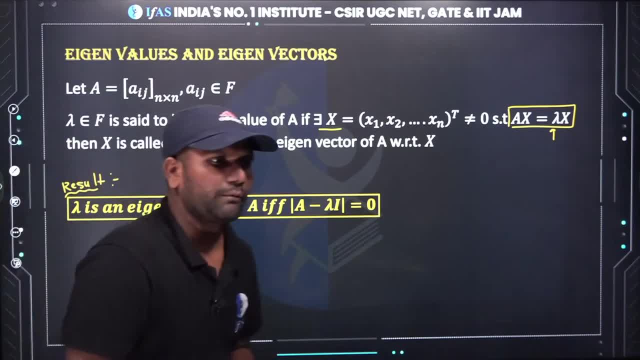 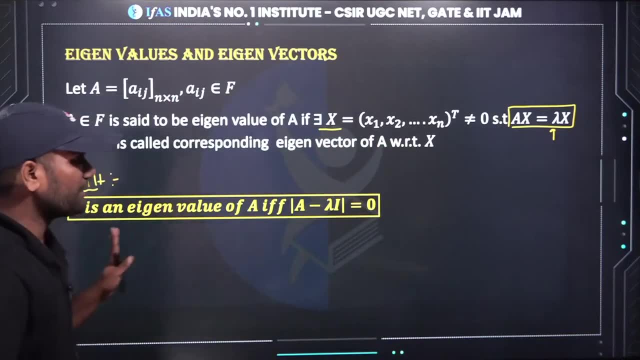 that is lambda, is an eigen value of A. if you get the determinant of A minus lambda I, you will get 0. but keep in mind all of you are going for the exam, the result you are seeing that the determinant of A minus lambda I is equal to 0. 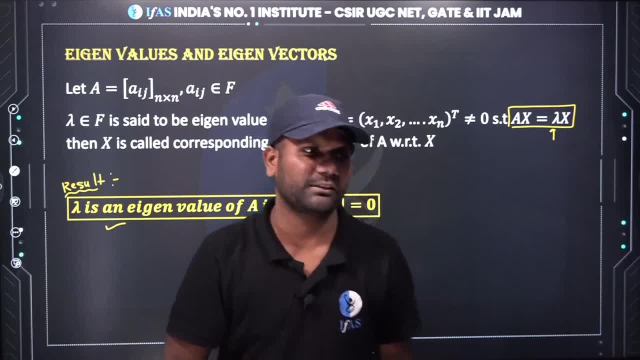 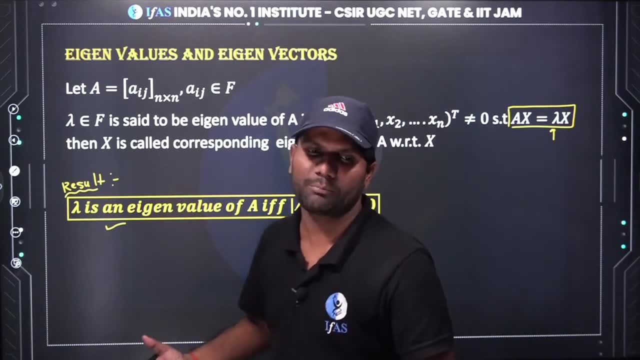 you will apply this only when you don't have any way. what does it mean when you use any other result or property if you are not able to find the eigen value? if you don't have any way, then go and apply this result at the very end. 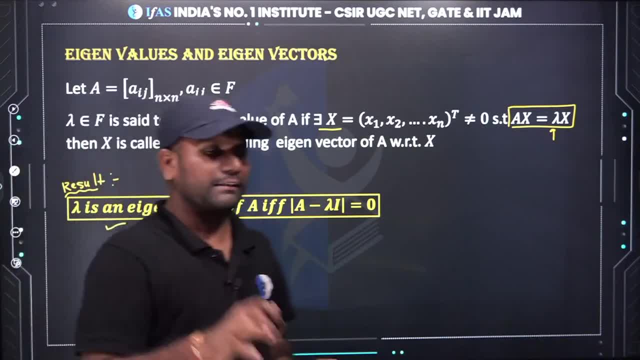 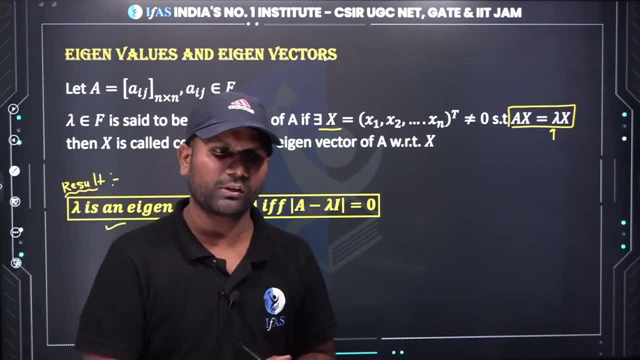 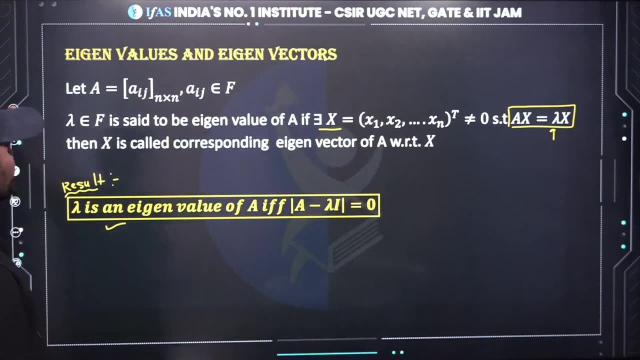 otherwise we have results, properties, all these things. we will use them to solve. ok, those who are joining. if you don't like the session, then like it. I will get this PDF. I will upload it tomorrow. ok, now, what is characteristic polynomial? characteristic polynomial if you take a polynomial. 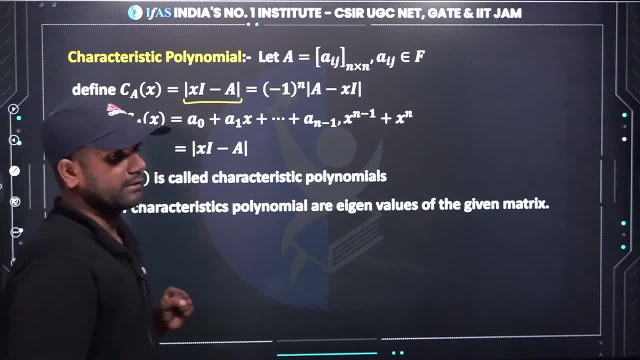 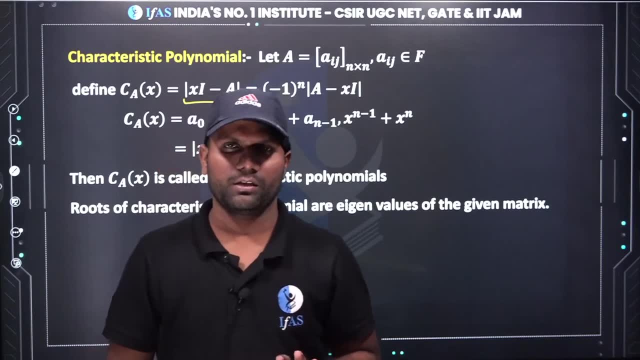 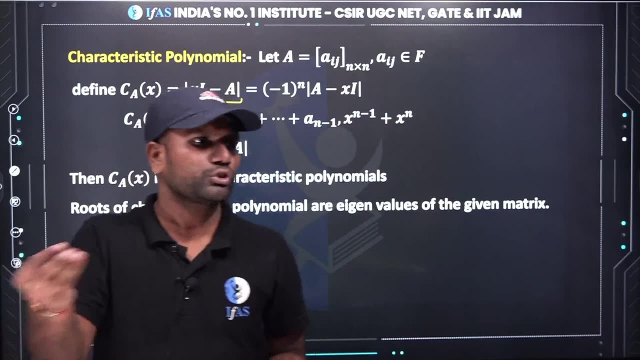 if you solve the determinant of XI minus A, you will get a polynomial. this polynomial is called characteristic polynomial and the roots of characteristic polynomial are the eigen value. how can you find eigen value, find the characteristic polynomial, take its root, or you can find the determinant of A minus lambda I. 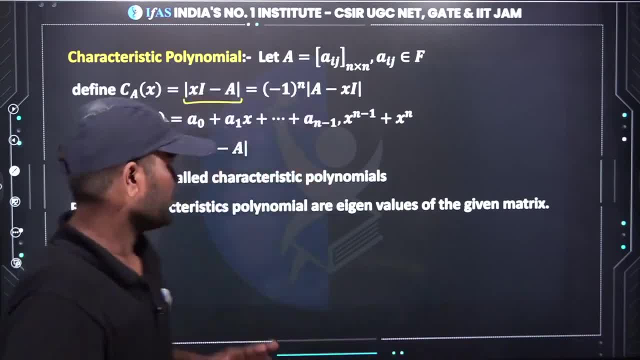 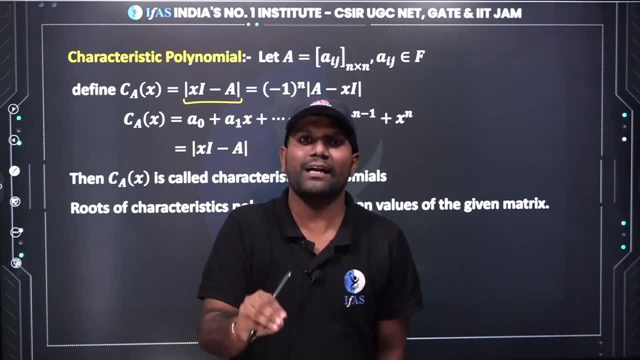 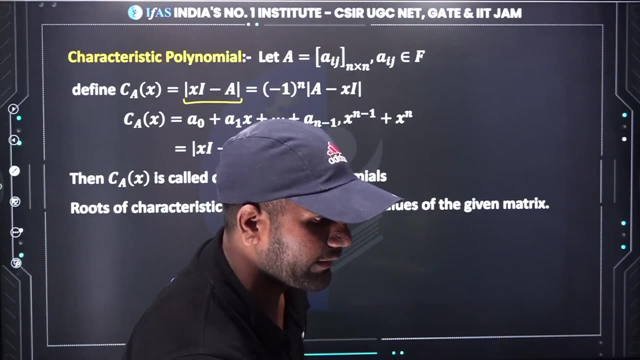 is equal to 0. you have both ways. now keep in mind there is not much time left in the exam in linear algebra. if you see matrix, then to discard, you have to discard the options in the exam. so to discard. we will talk about what kind of counter example. 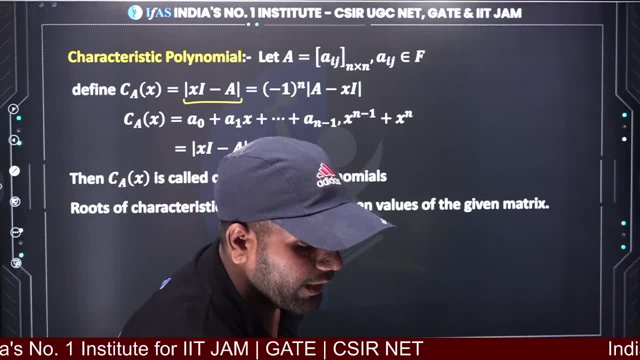 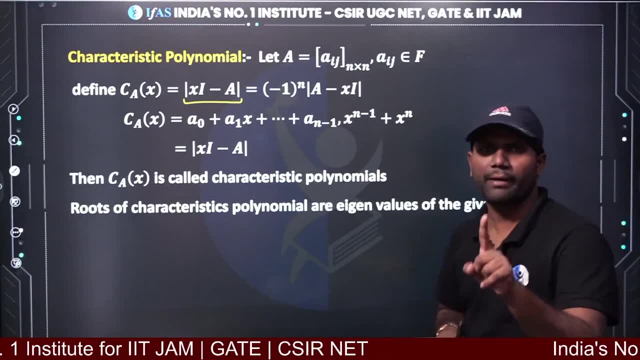 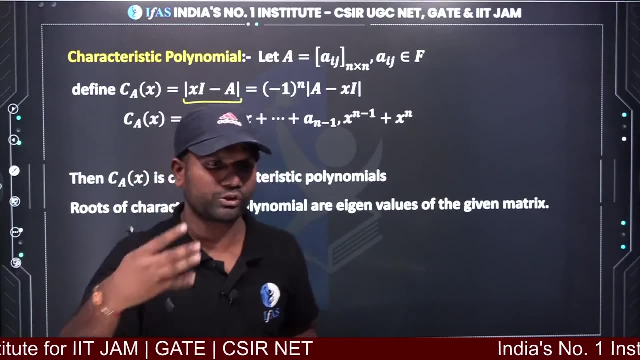 is used for maximum time. so here you can see if we talk about discard, keep in mind it is very important for the exam. if there is a question of linear algebra, then there are four types of counter examples. your one or two options will definitely be discarded. one or two will definitely be done. 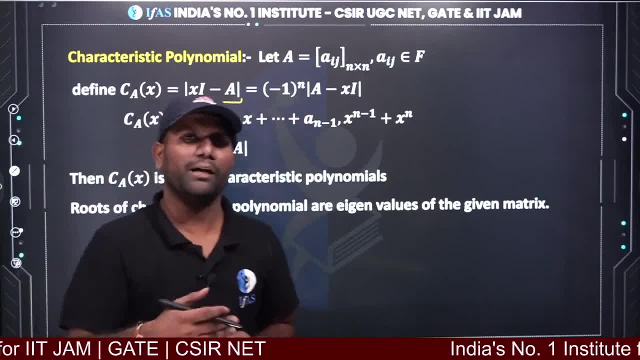 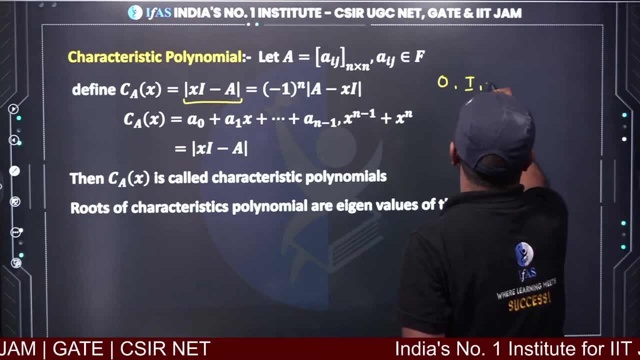 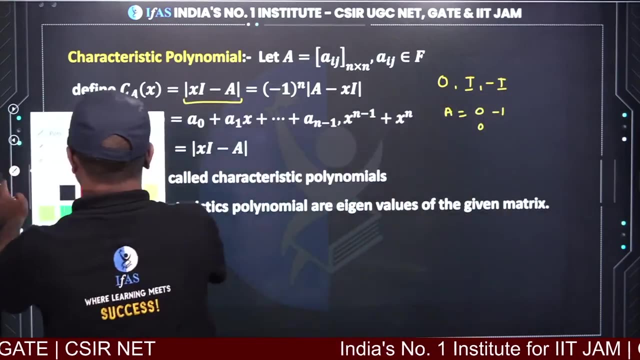 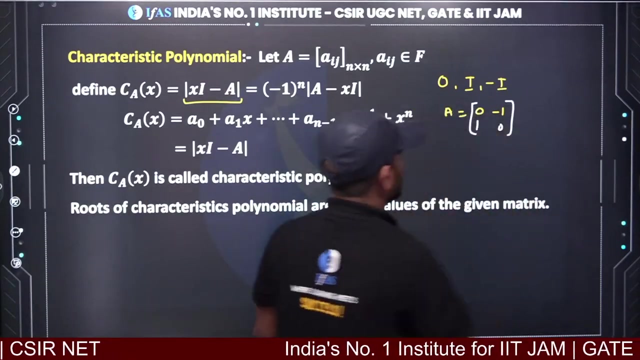 in the recorded course. pdf is not downloaded. you can view it there now, see here: take zero matrix, identity matrix minus of identity matrix, and take a special type matrix minus one zero. sorry, here will be one, keep in mind here- one zero. there are four types of matrix. 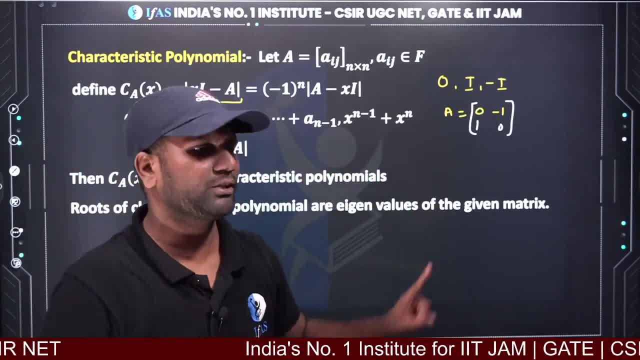 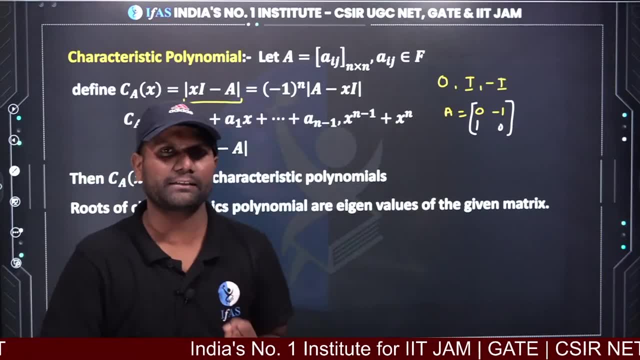 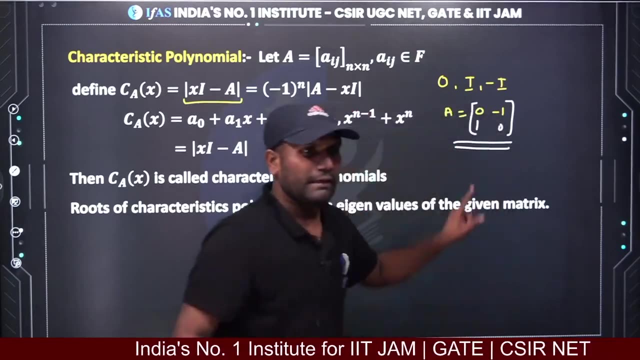 if any question comes from matrix, these four will be discarded for counter example. if you need to make counter example, then use them: zero matrix, identity matrix, minus of identity matrix, or you can take a special type matrix. what is special about this? what is special about this? what are the entries of this matrix? 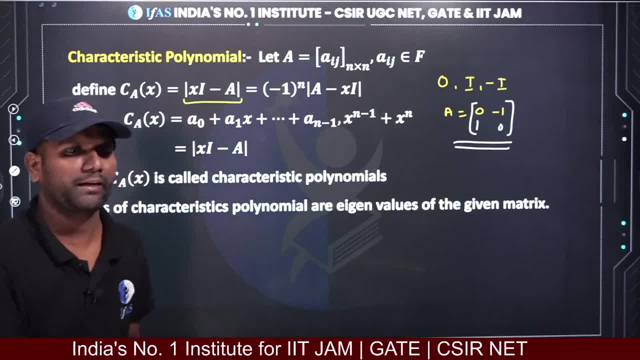 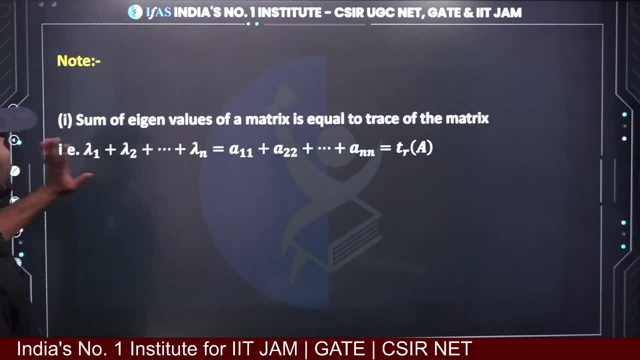 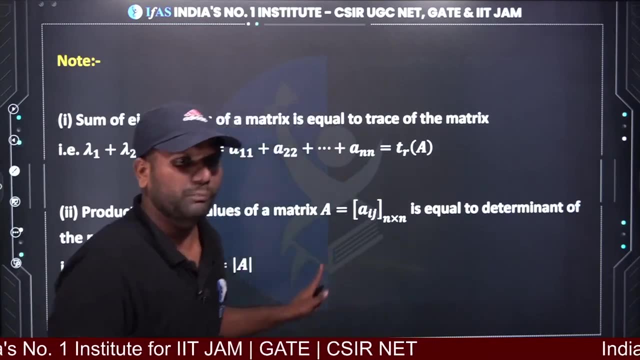 real number, but what are the eigen values of this? you will get imaginary number, so you have to use this. now we move ahead. there are some notes here. if you will add eigen value, sum of eigen value, what you will get trace. many times in exam questions were asked. 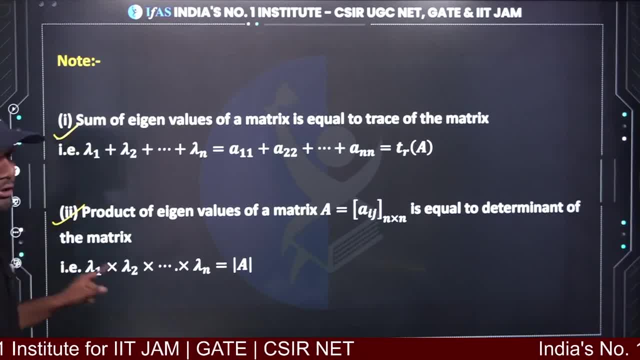 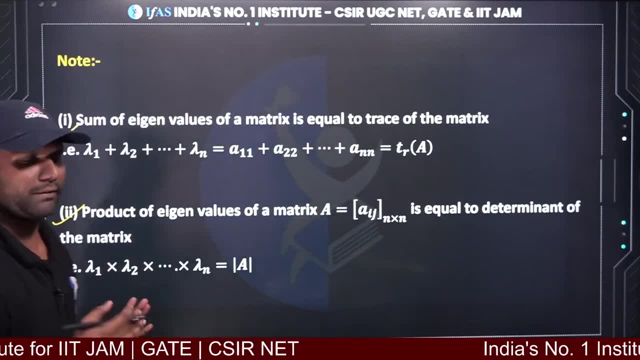 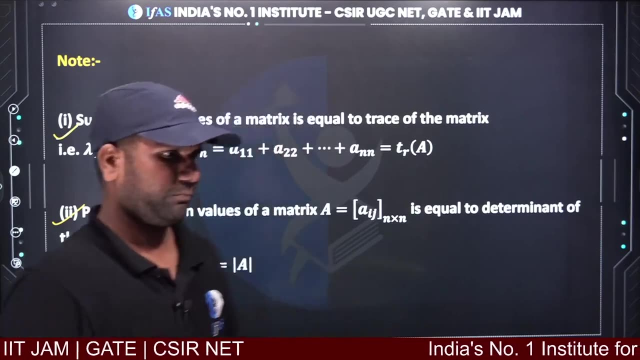 if you will add eigen value, you will get trace. if you will take product of eigen value product of eigen value, you will get determinant. there are some special things you should know. some small things i am telling you. after that we will go to question. there are some results and properties. 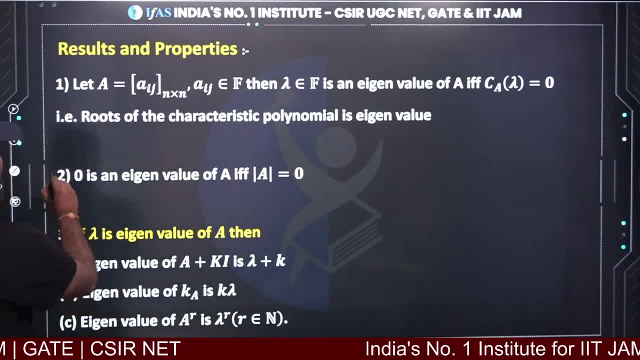 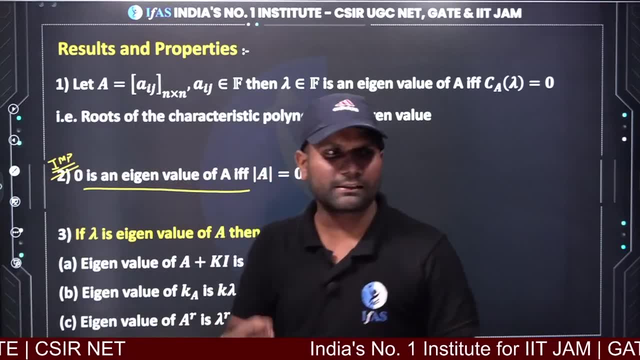 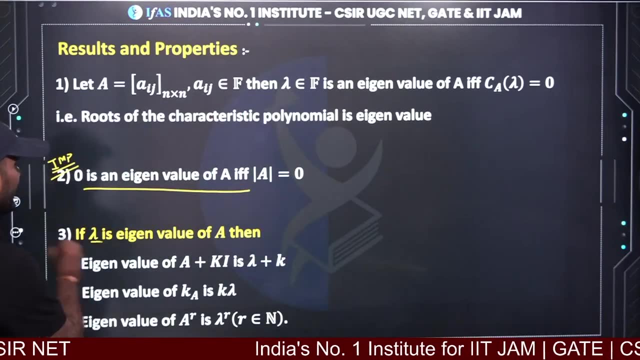 which are important results. for example, if any matrix eigen value or determinant is zero, in that case eigen value will be zero. if any matrix eigen value is zero, then determinant will be zero. everyone knows this. if you are given any matrix like A, if eigen value of A is lambda, 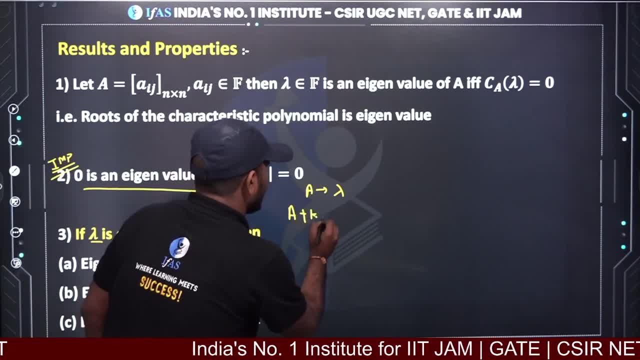 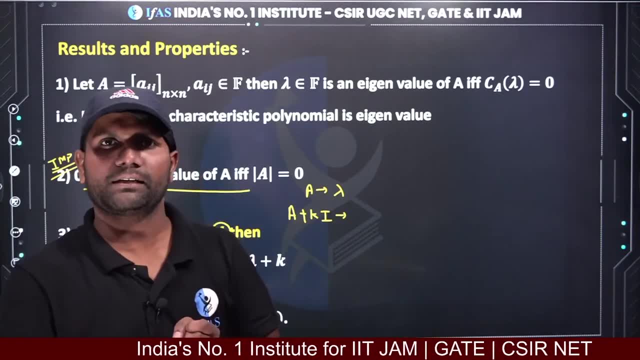 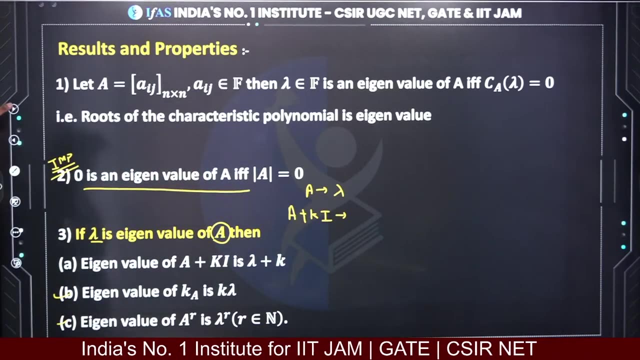 suppose eigen value of A is lambda. now someone ask you what will be eigen value in this case? you have to replace A with lambda and identity with 1. whatever you get will be eigen value. similarly, you can do it here or here. here one more important result. 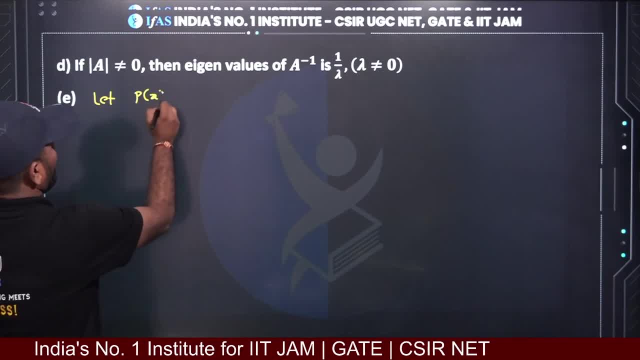 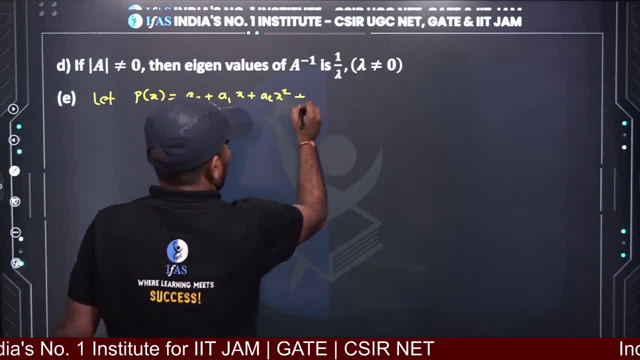 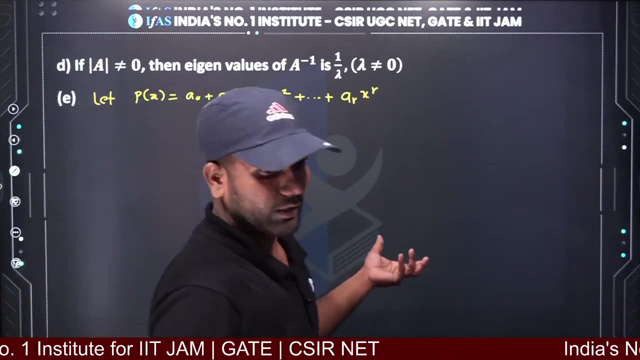 suppose i give you a polynomial late P of x, like A0 plus A1x plus A2x, square, and so on, plus Arx raise to R. i have given a polynomial. you are watching a polynomial. good morning, kavita. now, if i convert this polynomial, 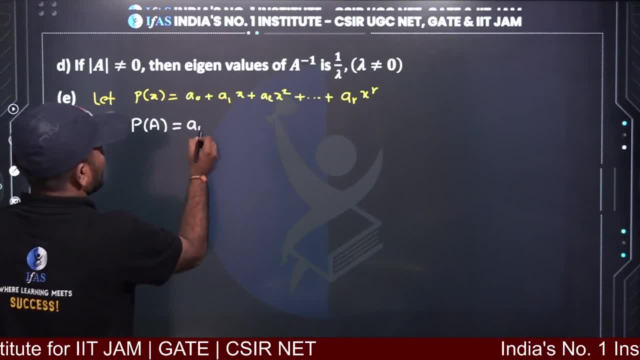 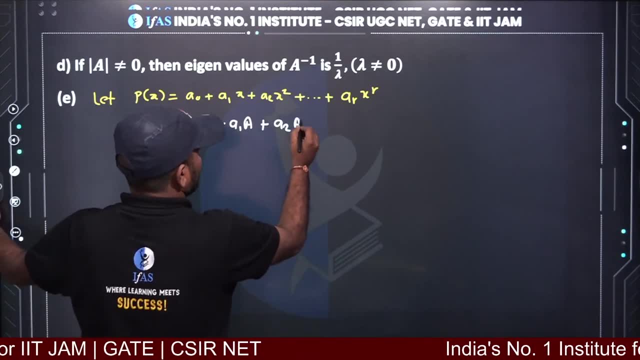 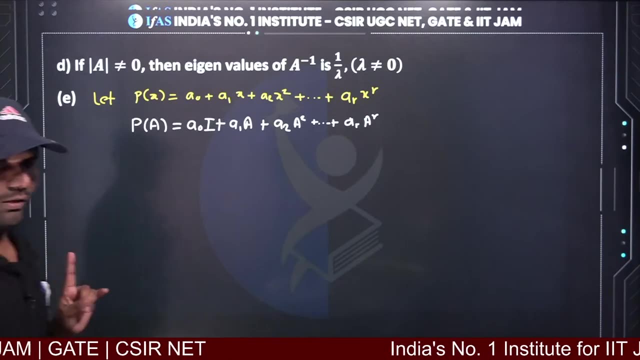 into matrix. then what will i get? P of A A0 into identity matrix, plus A1 into A, plus A2 into A square, and so on, plus Ar into Ar, raise to R, so you will get a matrix. now the thing is, if you have eigen value of 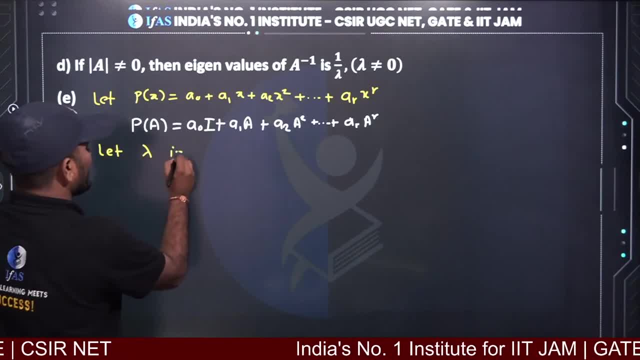 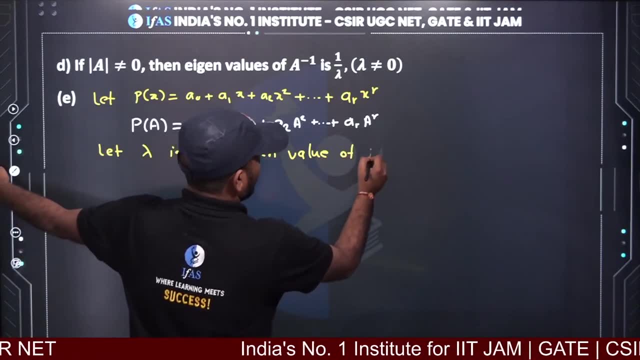 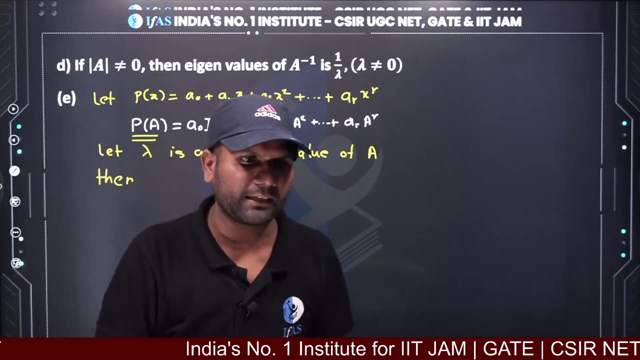 let suppose you take lambda. what is lambda? lambda is an eigen value. lambda is an eigen value, eigen value of A. if A eigen value is lambda, in that case now someone ask you: what will you get? P of A, P of A? you will get matrix. yes, you will get pdf. 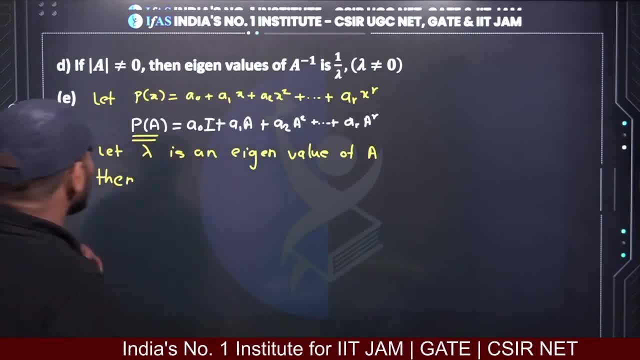 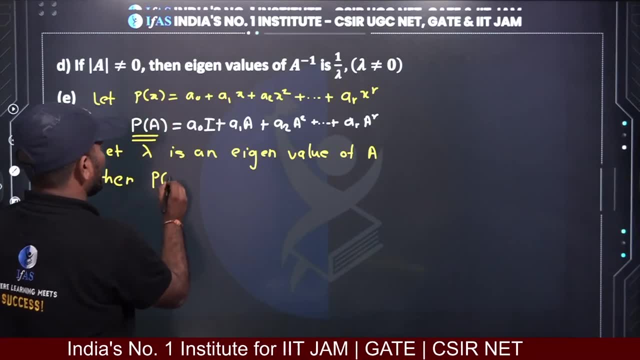 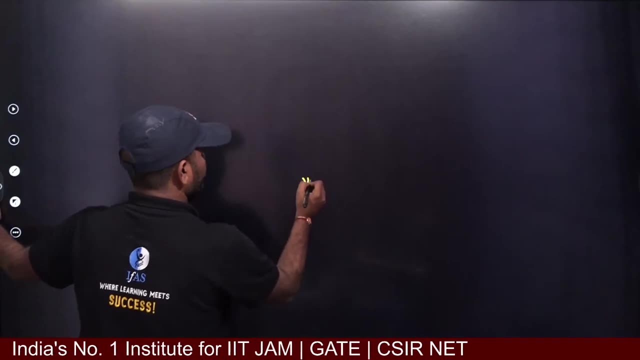 pdf. you will get in color app. ok, if someone ask you: if lambda is an eigen value, then what will you get? P of A eigen value in that case, you just have to substitute lambda in one place. P of lambda will be: is an eigen value, of is an eigen value. 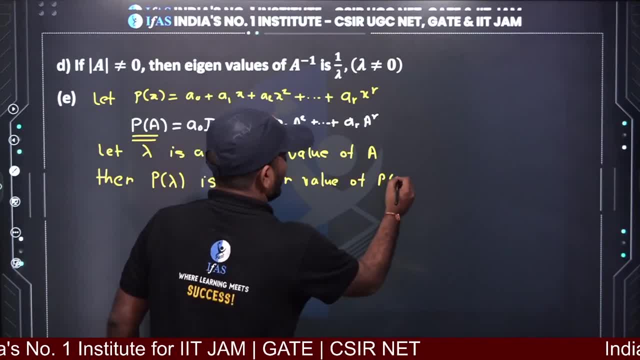 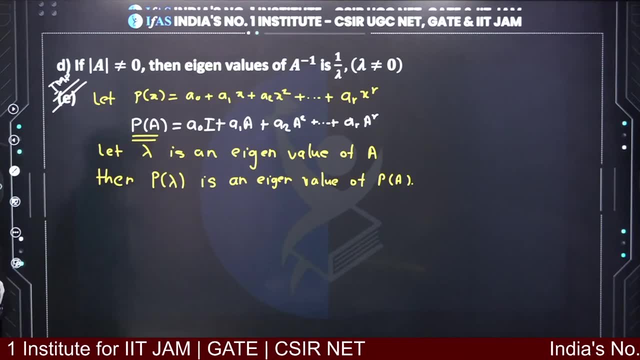 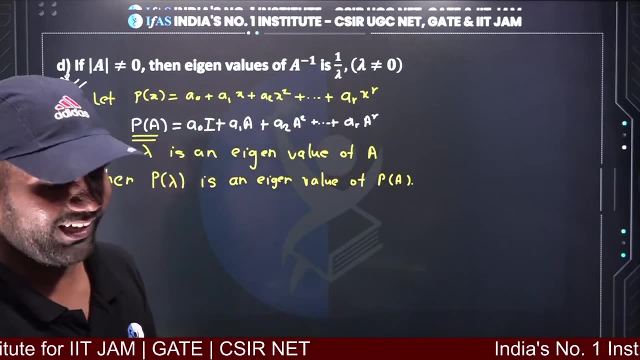 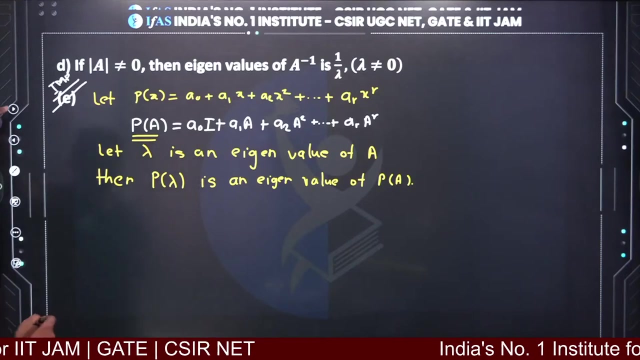 of P of A. if i say the most important result of P eigen value is this, because last time in exam this question was asked based on this result, and here in exam, question is always asked. i hope you will clear. yes, yes, you are coming, ok. ok, let's move to next slide. 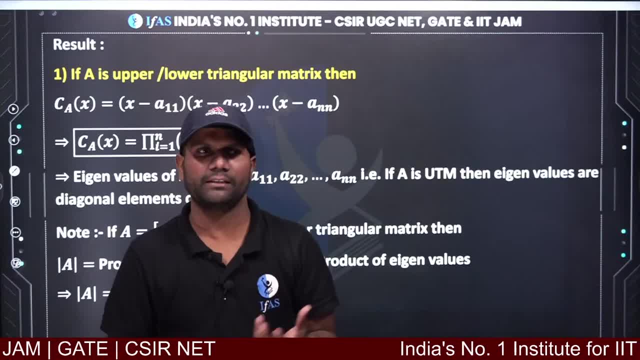 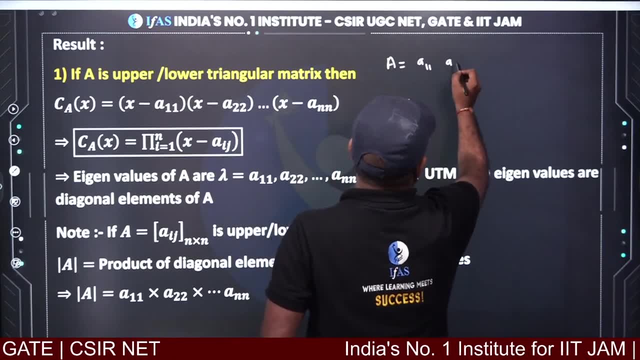 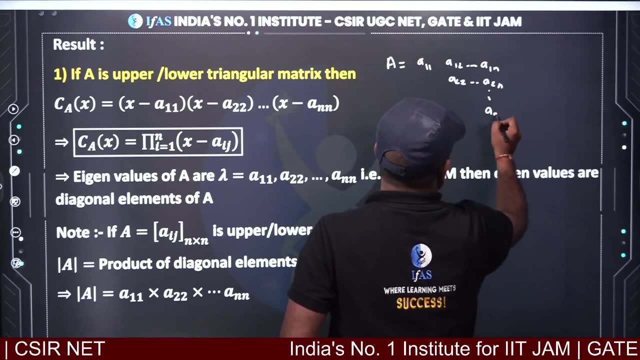 so here some special things like upper triangular matrix or lower triangular matrix. so what are their eigen values? suppose i give you upper triangular matrix A11, A12 and so on, A1n, A21, 22 and so on, A2n. let's continue like this. 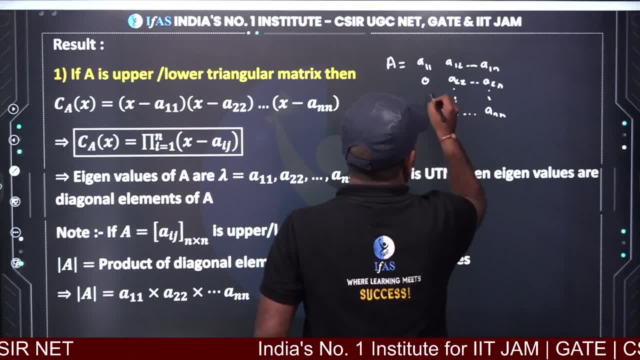 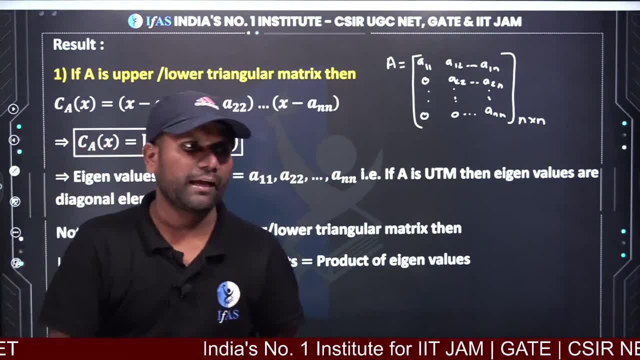 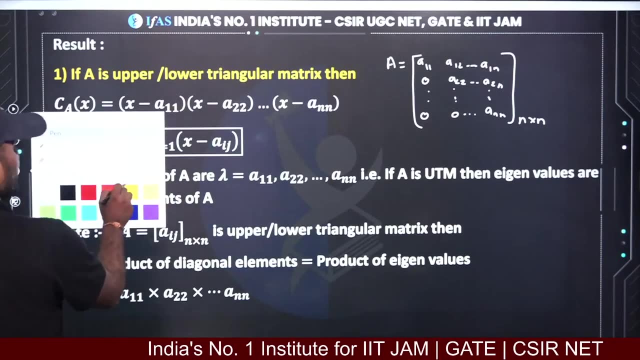 so here, if i give you any upper triangular matrix or lower triangular matrix, ok, whether it is upper triangular matrix or lower triangular matrix. so what are their eigen values for upper triangular or lower triangular matrix? so their eigen values are diagonal entries. diagonal entries are their eigen values. 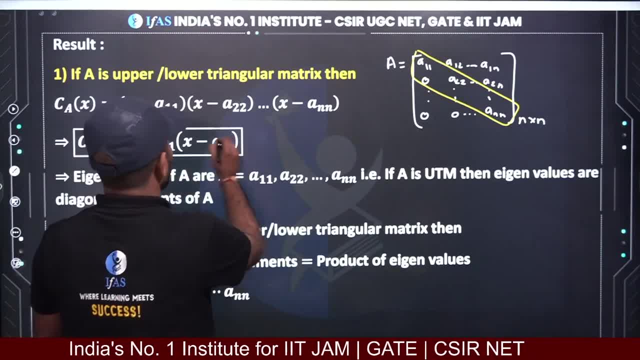 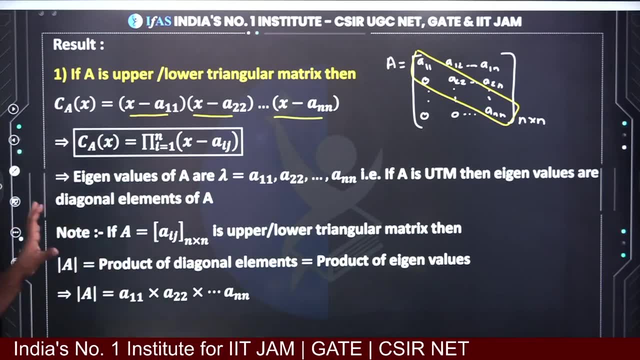 so in this way you can get characteristic polynomial. what will you get? X-A11, X-A22, X-ANN. so this is an important result about diagonal matrix, or we can say for upper triangular and lower triangular matrix: ok, let's go. and here is one more special result. 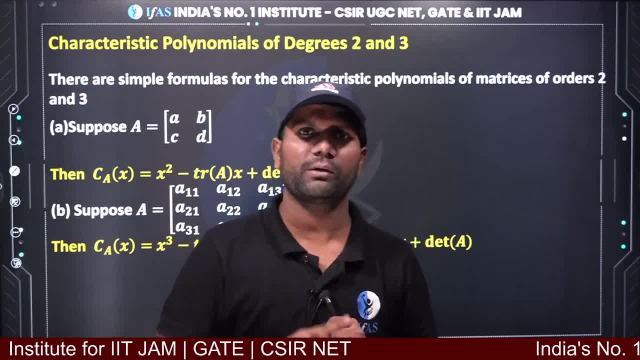 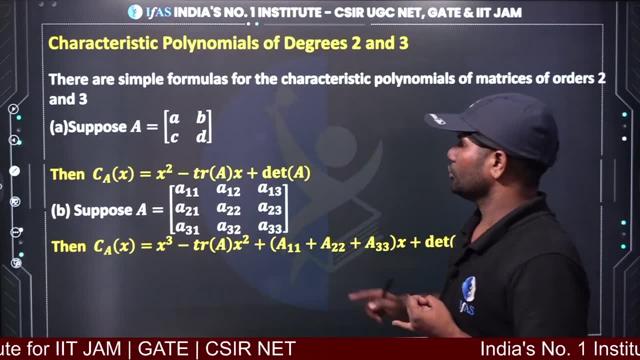 if you get question of eigen values, then in last you have to apply determinant of A-lambda I. otherwise what you have to do, you have to apply all these results like 2x2 matrix. so to solve 2x2 matrix what we have to do 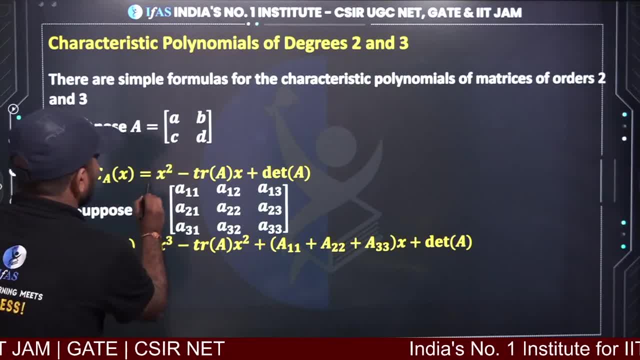 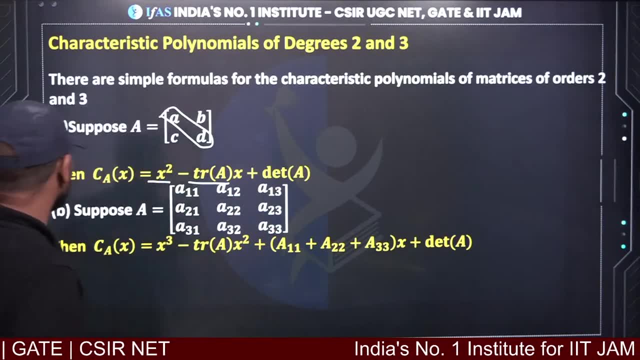 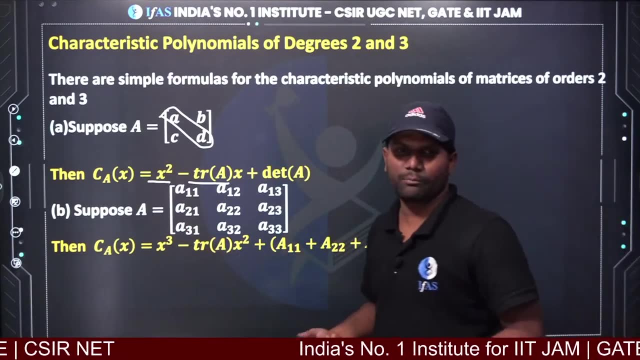 so characteristic polynomial of 2x2 matrix is X square minus trace of A, X square minus trace of A into X plus determinant of A. ok, and suppose we have a 3x3 matrix. suppose you have taken 3x3 matrix now if you have to find its characteristic polynomial. 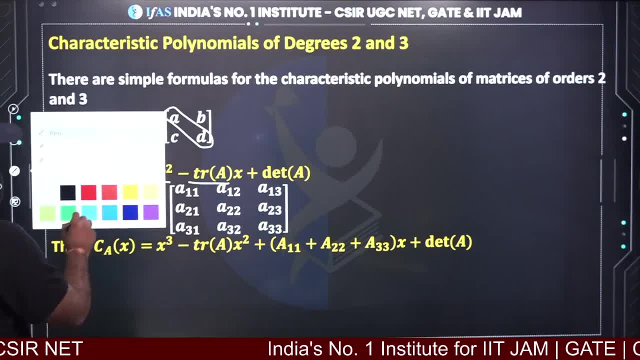 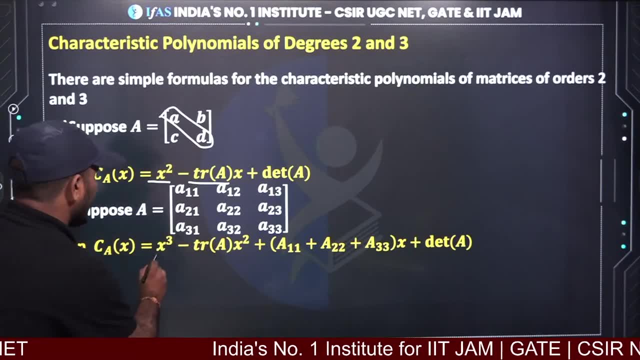 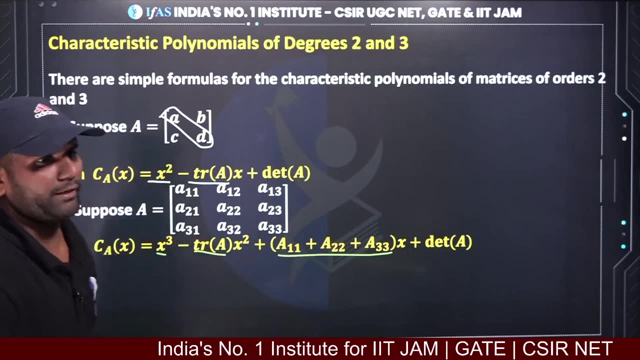 then what will you get? so if you have 3x3 matrix, then to find its characteristic polynomial we have one more result. you have to apply this X cube minus trace of A into X square plus A11, A22 plus A33, into X plus determinant of A. 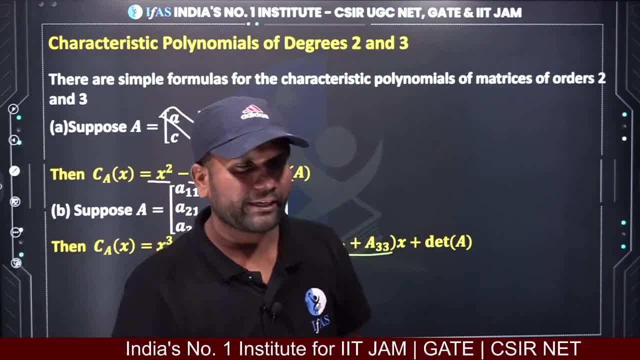 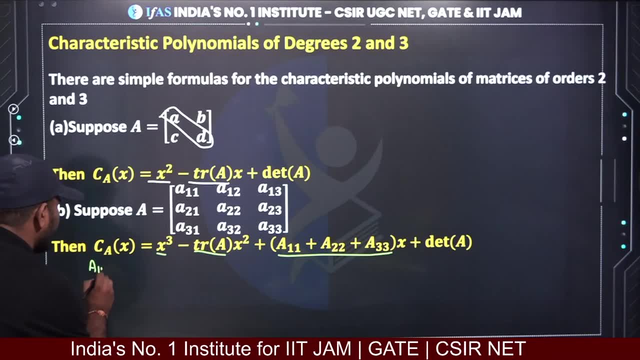 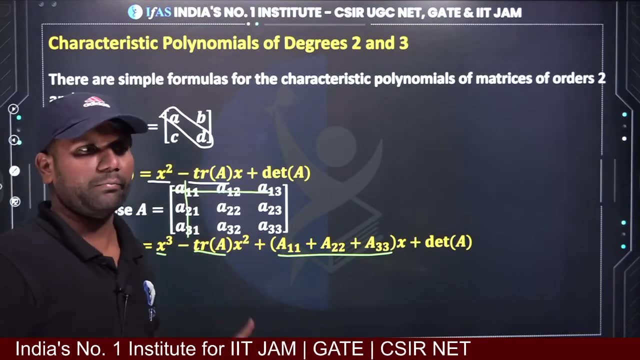 now, here it comes: A11, A22, A33, what will be? I have told you many times. you must be knowing, if you want to find A11, what you have to do: delete first row and first column. remaining matrix determinant. determinant of remaining matrix. if we remove first row and first column, 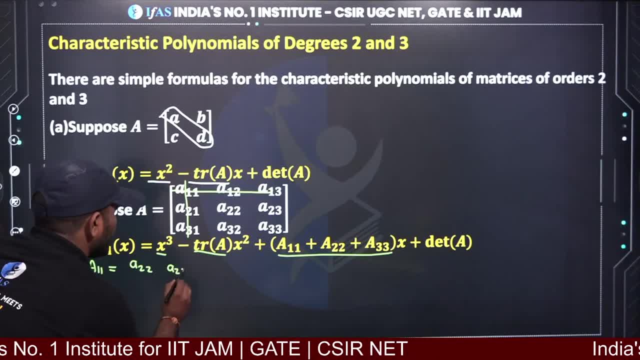 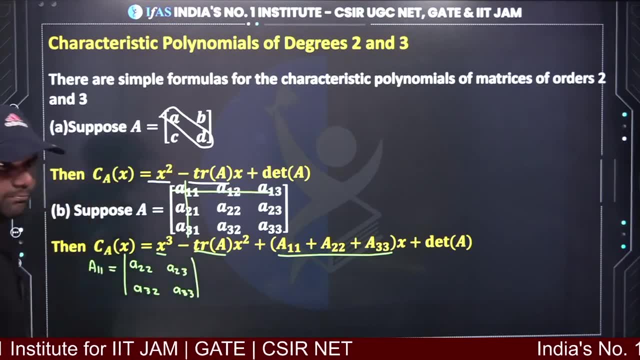 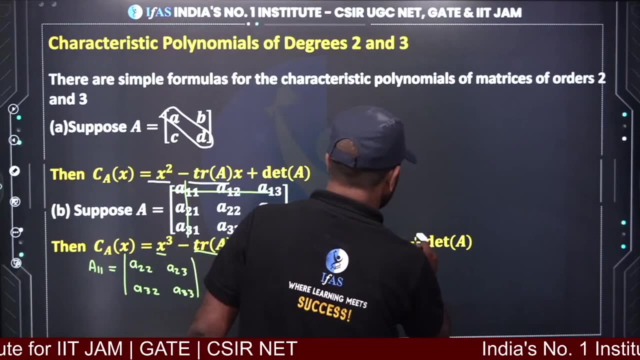 this is equal to A22, A23. this will be A32, this will be A33. so determinant of this 2x2 matrix. now, if we come here- yes, here- we have to go with alternate sign. so this is typing mistake. this is not rough, this is printing mistake. 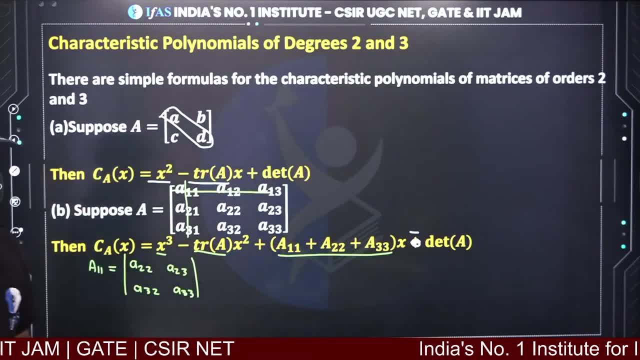 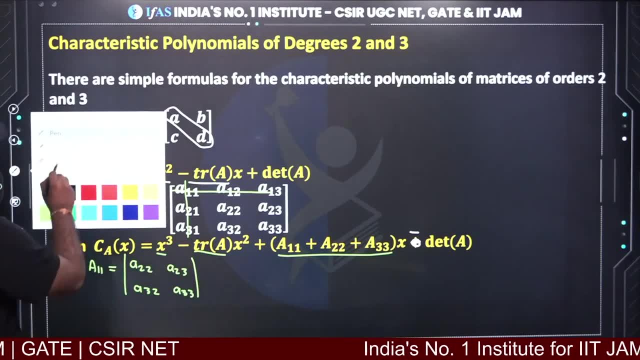 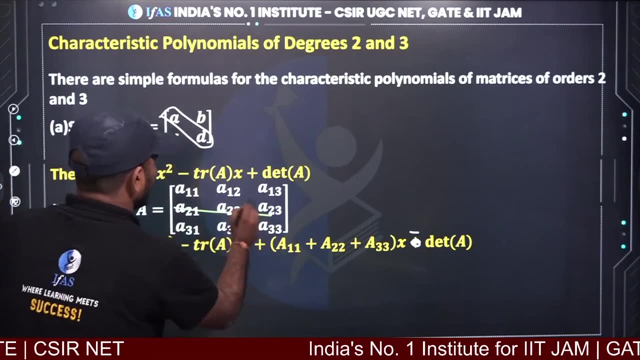 minus plus. this will be minus. this will be minus. this is 3x3, this is shortcut for 3x3. now see here: if someone says to you what will be the value of A22, then what will be the meaning of finding A22? see. delete second row and second column. 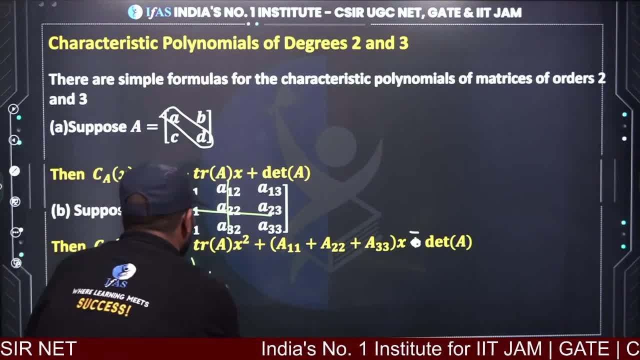 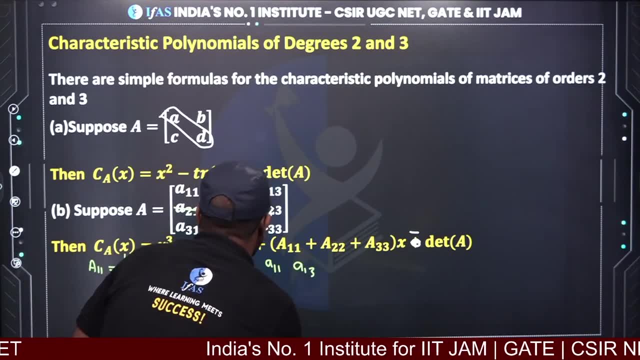 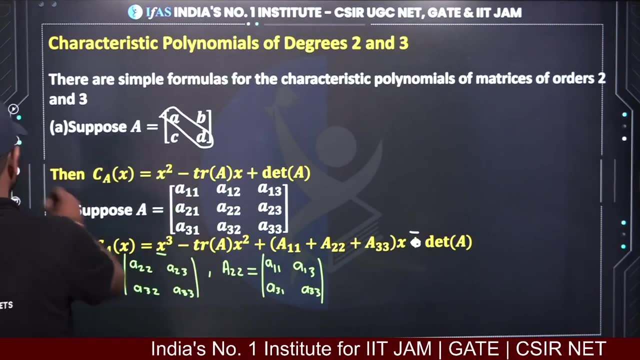 determinant of remaining matrix. so see here: if I do A22, then what will you get? A11, A13, A31, A33. this is the determinant. if you want to find A33, then A33 means remove third row and third column. determinant of the remaining matrix. 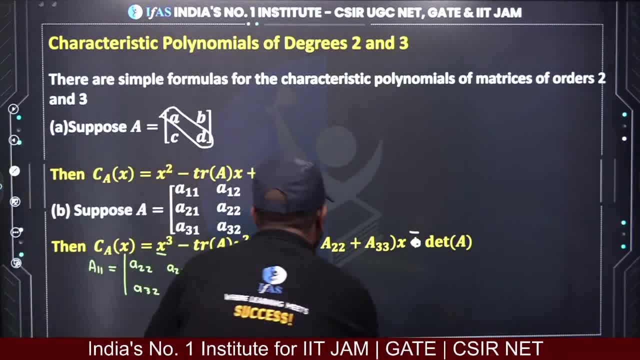 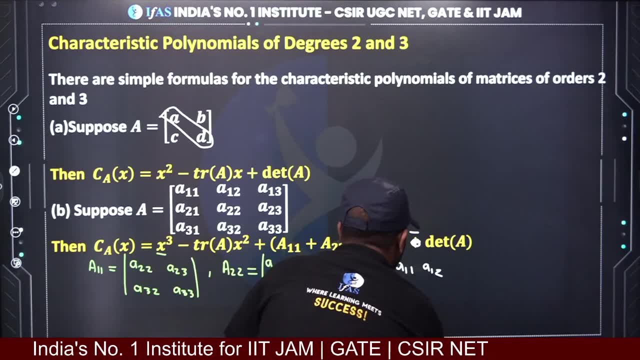 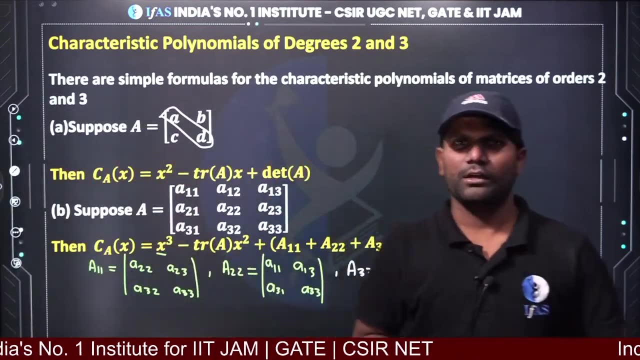 alright. so here what will you get? so A33 is equal to A11, A12, A21, A22, so determinant of this 2x2 matrix. so here you have to keep this in mind if any question comes in the exam. eigenvalue, eigenvector, characteristic polynomial. 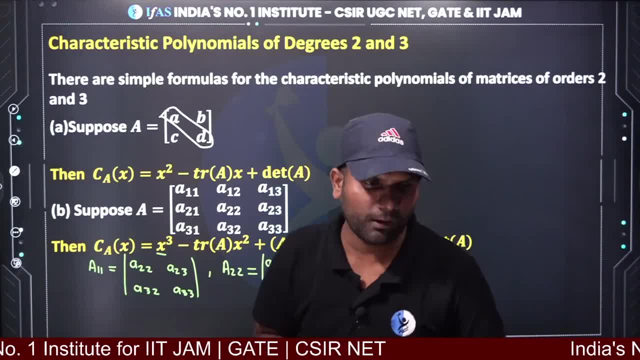 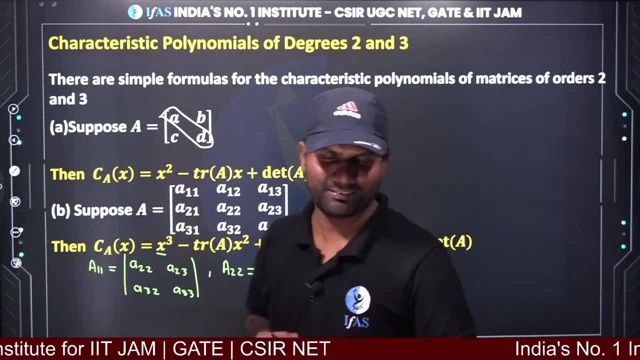 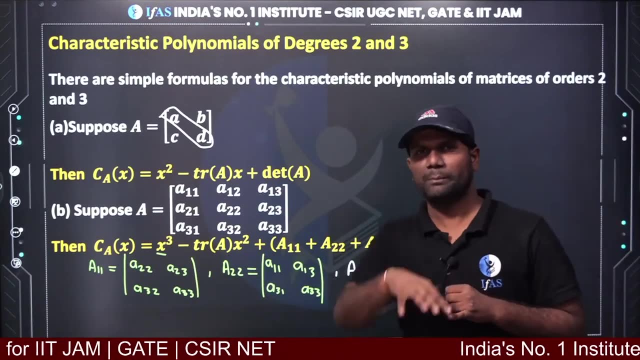 so if any special type matrix, then you will know. if you are used to printing mistake, then it was really printing mistake. I didn't write this, it was typed alright. now see here: if you have any special type matrix, eigenvalue, you can find that special type. otherwise you will use these 2 results. 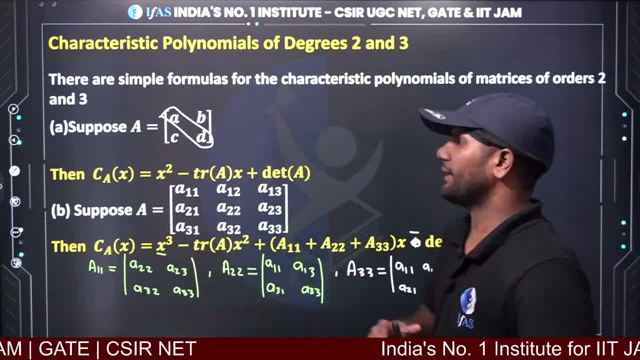 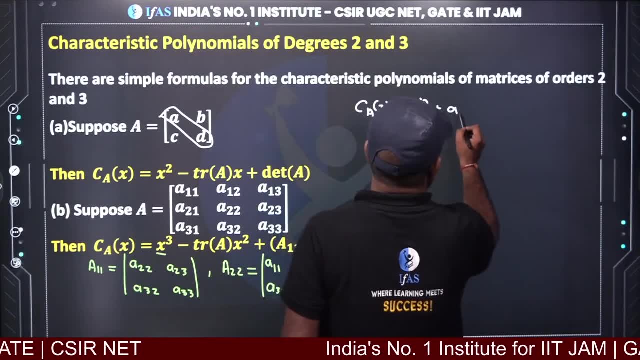 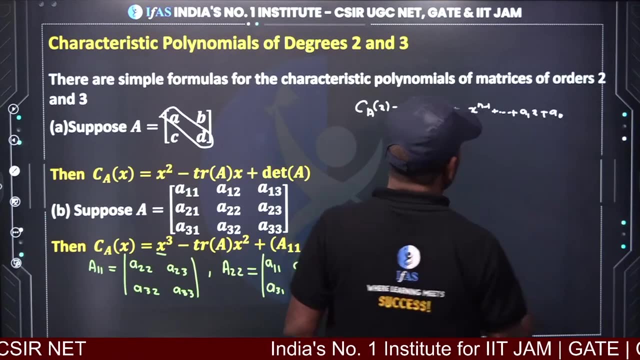 and one special thing you have to keep in mind. suppose any matrix is given to you. suppose A is any matrix. A will be something like this: x raise to n plus an minus 1, x raise to n minus 1, and so on: a1 x plus an. 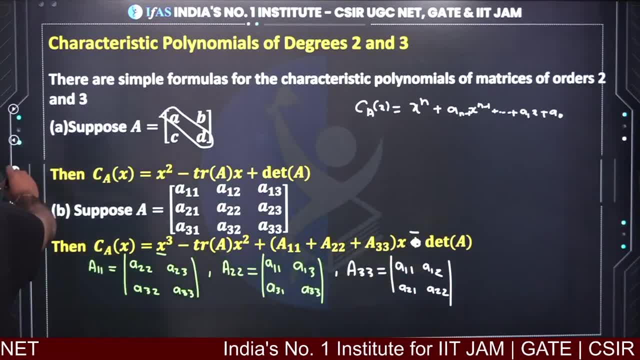 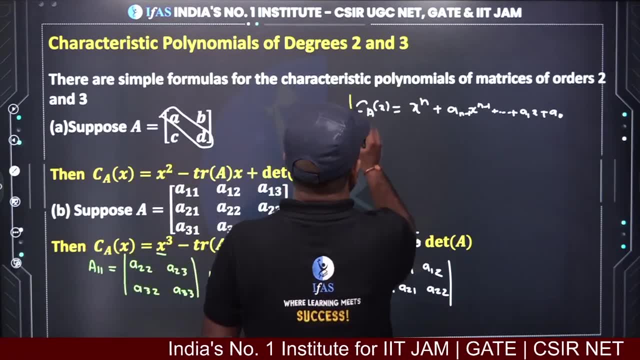 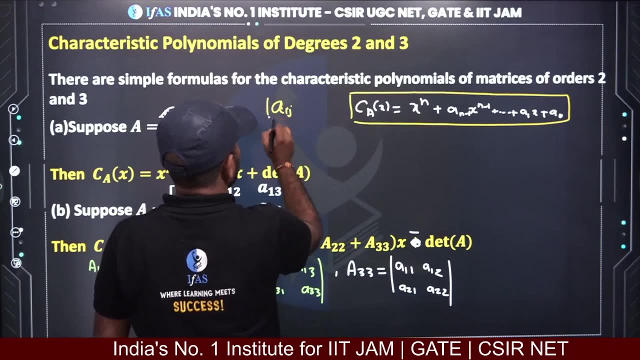 some number here. a1, a2, a3 will be any number, but we will not do it like this. now see here. you have to keep in mind if anyone is given to you matrix of n cross. n suppose someone is given to you whose entries are aiz and its characteristic polynomial is a. 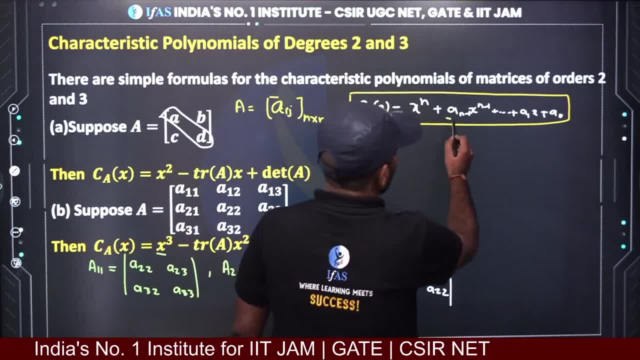 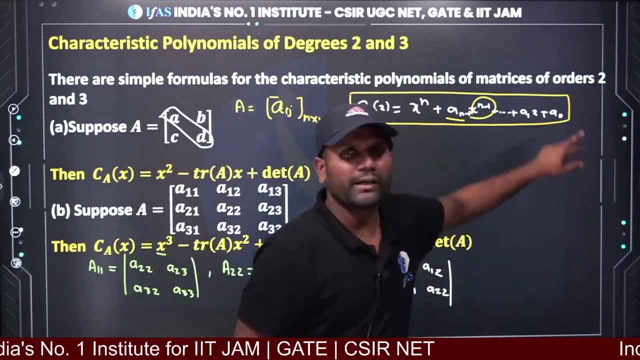 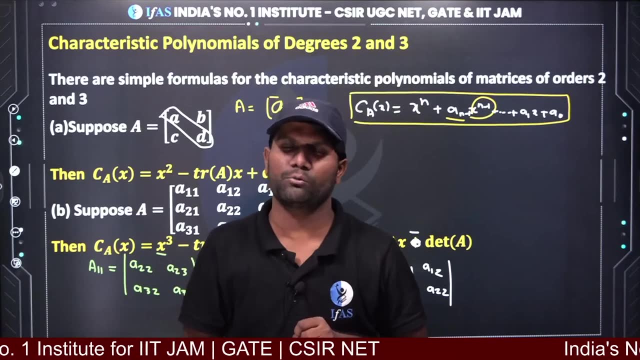 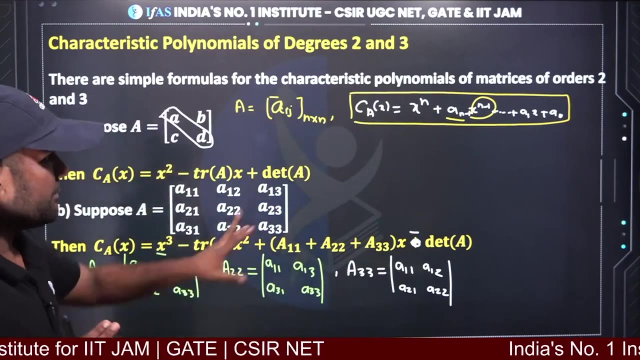 so in that case the coefficient of x raise to n-1 is trace and constant term is determinant, but the sign will be alternate. coefficient of x- raise to n-1 is trace and constant term is determinant. remember this. I told you a lot about this other thing, but the exam is near. 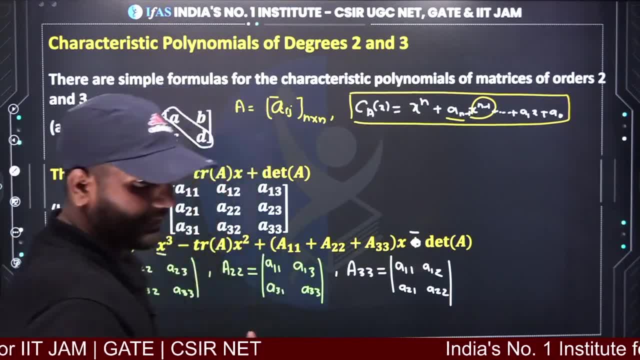 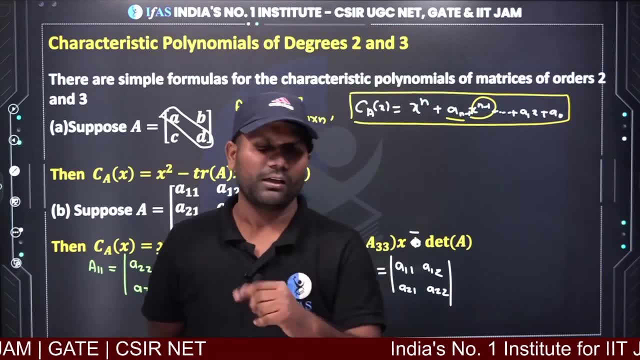 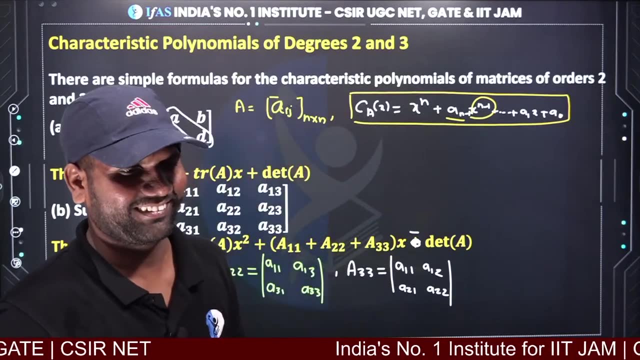 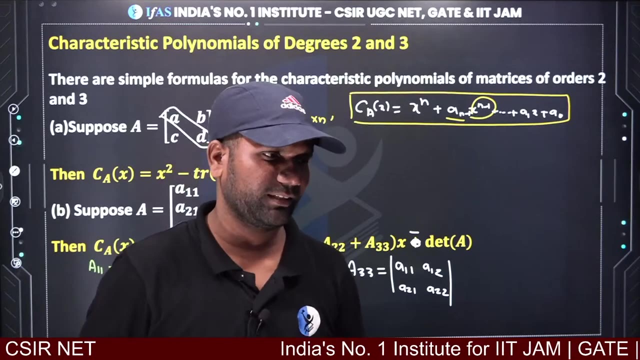 so let me recall it once again: is it clear so far? tell me one thing: everyone is watching. which one is watching? I am not sure that. who is watching 81? who did not like Veenu sarma? explain something to them. yes, know, Absolutely. Vinnu has done it. from now, okay, let's come. 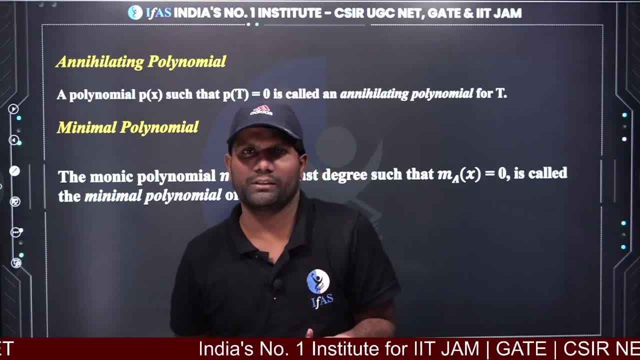 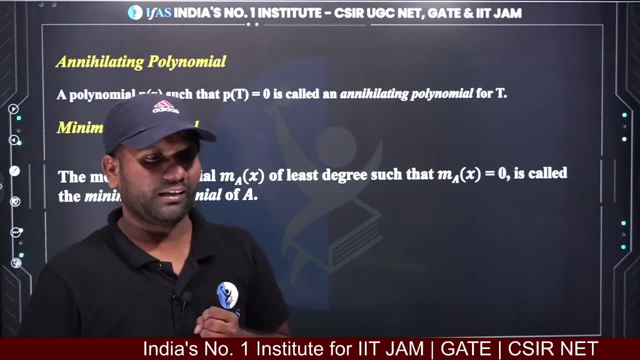 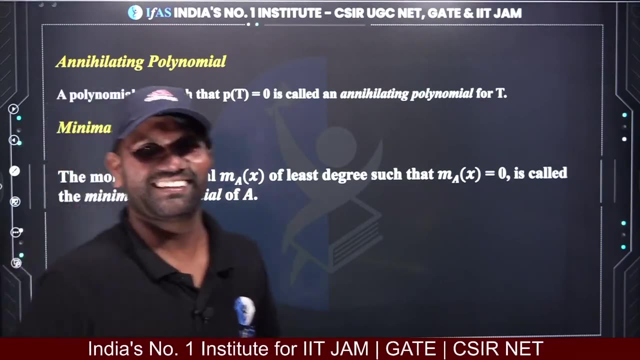 Now, here you know the characteristic polynomial. Yes, now what is the annihilating polynomial. And see how many 85 are watching now, while the likes are 64, some people have not done it yet. Okay, now let's come here, see what is the annihilating polynomial. 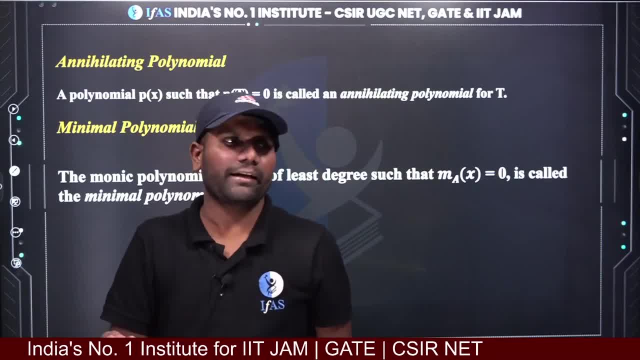 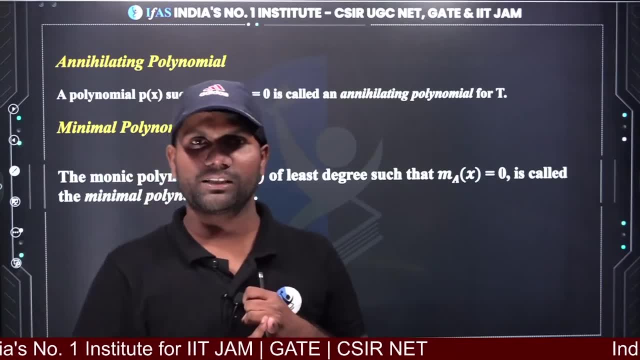 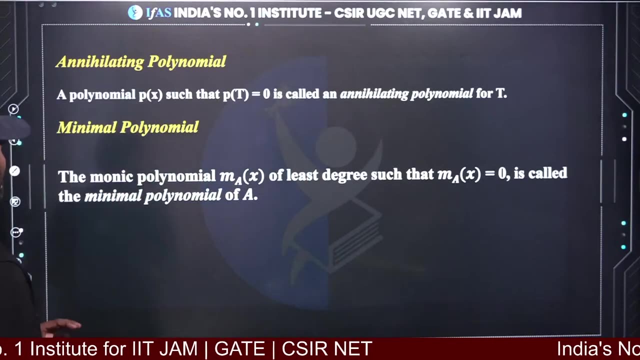 Any polynomial that satisfies the matrix, what is called annihilating polynomial. Now, we will use this annihilating polynomial tomorrow when we will study the diagonalization in minimal polynomial. Some questions like this are asked in the exam: how to solve it? we will see Any polynomial that satisfies the matrix. what is the annihilating polynomial and what is the minimal polynomial? 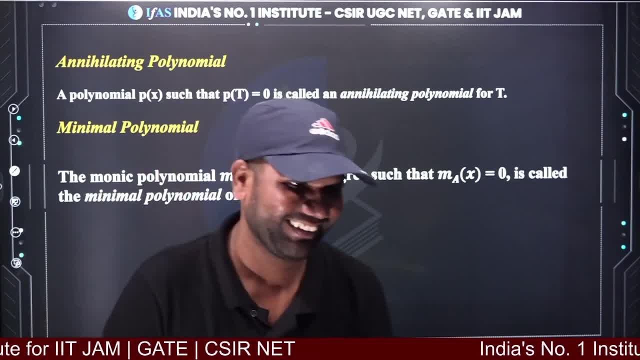 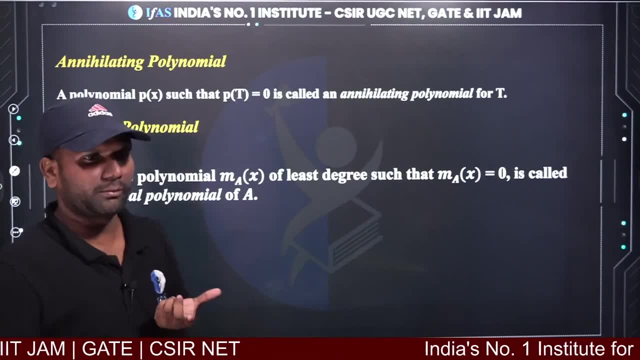 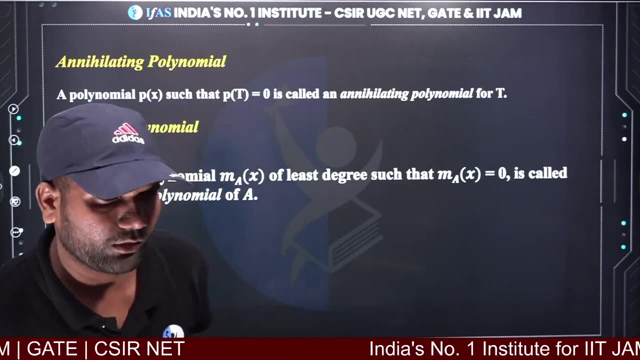 Okay, what is the minimal polynomial? Minimal polynomial is a monic polynomial. what does monic polynomial mean? Such a polynomial, whose leading coefficient means the coefficient of the highest power will be 1 Leading polynomial. good morning, Soni Parveen, Nishi, okay, Nishi has liked it. 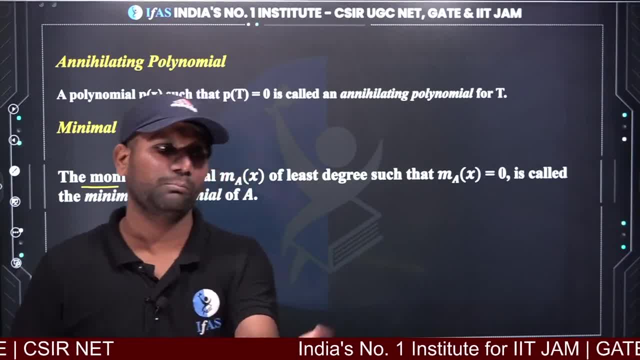 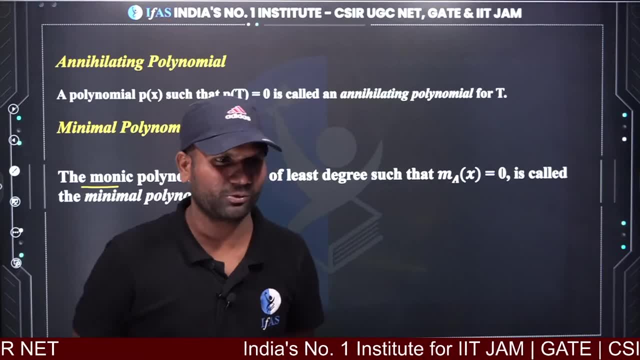 Sheetal is saying: yes, see, Sheetal is saying that such a session is going on. you guys are not liking it. tell me You guys are not liking it. Manohar sir is feeling sad from behind. Yes, the lowest degree, monic polynomial. what does the matrix do to satisfy it? what do we call it? 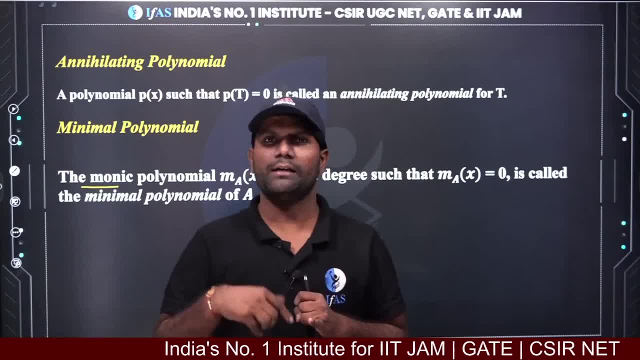 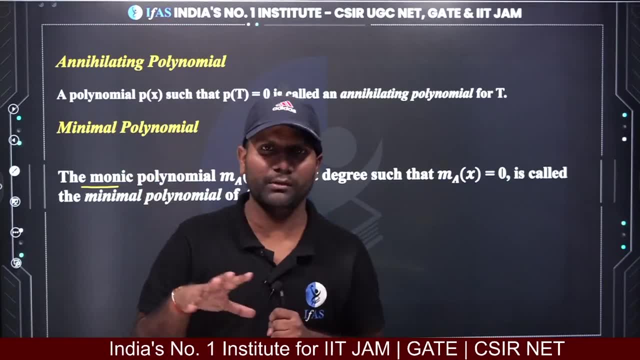 It is called minimal polynomial. Minimal polynomial plays a very important role in diagonalization. What is the very important role we will see tomorrow? I told you about diagonalization. we are going to see you tomorrow, Okay, so characteristic polynomial, minimal polynomial, annihilating polynomial and some important results. 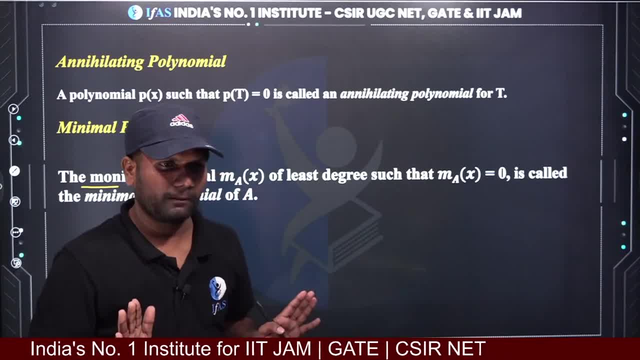 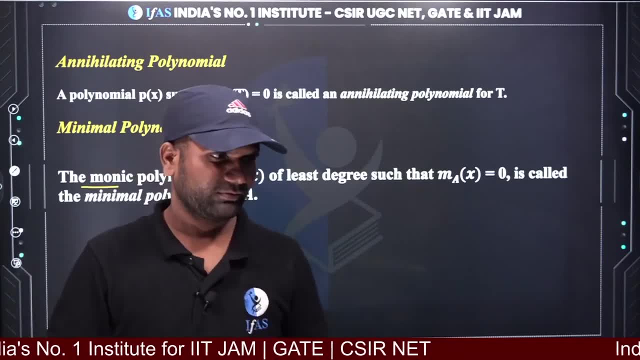 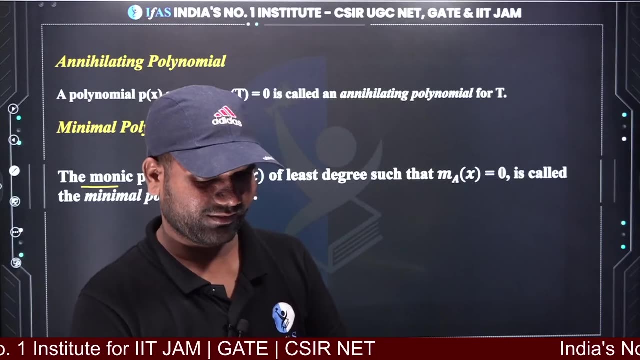 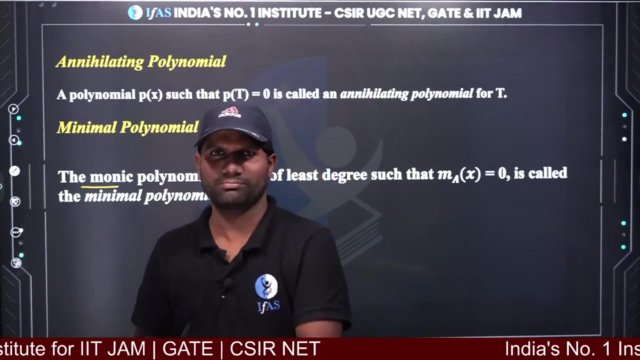 I have told you guys. I hope it is clear till here. Okay, good morning everyone who are joining now. So if you guys did not like it, then like it. Okay, let's go ahead. Thank you, Rinku Yadav. Abhishek must be watching on mobile from somewhere. he is not here. he has gone home. 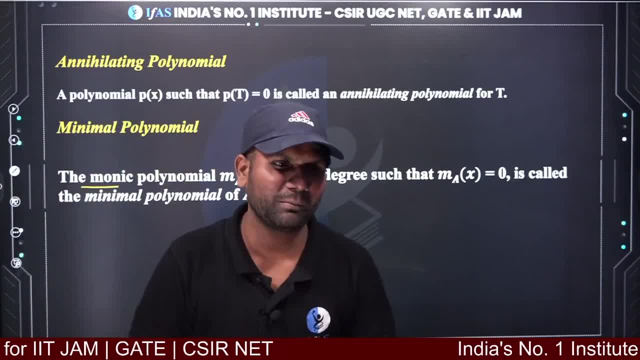 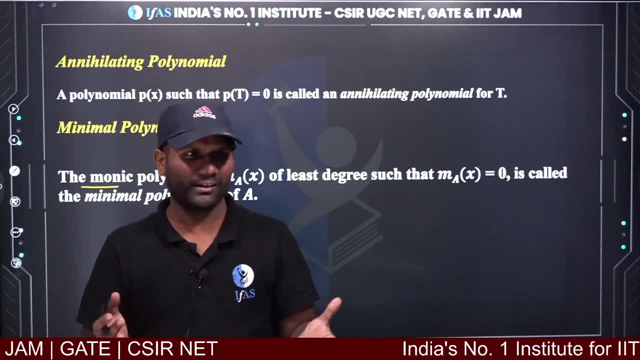 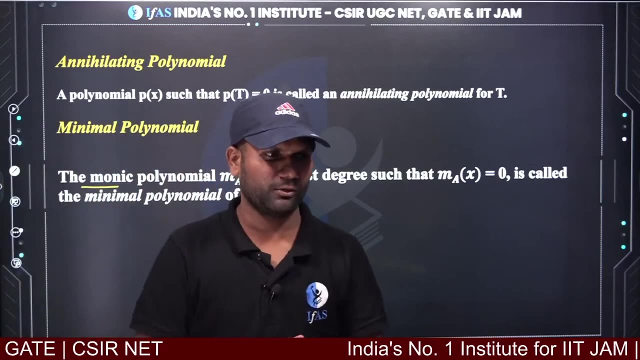 He was going sick, so he went home. Come on, it's already 92, So do 100 once you guys. Minimal product of: yes, absolutely, we will do NKG classes. Okay, absolutely, Now let's come. I think the question must have come now. 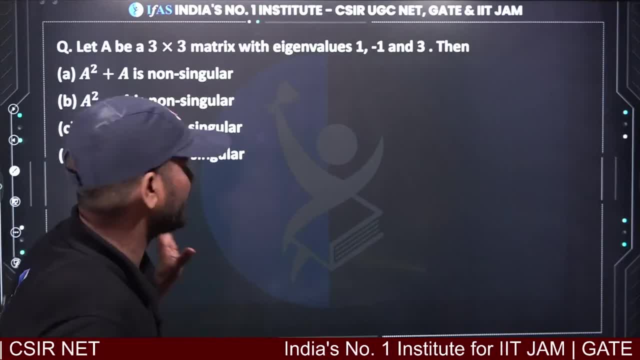 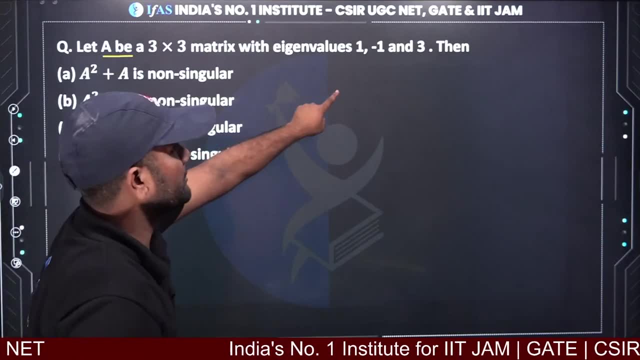 Now see here: this type of question was asked in the exam. this time also, It is possible that it will be asked again. See what is here. Lat ABR 3 cross 3 matrix whose eigenvalue is 1, minus 1, 3. 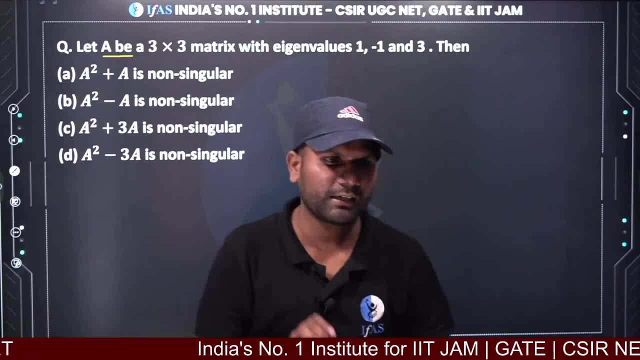 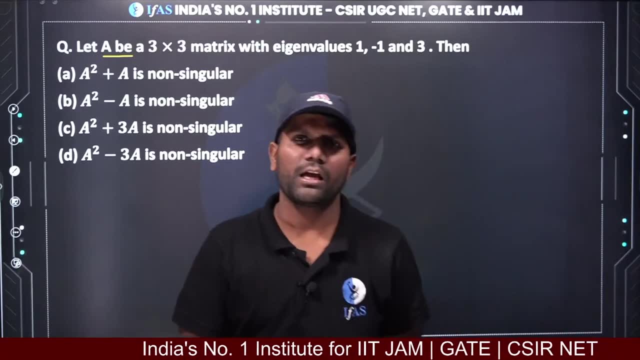 So here these four options are there. Which of these will be correct? What do you think? So see, what did we ask? Singular and non-singular. When do we call any matrix singular If the determinant of that matrix is not equal to 0? 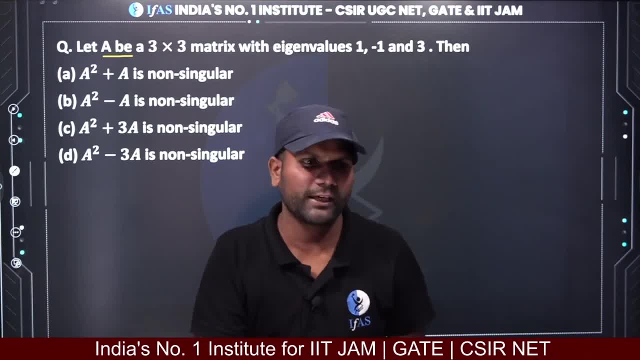 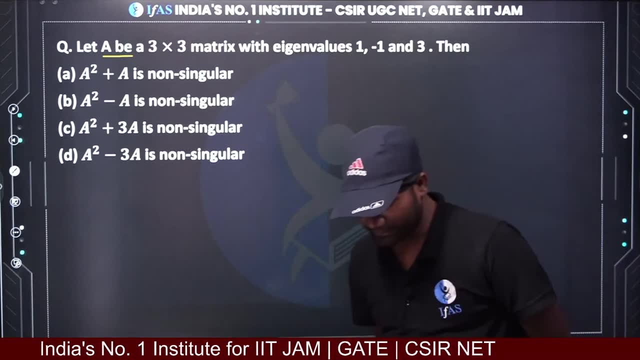 So what is called non-singular? If the determinant is 0, then it becomes singular, right, Right or not, Abhishek? I think you have not shared, otherwise there would have been 100 today. Okay, come on, tell me. 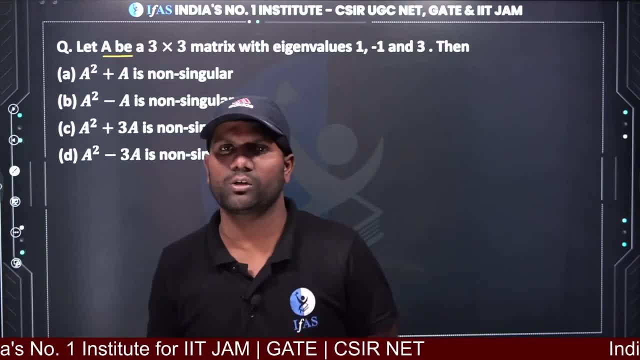 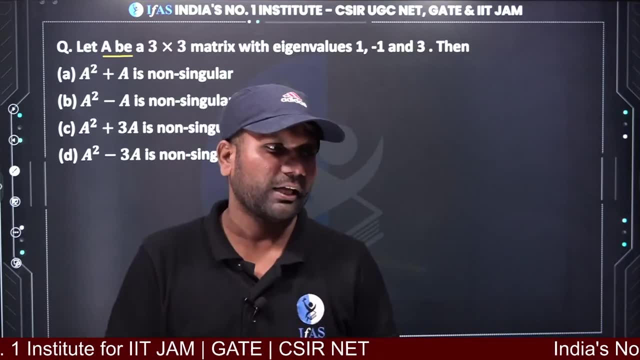 And what we will do in tomorrow's session: Diagonalization, JC form, quadratic form, inner product. From there, 100% questions will be made. Questions will also be made from here. But that topic many people have doubts. Your revision will be completely linear. 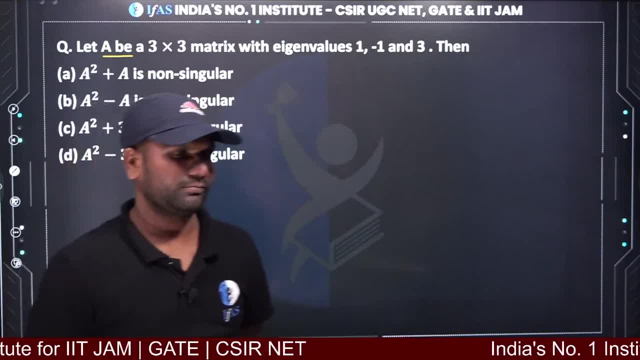 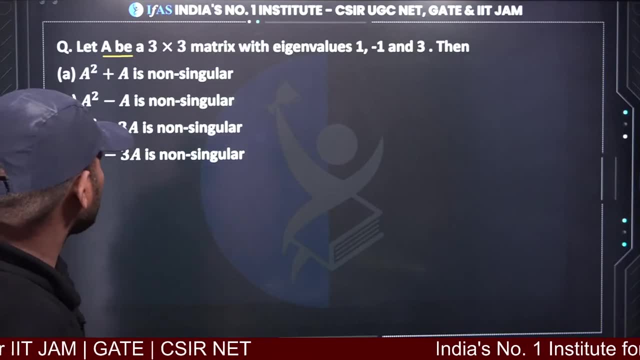 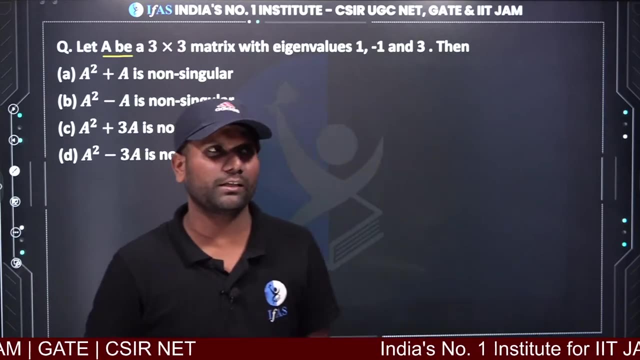 Good evening, Alpha A. Okay, Okay, tell me What will be the answer to this. Solve it. this session is for you guys, right? You guys are not like once Before going to the exam, you are doing rehearsal once Or going to play warm-up cricket or some match. 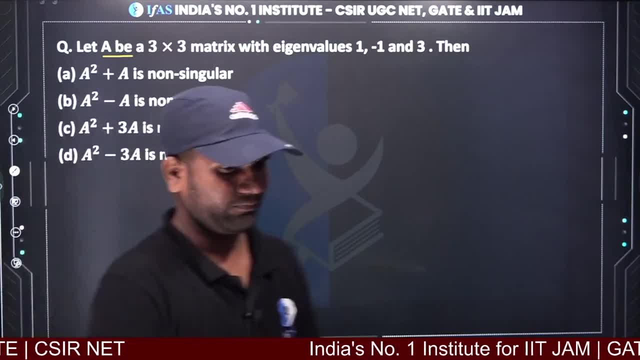 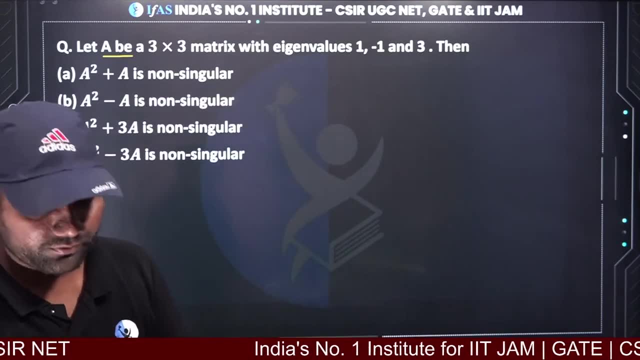 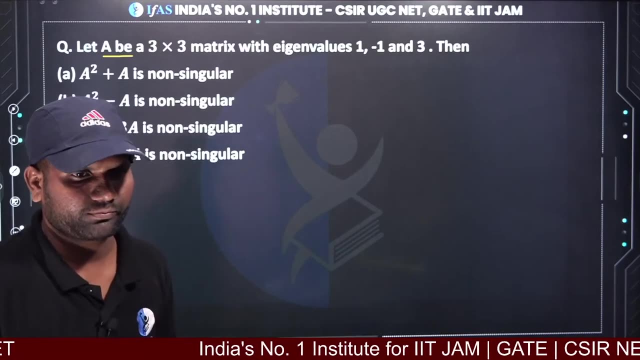 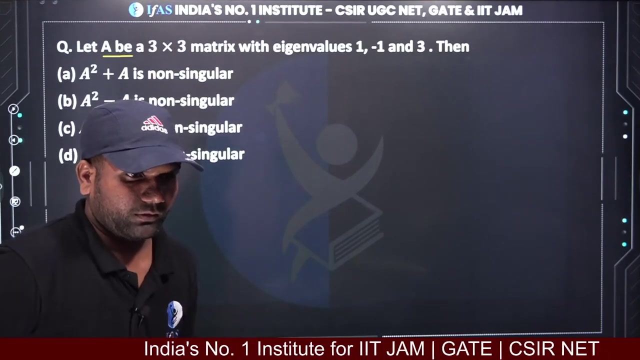 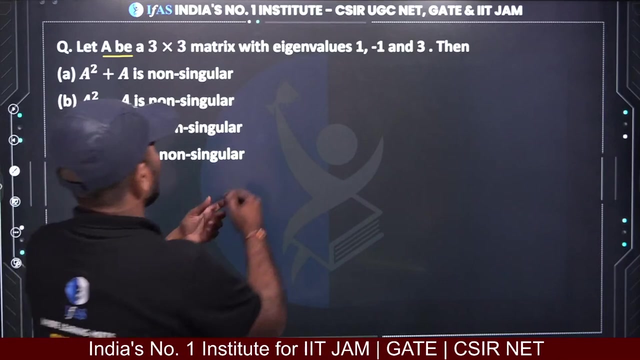 See once you guys tell me what will happen. Come on, tell me Magic honey, hello, how are you? Almost everyone is saying C answer. They are saying C okay. So look at the point of view. What is the eigenvalue of A? 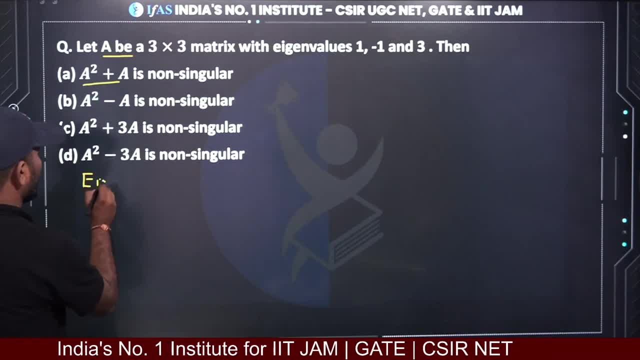 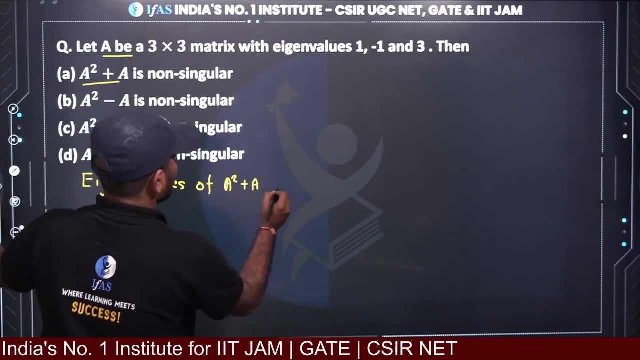 What will be its eigenvalue? So here, if you talk about eigenvalues of Eigenvalues of A square plus A, What will be the eigenvalues of this? See the eigenvalues of this. Now, if you keep 1 from here, then you will do 1 square plus 1. 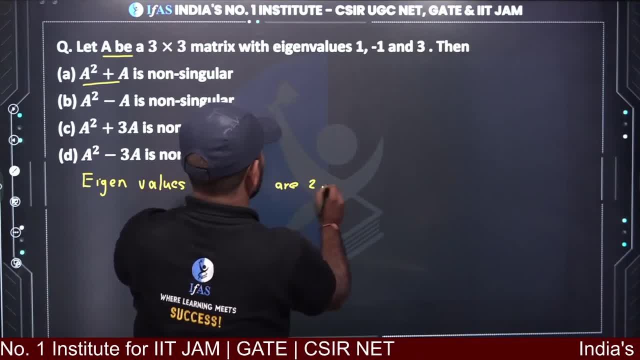 It will be 2, you will do the square of minus 1. 1 square will be zero. And what will happen here? 3 square. 3 square means If you do 9 plus 3, then how much will you get? You will get 12. 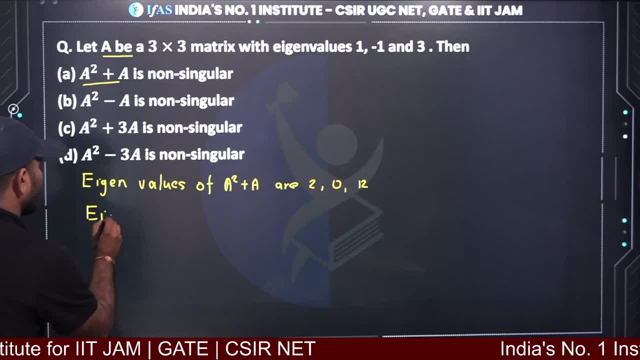 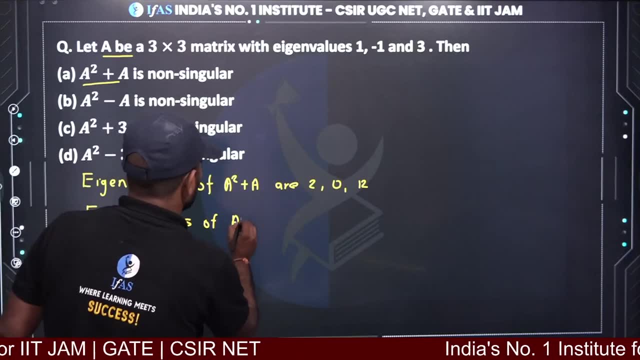 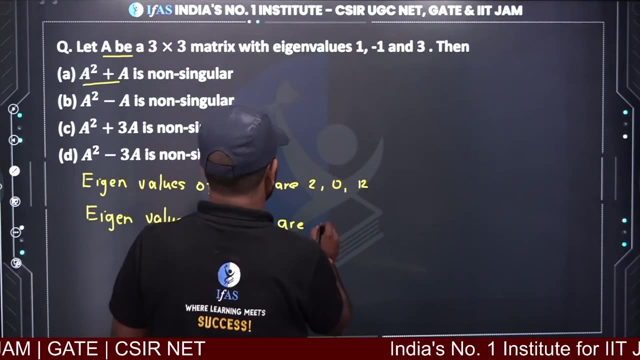 You will get the eigenvalues of this If I talk here Eigenvalues of A square minus A. So what will be the eigenvalues of A square minus A? You will get the eigenvalues of A square minus A Keep 1. So if you do 1 minus 1, it will be 0. 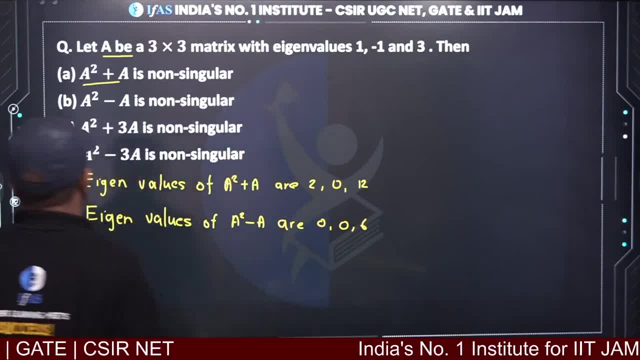 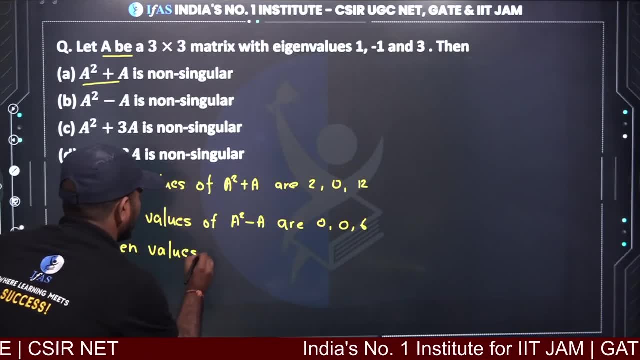 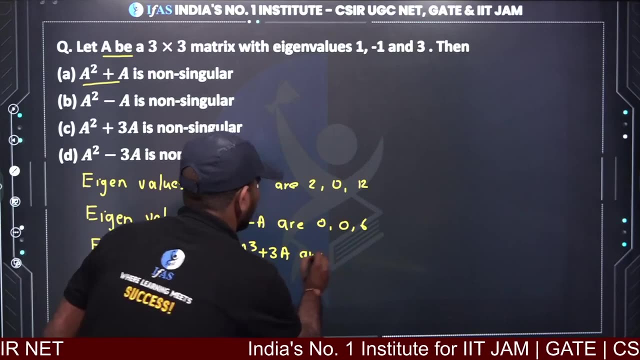 This will also be 0. If you do 9 minus 3, it will be 6. Okay, Now, if I talk about eigenvalues of Eigenvalues, Eigenvalues of Eigenvalues of A square Plus 3A. So what will be the eigenvalues of A square plus 3A? 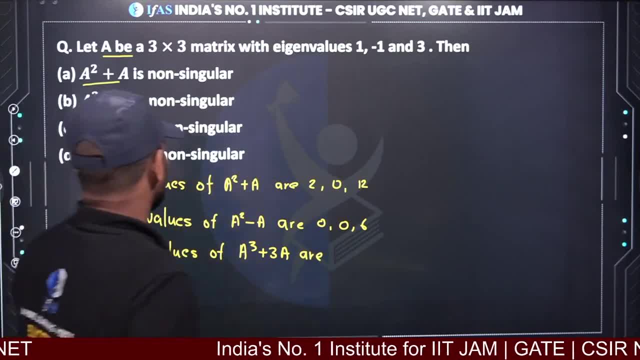 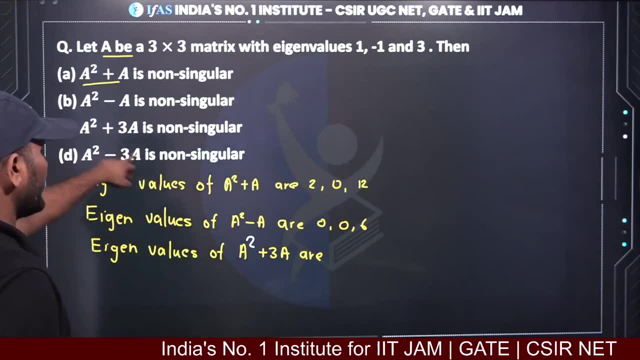 So what will be the eigenvalues of A square plus 3A? So what is A square of this? I have written A cube here, wait. So if you find the eigenvalues here, So what is the eigenvalue? Eigenvalue of A square. 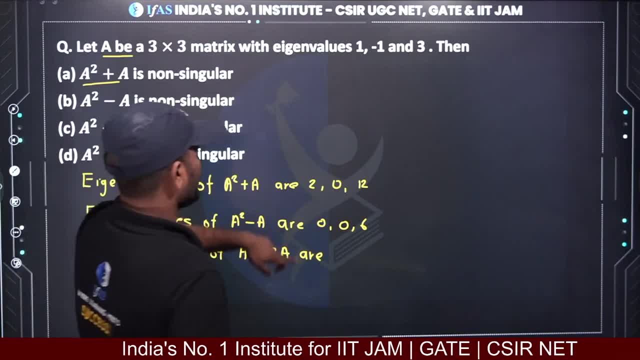 See here: now keep 3, here 3 square will be 9. Means if you keep 1, then 1 square will be 1 and 3 It will be 4. If you do 1 minus 3, it will be minus 2. 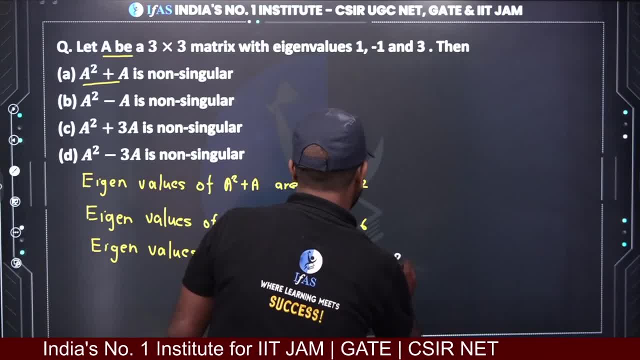 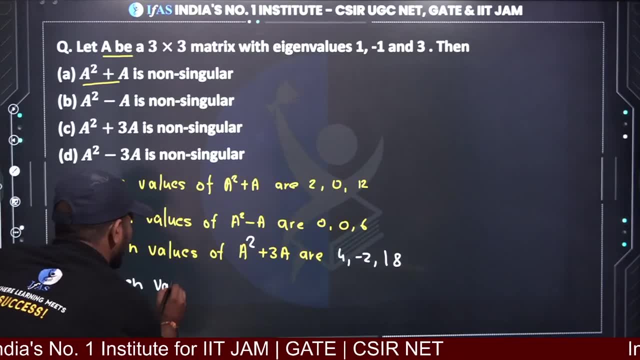 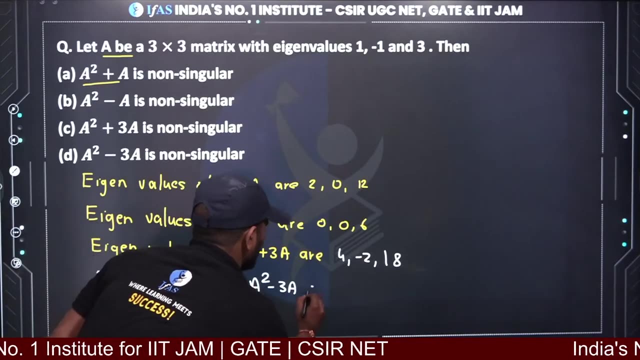 And here, if you do 9 plus 9, it will be 18, Okay, And here, if you see the eigenvalues of Eigenvalues of Eigenvalues Of A square minus A square minus 3A, So if you talk about the eigenvalues of this, 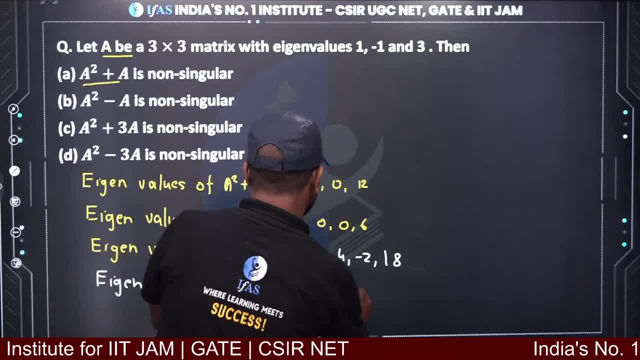 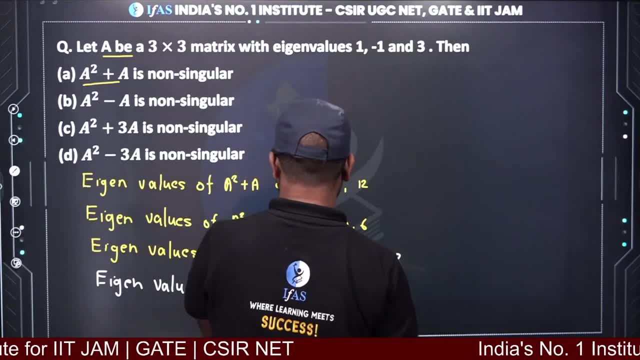 If you do 1 square minus 3, So it will be minus 2, And 1 square minus minus 1 plus 4 will be 4. And here what will you get? A square will be 9. If you do minus 9, then it will be 0. 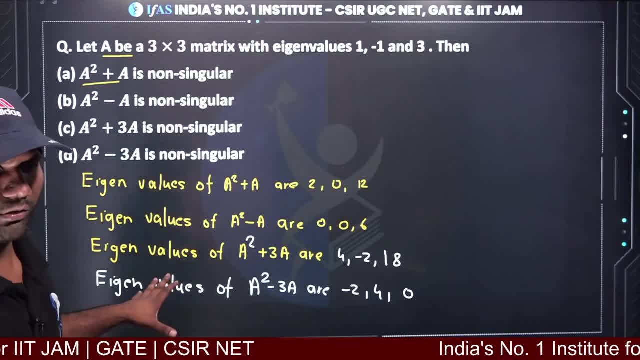 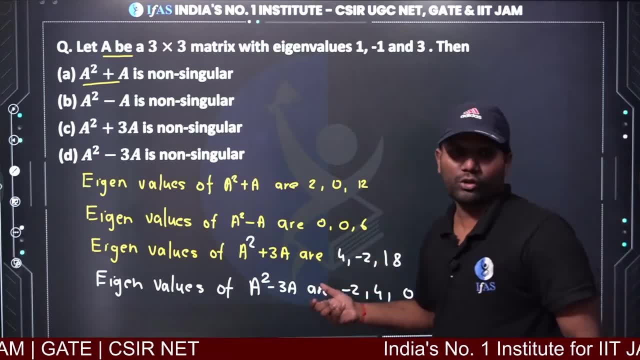 So from here you can see clearly. So we were asked which of these will be non-singular. Non-singular will only be found where the eigenvalues are not 0. So where do you see non-zero eigenvalues? If you see, then you see non-zero eigenvalues only in the third case. 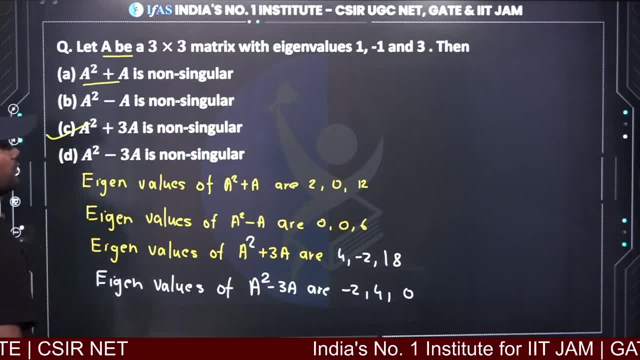 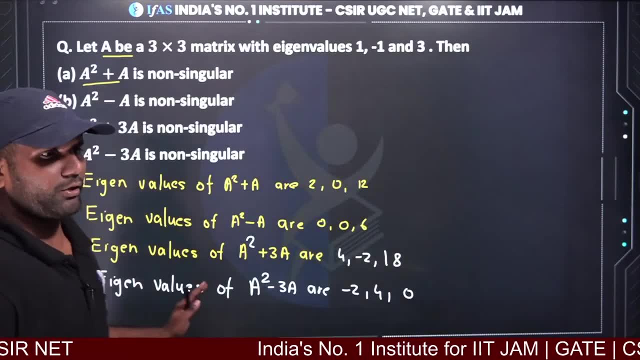 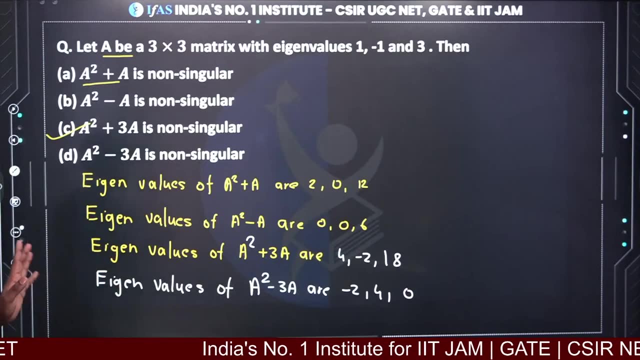 It means that option C will be what? Option C is non-singular. Is everyone clear? See once, Is everyone clear? Is everyone clear? Okay, See, everyone is clear. till here, Go ahead. I hope this question will be clear to you. Now we move on to the next question. 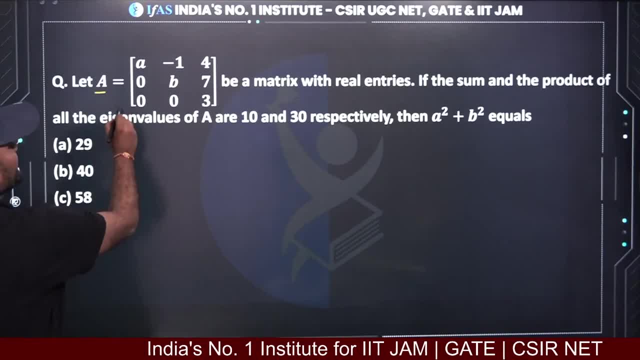 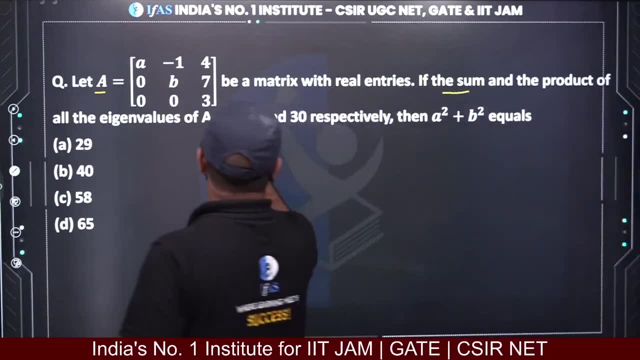 Now see here: one question has been given to us. Let A is this matrix Be a matrix with real entries? And what has been given to us? If sum and the product of eigenvalues of A are, A are 10 and 30, We have been given the sum of an eigenvalue. 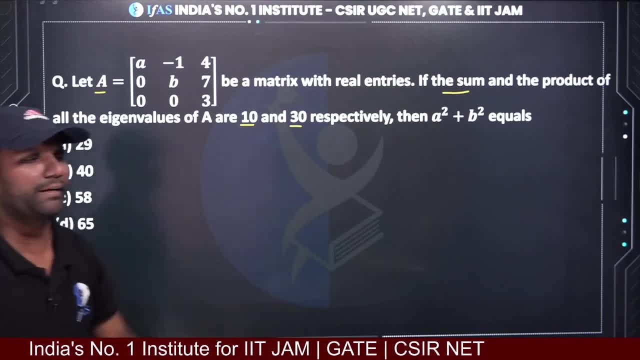 Is 10, If sum and the product of eigenvalues of A are 10 and 30, Then you have to tell what will be A2 plus B2. Come on, quickly tell Absolutely. So 100 has been given, finally, But like is less till now. Okay, come on. 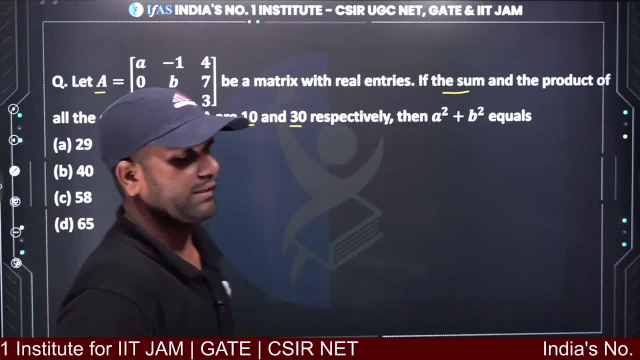 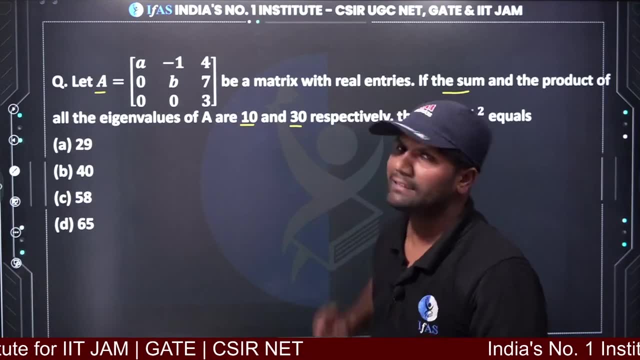 Tell what will happen. Everyone see and tell what will happen here. Now see A3 cross 3 matrix is given. Now the simple thing is that there is such a matrix. There is an upper triangular matrix If A is the upper triangular matrix, So you can easily find it. 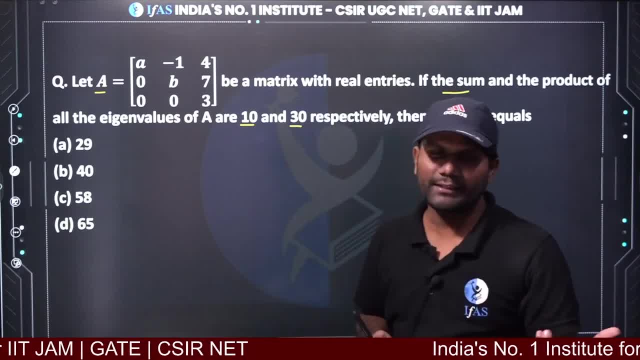 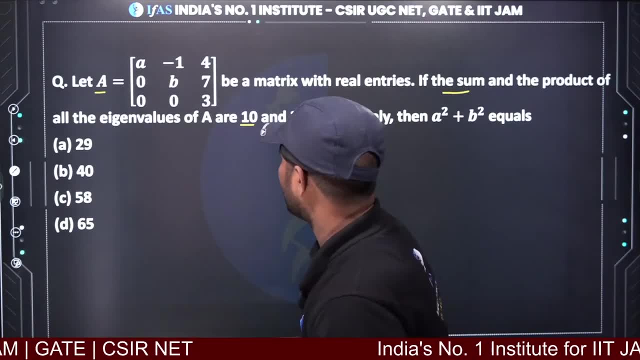 You can easily find its eigenvalue, Isn't it? You can find the eigenvalue very easily. So if you can find the eigenvalue very easily, Then tell me what will happen. Parul is saying A- Very good Parul. Kailash is also saying A. 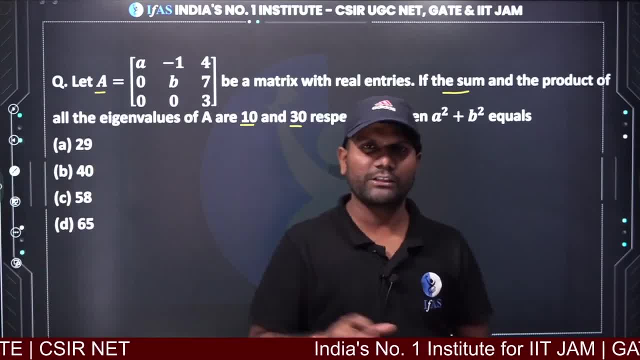 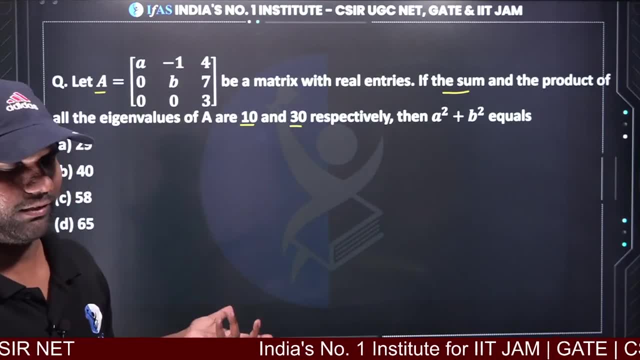 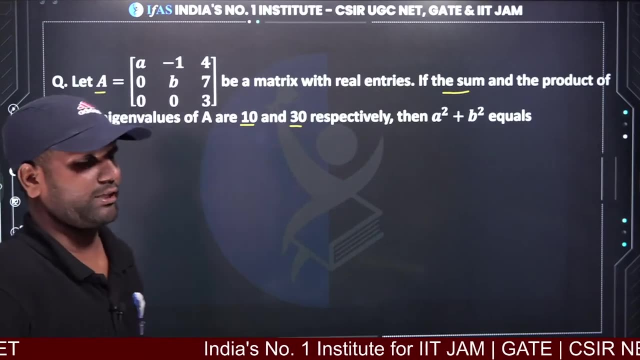 Tell the rest of the students what will happen. See, such questions can be asked in the exam. A good question is also A. It will be asked for 3 months. It can be asked. Okay, Sabina A Ramshin A. Absolutely right, Very good, Everyone has given the correct answer. 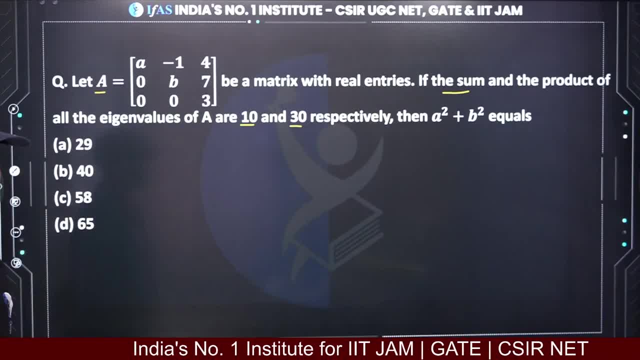 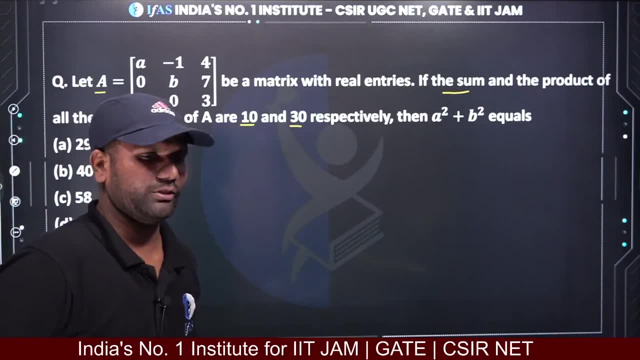 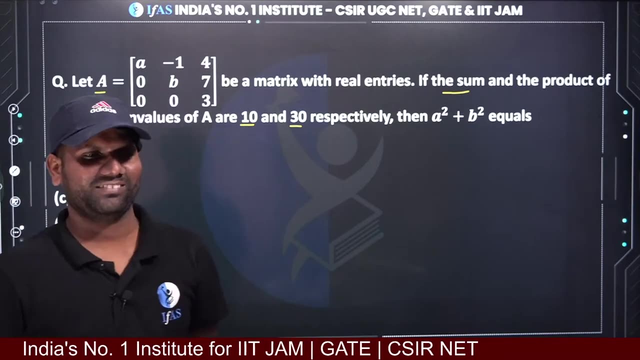 Absolutely right. Gunjan is saying A Robin, A Indian work, A Sabina is correct. Absolutely right, Dipanshi Amrind. Everyone is saying A 29. Absolutely. Hinduja, Nishi, All people, Hari Om. Yes, absolutely, Parul has done it 3 times. Okay, okay. 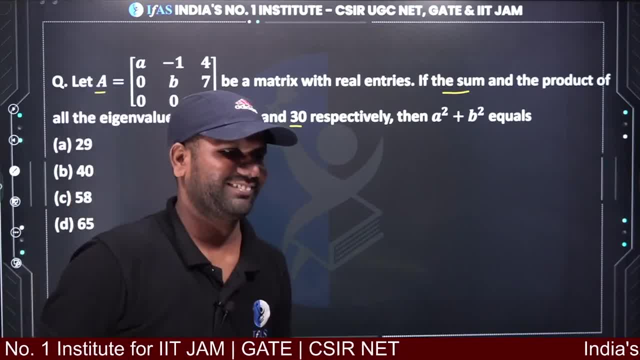 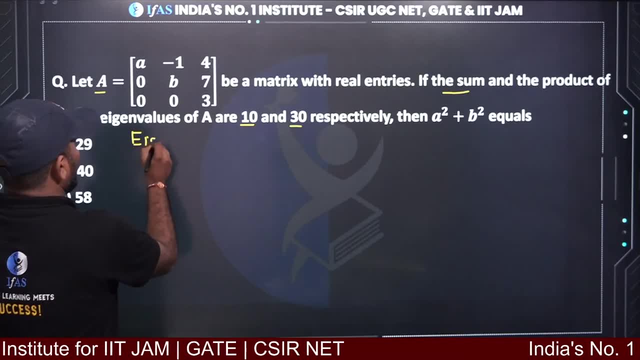 Good that you did it 3 times. If you had done it 2 times then it would have been wrong. Now see here Can you see the eigenvalues of A. So eigenvalues, Eigenvalues Of A are. So what are the eigenvalues of A? 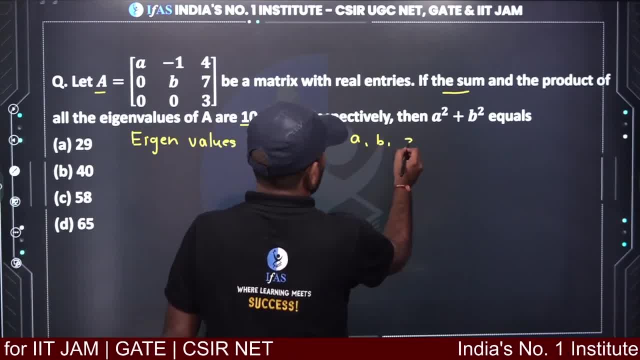 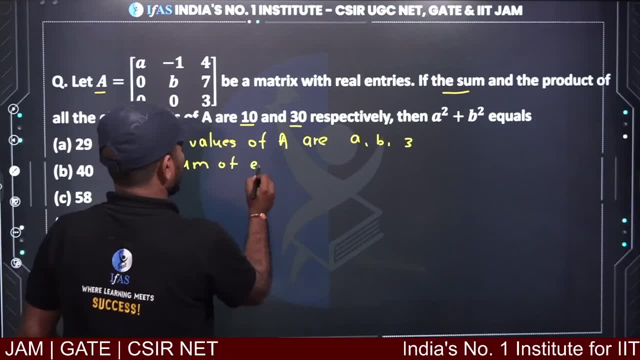 So eigenvalues of A are A, B, 3, But we know that sum of eigenvalues is same as the trace. If you take the sum of eigenvalues, Then what is the sum of eigenvalues? Sum of Eigenvalues If you add the eigenvalues. 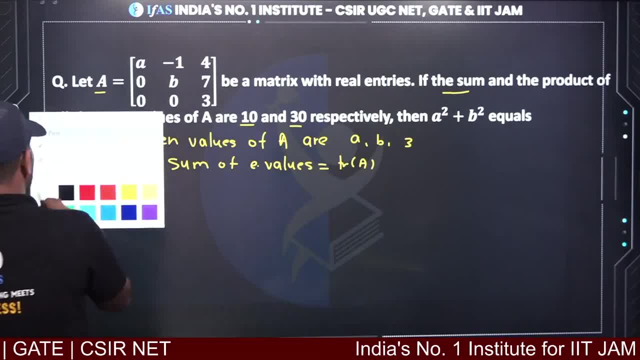 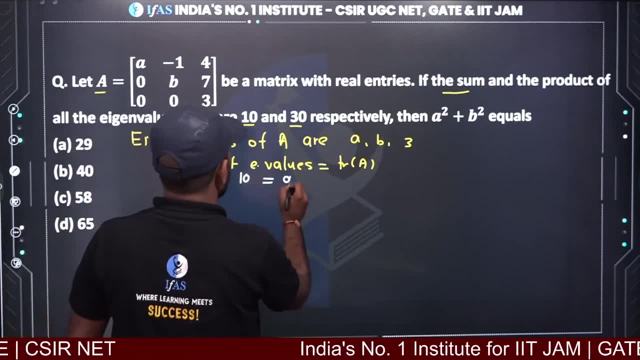 Then what do you get? Trace of the matrix. Now see here: What is the sum of eigenvalues given to us? The sum of eigenvalues given to you is 10. 10 is equal to trace. What is trace? If you see trace A plus B plus 3. 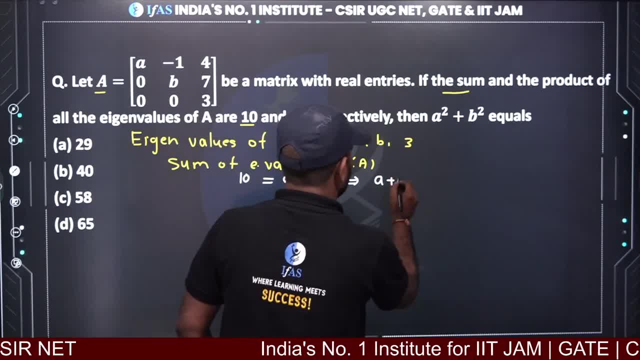 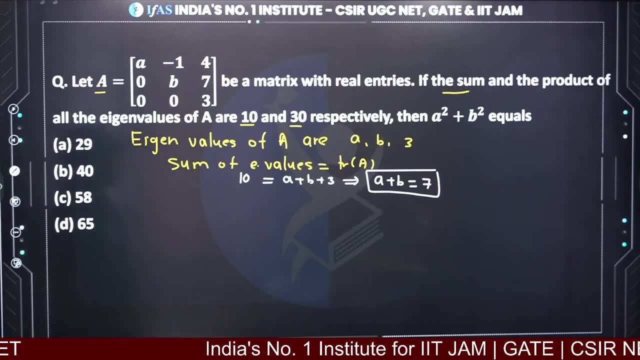 So from here you can tell What did you get. A plus B is equal to 7. So you have a condition here: A plus B is equal to 7. Okay, A plus B is equal to 7. Okay, Now, if we come here, This is done. 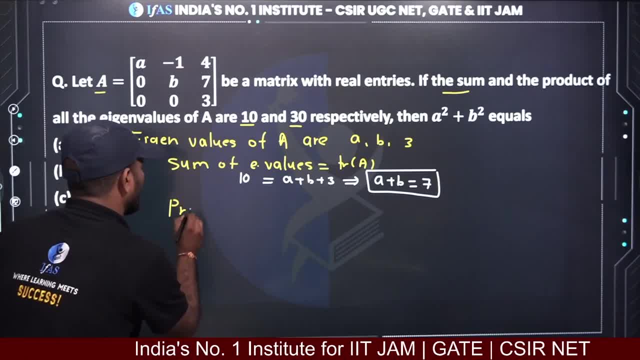 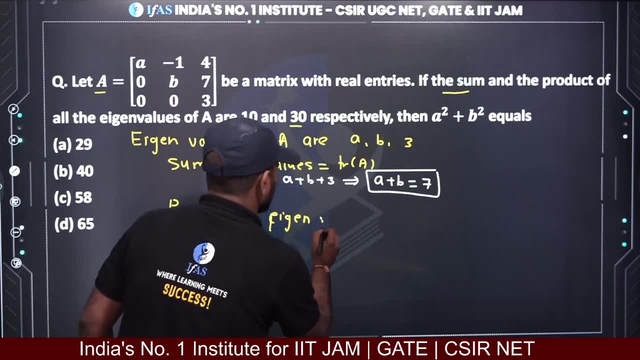 This is our eigenvalue, Sum of eigenvalues. And one more information is given to us: What is given Product of eigenvalues? What is the product of eigenvalues given? Product of eigenvalues. If you see here, The product of eigenvalues is same as Determinant of A. 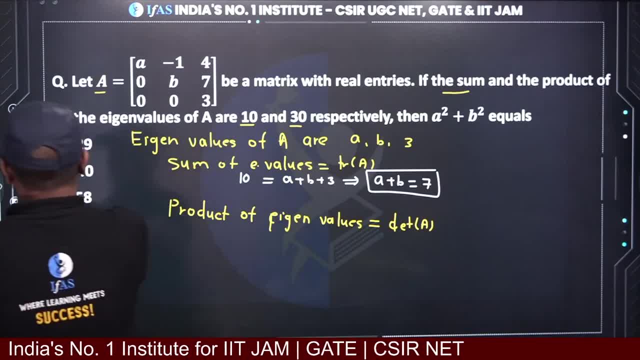 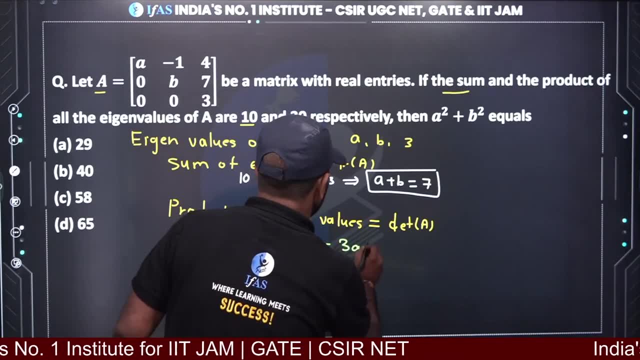 Okay, But what is the determinant given to you? 30 is given. Determinant 30 is given. So this is equal to 30 is equal to What will happen. Product of eigenvalues 3. A into B will happen. So from here you get to know. 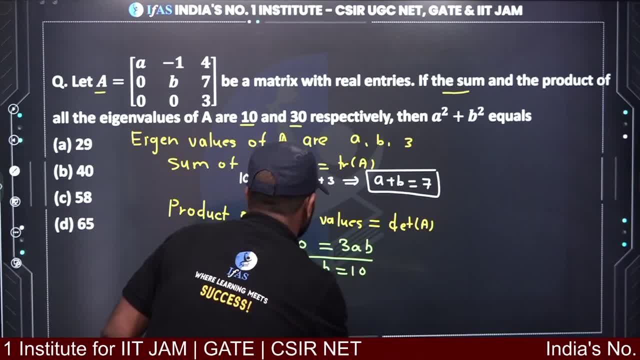 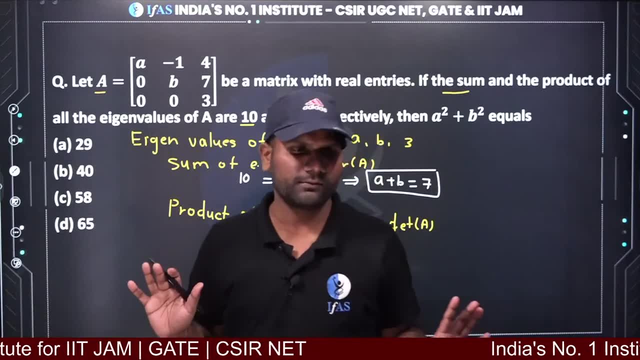 What is the value of AB? What is the value of AB 10? Okay. What is the value of A plus B 7? What is the value of AB 10? Okay, Till here. Remember Mungra and Chiku. You have seen after many days. 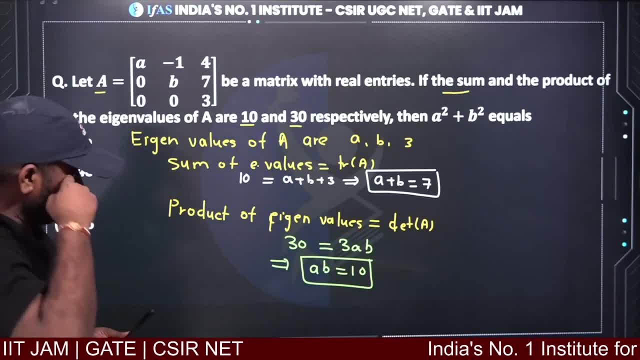 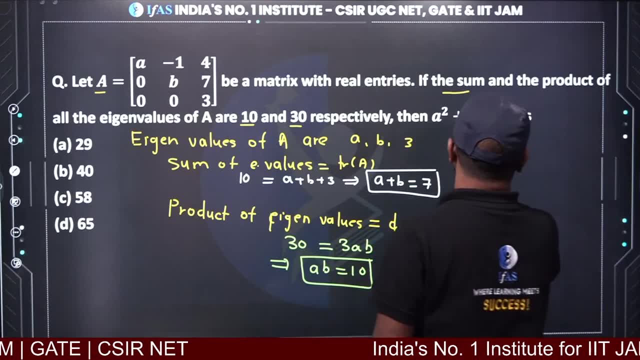 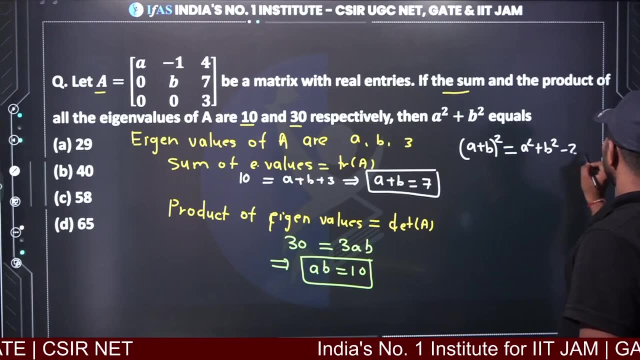 Okay, Now let's come here, What we have to find Now we want to find out Value of A square plus B square. If we want to find A square, B square, What do we know? A plus B, all square is same as A square plus B square minus 2AB. 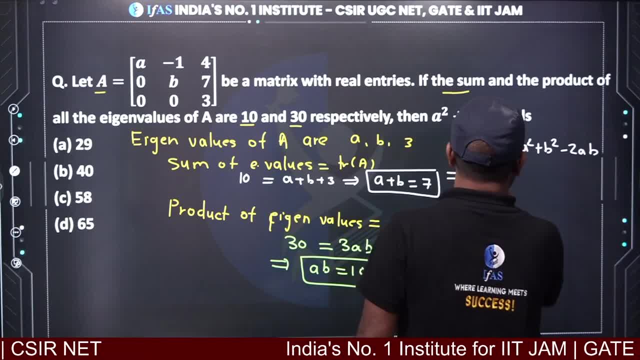 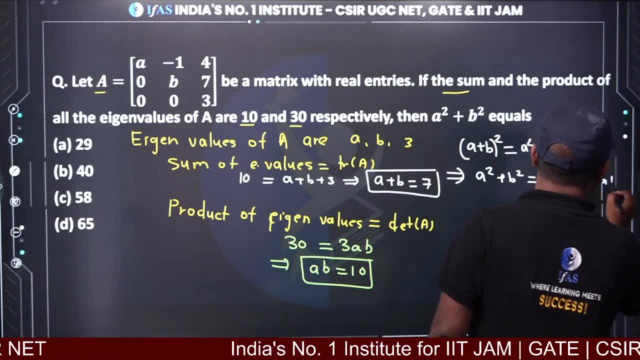 So we can write it like this. We can write it as A square plus B square is equal to A plus B. whole square minus 2AB. It will be plus 2AB, Shifted to this side. Now what is the value of A plus B? 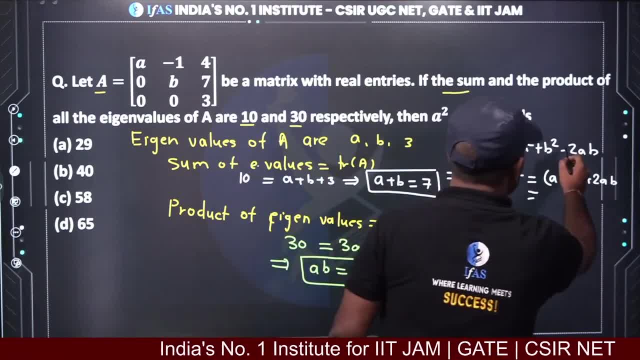 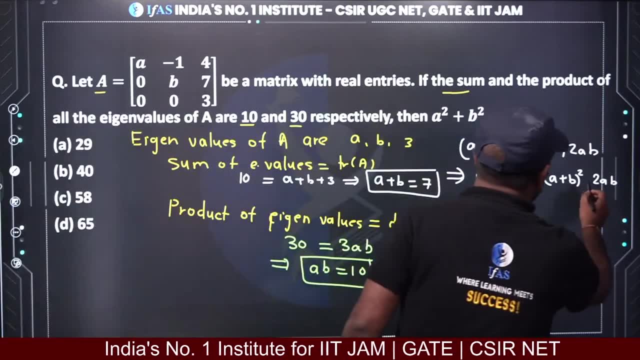 What is the value of A plus B? Okay, one minute. Here is plus, so it will be minus. It will be minus here. Just wait, It will be minus here, Okay, Minus. So A plus B square means 7 square. What will be 7 square? 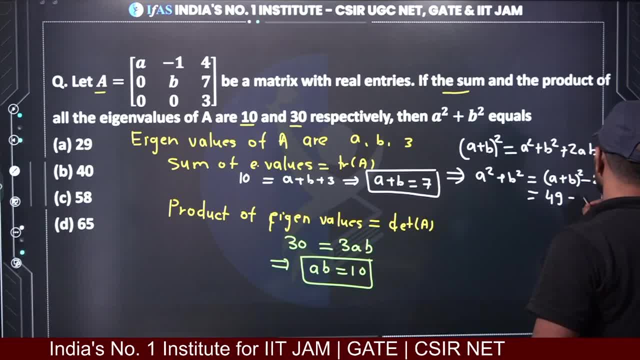 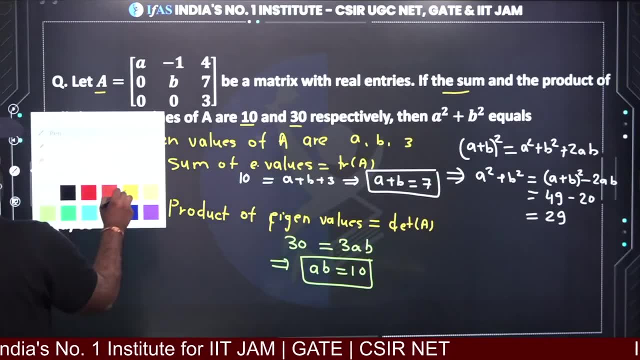 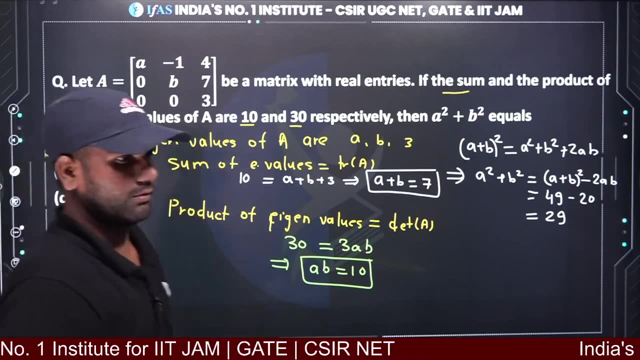 49 minus 2 times AB. 2 times AB means 20, So this is equal to 29. So what will be the correct answer for this question? So option A is correct for this question. Is everyone clear? See it? Okay, Come on, very good. 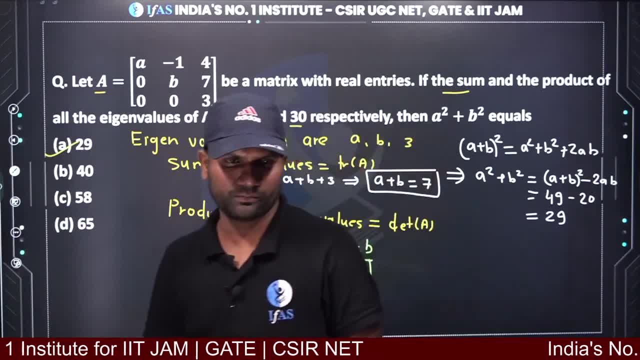 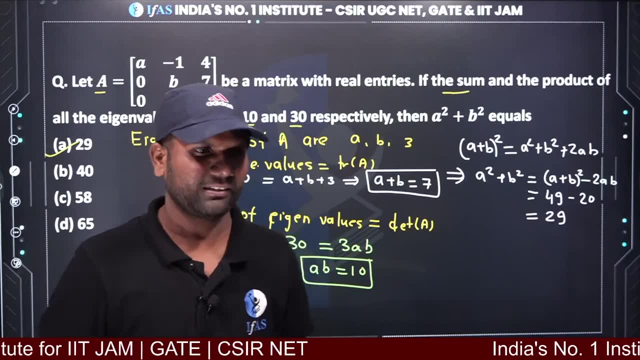 What is one? Okay, Come on. I hope everyone will be clear till here. See, Mano sir is here. I had told you Mano sir is watching from behind. He is here. See you guys Now see this. Okay, Come on, Sir. IFS's branches are available in Jabalpur. 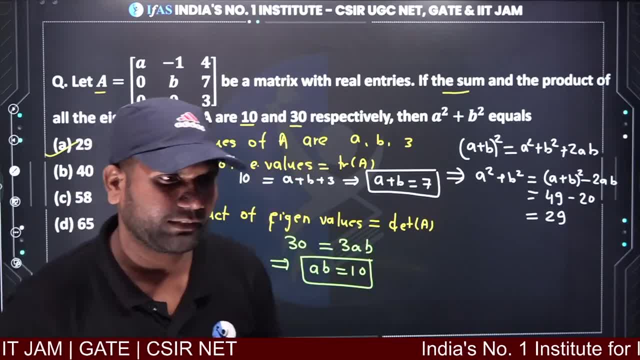 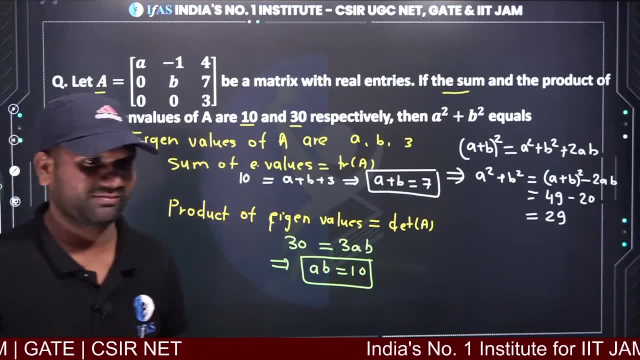 For now Priti is not in Jabalpur In Pune, and one is in Jodhpur. Okay, Come on. Yes, Priti, See your comment. I have also replied. Okay, Now Mano sir is saying Click to like: Come, Come, Come, Come, Come Come. 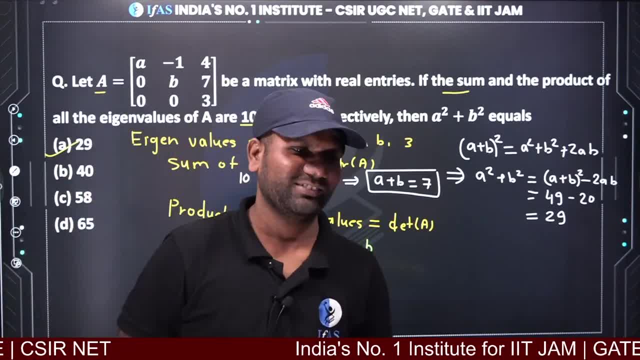 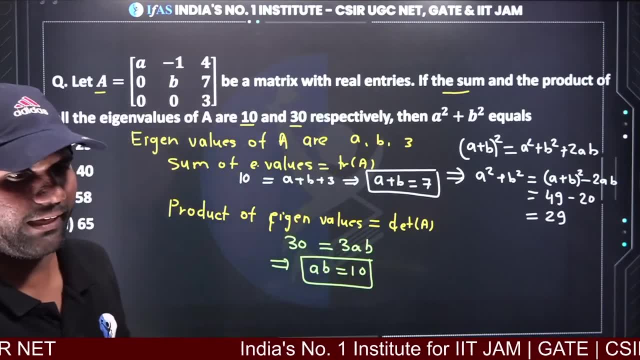 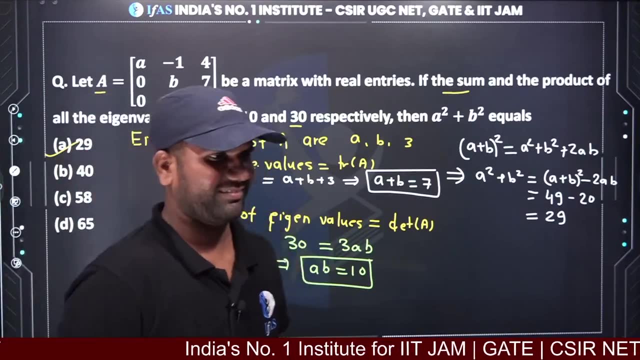 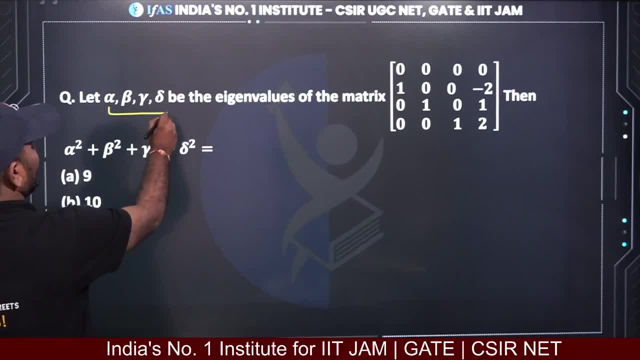 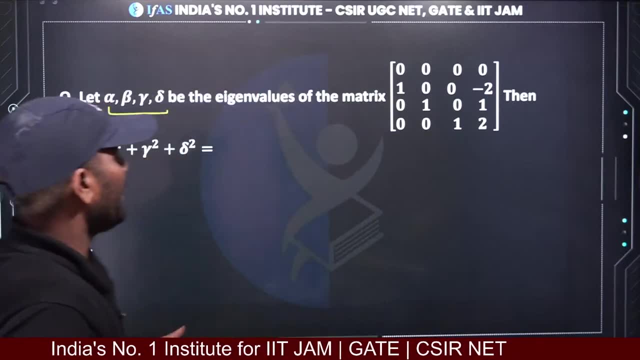 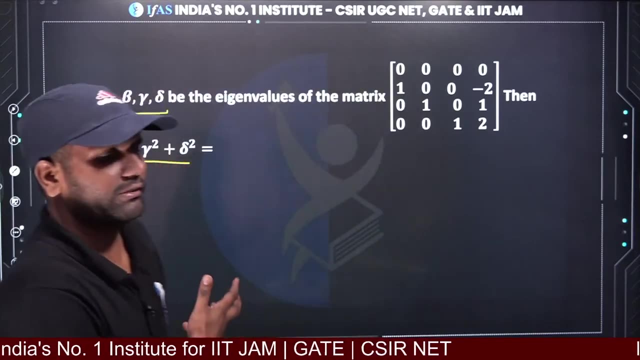 B, Eigenvalues Of this Matrix. So What will the value be? Alpha, Beta, Gamma And Eigenvalues value of this matrix. then, alpha square, beta square, gamma square, delta square, equals to what will happen. tell everyone what can happen, this value. come on quickly, tell me what will happen. 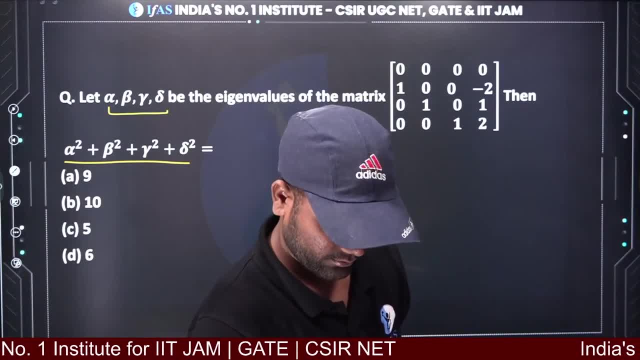 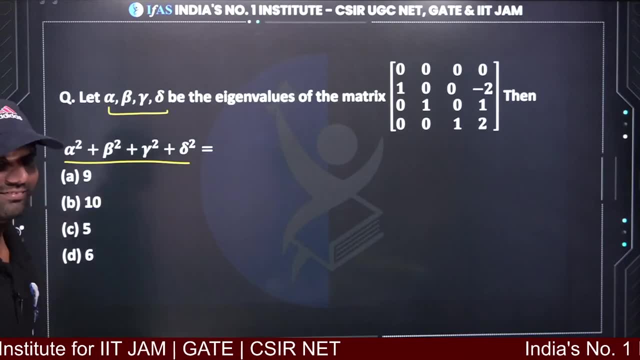 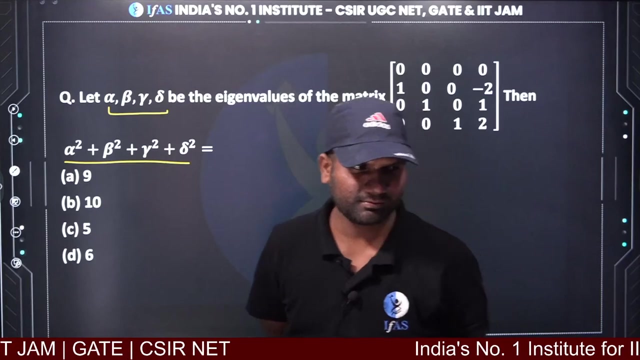 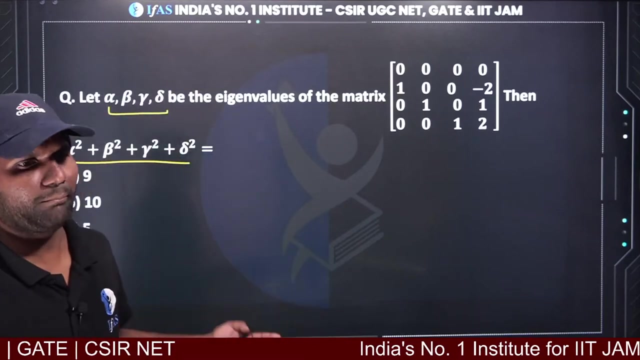 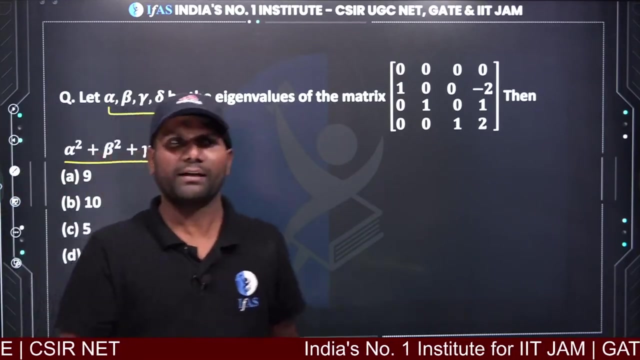 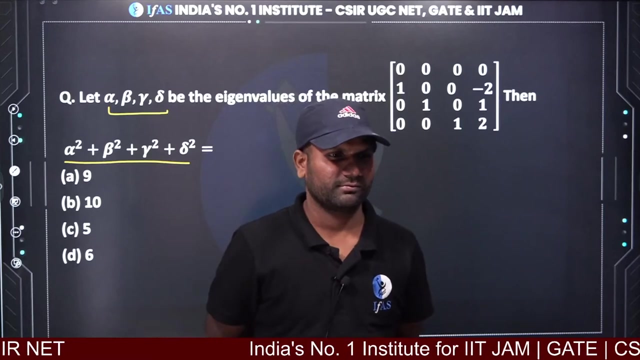 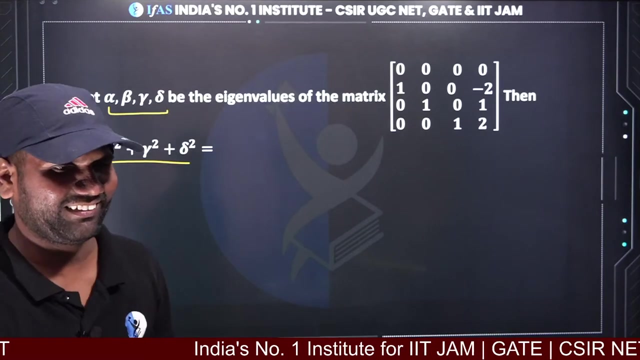 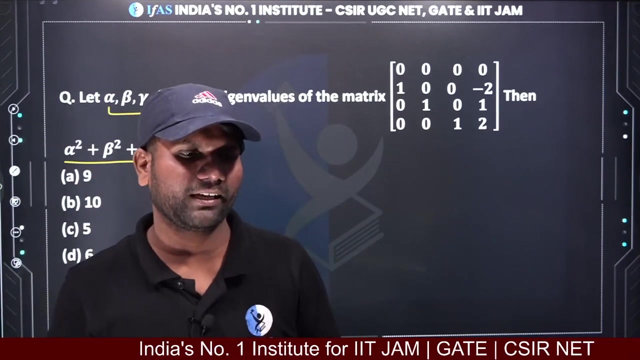 this value? what do you think? come on quickly, tell me what will happen. value of this value. come on now, tell everyone what is important. this value is real. Hari Om is correct. Hari Om has been done once right. tell the rest of the people. after this, something new will come. Hari Om. 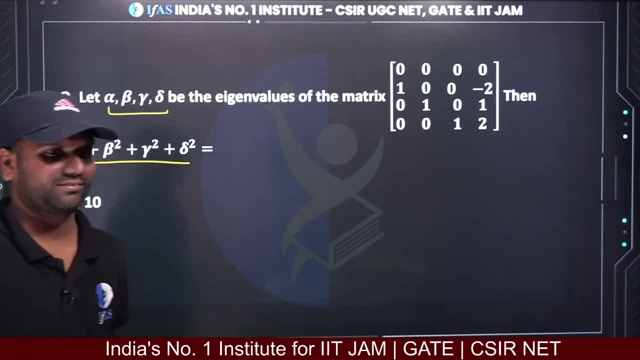 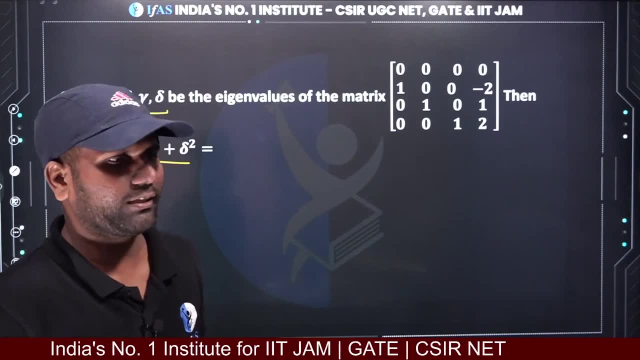 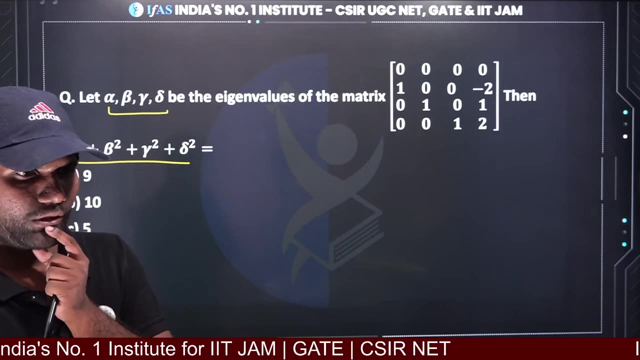 yes, yes, companion is Abhishek tell the answer of this. Abhishek will tell the answer. almost everyone. Varsha has told six. it is good. Rupendra Kaur has told A Rupendra, once you check again. 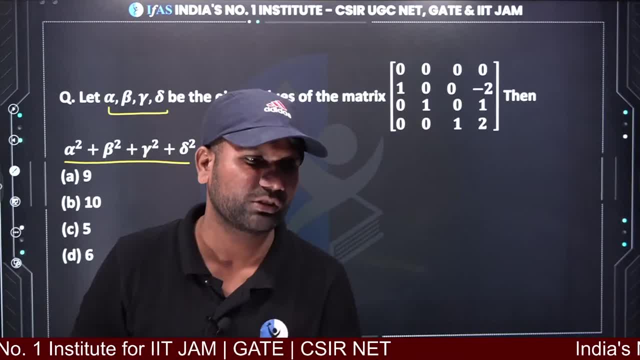 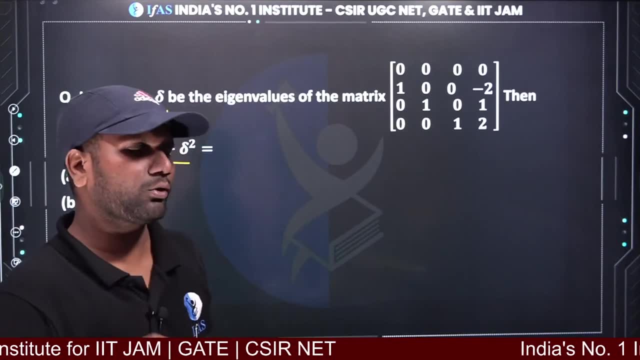 maybe something has gone wrong. check once, you guys. maybe something has gone wrong again. now see here, what is this? there is a result about companion matters. does everyone know, or should I tell you? tell me once, if you know. if you don't know, then I will tell you. 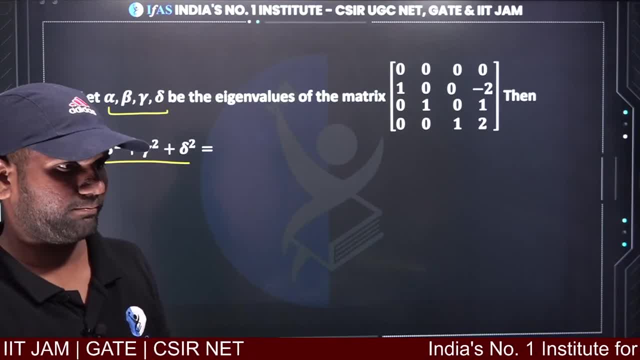 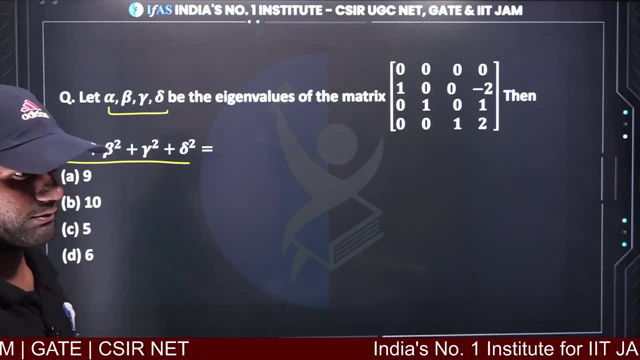 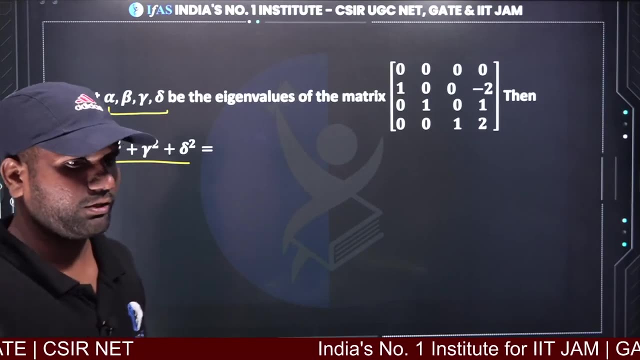 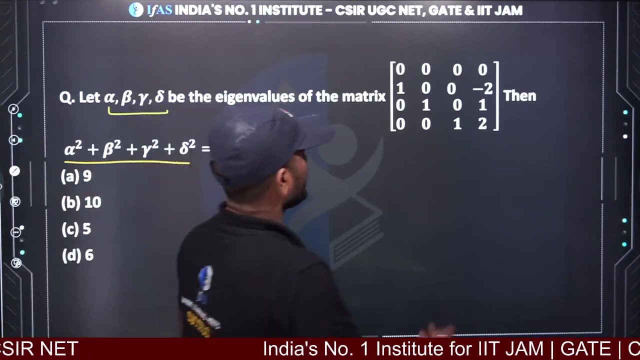 Vandana is saying six. very good, Vandana. I am saying option D, master six. yes, the option D 6 will be correct. take care, see it here. what is the companion matrix? I think you must all know one time. so see here. the special thing of this companion matrix is that the line below the diagonal 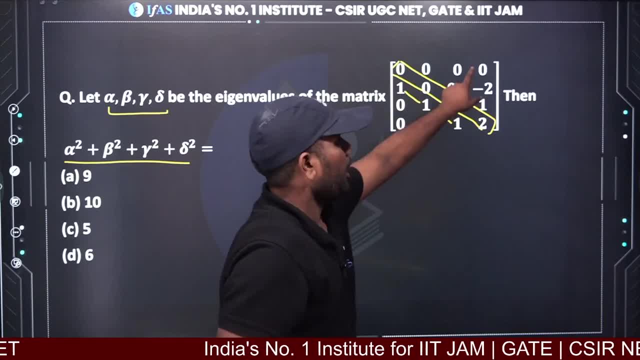 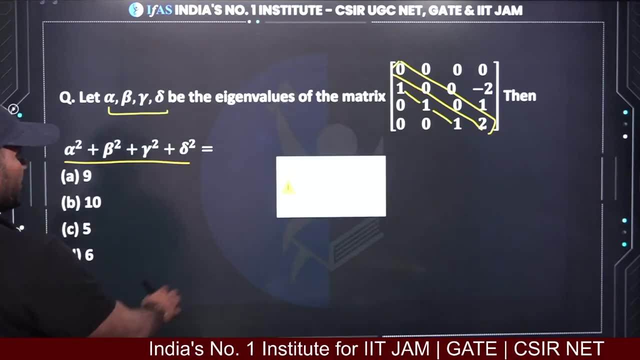 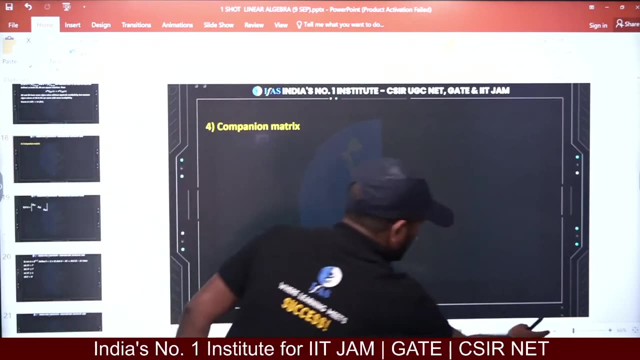 is not. look below the diagonals. if all the lines are one and on the side, they will get it constant. I will tell you in 1-2 minutes how the companion will be then. I will move ahead now. what is the meaning of companion matrix? first of all, I take a polynomial. 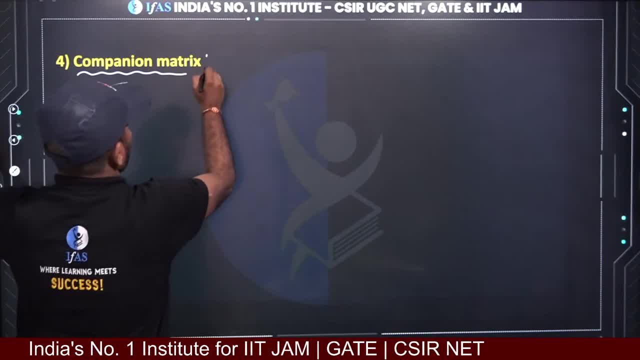 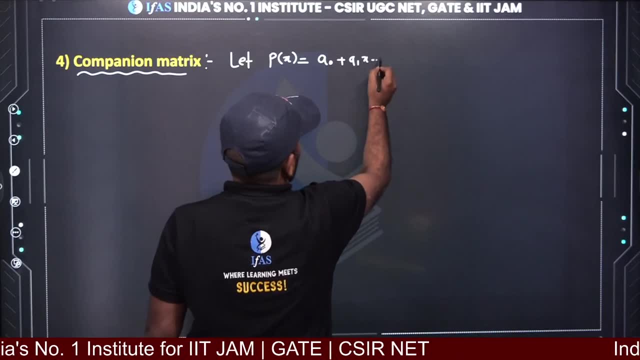 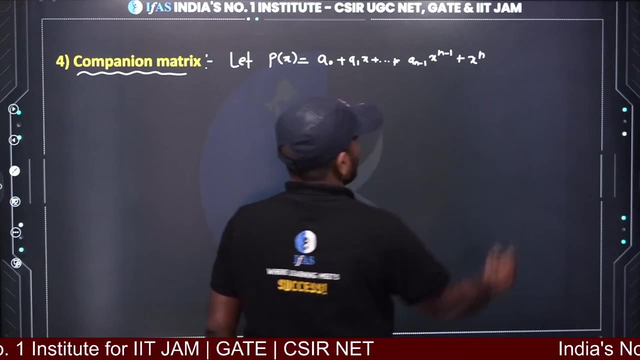 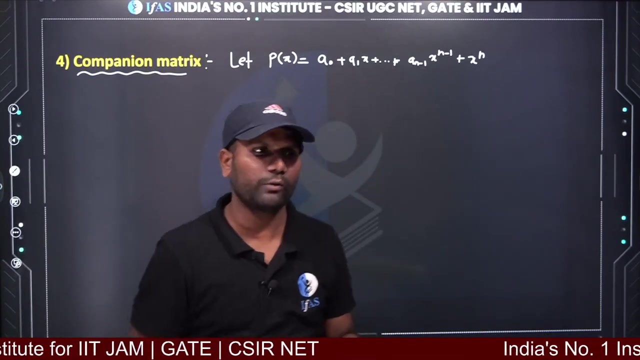 so let: p is a polynomial which is a 0 plus a 1x, so on: plus a n minus 1, x raise to n minus 1, plus x raise to n. so here I have taken a polynomial. so take care that the coefficient of x raise to n of polynomial is 1. 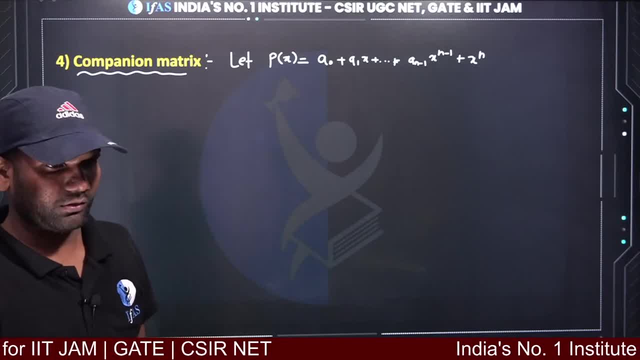 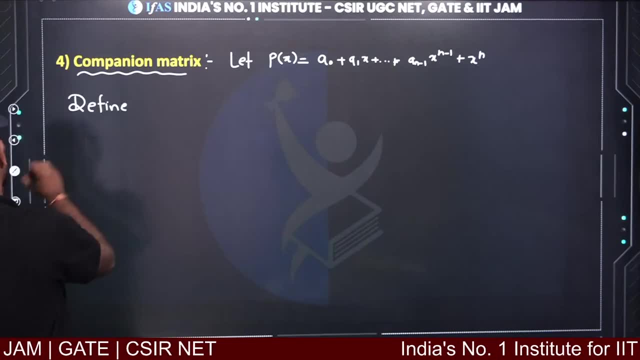 so the coefficient of x raise to n is 1 and x raise to n is 0. Now I will define a matrix. I am making a new matrix. There is something special about this matrix. What is special You will get to know now. 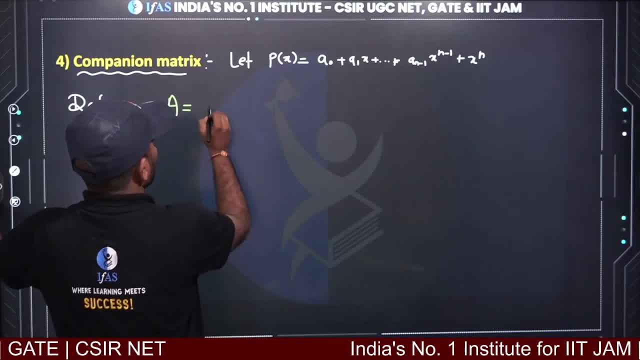 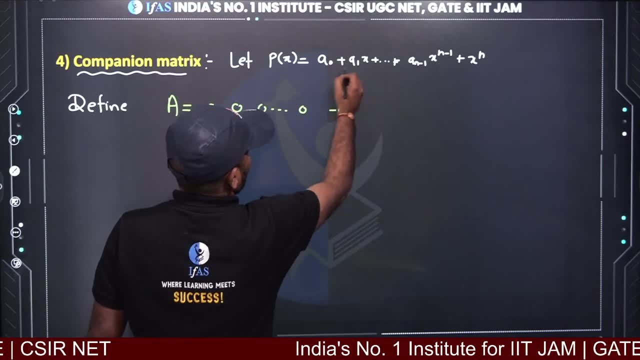 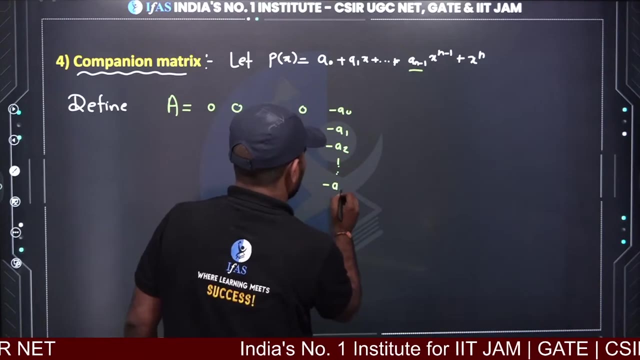 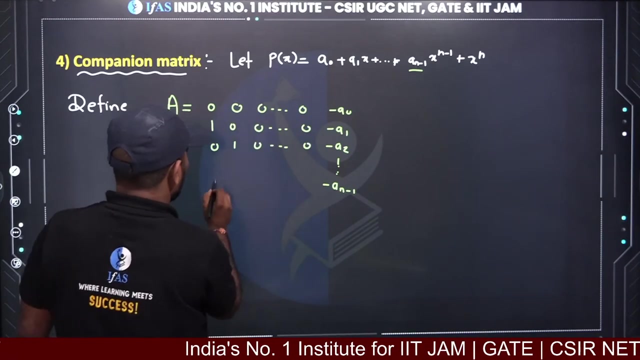 Suppose I have taken a matrix whose diagonal is 0, 0, 0, and so on 0. Here I am taking all the coefficients minus a0, minus a1, minus a2, and so on. In the last I have taken its coefficients minus an minus 1, and here 1, 0, 0, 0, 0, 1, 0, 0, 0, 0, 0, 0, and so on, 1.. 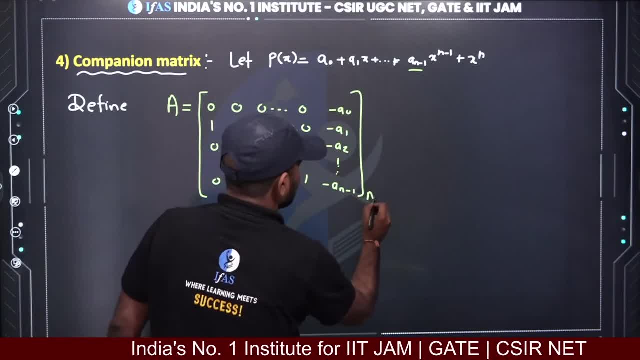 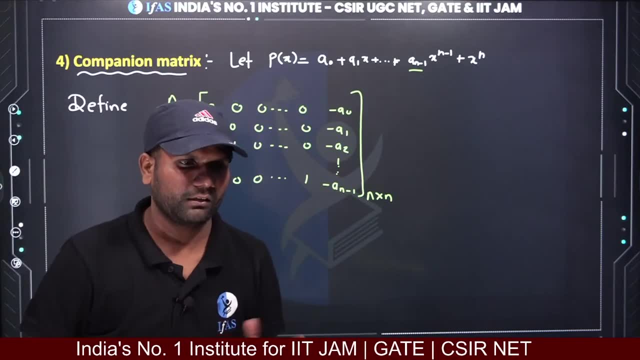 So we have taken a matrix here. Now what is its order? It is n cross n. Now this type of matrix is called a companion matrix. Do you understand? This type of matrix is called a companion matrix. So if you see here, 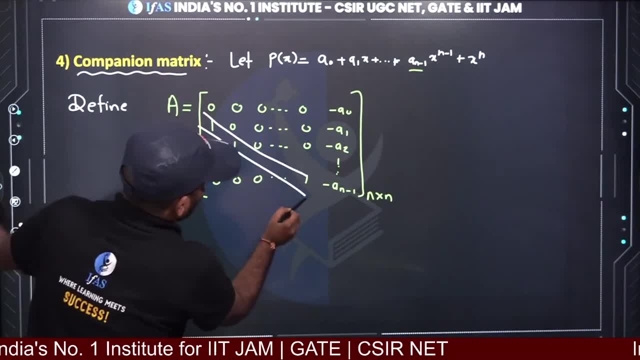 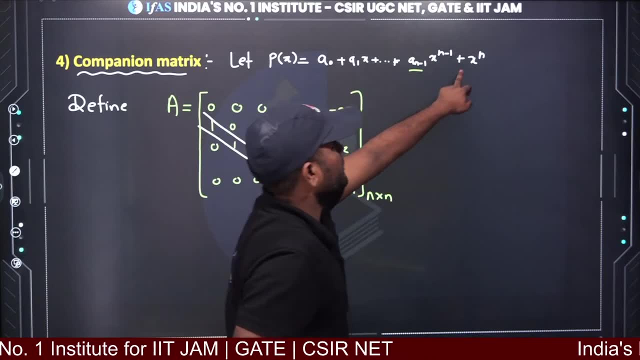 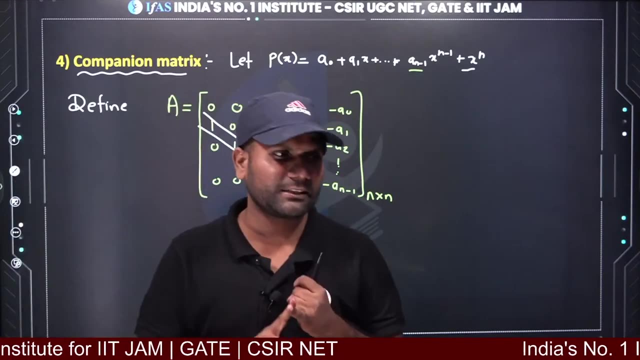 The line below the diagonal. What do you get there? You get 1.. And the last column. What is the last column? These are the coefficients of the polynomial, except x raised to n. So the matrix of this type, its characteristic polynomial and minimal polynomial. 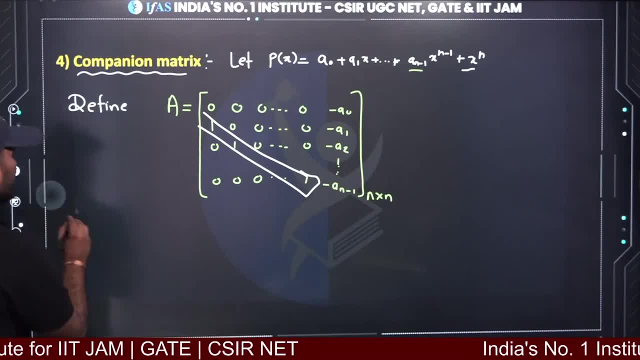 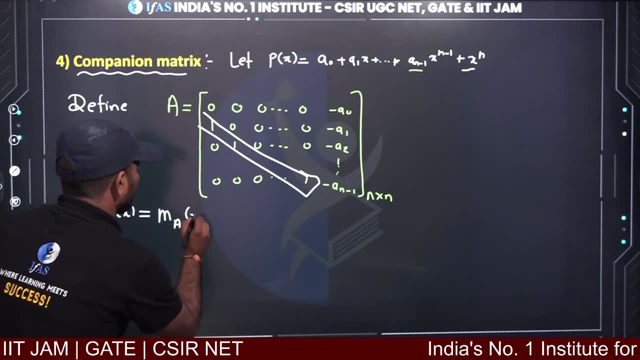 What do we always get? The characteristic polynomial and minimal polynomial for this type of matrix is always is equal to Its characteristic polynomial and minimal polynomial. What do I always get? I will always get a p of x equal to Okay, And here we have a result. 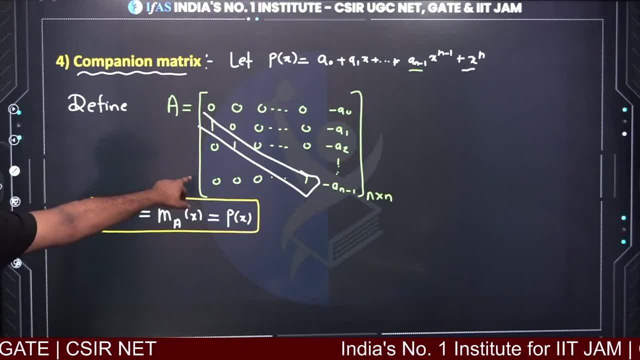 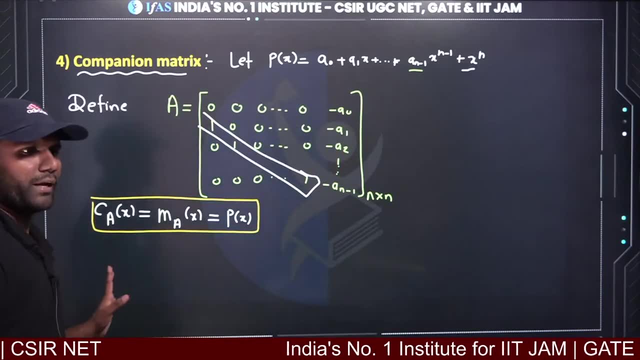 We have to keep this result in mind. So this type of matrix is called a companion matrix. With this you can find its characteristic: polynomial and minimal polynomial. I hope it will be clear to everyone here. Look at it once. Is everyone clear? 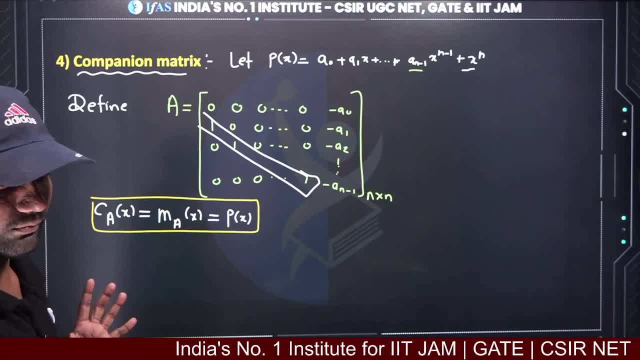 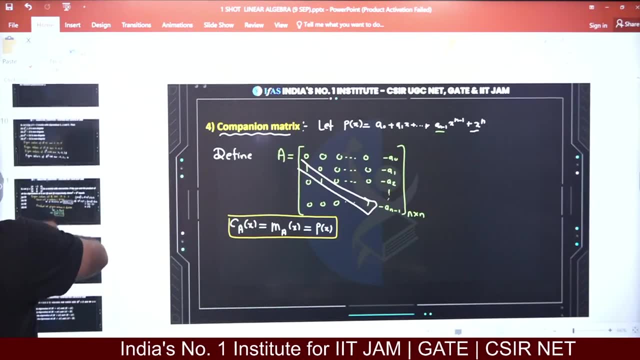 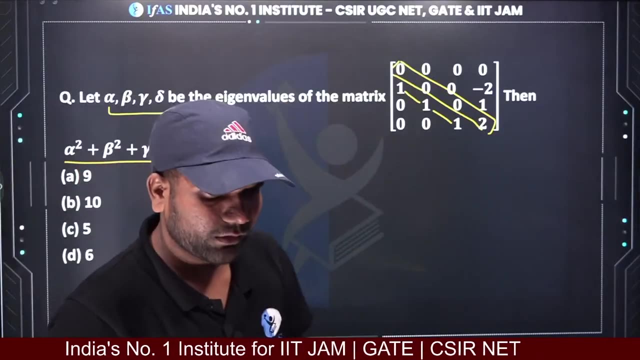 Clear. Okay, Let's go Now. let's come here, The one. we did a question, The companion one Which you have ever seen- to solve the question Now. see the question. Now there is a companion matrix. Is there a companion matrix? 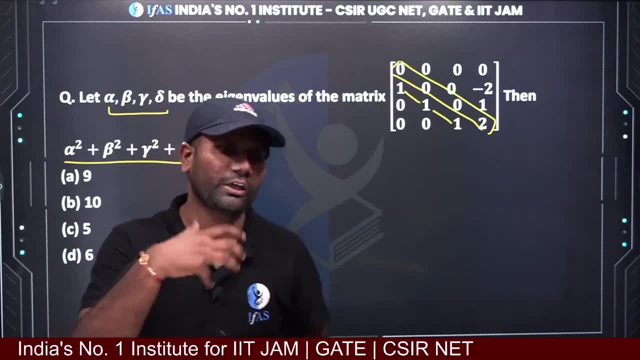 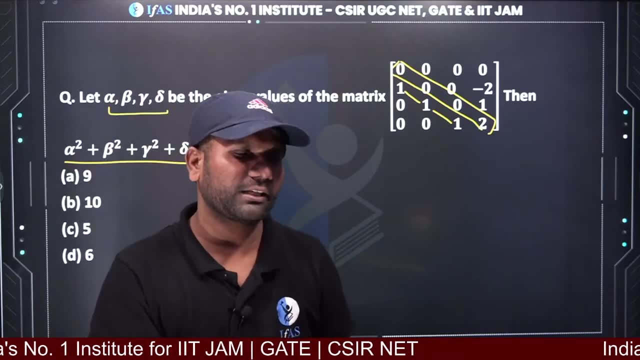 Subina is not always diagonalizable. It depends on the minimal polynomial. If it is linear, then it happens. Otherwise it is not always the same Companion. When is the matrix diagonalizable? I will tell you about this in detail tomorrow. 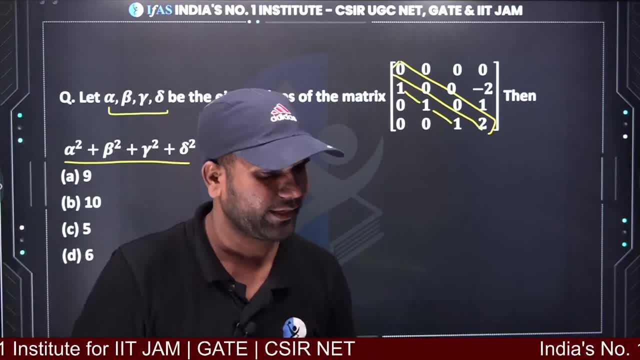 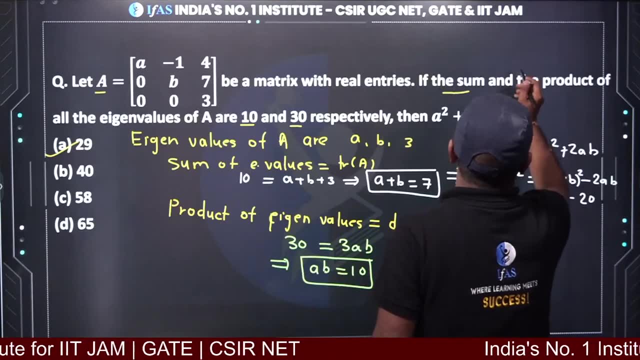 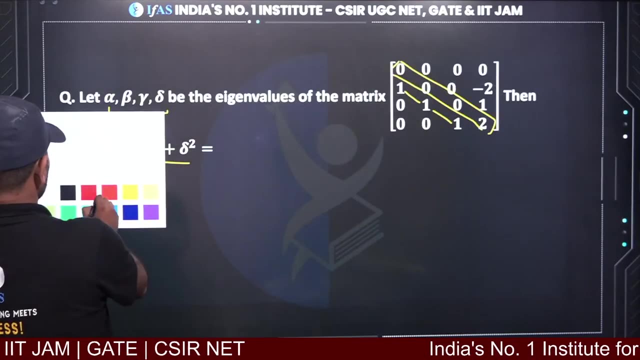 Some important results properties that will work for you in the exam. Okay, Now see here. What did we take in the last Coefficient? What did we get in the last We used to get coefficient? Its coefficient was polynomial. Here is the matrix of 4 cross 4.. 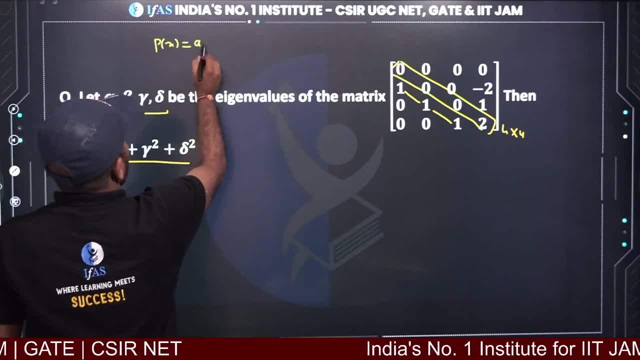 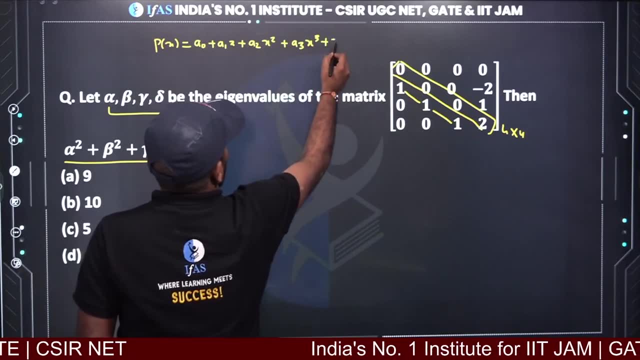 So our polynomial. What will happen in this case? a0 plus a1x plus a2x, square plus a3x, cube plus x raised to 4.. This will be the polynomial. See everyone, This will be the polynomial, Okay. 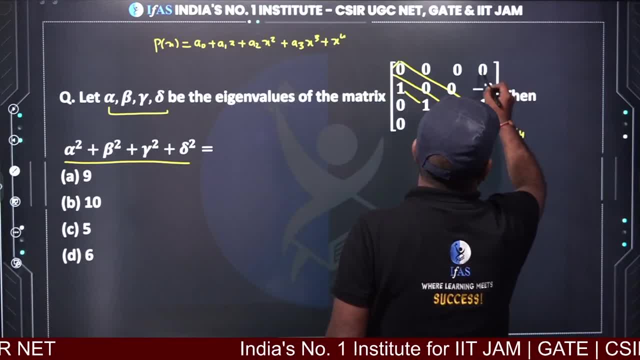 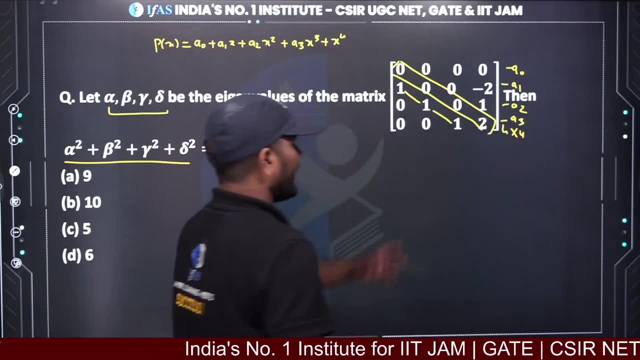 If the polynomial is a. So what is this here? This 0 means This is your minus a0.. This is minus a1.. This is minus a2.. And last is minus a3.. So from here you can find the values of them. 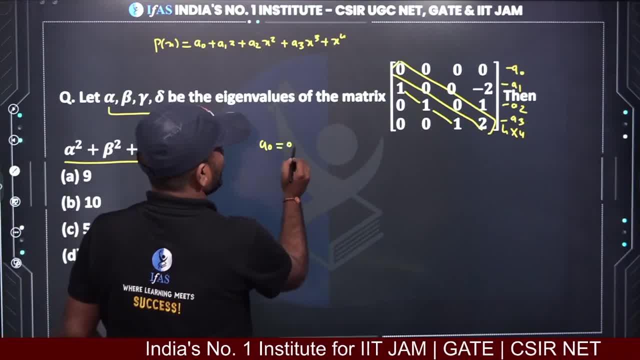 So what is a0?? If you see the value of a0.. This is 0.. This is 0.. What will be the value of a1.. This will be 2.. What will be the value of a2.. This will be minus 1.. 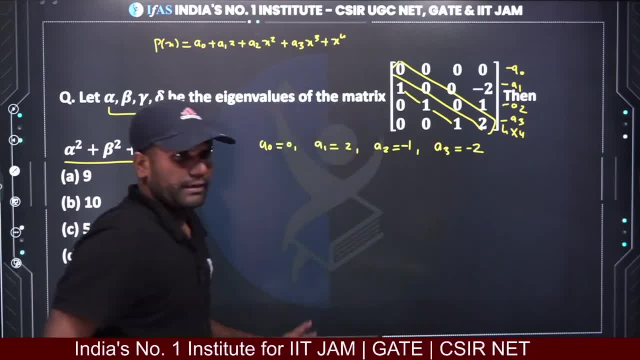 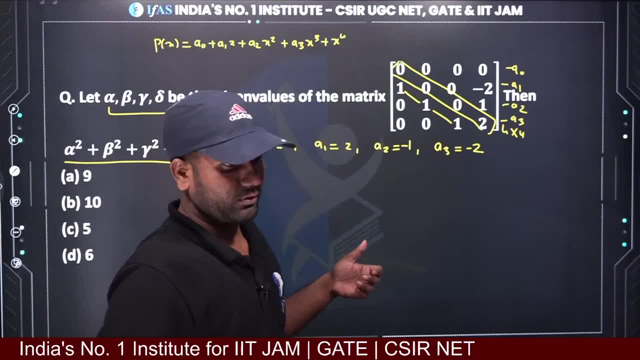 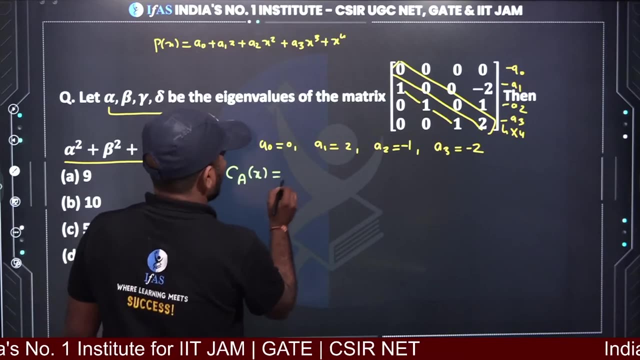 And what will be the value of a3.. This will be minus 2.. Is everyone clear? till here, Okay, See, everything was fine. till here, Okay. Now see What will you get in its characteristic polynomial. So the characteristic polynomial of this matrix is a0. 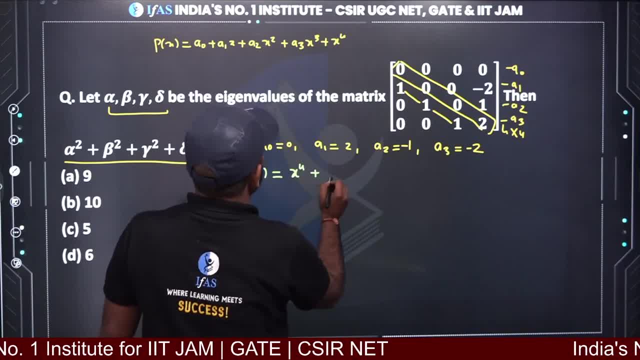 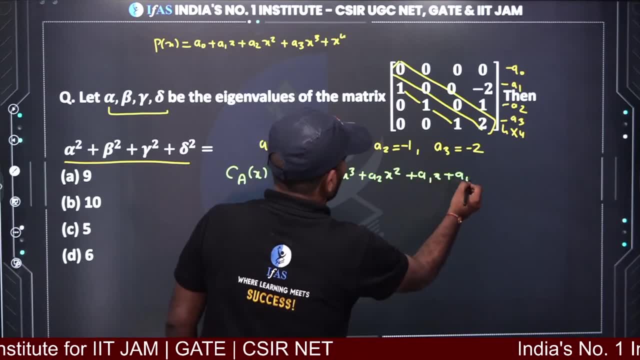 That is, we write it reverse- x raised to 4 plus a3x cube plus a2x square plus a3x square plus a3x cube. So what will be the value of this matrix? 3x3 plus a2x2 plus a1x plus a0? here it is x raise to 4. 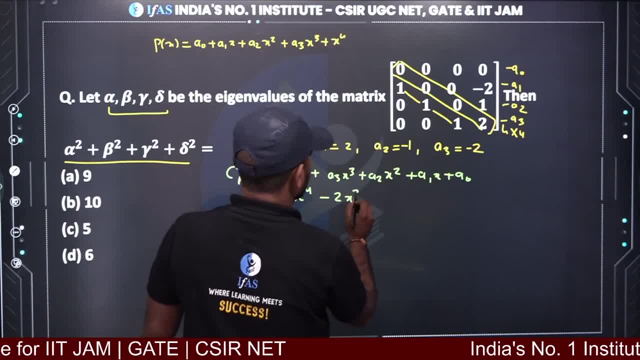 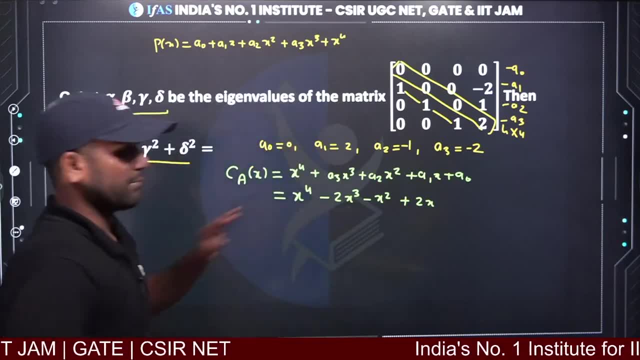 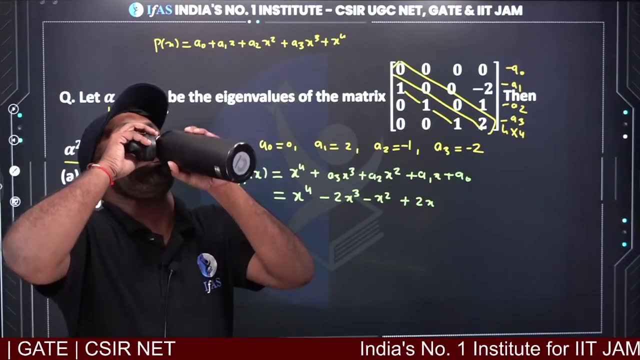 what is the value of a3? minus 2, minus 2x3. what is the value of a2? minus 1x2, plus 2x. and what is a0?? you got 0. see everyone. till here. is it clear? till here. 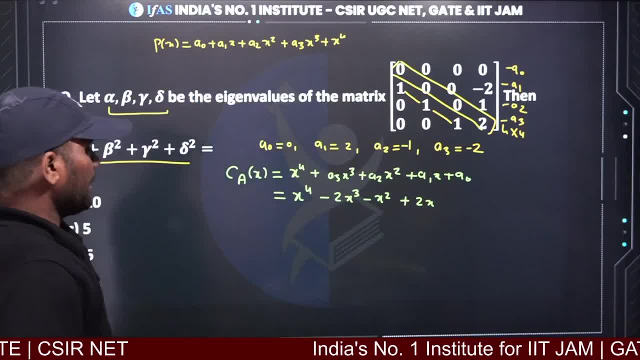 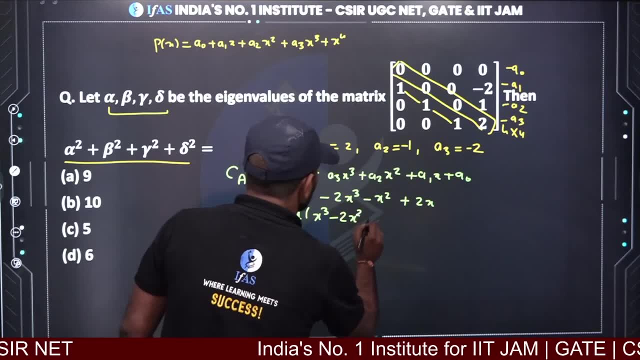 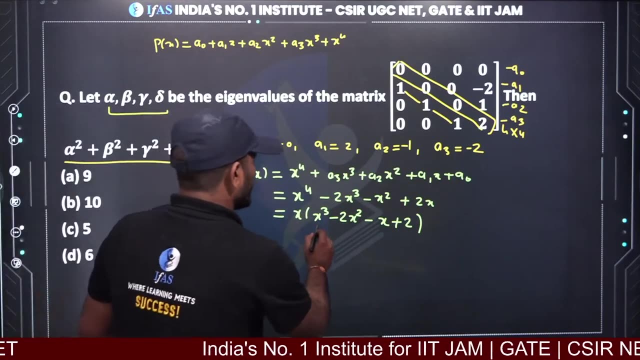 is it clear now what we can do? we can take x as a comma. if we take x as a comma, so this is equal to x3 minus 2x2. what will happen? minus x plus 2. ok, now what I do from here. I take x2 as a comma. 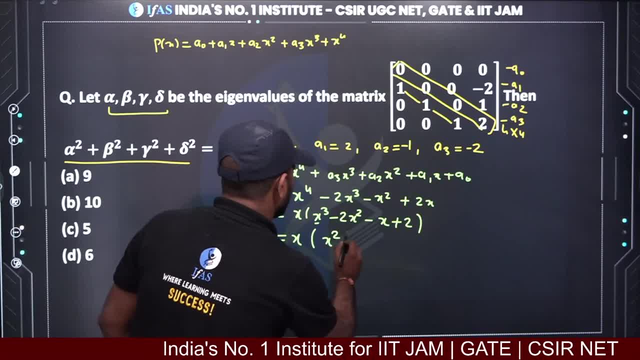 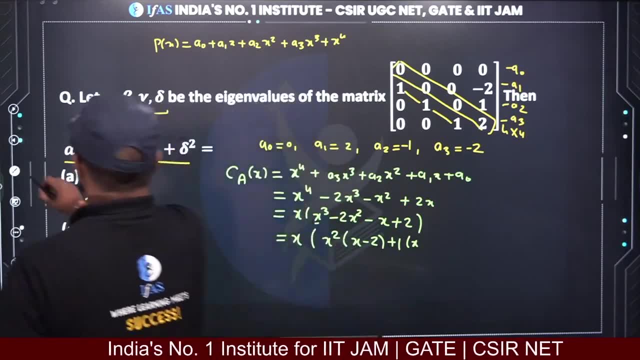 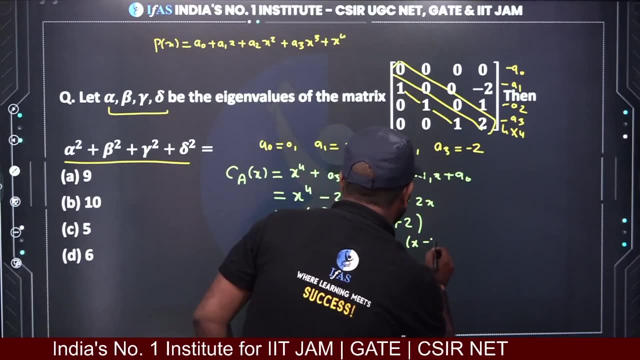 so what will I get if you take x2 as a comma? what will happen? x minus 2 plus 1? what will happen? let's take minus here. if you write minus, what will you get? minus x minus 2? ok, so from here you can tell what will you get. 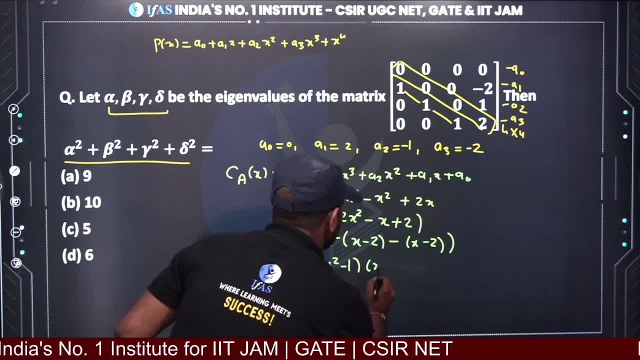 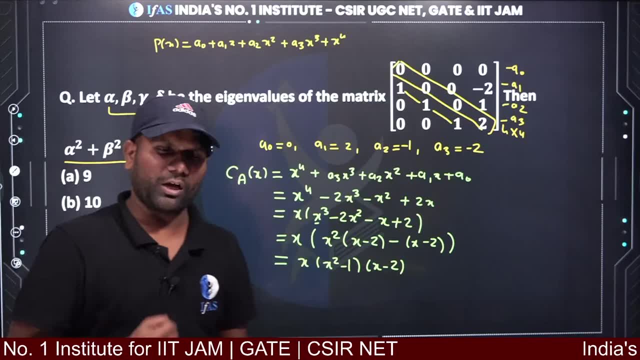 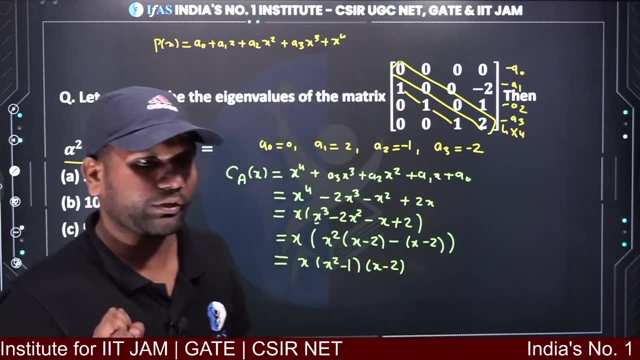 x, x2 minus 1, and this will be x minus 2. now you got its characteristic polynomial. if you have characteristic polynomial, then you can get eigenvalues very easily, isn't it? you can get it very easily. there will be no problem here. I don't think there should be any problem. 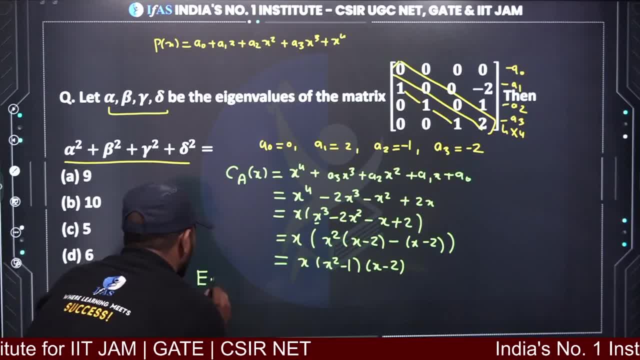 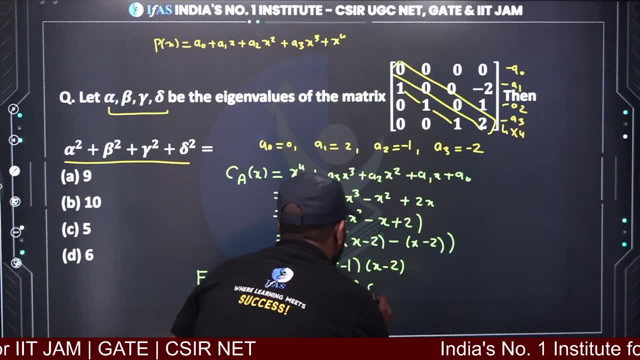 ok, if you have eigenvalues, then what will be the eigenvalues here? so, eigenvalues, if you see the eigenvalues of a, what will be the eigenvalues of a? one will get 0,, one will get plus minus 1 and one will get 2. 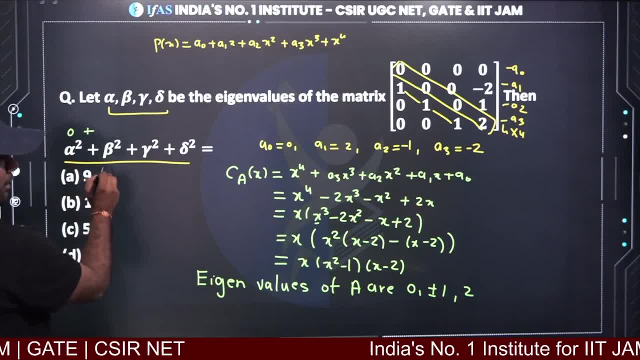 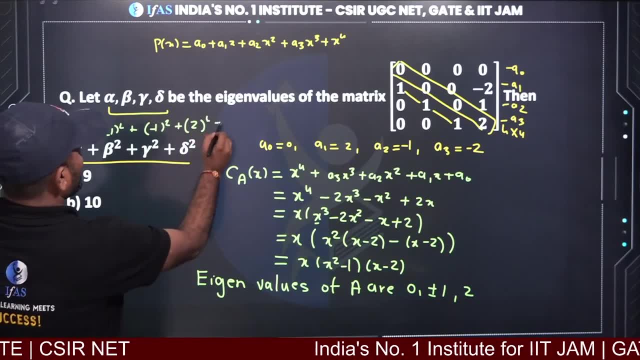 ok. so see, suppose alpha is 0, one is 1 square. what is the other? it is minus 1 square and the third is 2 square. so if you add, then what will you get? it will be 6. it means that option b will be correct here. 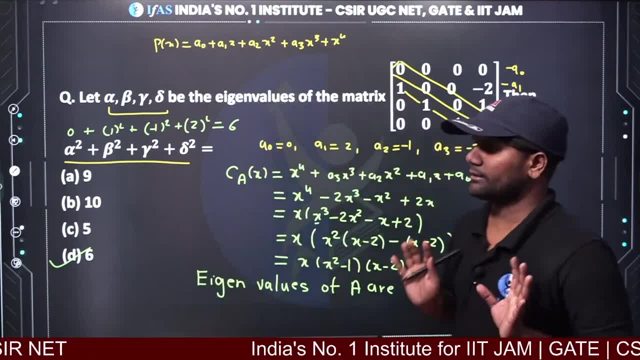 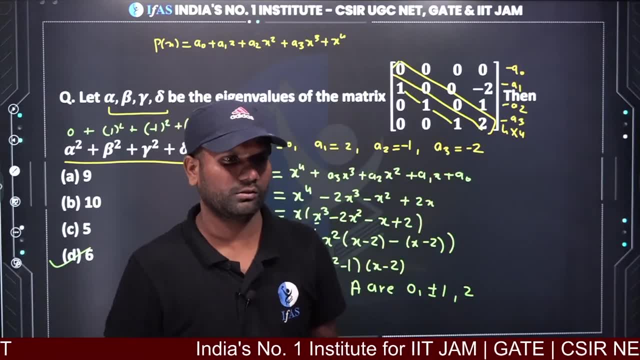 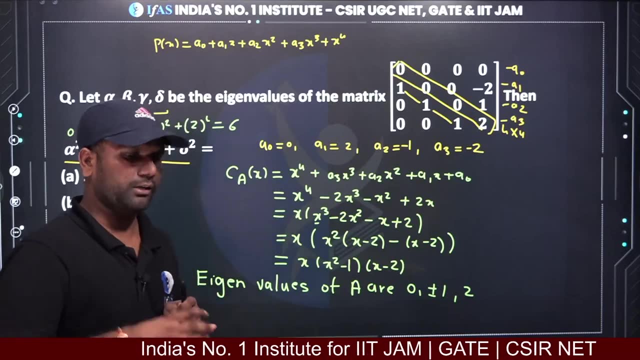 ok, is it clear to everyone? see it once. there is no doubt till here, right? ok, come on, just sit with cool mind in the exam. and as I told you in the start, that in linear algebra if any question looks related to matrix, then there are 4 types of counter examples. 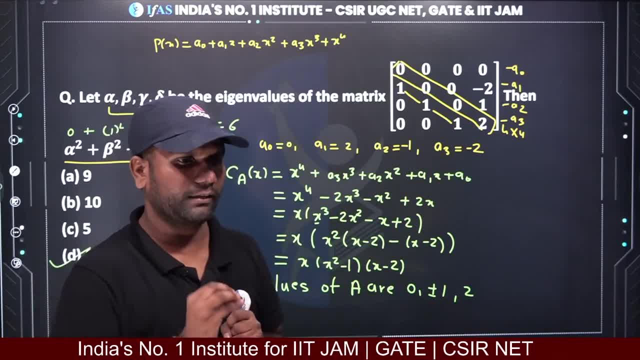 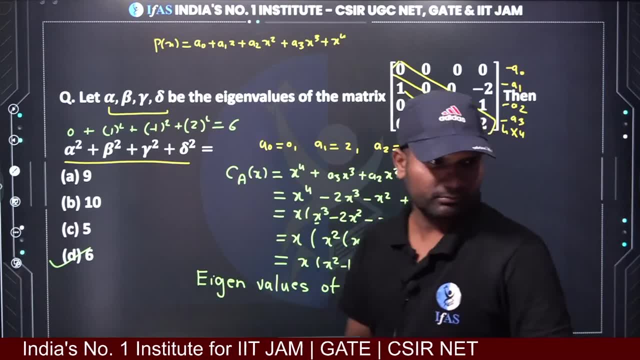 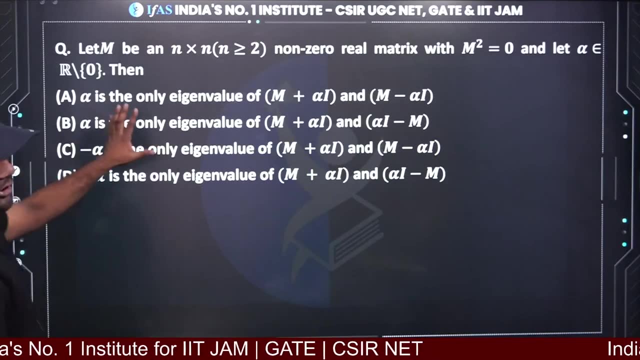 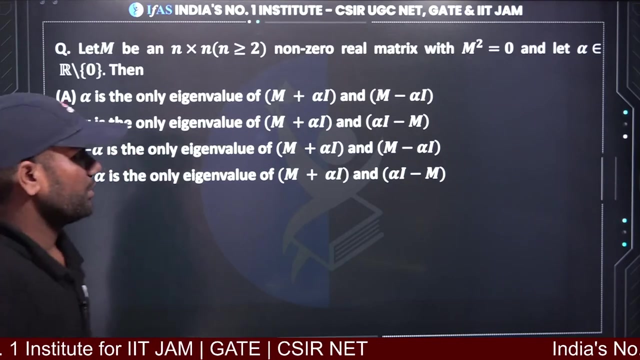 which definitely discards one or two options. you also have to take care of that, ok, ok, now let's move on to the next slide, to the next question. you can do this question very easily. you can do it see. tell me the answer of this once. hint for you is that. 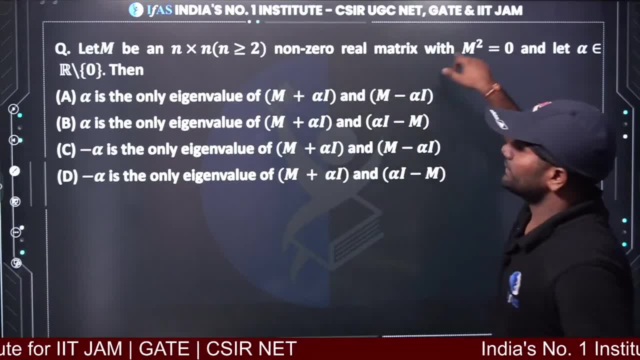 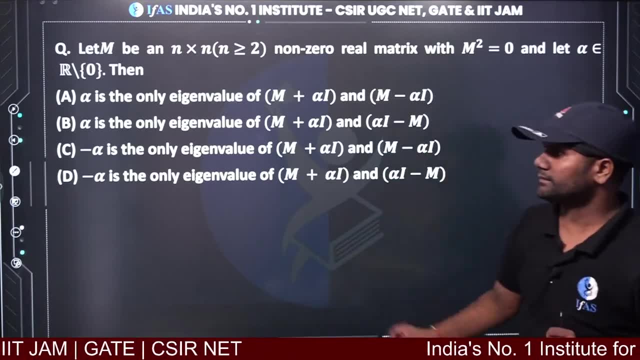 m square equal to 0. m square equal to 0. it means that it is a nilpotent matrix. and we know that a matrix is nilpotent matrix if, and only if, all its eigenvalues are 0. so apply that result, you will get answer. 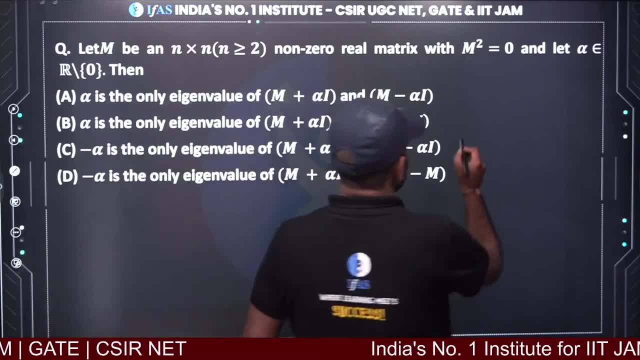 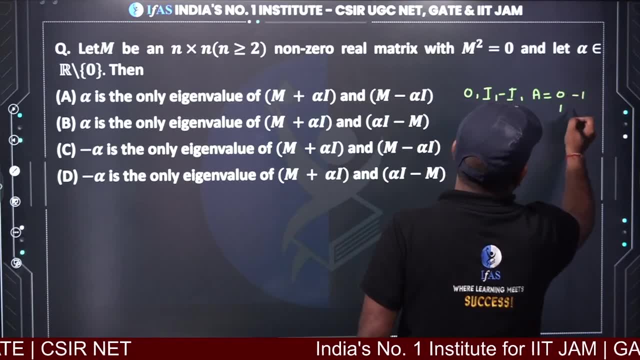 yes, that counter example. yes, I will tell you that counter example I told you in the start. one is zero matrix, one is identity, one is minus identity and one is special type matrix minus 1, 1, 0. these four use them in the exam. 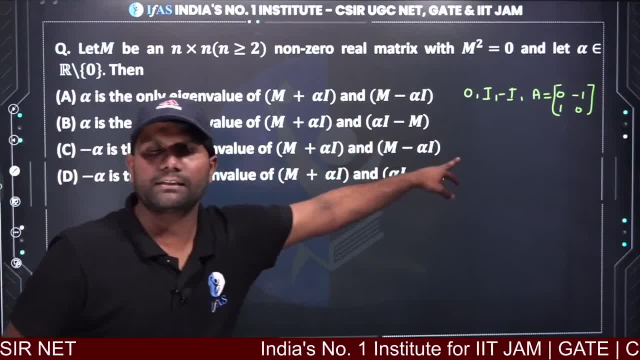 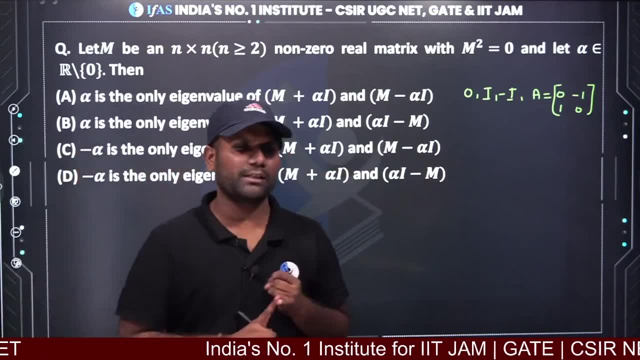 the special thing of the last one is what are its entries? they are real numbers but eigenvalues are plus, minus i we get imaginary in the exam. when you want to make counter example for any matrix, then take simple matrix, not like 1, 4, 5, 6. 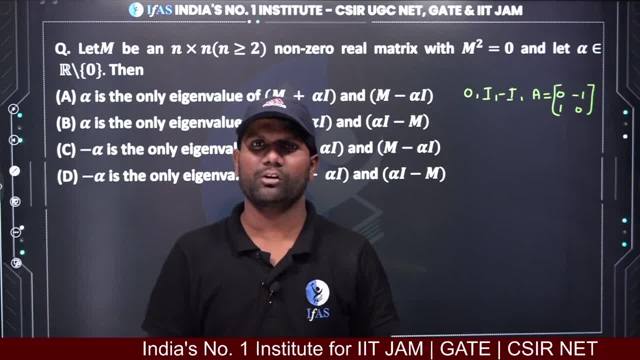 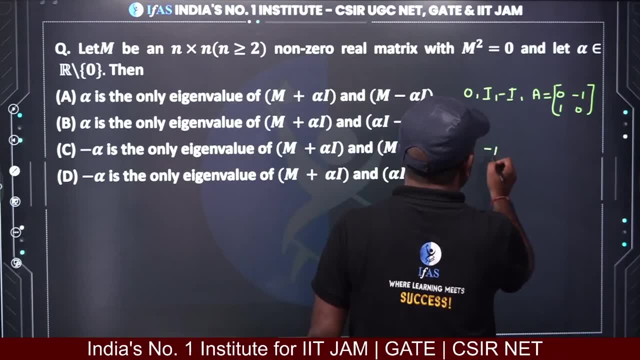 take anything. you don't have to do this. start with simple. first, look at zero, look at identity, look at minus identity. if it is not working, then take such a matrix: 1, minus 1, 0, 0. take work with this if it is not working. 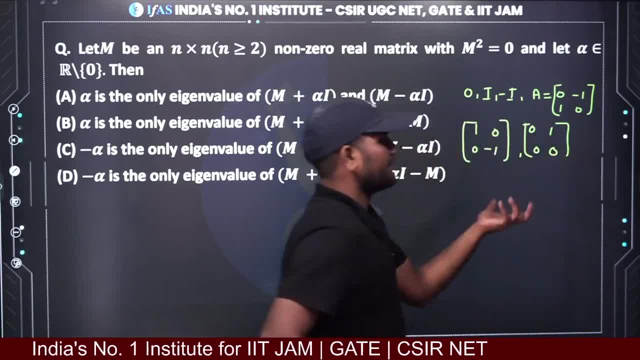 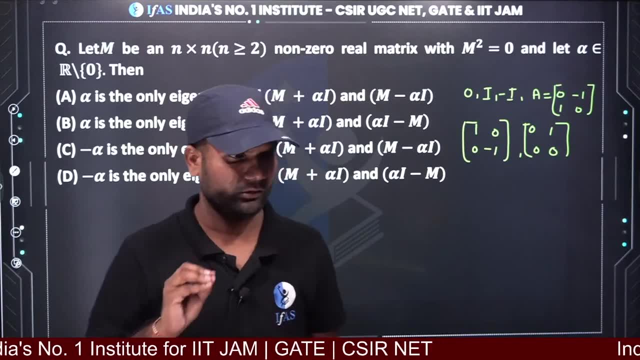 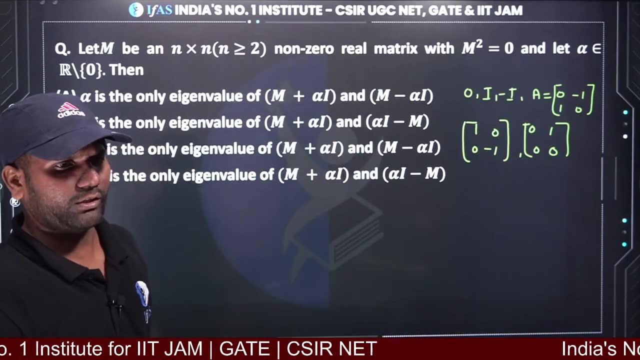 then 0, 0, 1, 0 work with this. so try to make simple matrix as counter example for counter example. don't take any complicated matrix for counter example. it is very easy. ok, now this question. I think you guys will solve it very easily. 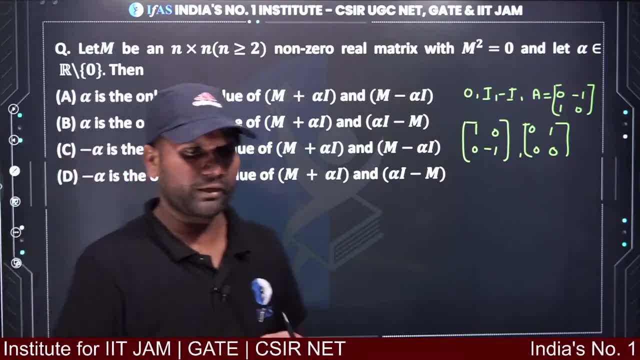 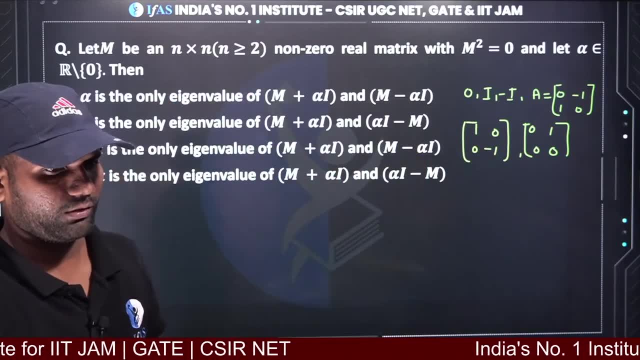 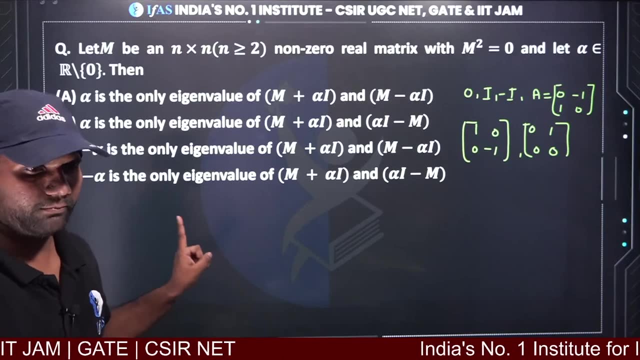 almost all people are saying now. so many people are saying so I don't have the courage to say wrong. ok, very good in this question. does anyone have doubt that should I move forward? I think you all will do it. ok, tell me once if anyone has doubt. 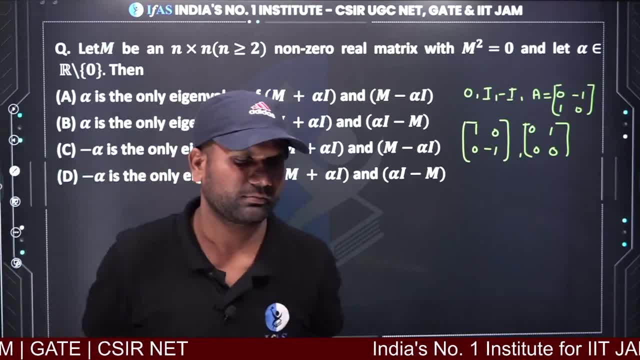 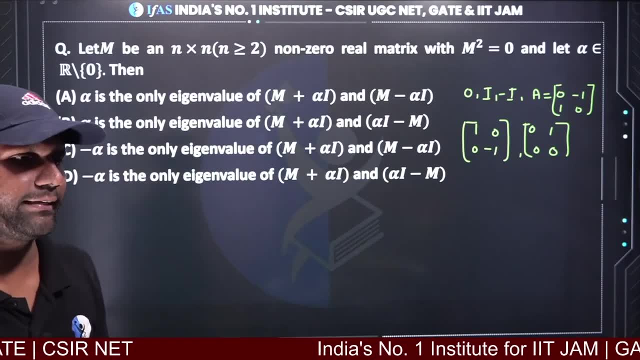 then I will do it. otherwise, if anyone has doubt, then I will keep going, then only those who have doubt, and if anyone has doubt, then think that you can work with me, ok, ok, answer 1, 2, 3, 4, 5, 6. 7,, 8, 9,, 10, 11,, 12, 13,, 14, 15,, 16, 16,, 17, 17,, 18, 19, 20, 22,, 23,, 24, 25,, 26,, 27. 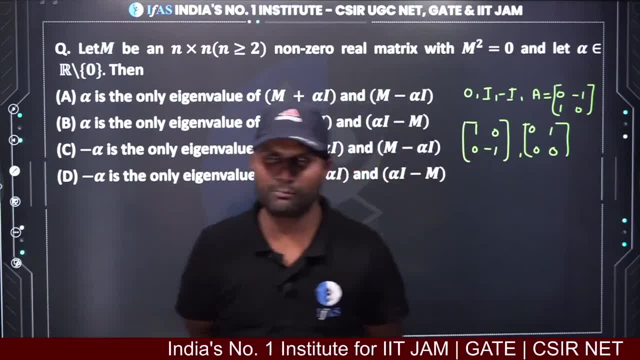 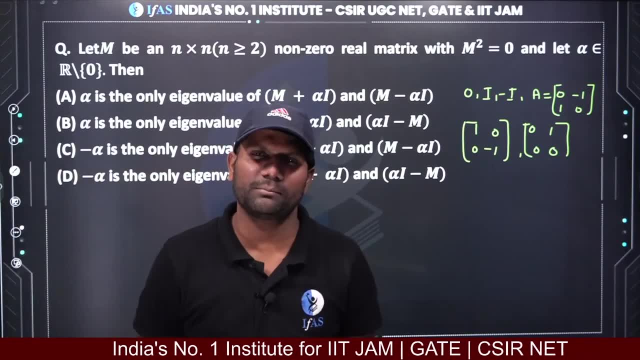 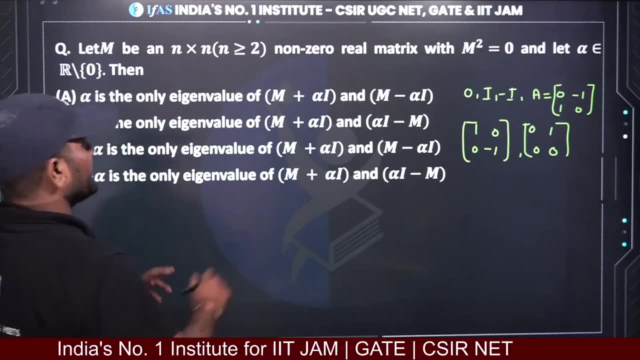 28, 28,, 29, 30, 35, 24. like a child, think of the simple one. that's the right thing. it should never be complicated. tell me what is m square? m square is equal to zero. it means that what will be m? m is a. 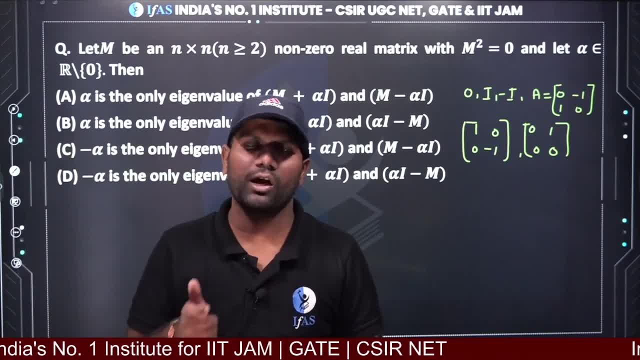 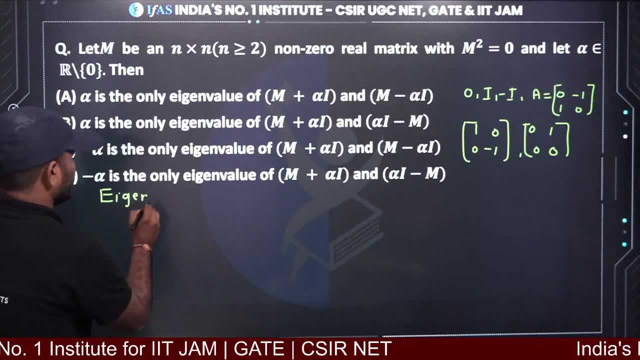 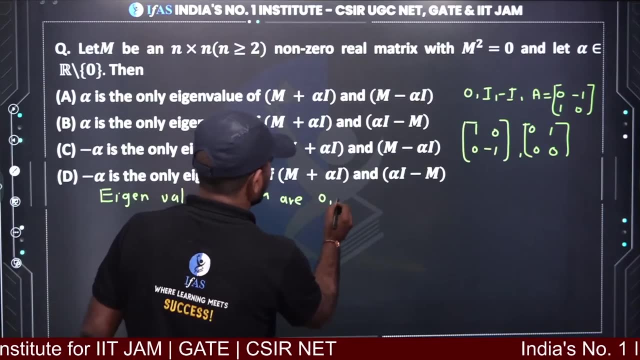 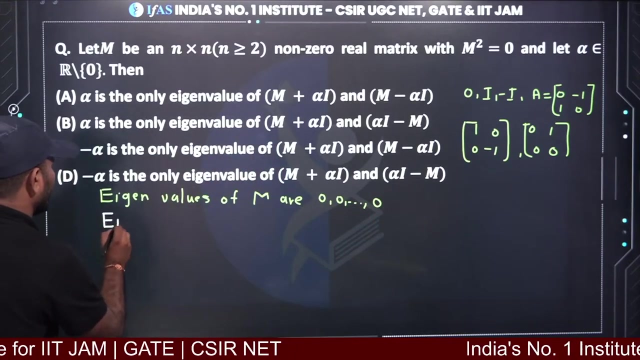 nilpotent matrix. if m is a nilpotent matrix, then all its eigenvalues will be zero. so eigenvalues of m are, so all the eigenvalues of m will be zero, zero and so on, zero. now here we talk about the question given to us: m plus alpha is so eigenvalue of m plus alpha? 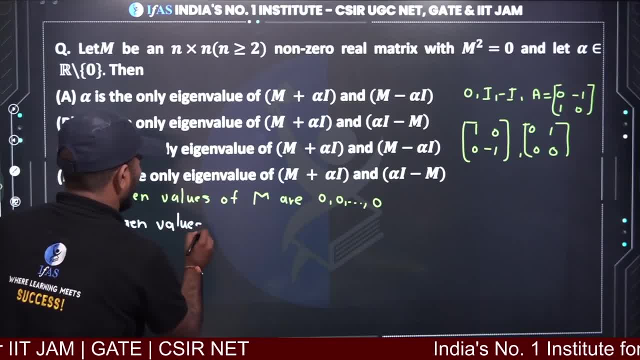 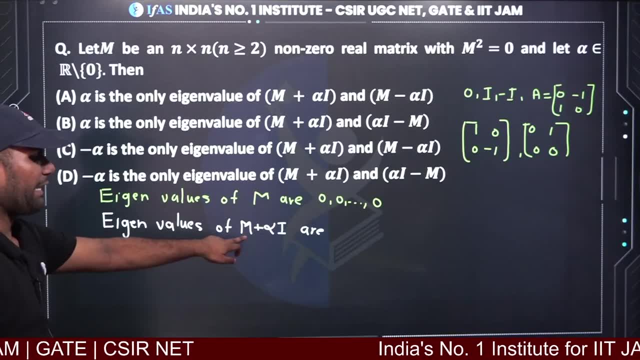 i will be eigenvalues of m plus alpha i. if you remove eigenvalues of m plus alpha i, then what to do? instead of m eigenvalue, eigenvalue of m plus alpha i will be eigenvalues of m plus alpha i. on but one instead of identity. eigenvalue is zero. all its eigenvalues will. 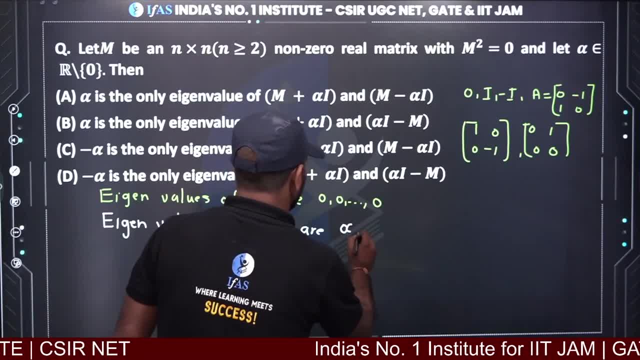 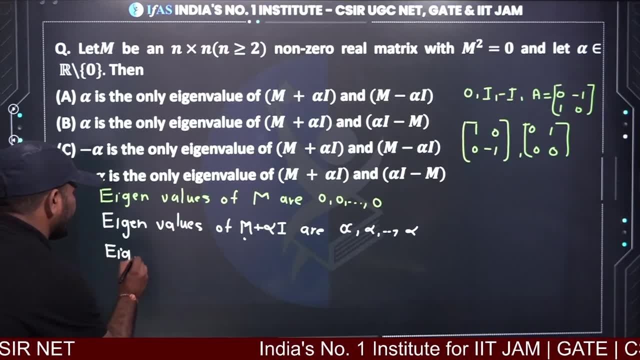 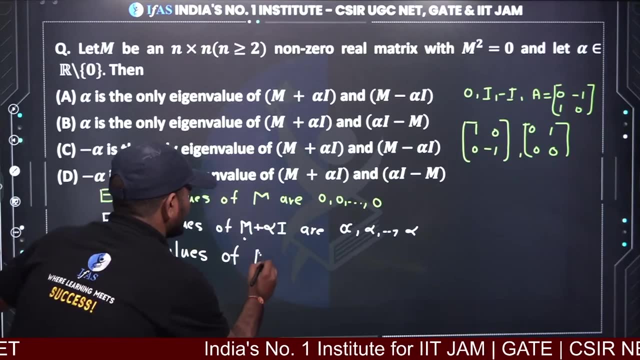 be 0 plus alpha. 0 plus alpha i means alpha i, alpha, alpha, alpha. you will get its eigenvalues. similarly, if you have to find here eigenvalues of whose eigenvalues, so eigenvalues of you, will be asked about eigenvalues of m minus alpha i. so what eigenvalues of m minus alpha? 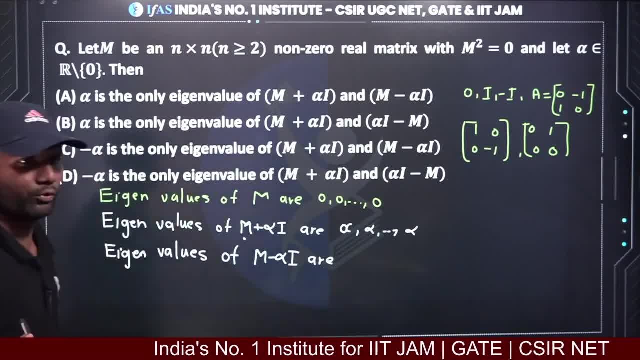 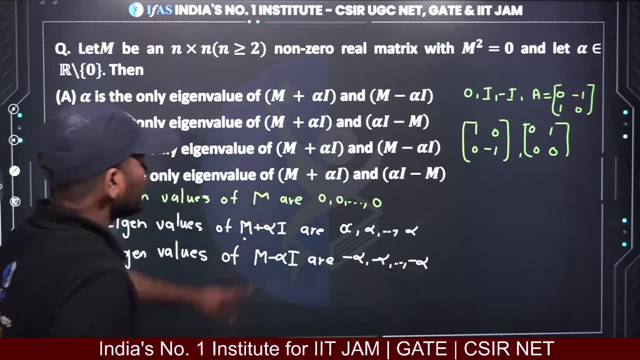 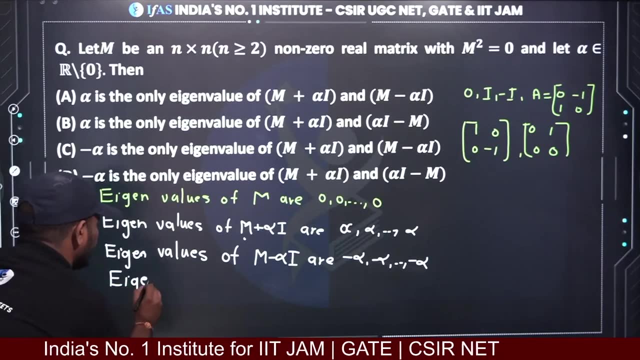 i will be so if you look at the eigenvalues of m minus alpha i, then what will happen? now you will get minus alpha, minus alpha, and so on, minus alpha, and what is remaining, m minus alpha is alpha i minus m. so here you have seen the eigenvalues of 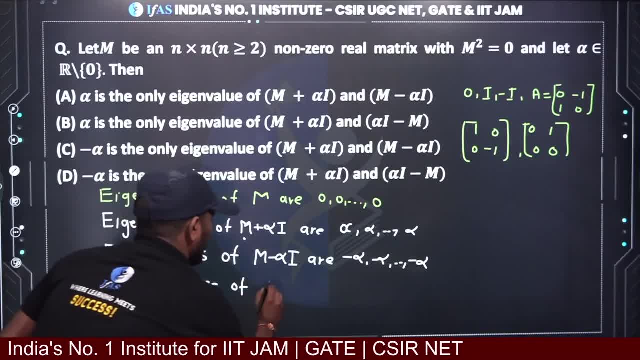 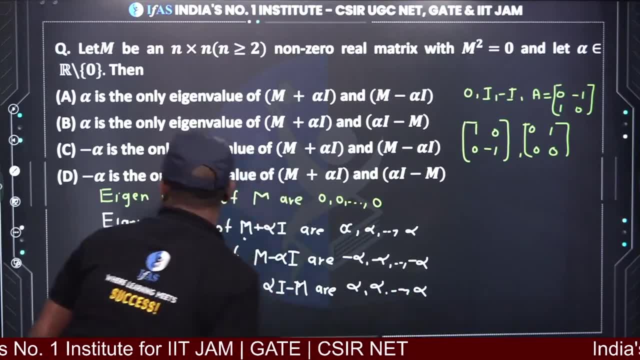 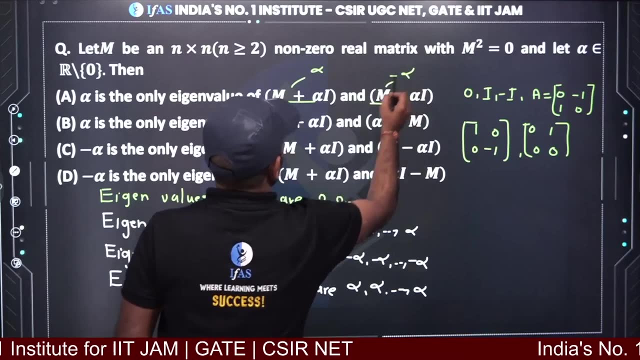 eigenvalues of alpha, i minus m. so what will be the eigenvalues of this? you will get the eigenvalues of this alpha, alpha and so on. alpha- now you can see the option. from here, its eigenvalues will be alpha and its eigenvalues will be minus alpha. 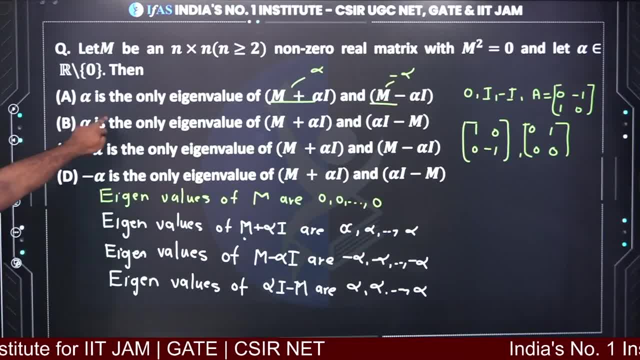 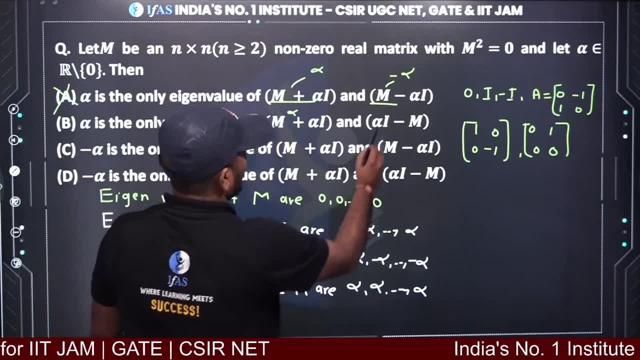 so the first option is incorrect. first option is saying that alpha is the only eigenvalues of these two matrices, which is incorrect. second option is: what will be its eigenvalues? its eigenvalues will be alpha and its eigenvalues will be also alpha. second option is: what will be its eigenvalues? its eigenvalues will be alpha and its eigenvalues will be also alpha. 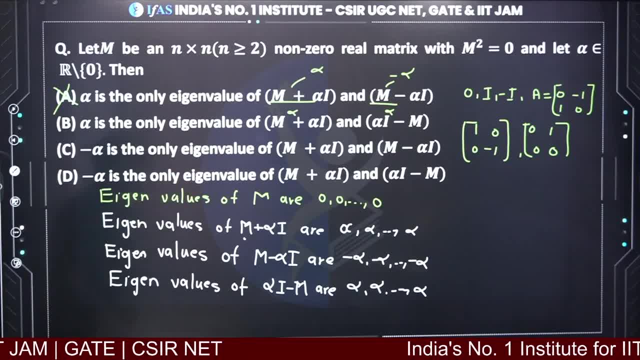 see what will be its eigenvalues. its eigenvalues will be also alpha and its eigenvalues will be also alpha. see what will be its eigenvalues. its eigenvalues will be also alpha and its eigenvalues will be also alpha. alpha is the only eigenvalue which is correct. 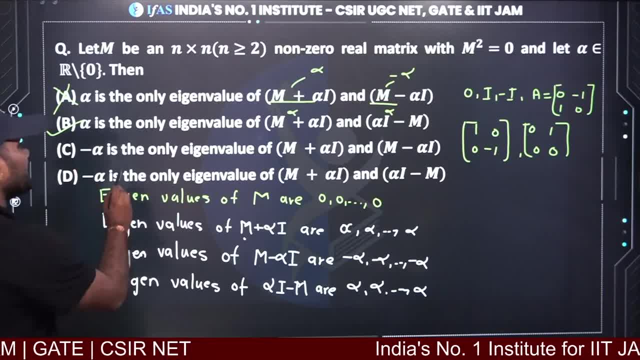 absolutely. and option C is saying that minus alpha is the only eigenvalue of its eigenvalues is alpha. but what is it saying? minus alpha is incorrect and what is its eigenvalues? alpha. but what is it saying in option? minus alpha is also incorrect. 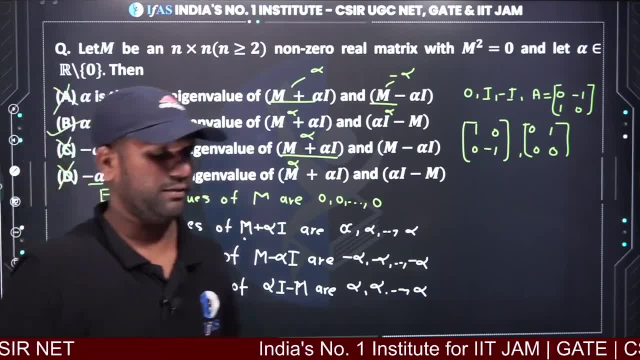 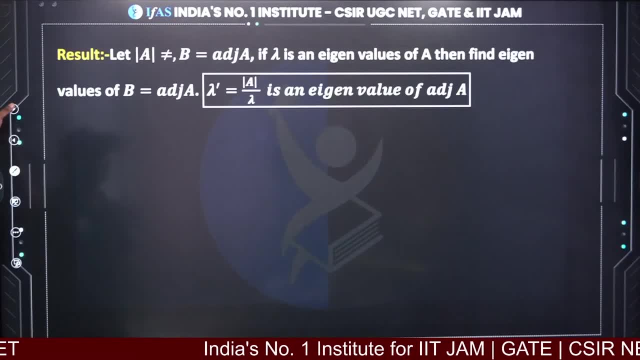 so here only one option will be correct, that is option B. is it clear? I think everyone is clear. now let's go to the next slide come. so, next question. there is a result for you guys. this result is also an important result. remember this in the exam. 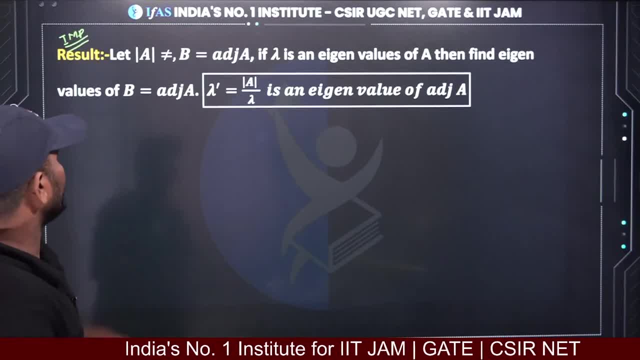 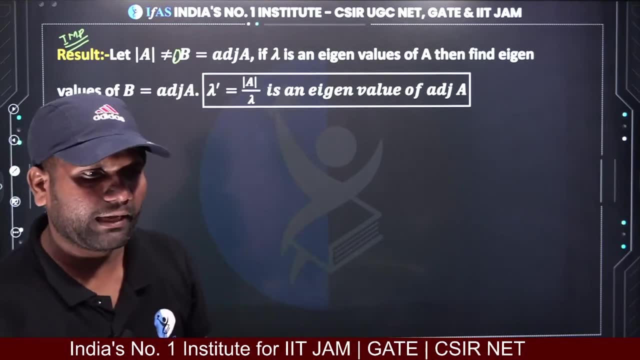 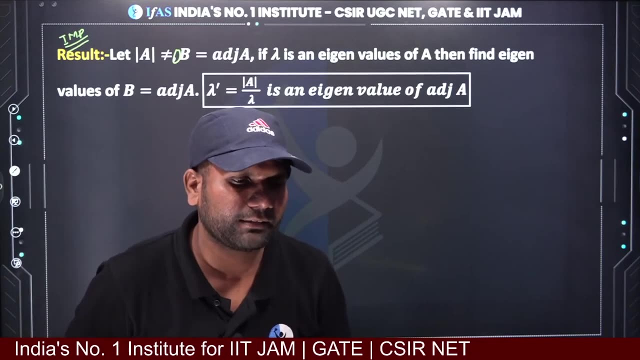 ok, what does this result say? suppose any matrix determinant is not equal to 0. here, determinant is not equal to 0 means this inverse should exist. what did we take? sorry, NKG classes. this is not idempotent. this is zero matrix. sorry, nilpotent matrix. 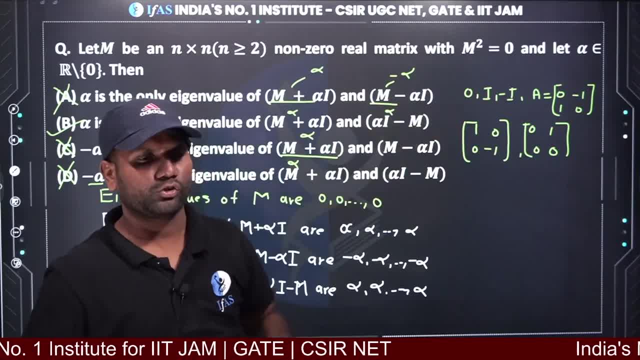 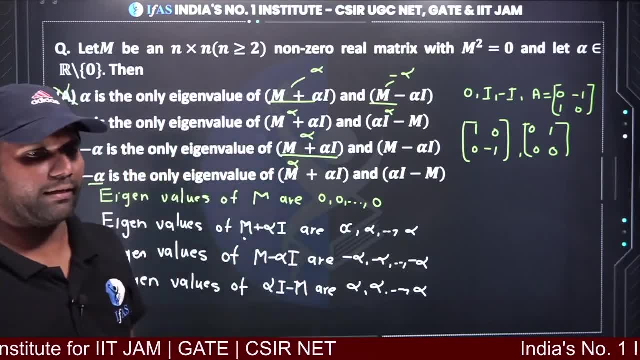 this matrix is not idempotent. sorry, this is nilpotent matrix. so all eigenvalues of nilpotent matrix are 0. ok, see this once. this is nilpotent matrix. if eigenvalues of nilpotent matrix are 0, then if eigenvalues of nilpotent matrix are 0. 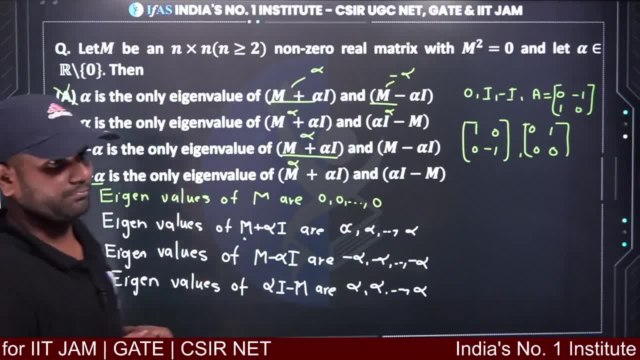 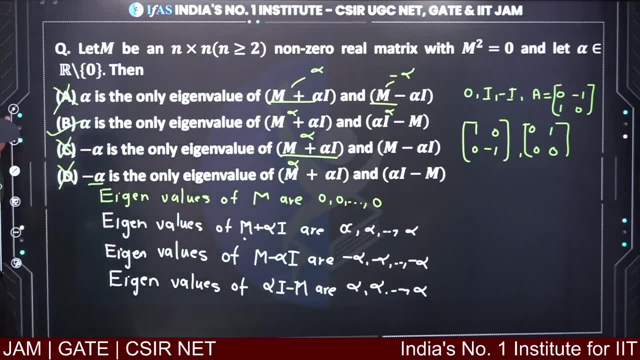 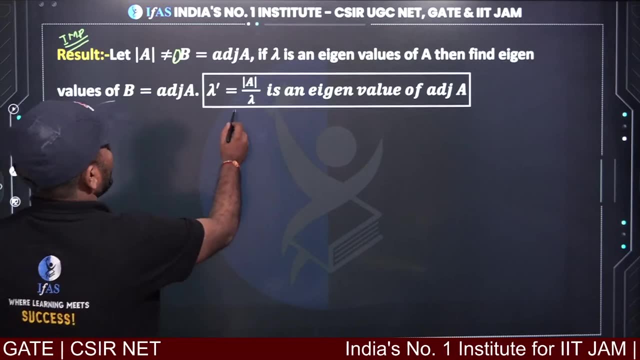 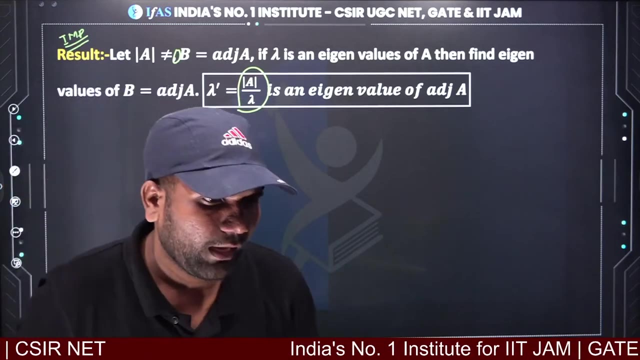 then you can easily get out of this. ok, understood, NKG classes come. so here. keep in mind: if eigenvalues of A is lambda, then the eigenvalues of adjoint of A is determinant of A by lambda. ok, ok, you asked. general eigenvalues are either: 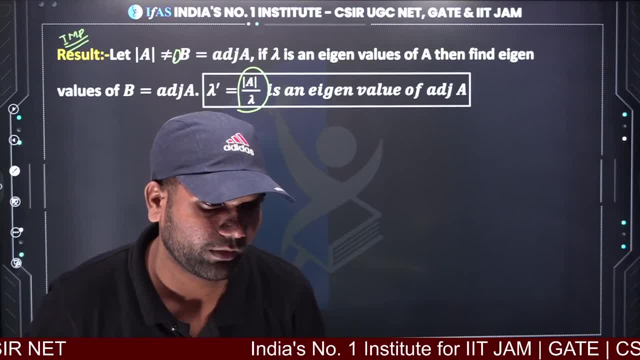 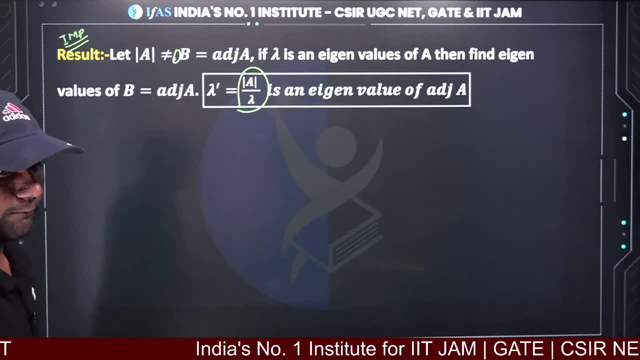 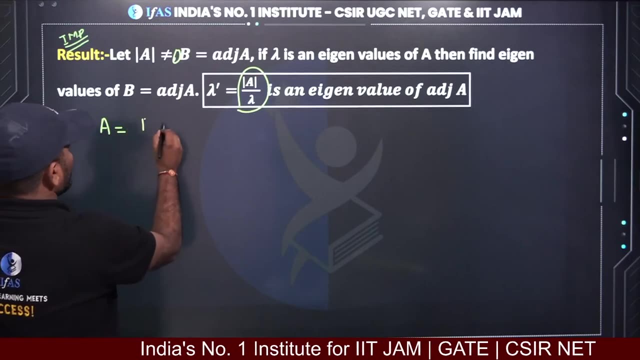 1, 0 or 1, correct in idempotent. once again write the question. NKG classes. the question is not clear. once again write here. suppose I gave you a question. a matrix is equal to 1, 2, 3 and so on, up to 1. 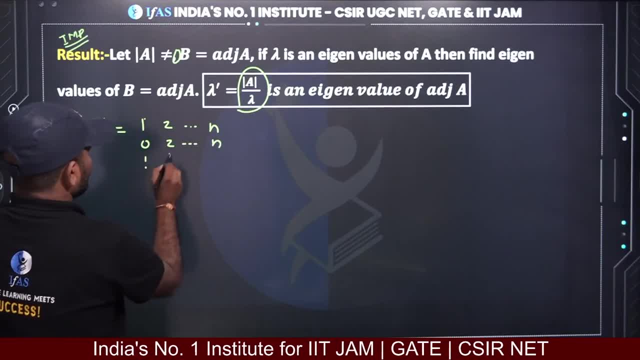 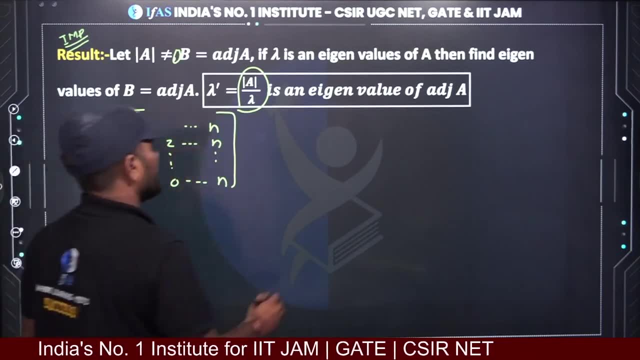 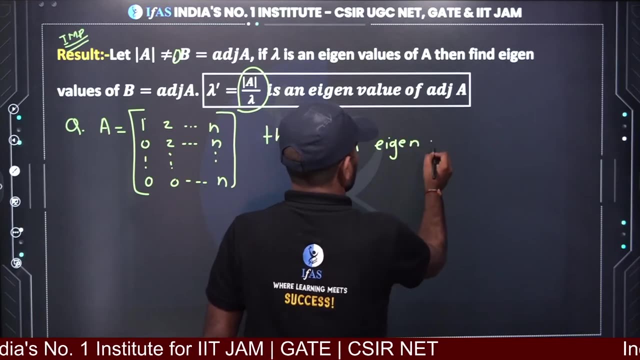 0 here. 2 and so on up to n and so on. here we took 0, 0 and so on up to n. ok, gave a matrix. then find eigenvalues of. then find eigenvalues of. then find eigenvalues of adjoint of A. now, what eigenvalues of adjoint of A. 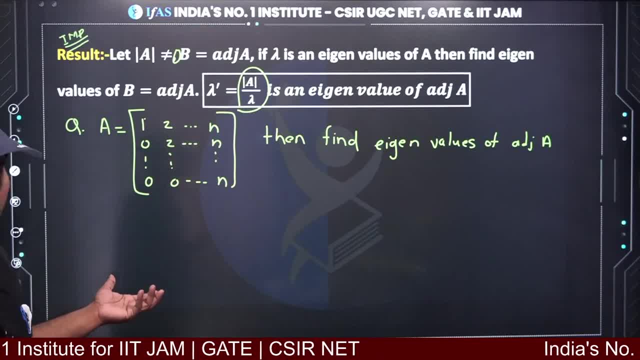 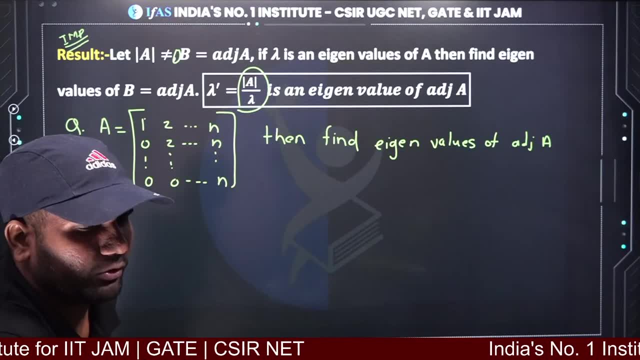 what eigenvalues of adjoint of A. let's see what eigenvalues of adjoint of A. let's see about what NKG classes I am talking about. I am not able to understand. 1 0 first row. 0, 0 second row. I am not able to understand what you are saying. 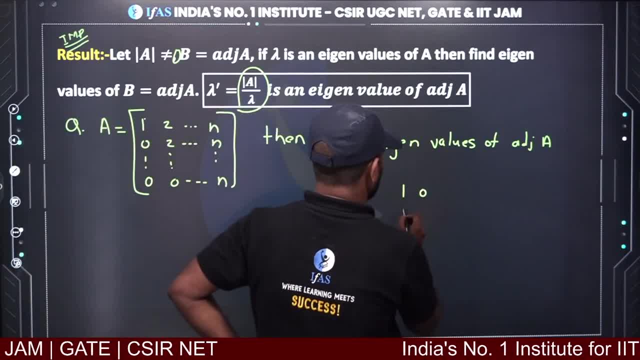 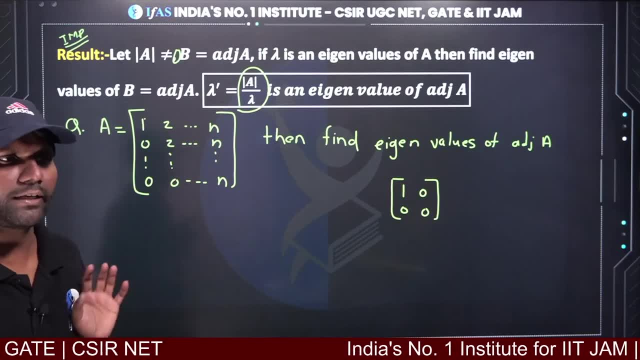 what you are saying is that you have taken a matrix: 0 0- 0. if you have taken such a matrix, then its Eigen value will be 1 and 0. if you want to say this, if you are saying this, then you are saying absolutely right. 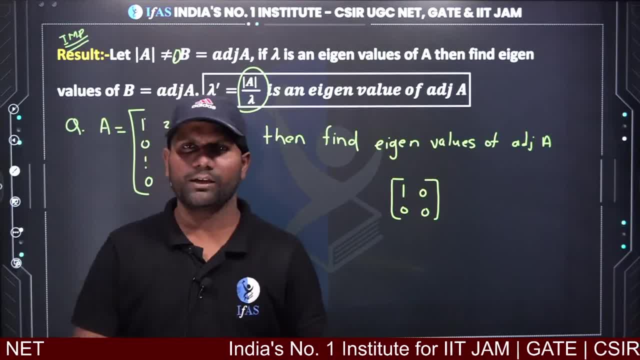 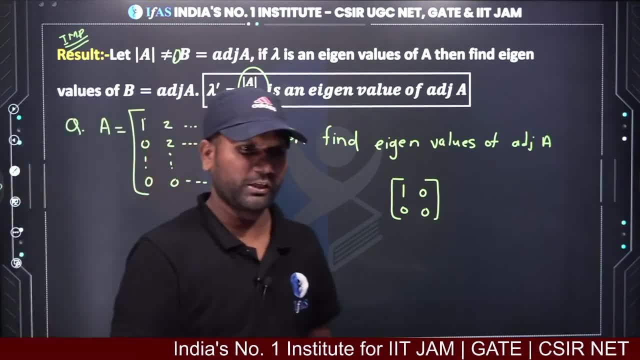 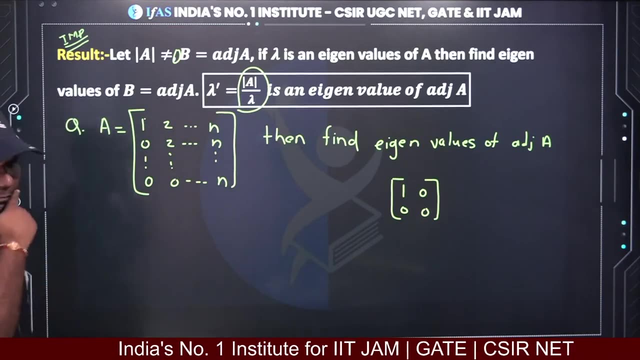 yes, absolutely, Vizhendra. if you have, it is important for IIT jam. we will read the whole jam. it is in the syllabus of jam. from here, you will be able to practice some questions, absolutely ok. ok, now tell me what will be its answer. 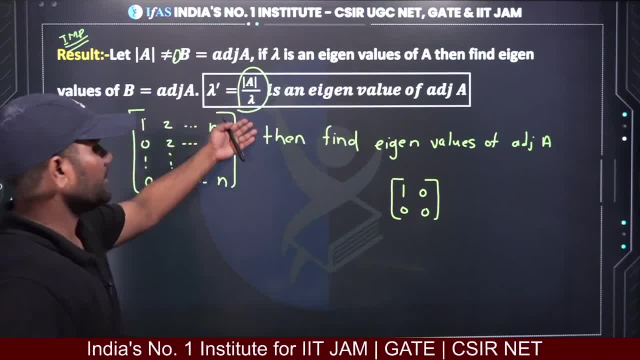 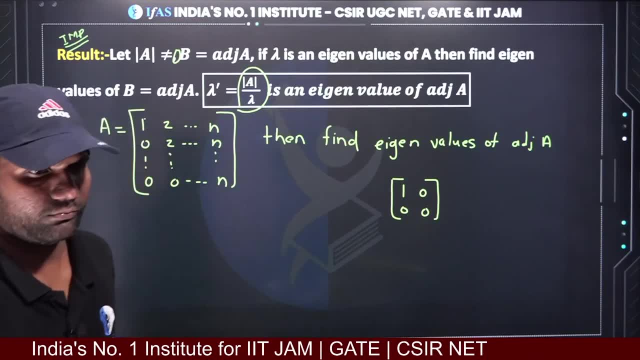 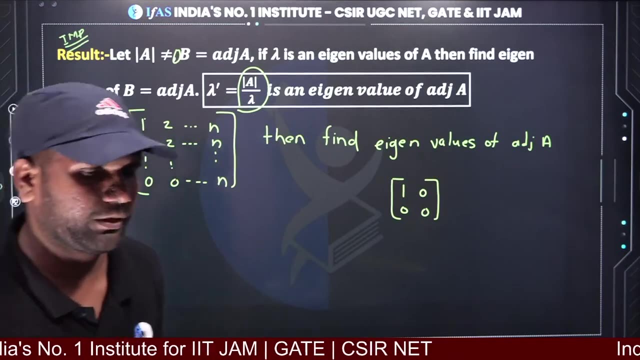 Vizhendra, you tell it is a simple question. apply A result. clearly you can tell what will be its answer: it will be idempotent. when A square will be equal to 1 means it is idempotent matrix, absolutely correct. ok, now see what is A's eigenvalues. 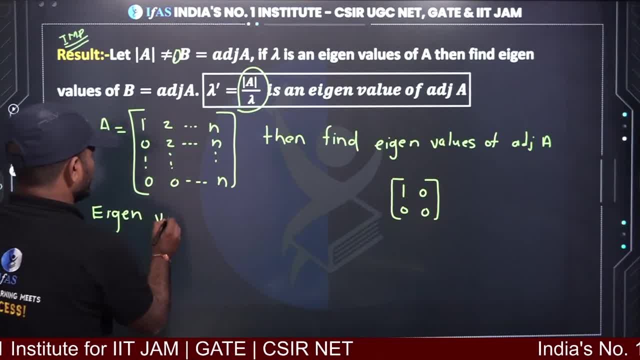 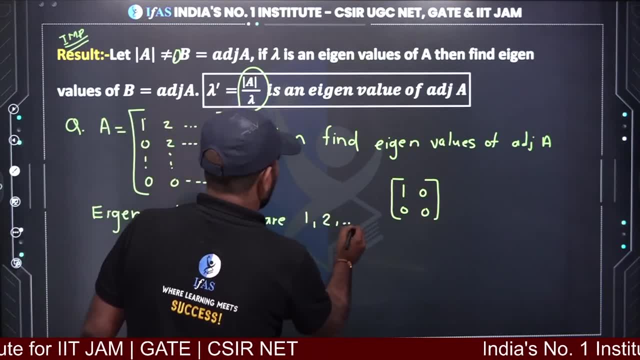 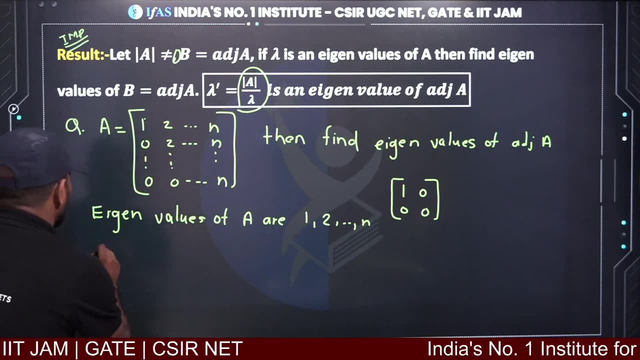 eigenvalues of A. if you will see eigenvalues of A, what is A's eigenvalues? you will see A's eigenvalues 1,2 and so on and will be seen. ok, now A's eigenvalues are there? now talk here. what will be the eigenvalues of adjoint of A? 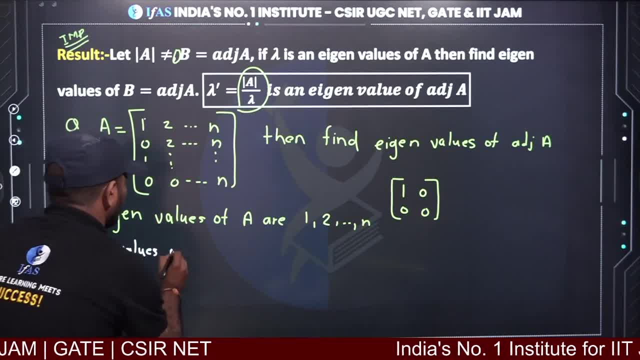 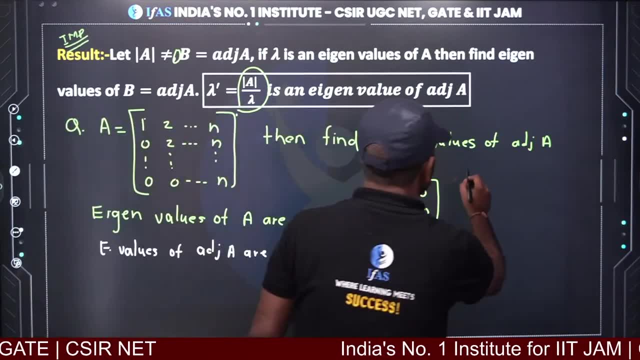 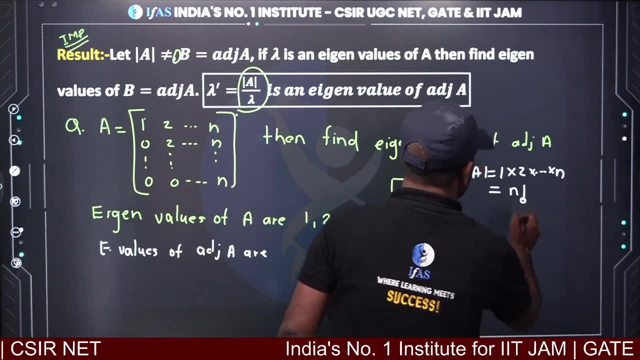 so, eigenvalues of eigenvalues of adjoint of A, what will be the eigenvalues of adjoint of A? look, what is this determinant of A, so what is its determinant determinant? 1 x, 2, x, n, so on. what is n? and one is equal to n factorial. 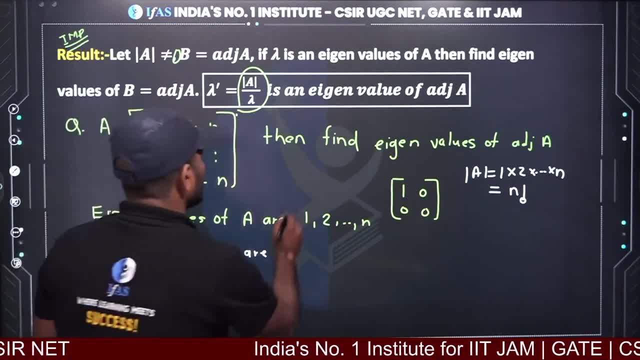 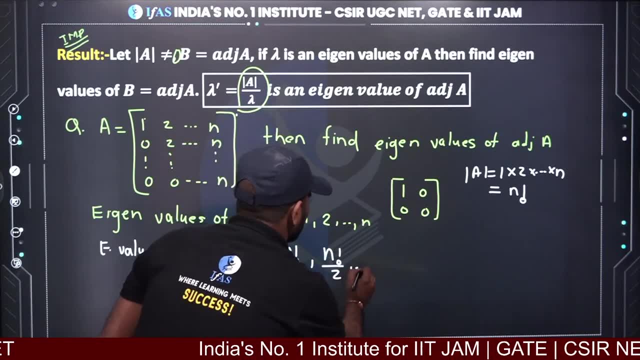 so its determinant. you have got n factorial, so what will be this determinant? n factorial by lambda. keep the value of lambda as 1. keep the value of lambda as 2. similarly, keep the value of lambda as the eigenvalues. so So you got the eigenvalue of this. 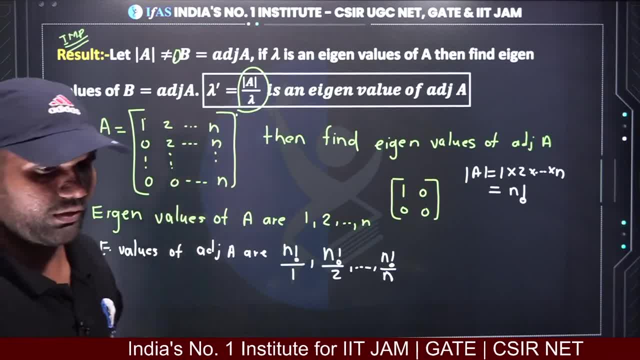 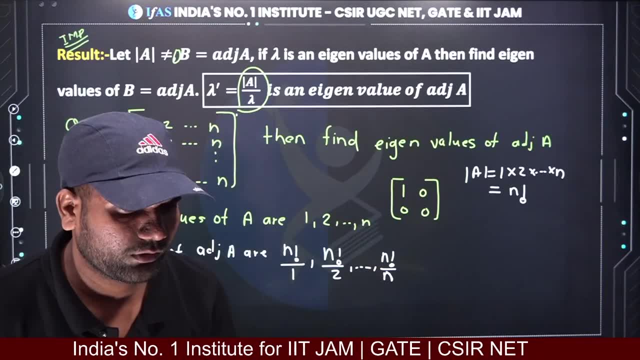 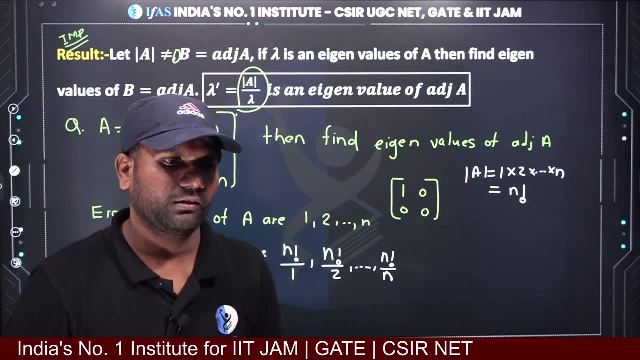 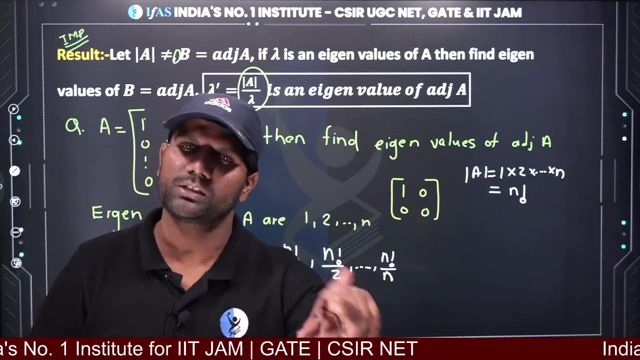 Okay, see Clear. Yes, Let's go. No, NKG classes are not like that. What they mean to say is that either it will be 0 or 1, or both will happen. there is no problem. It is not that only one of the two will happen. 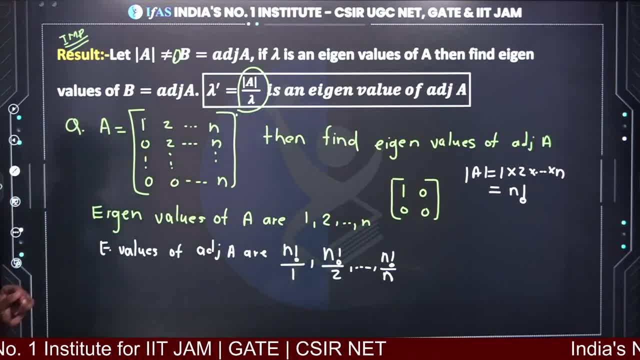 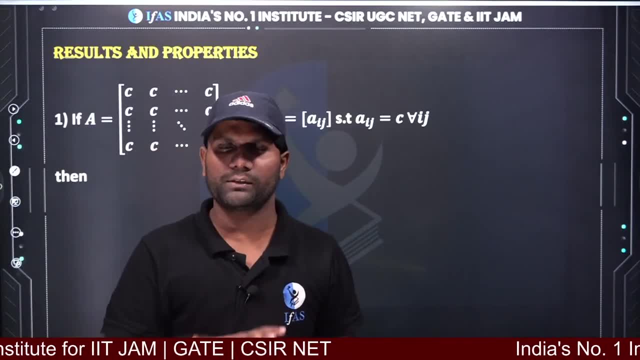 It does not happen. Okay, Let's go Now. let's go to the next slide. Now some important results are for you people. You know about the constant matrix. A is given to you as a constant matrix. If you look at the PYQ in the exam, then questions have also been asked on it in the exam. 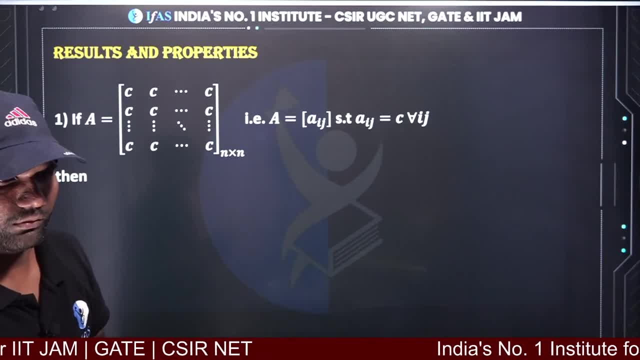 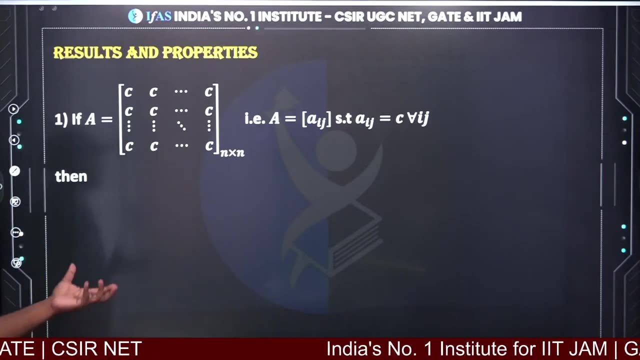 Okay, Okay. So here, suppose you are given a characteristic, a constant matrix. So about this you have to know all the things about it. I am giving it to you by writing Before going to the exam. you should know that the characteristic polynomial of this type of matrix 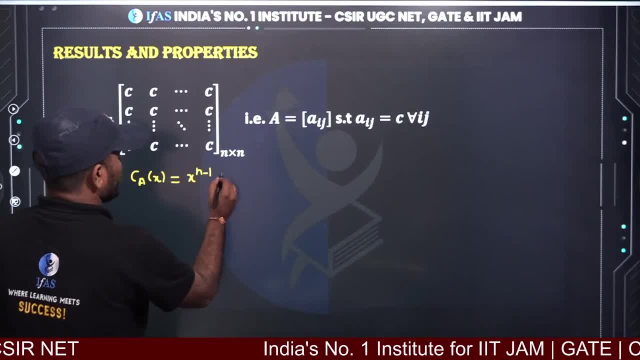 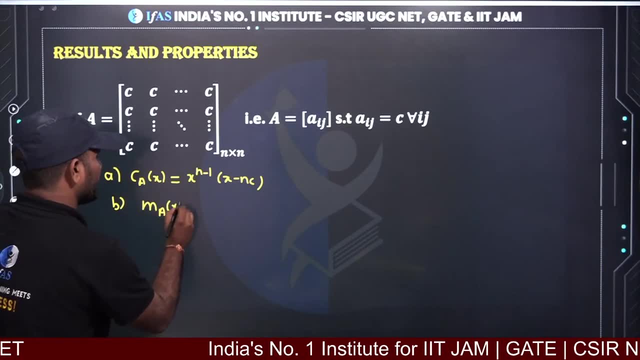 what will be its characteristic polynomial? x raised to n minus 1, x minus nc will be, If I talk here, its minimal polynomial. So minimal polynomial of constant matrix is x, x minus nc, And constant matrix is always diagonalizable. 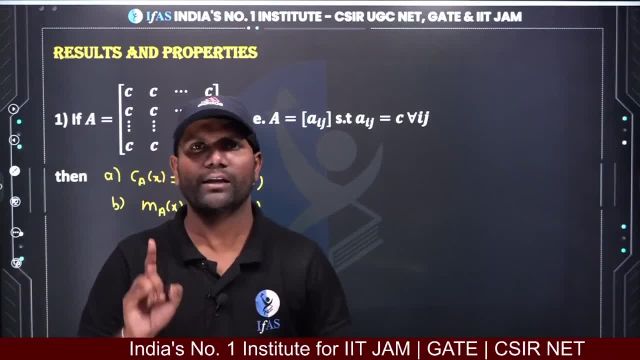 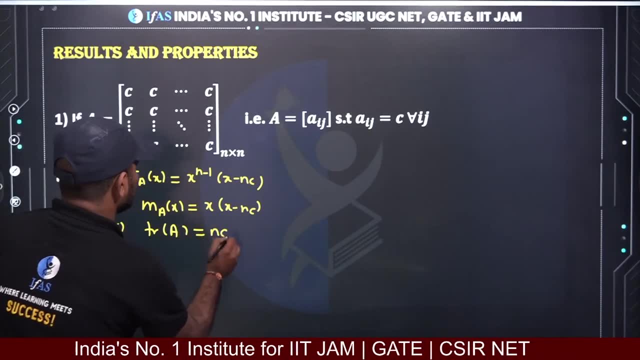 You have to keep this in mind too. Constant matrix is always diagonalizable. Okay, And take the third here. What will be its trace? What will be the trace of A? It will be nc, Option D, If I talk. what will be its rank? 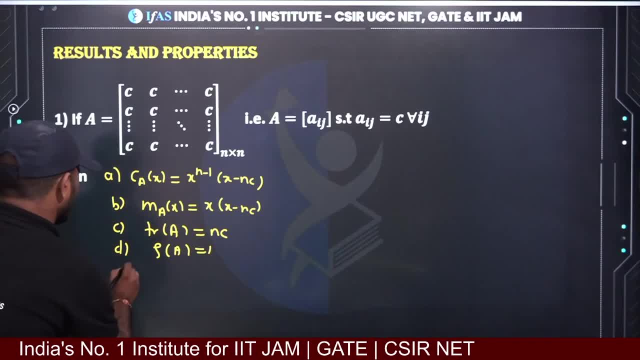 Its rank will be 1.. Determinant will obviously be 0.. What will be the determinant of A? You will get the determinant of A as 0.. And remember one more thing here: Result number F, A is diagonalizable. Constant matrix is always diagonalizable. 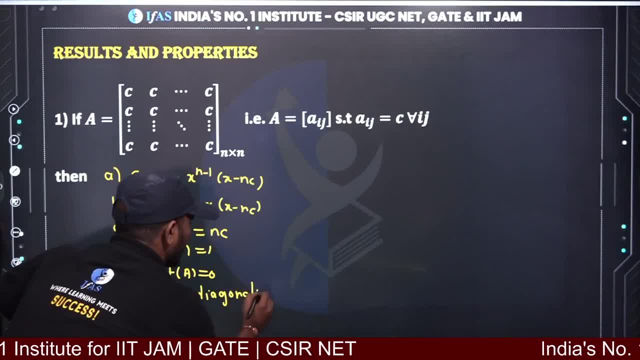 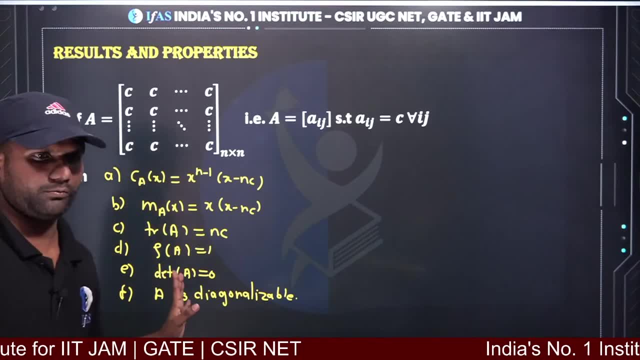 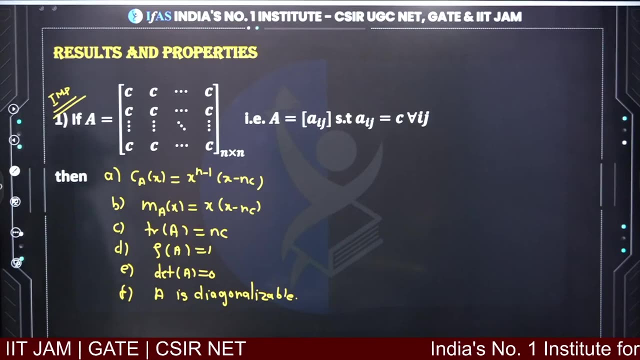 Okay, It will always be diagonalizable. This is some important result. You should know it before going to exam. Yes, absolutely Okay. Come on, Is it clear to everyone? This is important result. Okay, Look at this. Yes, it will be rank 1.. 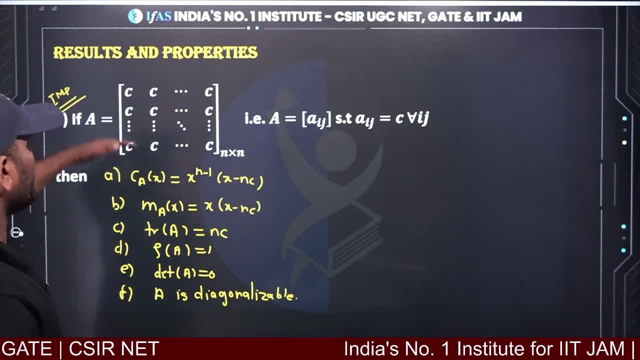 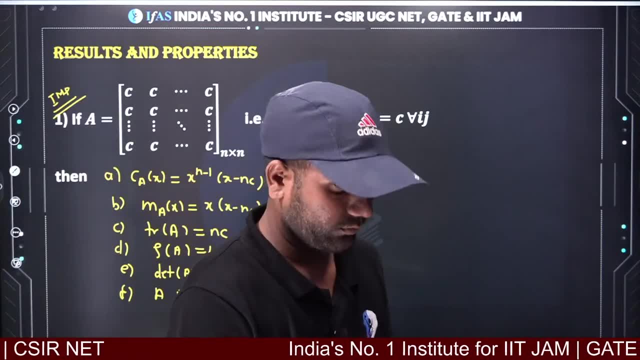 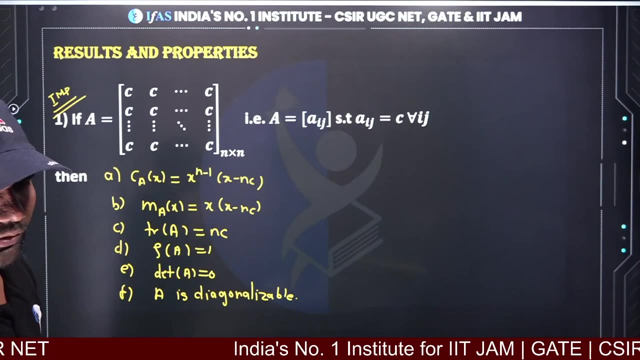 Absolutely, See, it will be rank 1.. See, all the rows have become the same, So we can do zero. Okay, Yes, absolutely. Look at this. See, the rows are the same. Let's go. What is the doubt about NKG classes? 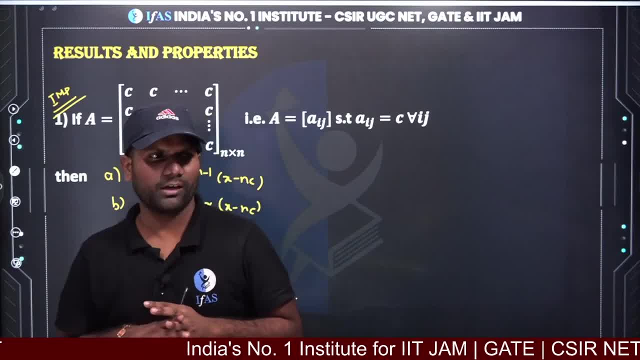 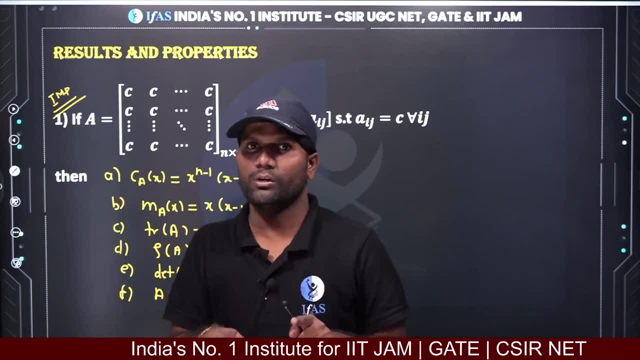 Look at the eigenvalues of the idempotent matrix. Either it will be 0 or 1. It is not that only 0 or 1 will be possible. Both are also possible. As you have found an example, It means that any of 0 and 1 can be possible. 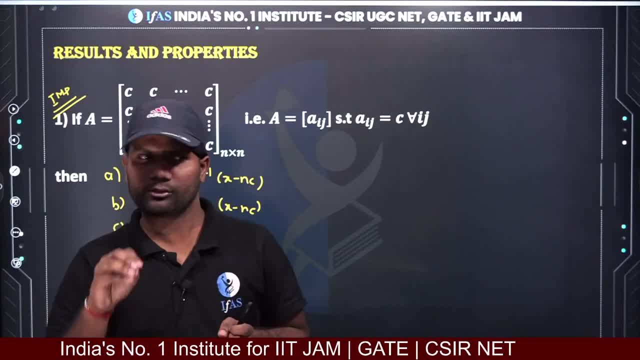 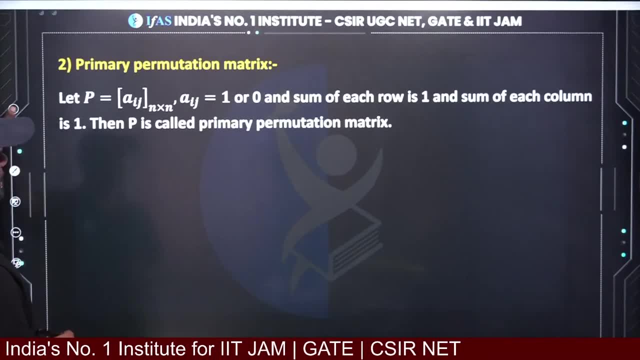 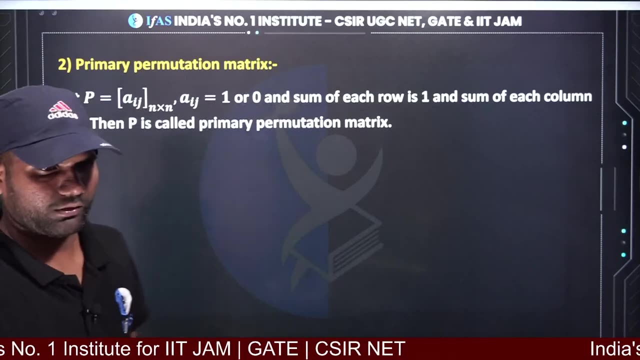 Both are also possible, Or only 1 can be possible, Or 0 can also be possible. Now here I am thinking. I will tell you about some permutation matrix, Because permutation is also a favorite topic in the exam. What is permutation matrix? Permutation matrix is such a matrix. 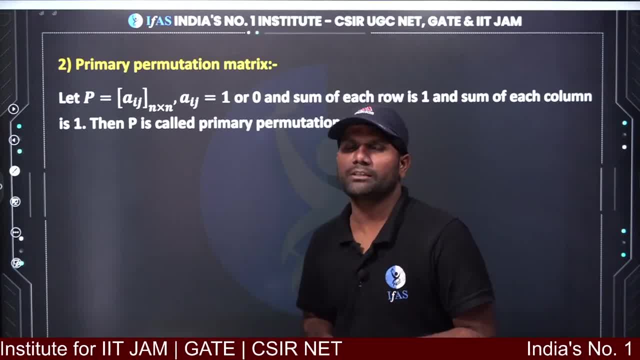 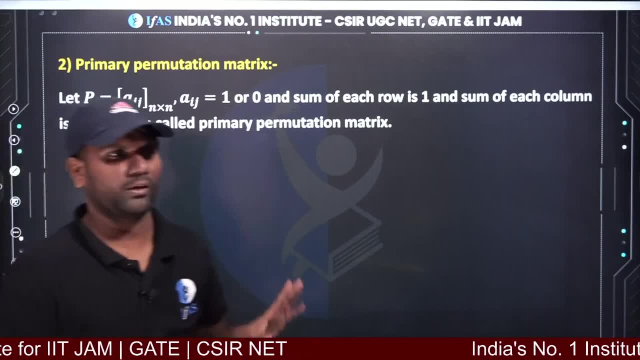 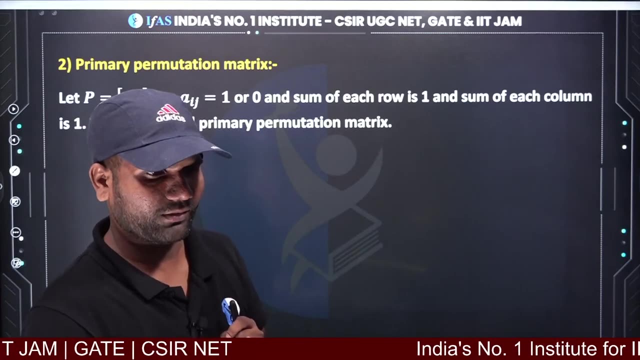 Where the sum of each row, Or talk about the sum of each column. Get 1 And remember What will be the entries of it. Either it will be 0 or 1. What are you going to use? the entries 0 and 1? Yes, Amit, I told them the same. 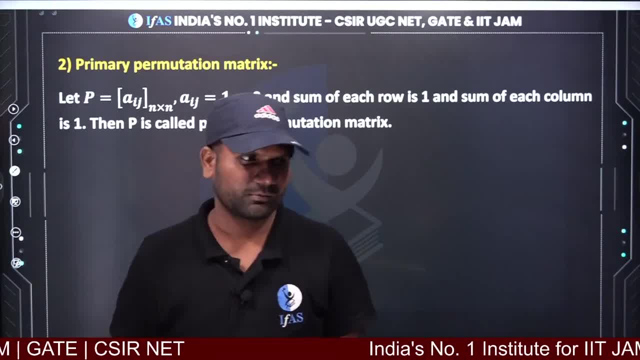 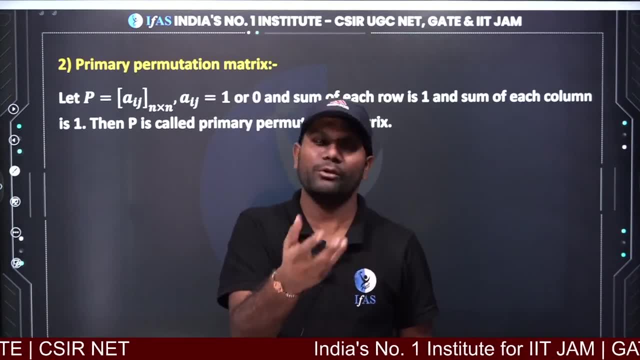 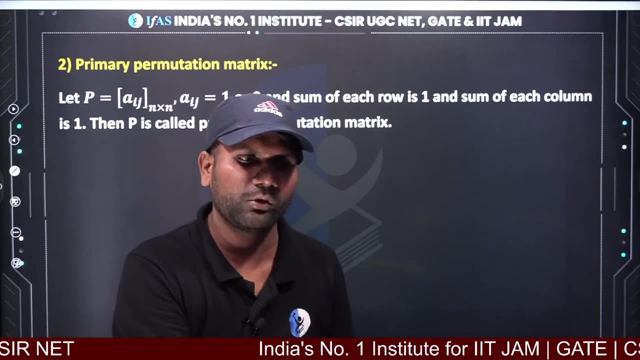 Ok, Ok. The meaning of OR is not only this. Look at it. there is either Either A or both. It is not necessary that only 0 will be available Or only 1 will be available. Both are possible. You have seen the example in front of you. 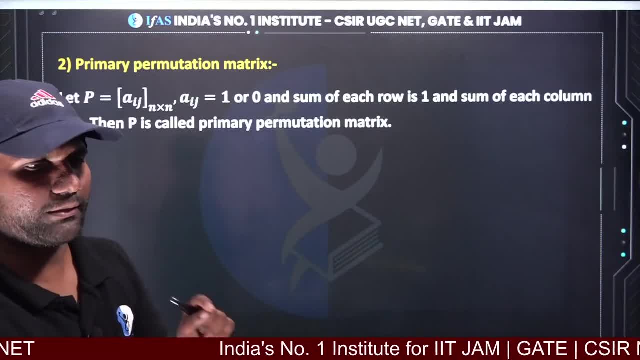 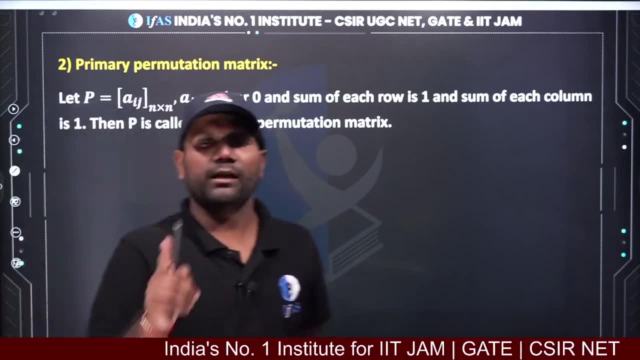 Right. For which exam are you preparing the NKG classes? Are you a Jain student or a Net student? Ok, So such a matrix Where the sum of each row, The sum of each column, is 1 And its entry is either 0 or 1. 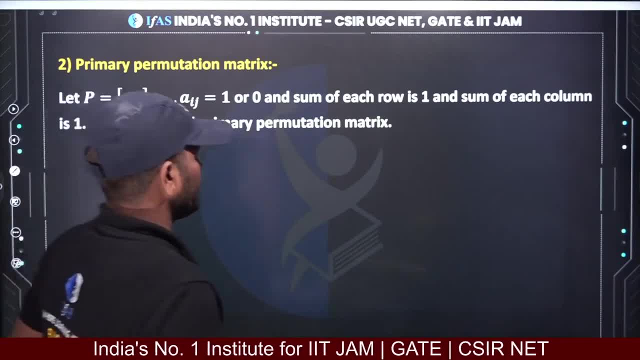 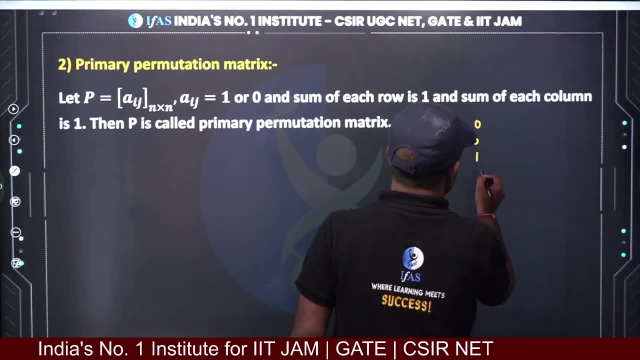 What do we call it? We call it permutation matrix. For example, as I gave you a matrix: 0, 1 0 0 0 0 0, 1 0 0 0, 1 0 0 0, 1 0 0 0 0 0 0. 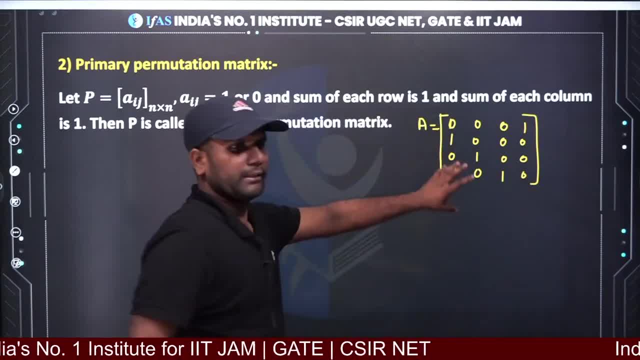 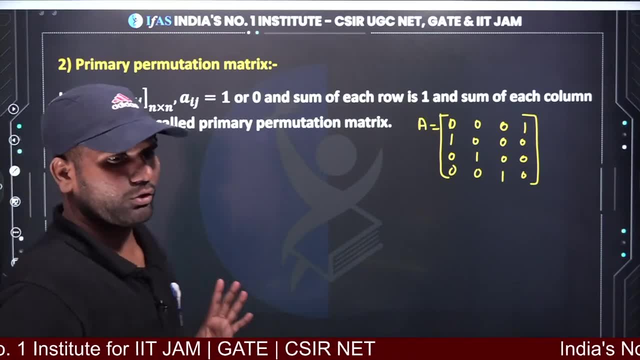 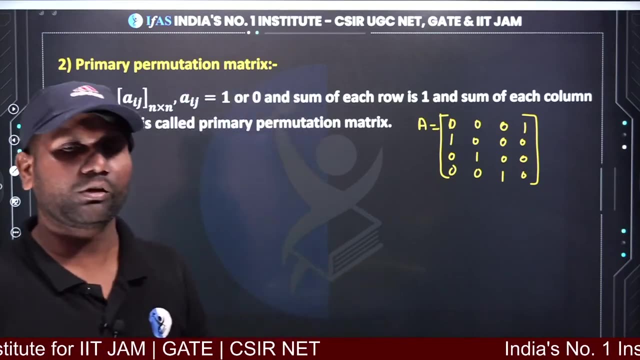 You are seeing this matrix. Add any row or column of this matrix. You will always get 1 Right For net, ok. ok, Don't get confused. The eigenvalues of an idempotent matrix Can be anything between 0 and 1, Ok, And can be anything between 1 and 1 of the involuntary. 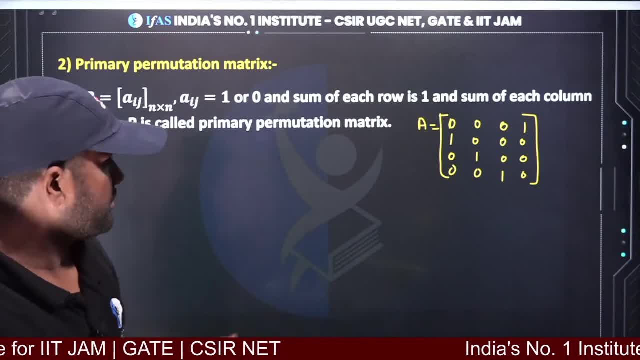 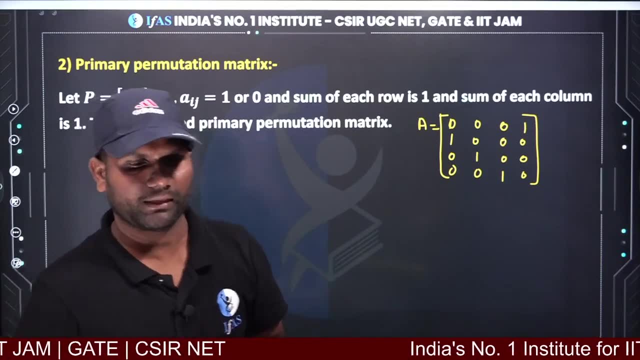 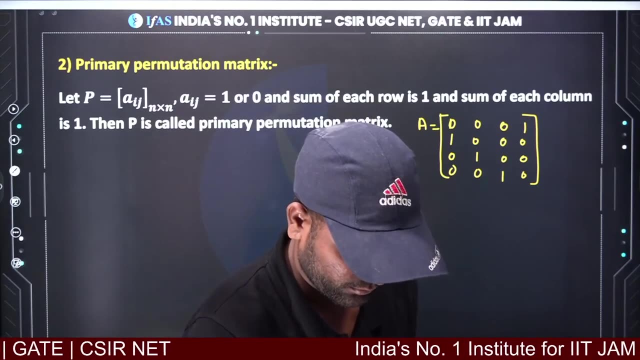 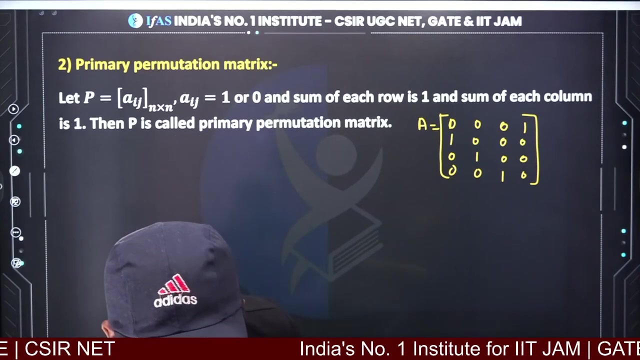 It is not that there will be only one. Ok, Now see this type of matrix. What do we call it? We call it permutation matrix, And here you also get a permutation. You must have seen permutation. Here you also get a permutation. Good morning, Apoorva. Ok. 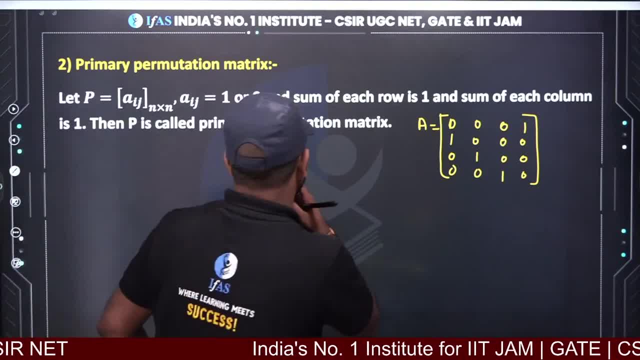 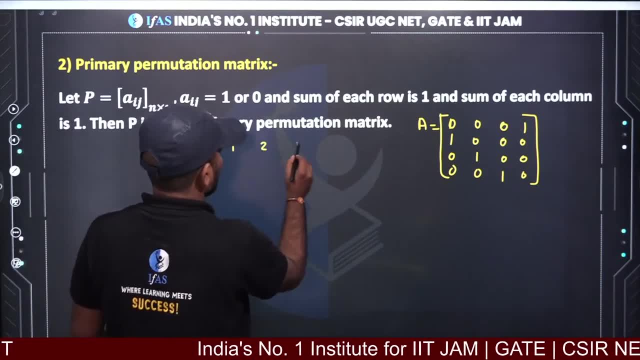 Yes, both are possible. Now come here, See If here we get a sigma, Like if you write it in the form of permutation, There are 4 symbols: 1, 2, 3, 4. So who went to 1? 1 goes to 2, 2 goes to 3. 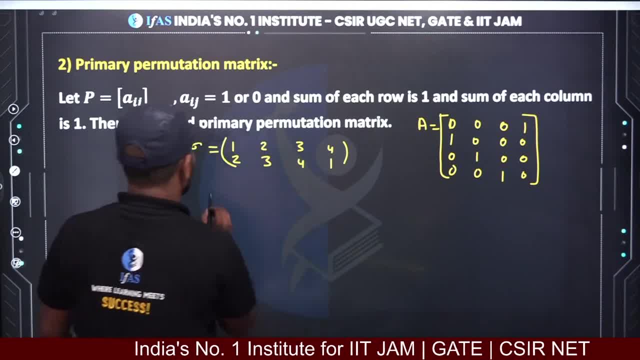 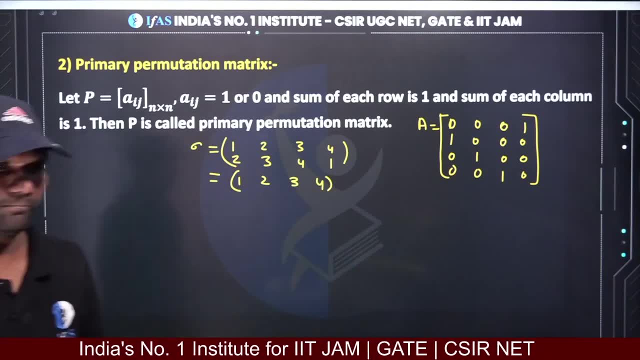 3 goes to 4 And 4 goes to 1. So here permutation: 1 goes to 2, 2 goes to 3, 3 goes to 4, 4 goes to 1. You got permutation, Ok. So this type of matrix, We call it permutation matrix. 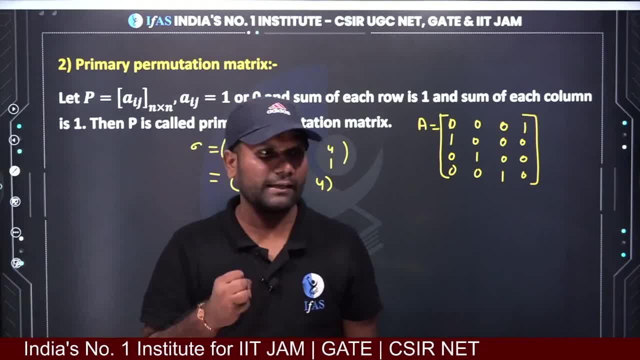 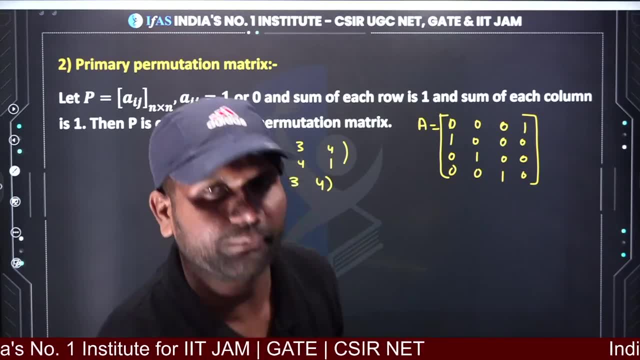 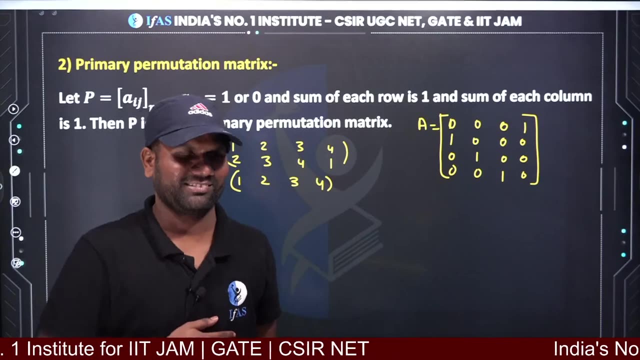 Cycle decomposition. Everyone knows Cycle decomposition. If we divide permutation By 2, If we write permutation In the form of disjoint cycle, So when we write the length of each cycle In set, In multi set, What do we call it Cycle decomposition? Tell me once. Thank you, Apoorva. 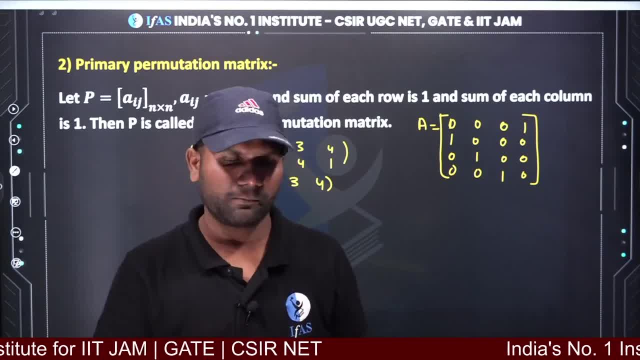 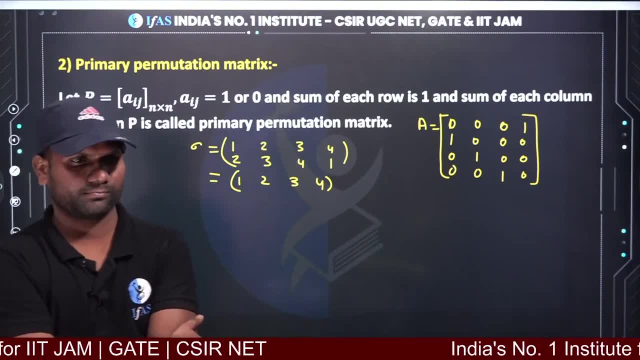 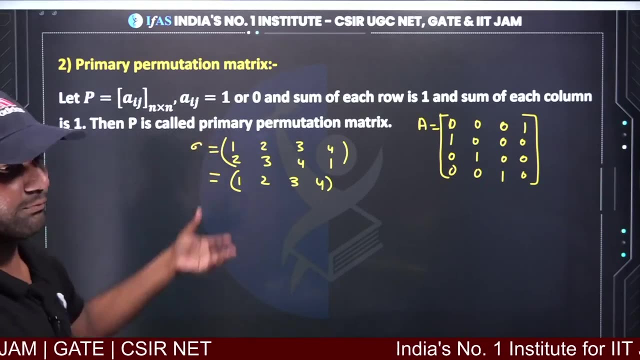 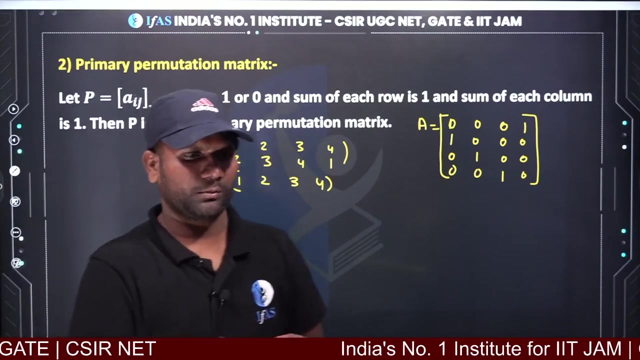 Tell me once: Is cycle decomposition clear to you? Do you know cycle decomposition? If you know cycle decomposition, Then the result will be very easy for you. Pooja Pooja, Have you studied permutation in group theory? Tell me once If you know permutation. 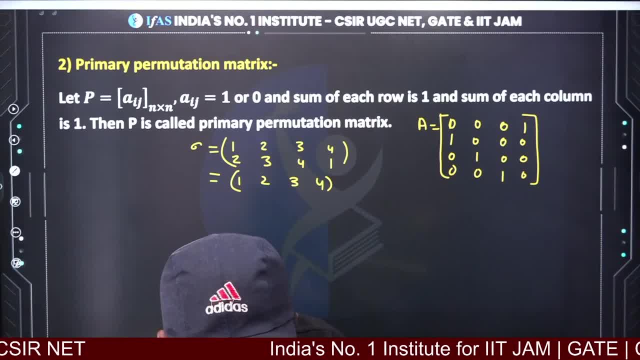 Then only you will be able to do it. Do you know there is a permutation Which you can do in group theory? If you know, you will be able to do it easily. Go When you study group theory. Do you know there is a permutation Which is鉛. 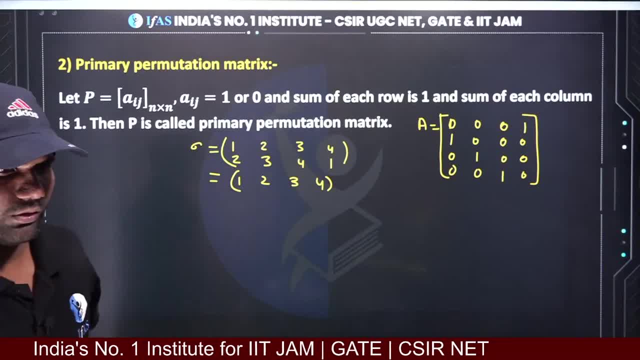 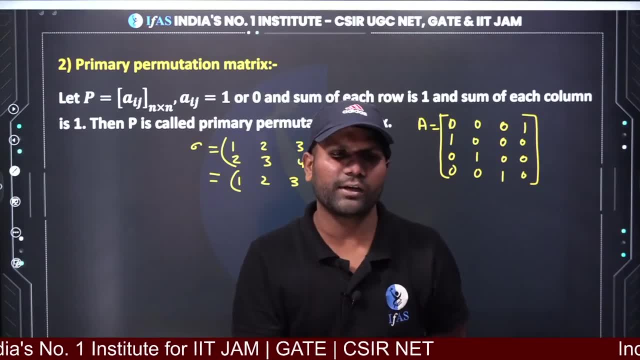 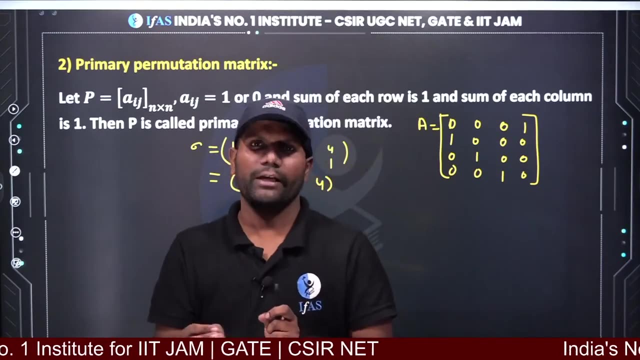 Podcast. let me tell you once what is the meaning of cycle decomposition. when you write any permutation in the form of design cycle, then the length of the cycle. if you write the length in increasing order, including cycle of length 1, what do we call it? permutation? CD is called. 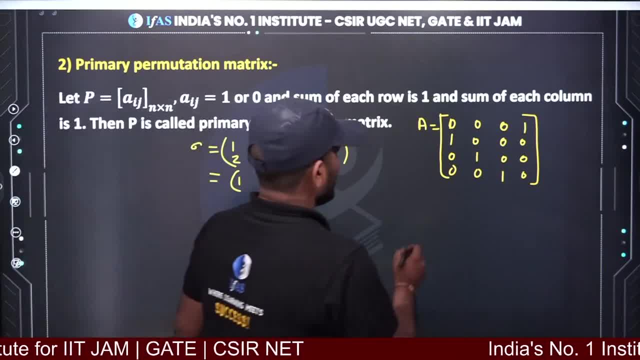 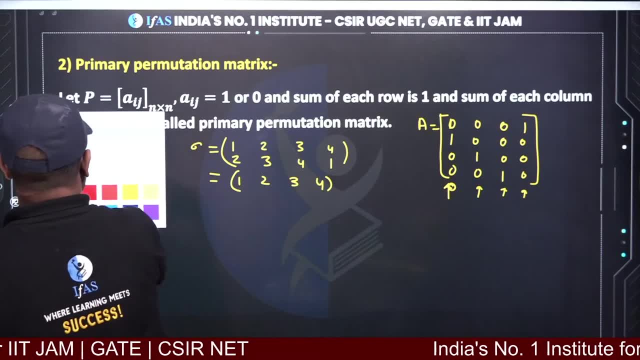 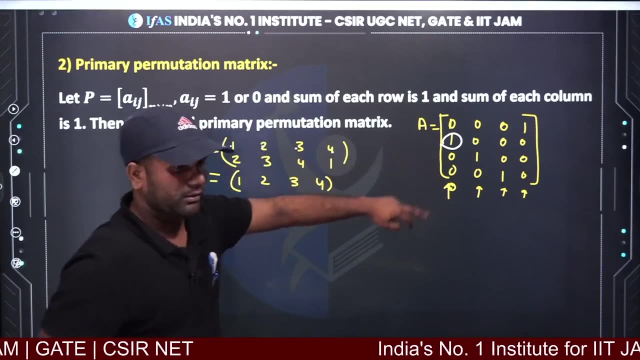 Pooja says: how did you write for matrix Pooja? see here, the first column is second column. the third column is fourth column. the entry of the first column goes to second column 1,2,3,4. I have written like this: first column is on second column. 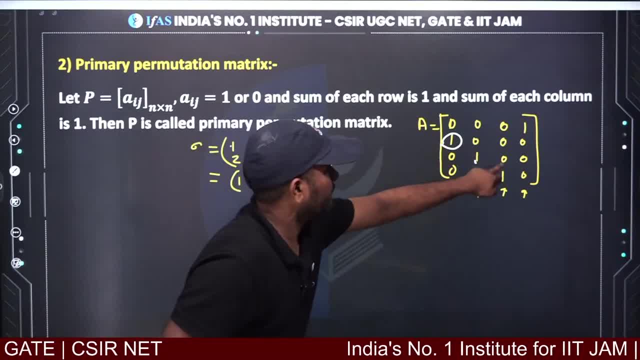 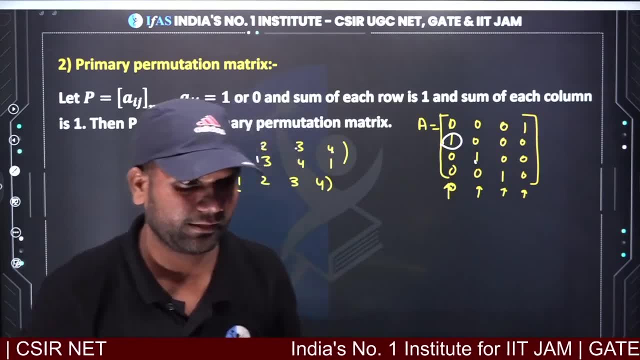 second column is on third column, so 2 goes to 3 and third column is on fourth column means 3 goes to 4 and on fourth column 1 is on top means 4 goes to 1. see from column. ok, yes, I was talking about matrix only. 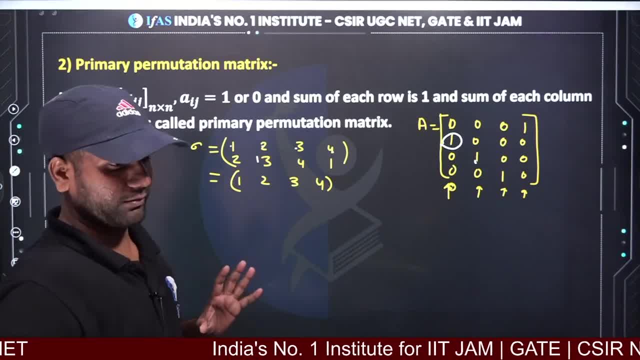 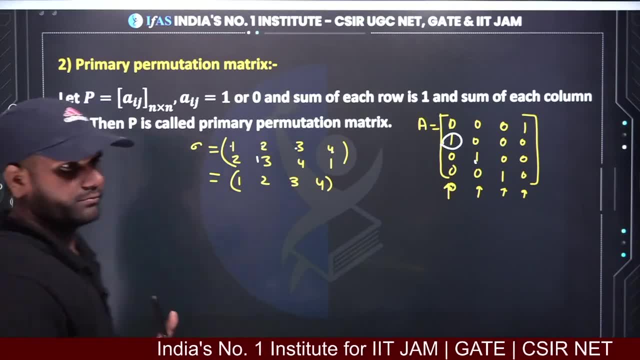 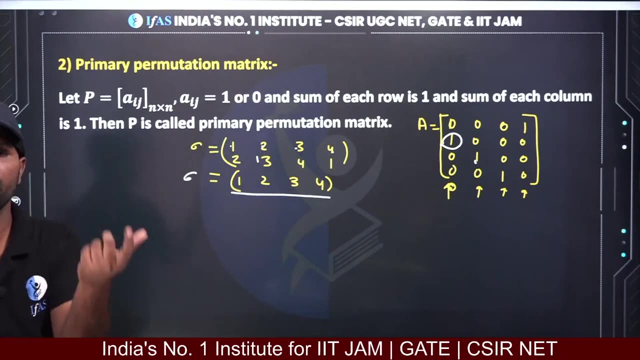 ok, that's why I wrote like this in matrix. did you understand now? did everyone understand now? see here, there is only one cycle in sigma. now what is its length? what is the length of this cycle? its length is 4. its cycle decomposition will be 4. 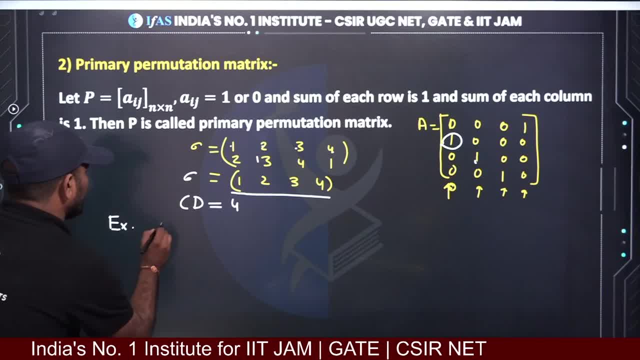 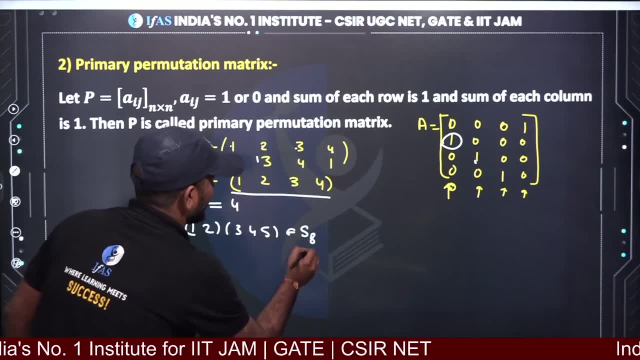 now let's take one more example. suppose I gave you a sigma. what is sigma 1,2,3,4,5 belongs to s8, so what will be its cycle decomposition? what will be the cycle decomposition of this permutation? tell me once you people. 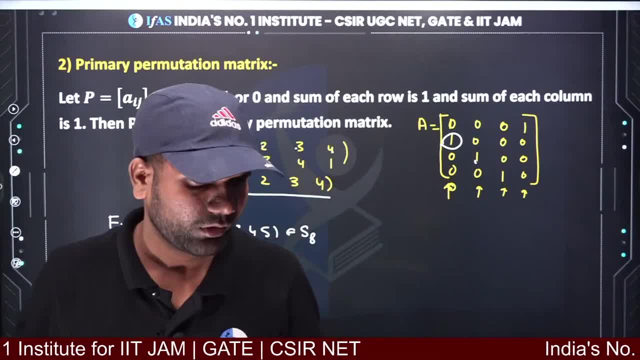 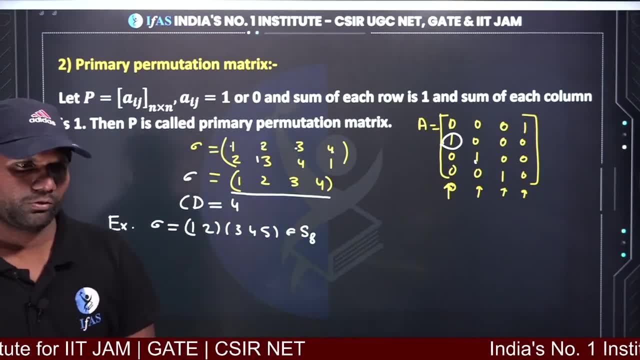 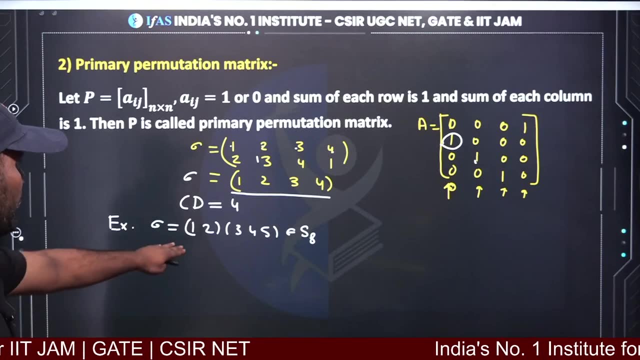 what can you say about this permutation? yes, you can do it from row and column. normally we do it from column only, so do it from column also. if you do it from row also, then there will be no sin. you will get correct answer. ok, now see what will be its cycle: decomposition. 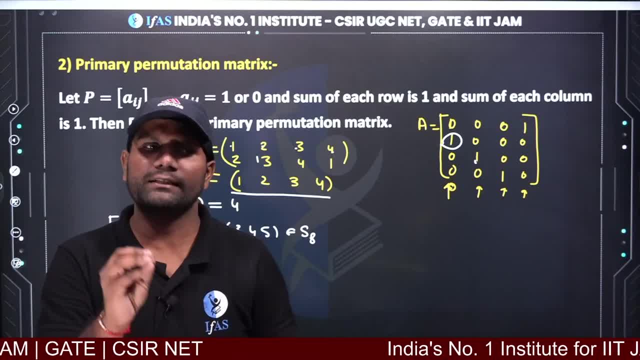 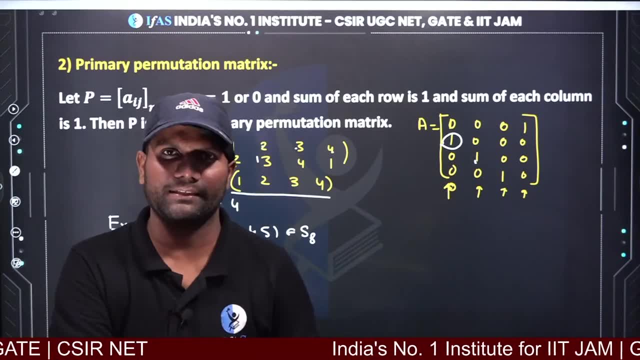 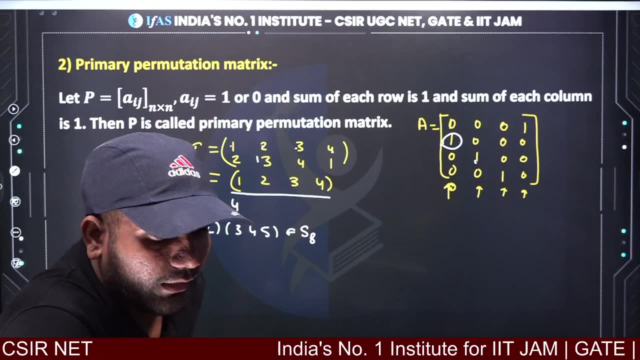 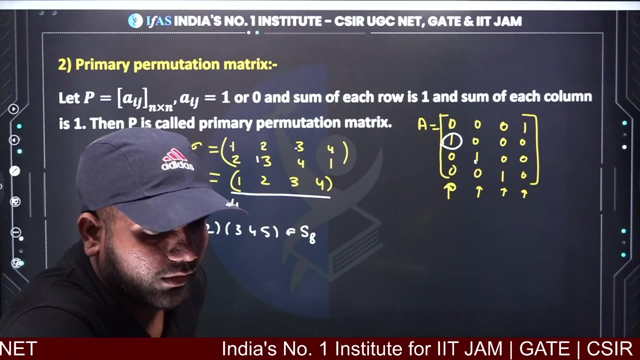 cycle. decomposition means write any permutation in the form of disjoint cycle. then, whatever is its length, write length in increasing order. set means multi set. elements are repeated in multi set. sir, if the sum of any row is 2 of any matrix, then in matrix, in matrix, you can write the sum of row 2. 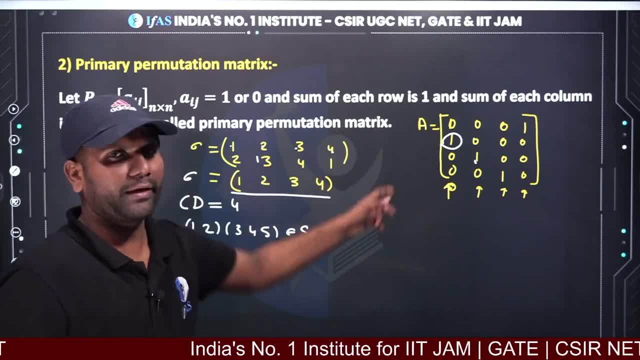 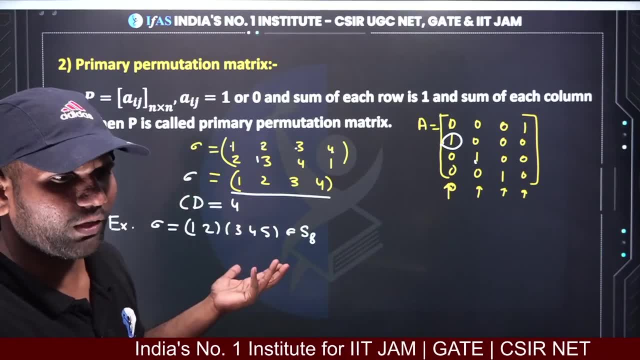 no, no, in nkg classes. here we need the sum of matrix as 1, not 2. it should be 1. only sheetal is saying it will be 6. what are you people doing? I am not asking the order of this. I am not asking the order. 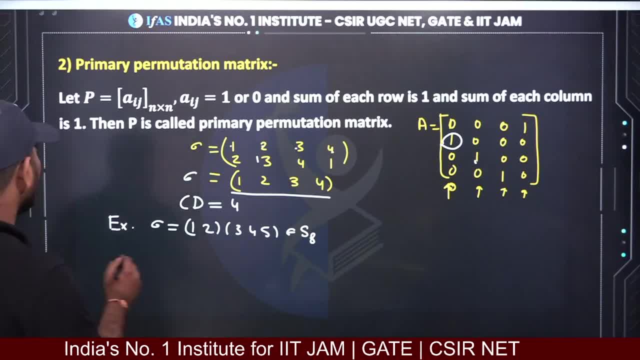 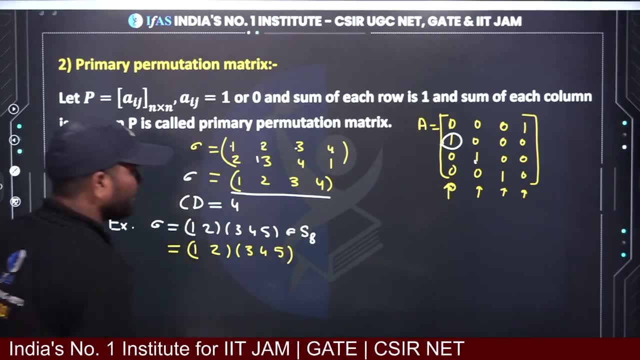 I am asking the cycle decomposition. see what is this. what are you people doing today? see what is this: 1,2. what is this 3,4,5? now see here in which it belongs. it belongs to s8, right, if it belongs to s8. 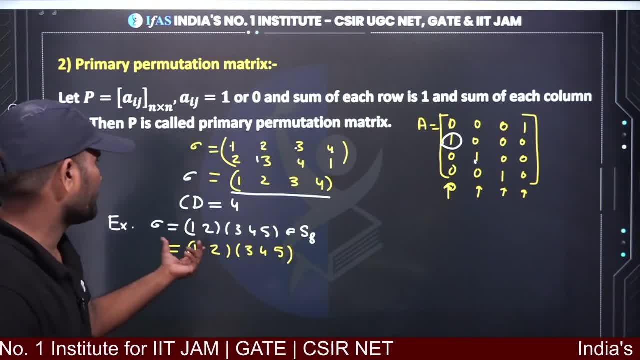 then there should be 8 symbols in it. there should be 8 elements. how many do we see? only 5 are visible. 3 are not visible. it means they will be mapped on themselves. that's why they are not visible. they will be mapped on themselves. 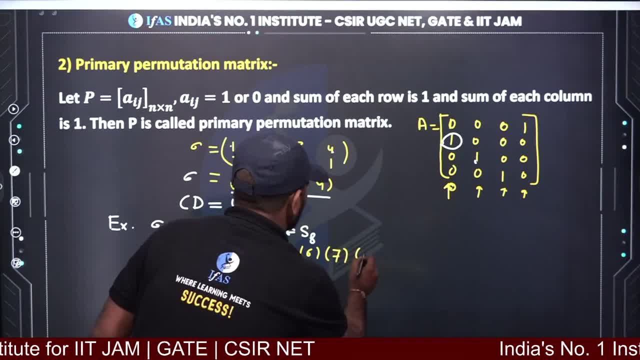 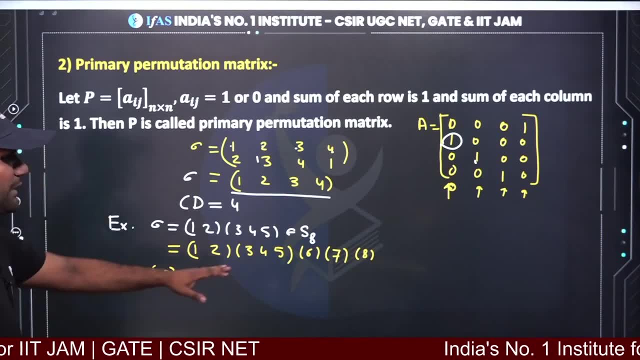 it means 6 goes to 6, 7 goes to 7, 8 goes to 8. this is your permutation. now what is the meaning of finding its length? cycle decomposition means length. see the length of the cycle. you have to write in increasing order its length. 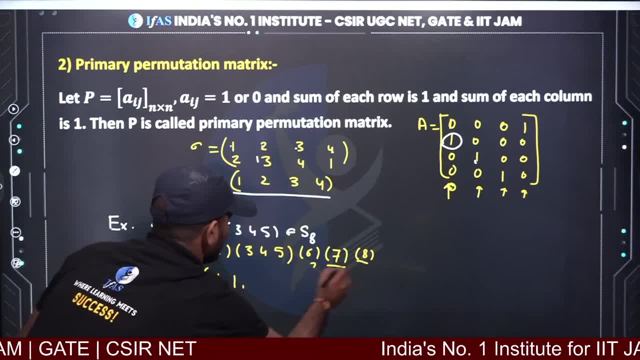 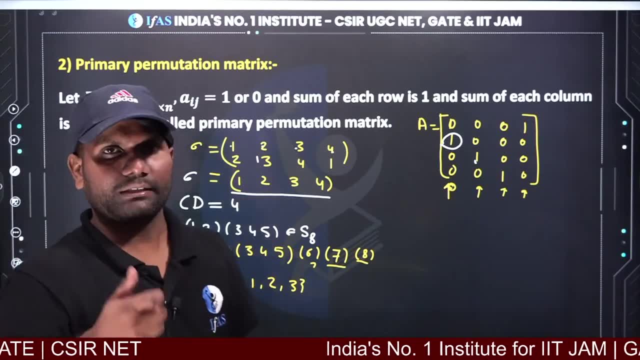 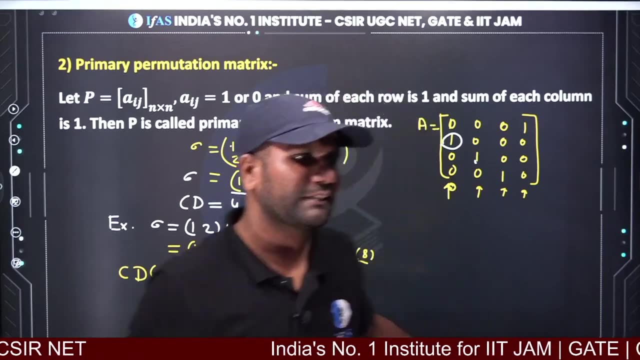 1. the length of the one next to it. its length 1. its length 1, here 2 and here 3. this is its cycle. decomposition means write permutation in disjoint cycle form and after that write the length in increasing order. this is what we call its cycle decomposition. 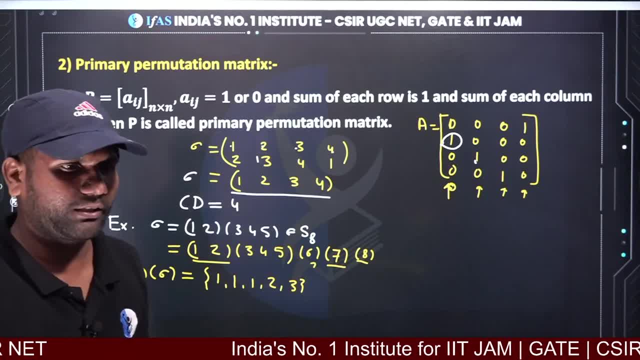 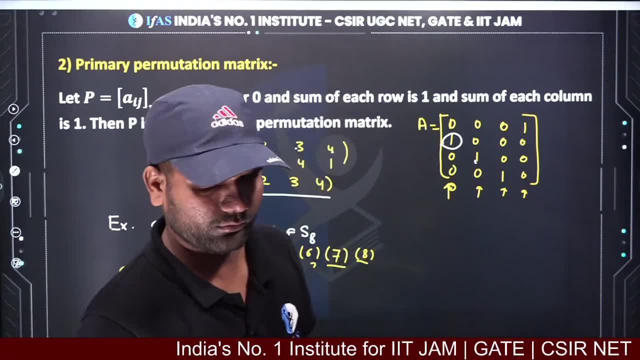 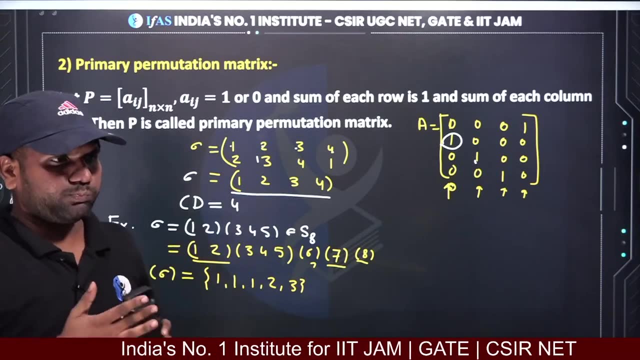 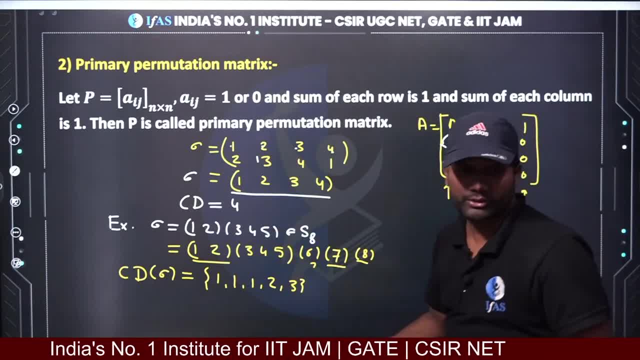 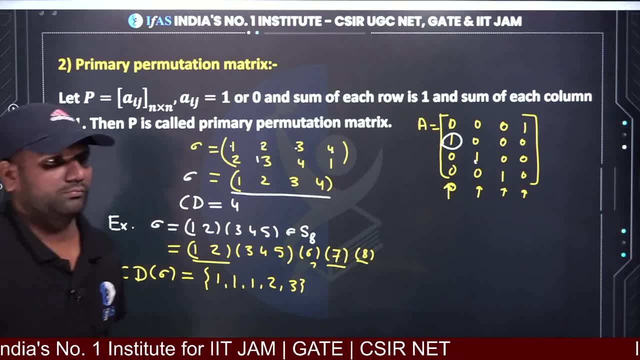 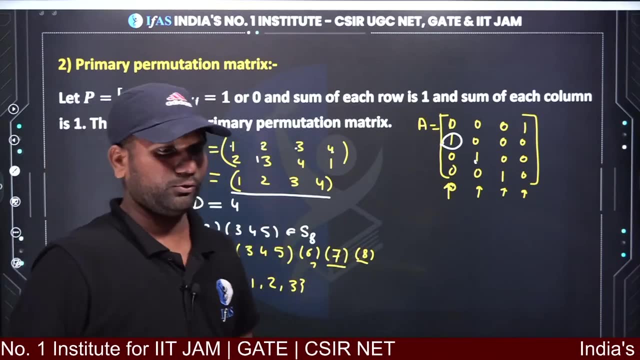 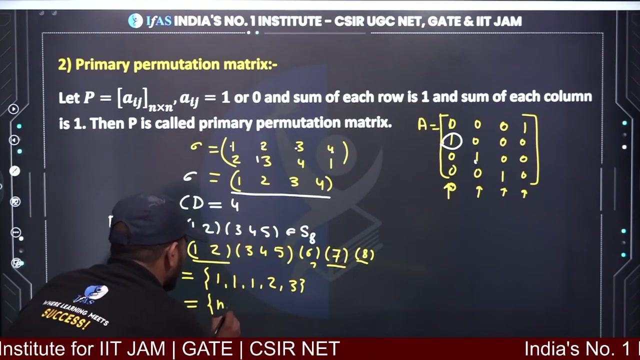 did you understand cycle decomposition or I'll give you some other examples? tell me once you sure understood. yes, I will write this cycle decomposition like this: First I call it N1,, second N2,, third N3,, fourth N4, and fifth N5. 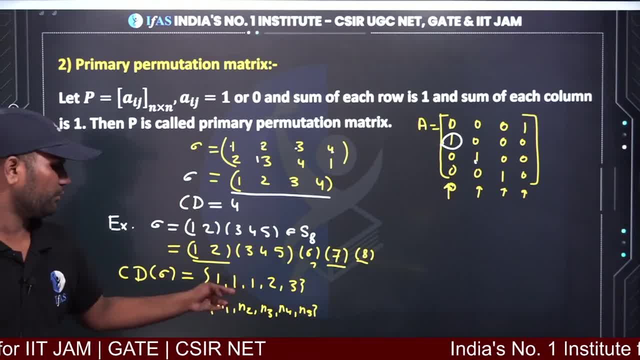 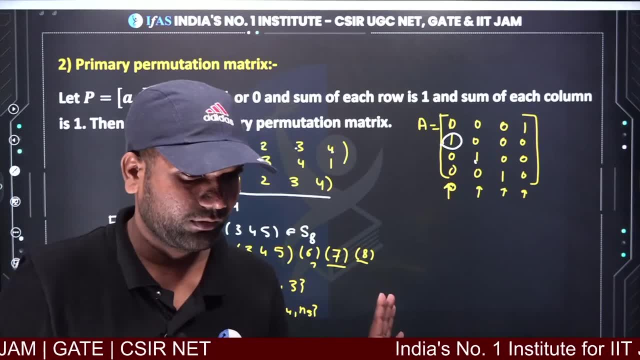 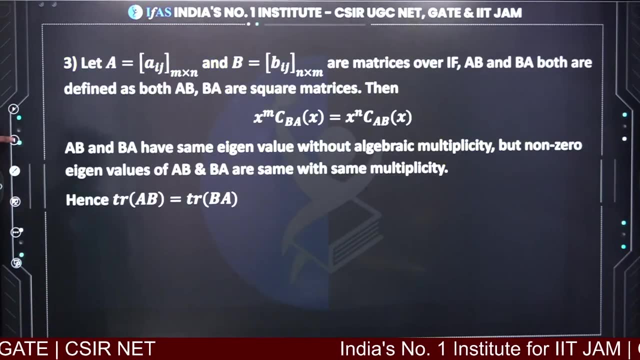 I can say that I gave it a name: N1 is N1,, N2 is N3,, N4 is N5, I just gave it a name. Ok, Yes, I think so too. Ok, let's come to the next slide. There is something else on the next slide. wait, let's add a slide for you. 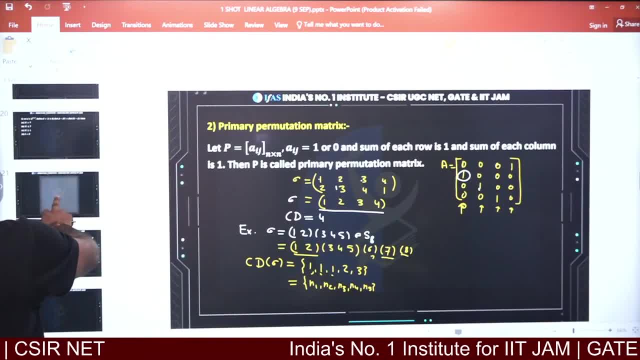 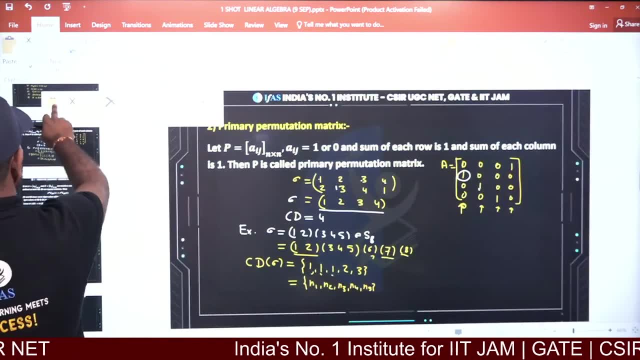 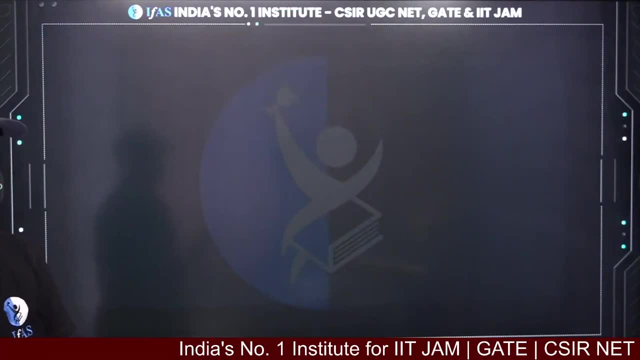 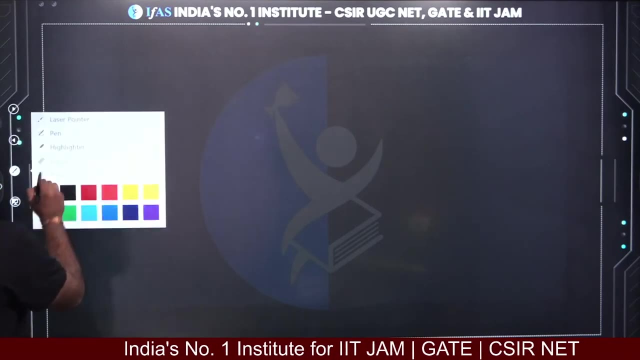 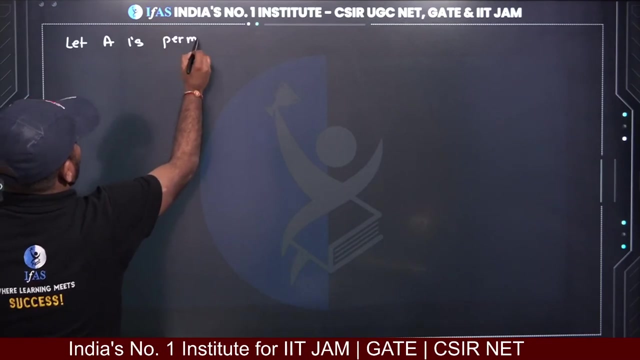 Ok, wait Now let's come here. Suppose I took a permutation matrix, So you have to take care of some important results about permutation matrix. So suppose I took a permutation matrix here. Let A: A is a permutation matrix. If A is a permutation matrix. If A is a permutation matrix. 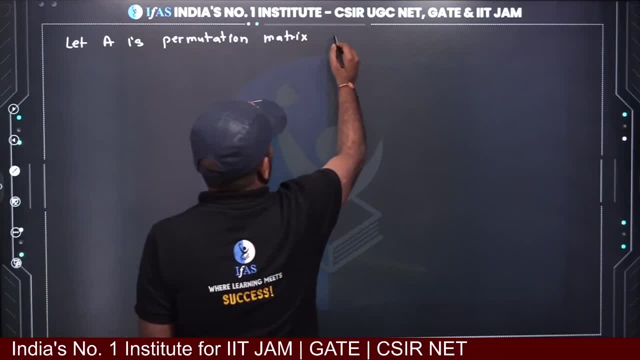 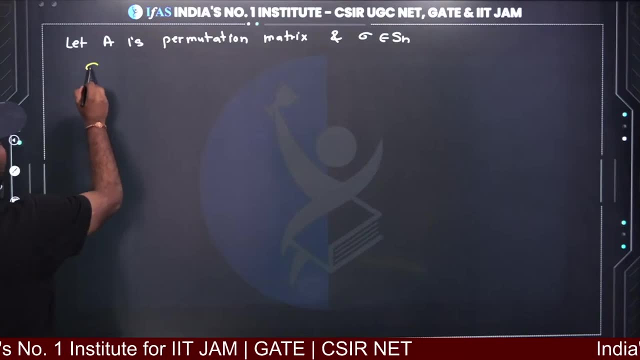 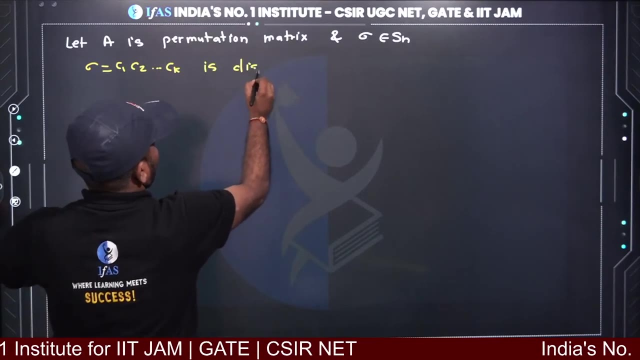 If A is a permutation matrix And what I have taken is a sigma, permutation will be made, it belongs to Sn And I write sigma in disjoint cycle form. What is sigma C1,, C2, and Ck? This disjoint cycle form is disjoint cycle form. 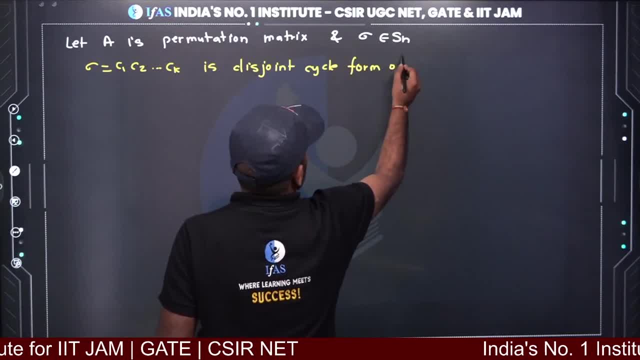 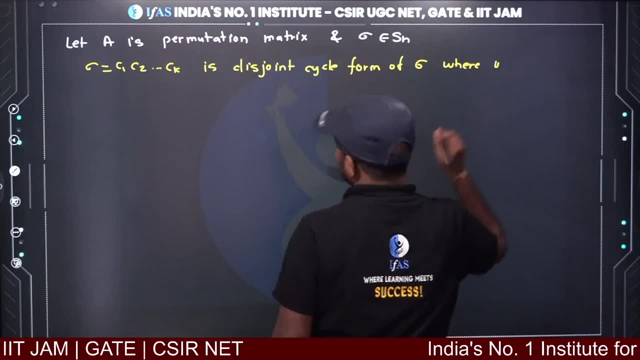 I have taken a disjoint cycle form of sigma Where C1,, C2, and Ck are cycles, Where Cis are cycles of length. For example, the length of this cycle is N1,, its length is N2, and its length is Nk. 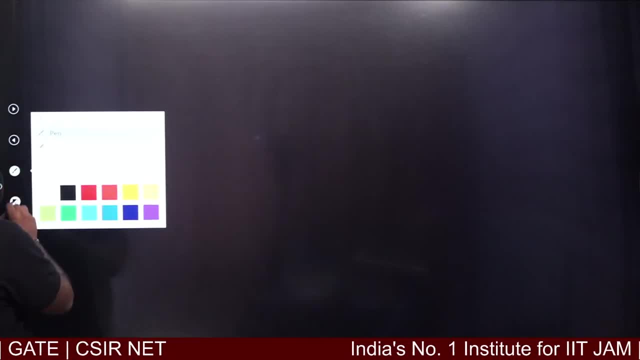 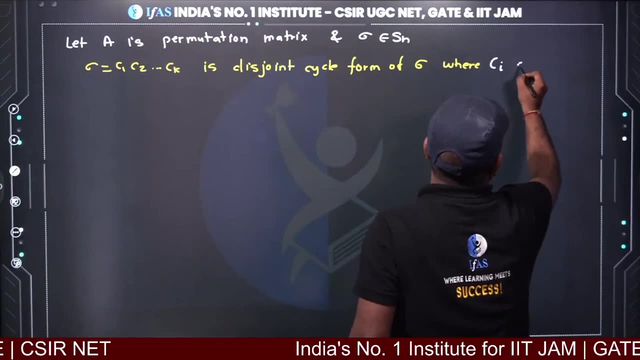 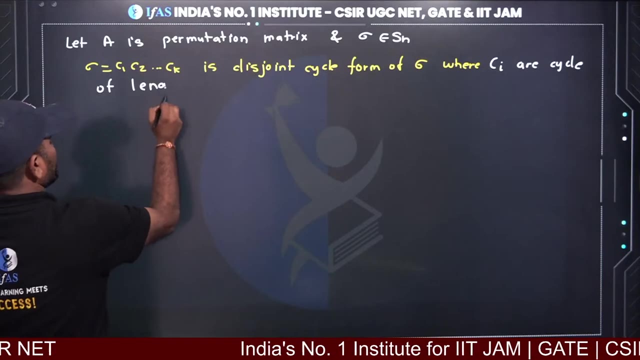 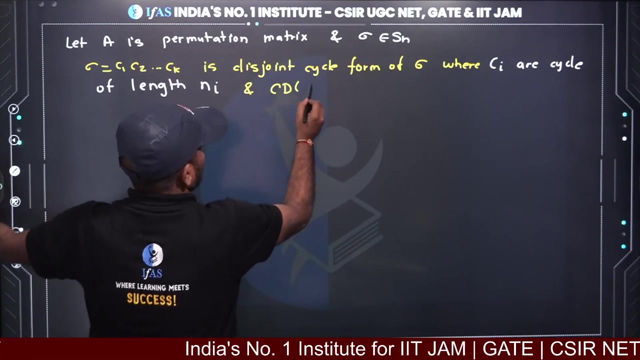 Ok. So what I am saying here is There is only one permutation use, otherwise the rest is simple: only Where Cis are cycles- Cycles of length, ni Cycles of length, ni Cycle decomposition- And Cd of sigma- Cycle decomposition of sigma- is taken for n1, n2 and so on. 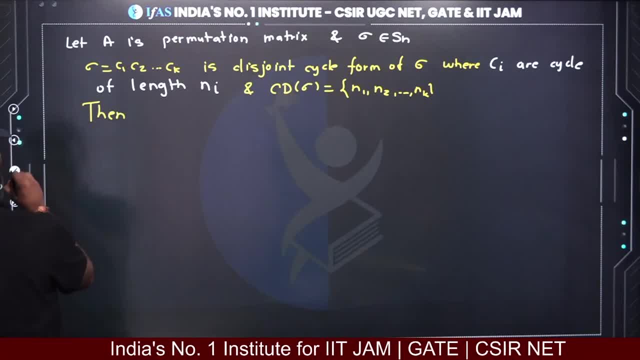 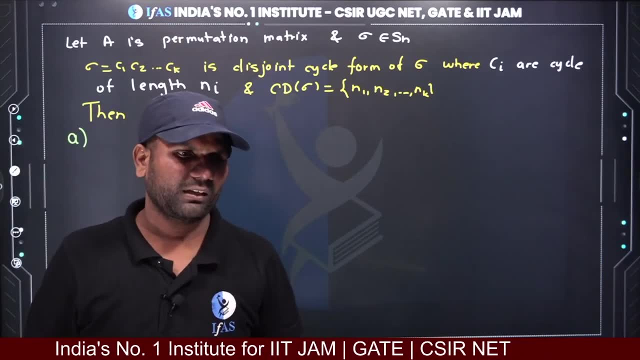 Then Now, here we have some results and properties that you should know. Now let's see one by one, Property Number A: Permutation matrix is clear for everyone. Class is done till about 10th grade. Permutation matrix is clear for all students. The permutation matrix is clear to everyone. see it once. 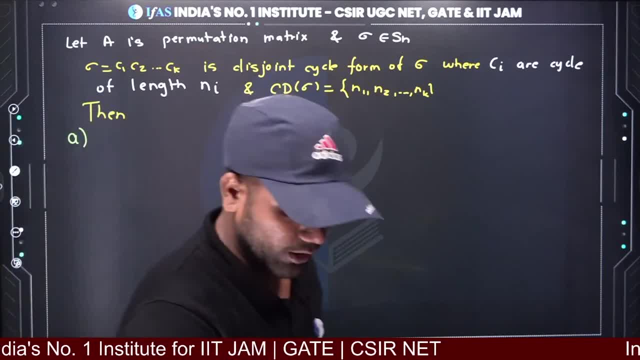 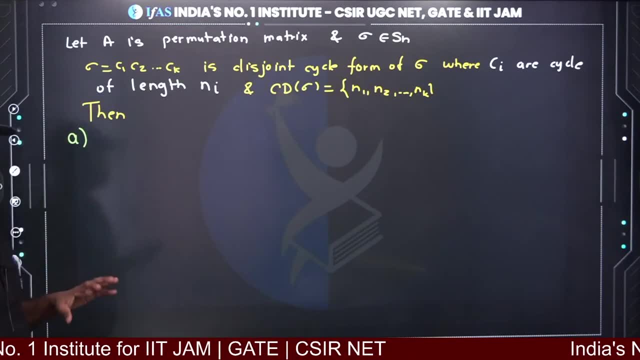 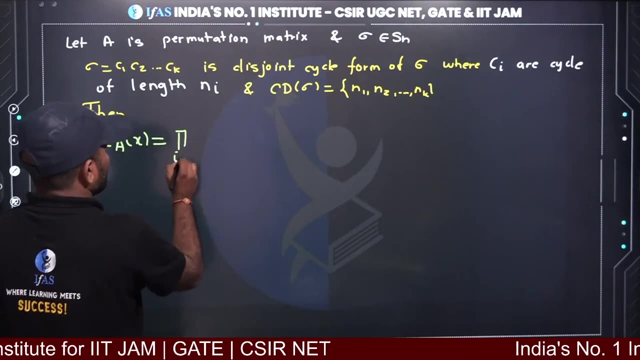 Ok, I hope everyone will be clear that the permutation matrix is not a problem. Now see here: If the answer is given, then you will be asked that what will be the characteristic polynomial of this type of matrix? So what is the characteristic polynomial of A Product? i is equal to 1 to k. 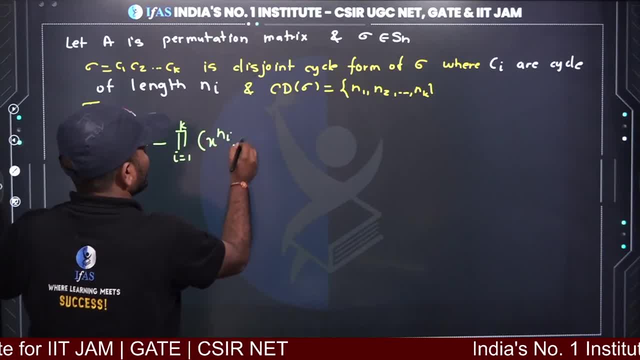 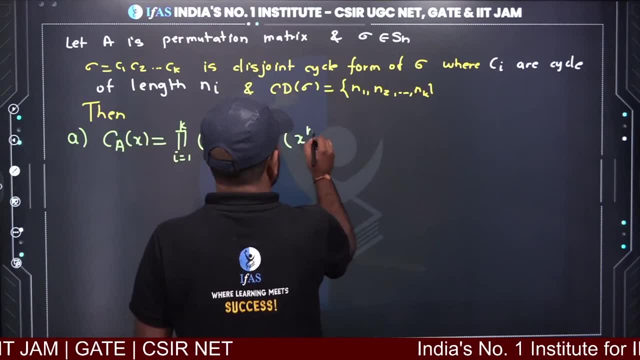 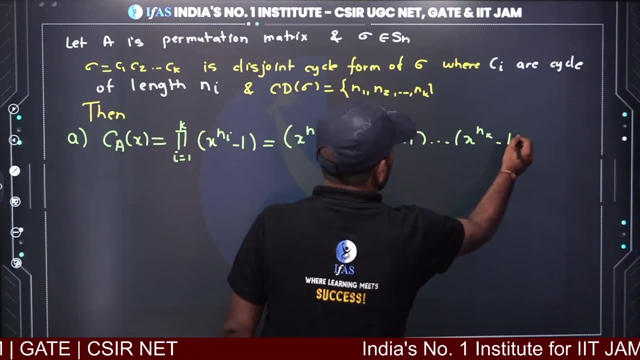 n1, n to nk. x raise to ni minus 1 Means what will be its characteristic polynomial. So you get the characteristic polynomial of this matrix: x raise to n1 minus 1, x raise to n2 minus 1, And so on: x raise to nk minus 1. 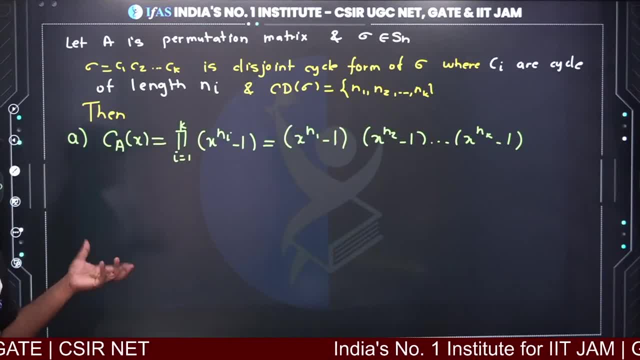 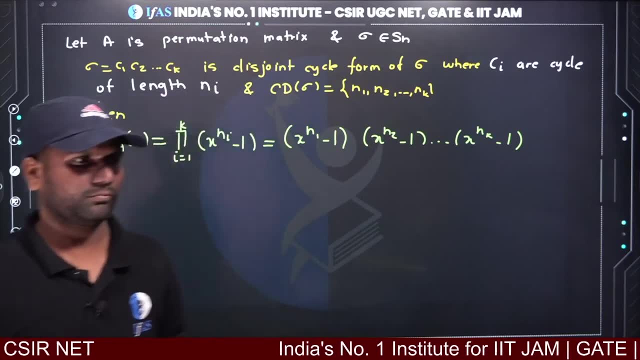 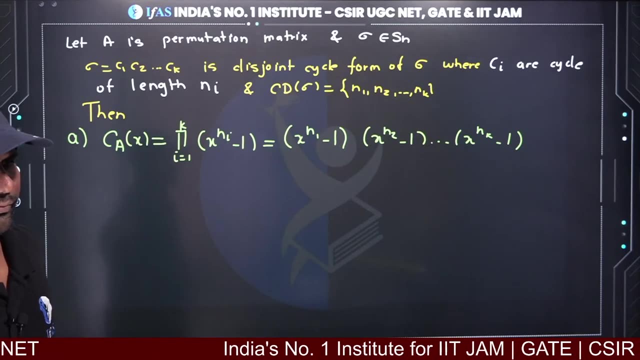 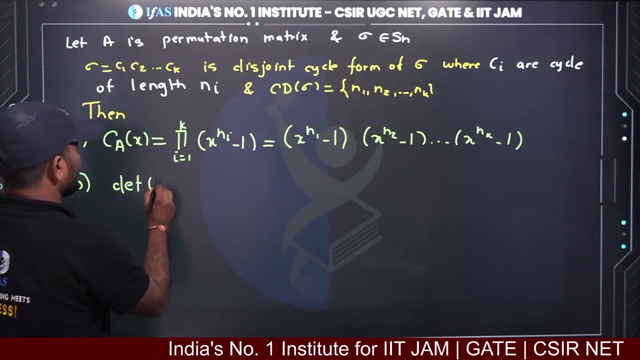 So you get its characteristic polynomial. Ok, Do you understand the characteristic polynomial? See it? Ok, Come on, I hope you will be clear till here, And if I talk something about it, What is its determinant? The determinant of permutation matrix is either 1 or minus 1. 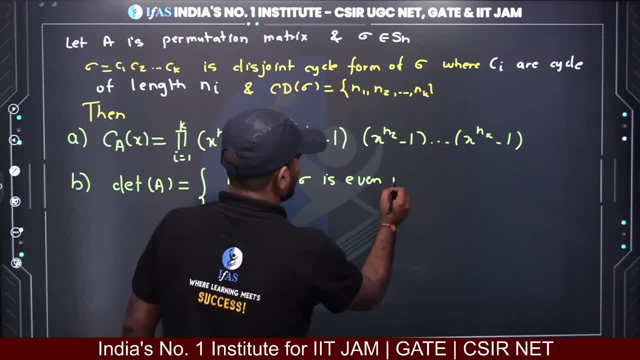 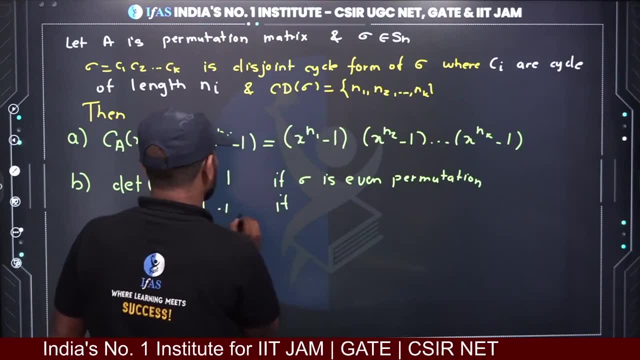 When sigma permutation is, Sigma is even permutation. Ok, Test for its permutation. when sigma is even permutation, we will get1 as determant and you will get the. when sigma becomes odd permutation. When sigma is odd permutation. When sigma is odd permutation. 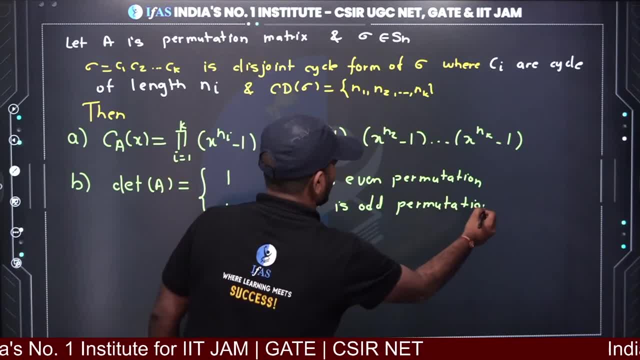 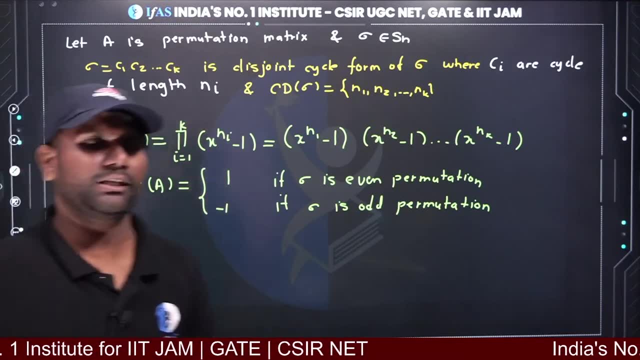 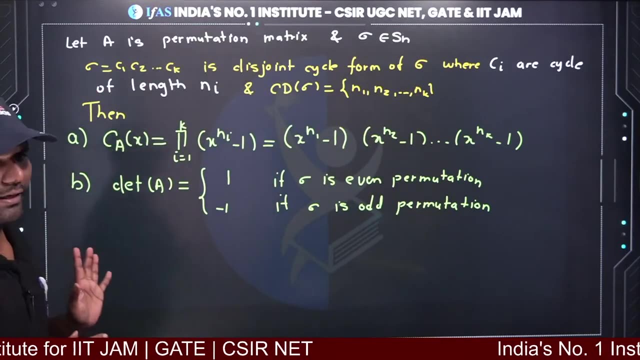 Come now. This is the way ofайт what will happen to you when there is an odd permutation. till here it is clear to everyone. there are some important results and properties about permutation matters that you should know, and some more things about it I will tell you tomorrow when we will do diagonalization. till here it is clear to everyone. 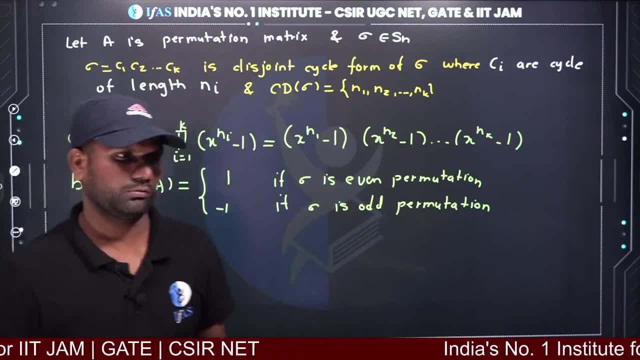 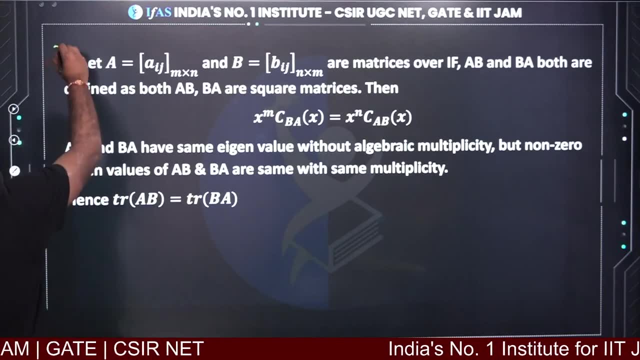 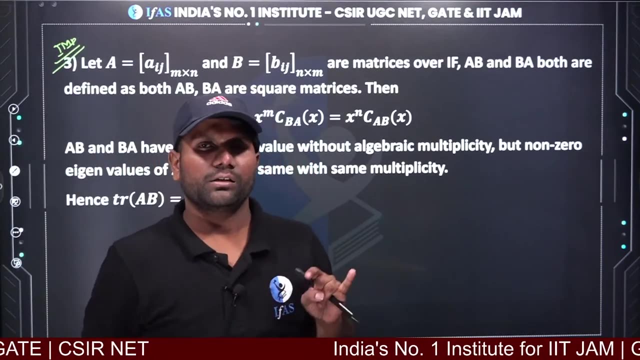 yes, you can do it absolutely, Rakesh. now let's move on to the next slide. now here is one more important result. this result has also been asked a lot of time in this result in the exam. understand the meaning of the result once. what does the result say? suppose A and B are two matrices, whose product? 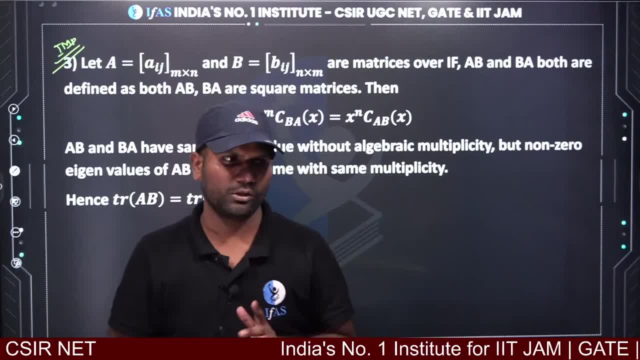 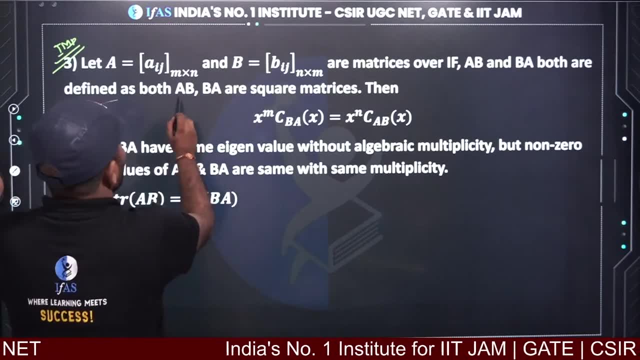 A, B and B are well defined, that is, you can multiply if A, B and B are possible. in that case, the eigenvalues of A, B and B are the same eigenvalues without algebraic multiplicity. A, B and B are the same eigenvalues without algebraic multiplicity. 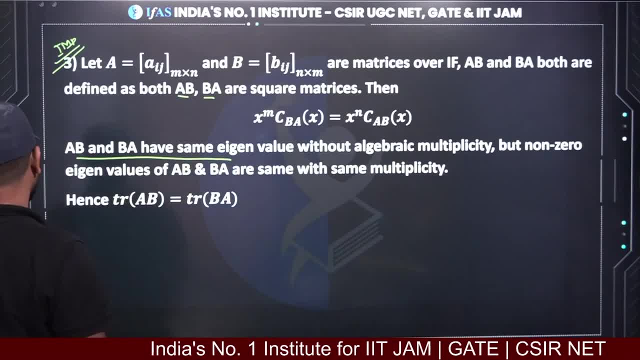 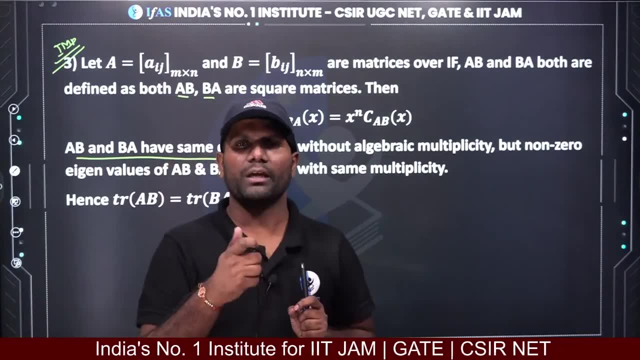 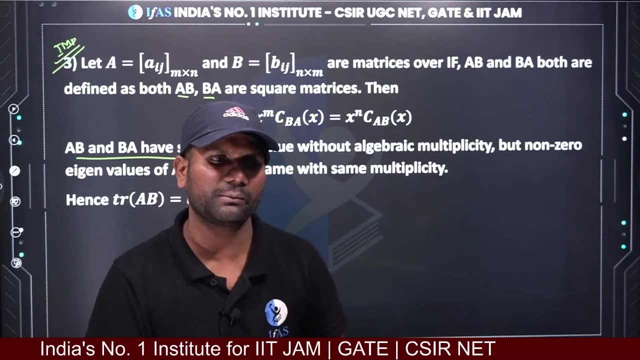 but non-zero eigenvalues of A, B and B have the same algebraic multiplicity. so what does it mean to say here? what does it mean to say here: if you are given two matrices, A, B and B, then the non-zero eigenvalues of A, B and B are the same. their algebraic multiplicity is also the same. 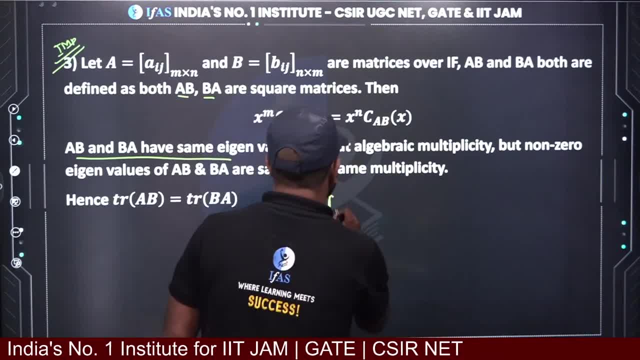 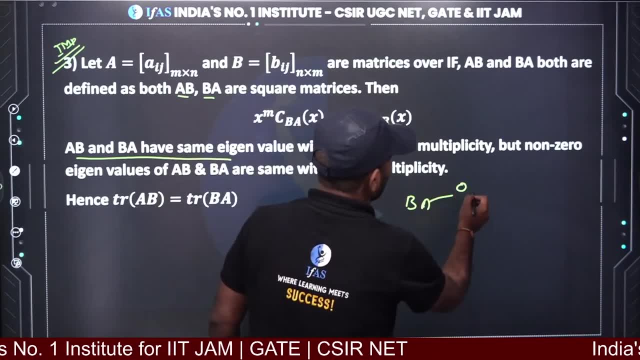 but what is the difference in this? it may be that A B has one eigenvalue, 0, if the eigenvalue of A B is zero, then two times will come here, here more than 2,, 4,, 5,, 6,. 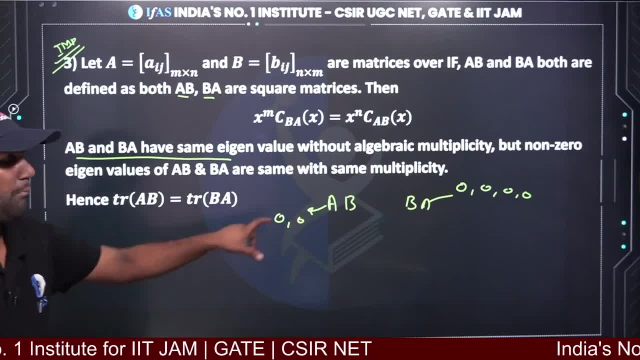 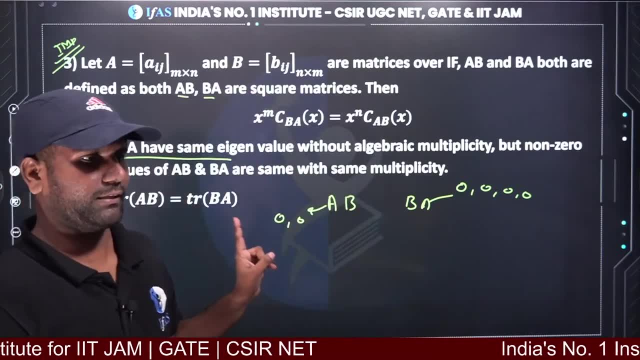 there can be a difference in the multiplicity of zero, but there is no difference in the multiplicity of non-zero eigenvalues. it's the same. this is also an important result. if you have solved the PYQ in the exam, then 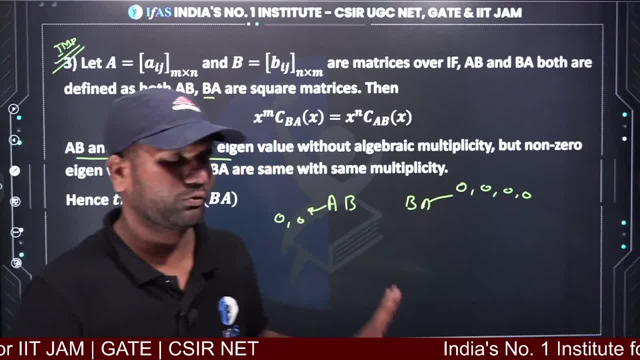 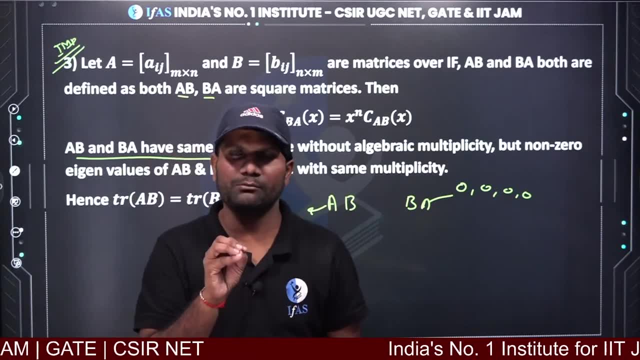 at least 4, 5 questions have been given where the question could have been solved easily using this result. Did you understand the result? that is, first tell me whether you understood the results. if you understand the results, then only you can apply. it is very important that you can apply, then only you can apply. 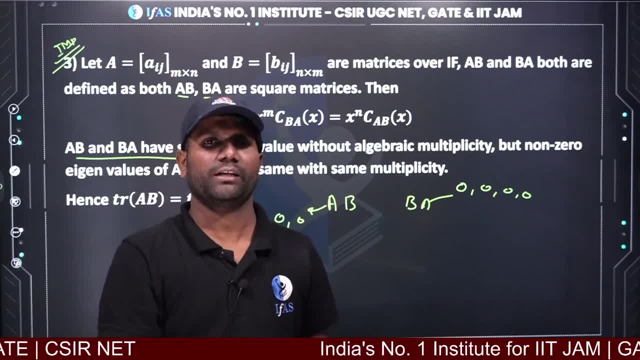 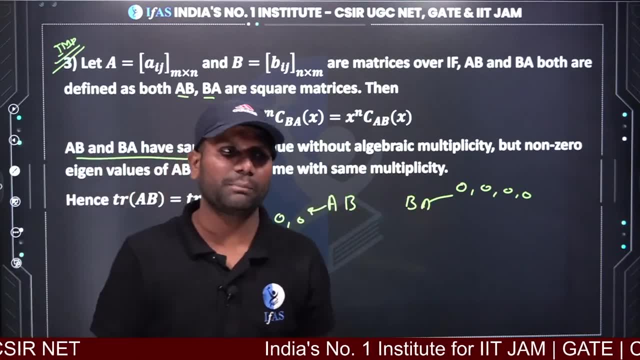 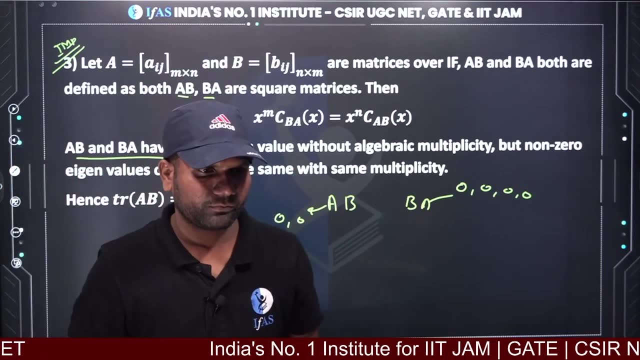 non-zero eigenvalues of AB and BA are same and their algebraic multiplicity is also same. the only difference is in the algebraic multiplicity of zero eigenvalues. you can see the difference. ok, I will tell you where the difference will come. the difference is the eigenvalue of zero. 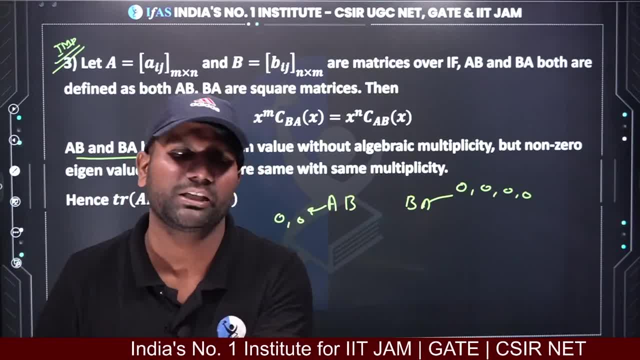 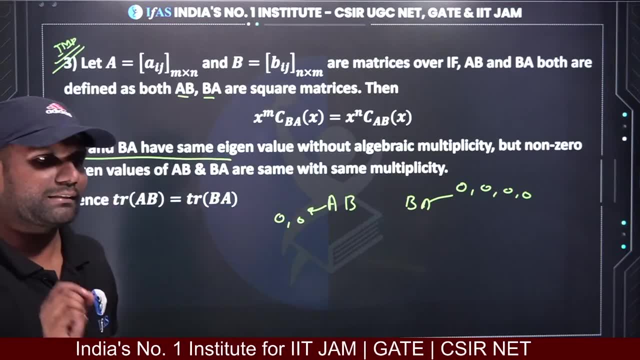 it can be 0, 2 times, 5 times, 6 times. the algebraic multiplicity of zero can be different in both the matrixes, but the algebraic multiplicity of non-zero will always be same. and there is one more special thing about this matrix. 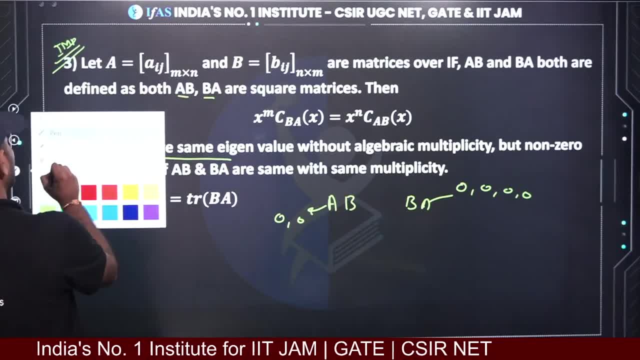 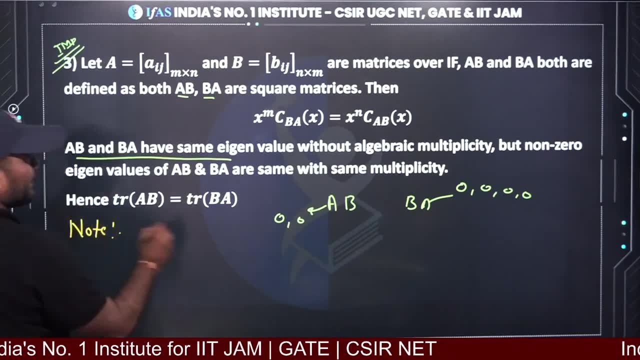 what is special about this matrix? suppose I have the same result. what should I do now? I will add a note. till now you have seen the order of AB and BA. we did not take A and B square matrix. A is any matrix, B is any matrix. 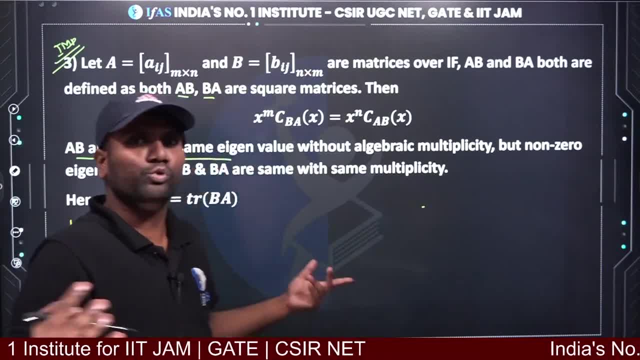 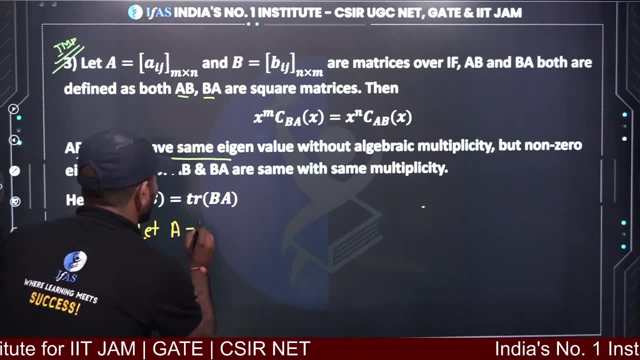 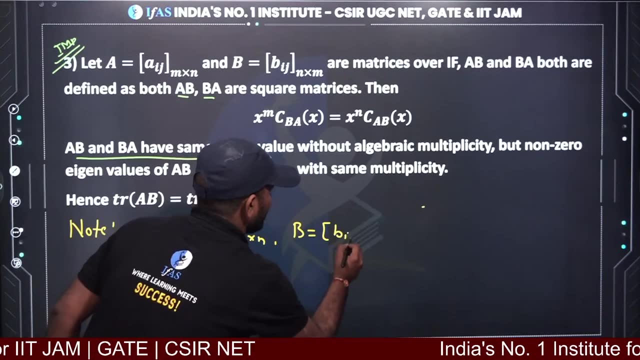 we did not take square matrix. what will happen if I take square matrix? suppose I take A plate, A and B. both are square matrices. suppose what you have taken, A is equal to A- ij and order is n- cross n and B, B is B- ij. order for this is n cross n. 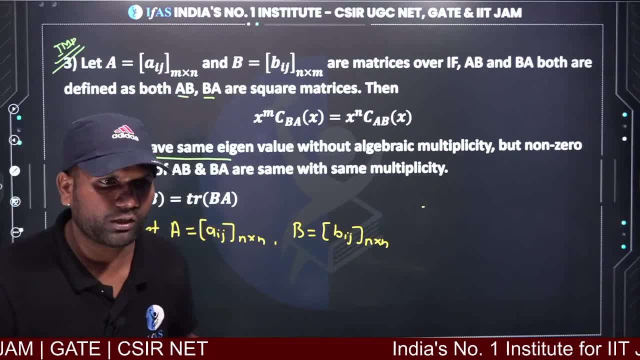 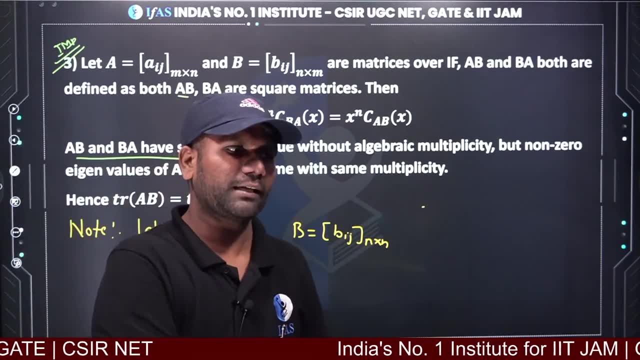 so here you will see what is the order of A and B: n cross n. yes, I am doing it. I am doing the question, alpha. wait a minute. I will tell you the result and ask you the question so that it is more clear. I am doing it. I am telling you. 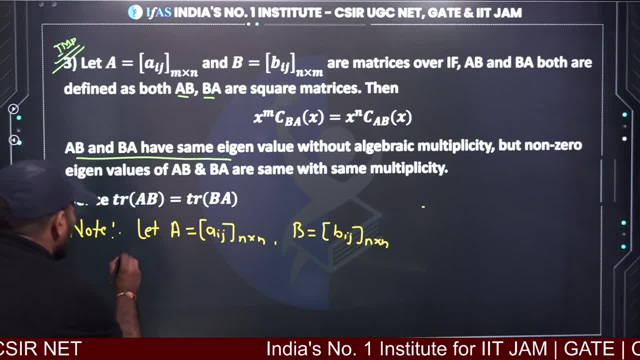 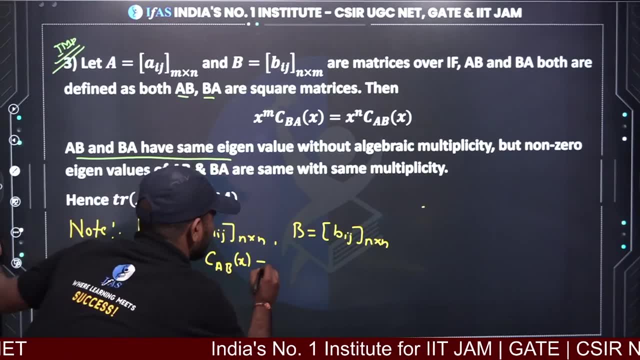 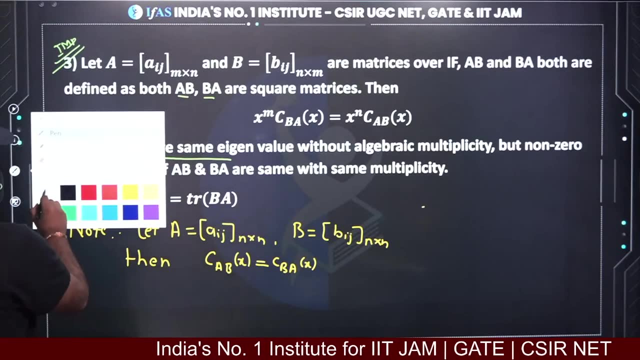 suppose I have taken A and B, two square matrices. so in that case, if A and B are square matrices, so in that case characteristic polynomial of AB and BA: both are same. so characteristic polynomial of AB and characteristic polynomial of BA, both are same. so what do we know from here? 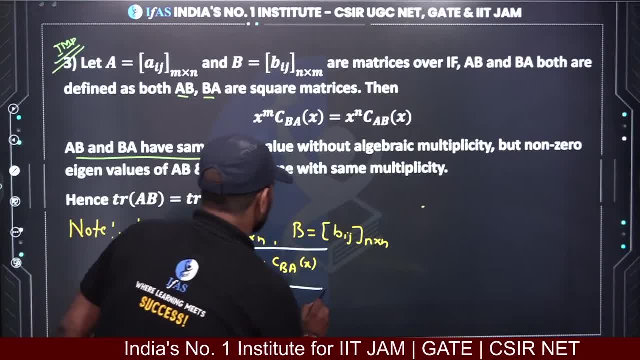 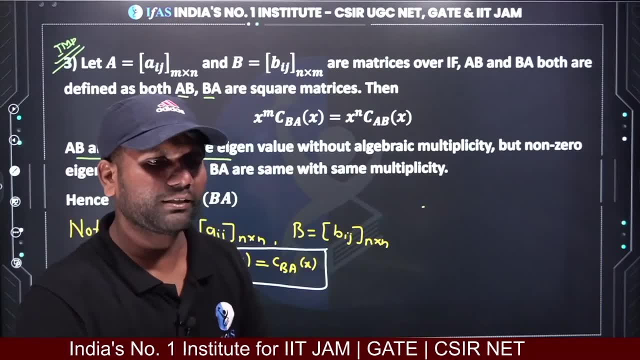 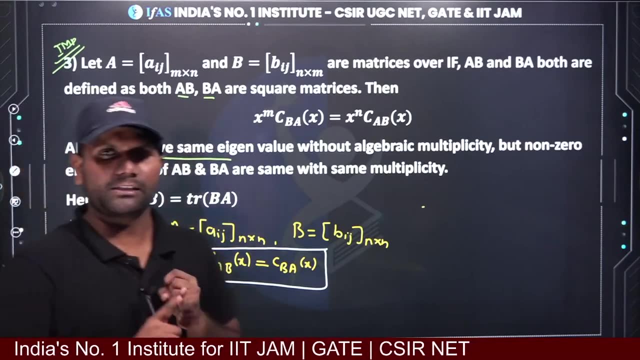 if A and B are square matrices, so in that case the algebraic multiplicity of every eigenvalue in AB and BA is same. there is no minimum requirement, but characteristic polynomial will be same here. if the matrix is square, then the algebraic multiplicity of every eigenvalue in AB and BA 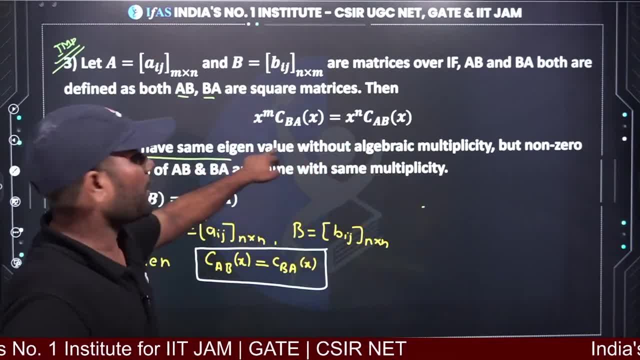 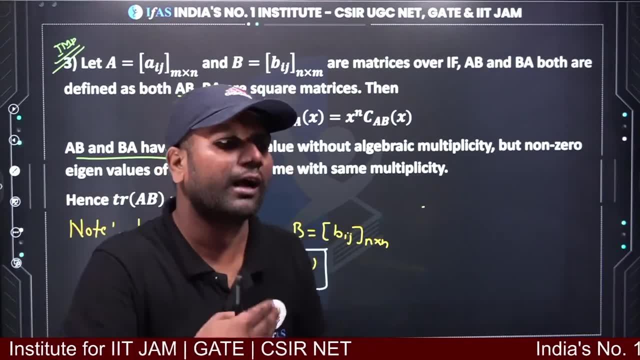 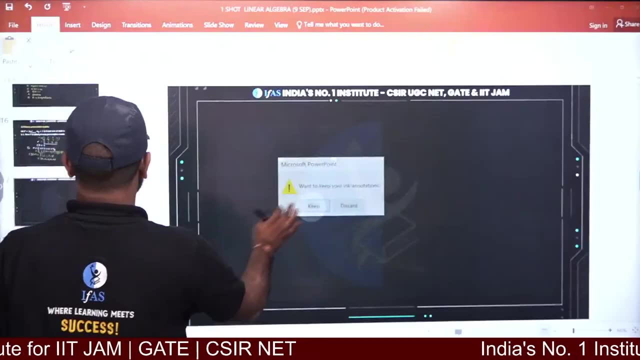 will be same. if the matrix is not square, then the algebraic multiplicity and geometric multiplicity of non-zero eigenvalues will be same. it may vary from zero. let's do an example, an example for you. suppose here I give a matrix. suppose here I give a matrix. 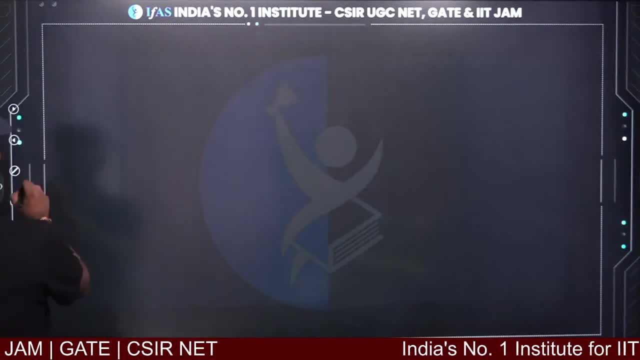 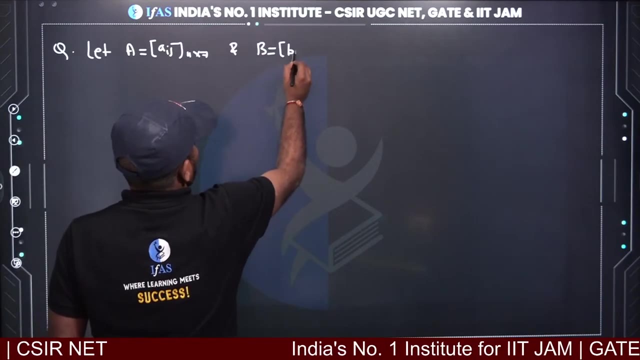 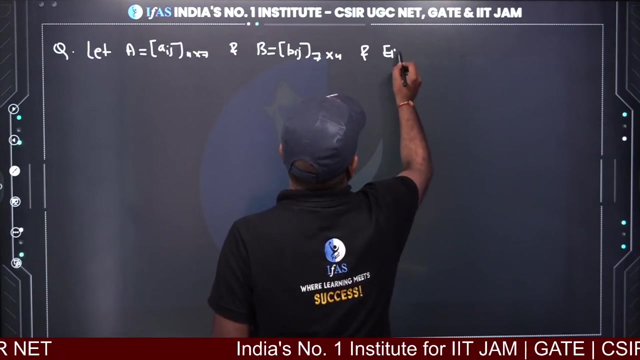 suppose here I give a matrix late A is a matrix late A is a matrix whose order is 4 cross 7, and B is another matrix whose order is 7 cross 4. now, what we have given here and eigenvalues of are eigenvalues of A. 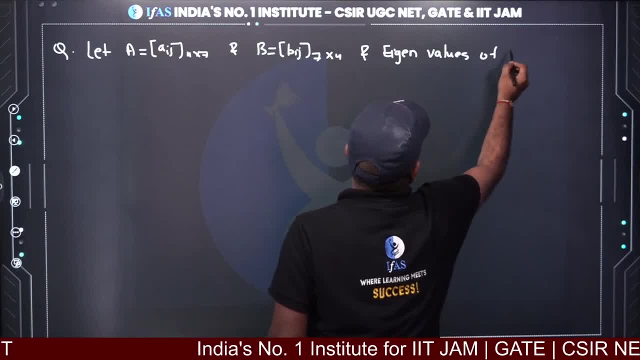 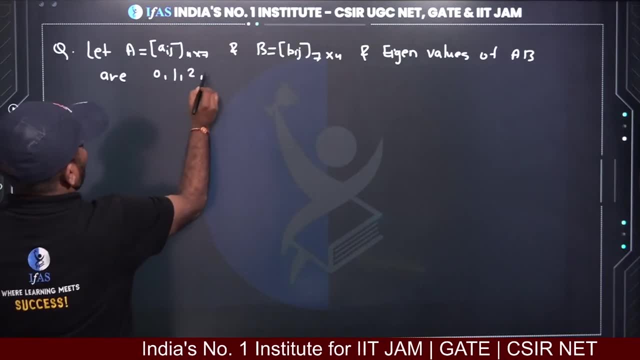 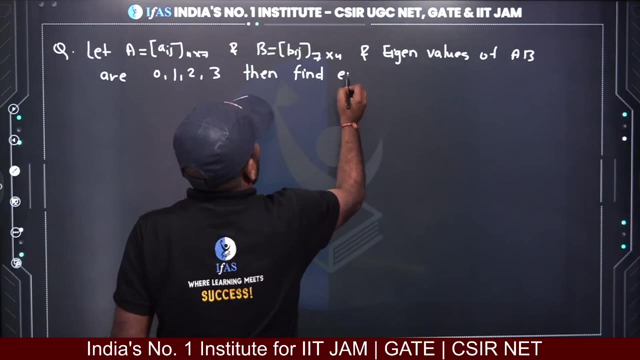 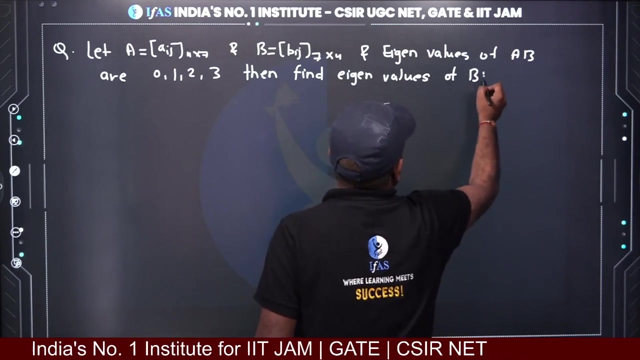 eigenvalues of AB are 0,, 1,, 2,, 3.. Then find eigenvalues of BA. Now what you have to do is to find eigenvalues of BA, So you have to tell what will be the eigenvalue of BA. 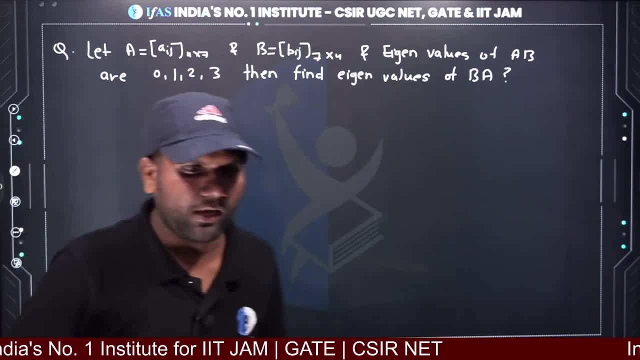 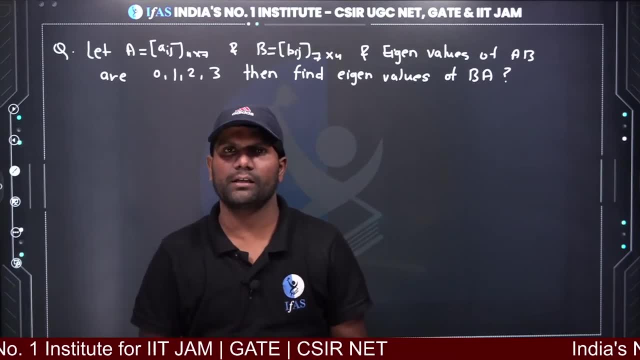 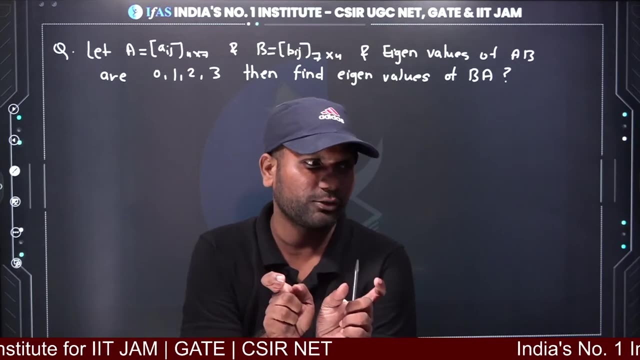 Now tell me what you think. What will be the eigenvalues of BA? Repeat the note, Amit. Amit, I was saying that if you are given A and B, both square metals of the same order, then AB and BA, which will be obtained after multiplying AB and BA, their characteristic polynomials are same. 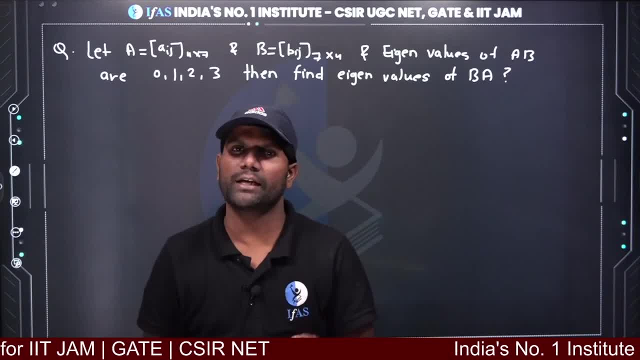 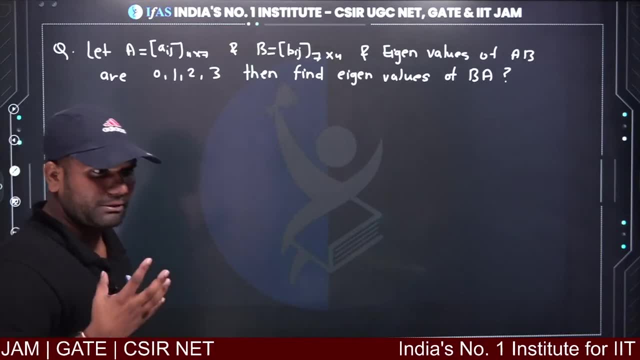 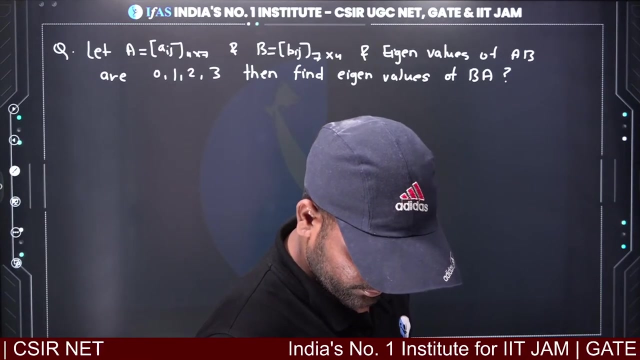 If AB and BA's characteristic polynomials are same, it means that every eigenvalue will be same and every eigenvalue has algebraic multiplicity. You know, Did you understand till this point, Everyone? clear, No problems, right? Yes, Very good, Mr Kaank Prajapati. 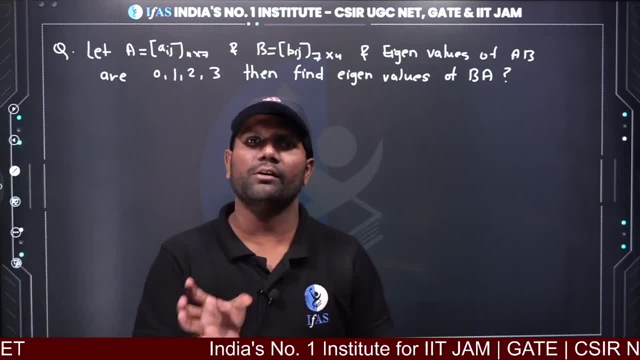 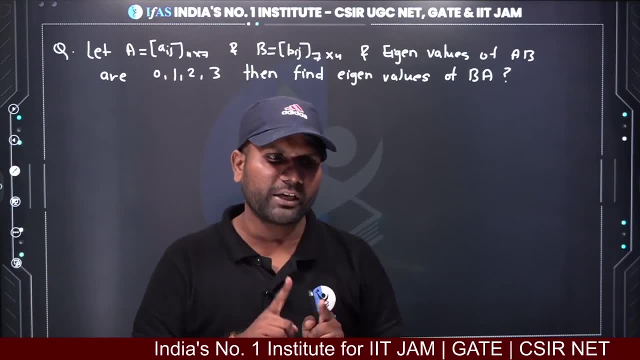 Now tell the rest of the people. Assume that here, if A and B are not square matrices, then in that case, if A and B are not square matrix- like here A and B are not square- then in that case AB and BA have same algebraic multiplicity of non-zero eigenvalues. 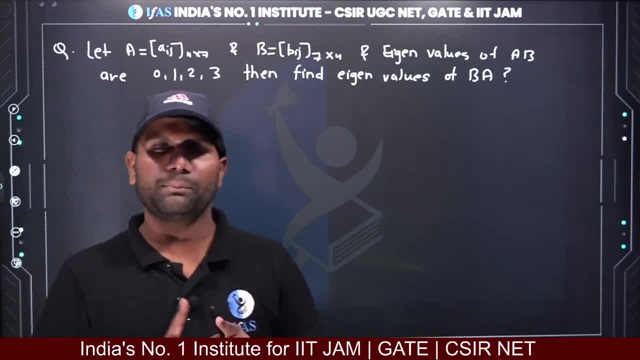 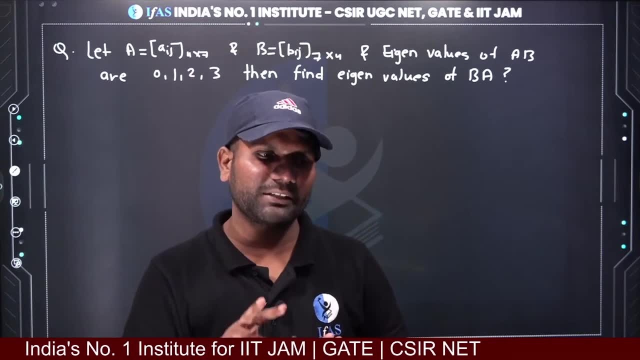 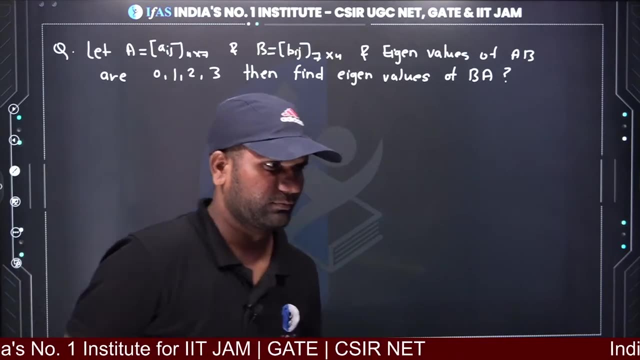 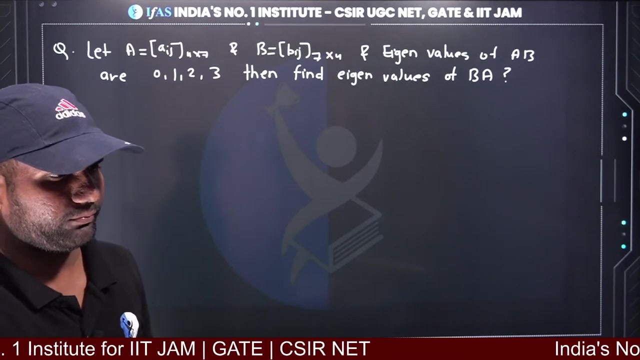 zero will have different multiplicity. first of all, their eigenvalues will be same. eigenvalues of AB and BA will be same. algebraic multiplicity of non-zero eigenvalues will be same, but there can be difference in zero. ok, perfect now, until now resume. 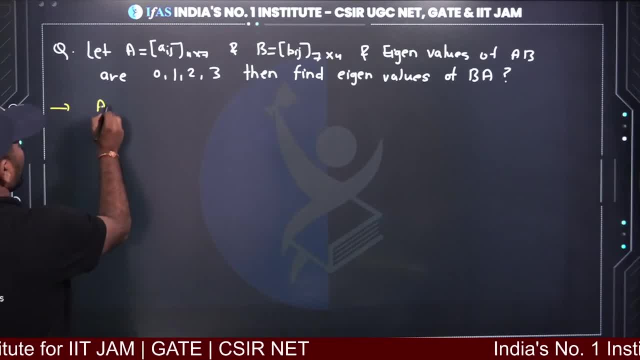 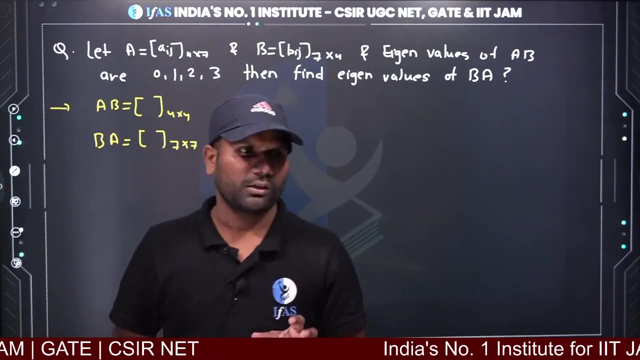 now observe 1 thing: what is order of A and B? If you check AB, order is 4x4, how will order of B and A is? if you check BA, order is 7x7 meansB will have 7 eigenvalues. so we can enjoy about AB and BA have same eigenvalues. 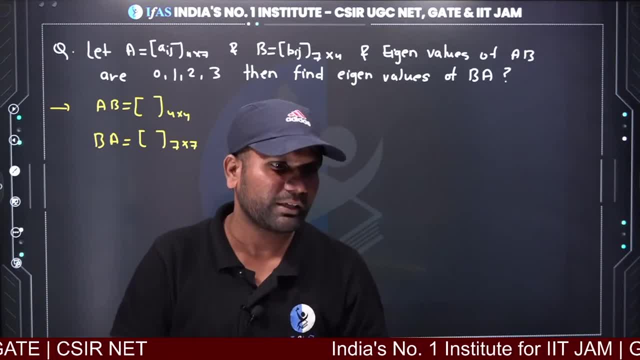 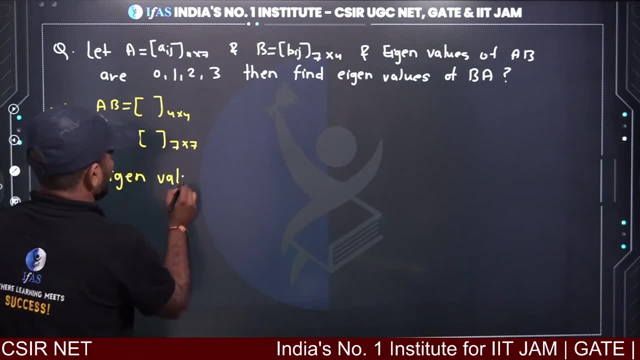 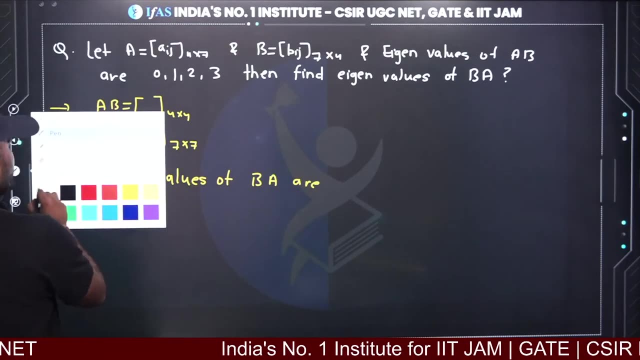 and non-zero eigenvalues are same with same algebraic multiplicity. so now we will find eigenvalues, eigenvalues of BAR. so what will be the eigenvalues of BAR? we know that the eigenvalues of AB and BA are same. 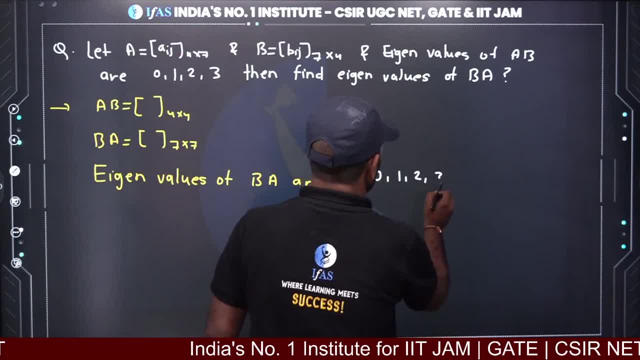 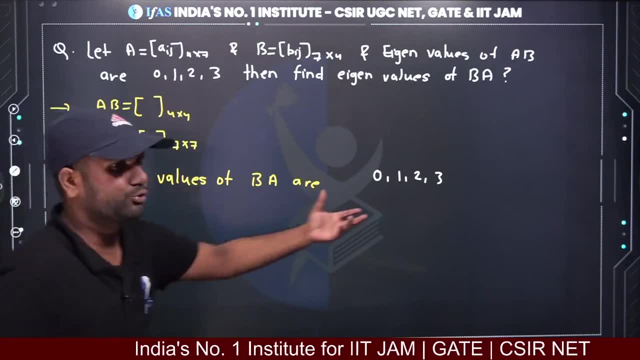 so first write the eigenvalues of AB: 0,, 1,, 2,, 3. but it has non-zero eigenvalues here and here. but we need total 7. we still have 4. the algebraic multiplicity of non-zero eigenvalues will be same with AB and BA. 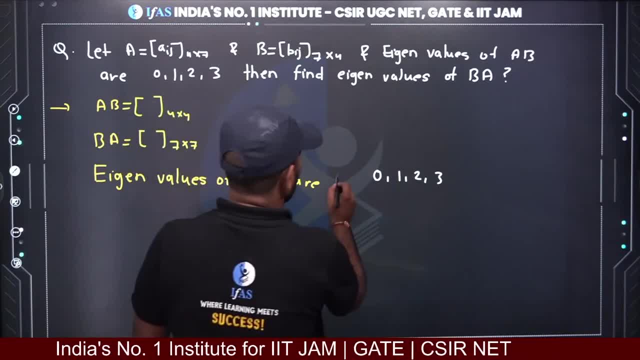 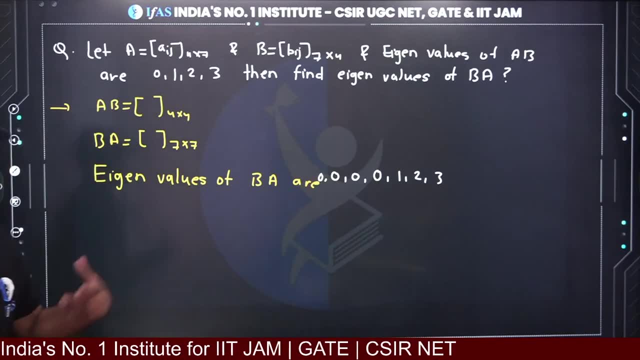 so what will be the rest of the time? then 0 will come. so what will be the rest of the time? 1,, 2, 3 and 4: we got the eigenvalues of AR. rest of the time is 0. so here you can see. 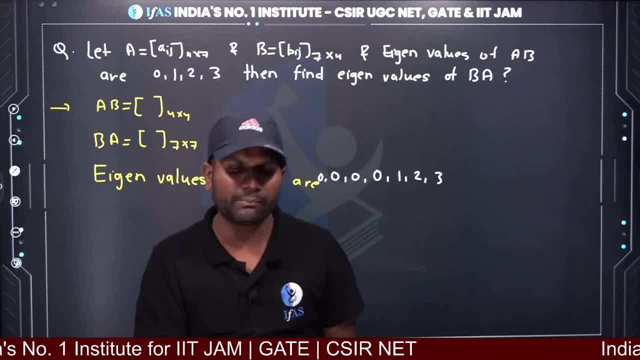 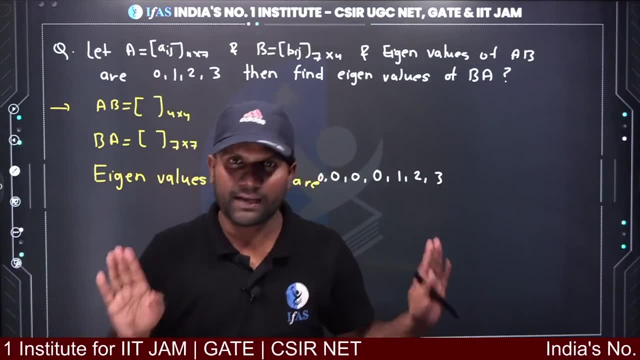 the algebraic multiplicity of non-zero eigenvalues is same. but if there is some difference in the algebraic multiplicity, then you can get the algebraic multiplicity of 0 in different ways till here you can understand there is an important result if you have solved the PYQ carefully. 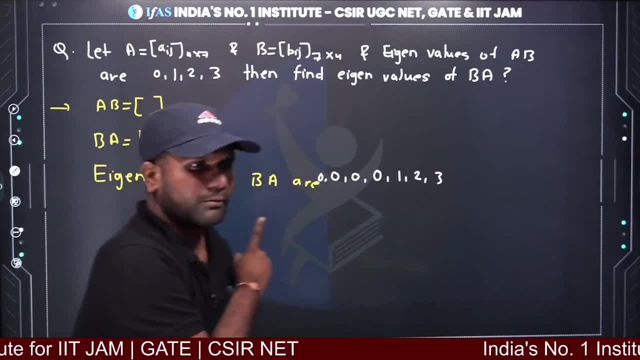 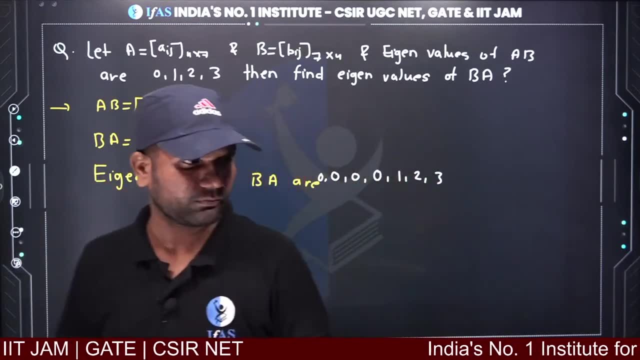 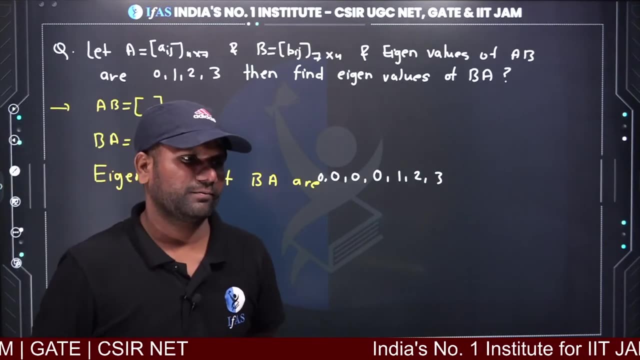 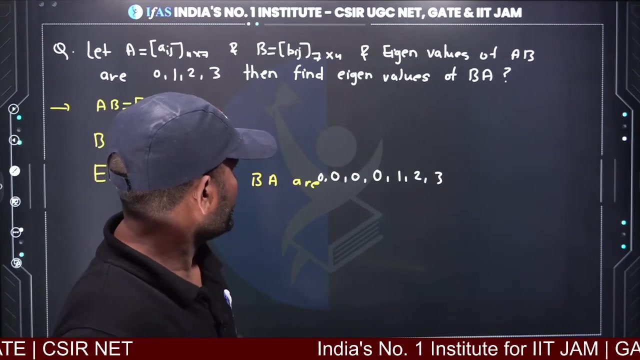 you must have got at least 4-5 PYQ on this result. ok, move ahead. tell me once all of you are clear: 2, 4, 3: yes, absolutely correct. magic is absolutely correct. magic is absolutely correct, ok. ok, now let's move on to the next slide. 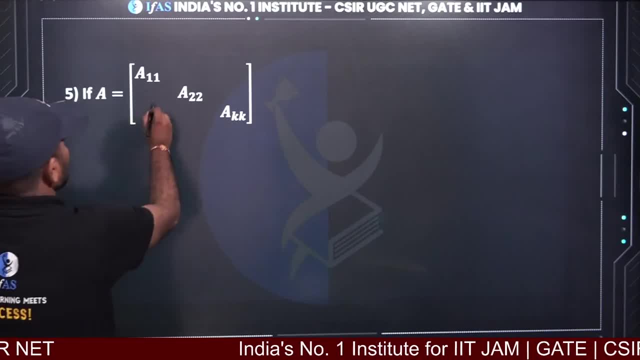 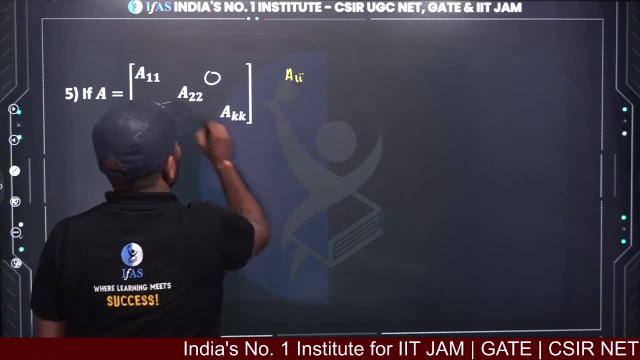 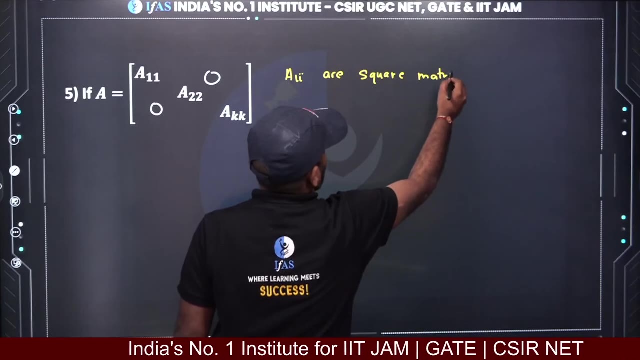 this is done. now you must be knowing this one. like you are given a block matrix, block diagonal matrix, where you know what is AI, these diagonal elements, these are not square matrix. these are not square matrix. what are all these? these are not square matrix. so, in that case, 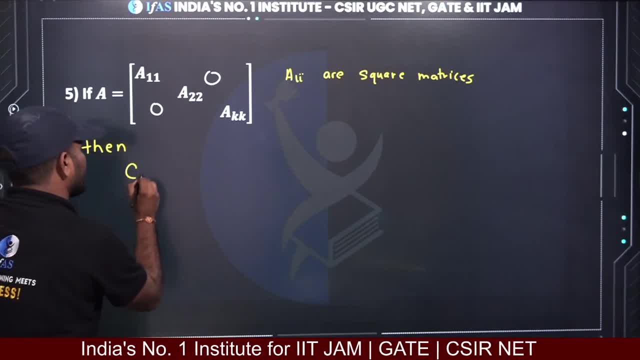 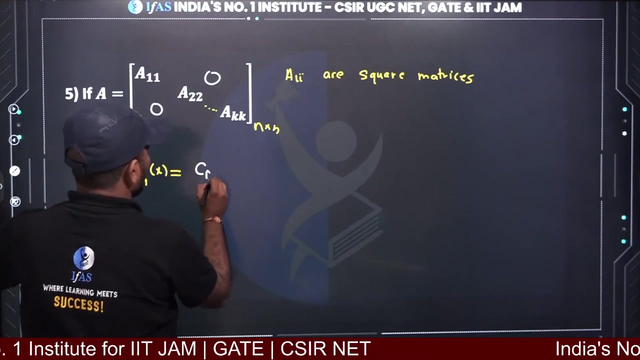 if you ask anyone about this matrix, its characteristic polynomial is 0. characteristic polynomial of this type of matrix. So what is the characteristic polynomial of this type of matrix? now, drop the characteristic polynomial, unplug and then multiply. you can remove, so as to do that you may get. 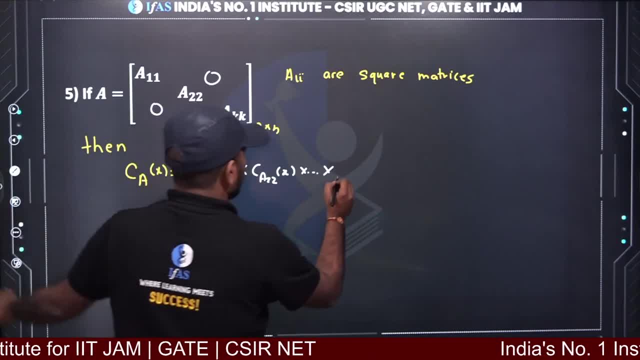 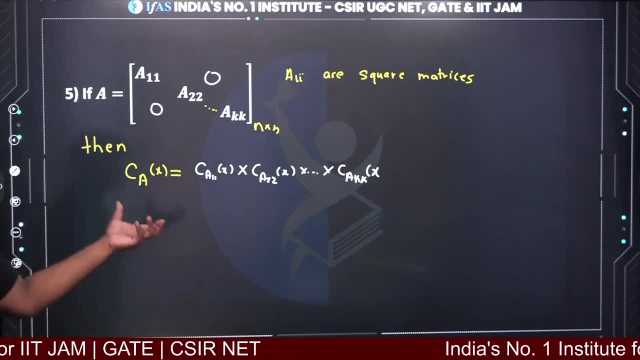 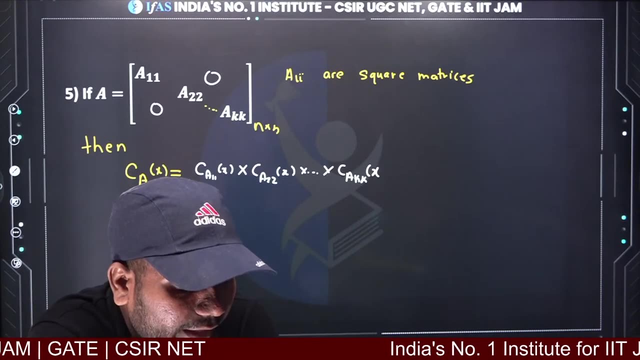 characteristic polynomial of A11. In2. characteristic polynomial of A22. polynomial of a and n. sorry, a, k, k, okay. so what can you do? in this way, you can get the characteristic polynomial of this matrix. now, avik is saying that a equal to one zero, zero, zero and zero, one, zero, zero. 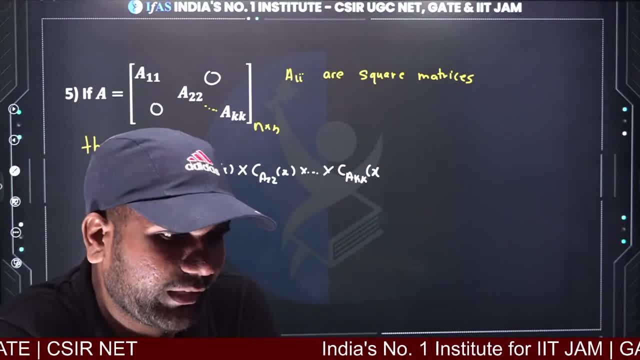 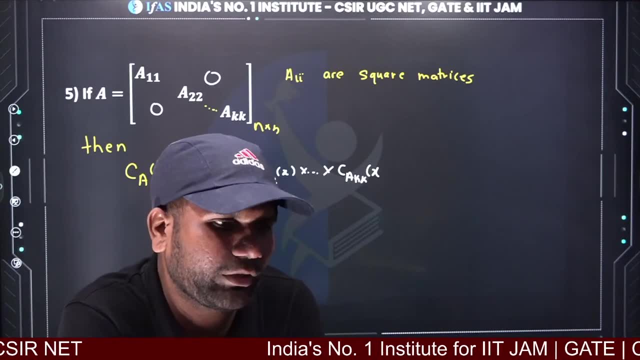 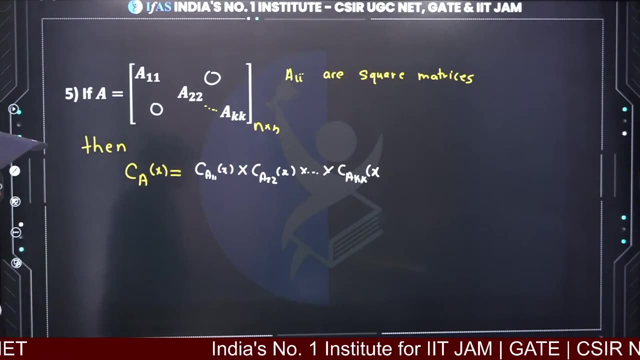 avik, then multiply this. we will say about their characteristic polynomial. first avik. you are asking about a, b and b a. the characteristic polynomial of a, b and b a should be same. multiply it and check it now. let's move on to the next slide. now here is a question for you. 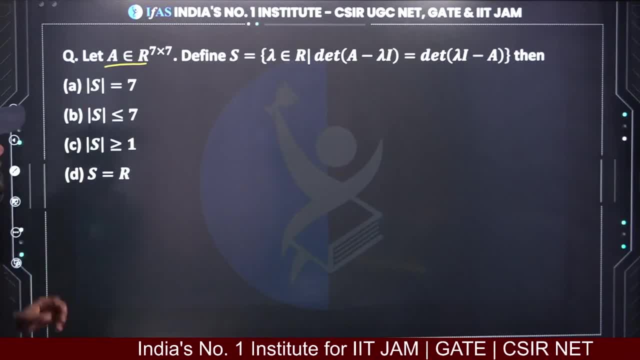 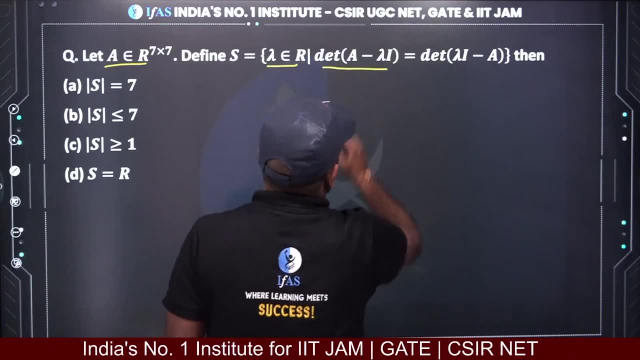 what is the question given here? the question is given to you late. a belongs to a. is the seven cross seven matrix? what is in s? in s, if you see, there are such numbers where the determinant of a minus lambda i is same as the determinant of lambda i minus a. so tell you what will be correct. 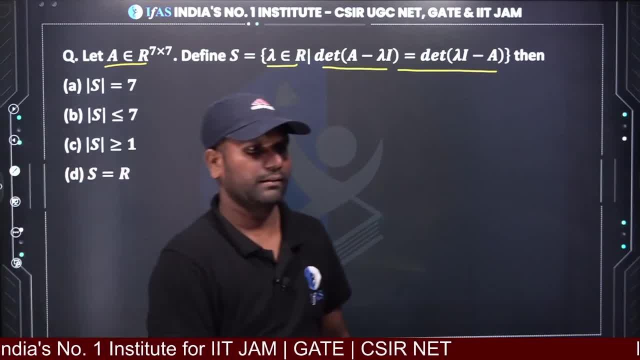 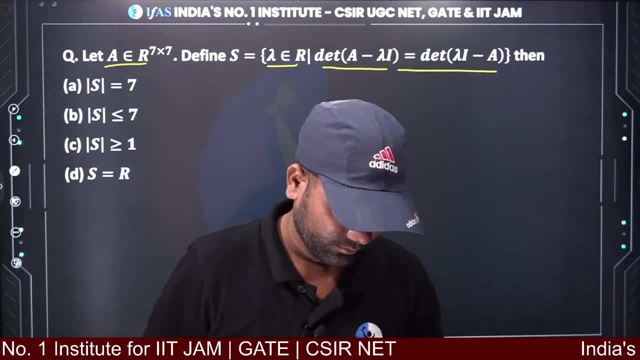 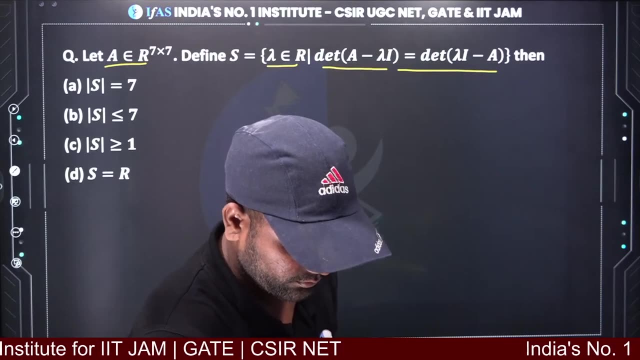 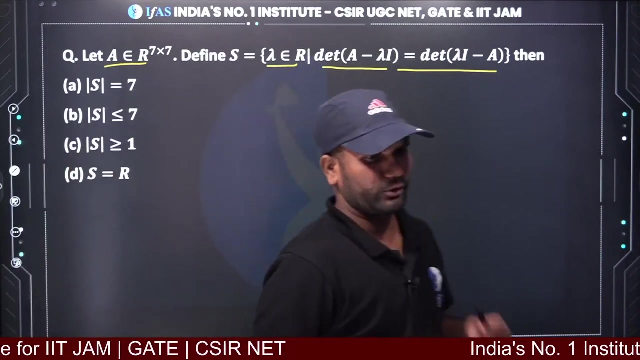 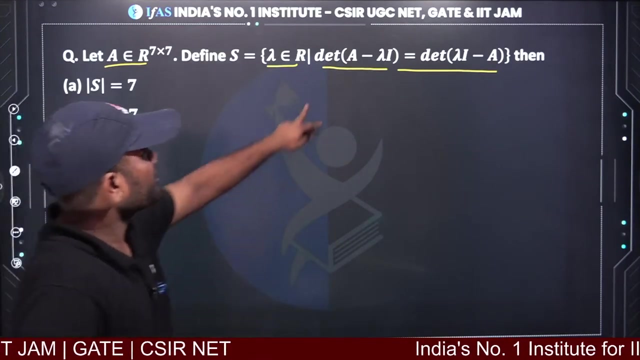 that means s can come into ifo, but you get in it. let's say you can solve this because try it everyone is a good question, try it. the answer should be met. answer ppl e. Just solve it by taking it. See when they are equal, Think about it and solve it. 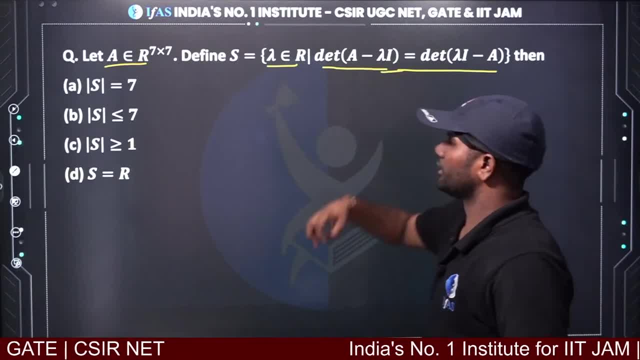 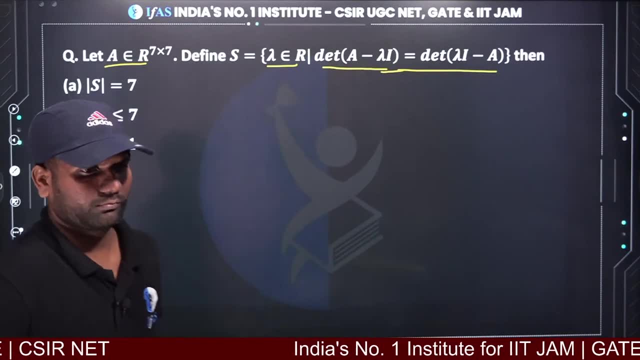 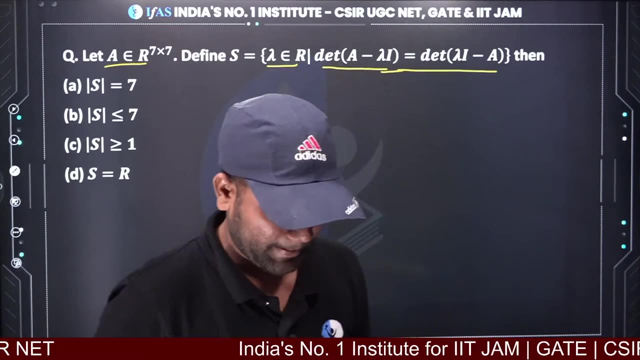 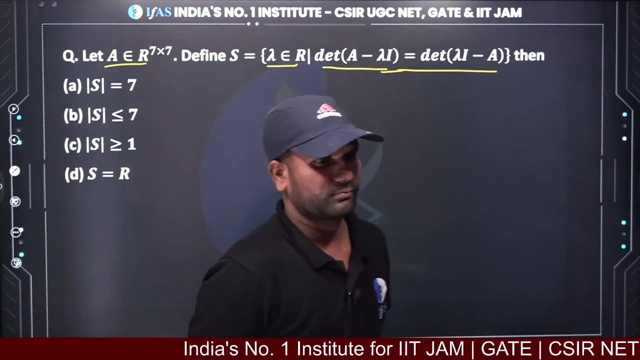 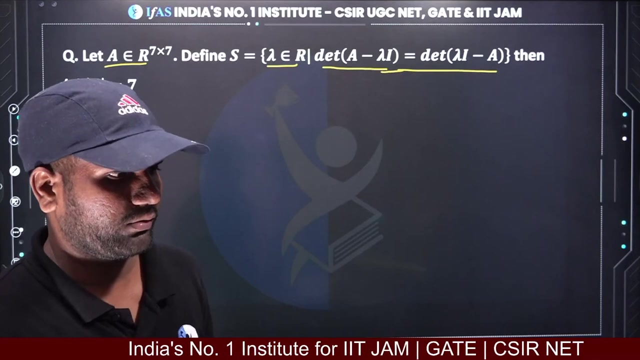 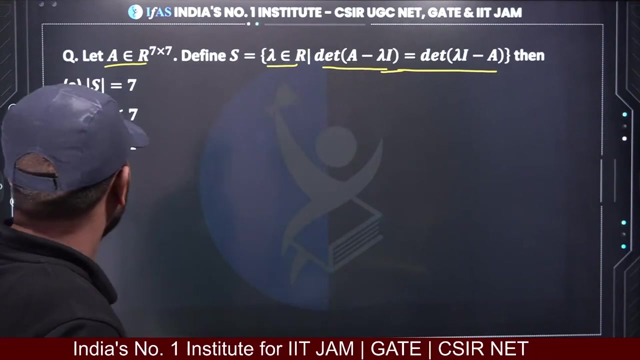 If you think the same, if you solve it keeping this condition in mind, then you can solve it. Tell me what will happen. Last question, The last result was also very important. Surajit is saying that A will be 7.. 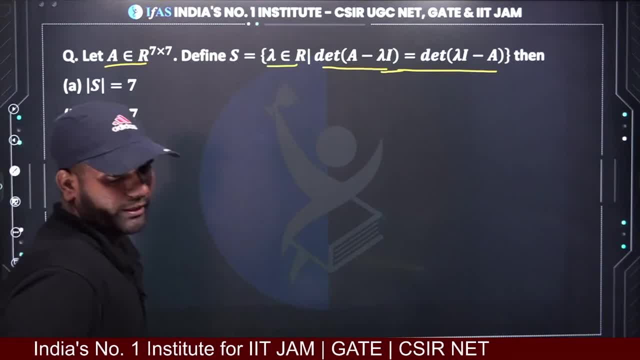 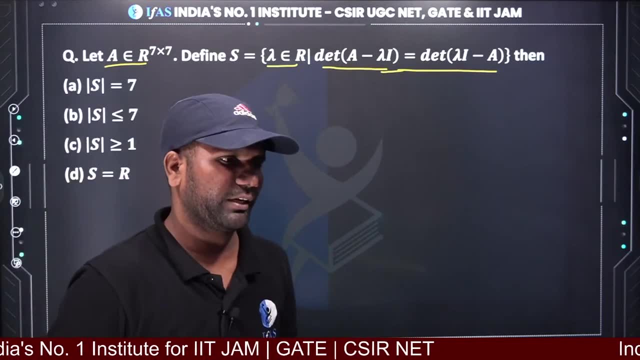 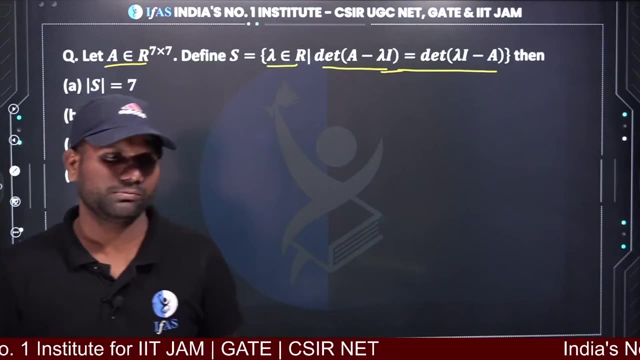 Surajit, think again. Surajit is saying that B will be 7.. Very good, You have done the right thing. Shikha is also saying that B will be 7.. The rest of the people tell me Good evening. Priyanka P, You are joining very late. 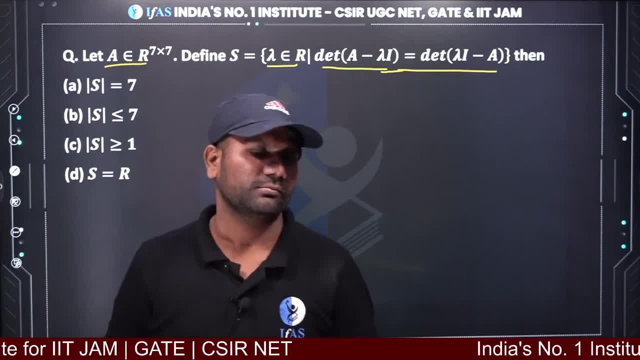 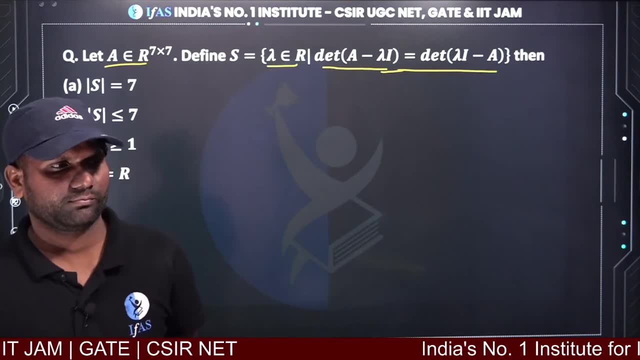 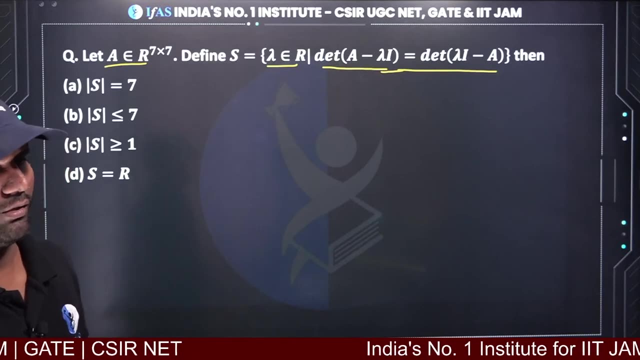 Tell me what will be the answer of this. Now look here. Yes, Alfa is saying that D will be Parul B, Prajakta B. The rest of the people also. tell something so that you know what you are thinking. 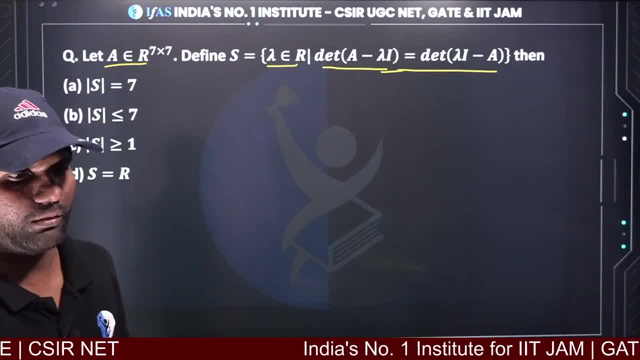 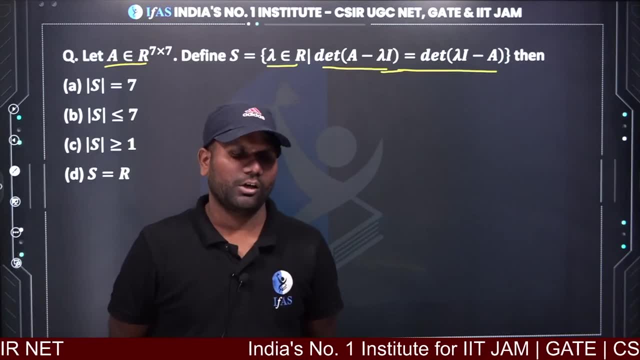 Diksha is saying that B will be Vijay Sharma, B. Prashanna B, Amrinder Srikanth. Almost everyone is saying B And guys who are joining new people with us. if you have not liked the session yet, then you guys like it. 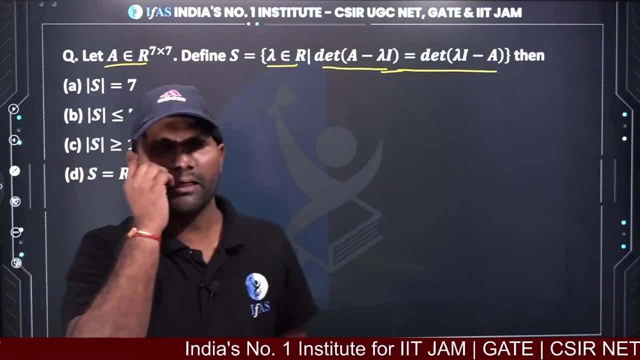 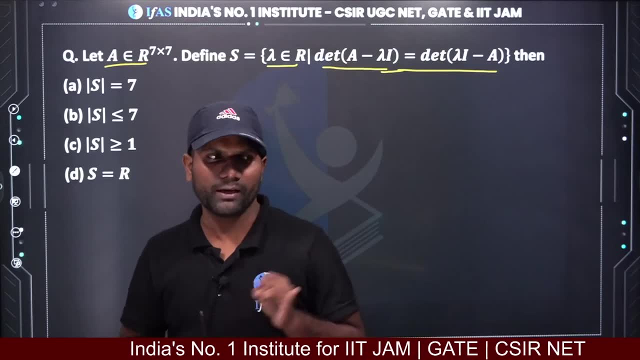 As I told you today that we are going to revise the entire linear algebra today and tomorrow. So what was our topic today? There were eigenvalues. Now we are going on eigenvalues. After that there is vector space, subspace and linear transformation. 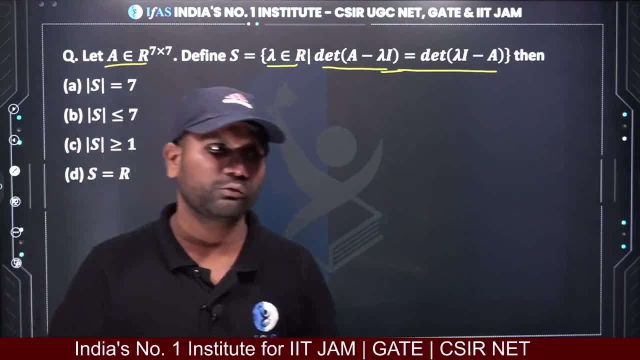 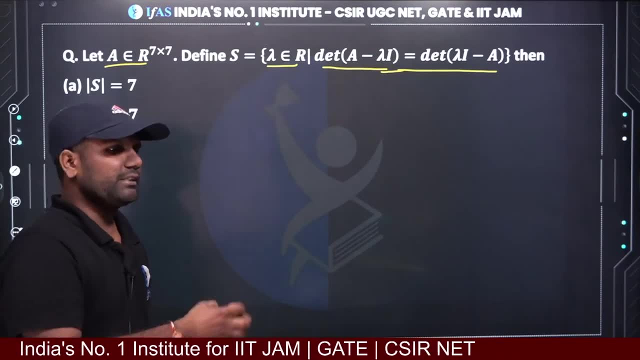 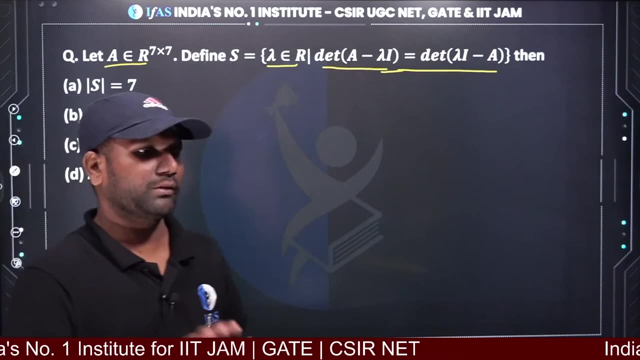 Tomorrow we will see diagonalization. JC form, quadratic form, inner product Means that once the important things that are completely linear are shown to you, Make you recall that you use this kind of counter example. apply this way. You should know all these things. Small results can help you in the exam. 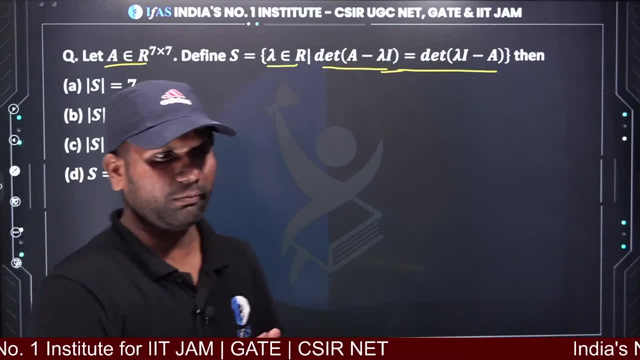 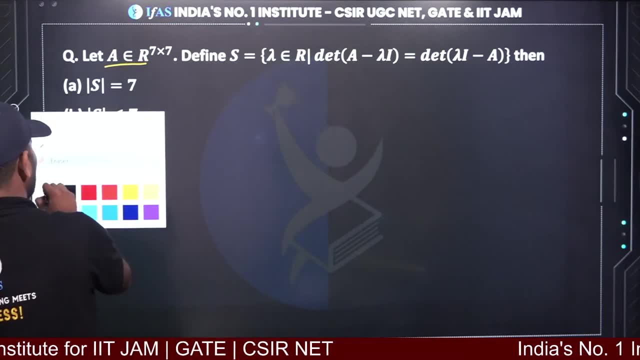 We are going to do all those things here. Almost everyone is saying B. So how did you do it? Tell me once, Why did you think of B? You must have something in your mind that this is why you thought of B. Something will happen. Why did you think? 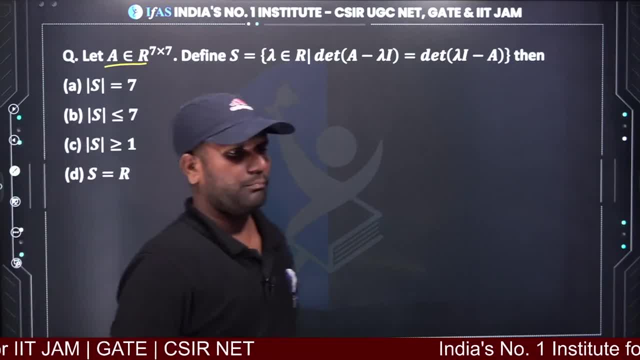 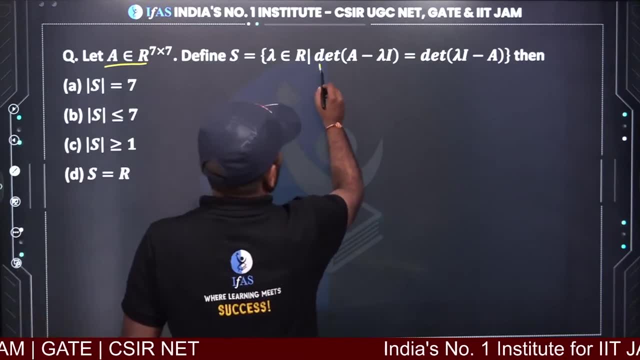 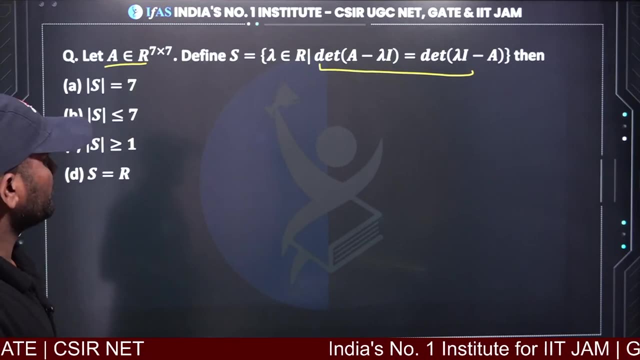 Come on Now. if you see here, why did you think of B? If you see here, what do you know? You have been given here that the determinant of this is equal to this. Now, what do we know? The order of the matrix is 7 cross 7.. 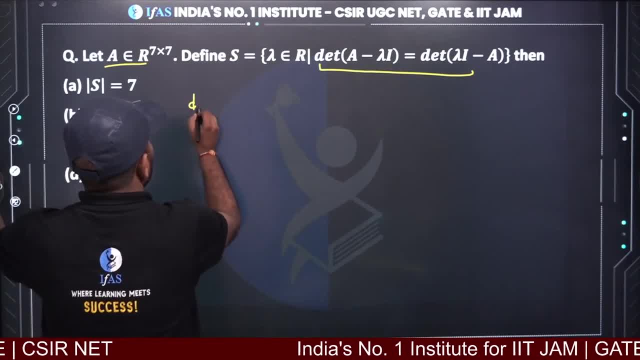 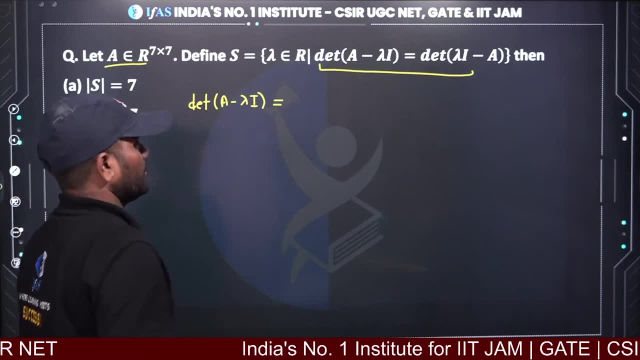 What is the order of the matrix 7, cross 7.. What do we know? Determinant of A minus lambda I. Determinant of A minus lambda I is equal to What have we been given? Determinant of Lambda I minus A has been given. 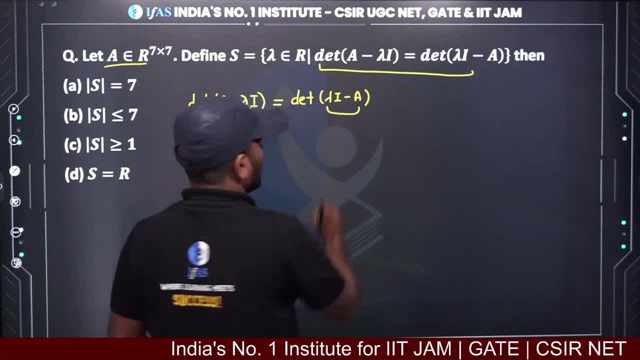 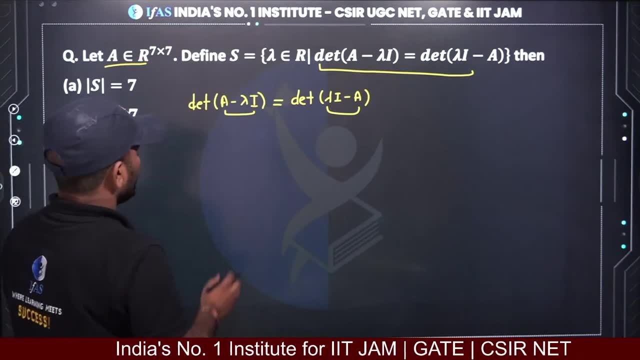 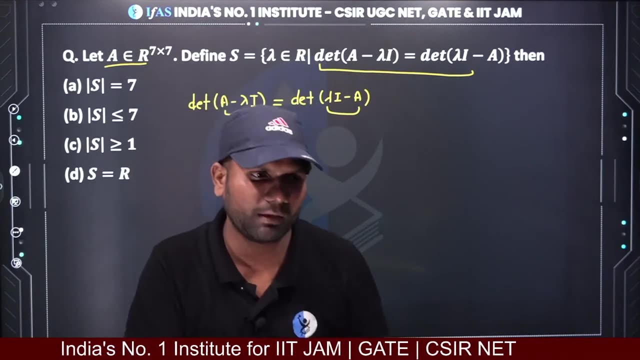 Keep in mind that there is a matrix. This is also a matrix- whose order is 7 cross 7.. 7 cross 7.. Now here comes one thing. Now see if I take minus 1 common from the determinant, If we take minus 1 common in the determinant of any matrix. 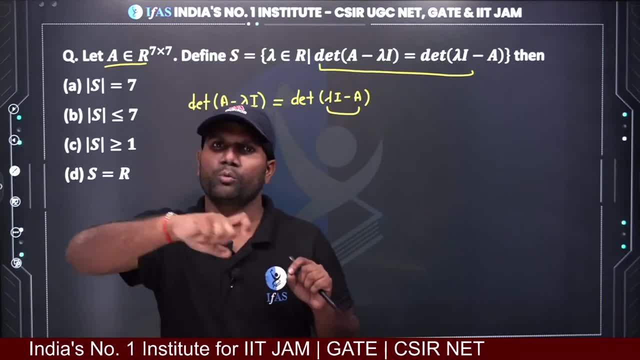 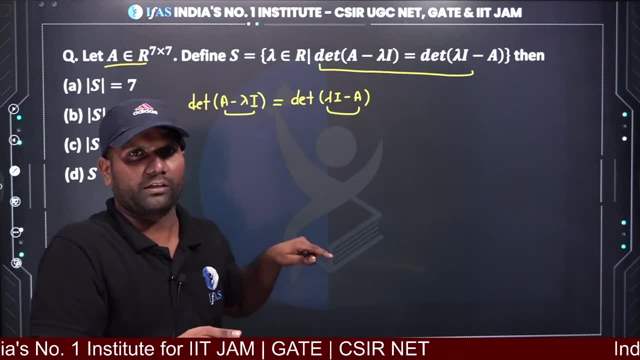 So what do we do? Either we will take common from the whole row or we will take common from the whole column, Is it not? What am I doing here? I am taking the minus 1 common from every row of this matrix, Because I am writing it upside down. 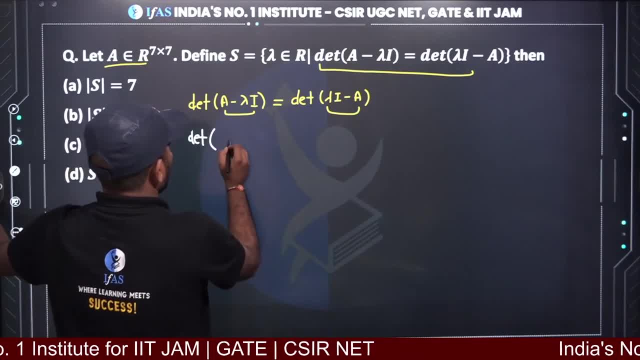 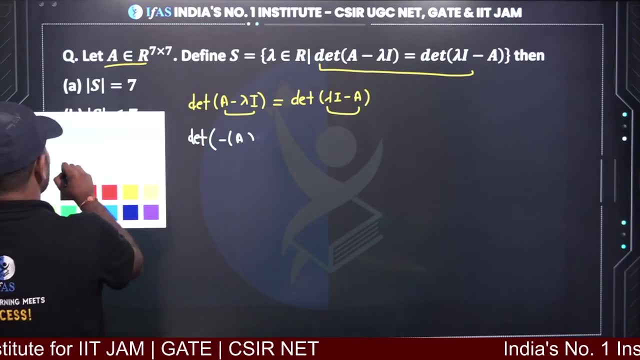 I will write it like this. That is, I am writing it like this. Determinant of A. I am writing like this: We are taking the minus as a common here. It will be A minus lambda, I minus A. I want to write it like this: 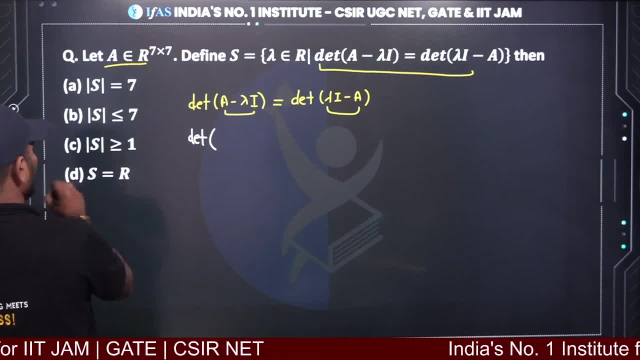 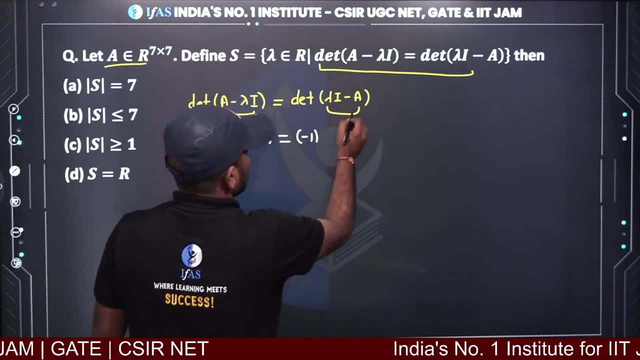 Or I can take the common from that side. I will keep it like this: A minus lambda I. I take a common from here. I will take the minus 1 as a common Minus 1.. It is a matrix of 7 cross 7.. 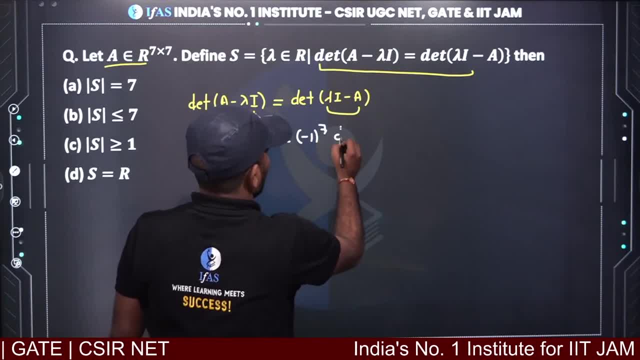 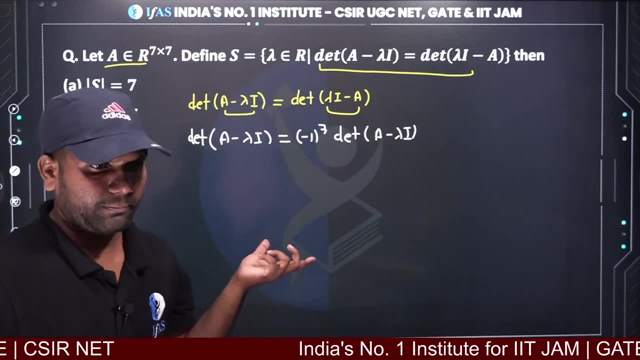 So every row will be common. This is A 7. And what will happen? Determinant of A minus lambda. I Did you understand this statement that I wrote here? Yes, Absolutely, Absolutely, Vijay, we had to apply the same result. 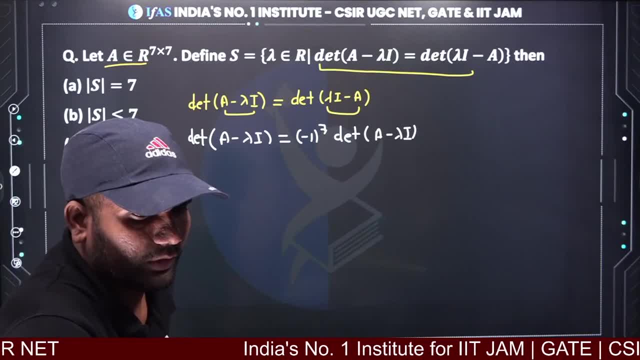 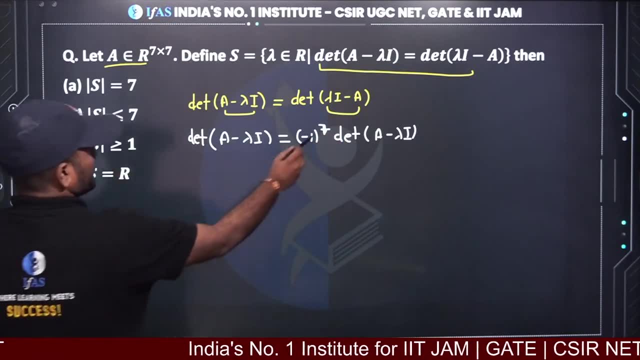 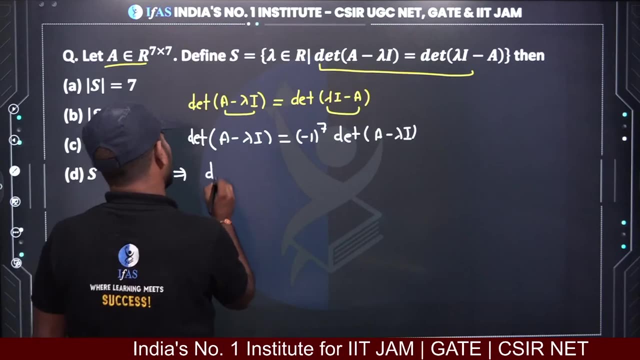 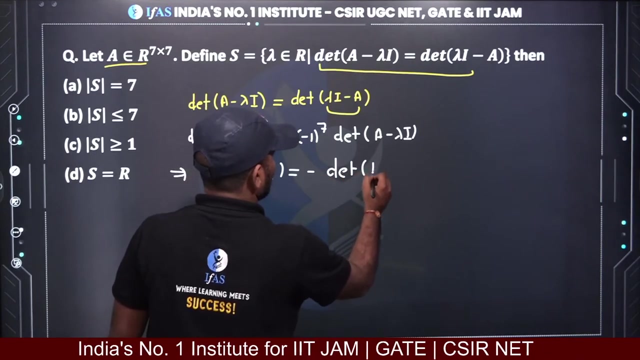 Yes, Absolutely, Asha. Yes, Absolutely, You can create it. Did you understand this one? How did we take it? Okay, Now see what will be the meaning of minus 1 raise to 7?. Determinant of A minus lambda I is equal to minus times. determinant of A minus lambda I. 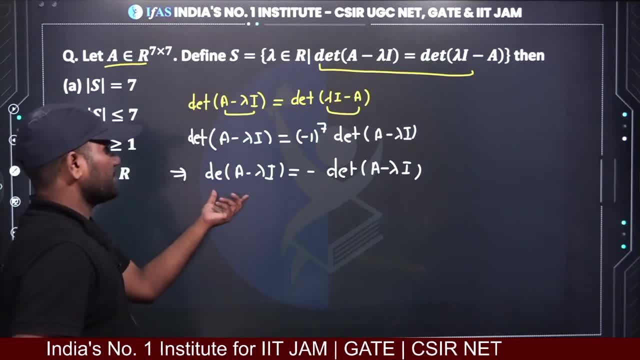 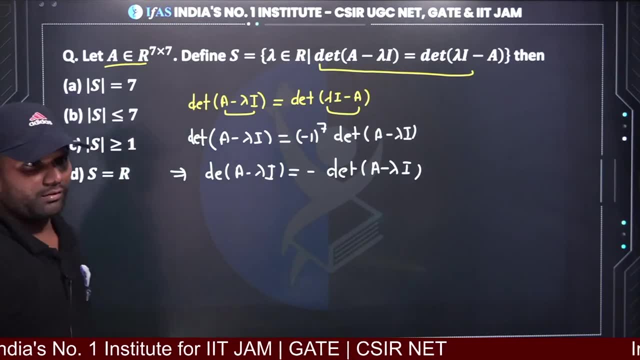 Now there are two numbers. There are two numbers, Such numbers. This number is same as the minus time of same number. When will this be possible? When will this be possible? This will be possible only when the determinant itself is zero. So determinant of A minus lambda I. 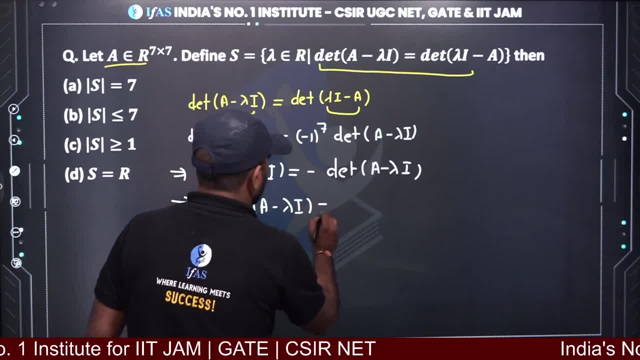 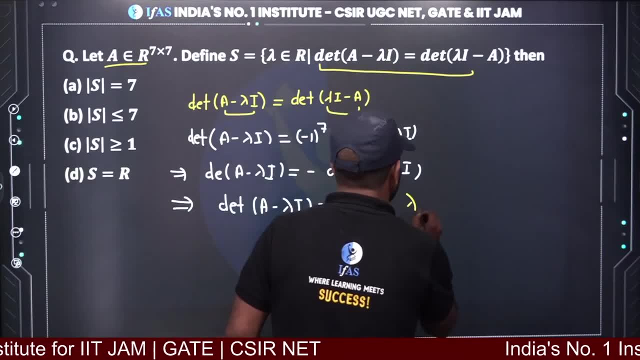 What will you get? You will get zero. When will the determinant of A minus lambda I be zero? If, and only if, lambda is an eigenvalue? If, and only if, lambda is an eigenvalue, What will be the lambda? It will be an eigenvalue. 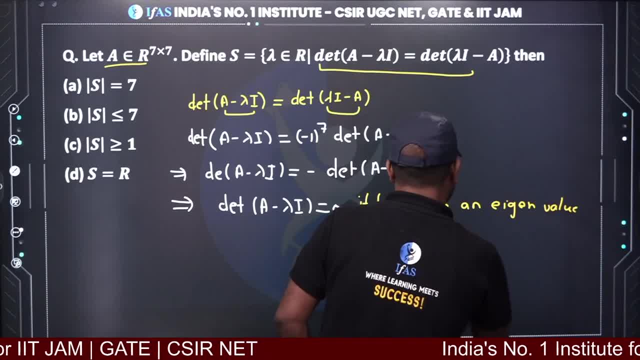 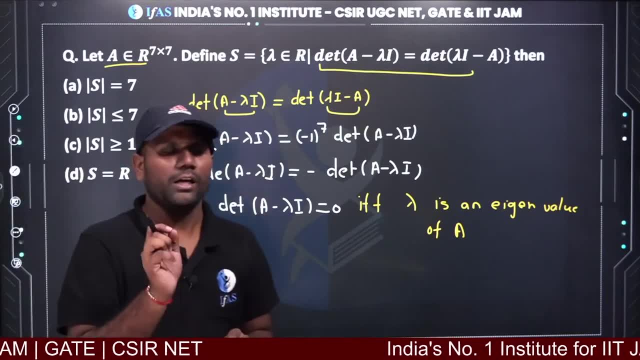 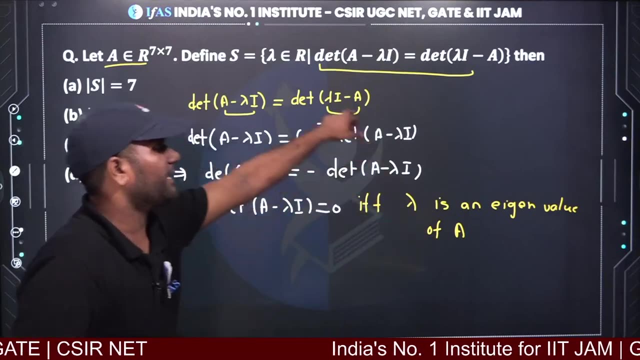 So from here, we get to know what we have been given. If we solve this condition, we will get to know the determinant of A minus lambda I, equal to zero. It means that what have we been given? We have been given that lambda should be its eigenvalue of this matrix. 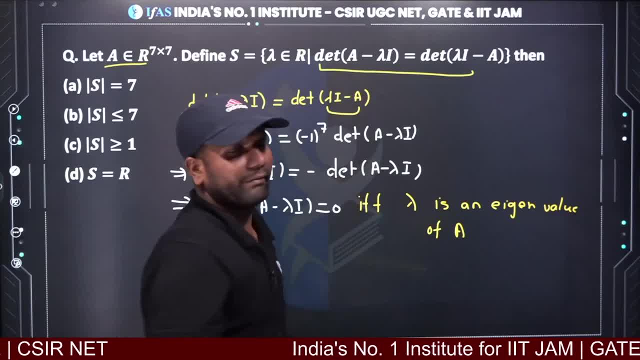 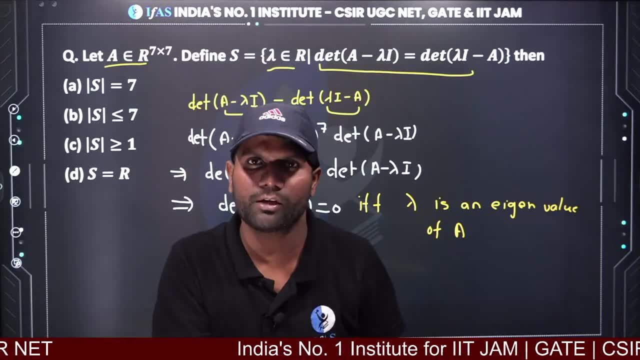 So see what kind of matrix is this? It is 7 cross 7 matrix. But we were asked what kind of eigenvalues of this matrix are Real eigenvalues? So it is not necessary that all the eigenvalues of the matrix should be real. 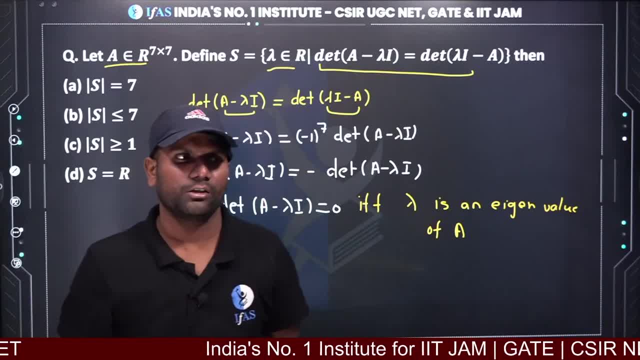 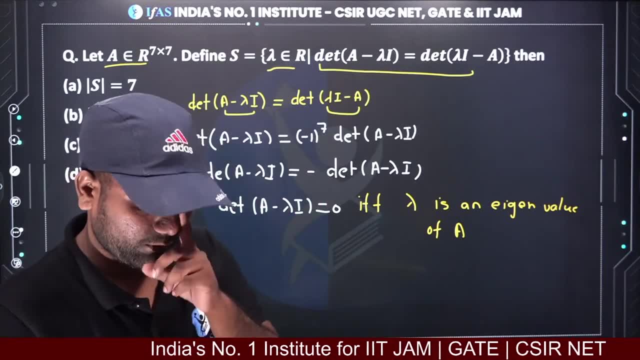 We can also get imaginary, but we have to keep it real here. So if we get real eigenvalues, then how many will we get? We will get maximum 7. Or it can be less than that. Naman- Naman has not been given to us. 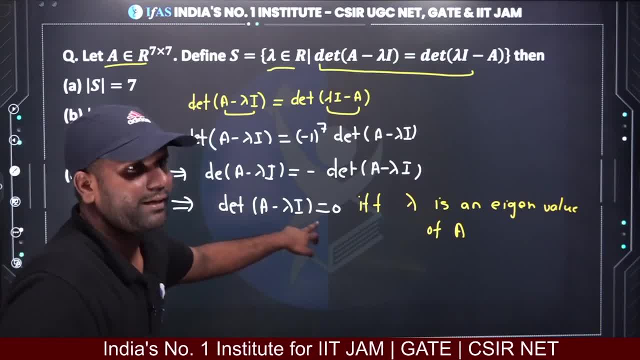 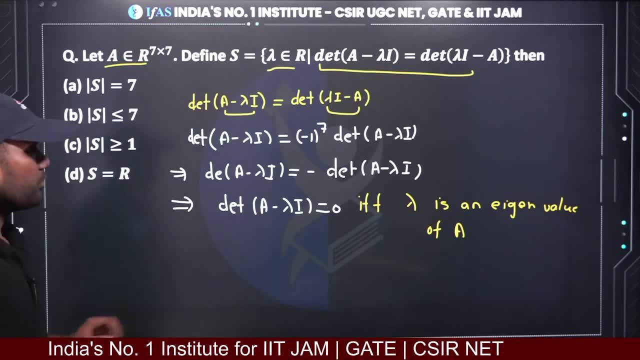 But what do we know? Determinant of A minus lambda I is zero if, and only if, lambda is the eigenvalue. This is the result. We have used this. So from here we get to know that in S, the cardinality of S will be maximum 7.. 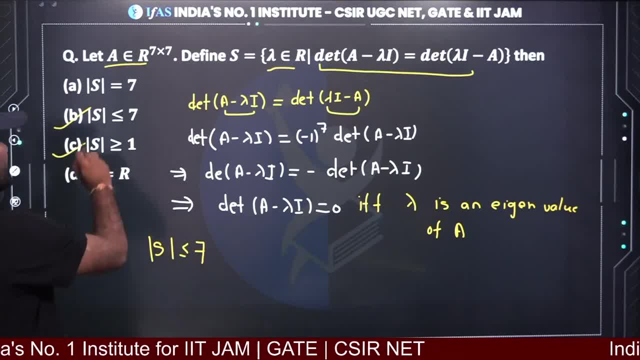 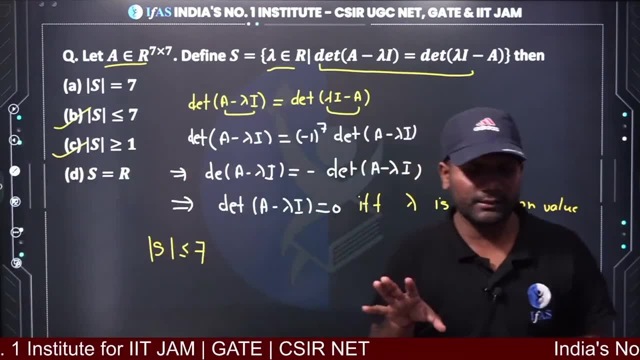 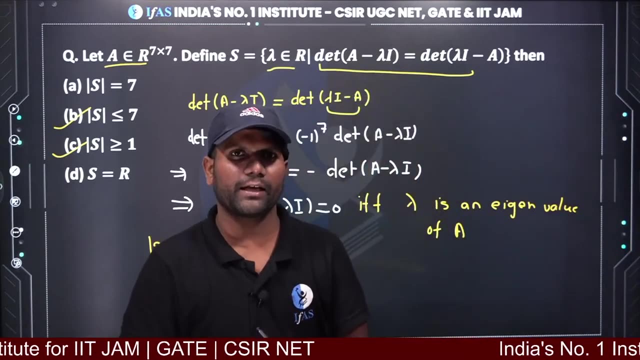 So option B will be correct here And option C will also be correct. It will be more than 1.. Okay, Did you understand? See, Can you see till here? If you have given a matrix, for that matrix the determinant of A minus lambda is zero. 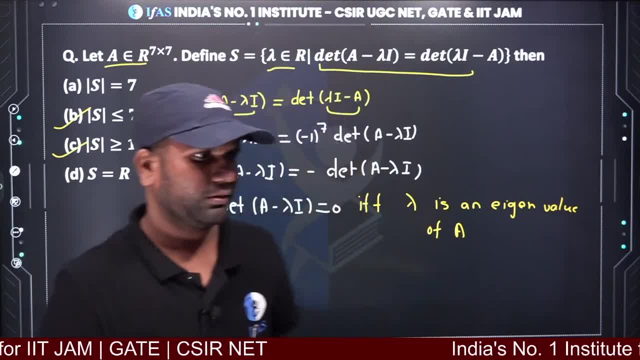 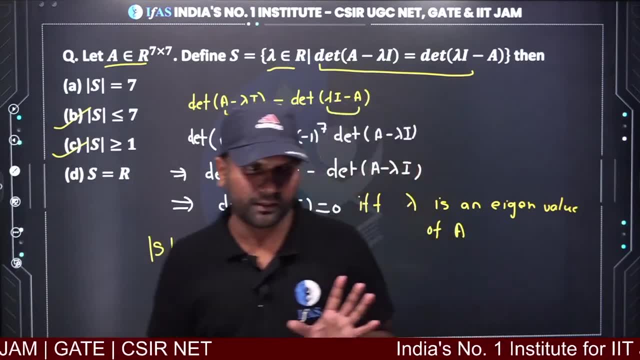 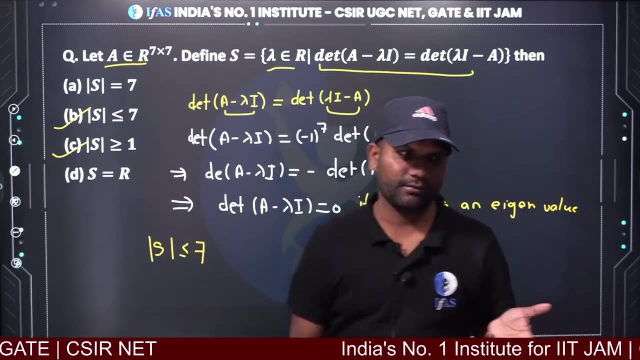 It means that lambda is its eigenvalue. B and C are correct for this question. Is it clear to everyone, or does anyone have any doubt? Good morning, Pallavi Rani. Okay, Is everyone clear? Let's go ahead. Let's go ahead. 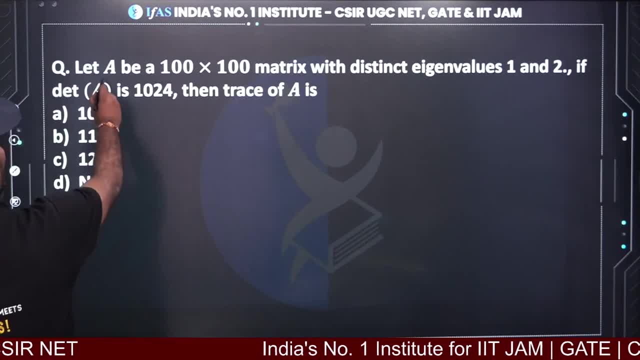 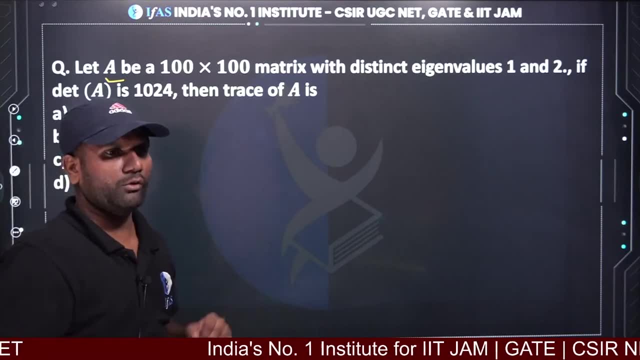 Yes, there is a good question here. Suppose you have given a matrix whose order is 100 cross 100. It has two distinct eigenvalues, 1 and 0. It means that its eigenvalues will be either 1 or 2.. 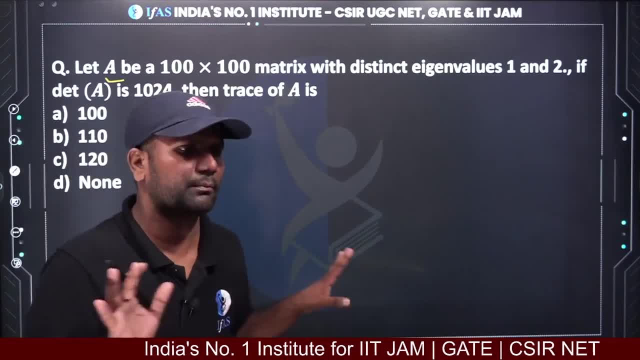 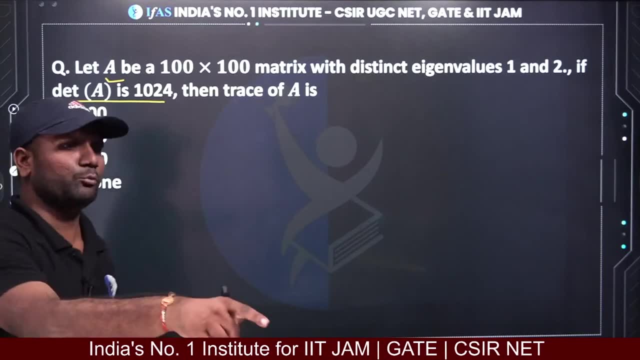 We don't know how many times either 1 or 2 will come, But we have been given the determinant of this matrix. The determinant of this matrix is A. You are being asked to tell its trace. What will be its trace? Yes, 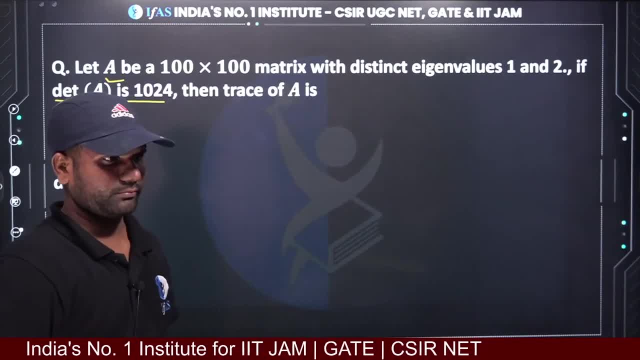 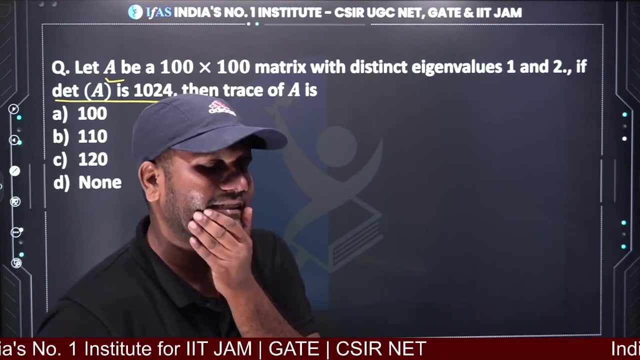 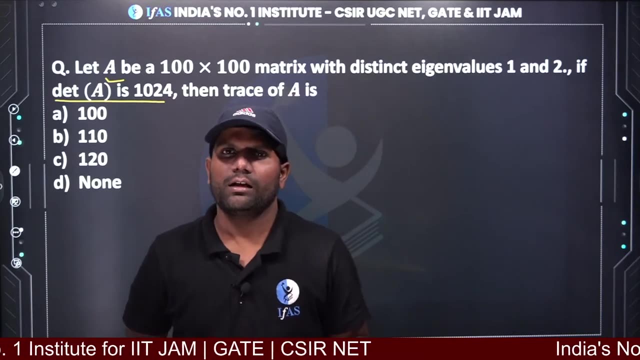 What do you think? What will be its trace Alpha? this does not happen. See, if you were given a real polynomial, then it is possible that all its eigenvalues will be real, Or there is an odd degree here, So at least one real will be found. 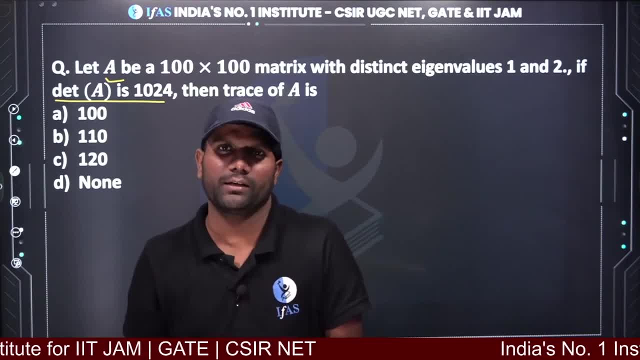 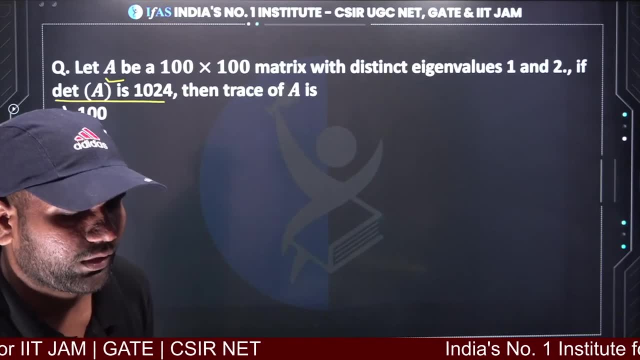 Guarantee of getting one real. Either it becomes completely real or some imaginary is found. From here we come to know that there will be more than 7. Or it can be less than that. Yes, we can say magic only then. Still, there are more than 6 real eigenvalues. 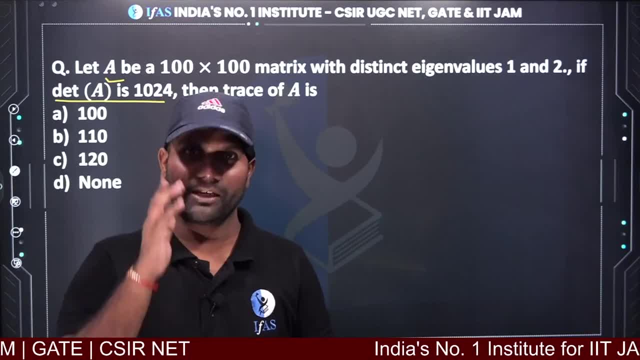 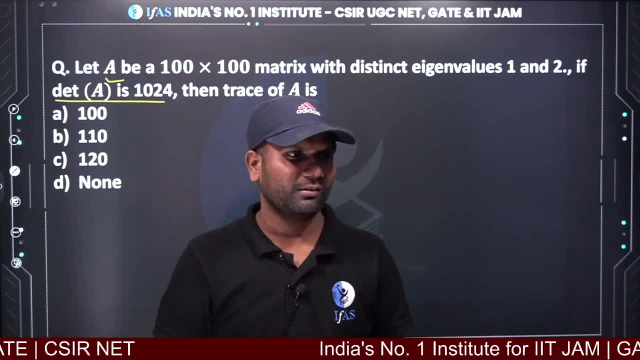 If there were 6,, then we would not be able to say: Then we would not be able to say: Then we can say magic math only when we take the determinant equal to the odd. Until you take the odd, there will be no zero. 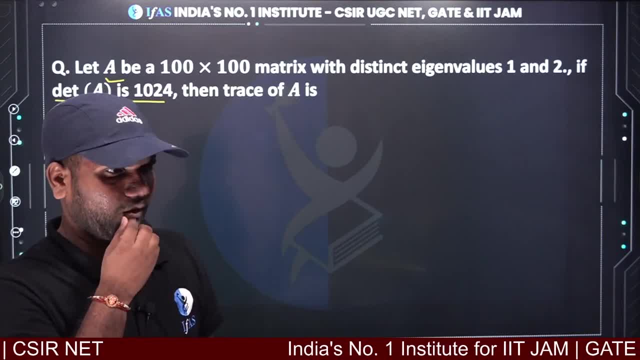 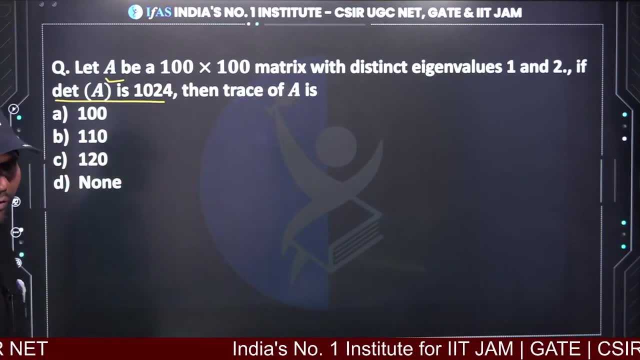 Do you understand In the odd case we would not be able to say in the even case: Ok, tell me about this, Tell me what will happen. Almost some people have given the answer. Vijay is saying that this will happen. 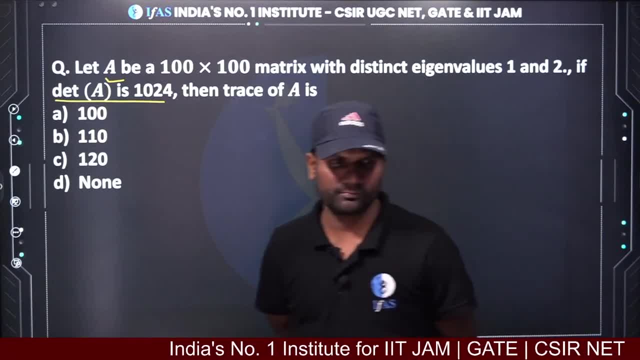 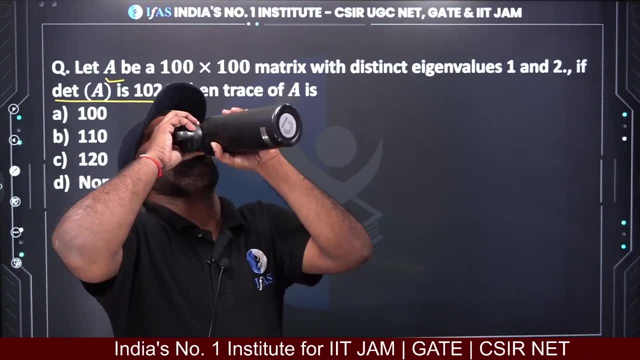 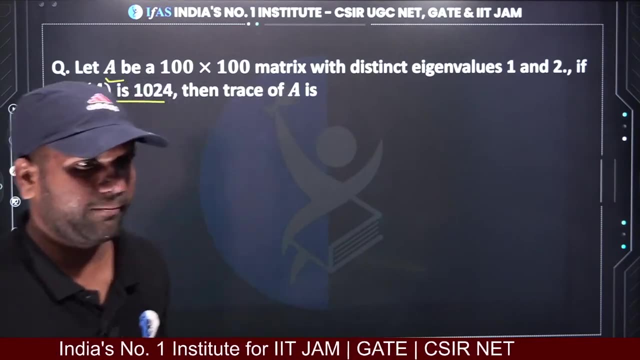 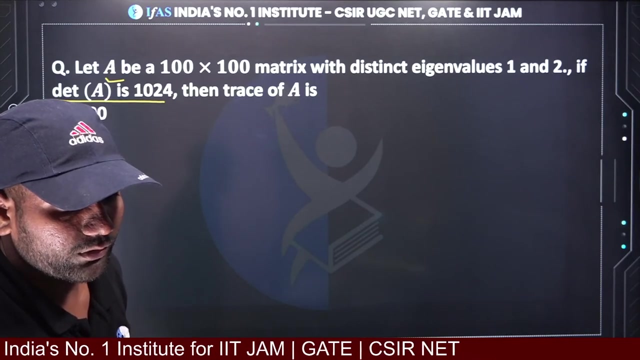 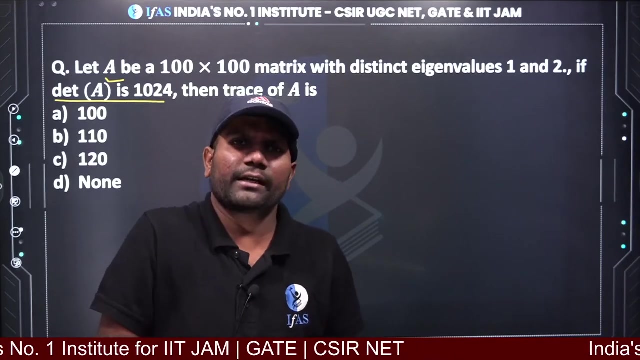 The rest of the people. tell me. Vijay has already told you. What are you saying? Ok, Come on, tell me. Yes, I mean there can be real alphas. There will be more than 7 real Either. it may not be real and imaginary will also be found. 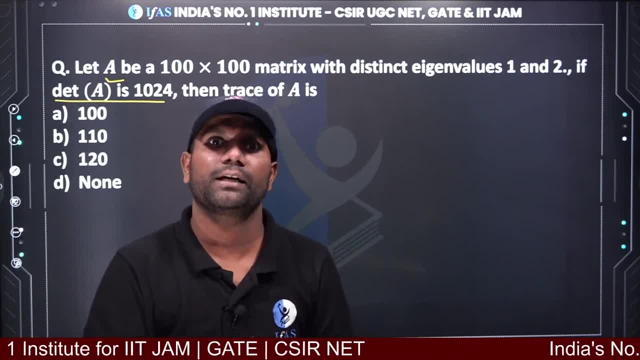 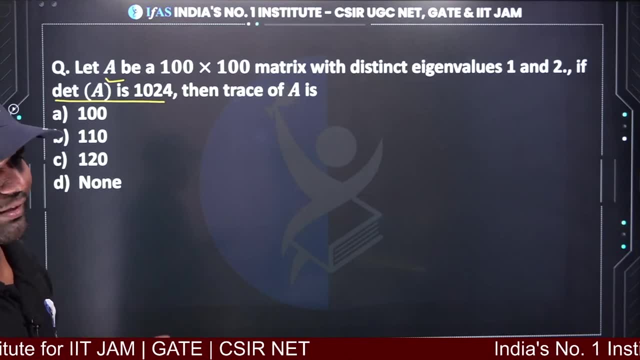 But there will be more than 7 real. We were asked how many there can be. We said there can be more than 7.. Ok, Almost everyone is saying B, Amerindra has said C, Vijay has said A And the rest of the people tell me. 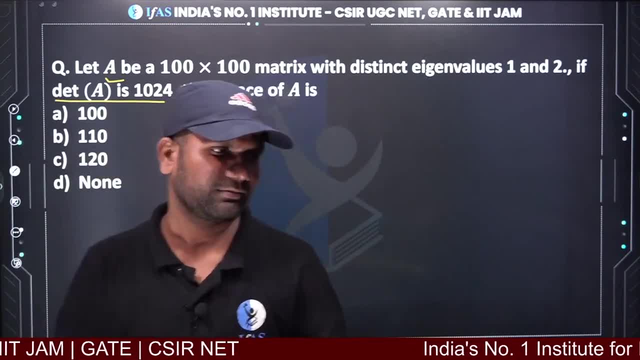 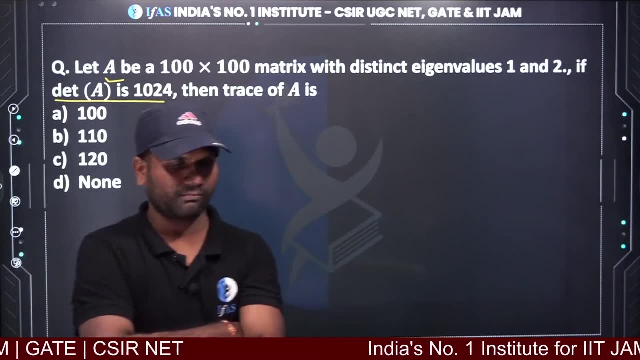 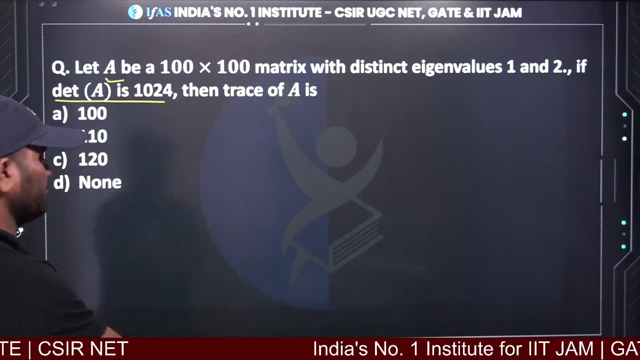 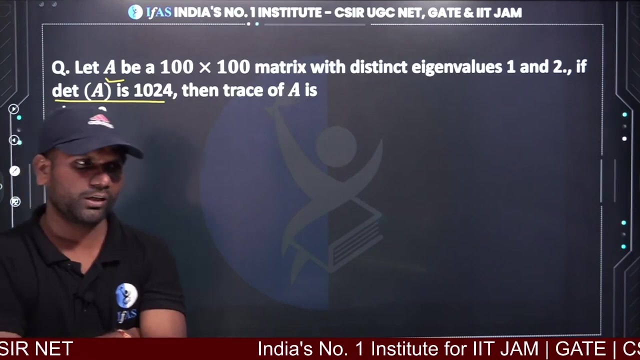 The rest of the people are not saying anything. What's the matter? Asha is saying 1110,. let's see, I also feel that it will be 1110, but come on, I will take a comment once and then I will try. 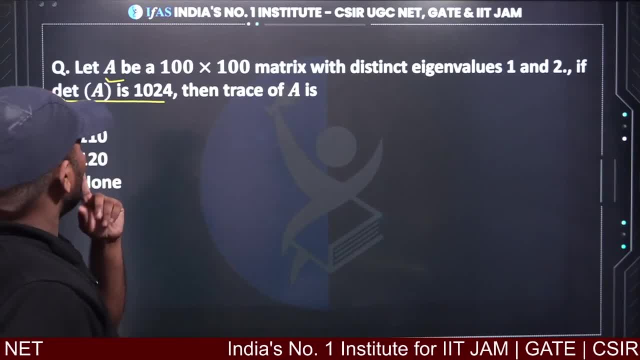 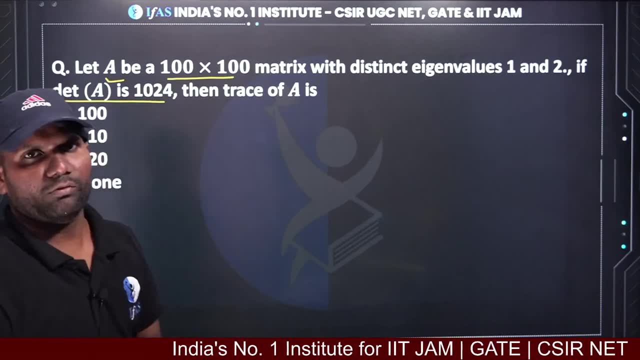 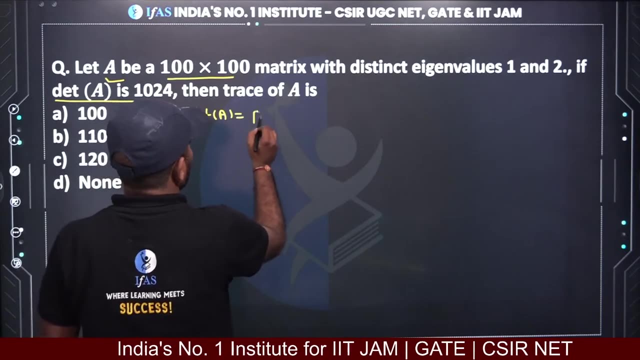 now see. the first thing is that we have been given a determinant. now, if you observe here what is the matrix, the matrix order is 100X100, and what is determinant? you are given a determinant is equals to what is a product of eigenvalues. When you multiply the product of eigenvalues, you get the determinant. 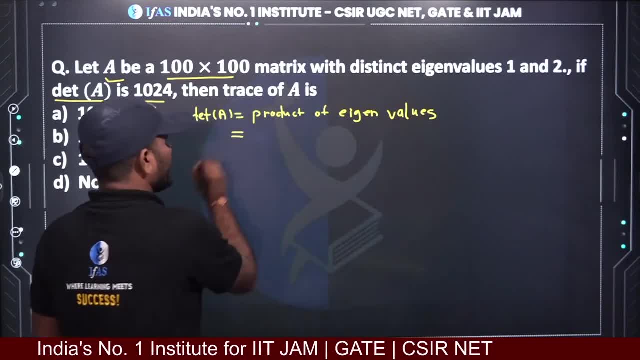 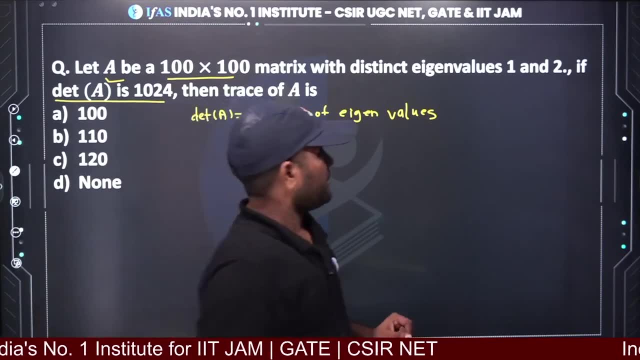 now, if you multiply the eigenvalues you will get 104, ie the eigenvalues are either 1 or 2, is 1 or 2, then we can diyor1034. remember that all the IP address. in the στο. you should also give some zero. 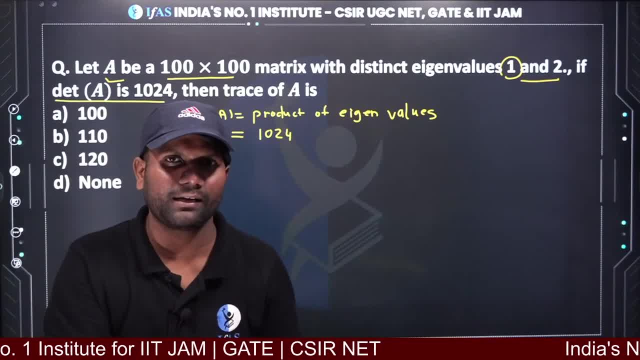 basically all are the same, since ym 18029 also include the initial price, which means values are also the same. when you multiply as many times as you want, then 1 will not make any difference. 1 is 1 only. it will not make any difference. 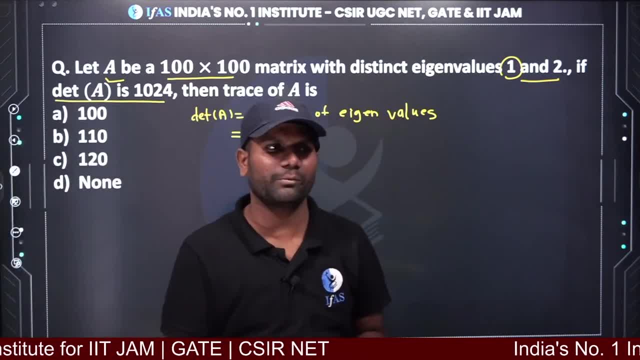 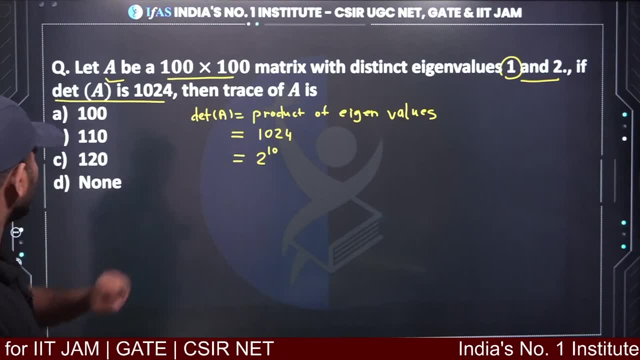 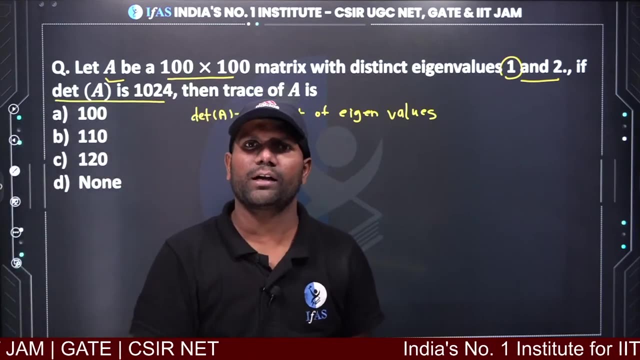 means the difference that will make in the determinant is 2, so we can write the determinant as 2 raised to 10. this is 2 raised to 10. this means if I take the 10 eigenvalues of this matrix as 2 and take the remaining 90 eigenvalues as 1, 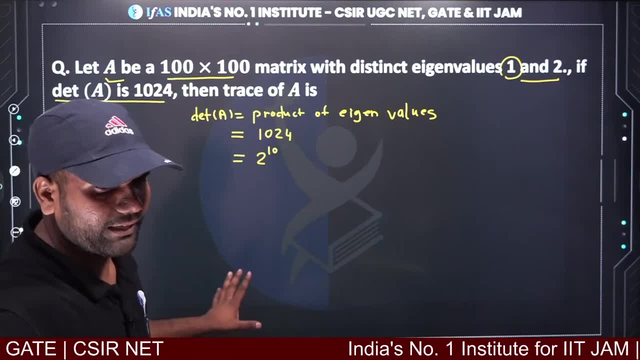 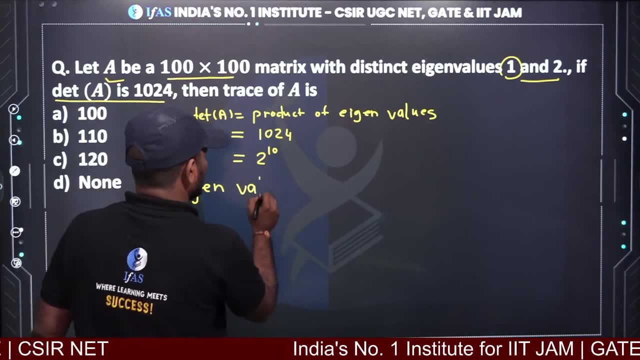 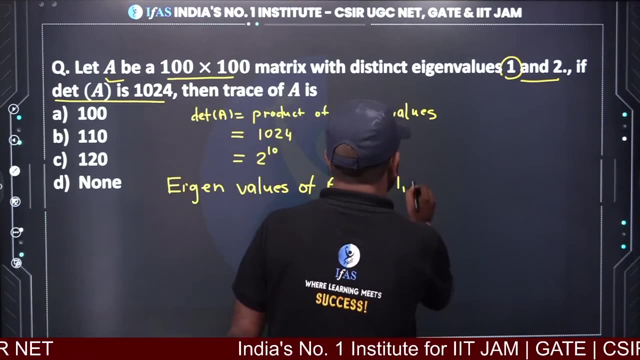 then this will be the determinant, isn't it? so from here we can say: eigenvalues, eigenvalues of ar. so what eigenvalues of a will you get? so eigenvalues of a are 1,, 1,, 1,. how many times 1 has come? 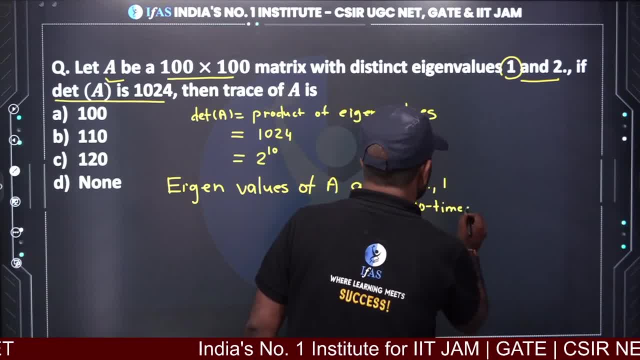 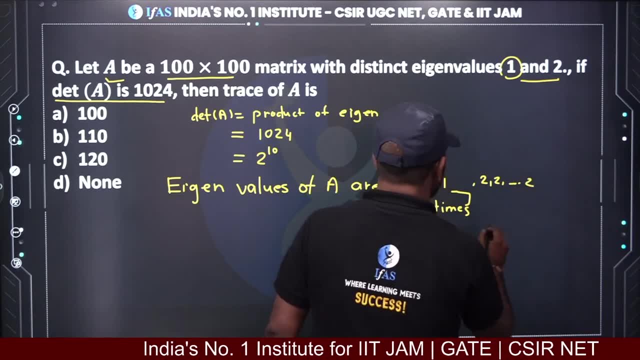 90 times. 90 times it has come here. and what will you say? how many times 10?? 2,, 2 and so on. 2? how many times 10?? sorry, how many times 2 has come 10 times? 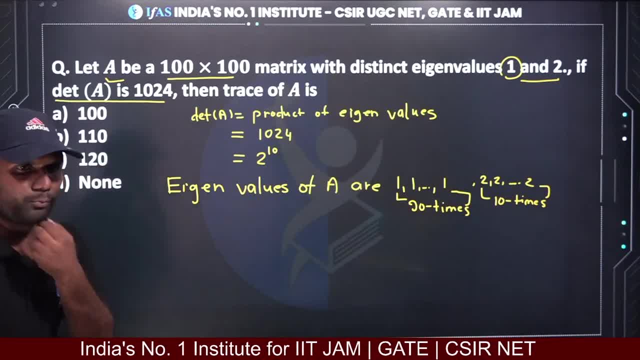 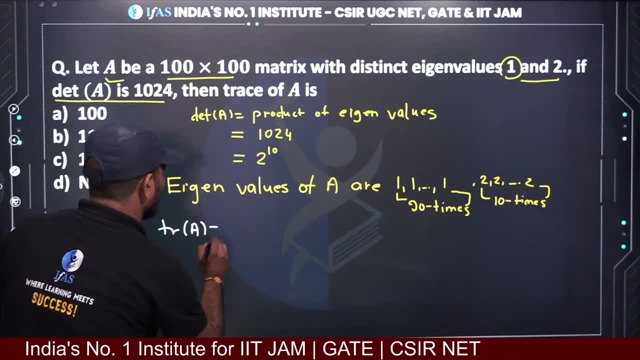 you got this, its eigenvalues. what did you ask us? we are being asked about trace, we want trace. so come on, we have to find trace. so what will be trace of a sum of eigenvalues? so 1 plus, 1 plus, and so on, plus 1. 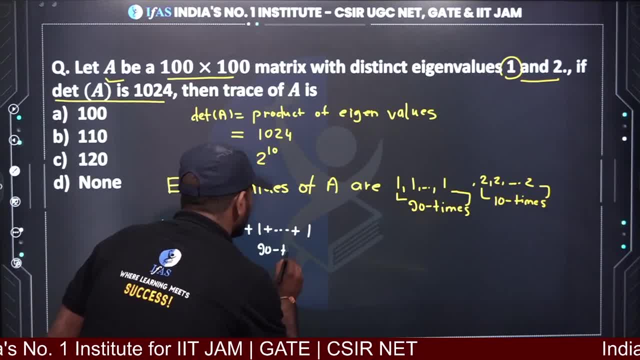 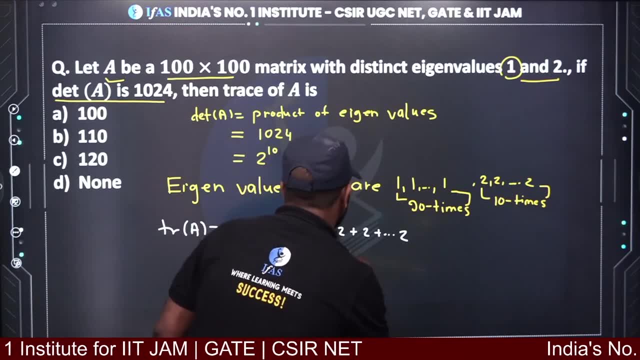 how many times you have added this? you have added this 90 times. ok, this is 90 times. and here plus 2, plus, 2, plus and so on: 2, how many times it has come? 10 times. so you can simply see from here. 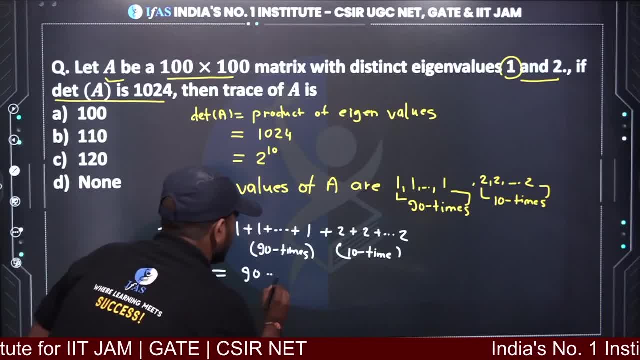 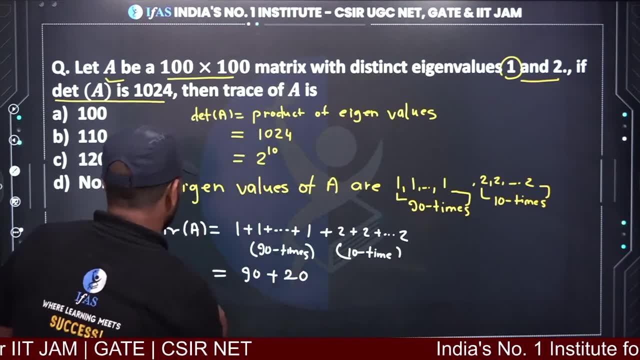 what will you get? first one will be 90, second one will be 40. sorry, add 10 times 2, it will be 20. so what will you get? you will get 1, 1, 0. so the correct answer of this question will be: 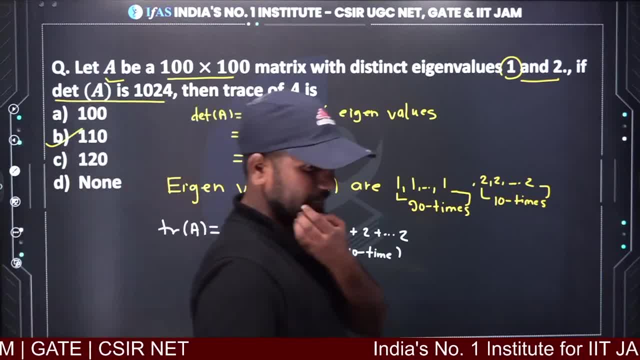 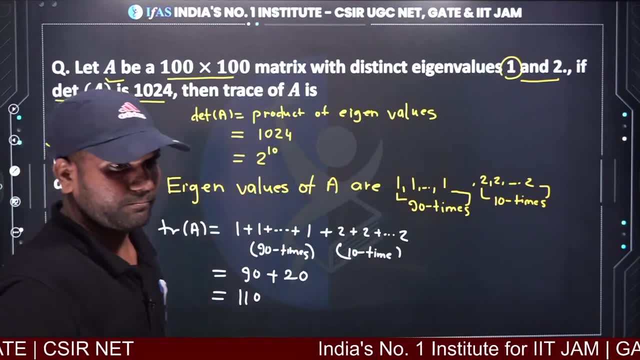 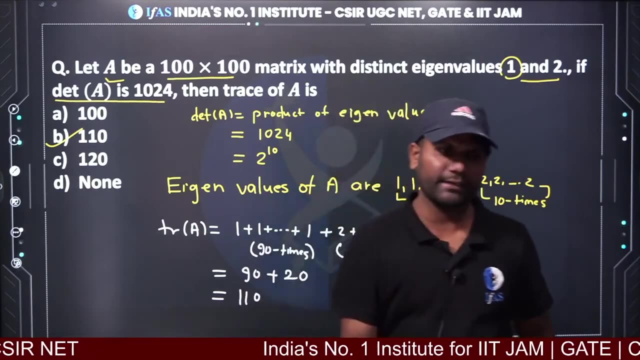 110. everyone understood. see, its correct answer is 110. right, come on. I hope you all got it clear. you must have understood and new people who are still connected. if you did not like the session, then like it if you are new to the channel. 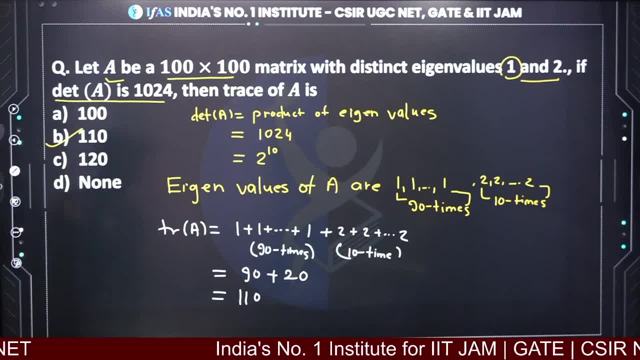 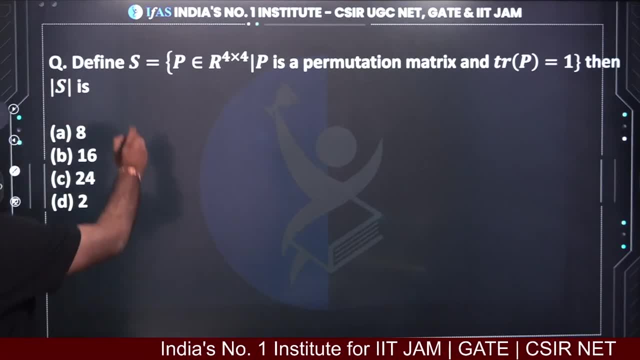 then subscribe to the channel. ok, let's go to the next slide. I hope you will be clear here now. what can you say about this matrix? see, what did we get? we got a matrix S. I am thinking. I will give you time to think about this question. 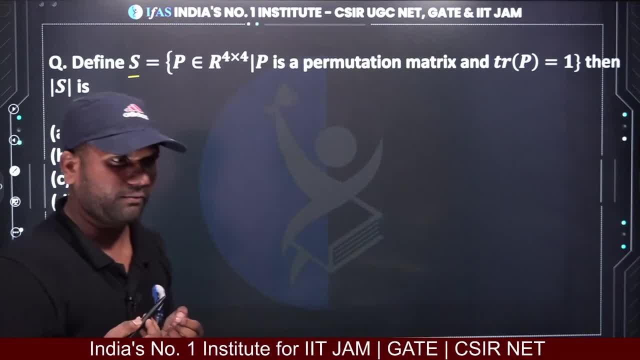 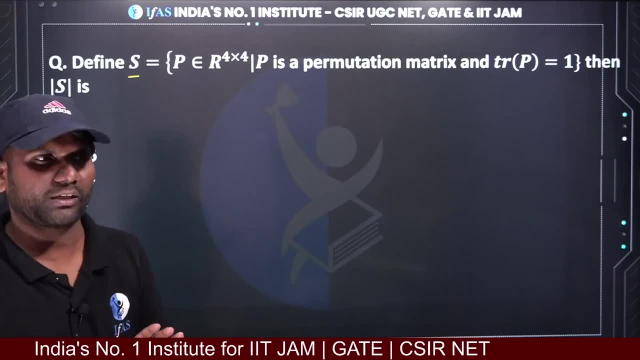 tomorrow you will tell me the answer. ok, see the matrix. I will tell you the question once and I will give you a hint what to do. here a little group theory is used. ok, here, what did you get? P, 4, cross 4 matrix. 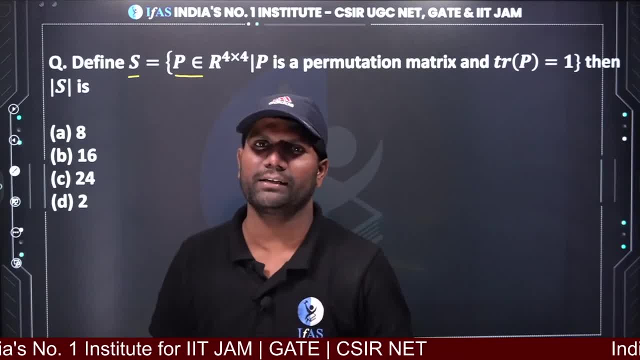 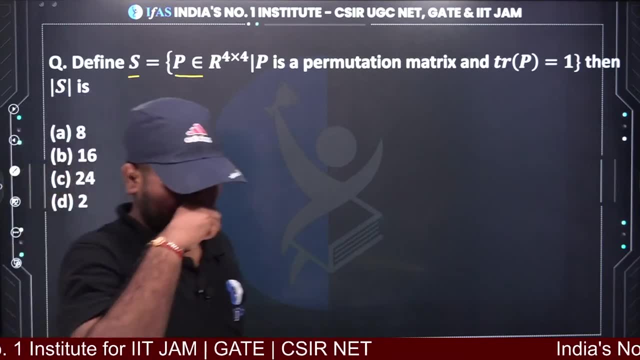 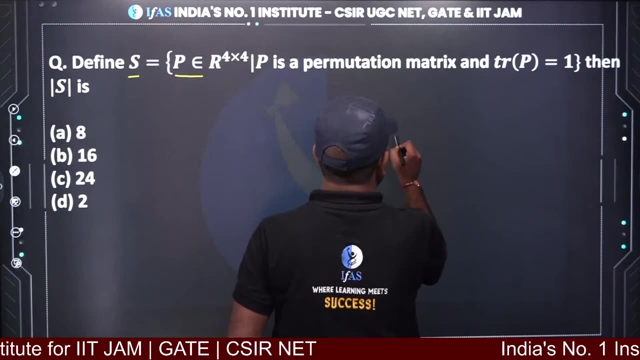 which is a permutation matrix. but such a permutation matrix whose trace is 1, ok, whose trace is 1. so you have to tell how many elements will come in this. see, what is the trace of permutation matrix. we did permutation matrix last time, so what is the trace of permutation matrix? 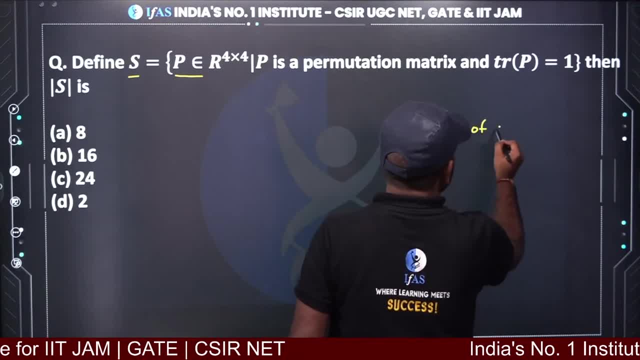 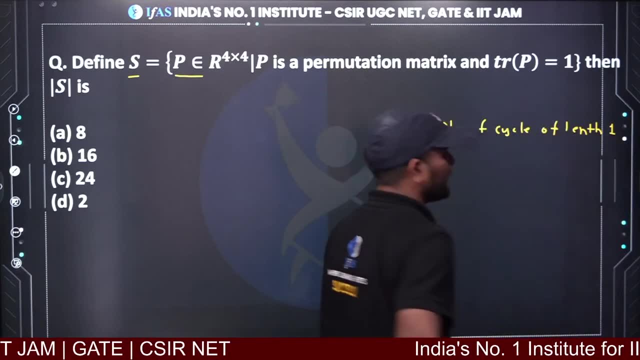 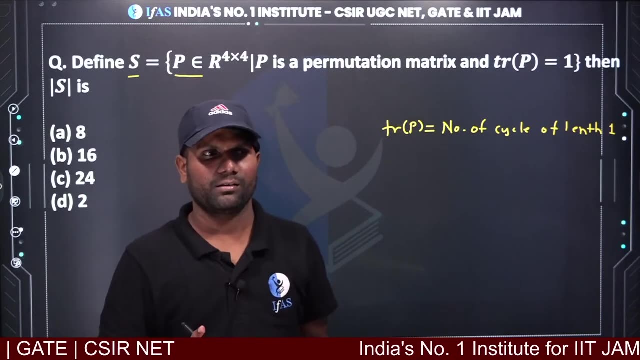 trace of permutation matrix is number of cycle of length 1. so the number of cycles of length 1 is the trace of permutation matrix. its trace is 1 means you have to find in S4. in S4 how many cycles will be sorry cycles, whose CD is 3,1. 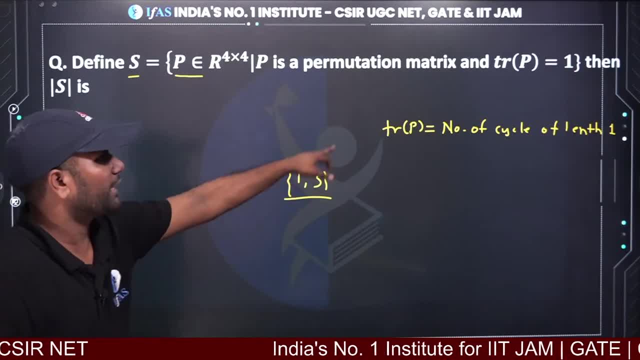 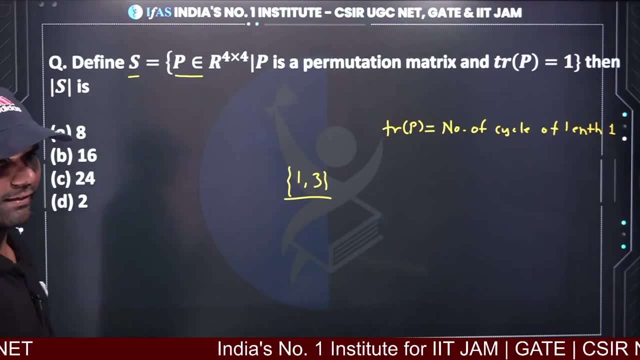 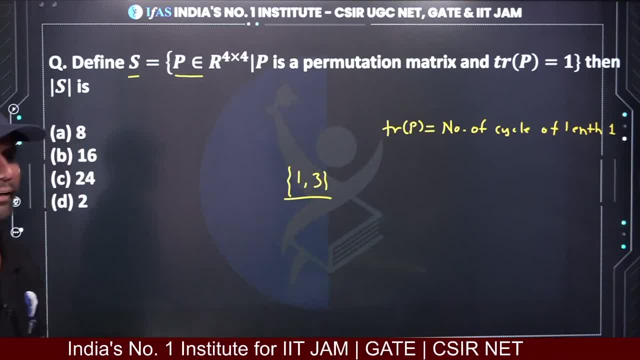 3,2, 3,2, 3,1, 3,2, 3,2, 3,2, 3,2, 3,1, 3,1. we will discuss it in the next session. ok, now here is one more example. 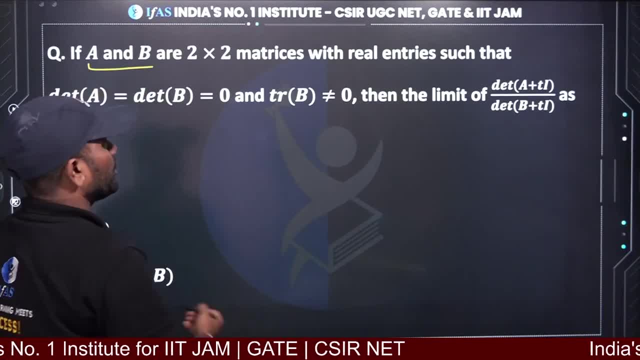 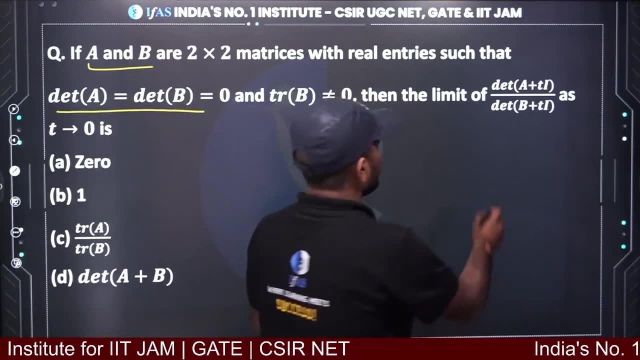 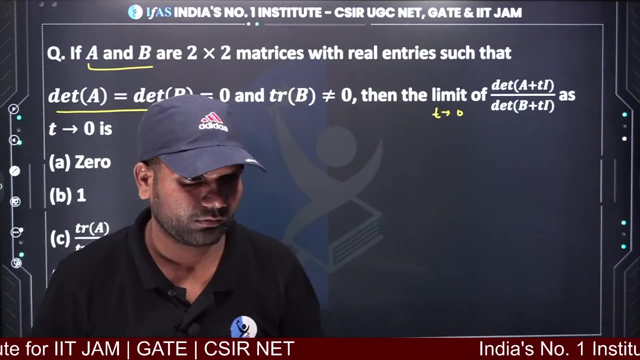 what is given here? if A and B are 2, cross 2 matrices with real entries, where determinant of A and B are 0, trace is non-zero, so you have to find the limit of this term. as t tends to 0, what will happen, tell me? 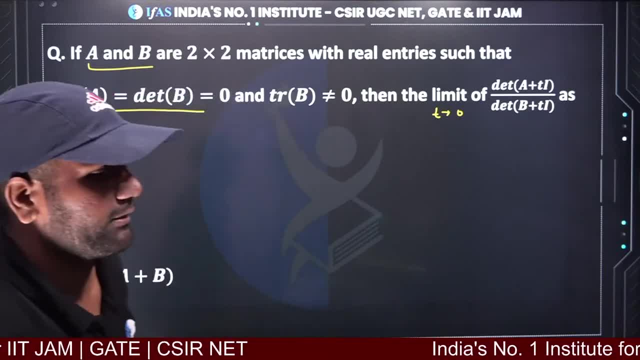 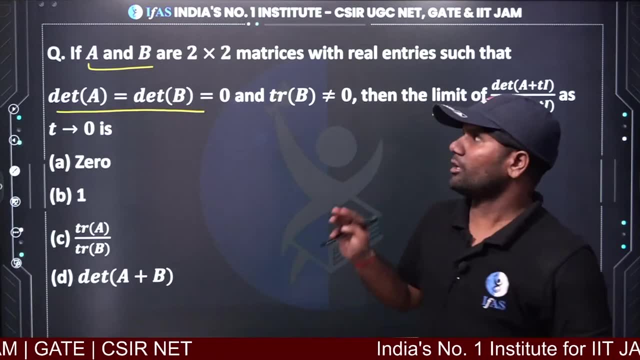 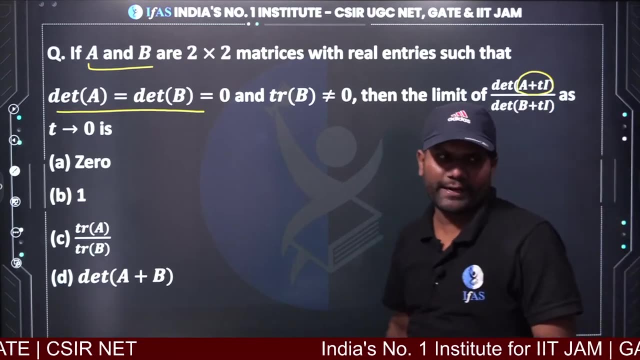 yes, absolutely. you can say like this: ok, tell me the answer, how to solve this question. so here, what is given? determinant of A minus t i. so we know that determinant is product of eigen value. so first of all, find eigen value of A plus t i and B plus t i. 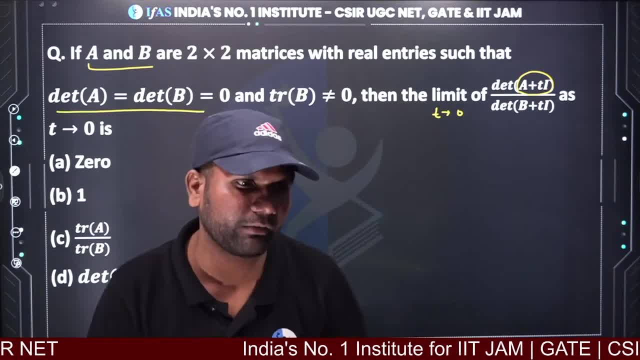 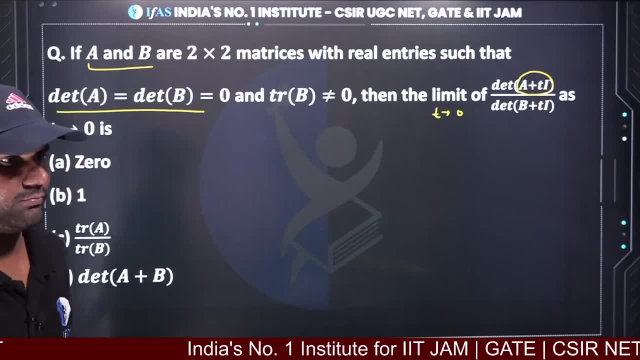 if you have determinant means, product of eigen value, then it will be easy for you, right? yes, aunt, very good, is it not? it will be easy for you to solve. ok, tell me what will happen. none of you are afraid of diagonalization. quadratic form jc form: inner product. 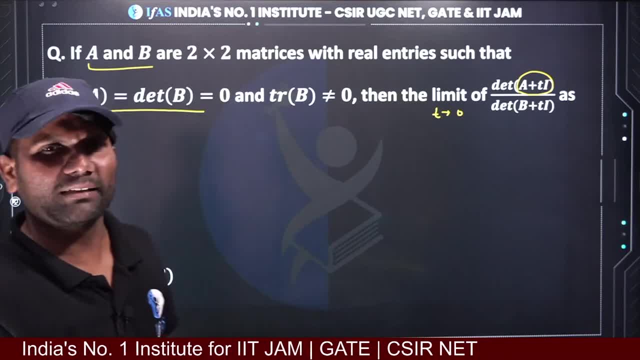 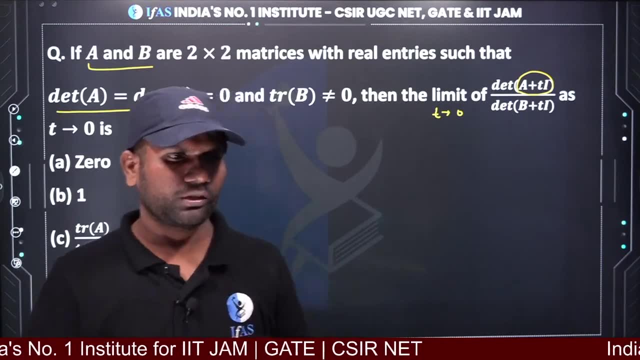 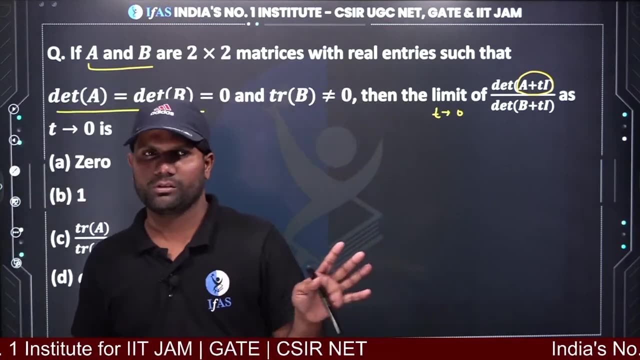 right, there is nothing to be afraid of. it is a very simple topic and it is a small and easy topic means it is interesting. so tomorrow we will do this topic. ok, what topic? jc form, quadratic form, ips and our A. what is left? inner product is done. 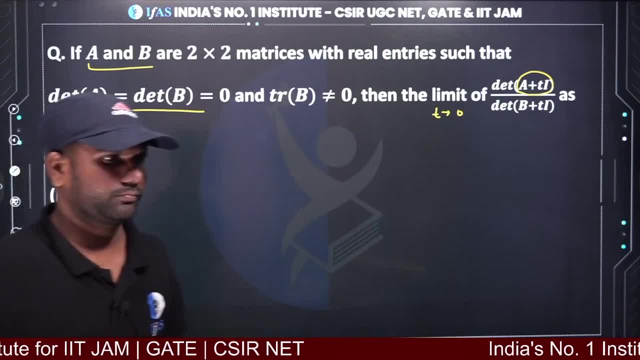 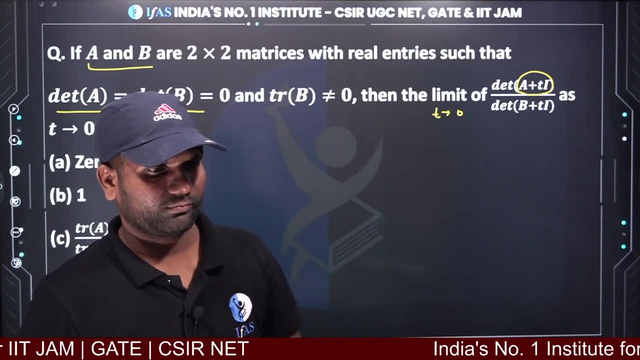 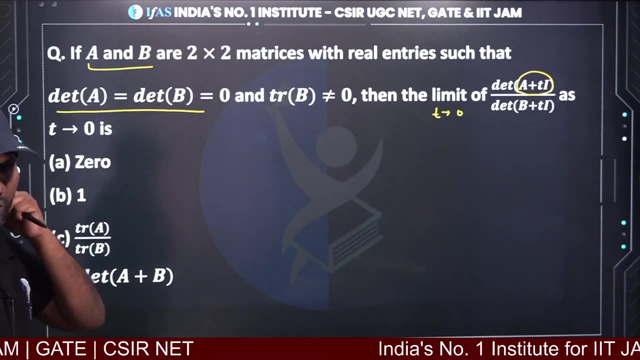 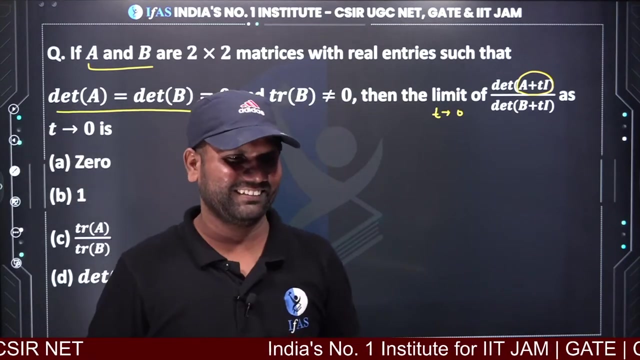 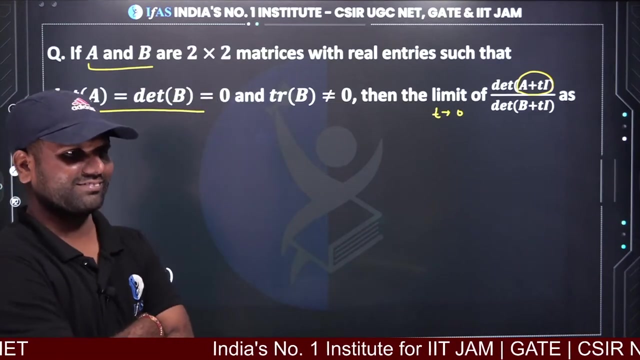 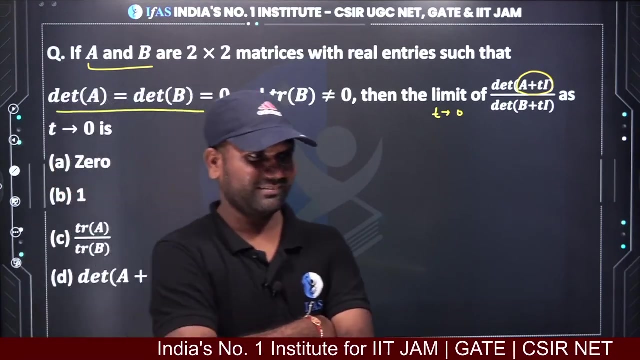 ok, diagonalization does not seem. yes, very good. ok, now someone tell me the answer of this. you all are telling me its B, B and C. you all are telling me we are afraid of ips. ok, ok, you will feel. ok, ok, ok, ok, ok, ok. This is a very simple question. 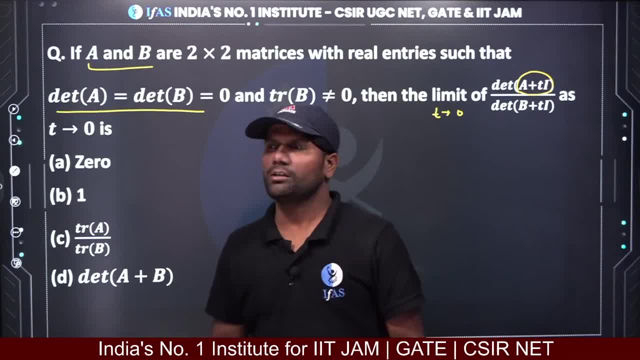 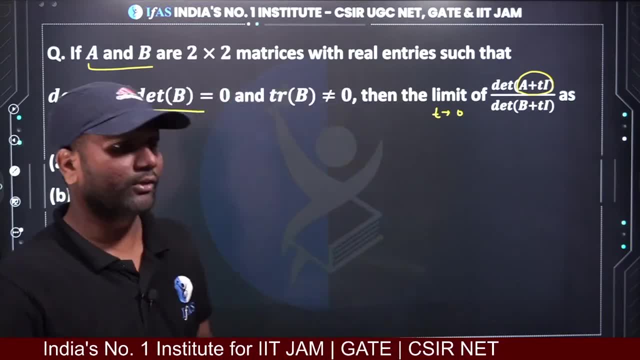 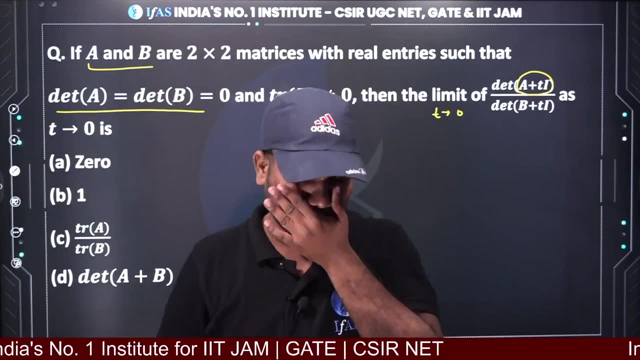 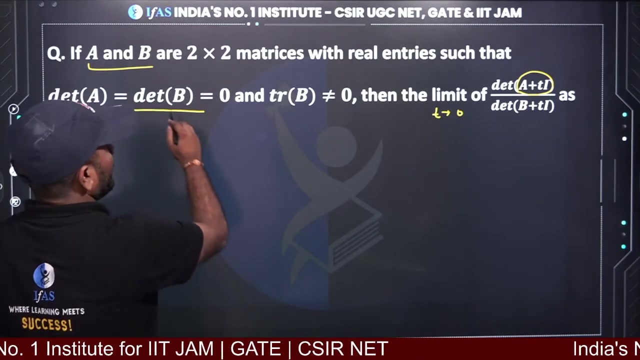 Hint for you is: find characteristic polynomial for matrix A and B And for 2 cross 2, we did a result in the start. use it. If you use it then it will be easy for you. You are applying L hospital Now. see here we know characteristic polynomial of 2 cross 2 matrix is: 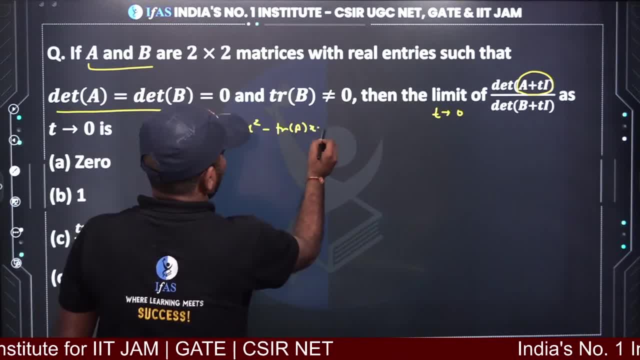 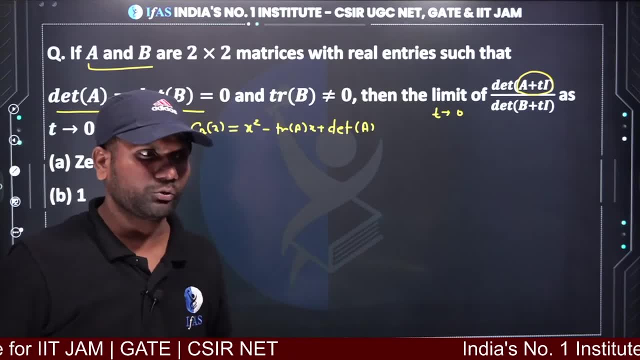 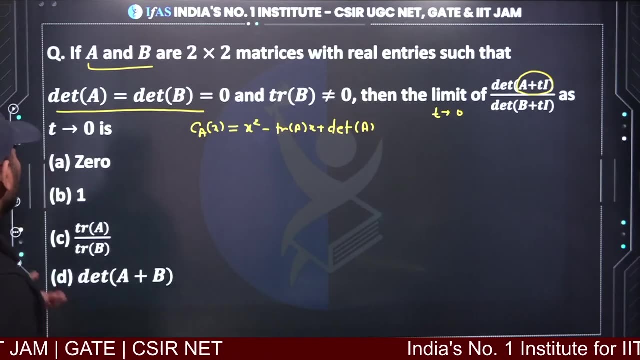 X square minus trace of A into X plus determinant of B, Determinant of A. we will use this result. If we have the result, then sometimes we should also use it. Vijay, try again. maybe there is some mistake. Yes, absolutely correct. Now if you see here: X square minus trace. 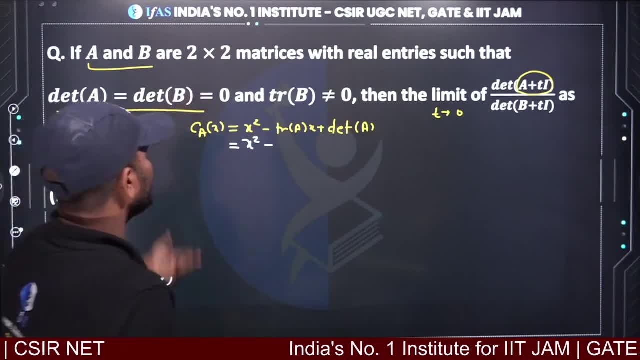 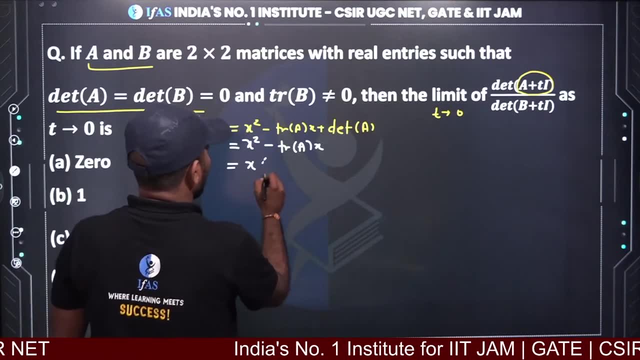 What is the trace of A? Trace of A is not given to you. Trace of A into X determinant is given 0. This is 0, so what will you do from here? X and X minus trace of A, So it got 2 eigenvalues. 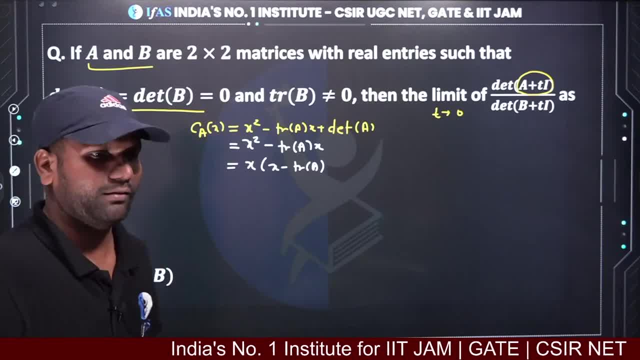 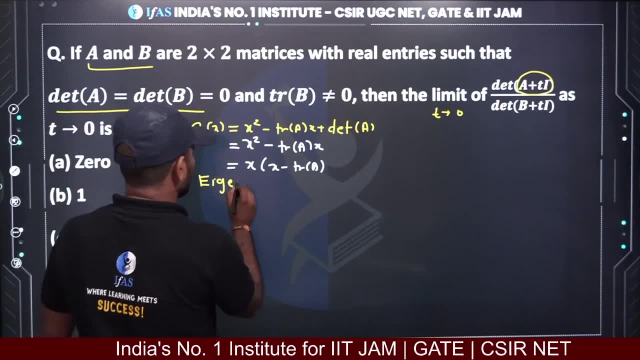 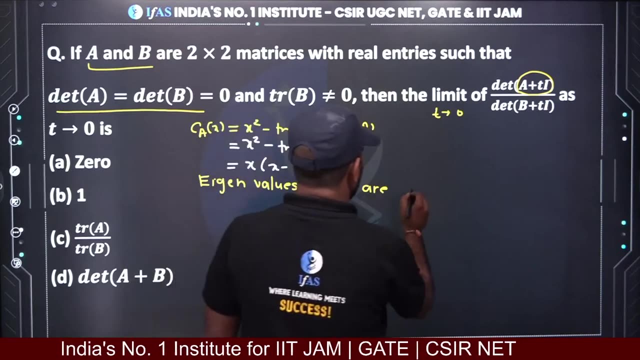 So eigenvalues of A are 0 and trace of A. It got 2 eigenvalues, which ones You can see. Eigenvalues. Eigenvalues of A are: What will be the eigenvalues of A? Eigenvalues of A are One will get 0, the other will get trace of A. 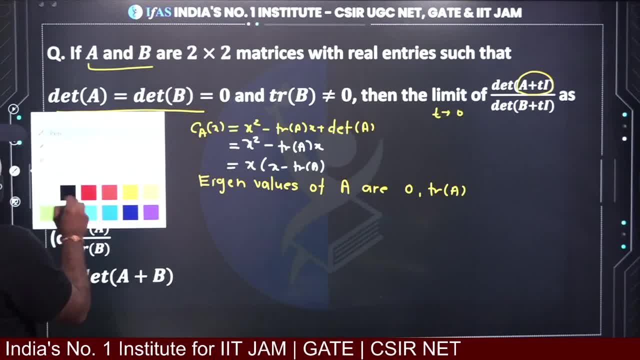 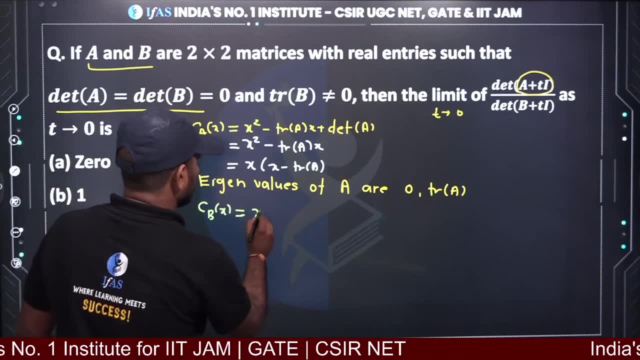 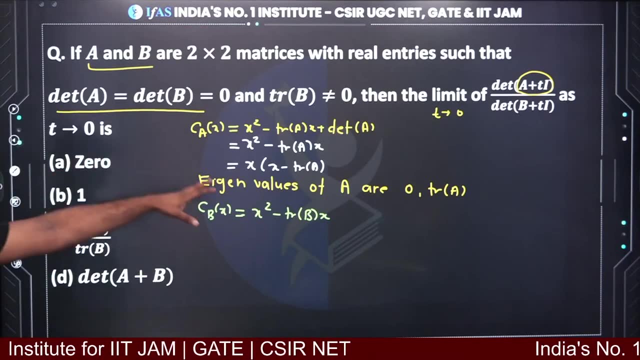 These 2 eigenvalues are there Now. similarly, what will we do? Now? we will find eigenvalue of B. So what is the characteristic polynomial of B? X square minus trace of B into X plus determinant of B Determinant is again 0. If it becomes 0 here, then what will we get? 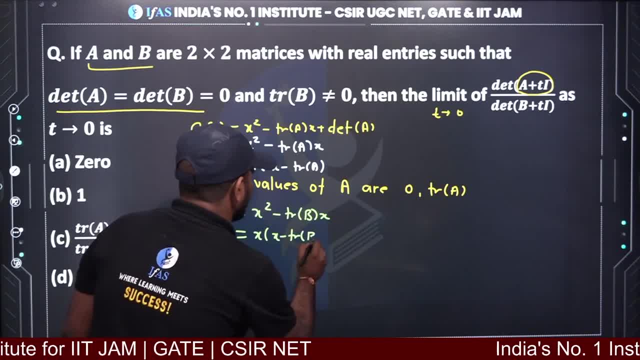 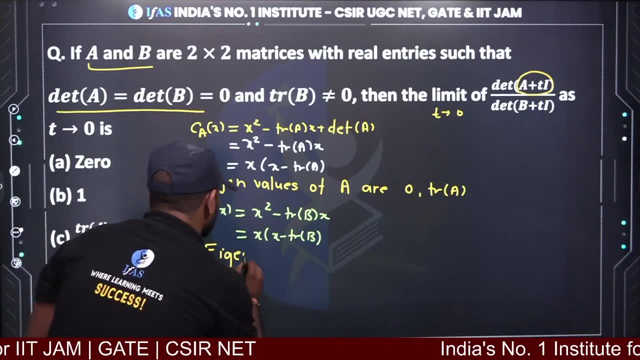 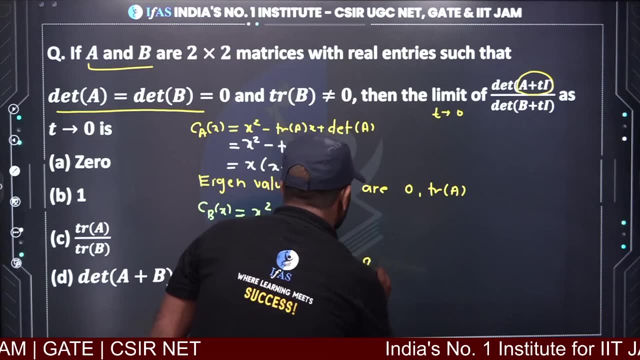 X minus trace of B. So from here you can tell Eigenvalues, Whose eigenvalues. So eigenvalues of Whose eigenvalues? The eigenvalues of B, What will we get? So eigenvalues of B are 0 and trace of B. So you got the eigenvalues of this. 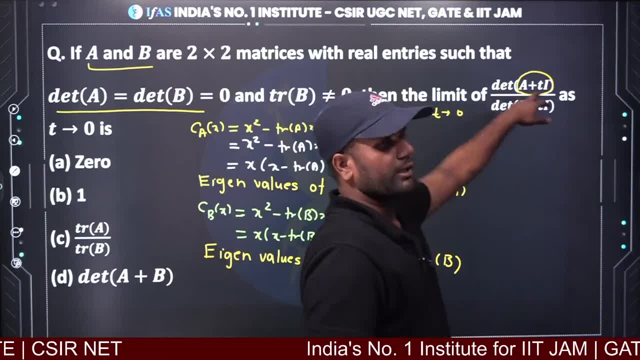 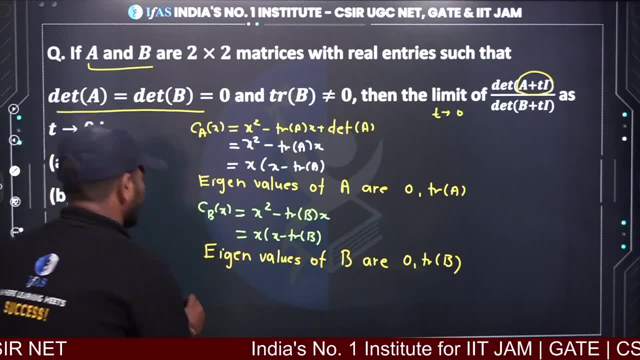 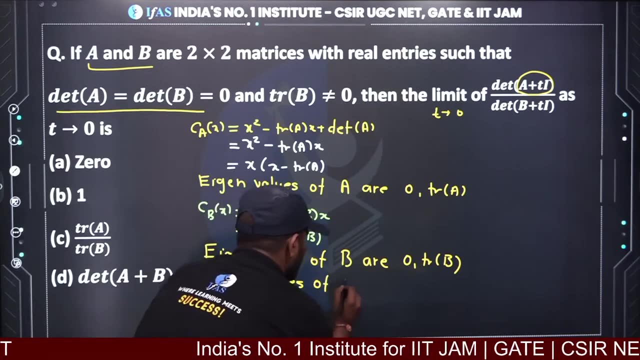 We have the eigenvalues of A and B, So we can find eigenvalues of A plus TI and B plus TI, Right? So what will be the eigenvalues of A plus TI? So from here you can say Eigenvalues of Eigenvalues Of A plus TI. 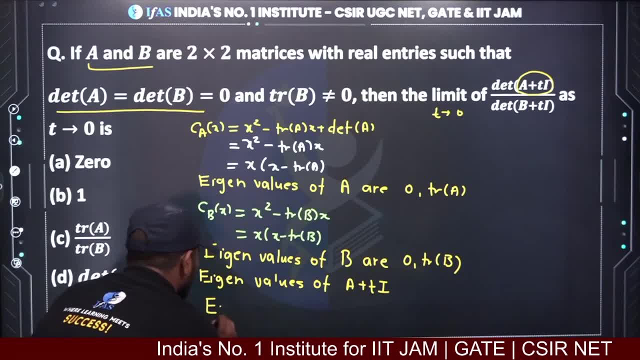 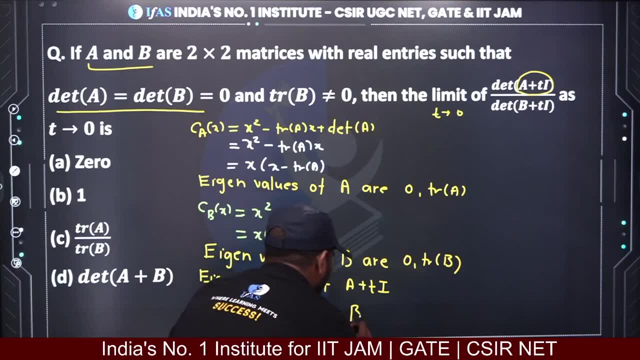 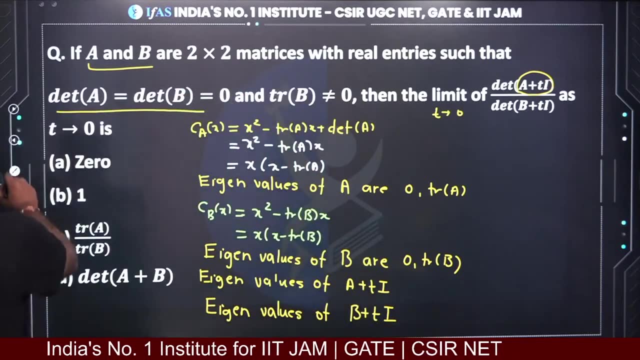 We have to find Along with that. what do we find Eigenvalues of, Eigenvalues of B plus TI, So A plus TI and B plus TI. What will we do? We will find the eigenvalues Right. So what will we get from their eigenvalues? 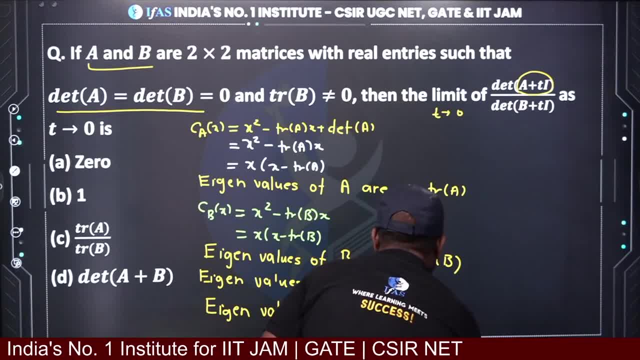 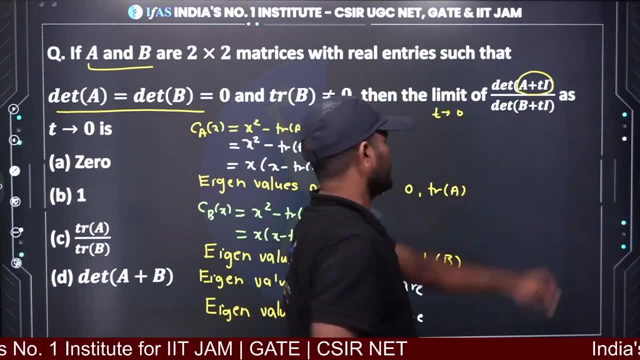 If you see that their eigenvalues will be R. See Now what to do here. instead of A, Keep the eigenvalues, and instead of T Into 1. So what will happen? If you do 0, then what will you get? You will get an eigenvalue of T. 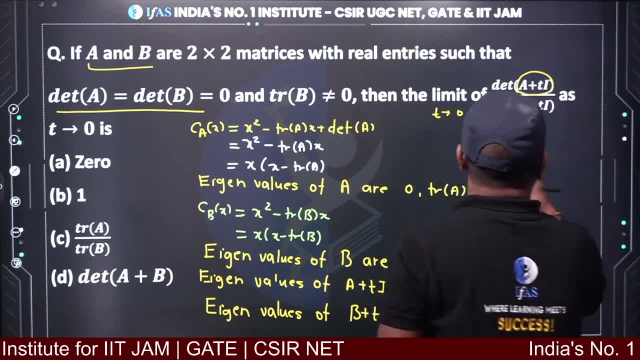 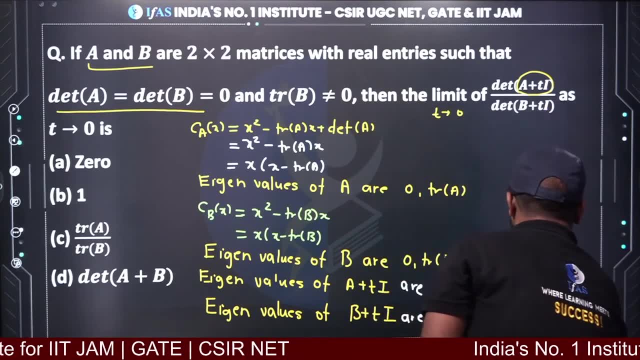 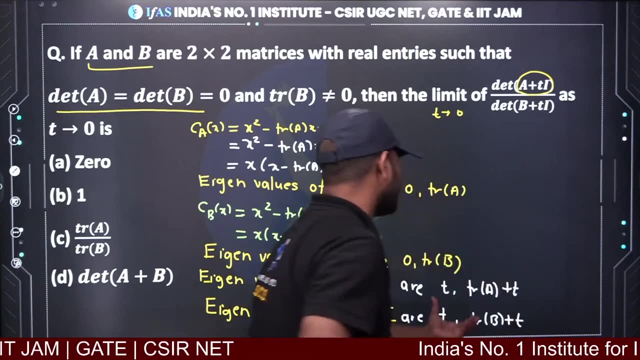 And here you will get a trace Trace of B into T, Trace of A into Into T, And you will get a trace Of B plus T. Ok, And similarly here, T, And what will happen to A Trace of B plus T? So we have the eigenvalues ahead. 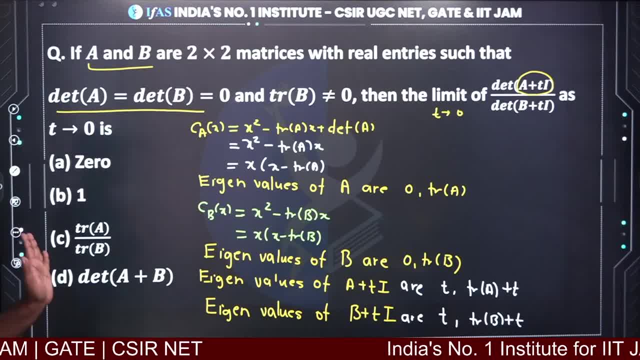 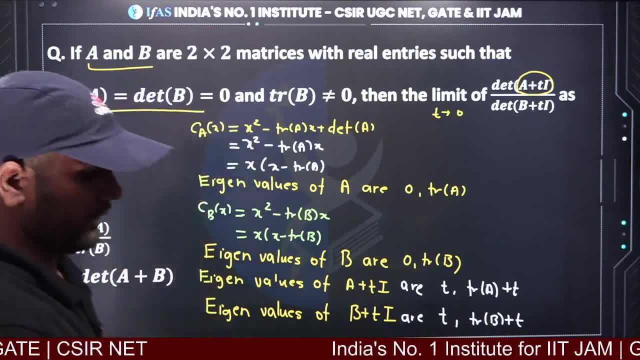 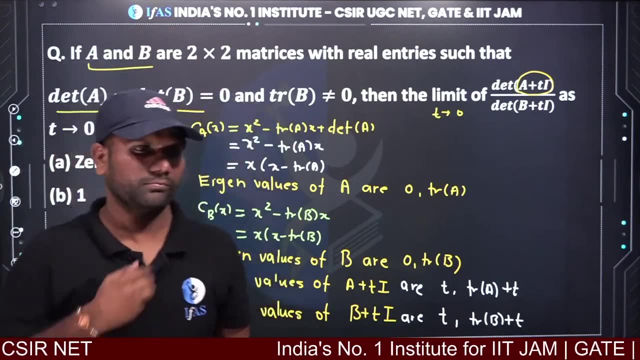 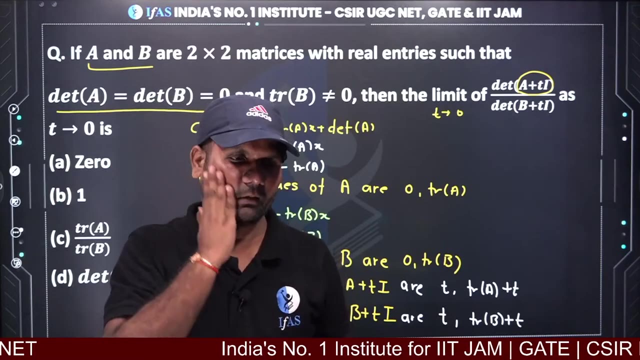 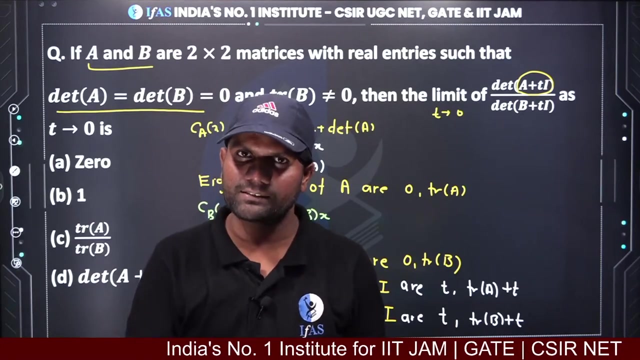 See the eigenvalues. The eigenvalues are clear to everyone, Right? Did you understand the eigenvalues Till here? I hope there will be no problem. If you have any problem, then you can ask. Ok, Now we move ahead. BEd and Net. Praveen, tell me once you have prepared a lot for Net, and what is the exam of BEd? is it an entrance exam or a semester exam? first tell me. 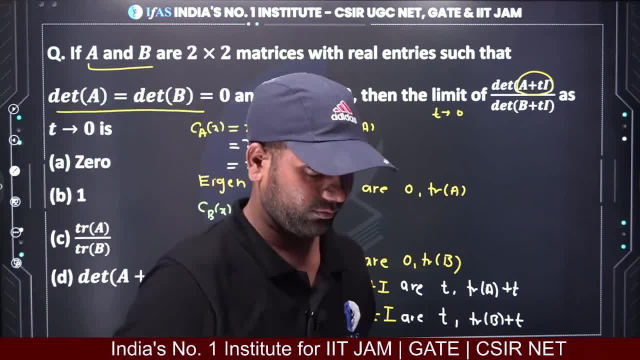 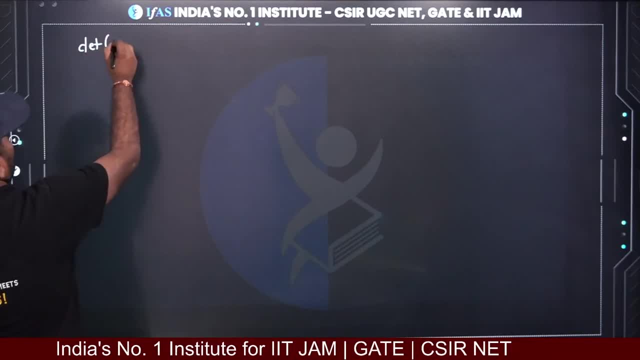 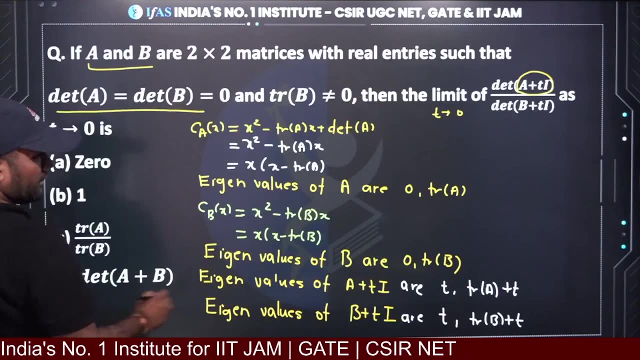 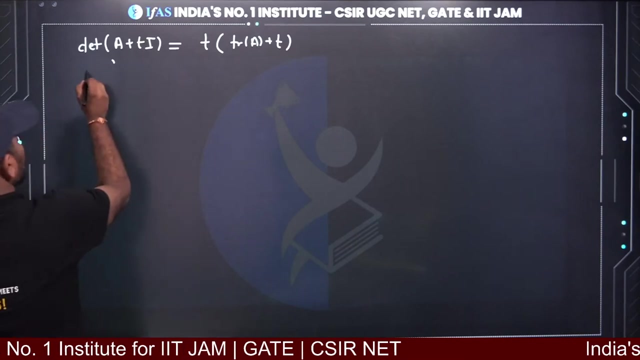 now let's find the determinant. so the determinant of A plus T i. so what will be the determinant of A plus T i, product of Eigen values? so what will be the Eigen values T, T into trace of A plus T. similarly, if I find the determinant of B plus T i, 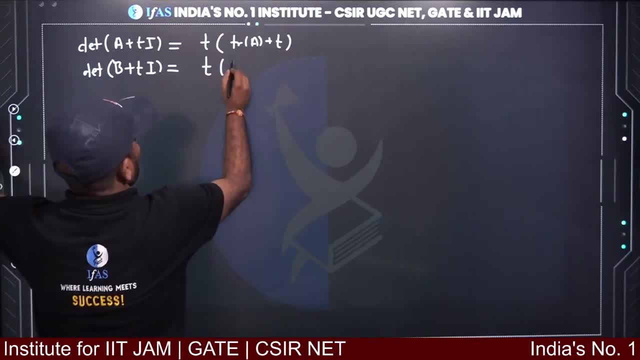 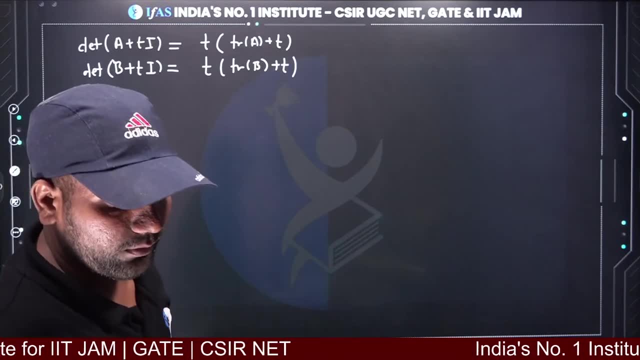 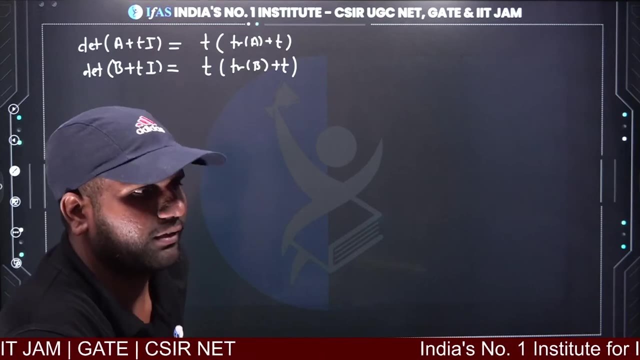 what will you get? so this is equal to T into trace of B plus T. what will you get? Sir, we are not calling the robot from the remote. we were turning on and off the AC. sometimes what happens is that the AC is on. 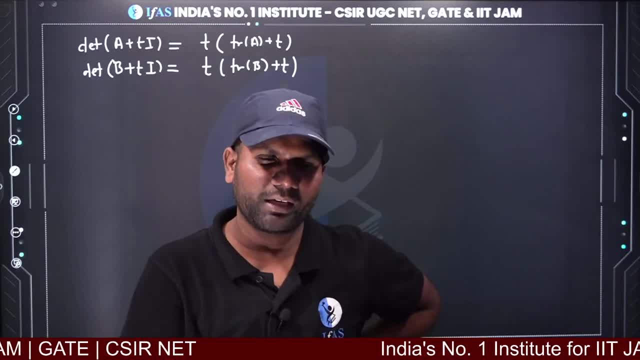 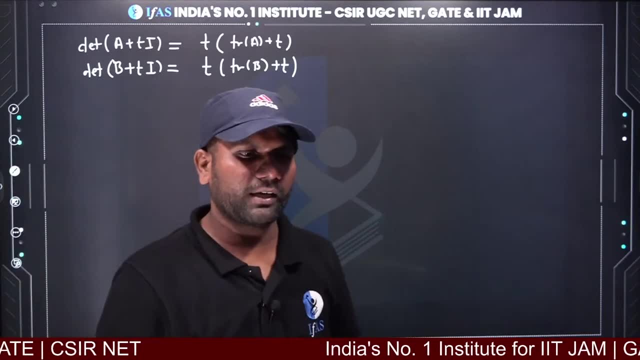 so after some time, when it starts to get cold, then I turn it off. so I just turned it off last time, then I turned it on last time. it has been read. well, see, if your preparation is good, then go for Net at all. 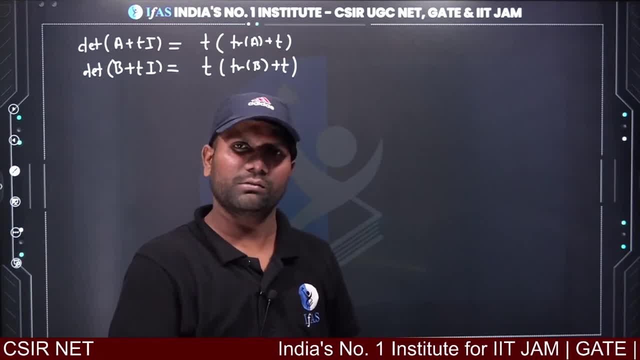 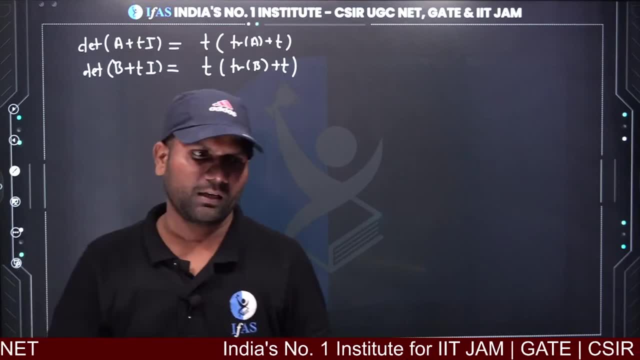 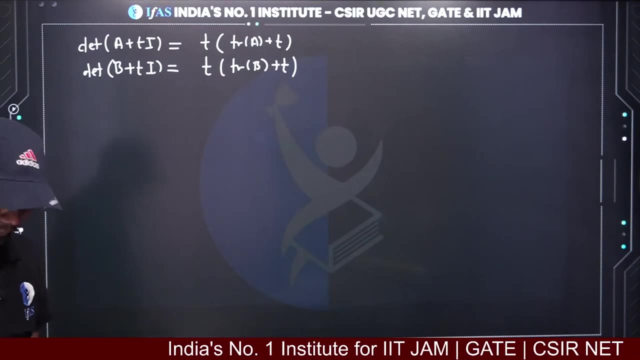 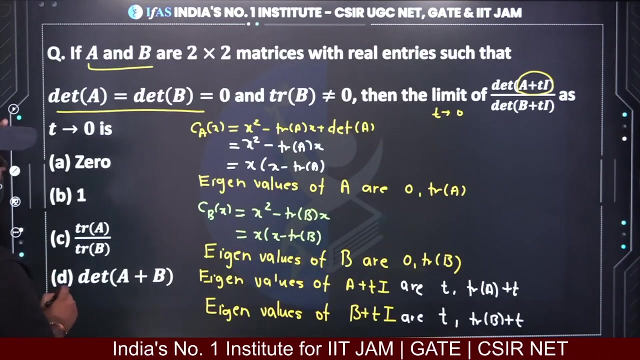 then the choice is up to you, because the exam of BEd, of Net, will be done again after 1-2 months. if your preparation is good, then go for Net at all. now let's come here. we have to find what to find. Limit T tends to 0,. 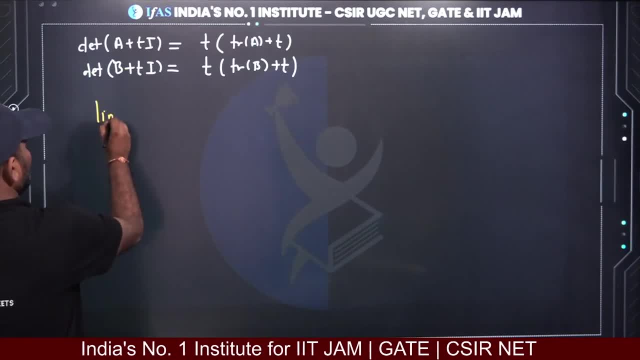 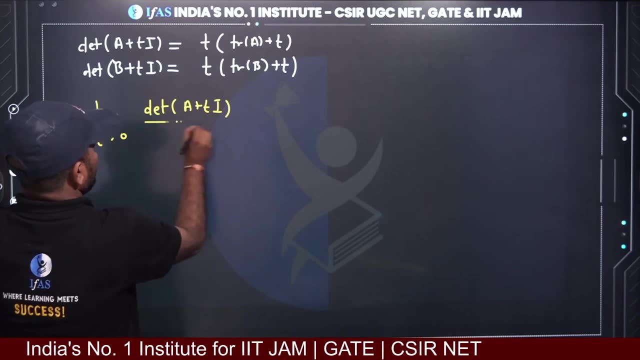 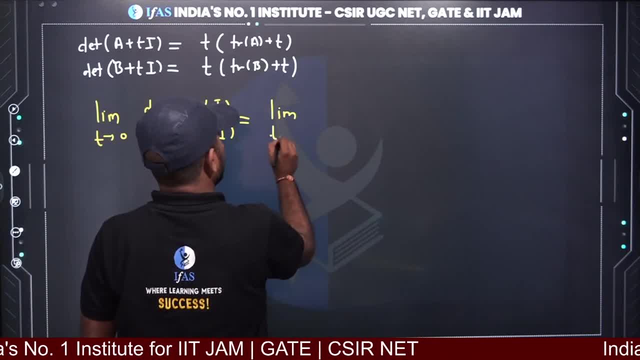 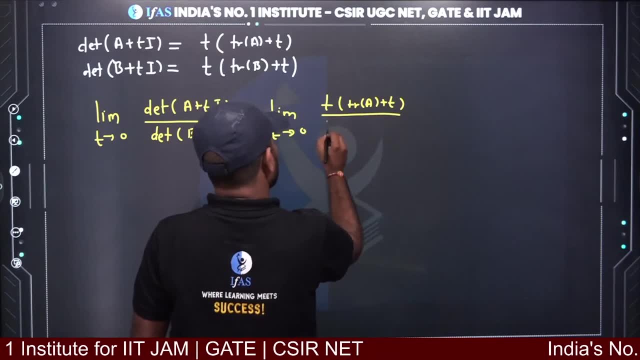 so what will you get? you will get A Limit T tends to 0,. and what is the determinant? trace of A plus T divided by T into trace of B plus T. now see T. T will be cancelled. what will you get? Limit T tends to 0,. 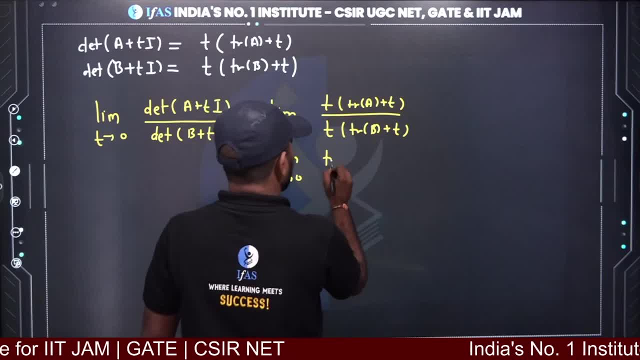 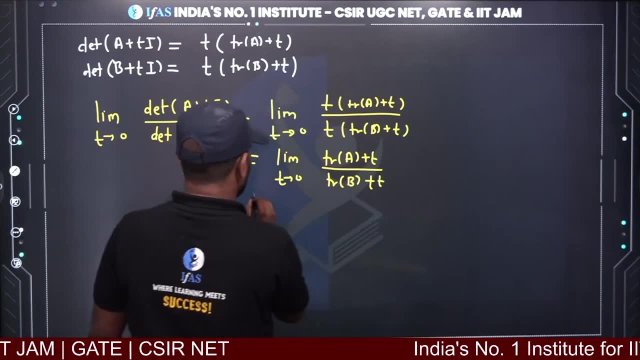 Limit T tends to 0, here it will be Trace of A plus T divided by Trace of B plus T. now see, if you keep the value of T as 0, then what will you get? Trace of A by Trace of B will be available. 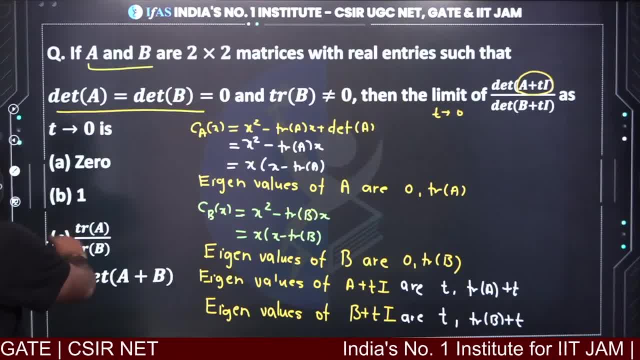 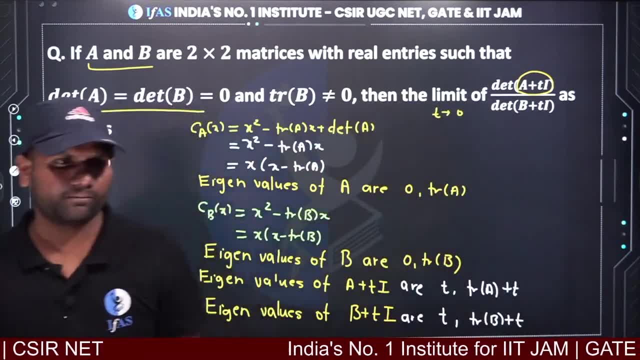 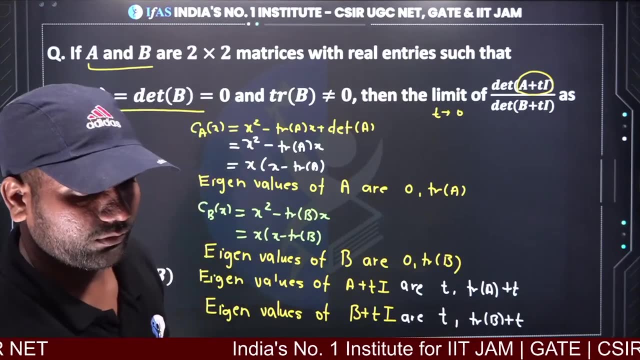 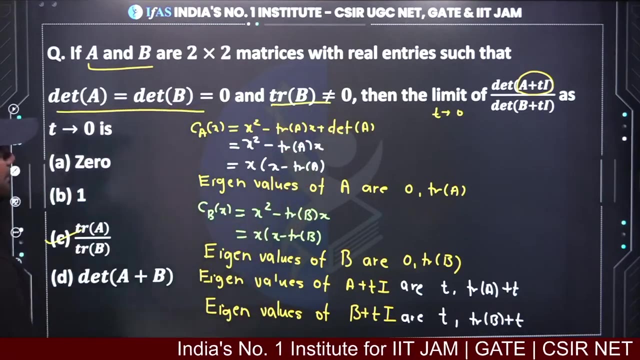 it means that your option T will be correct for this question. is it clear to everyone? B and C will not be the answer, only C will be the answer. I think you all will be clear till here, ok, ok, ok, see, here in denominator we get a trace of b, but it is mentioned here, which is not equal to 0. 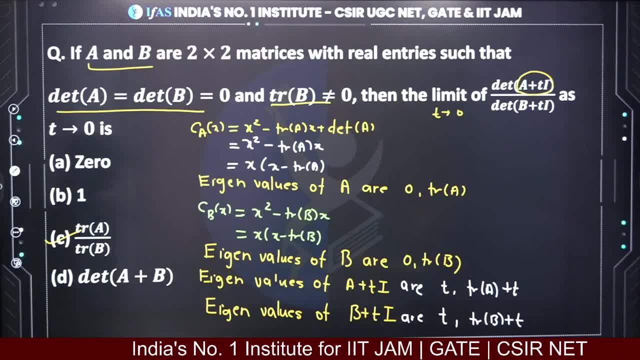 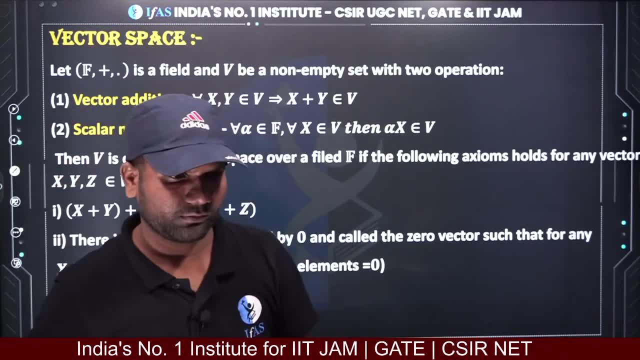 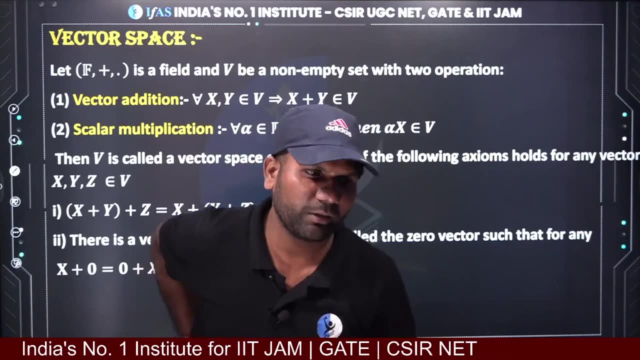 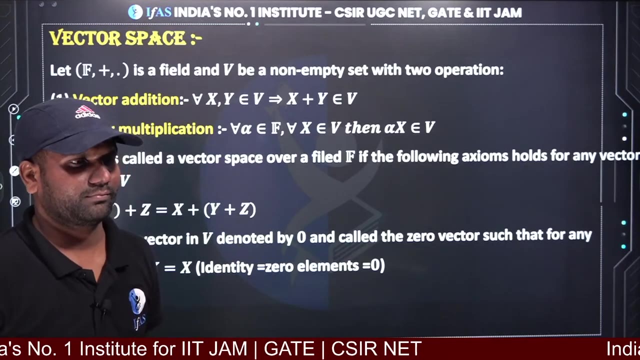 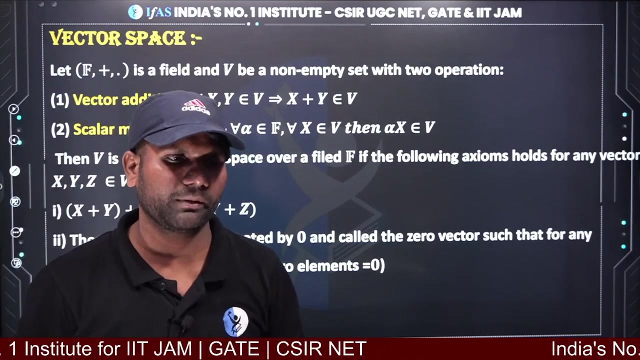 it means that tool is well defined. let's go to the next slide. now we have come to vector space. eigen value is summed up here. use double c. ok, tell me one thing: if you will use oil hospital and differentiate, then what will you get here? first we should know eigen value. 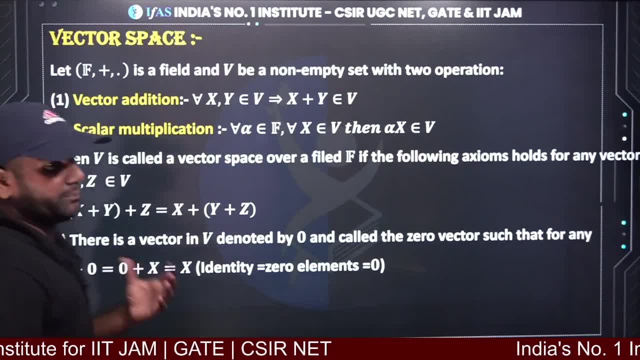 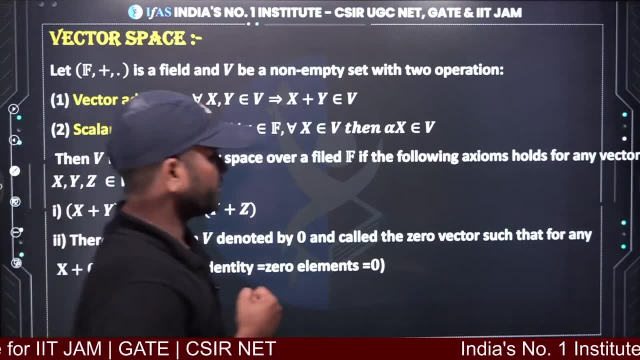 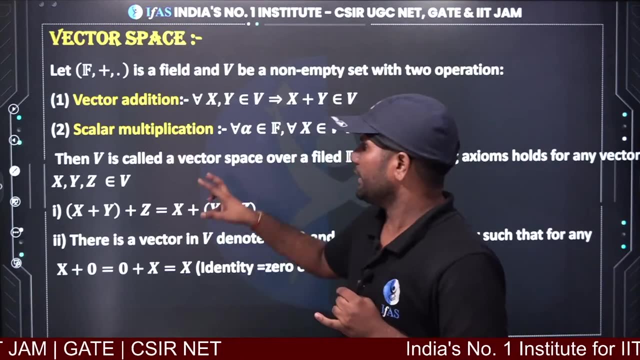 ok, now see here. I will give you information about vector space. I know you know the definition. still, I will give you a hint. see here. for vector space we need two operations of a field. ok, so the name of one operation is vector addition and other is scalar multiplication. 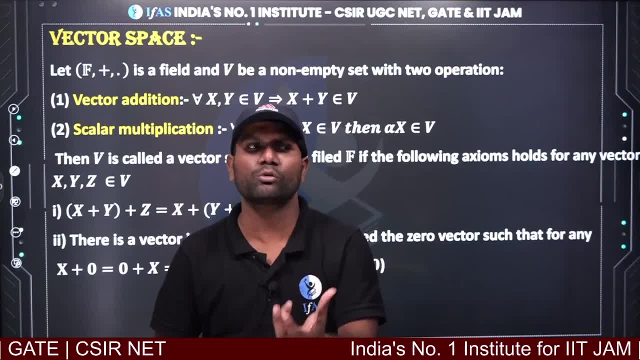 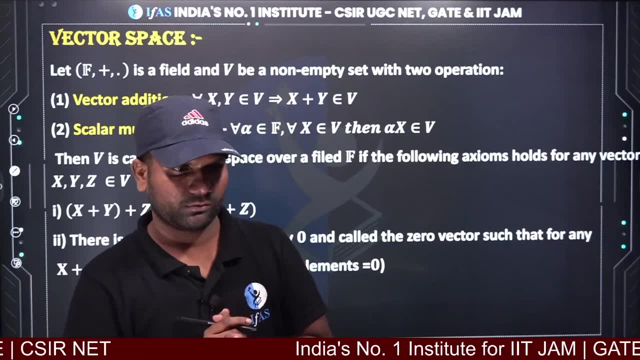 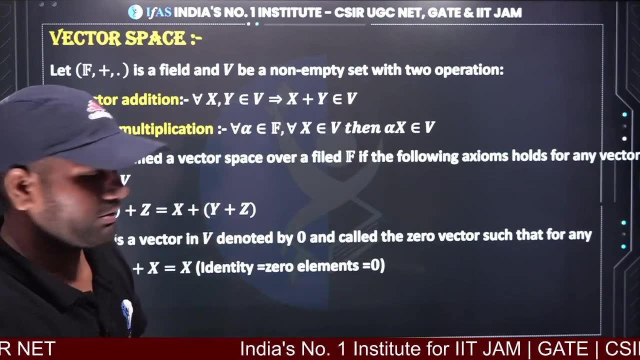 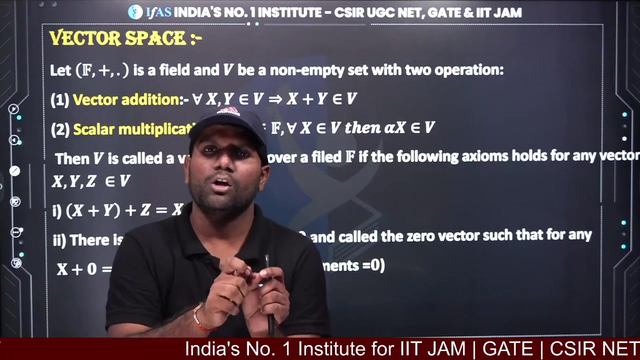 what we do in vector addition. we give a rule in vector addition. we tell a method how to add element of v. ok, we tell a method how to add element of v. ok, ok, ok. we tell a method how to add element of v. ok, ok, ok, ok. 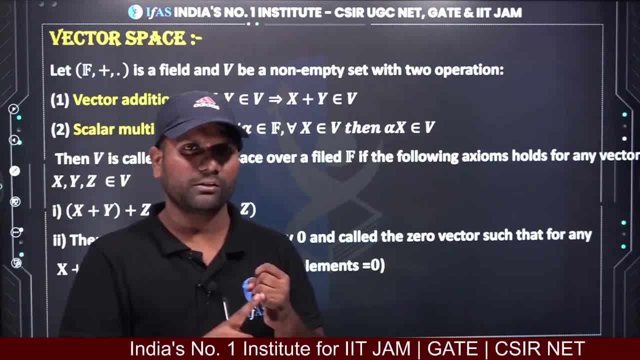 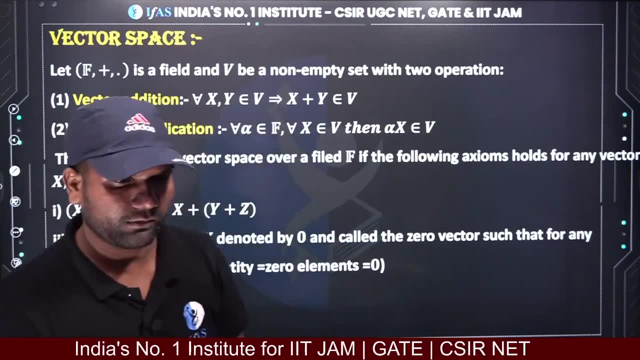 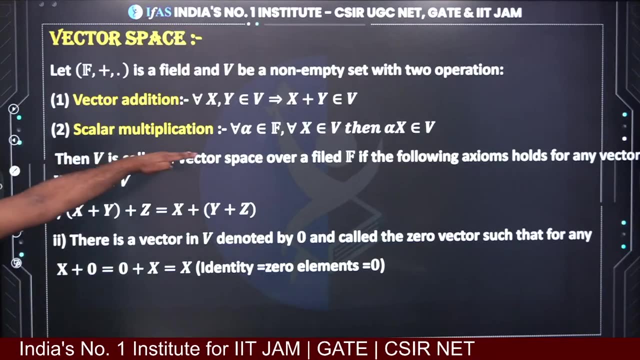 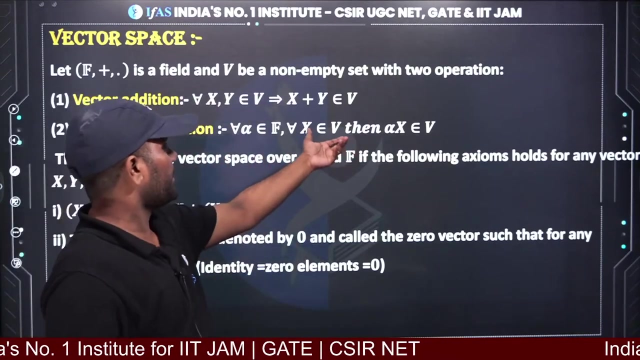 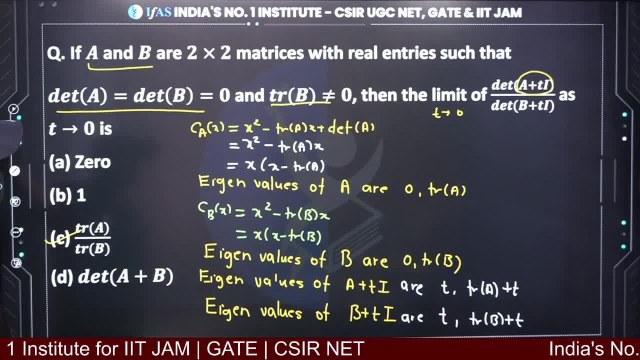 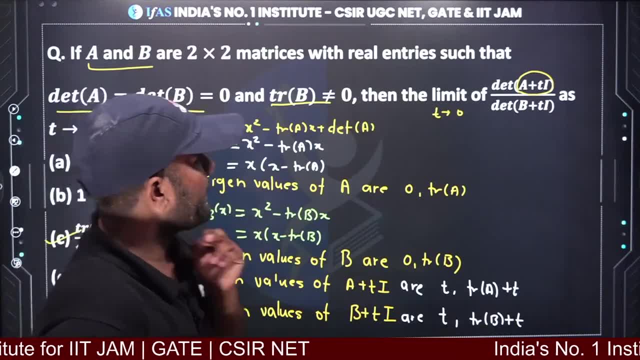 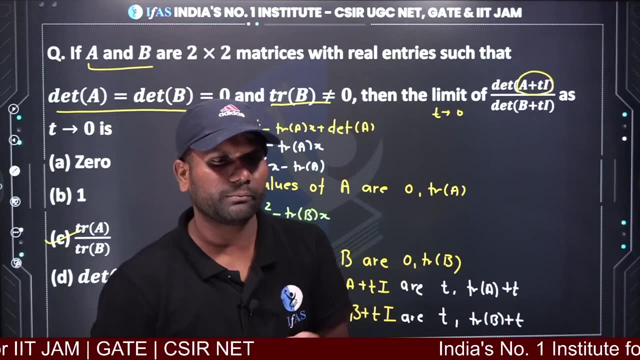 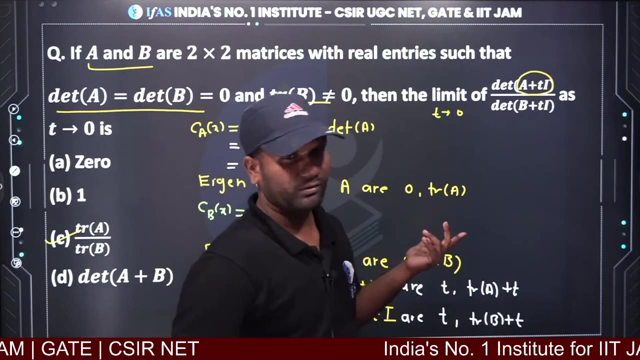 One minute. tell me one thing: how to use double C in hospital rule. what will be the determinant of this? tell me how will you apply it? Determinant will be a number. here we should have a determinant. how will you directly accept it? how will you do it? 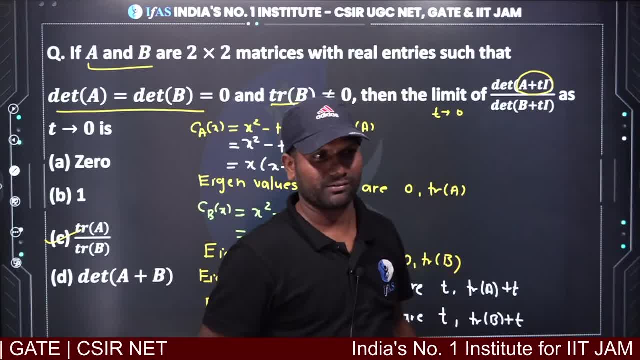 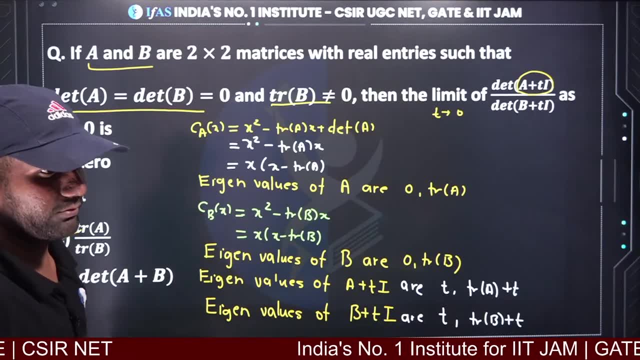 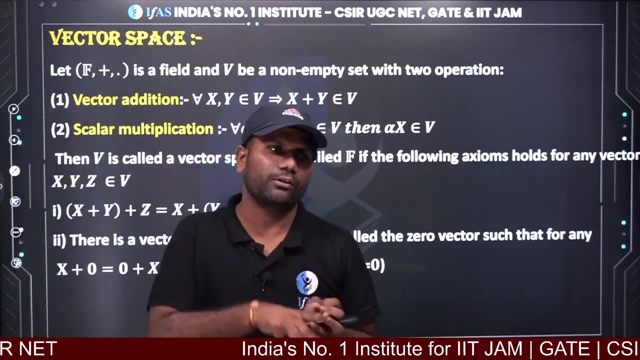 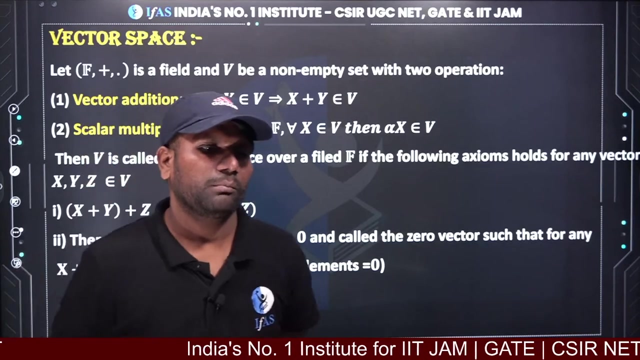 Now you will be leaving the determinant and applying it inside. how are you doing? tell me, sister, let's go ahead After that. once vector addition and scalar multiplication are closed, how will you write the polynomial? tell me, how will you write the polynomial of the determinant? 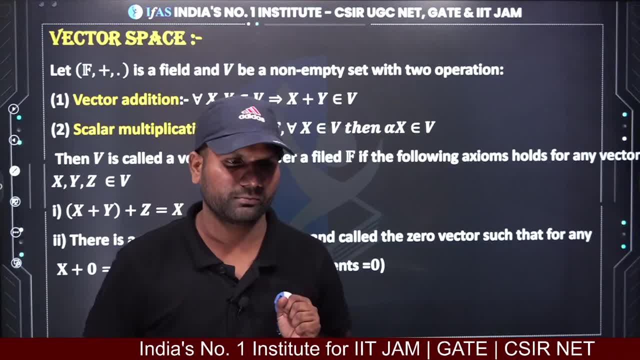 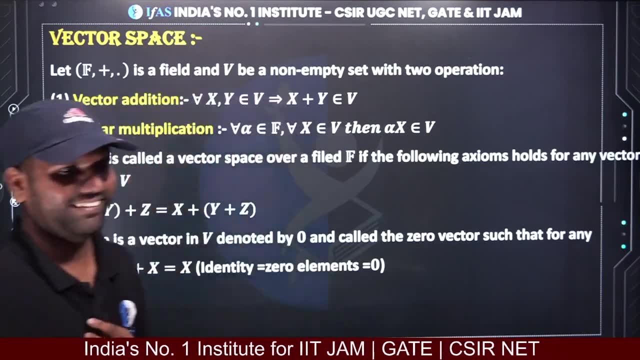 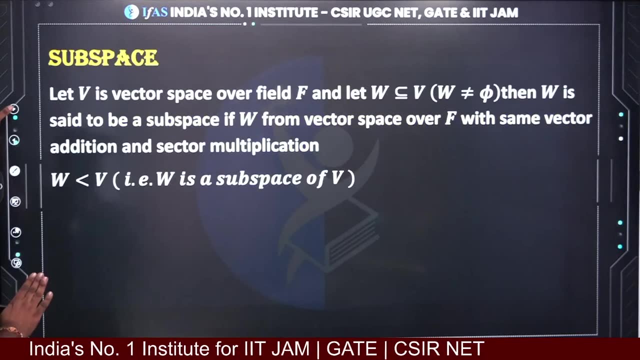 First, you will take out the determinant. tell me you are very far from us. good, good. after that, this art property satisfies. then what do we call it? we call it a vector, we call it a vector space. and look here, you have to be careful. 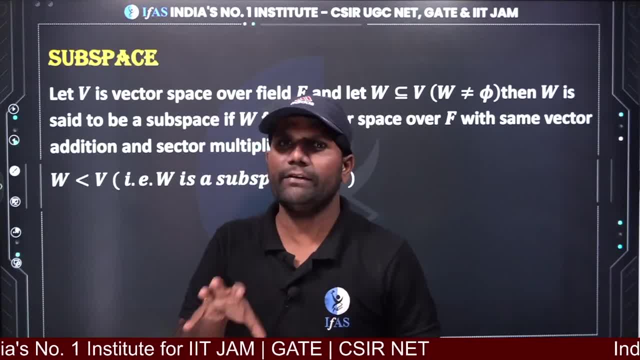 like: if someone tells you to write a vector, you have to write a vector. you have to write a vector. let's give example. in the example we don't ask the question of vector space. now the question is asked of a subspace. 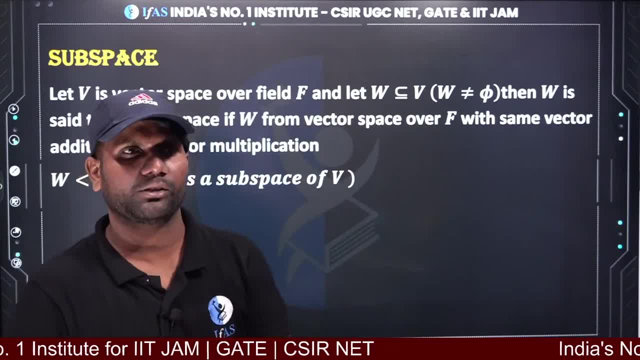 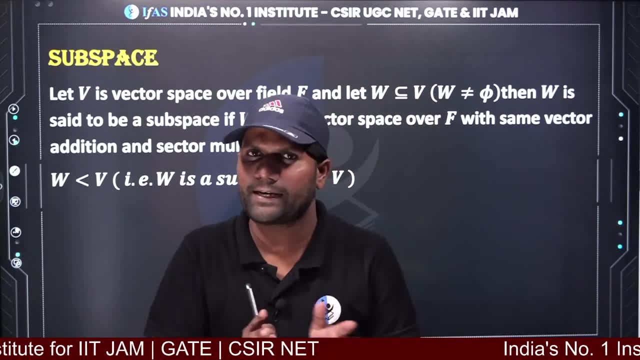 Ok, so how to talk to the subspace, or if I talk about a vector space. if there is a vector space and it will be non-empty set, so the addition will be closed, the scalar multiplication will be closed and the art property will be satisfied. what will happen if it does not happen? 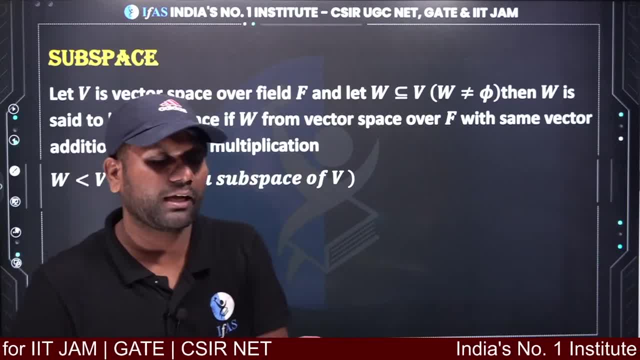 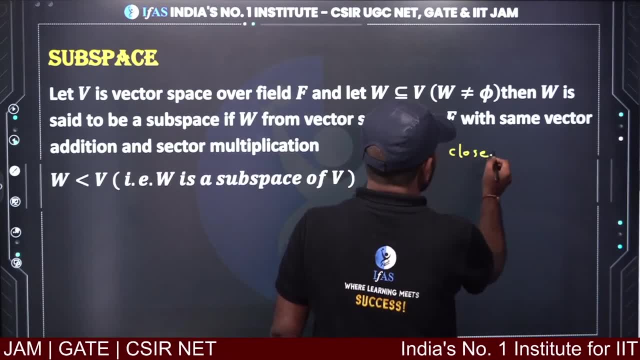 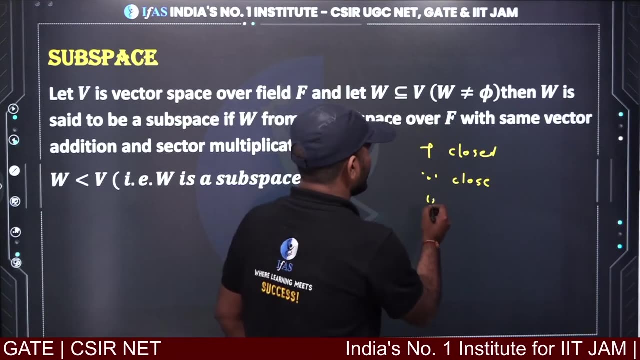 So what happens in 99% of cases? I will tell you what will fail from here. either vector addition should not be closed, either the scalar multiplication is not closed, or it may not be closed, or it may not be a zero vector, or it may not be equal to 1.x. 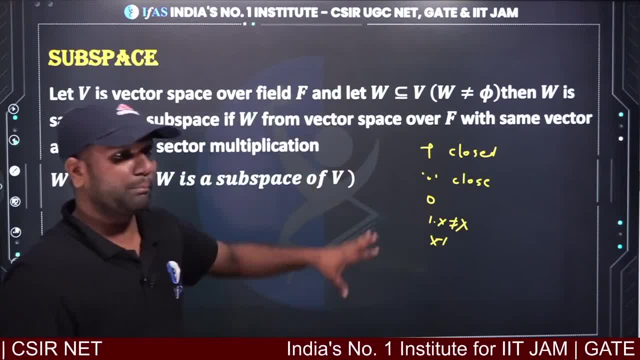 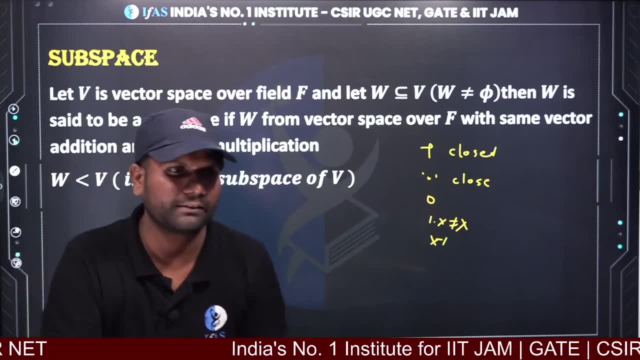 or it may not be an inverse. or it may not be an inverse, so if there is no vector space from these 5 or there is no subspace, then something or the other fails out of these 5. ok, so 99% of the time this fails out. 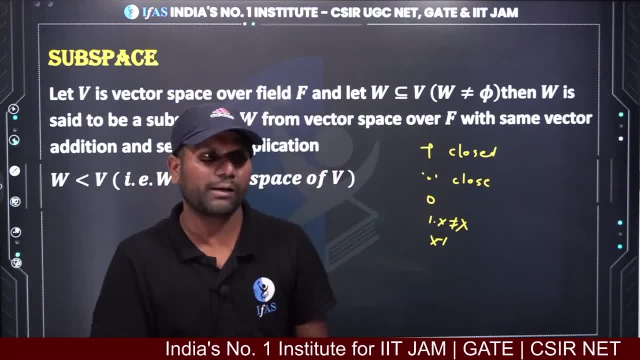 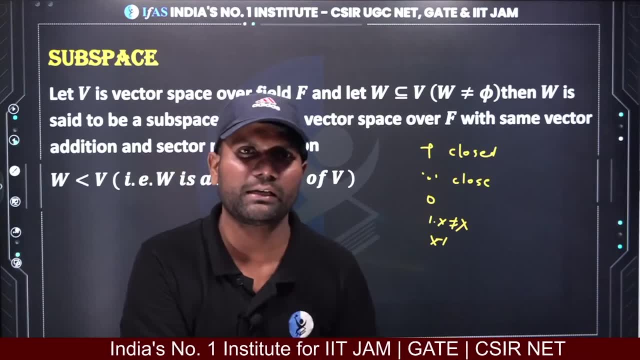 if you are doing the question of vector space and subspace, then you should practice so much that in the exam, if you see the question, then there are 4 options to solve. if you have to solve one, then it is ok. you should know by looking at these 3. 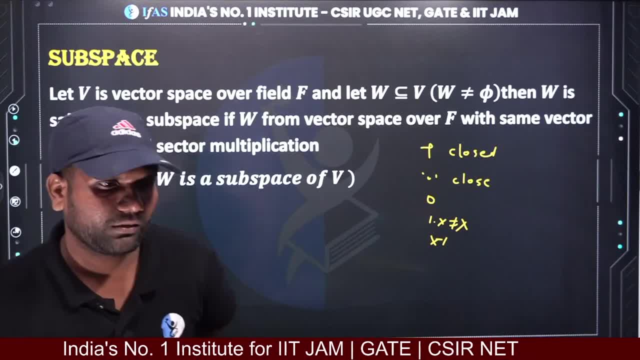 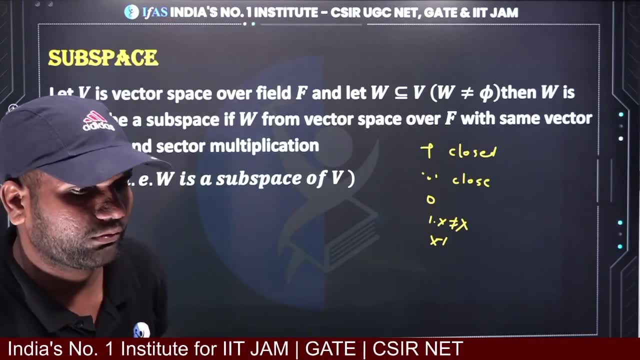 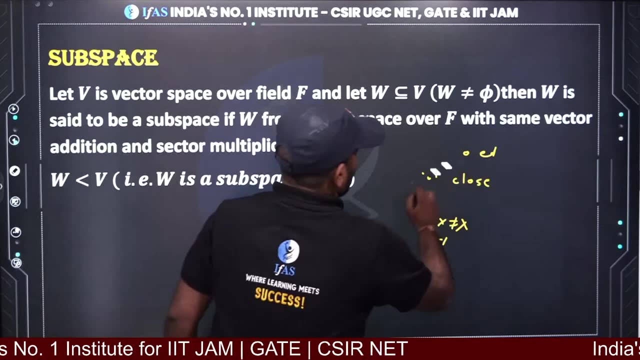 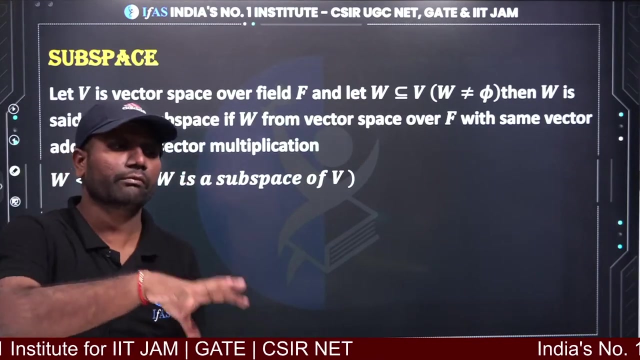 ok. whose initial and whose eigen value will you take? if eigen value is zero, then for whom should you take? ok, ok, subspace. subspace means if there is any non-empty set of vector space with the same operation from which V formed vector space, if that also forms vector space. 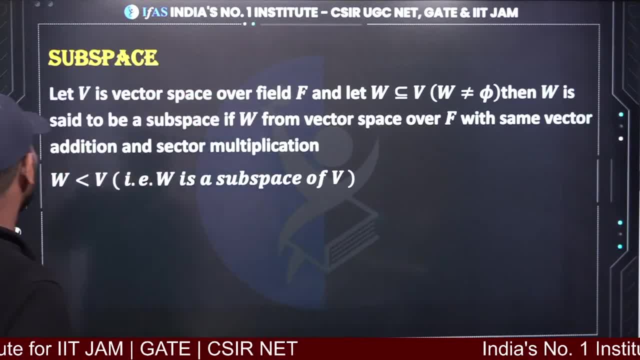 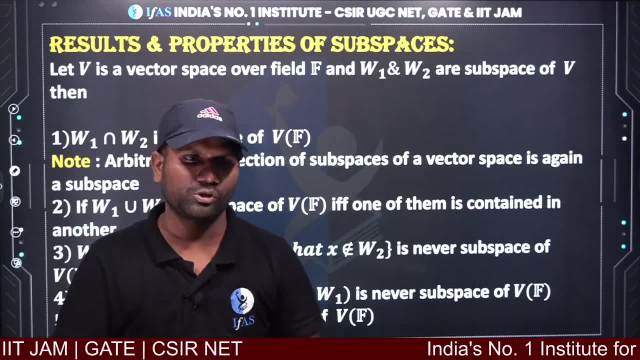 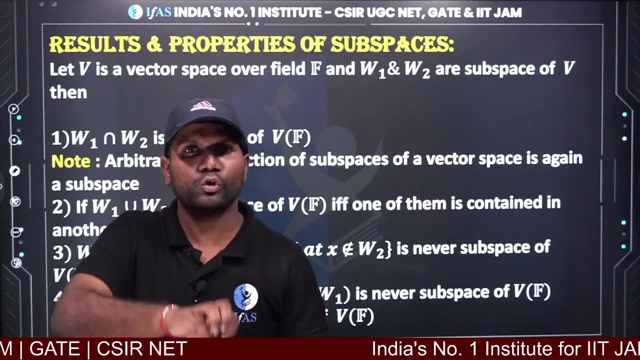 then that non-empty set is called subspace. ok, we move ahead. there are some results and properties which you should know. for example, if w1 and w2 are subspace, then their any, or w1, w2, w2's subspace, then their intersection will always be subspace. 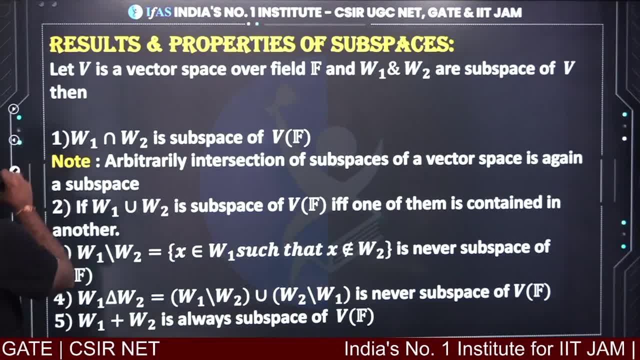 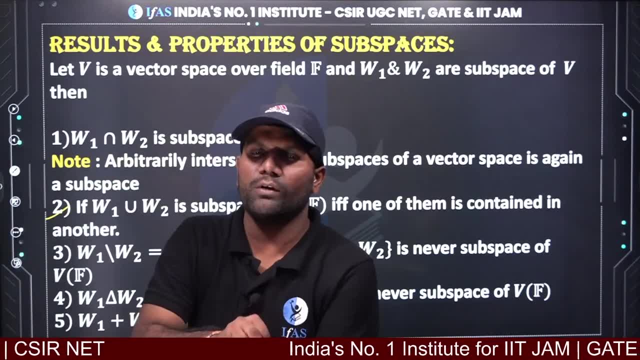 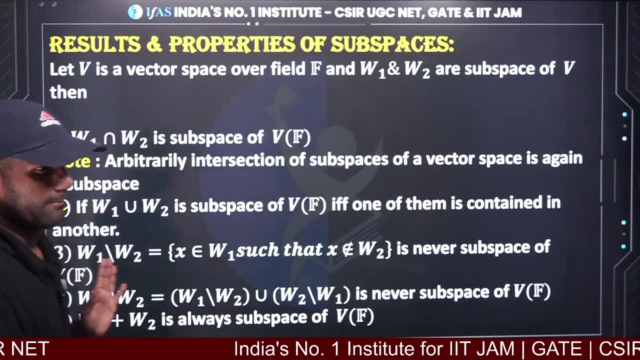 union is not required. remember: union is not required. when is union? if you talk about union, then their union is only subspace when either w1 is inside w2 or w2 is inside w1. when they contain each other, then they form subspace, ok. 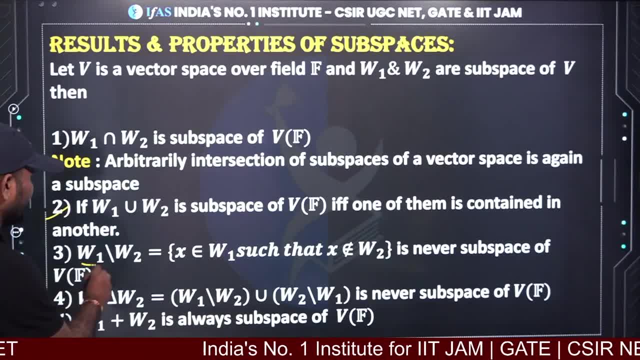 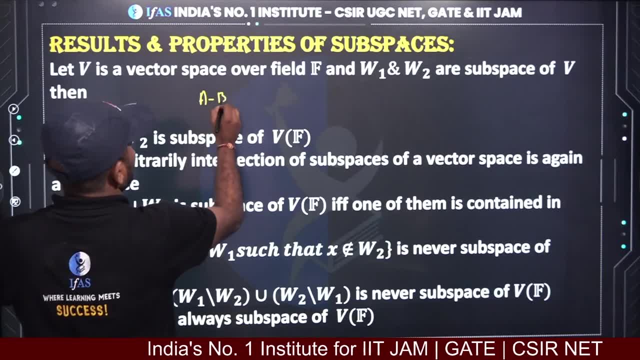 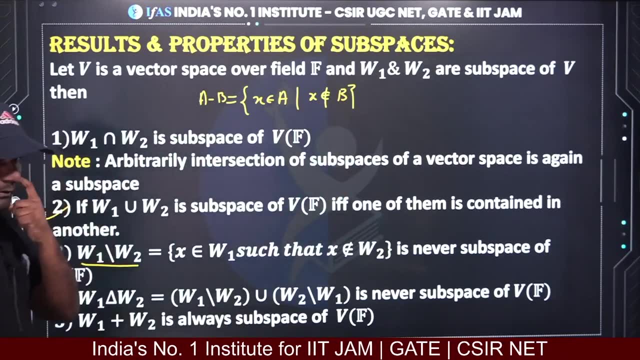 and keep in mind w1 minus w2, a will never form subspace. what does w1 minus w2 mean? like a minus b means x belongs to A, such that x does not belong to B. we are talking about this set. why it does not happen? because the identity has already come out from here. 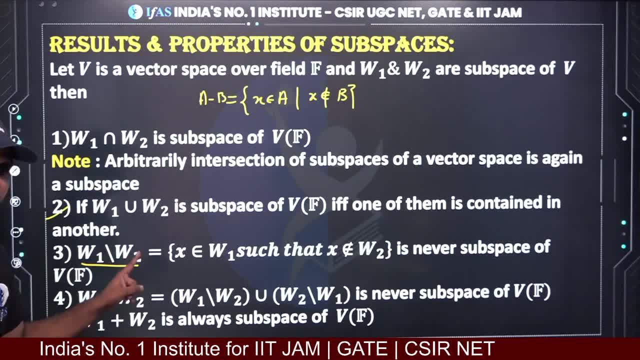 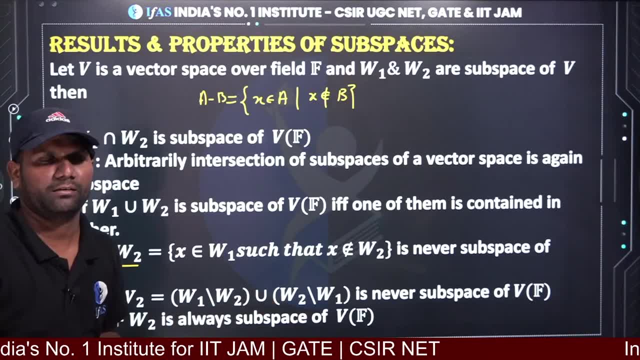 it does not have any zero vector. so W1 minus W2 will never be subspace. W1 symmetry difference will also not be W2. what is the reason? it does not have any identity? it does not have any identity. zero vector comes out. that is why it does not happen. 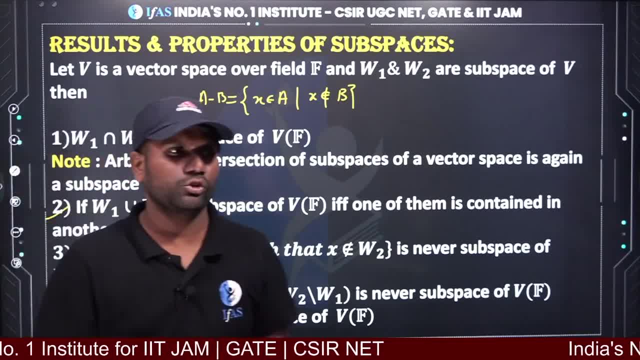 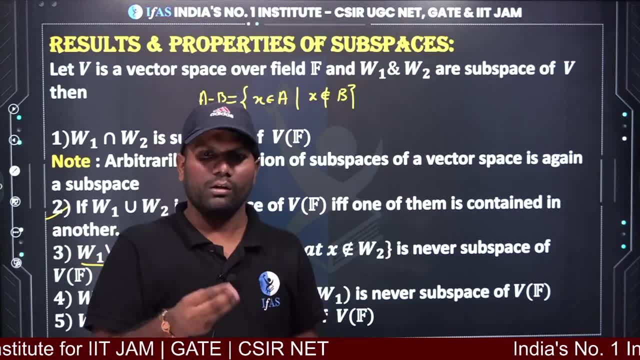 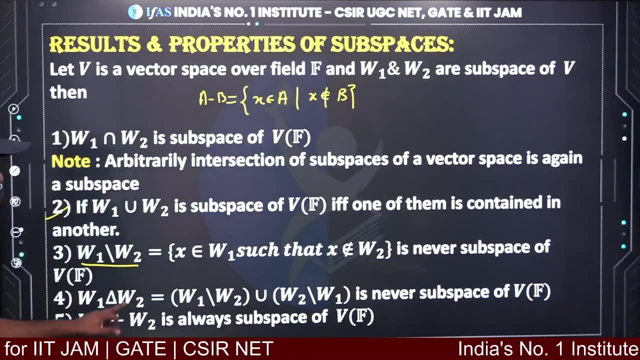 and keep in mind: if W is subspace, then W's complement will never be subspace. the reason is the same: it does not have any identity, because if W has identity, then W's complement will have identity. it will not happen. if W1 and W2 are subspace, then their addition is also subspace. 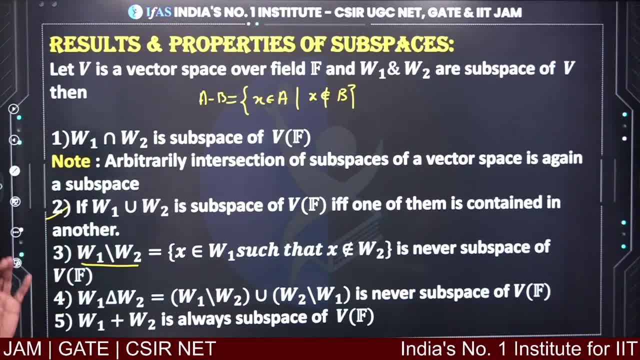 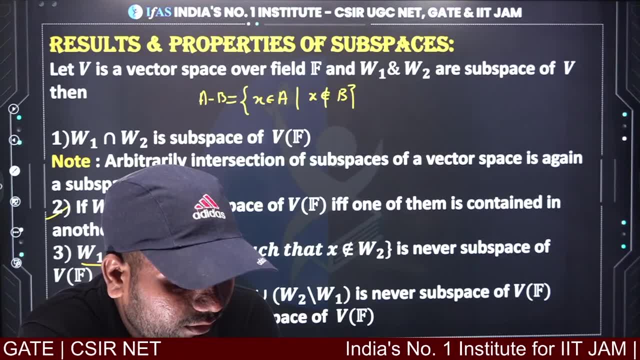 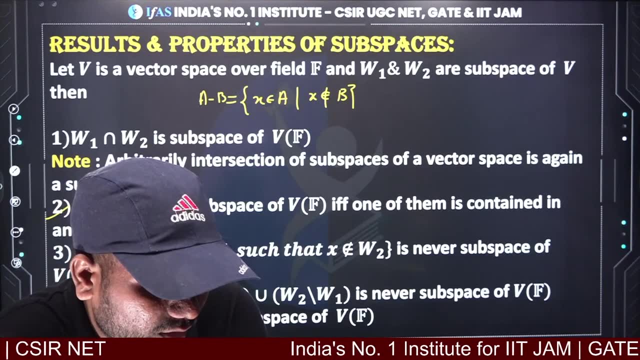 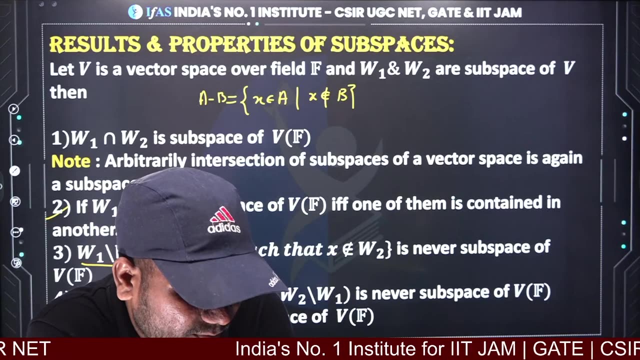 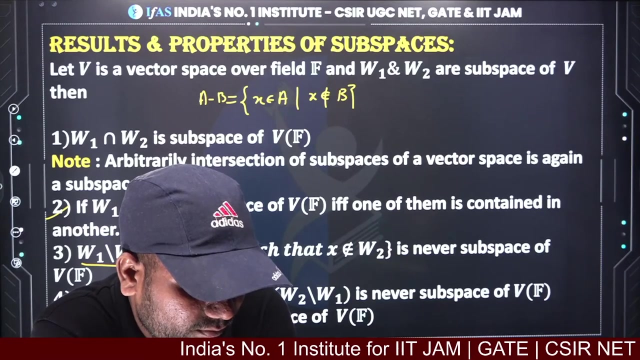 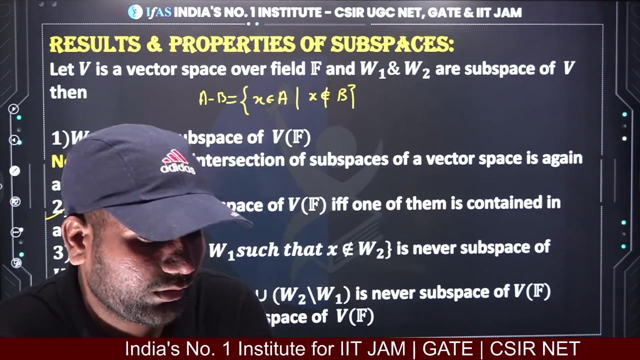 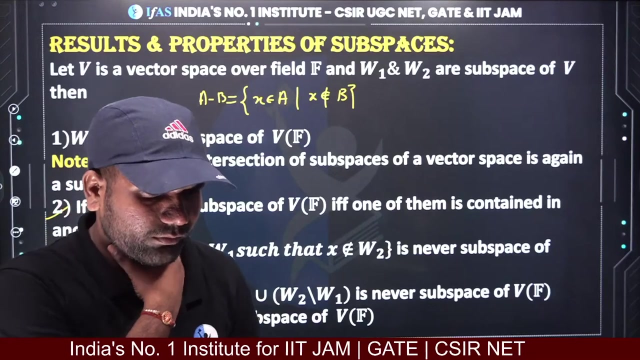 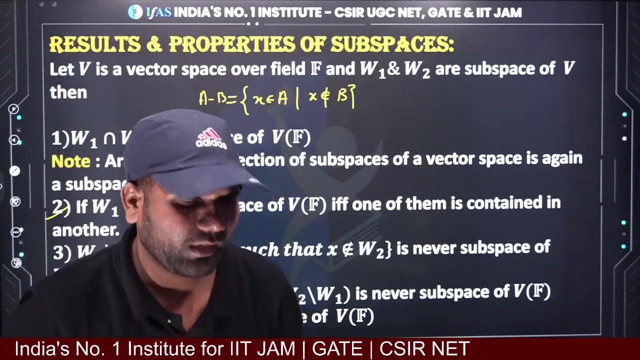 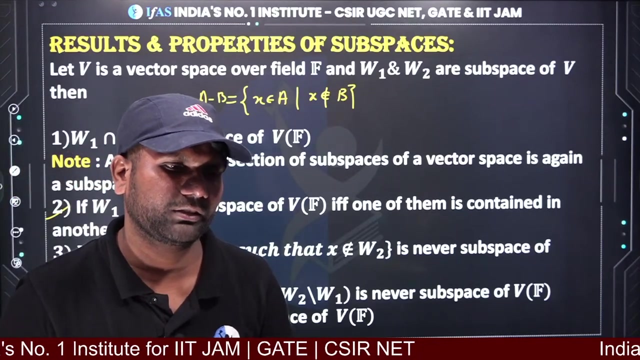 these are some important things which you have to see before going to the exam. determinant of A minus A, A minus C. C raised double C. what did you tell the determinant of A minus T I that you have written determinant of Intersection will always happen. How did you write the determinant of A minus TI as T square minus trace of A into T plus determinant? 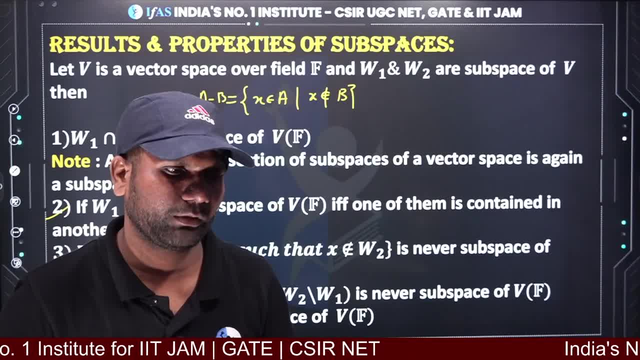 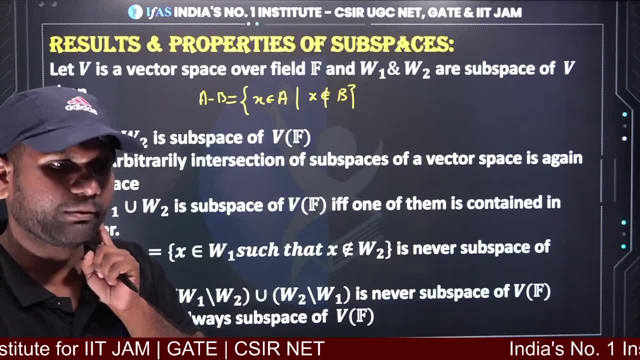 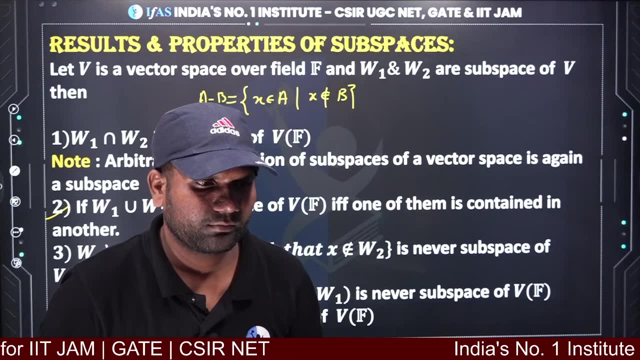 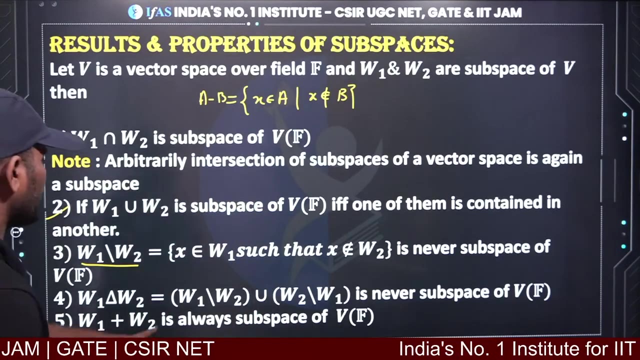 How did you come to know that this will be the same? You must have written something thinking, I feel, that this should not have happened. What did you think? Tell me once. Fourth point is that W1 Symmetry Difference is W2, then what does W1 Symmetry Difference mean? 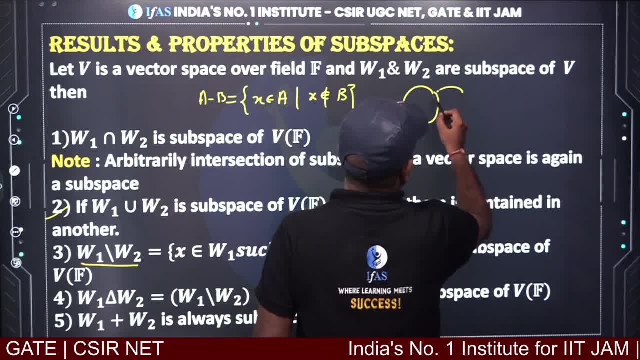 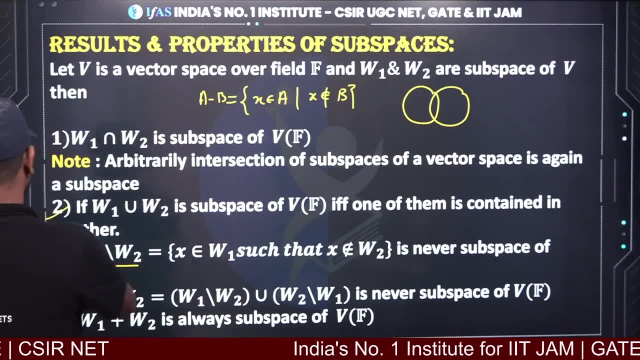 for eg. I make one. so what does it? says W1, Symmetry of W2, whose will be W2 from w1 If you will remove W2 from W1, so that will be: it is your w1 or it is w2. 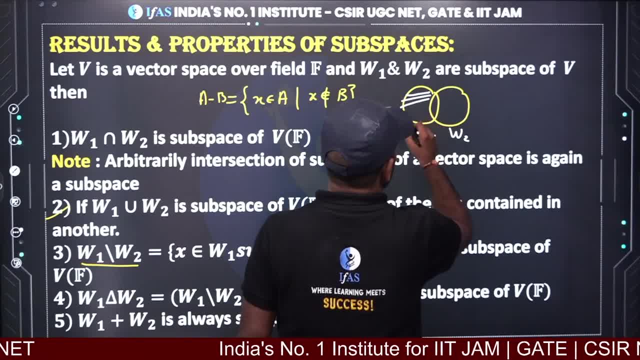 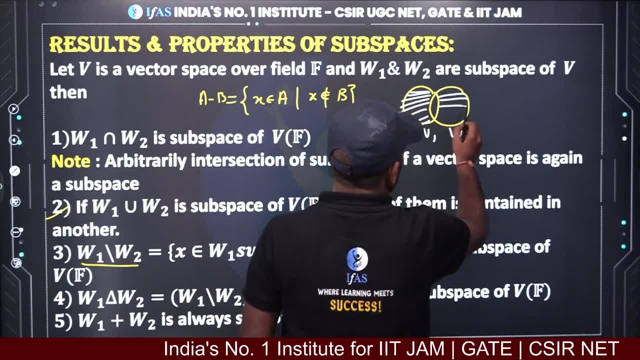 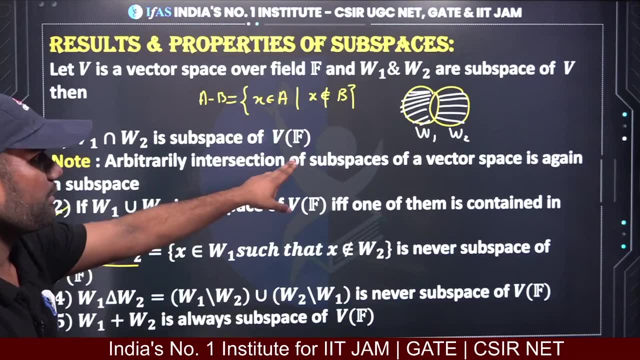 W1 minus W2, so instead of W1 minus W2, you get this. And the second is W2 minus W1, so you get W2 minus W1. Now, this one is talking about the saddled region. W1 and W2 are talking about the saddled region. 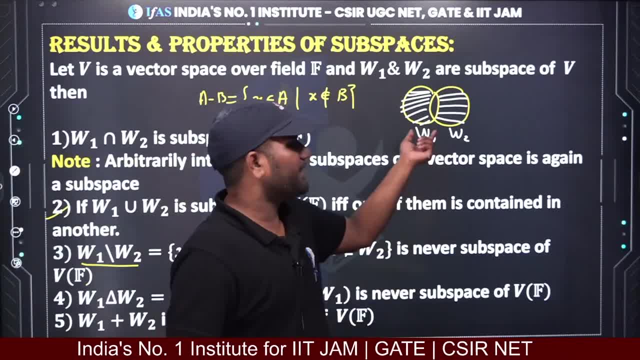 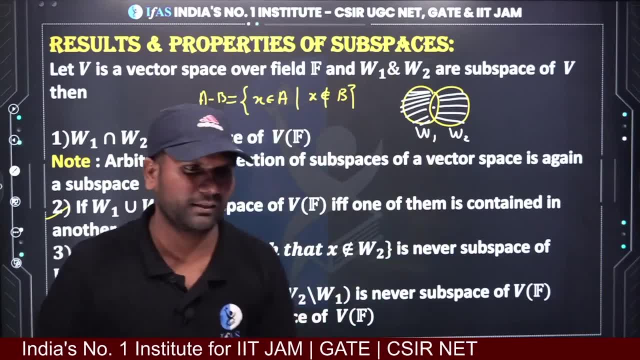 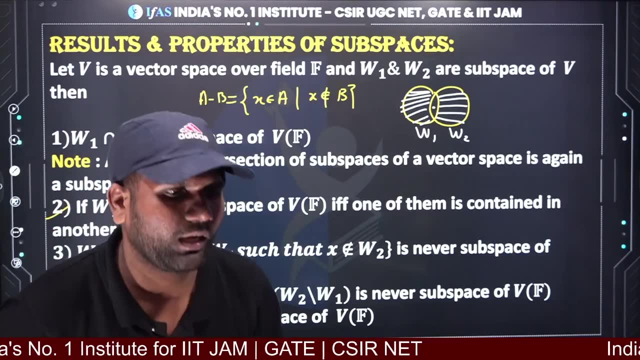 So if you see here the identity, that will be there. Identity is out of here because the identity will be somewhere here. So if you take their union, then they do not have identity. That is why there is no subspace Double C. that is fine. 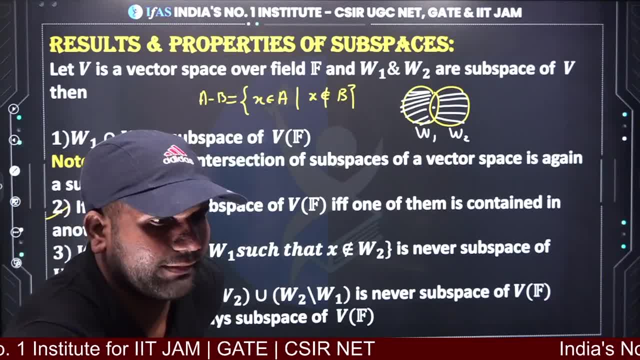 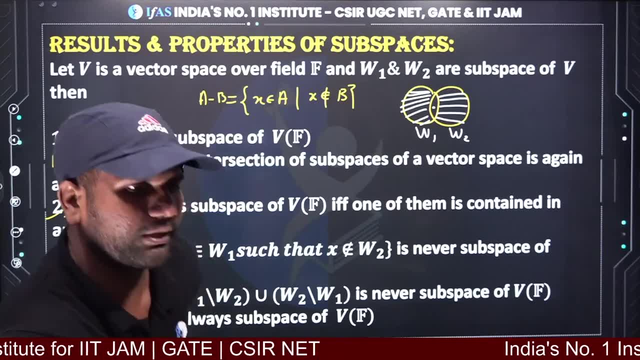 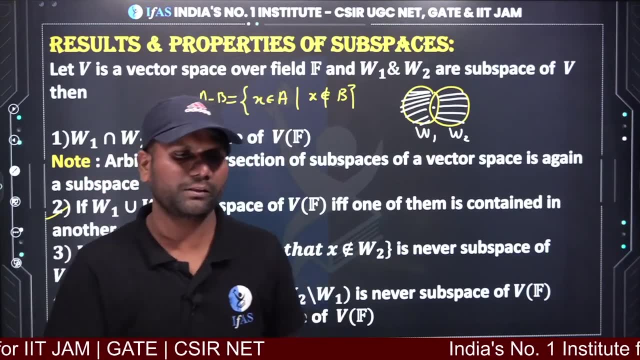 I was saying, like you take out the characteristic polynomial for the matrix. So how did you write the determinant of A minus TI directly like this? So we were not taking out the characteristic polynomial. Once you explain it to me, then you will know what is right. 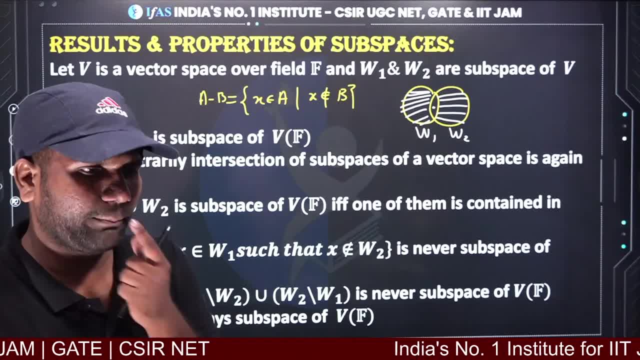 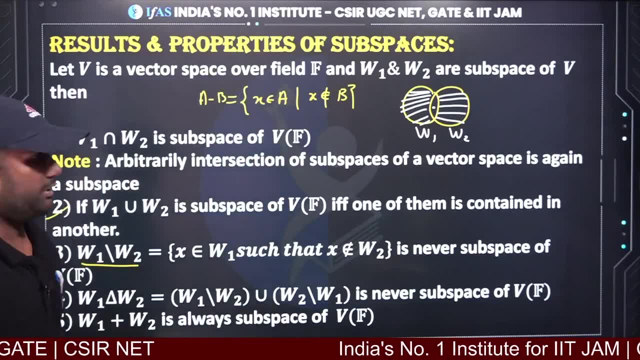 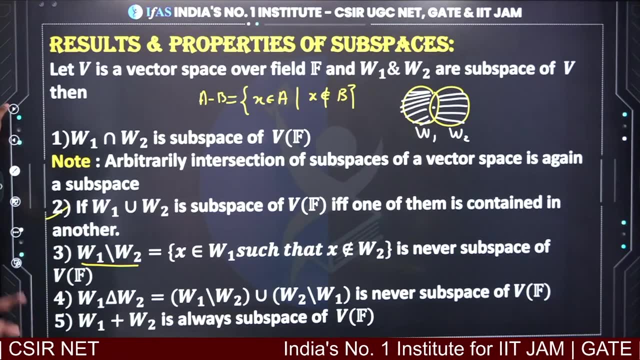 According to me, what you have written may not be like this. Still, you tell me once it may be possible. you may have thought of something. Now remember these things: W minus W2 will not be a subspace. There is no symmetry difference, there is no complement. 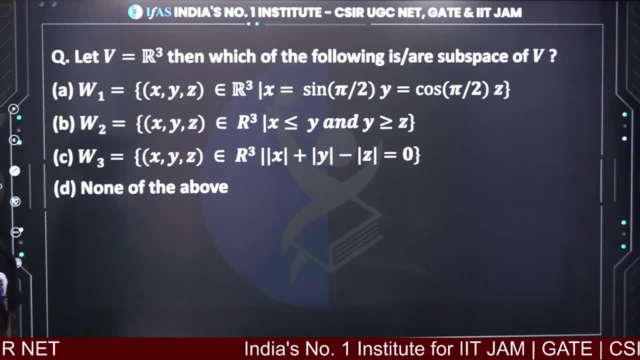 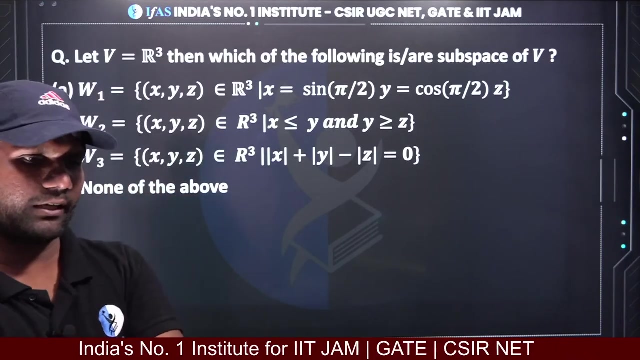 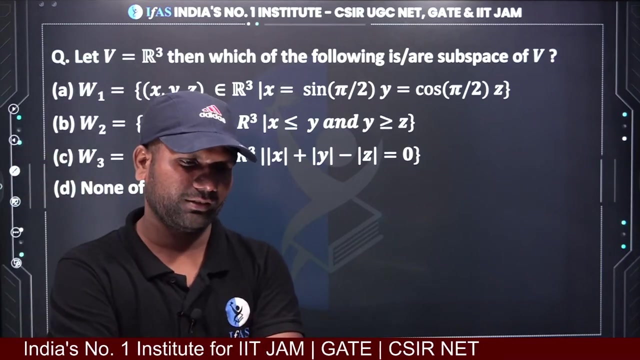 Union is also not necessary. there is always an intersection. Tell me about this. which subspace will be there in this See? Determinant of A minus TI is characteristic polynomial. Yes, yes, yes, absolutely right Now I will go and click the determinant of A minus TI. 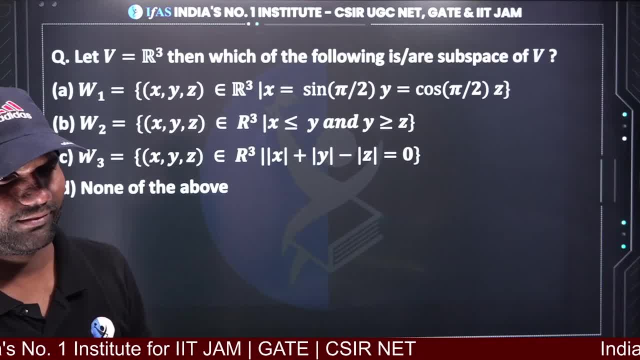 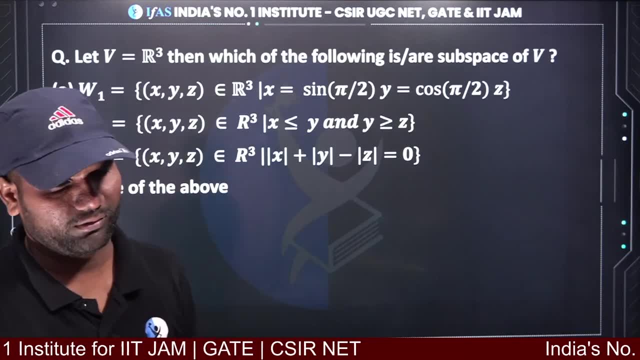 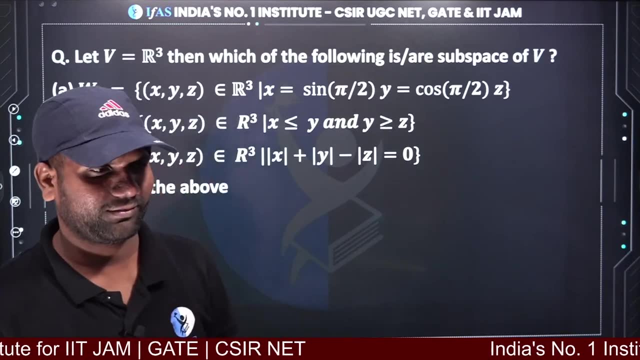 Yes, yes, yes, absolutely right, Yes, yes, absolutely right, Yes, absolutely right. double C is absolutely right. Now go and click me. It was a good observation of yours. Actually, what you wrote last time I was not able to click, what are you saying now? 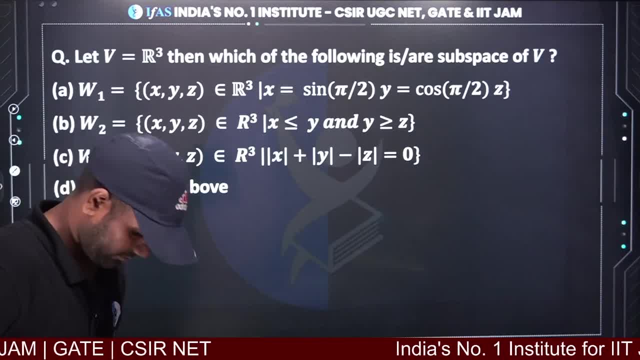 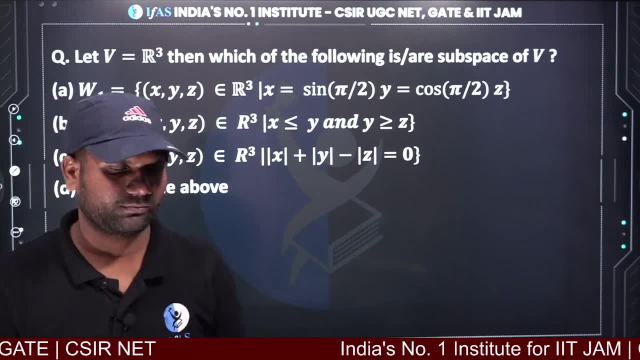 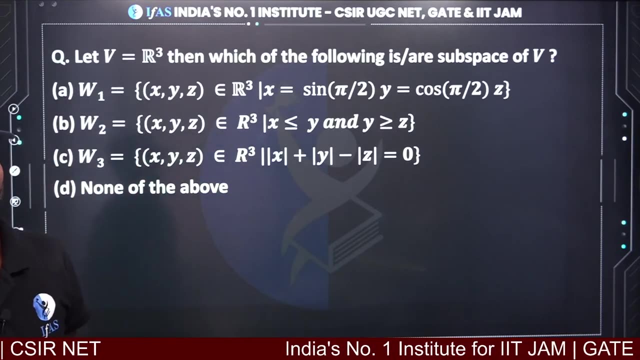 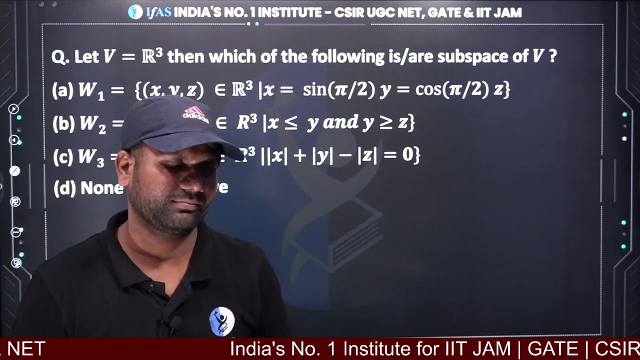 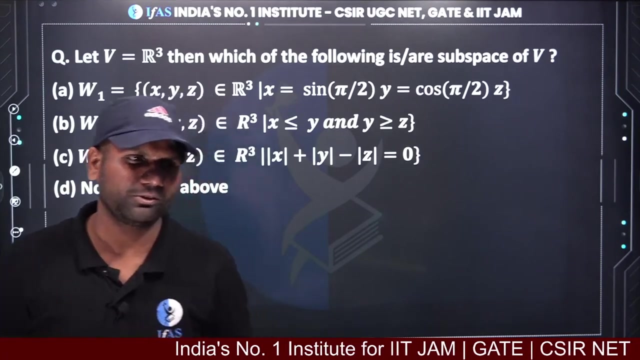 Yes, you can do it anyway. You can apply L-Hospital by doing this. Then it is possible from there. By the way, you observed. well, Ok, By the way, you made me happy, Come on. very good, Your observation was very good. Tell me about this. 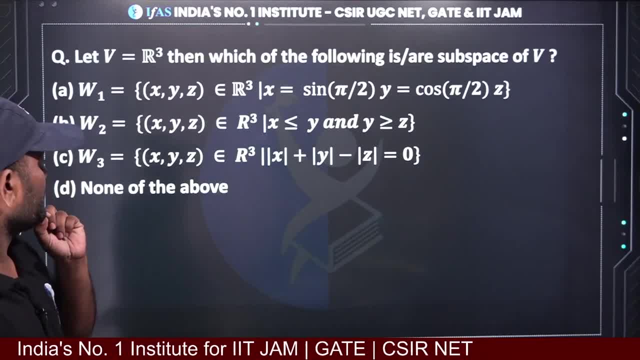 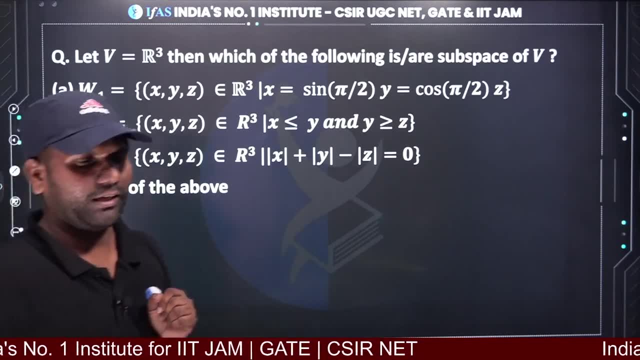 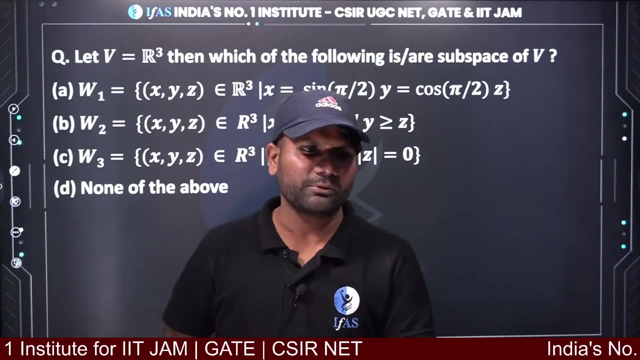 Will C be made? I think C may fail. No problem, double C. Actually this happens sometimes. Sometimes, what the student wants to say, If you were in front you would have told me absolutely. Now. if you were not in front, then typing By typing, the whole emotion cannot reach. 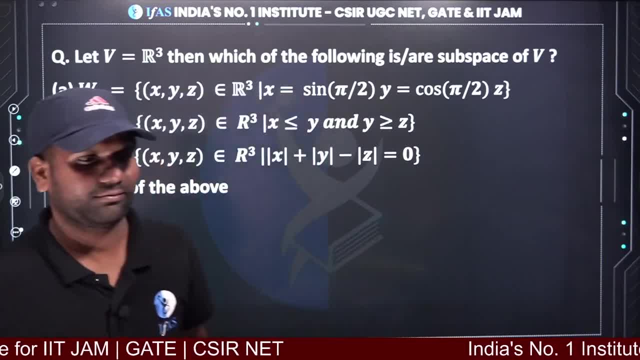 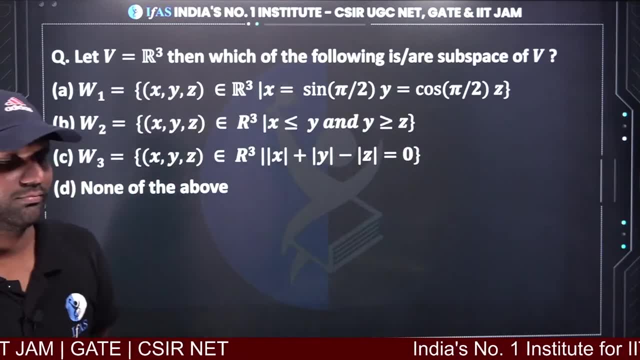 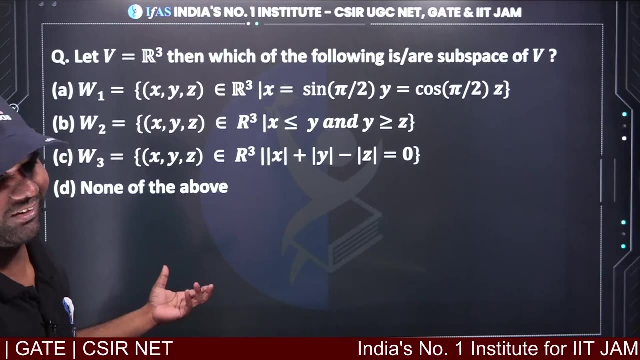 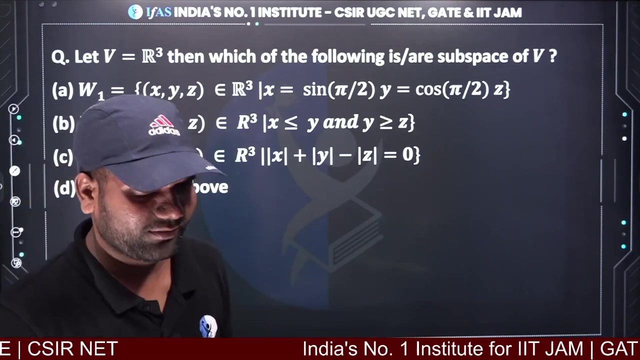 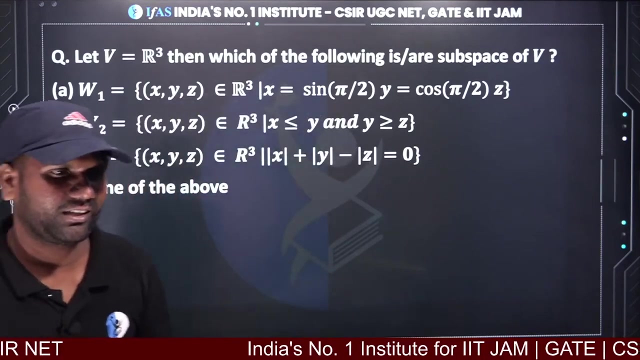 As if you finally went and finally reached, D will be none of the above. What are you doing Once? check carefully, Look carefully. Who has Alpha? Very good, Abhiya Joy. Abhiya Joy gave the correct answer, According to me. let's check once. 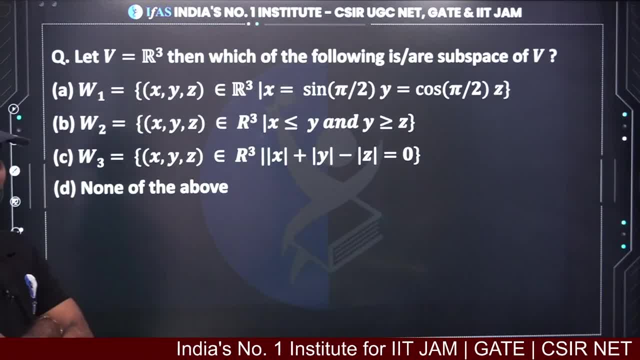 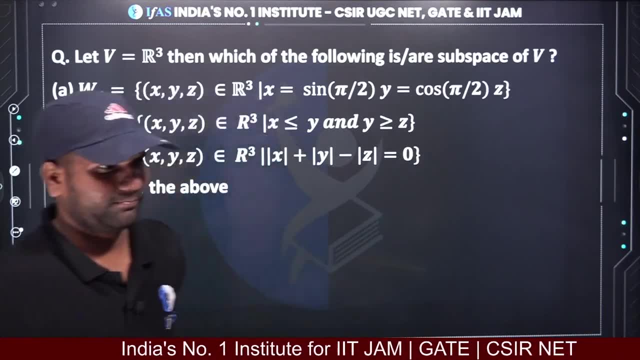 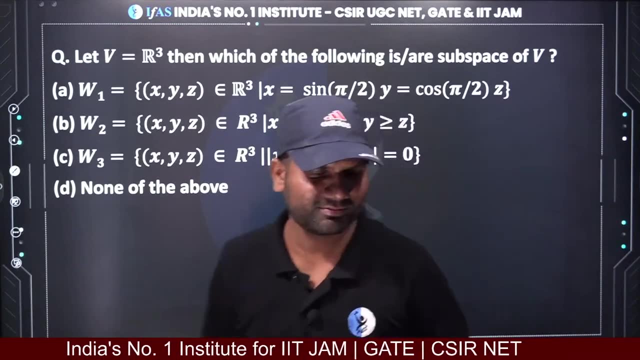 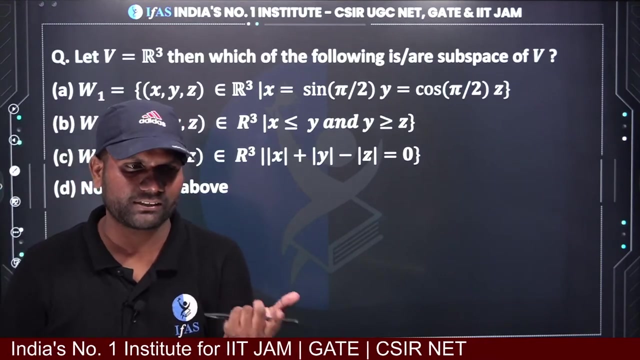 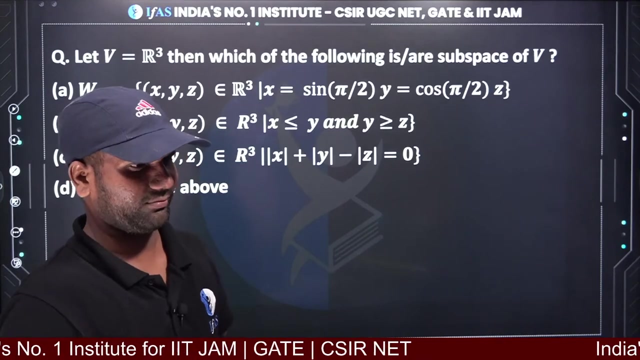 Let's see Only A, Only A. Yes, absolutely correct. Tell me the counter example for B and C. Do you have a counter example for B and C? Come on, tell So guys, the new people who are joining. So like the session, You guys? If you have not liked? 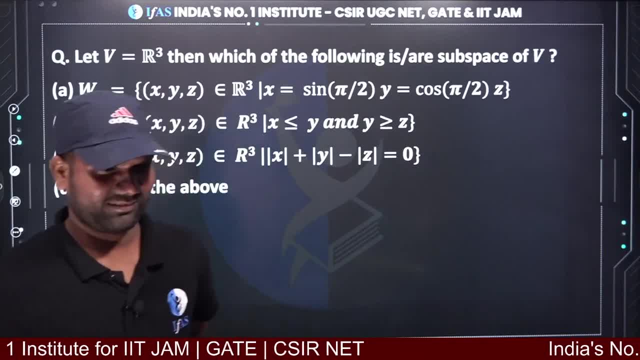 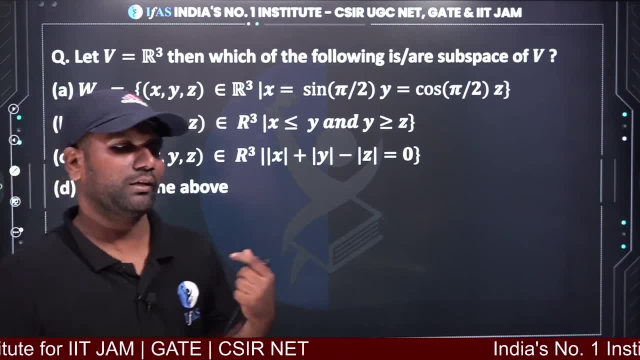 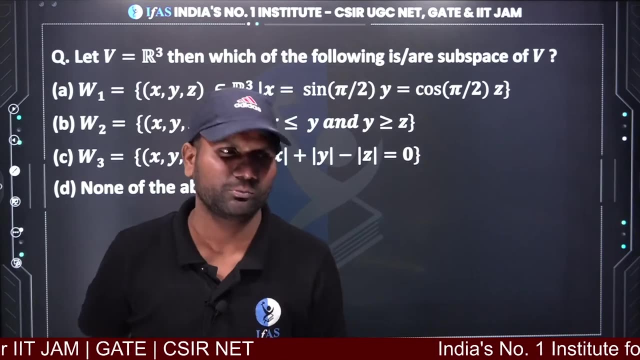 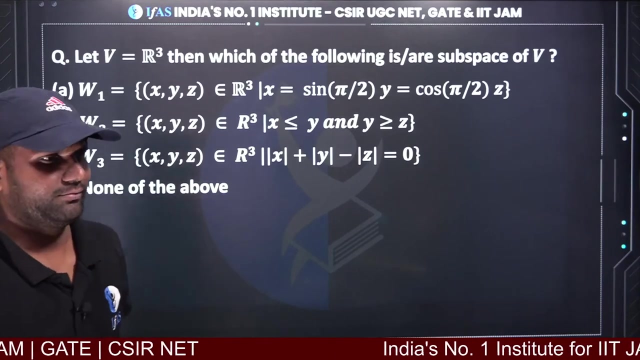 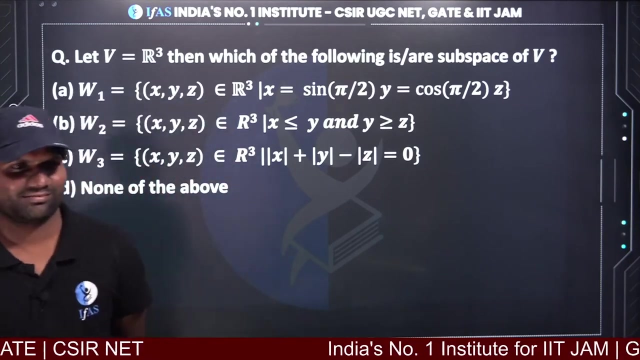 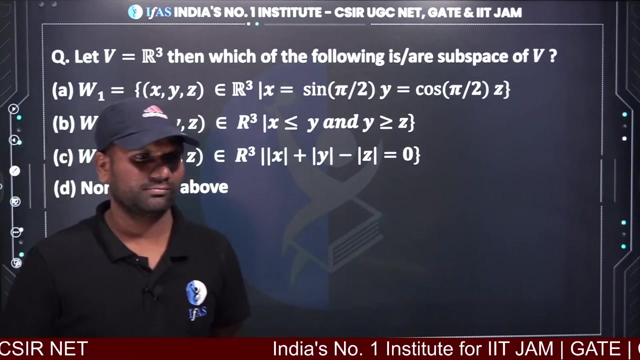 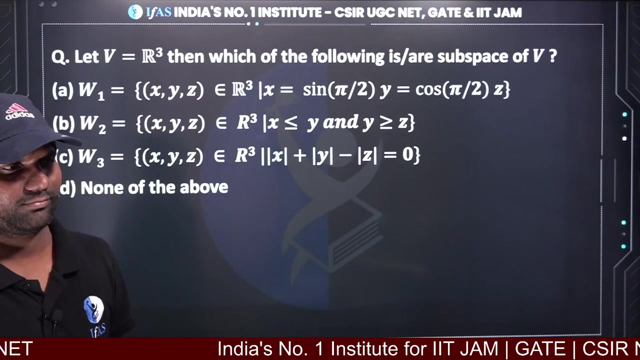 If you have not liked, If you like, If you like, I want to do it. If you have not liked W, So look here, guys, here I will tell you about W1,. till then, you guys, tell me a counter example for W2 and W3,. 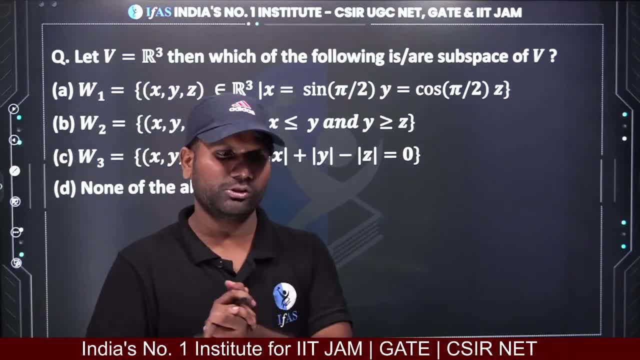 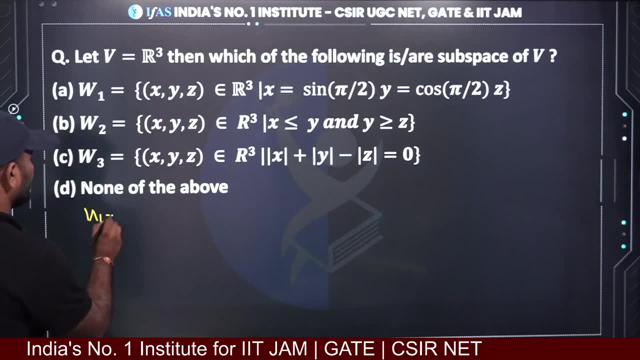 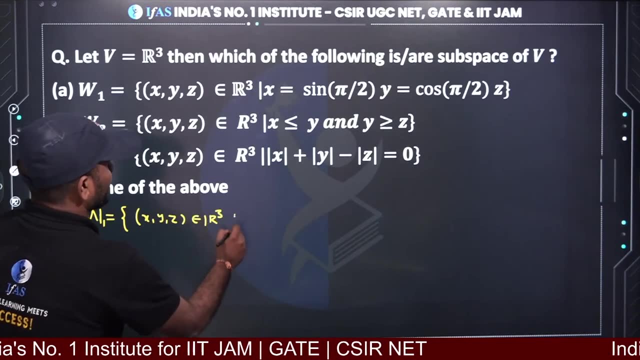 because if you are going to give an exam then you should have a counter example. right? you guys will tell me a counter example. look here: if I talk about W1, what is given in W1, in W1, such three tuples come x, y, z belongs to R3, where x is what sin pi by 2, sin pi by 2 into y. 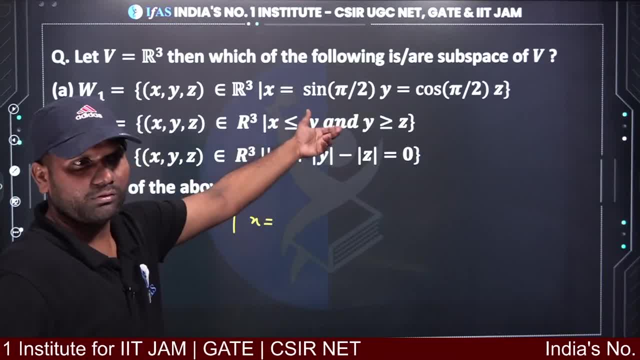 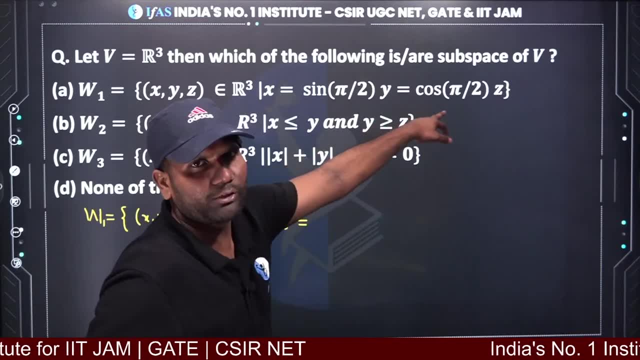 sin pi by 2 means what will happen. sin pi by 2 means sin pi by 2, sin 90. what happens 1, 1 in into y, so 1 happens. and cos pi by 2 into z. cos pi by 2. what happens 0, 0 into z means 0, so this has been given to you, W1, right. 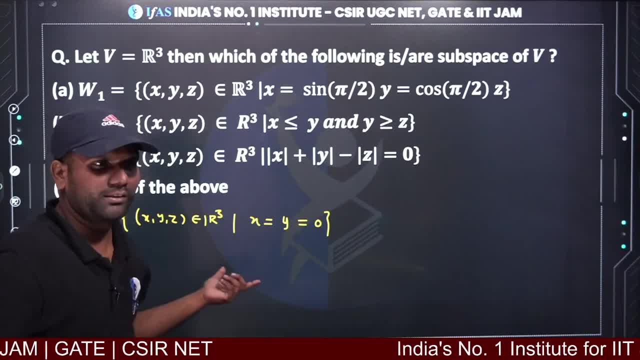 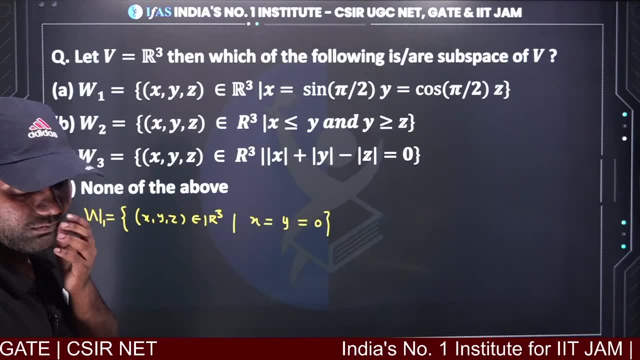 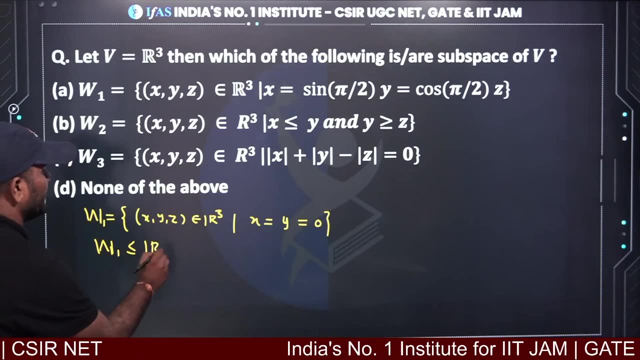 Ajay Mishra has also come. this has been given to you: W1,. this is W1,. this is W1,. now, if W1 is given to you, clearly, if you check W1, what will happen? sub space of R3 will be made. 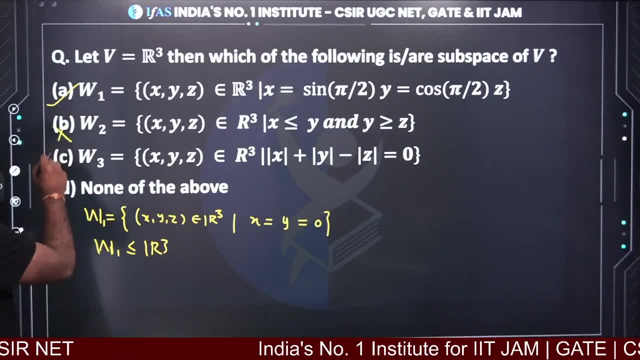 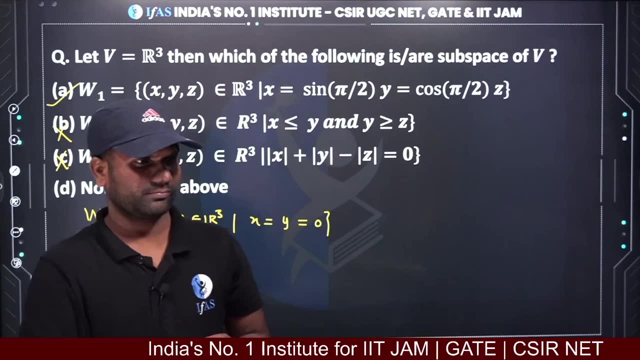 with respect to which F1 will be given to you, the first one will be correct, according to me, and c should not be. did I tell you guys? tell us the counter example, what will not happen. for what are you laughing here? 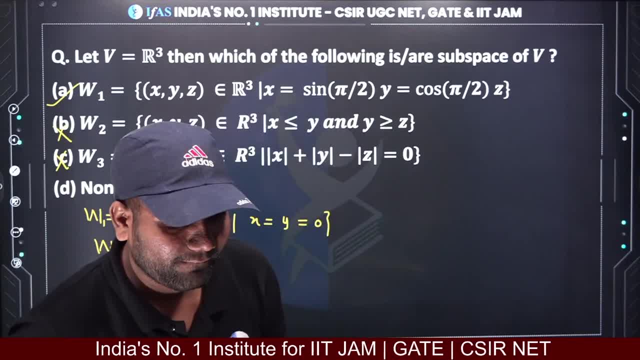 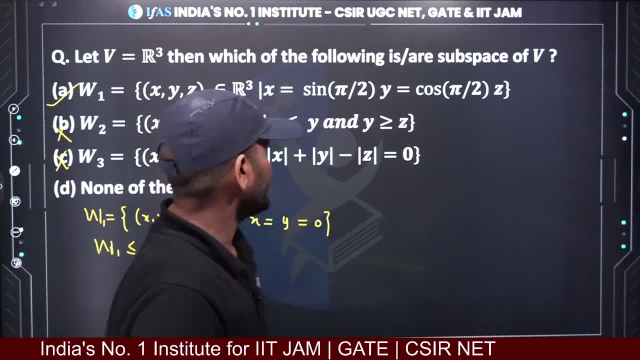 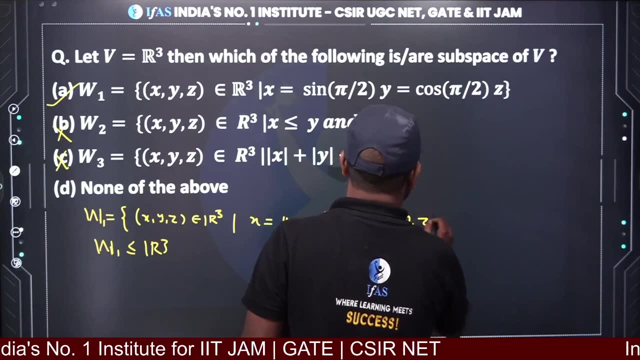 well, sir, probability again right, Morley, can anything? Olerle, anything can happen. if Z can happen, it means what is our set? it has been given to us 0,, 0, Z has been given so that Z belongs to R. so 0,, 0, Z is there, so 0 will come inside it. 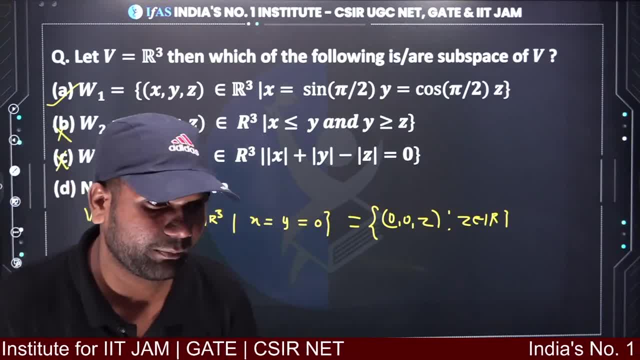 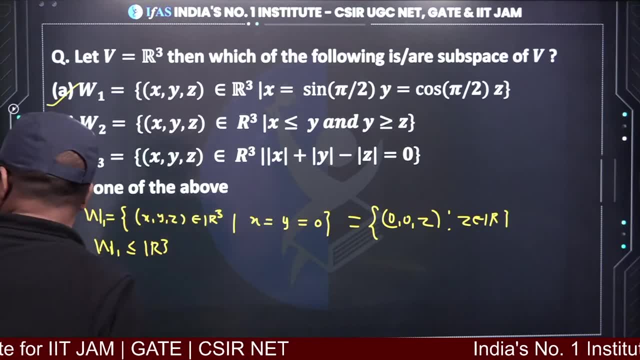 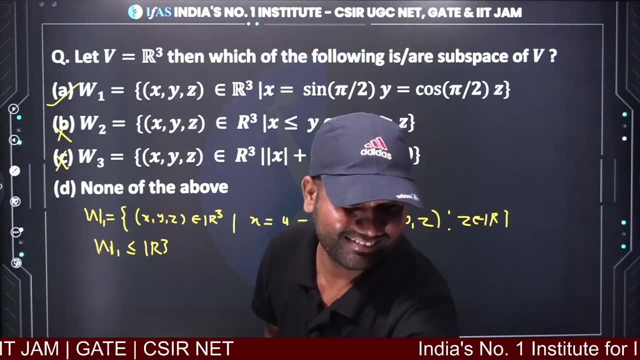 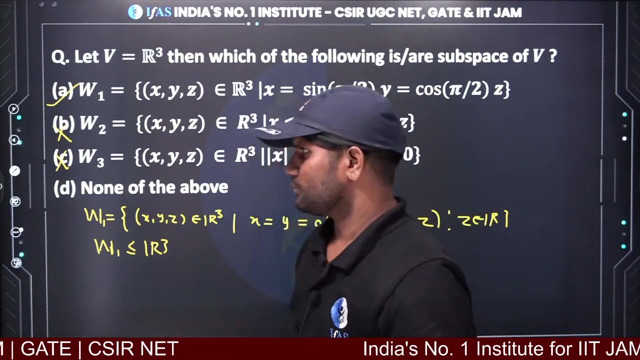 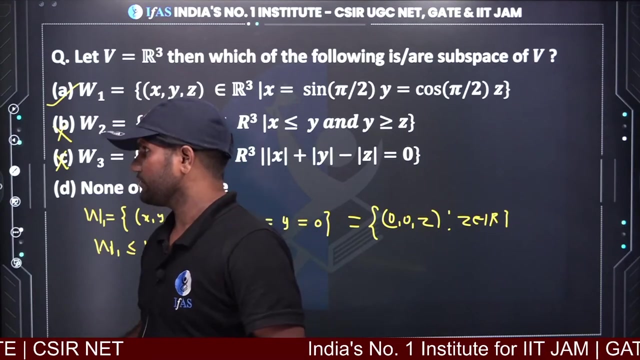 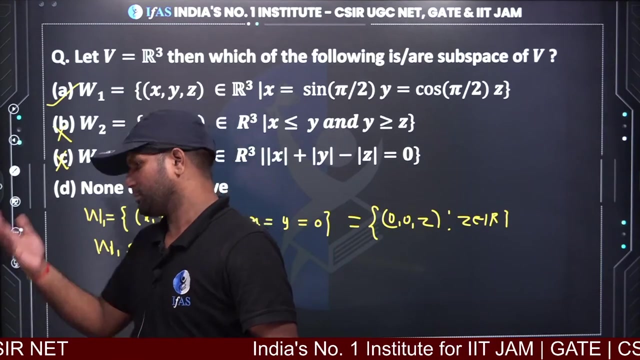 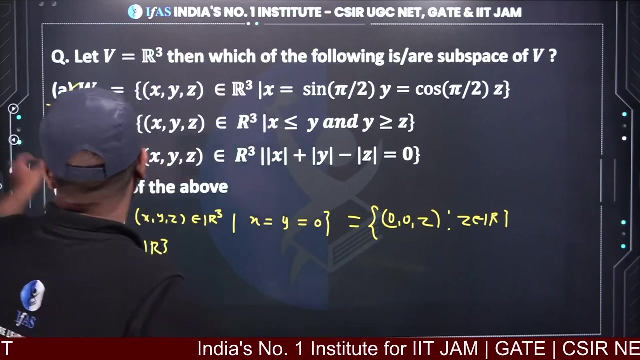 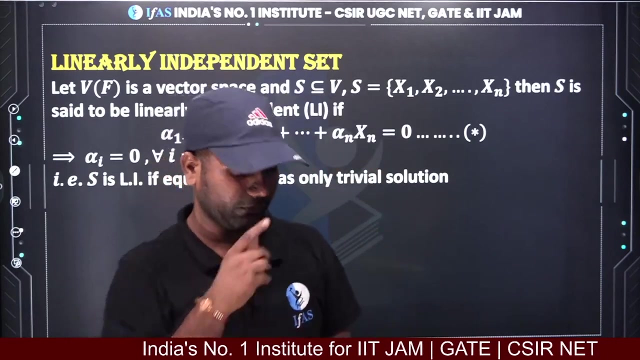 yes, absolutely, very good approval. Pallavi Rani is also telling for W2,. yes, absolutely, the mod one fails, it does not happen. okay, thank you very much. yes, let's move on to the next question. yes, now let me give a little information about linearly dependent and independent. 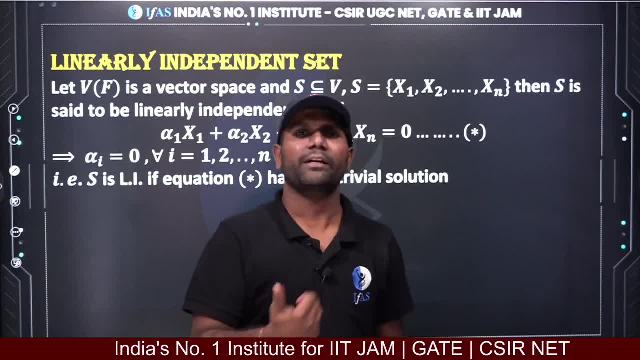 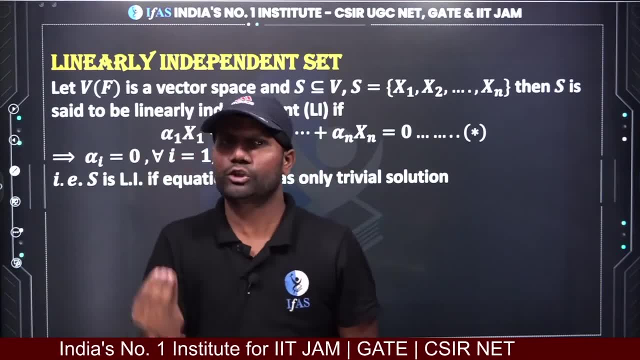 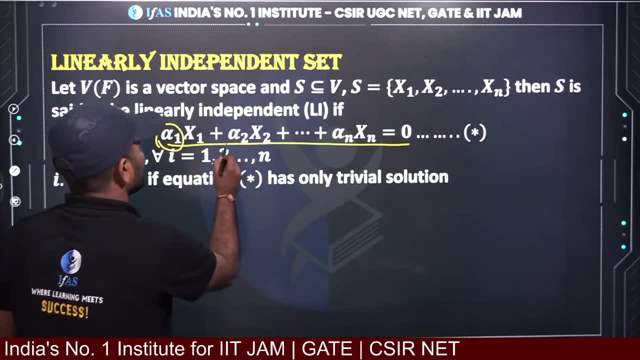 right. when do we call any set linearly independent? a set is set to be linearly independent if we take their linear combination. suppose whose linear combination is equal to. we took 0, like here you guys are looking, we took zero from linear information. if it is a linear combination, let me tell you how many. 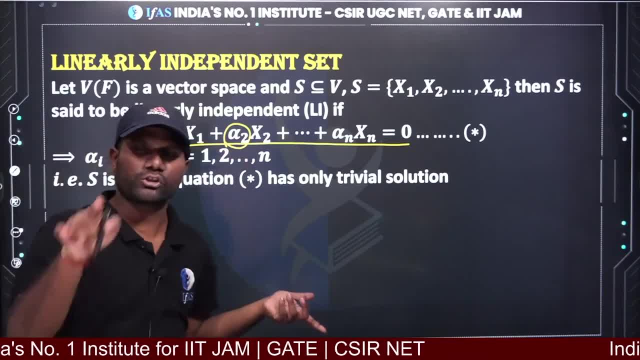 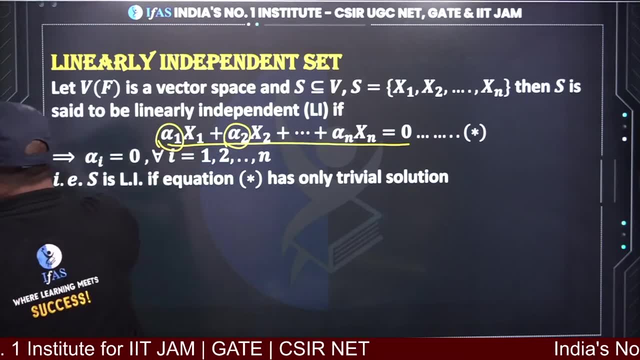 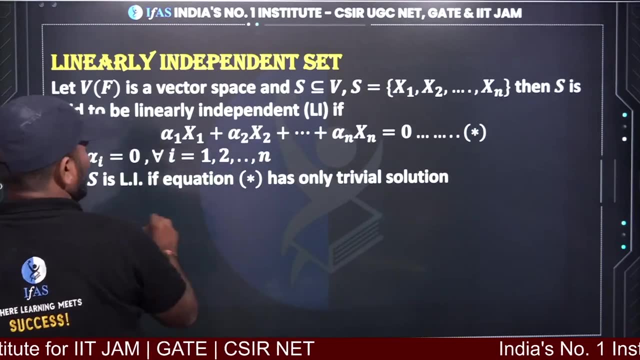 I am saying that this linear combination will be possible only when all the scalars will be zero. otherwise it will not be zero. or in another way we can say this: you understand it as an equation. understanding the equation means what will happen here. the value of α1, α2, αn should be zero. 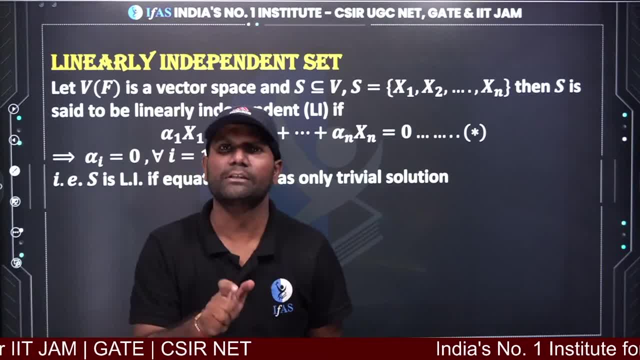 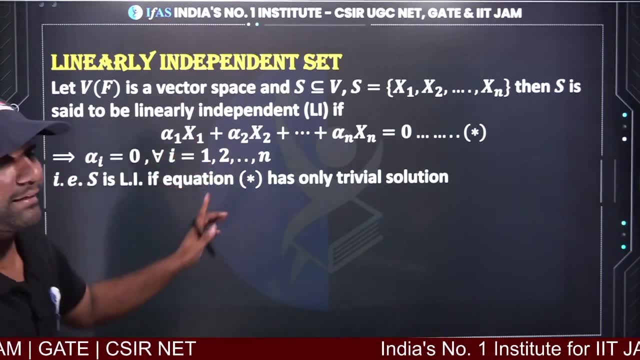 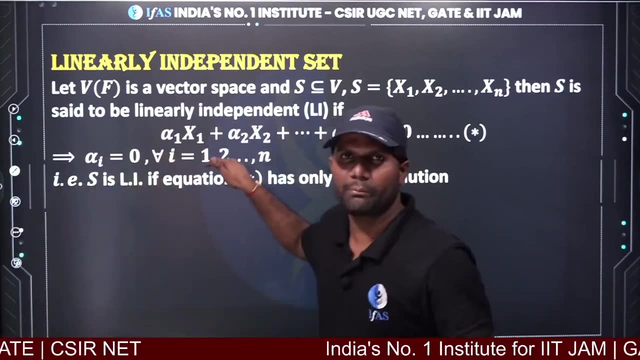 this means this equation is near the star. if there is only a trivial solution- trivial means if there is only zero solution- then we will call that set linearly independent. first take linear combination equal to zero. tell that all the scalars are zero, then only that linear combination will be equal to zero. 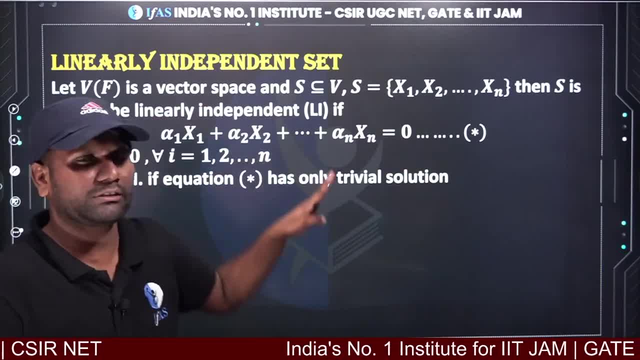 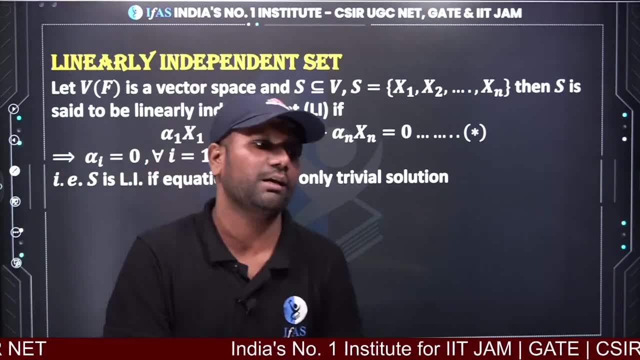 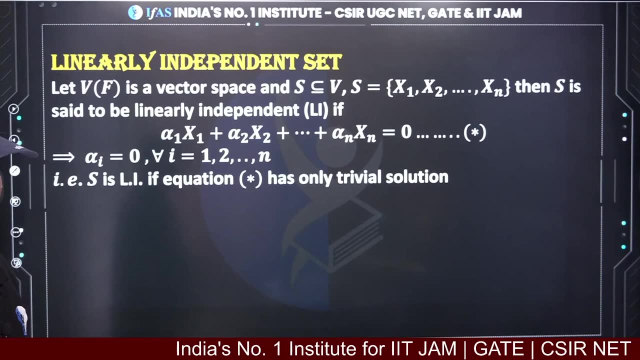 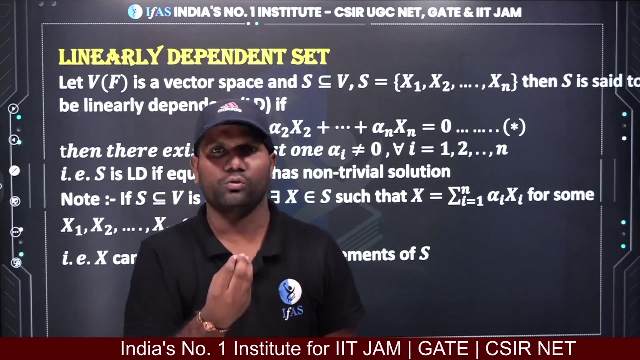 or both are same, or you tell that the equation is near the star. only trivial solution. in that case you can say that the set is linearly independent. understood. now let's talk about linearly dependent set. if you take linear combination equal to zero and tell that any value of αi is possible, 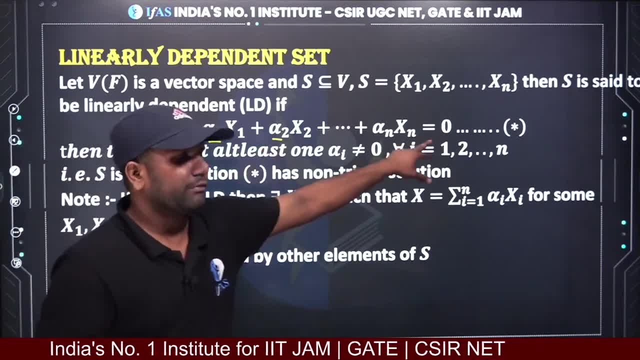 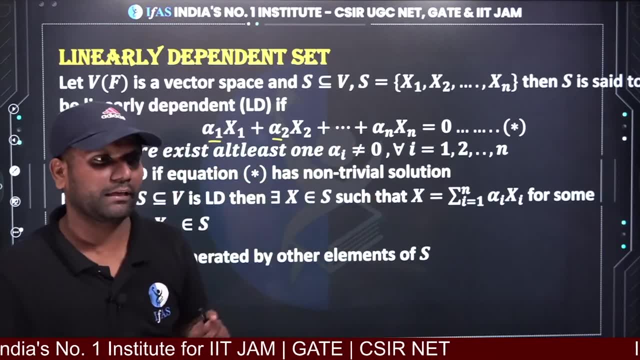 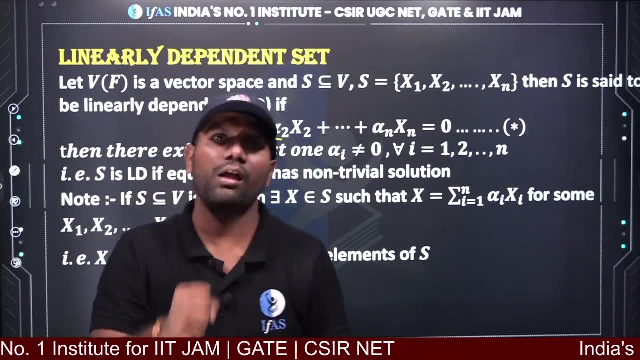 in another way you can say: if you take equation star, you tell that equation star will have trivial solution because it is homogeneous, it also has non-trivial solution. if it has non-trivial solution, then what will happen? it will become LD. I hope you understood the meaning of Li and LD. 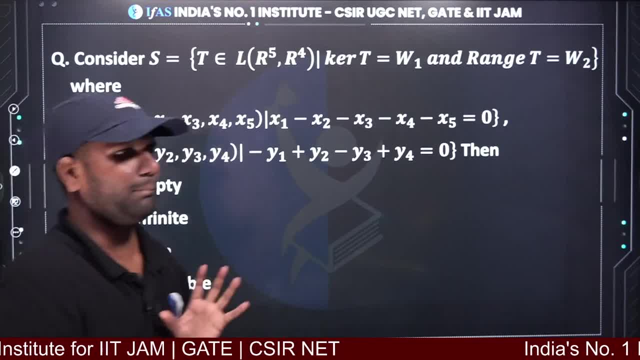 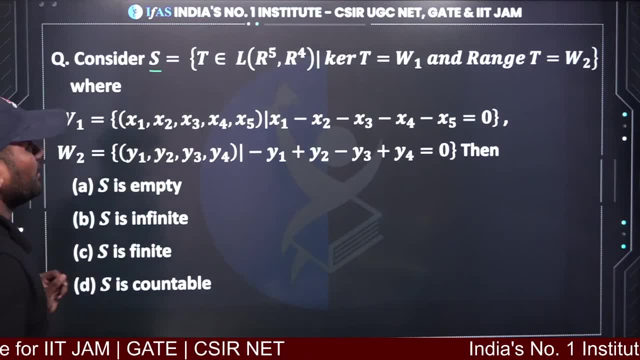 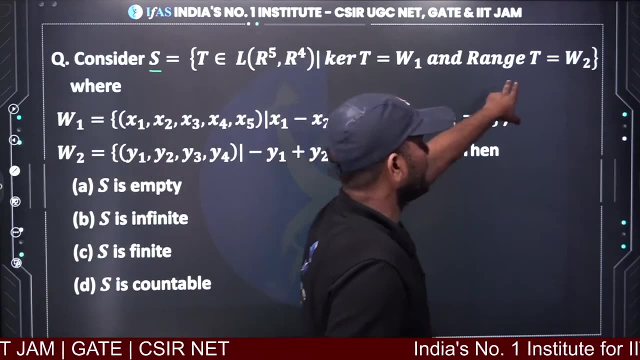 now, let's go now. here is a question for you. it is a good question. let's see how many people solve it. here we are given a set. S contains linear transformation from R5 to R4. kernel of T is W1, range of T is W2. 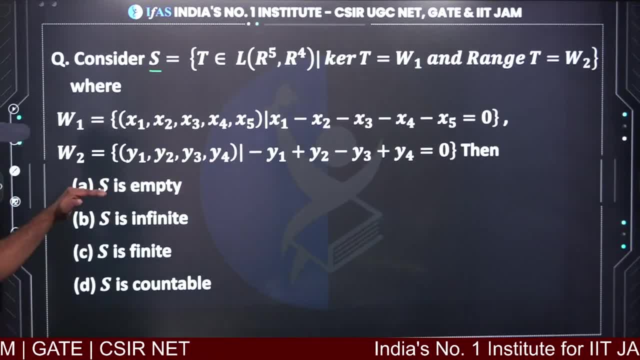 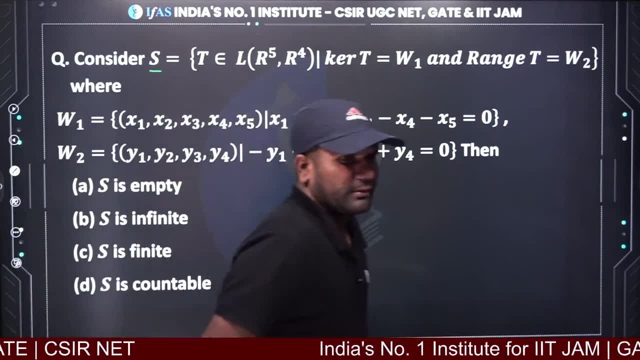 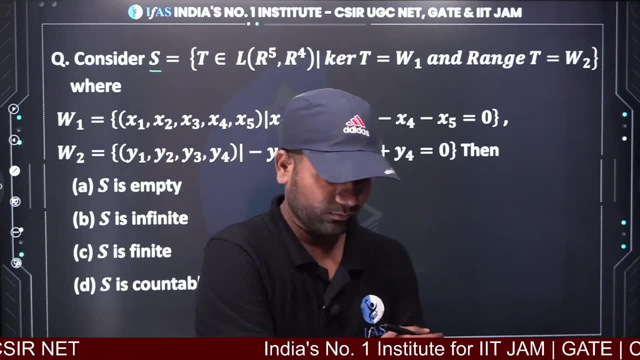 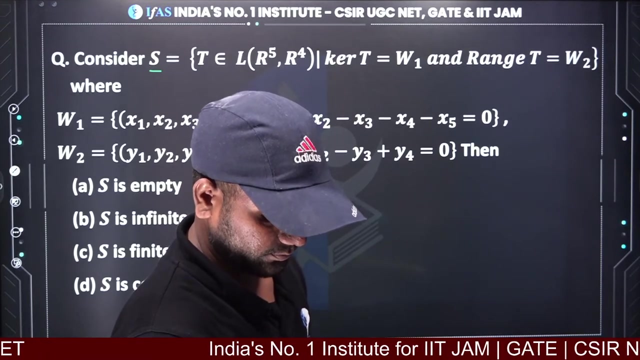 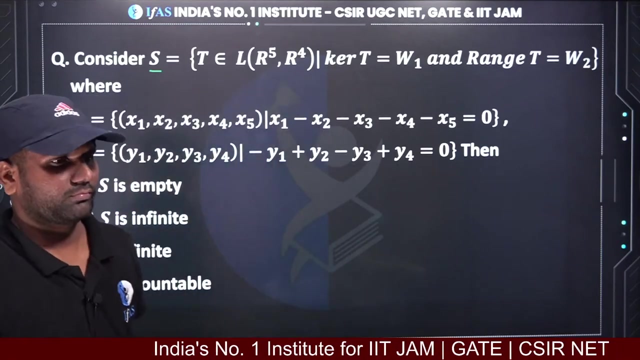 now W1 and W2 is this set? now you have to tell what will happen. it will be empty, it will be infinite, it will be finite, it will be countable. what do you think? what can you say? can you say something? yes, it will be A. 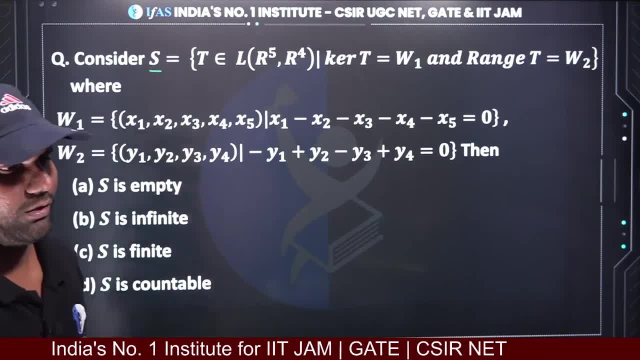 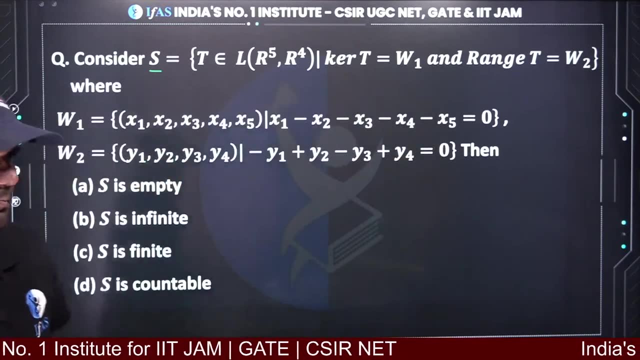 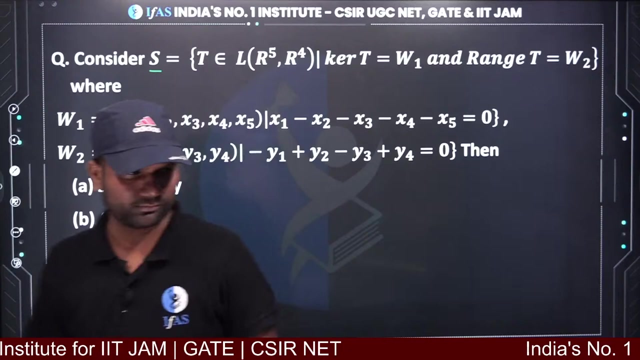 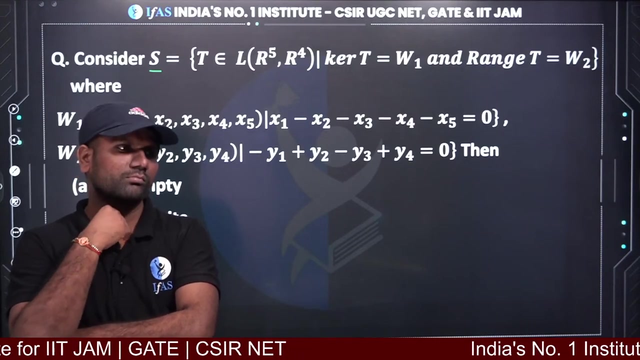 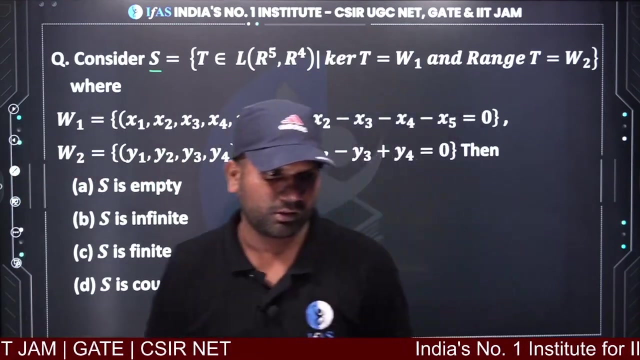 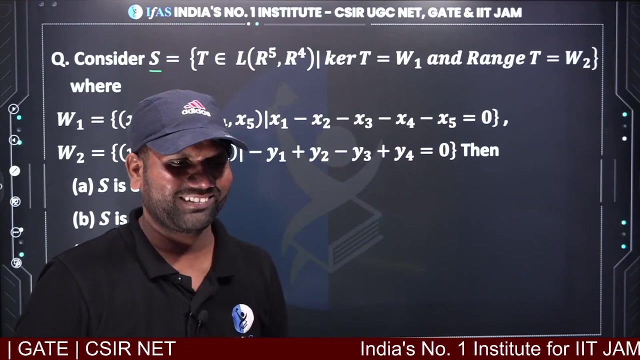 it will be S, S is empty. ok, what are the others saying? this one is D, S is countable. ok, other students tell me, tell me. okay, guys, quickly tell us what will be your answer. what will happen? so so far, no one has given the exact, proper answer. you guys read real too. 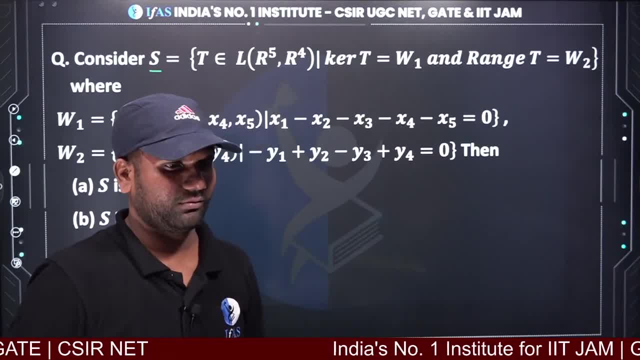 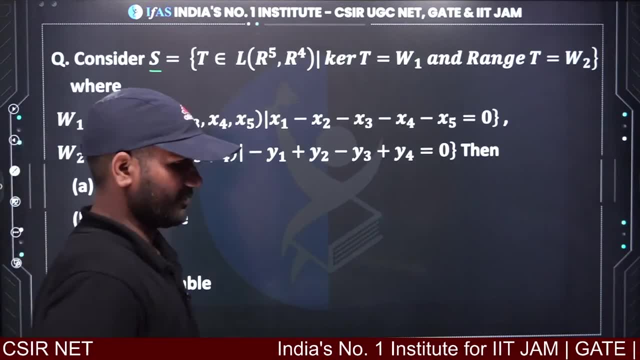 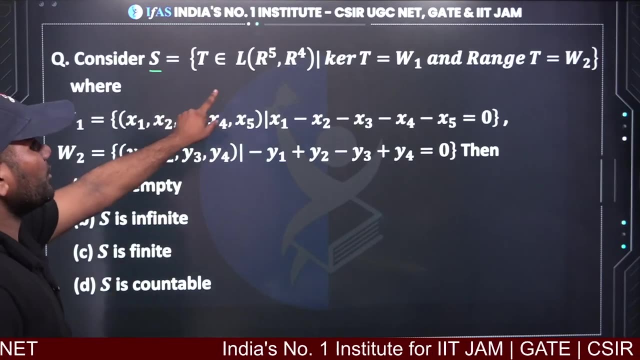 you read real, then tell me they are saying it will happen. princess is said to be finite. we will say C will happen here, guys, first of all see W1 is what. W1 is a kernel and W2 is a range and T is a linear. 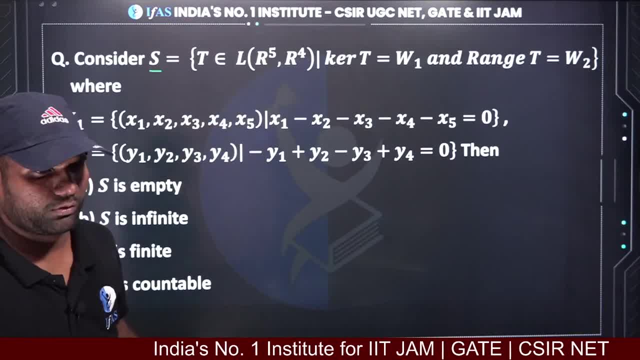 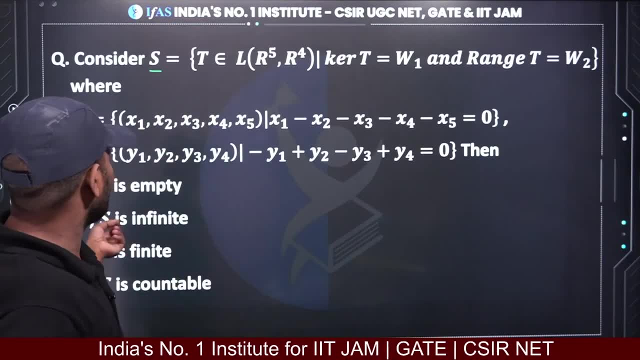 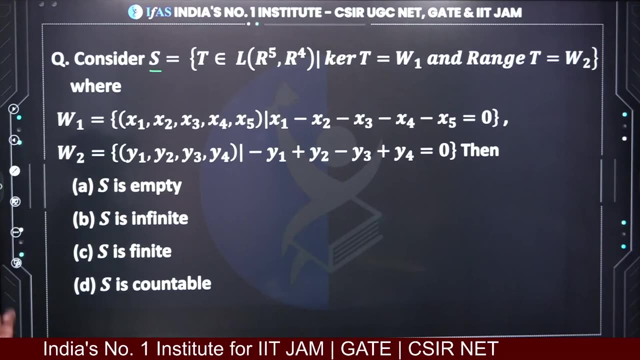 transformation from R5 to R4. OK, now look here. W1 is given means we are given kernel W1. it nothing but Kernel T, and W2 is nothing except kernel T and W2. nothing, nothing but range. so here, first of all, we will find dimension of w1 and dimension of w2. so what? 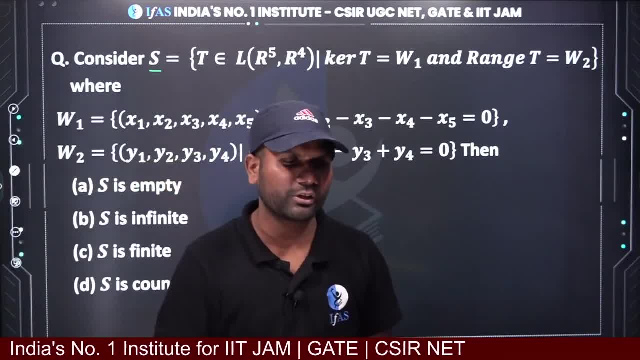 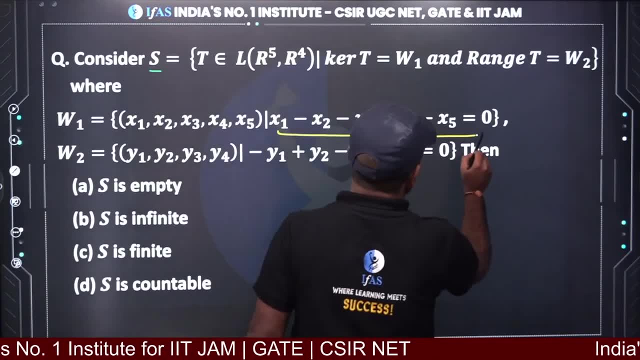 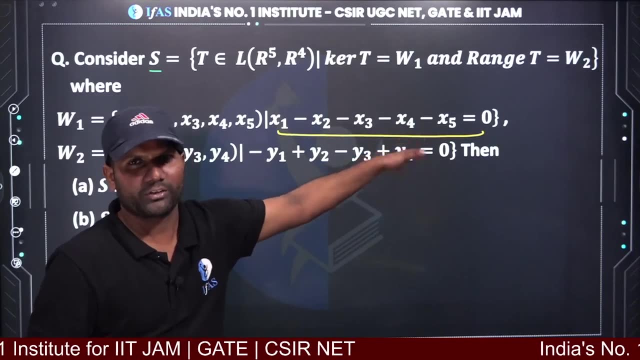 is the dimension of w1. if you find the dimension of w1, then what will you get see here if I talk about w1? so in w1 you are seeing how many elements are there? 5 elements, but from this I can write any element in the rest of the linear combination. from here we clearly know that its dimension will be 4. 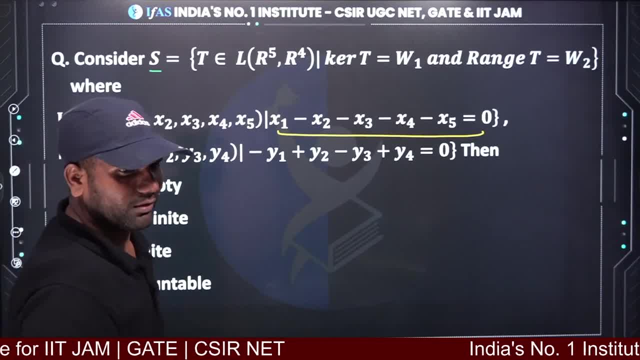 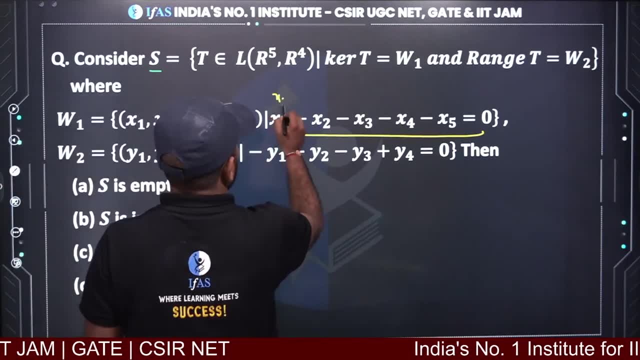 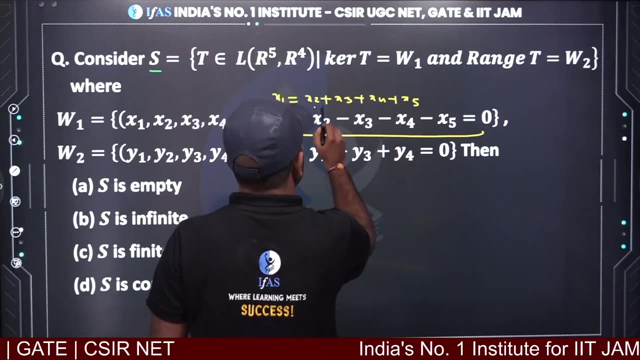 right. what will be its dimension? alpha 1, w1 will not be 1. see, this means you can write x1 like this: x2 plus x3 plus x4 plus x5 means, if you have x2, x3, x4, x5, then you can make x1. so its dimension clearly, you can say: 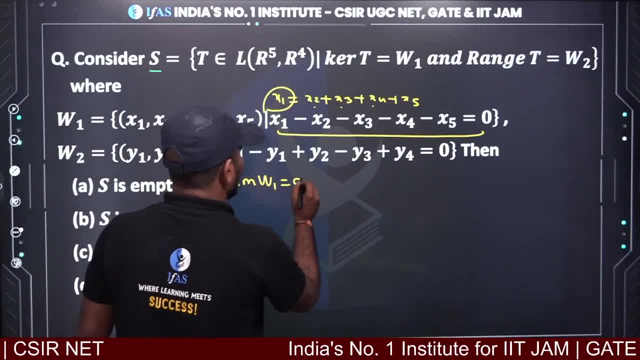 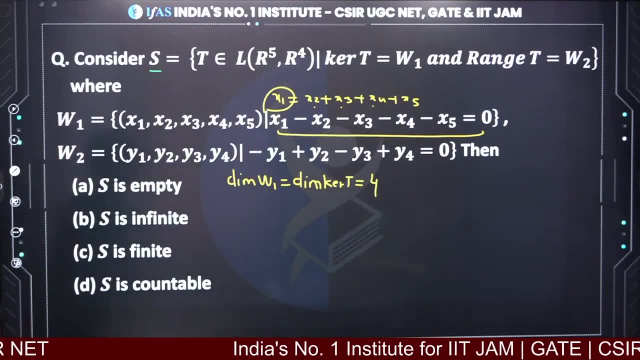 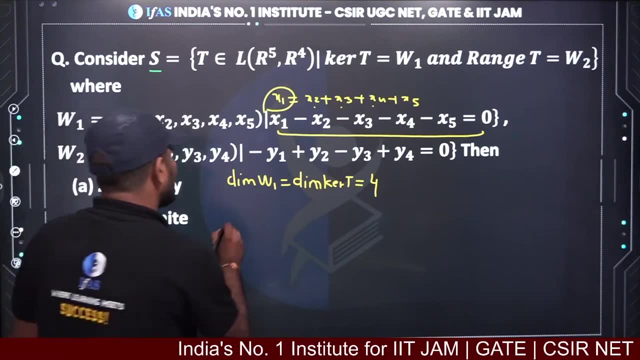 dimension of w1. dimension of w1 means dimension of kernel t. dimension of kernel t, what is given is dimension of kernel t4 is getting ok. similarly, what is the dimension of w2? what will be the dimension of w2 if you see here? so, dimension of w2. so if I talk about the dimension of w2, 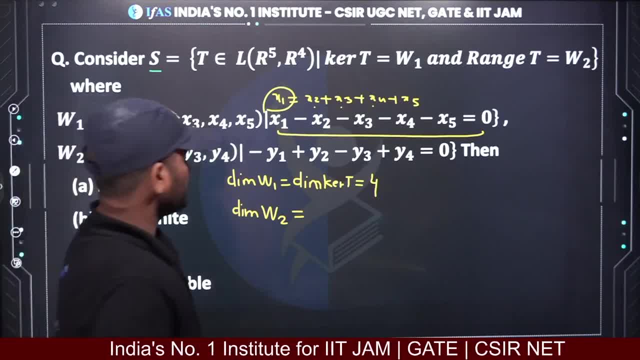 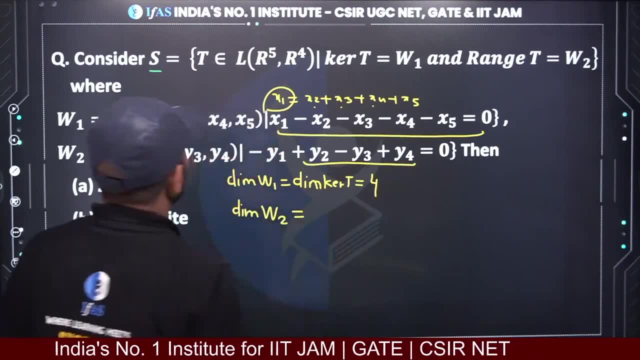 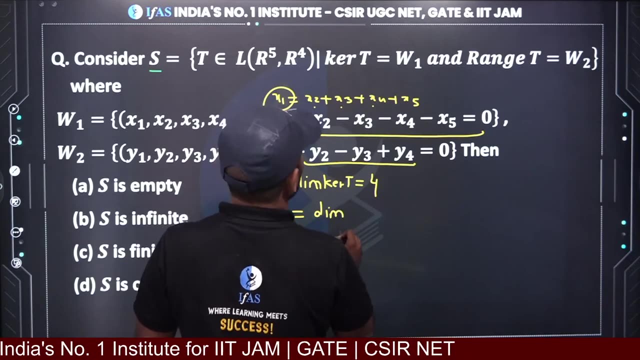 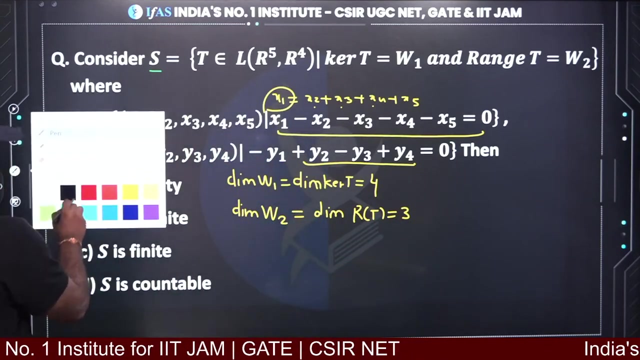 then what will be its dimension? dimension of w2. if you see in w2 then there are 4 elements. so what will be its dimension, its dimension of w2? how many elements are there in w2 and w1 transformation 3. ok, so if you are able to observe here, 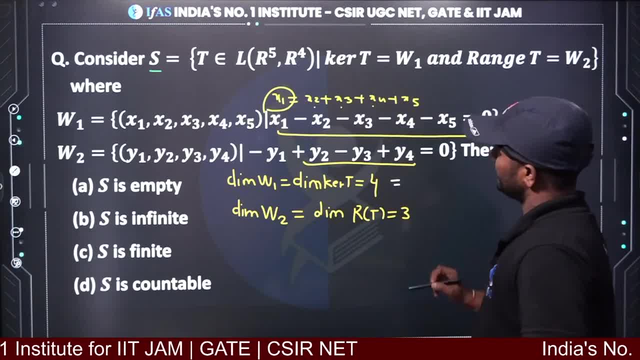 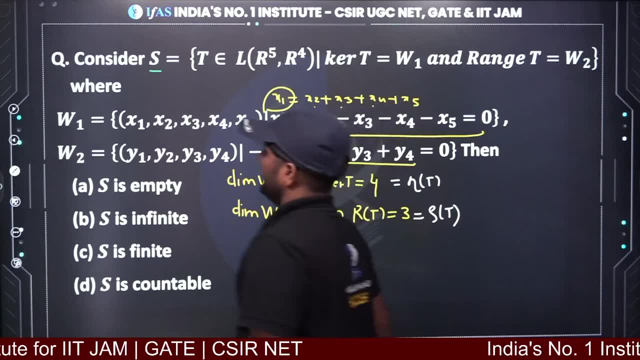 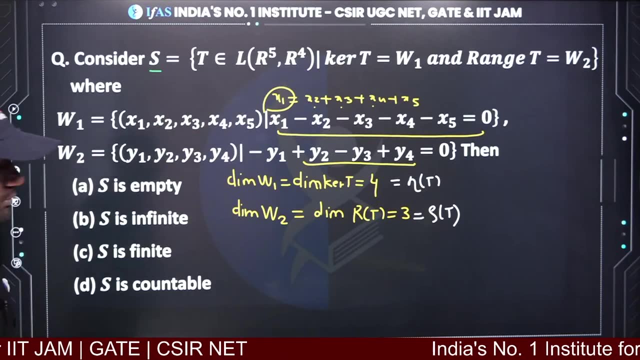 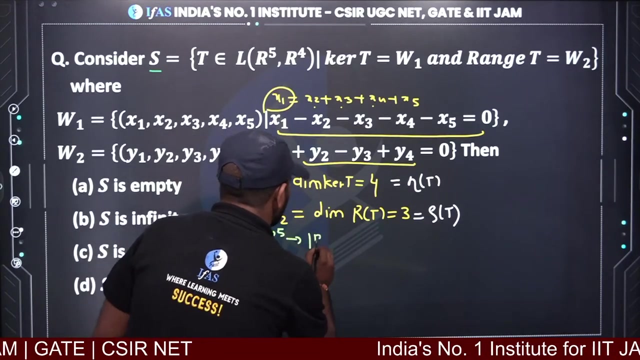 can you see? if its dimension of Kernel T is 4, then nullity is 4 and its rank is 3. and what has been given to us, we have been given T, is a linear transformation from R5 to R4. what has been given to us, T is a linear transformation from R5 to R4. ok, now we will apply rank and nullity theorem. 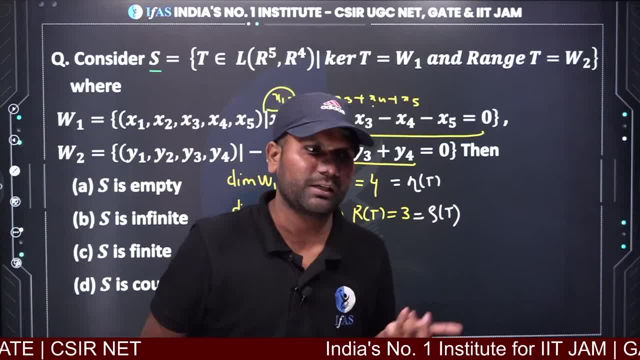 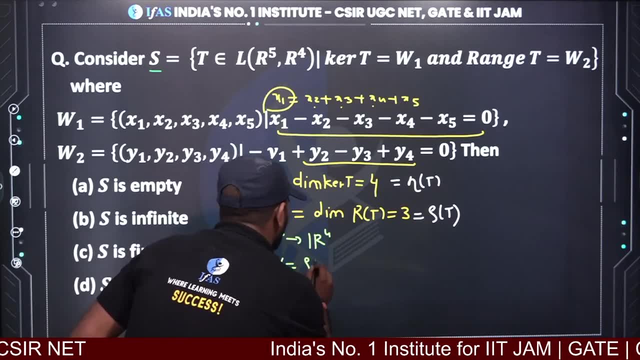 if you apply rank and nullity theorem here, then what will you get to know? so here rank and nullity theorem will apply. dimension of V. so what will you get? dimension of V is equal to rank of T plus nullity. so here dimension of V means dimension of domain. rank is 3 plus 4. 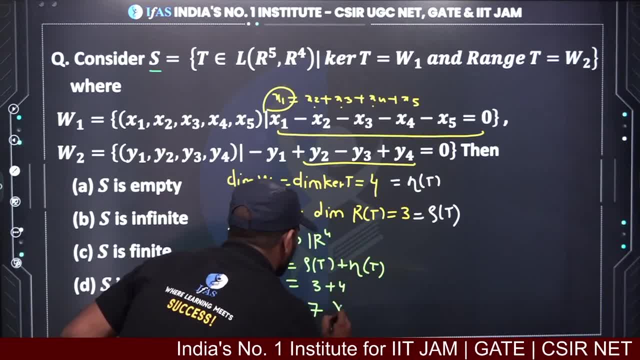 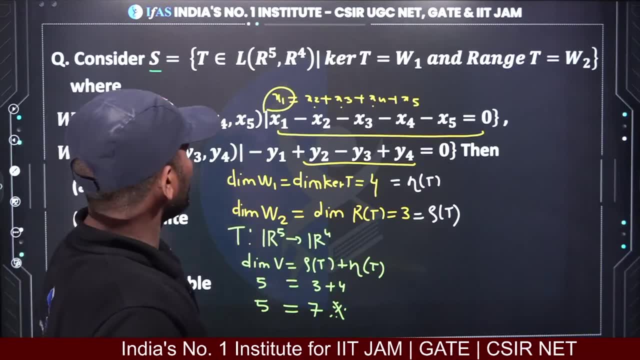 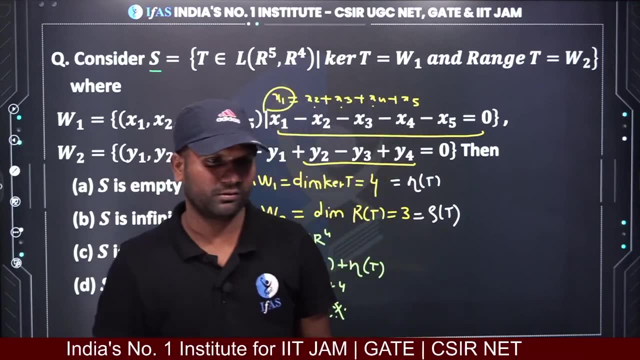 so here somewhere it happens that 5 equals to 7 in real number. we are getting this wrong. its not possible. its not possible. it means there is no such linear transformation where Kernel W1 is found and range W2 is found. understand, so we will not get any such thing. 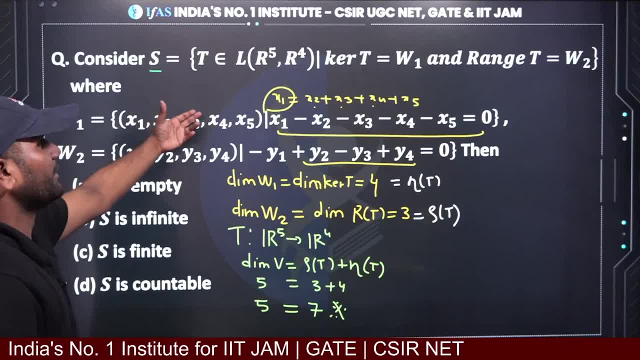 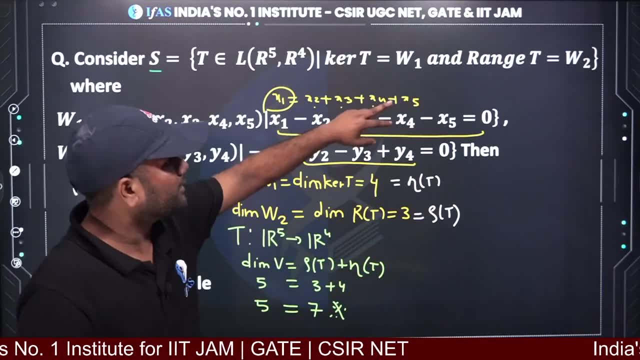 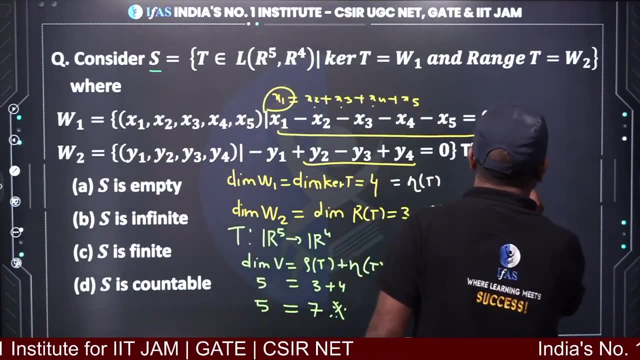 if such a no such linear transformation would not be found, then what does S mean? in S such linear transformation are found where Kernel T is W1 and range of T w2. but this can't happen, this means how many elements will come in S? no element will come in S. so what will happen? your S will be empty. 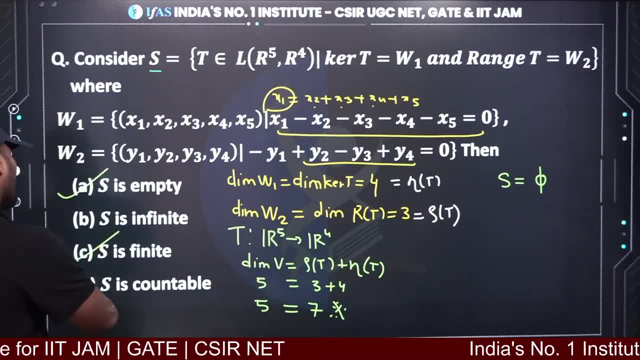 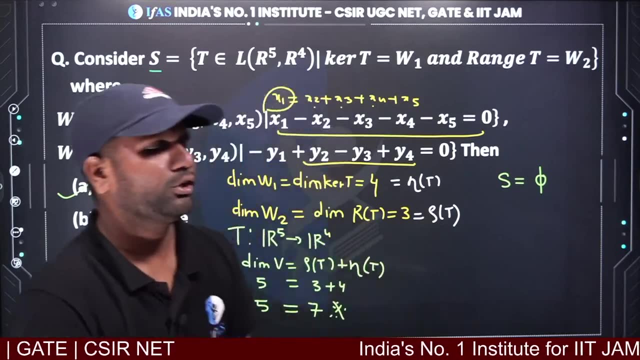 S is an empty set, and empty set is also finite and countable. so from here, A, C and D is the correct answer, understood all of you see once, is it clear? all of you? so, guys who haven't liked the session yet, who are new to it, now, you guys like it. 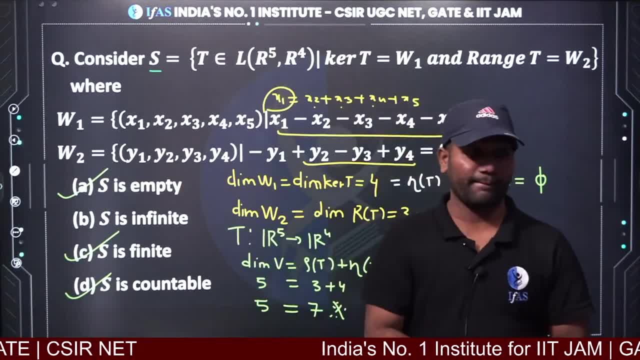 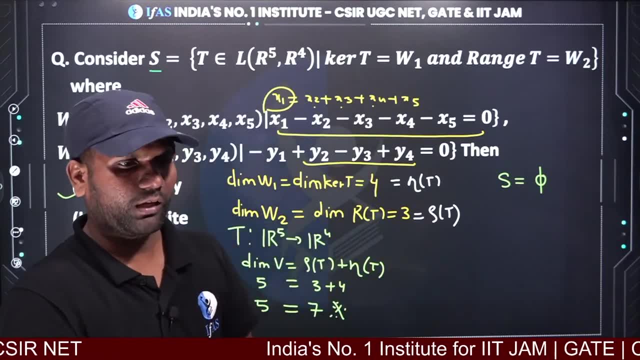 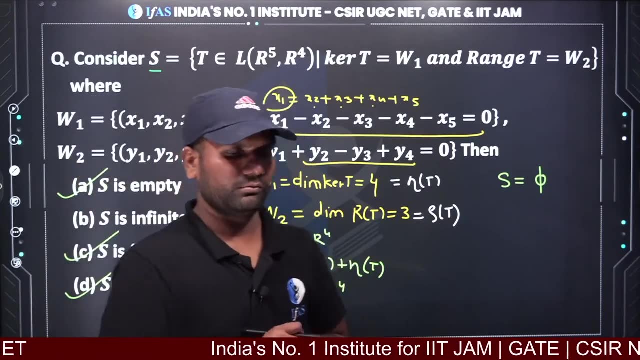 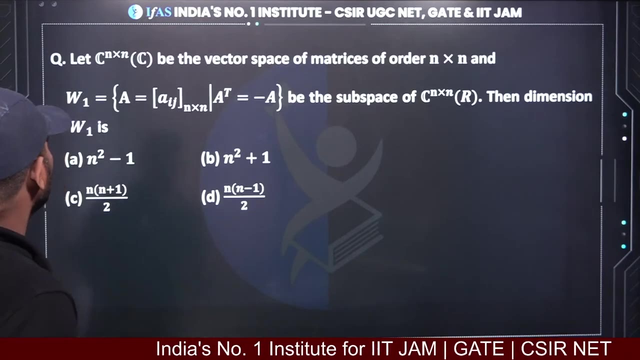 understood see. yes, absolutely. empty set is finite. finite is also accountable. now let's go to the next slide. now tell me about this question. what will be the answer here? let's see n cross n. c be a vector space of all matrices: n cross n. 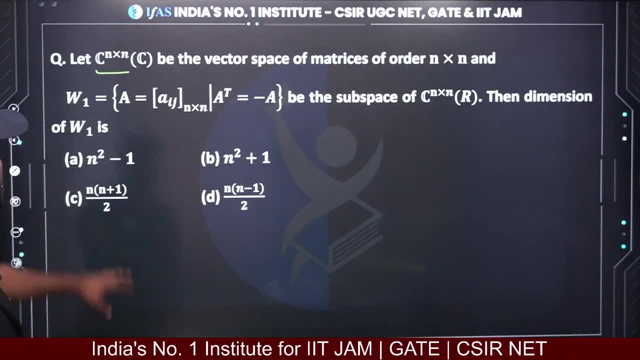 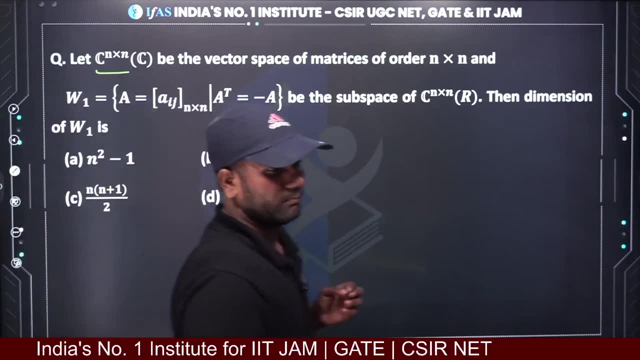 w1 is given to you. it is a subspace of this. so find the dimension of w1 over R. what will be its dimension over R? you have to tell what will be the dimension. see when you go to the exam. symmetric matrix skew. symmetric matrix. 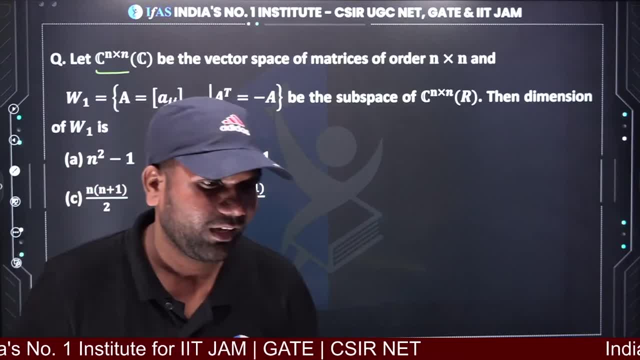 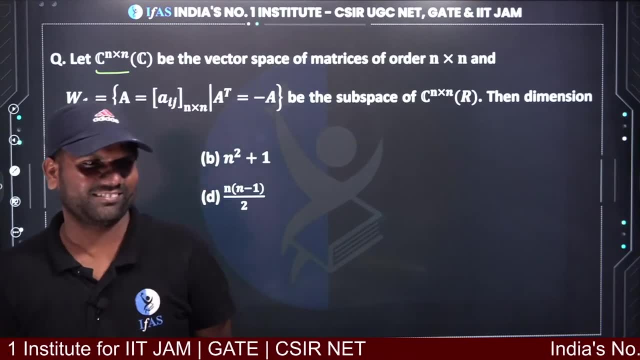 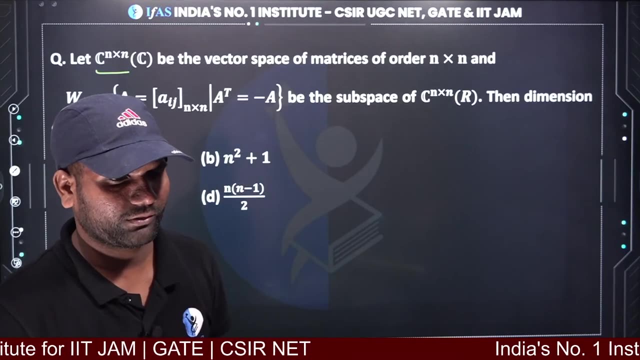 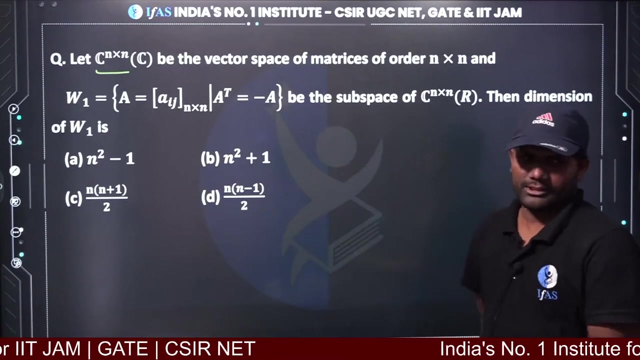 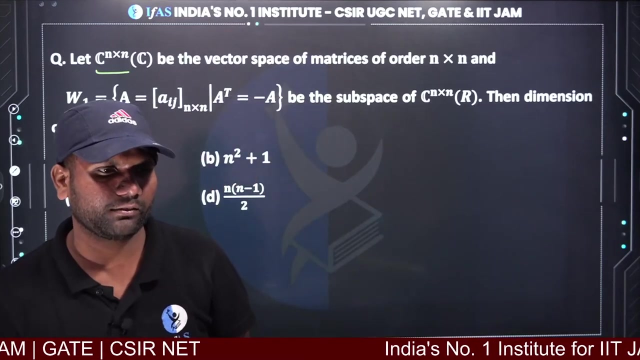 Hermitian matrix. see about its Hermitian Deepchandra. you did it very good. yes, absolutely, Sunil. yes, absolutely tell us. tell us about this. what will happen? what do you think about this question? if they also have some answers, then what will happen? Srikanth is saying c. 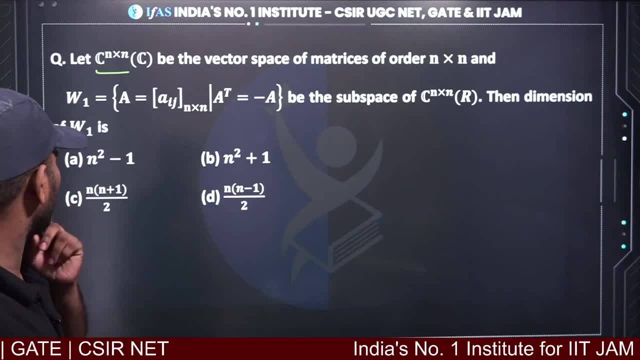 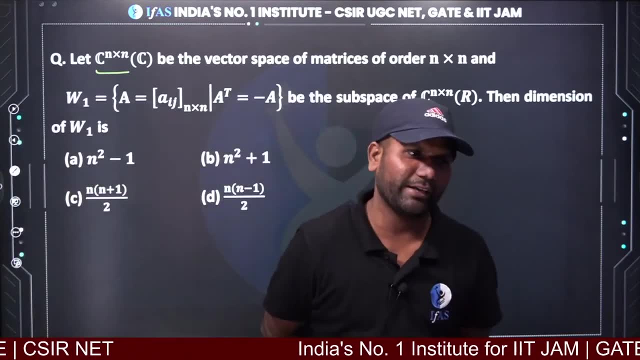 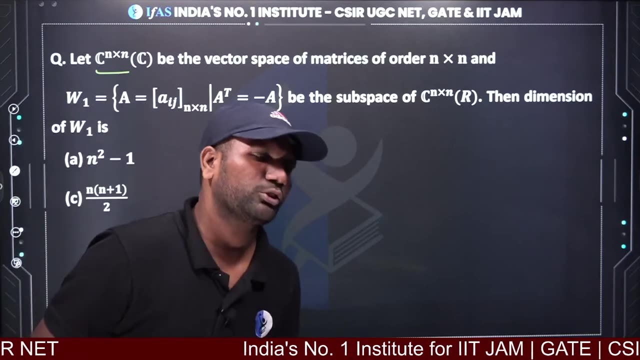 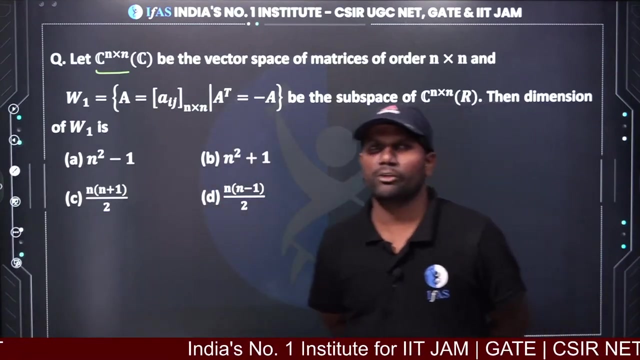 skew symmetric: yes, skew symmetric. then option d: yes, absolutely correct, absolutely correct, absolutely correct. Diksha Rajput is saying d ok, NKG classes ok. so read the question carefully, look at it carefully. ok, it is possible sometimes in the exam, as you will see the question. 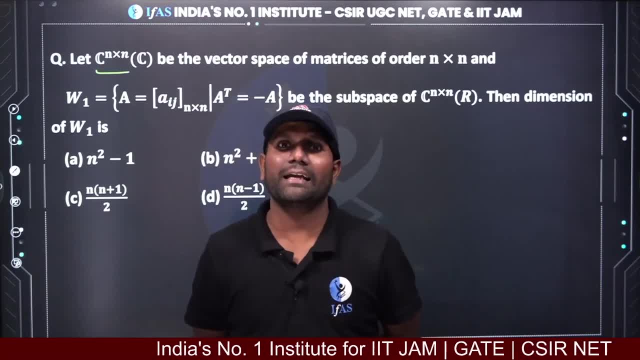 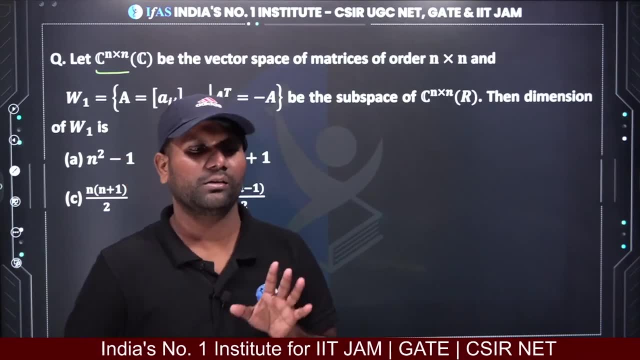 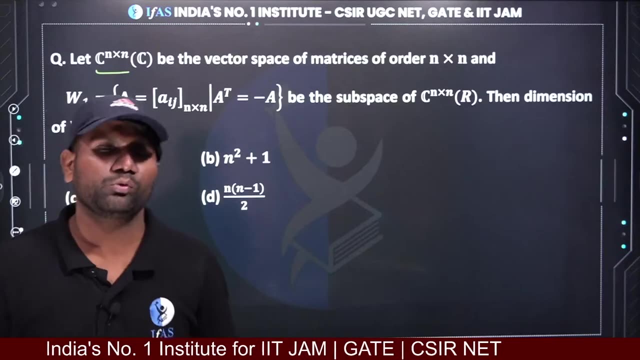 which of the following is, or are, correct or incorrect. there is a small in written. don't pay attention to it, then mistakes happen. so once you sit in the exam hall, read the question calmly and comfortably. read the question alright. prove or incorrect. see once what was asked in. 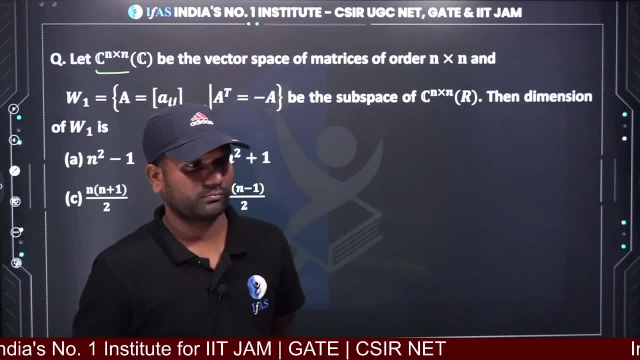 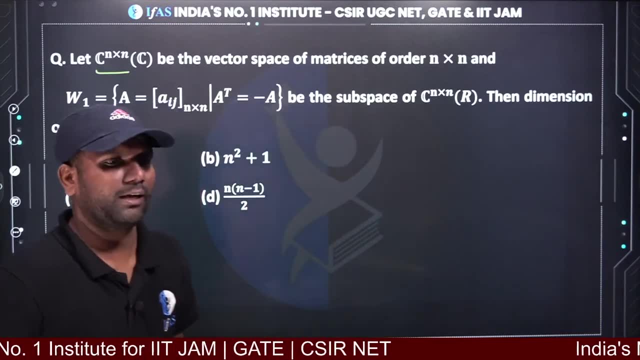 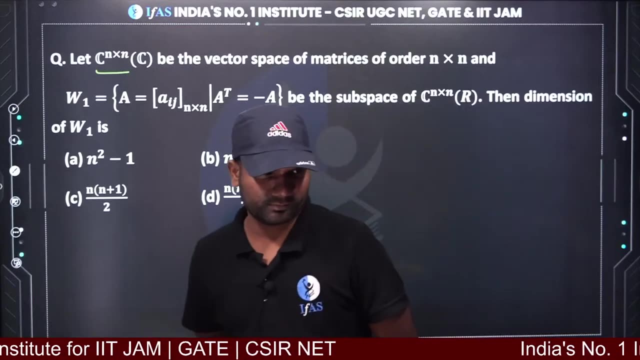 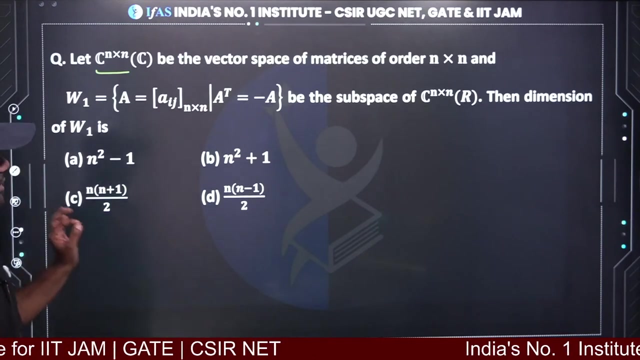 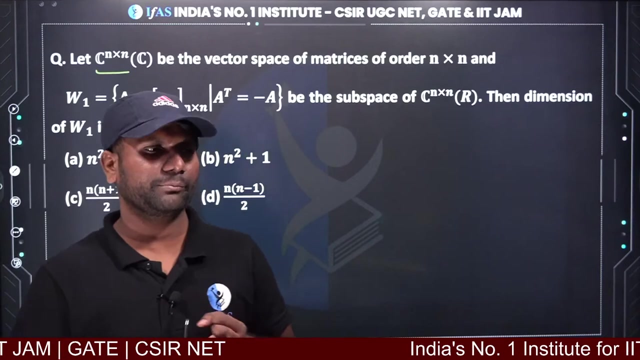 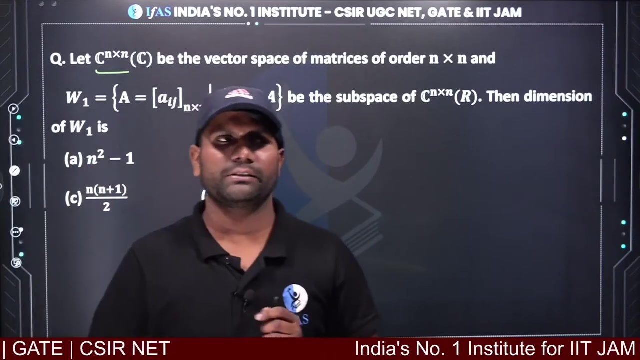 the proper question. yes, hurry up, absolutely, tell us you guys. D option: yes, absolutely right, look here. I have told you many more videos and tricks that what is the special thing about symmetric matrix, skew symmetric matrix Hermitian and skew Hermitian diagonal? yes, now here we have given skew symmetric matrix. so the special thing about skew symmetric is: 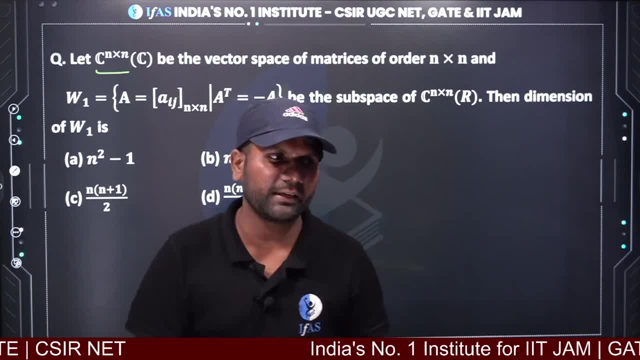 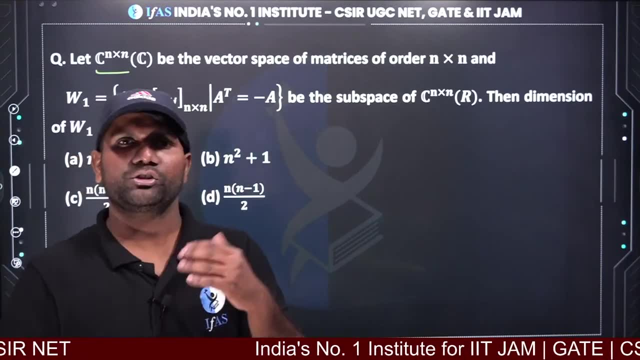 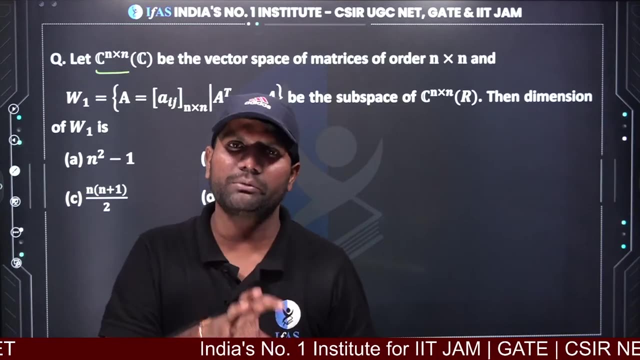 that its diagonal elements are always zero. the special thing is that diagonal elements of skew symmetric matrices are always zero. use this tip: see dimension of symmetric matrix over R. if you do, then you get dimension nn plus 1 by 2 of skew symmetric nn minus 1 by 2, Hermitian and. 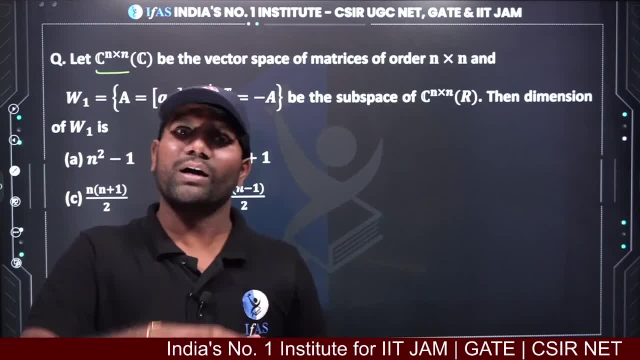 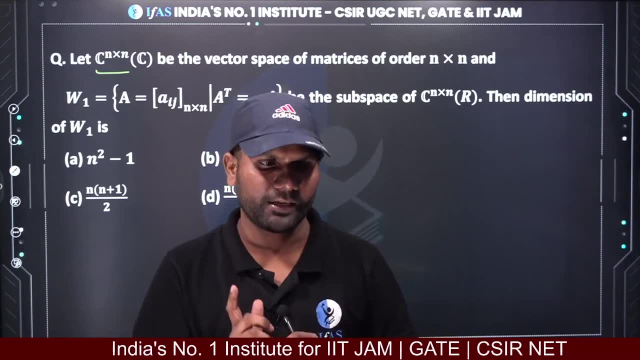 skew Hermitian matrix. if you are given those people form over R vector space, keep in mind, never do over C, because there the scalar multiplication fails, okay. so here, if you talk about symmetric, then what do you know? here, diagonal- sorry, Hermitian- is skew symmetric. 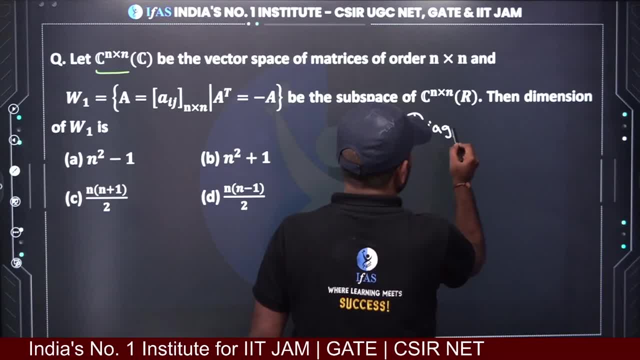 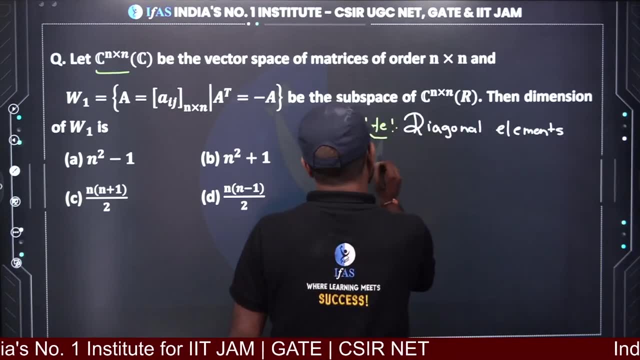 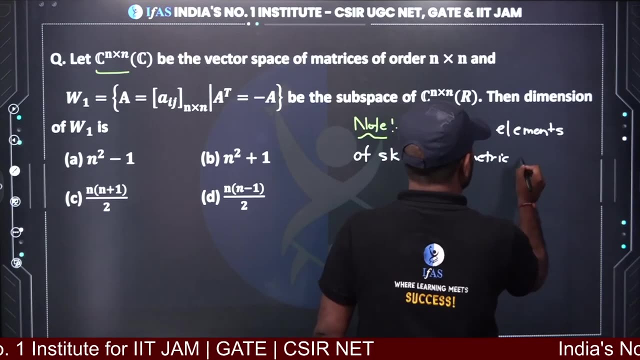 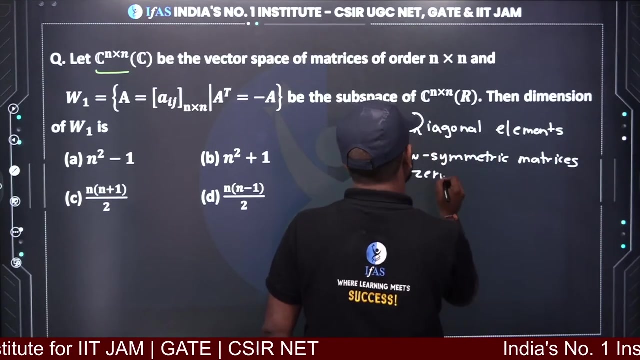 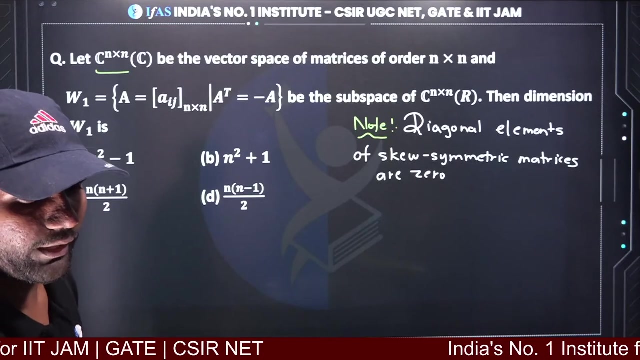 so diagonal element of skew symmetric matrices: diagonal diagonal elements of skew symmetric matrices. skew symmetric matrices: diagonal elements of skew symmetric matrices are zero. so skew symmetric matrix- diagonal elements are zero. okay, so any skew symmetric matrices over R. what did be said? yes, I said it is skew symmetric. all students listen carefully once. 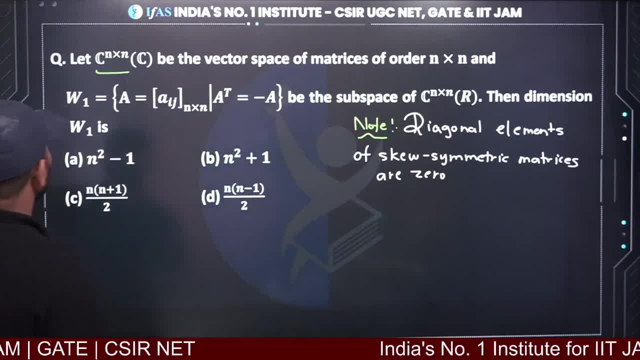 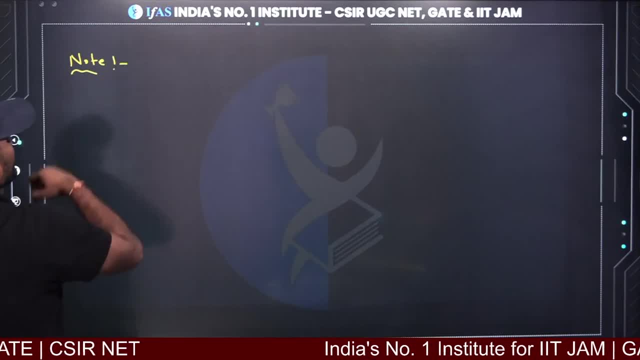 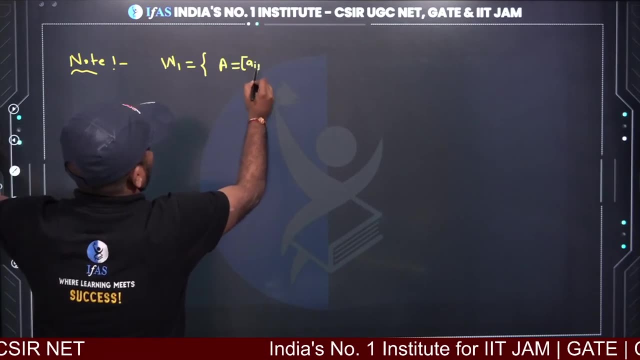 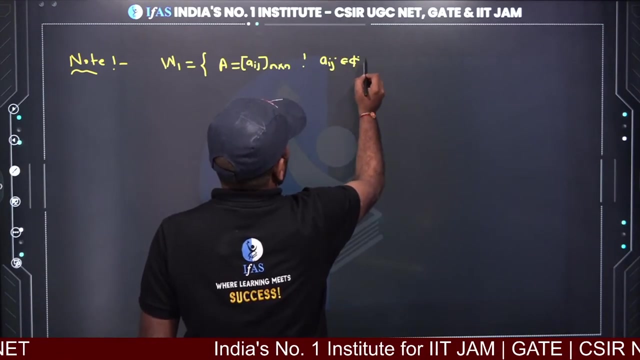 radish students. listen carefully if I tell you once here when I took it and said that, listen carefully, it is the matter of work here. do not make a mess. here I have taken a work such that a is equal to c and a is equal to a raised to theta. 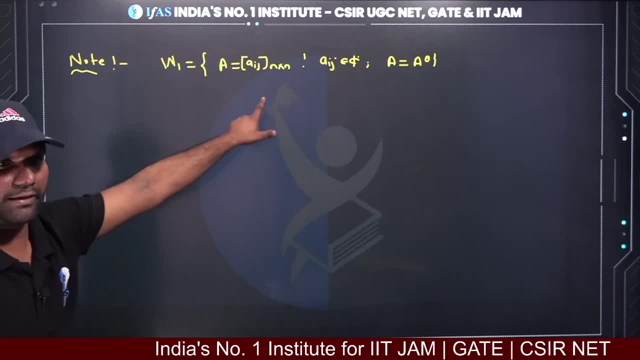 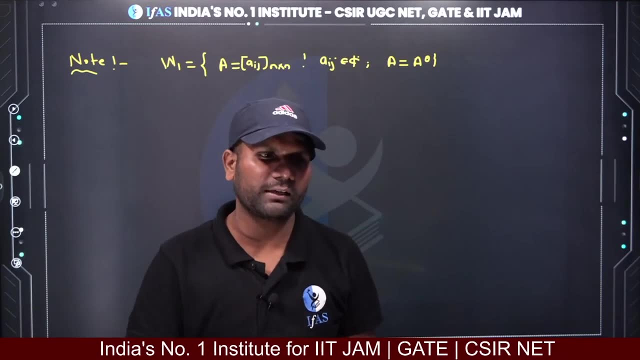 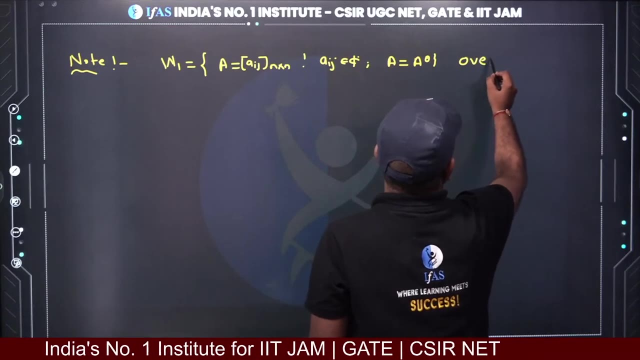 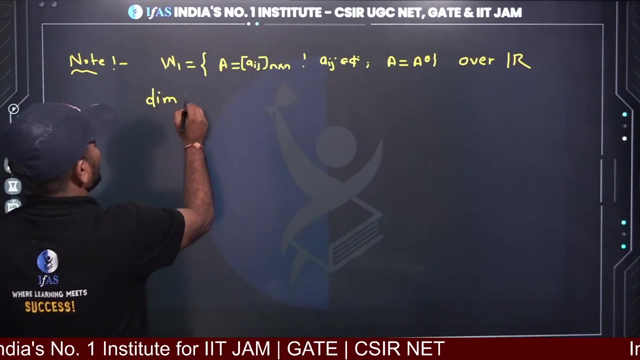 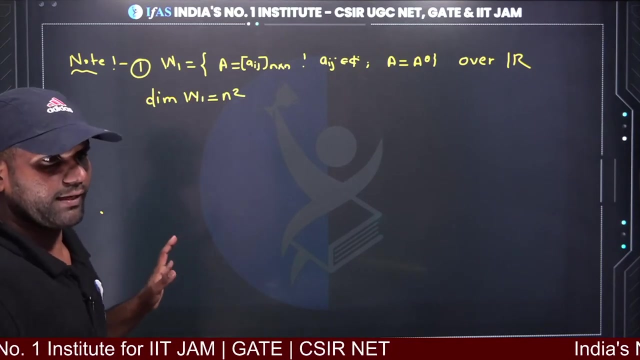 so this Hermitian matrix form a vector space or subspace. when your field is real number and not complex number, it always form over r vector space or subspace. dimension of w1 is n? square. this is the first result, one important thing to remember if you make mistake. 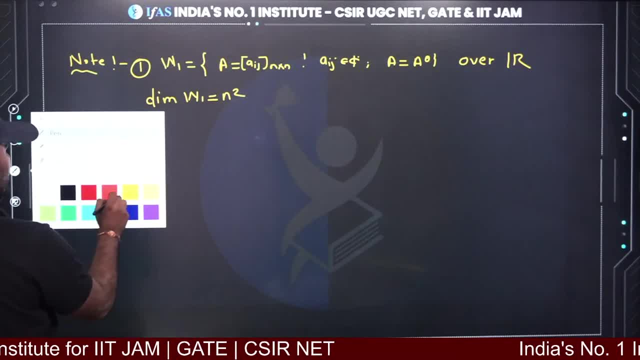 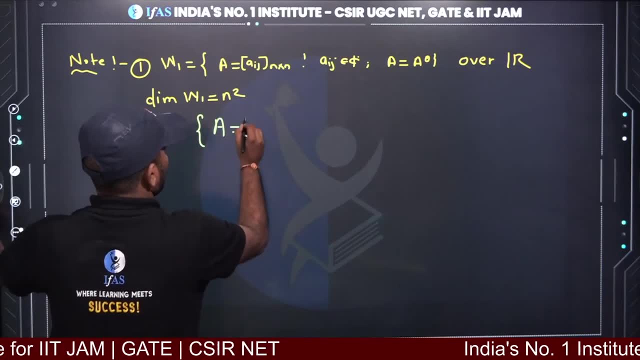 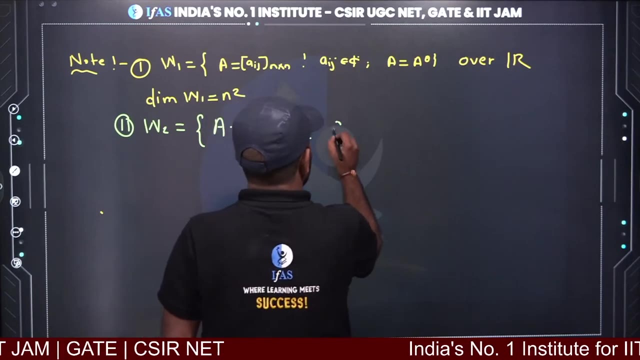 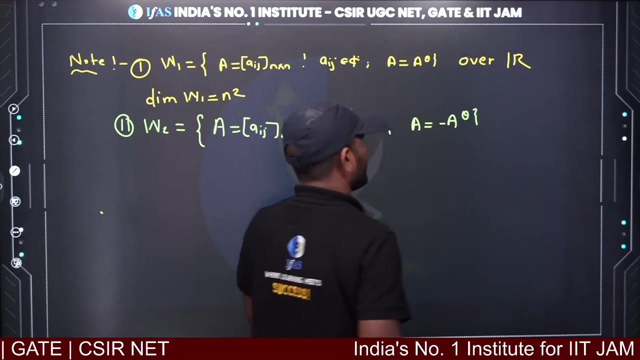 now see second. suppose we take w2. w2 is a set of all n cross n matrices where a ij belongs. a ij will be a complex number and a is equal to minus of a raised to theta. this set will form a vector space over r, not over c. 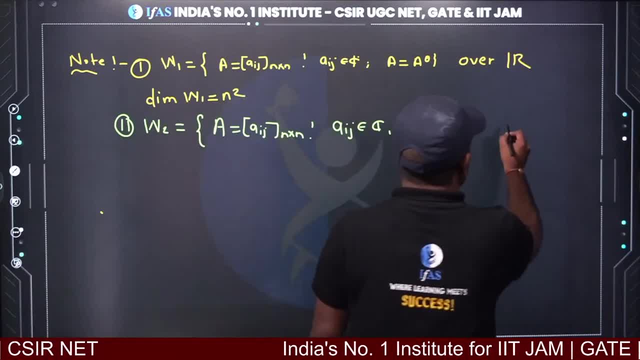 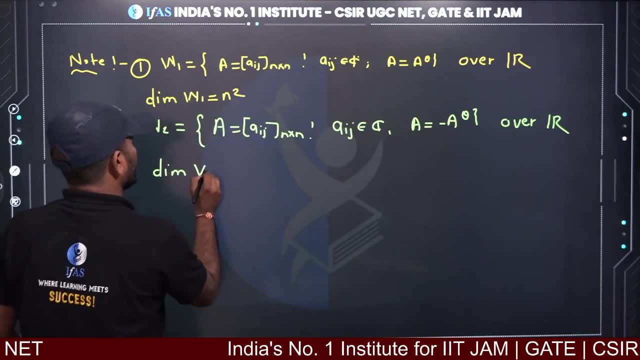 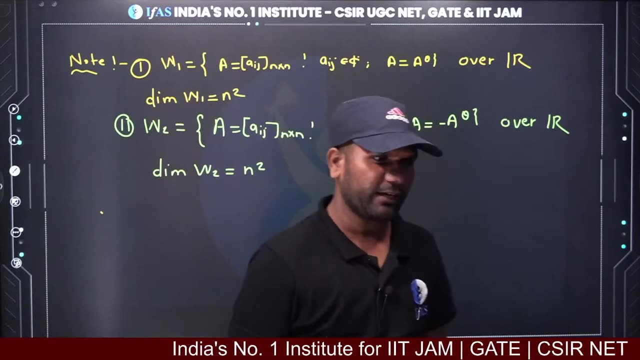 not over c, because scalar multiplication fails over r. so what is its dimension? its dimension is n square, so dimension of w2 is n square. so remember these two things before going to the exam. you should know. I hope you understood what I am trying to say, did you understand? 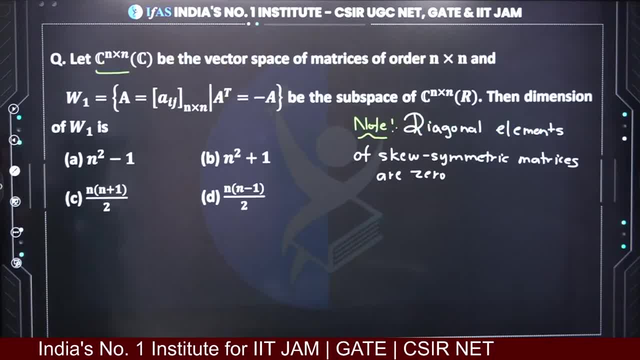 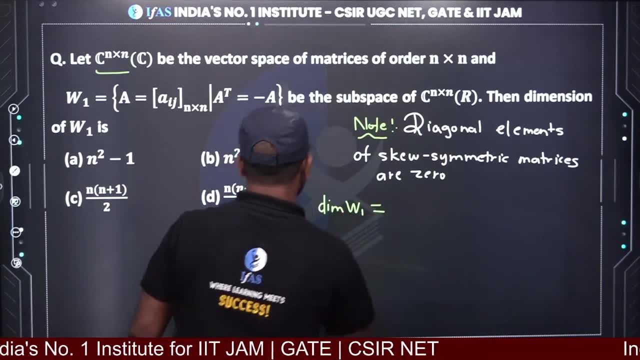 ok, now let's come to the last question. so here is a skew symmetric matrix, so what is its dimension? so, if you go to find dimension of skew symmetric matrix, so how is skew symmetric matrix? see, let's take a skew symmetric matrix 0, a12 and so on. 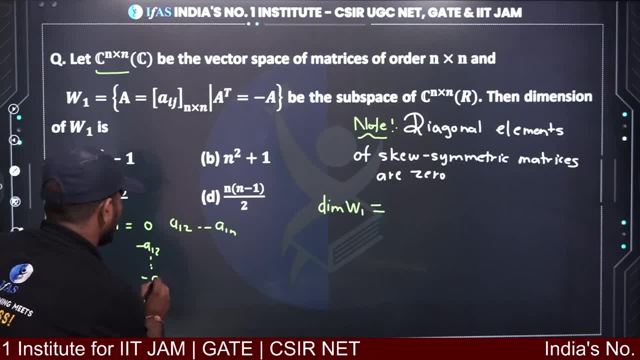 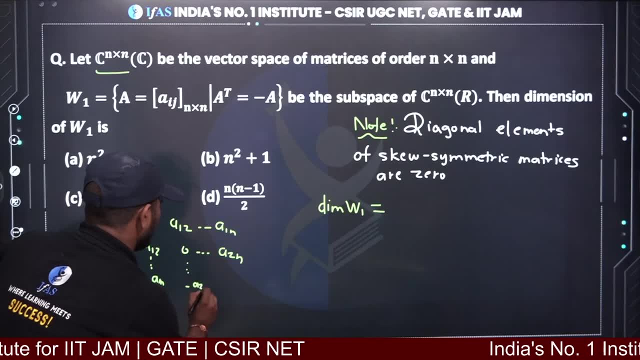 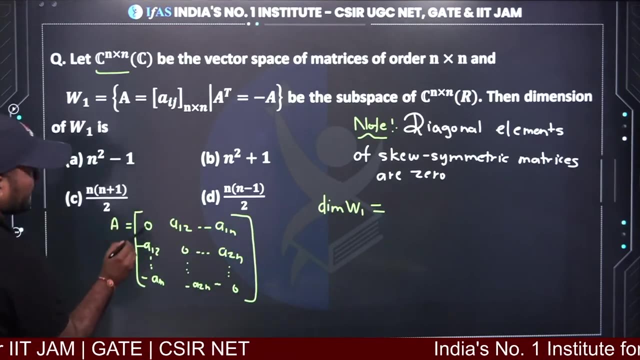 a1n here minus a12. and so on minus a1n. what will this be? 0, and so on a2n here minus a2n. similarly, at last you will get 0. see what is special about skew symmetric matrix? that what is its diagonal. 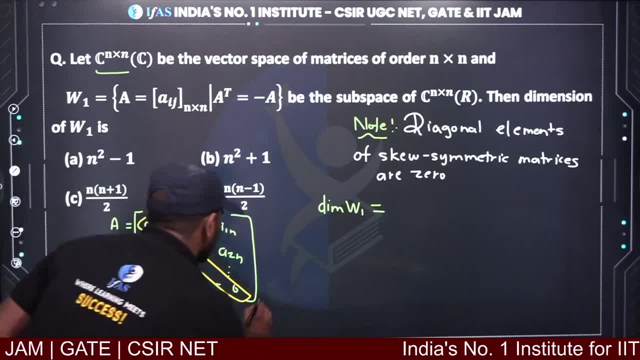 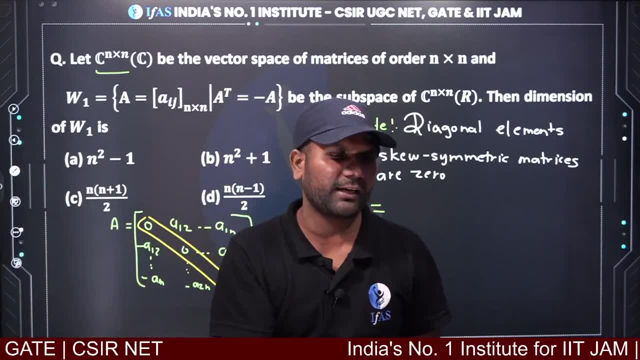 its diagonal is 0, ok, and if order is n, square n, cross n, if you have made first row, then in first column it will be made automatically, because if you are making first row, then you can make first column. if you have made first row, suppose you have generated this element. 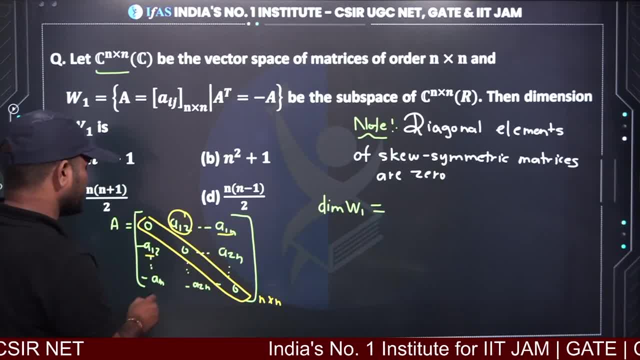 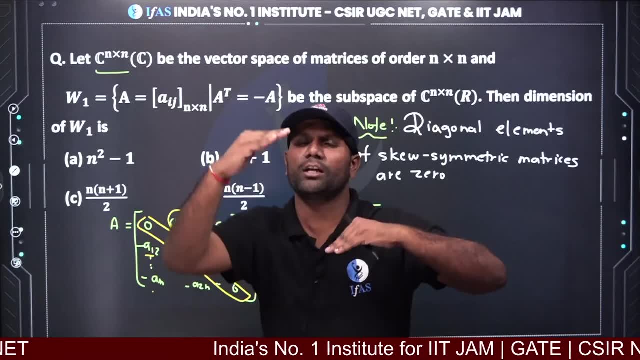 then you can multiply it with minus and make this. if you have made this, then you can multiply it with minus and make this. so from here we get to know: in skew symmetric matrix, if we have made elements above diagonal, then the ones below are made automatically, right? 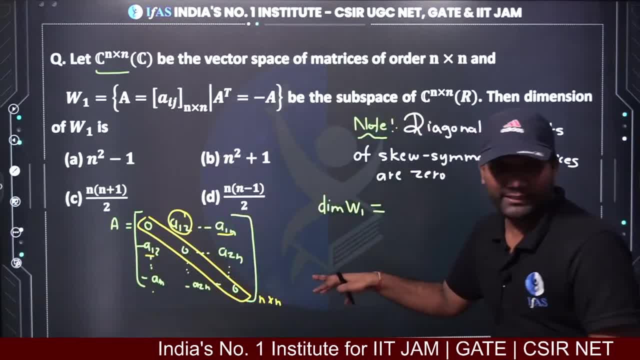 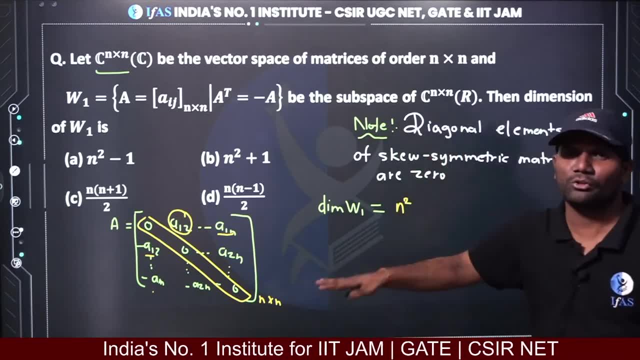 so from here you can say what is its dimension. how many elements are there in matrix total n cross n matrix total n square element. ok, but diagonal is 0. we don't have to make diagonal. so what I have done, I have taken out diagonal. but what we know, 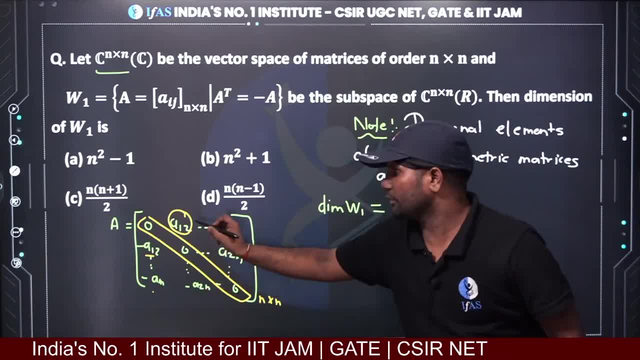 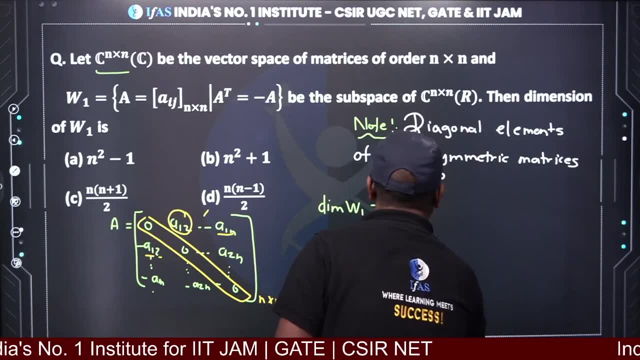 in terms of dimension, every element comes twice, because if A is made, then A is also made. if A is made, then A is also made. it comes twice. so what I have done divide by 2, so what we get: n n minus 1 by 2. 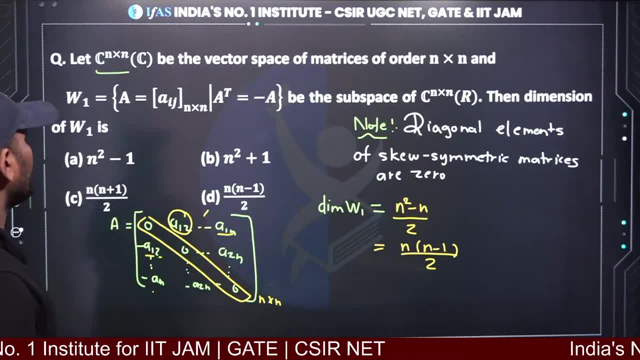 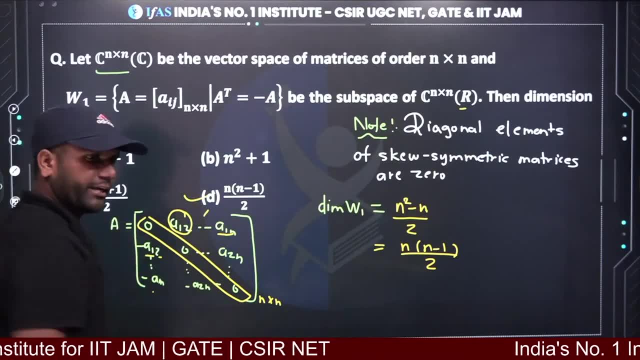 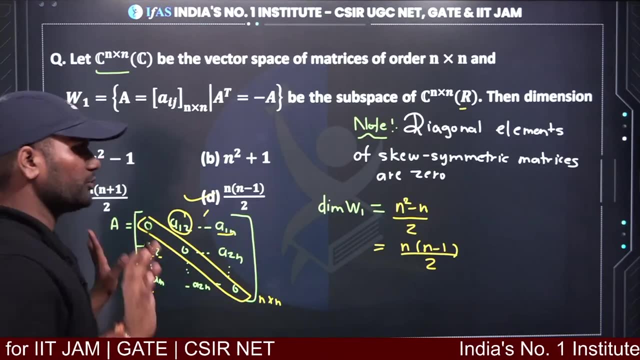 so what will be your correct answer? n? n minus 1 by 2. ok, well, we have been asked over R dimension, so one will be corrected here. ok, is it clear to everyone? see, all students. see once all things are clear. if anyone has doubts then you can ask. 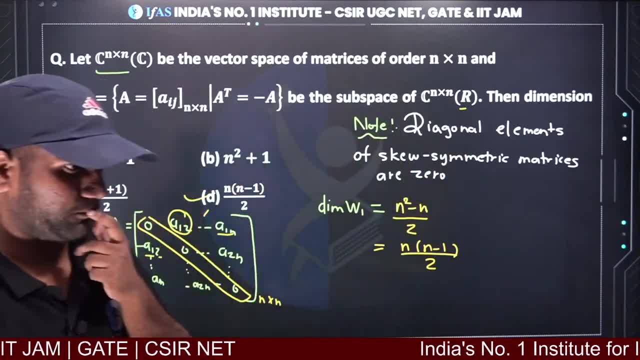 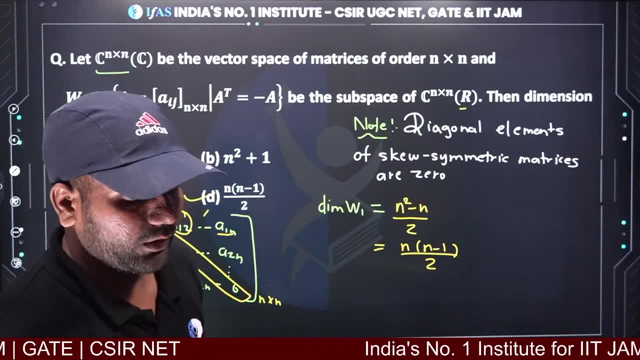 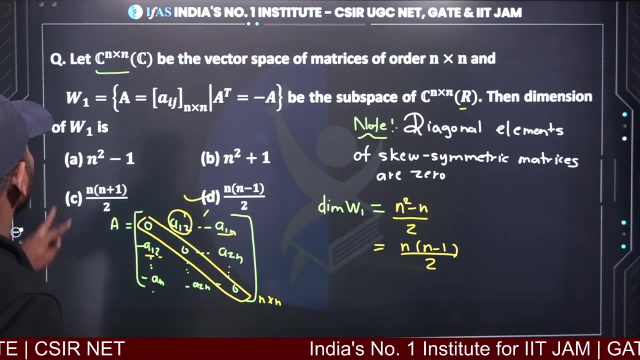 one minute. I will see. maybe if elements of matrix are complex, then something else will be there. we see, and since I have guessed that E is a fruit, then E is a square, I thought I have to do it again. wait, wait, let me check. matrix elements are complex. 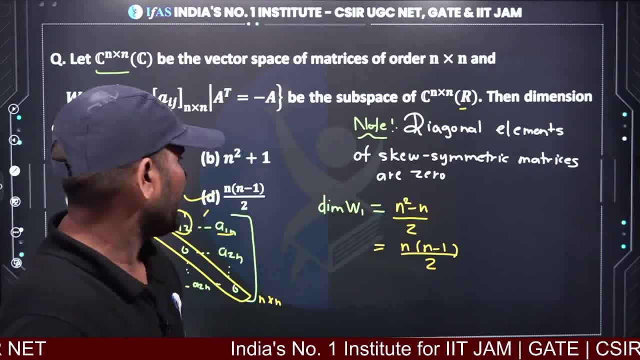 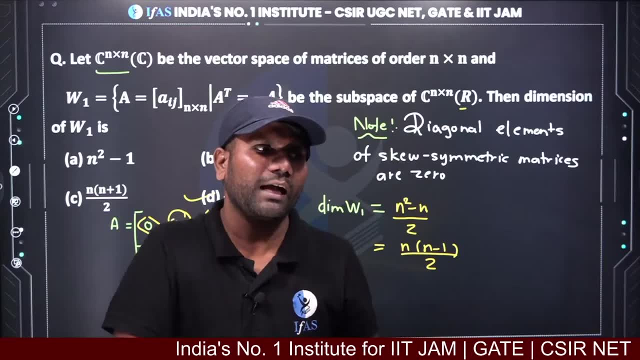 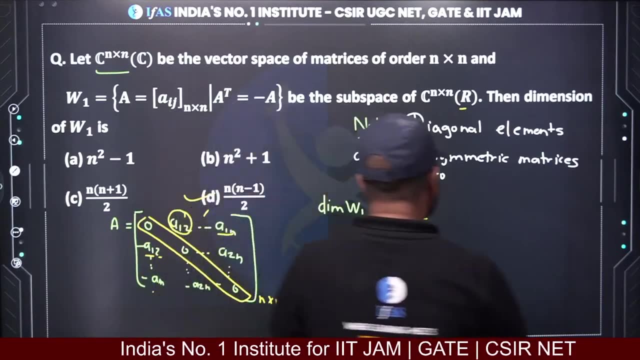 wait, wait, wait. matrix elements are complex. now we have done it as real. but what do we know? we know that to make any complex number over R, we need two elements, right or not? we need two elements. so what I will do? I will multiply it by 2. 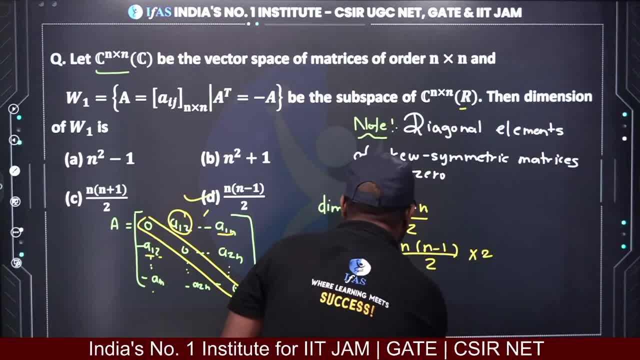 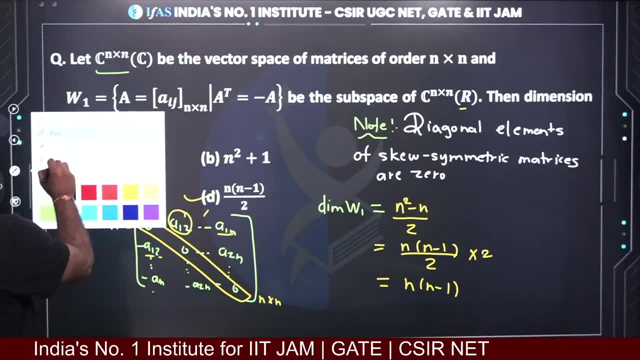 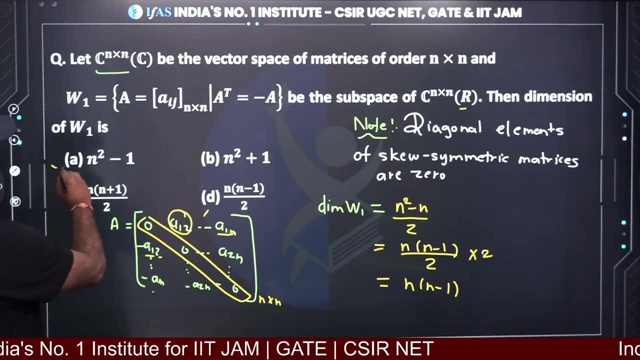 I am multiplying it by 2. if I multiply it by 2, then what will I get? N will be N-1, so in this case, see, if its entries were real number, then option D would have been correct. if entries are complex number, then option A would have been correct. 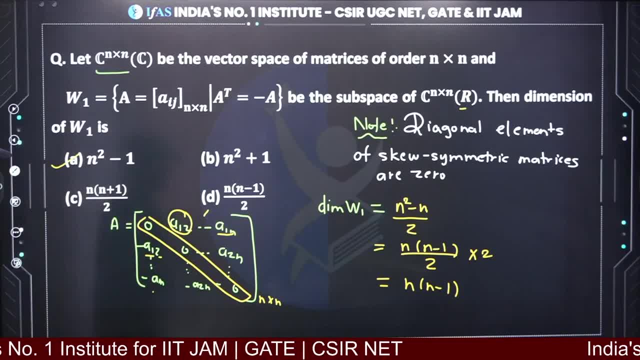 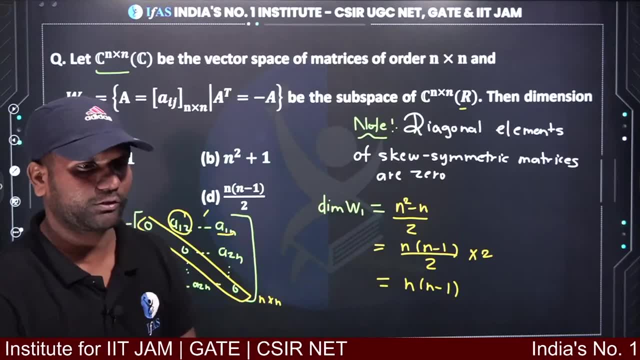 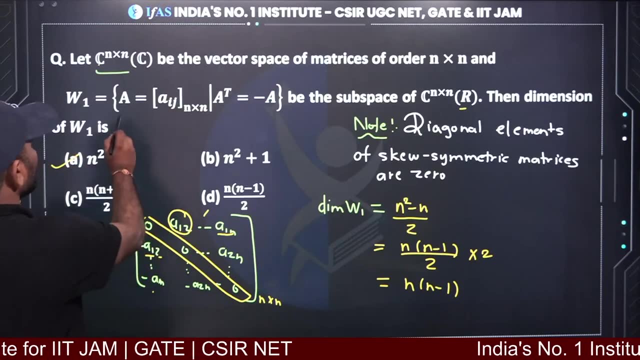 did everyone understand? did everyone understand? actually there was some confusion in the question. let me clear it once. listen carefully in the question we are given Cn cross C be a vector space of order N cross N. W1 is Wn N cross N matrix, which is Q symmetric matrix. 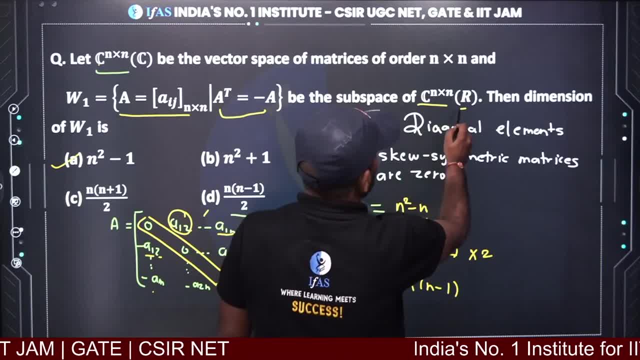 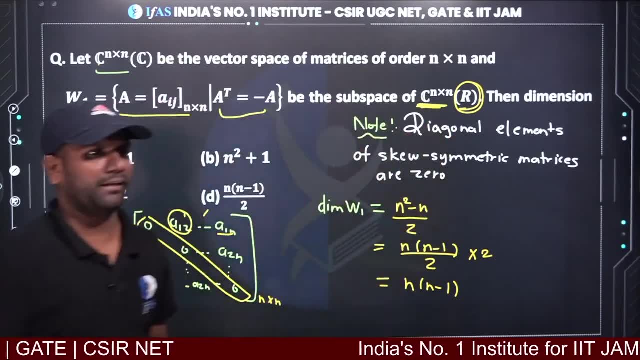 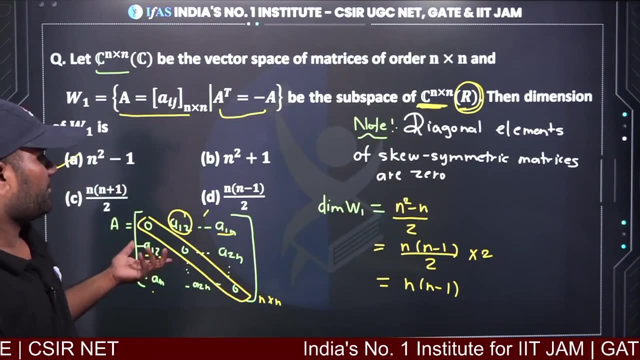 and we are given subspace of Cn, cross N over R. here we are given filled R, but entry of matrix is complex number. filled R is entry of matrix is complex number. so that's why now see, if I say C over R, how much is its dimension. 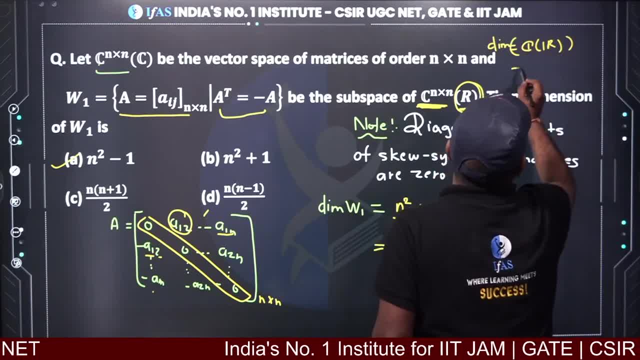 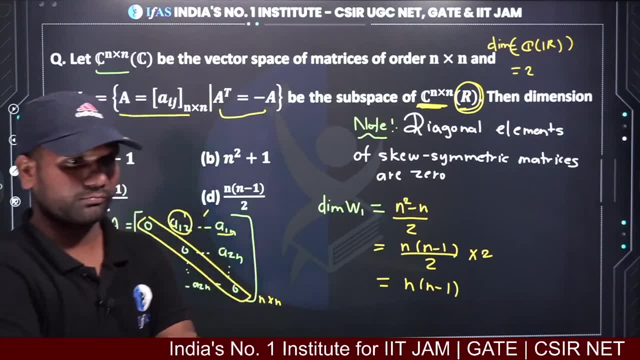 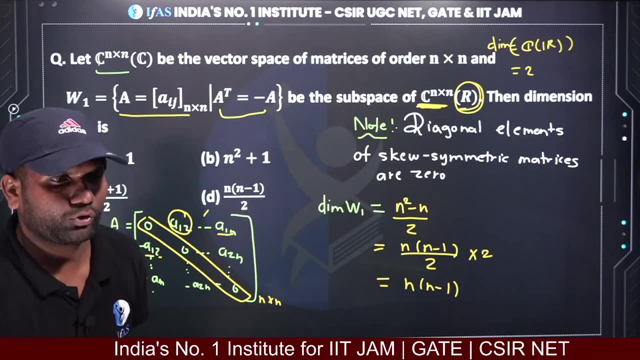 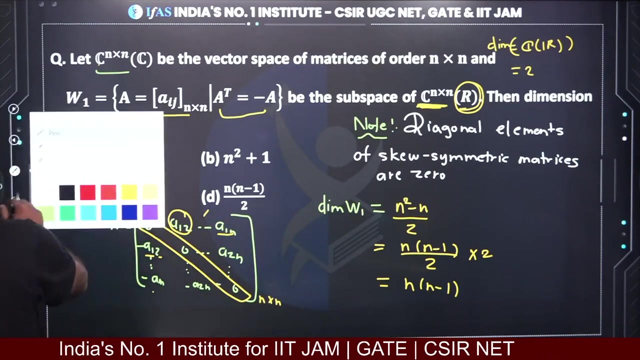 you guys tell me how much is its dimension? its dimension is 2. its dimension is 2, do you understand? let's see N square minus yes, N square minus N. so there is no option in this. so I think the equation is wrong. let me clear it once. 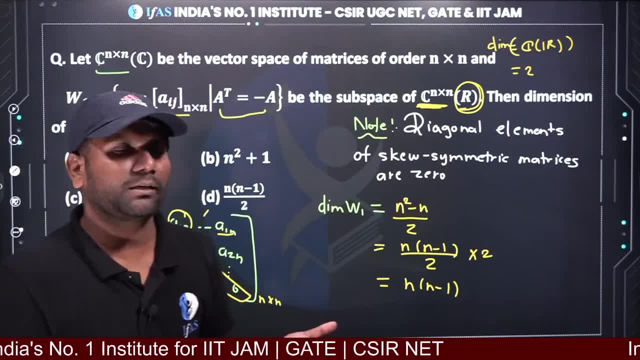 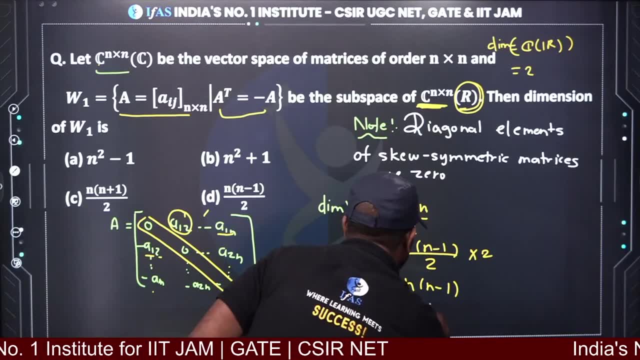 now, what is the entry of this matrix? entry of this matrix is complex number. our field is R, so in this case its dimension will be N, N minus 1, which will be N square minus N. so there is no such option. so let's correct the option. 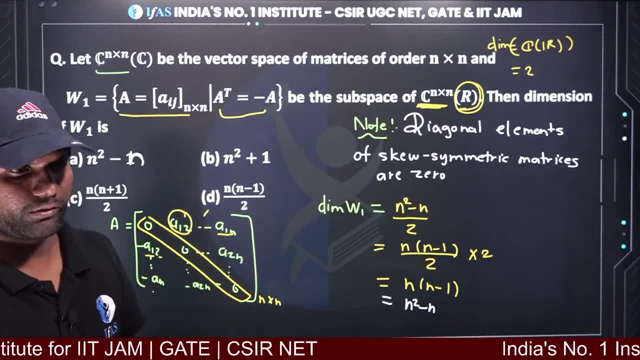 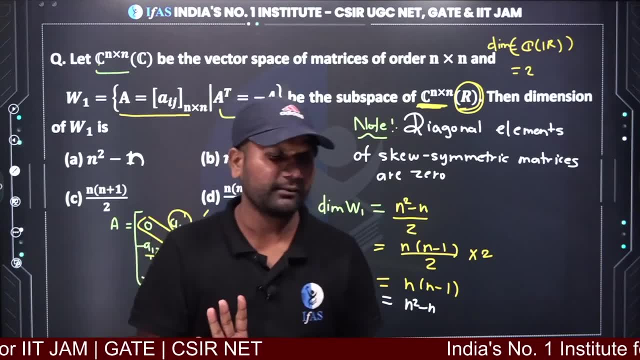 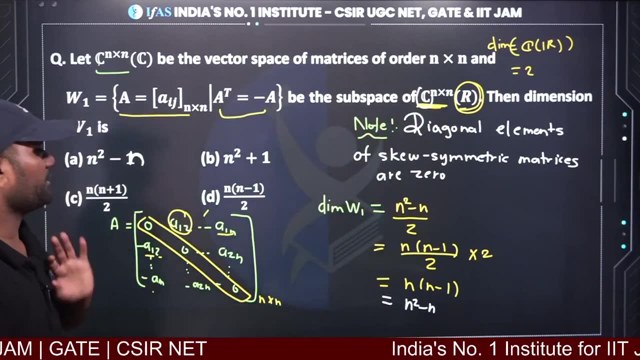 do N square minus N, then your option will be correct. yes, none of this is correct. I think the typing person has made a mistake, no problem. but you guys are clear, right? so let's say, if the entry of this matrix, if it was a real number, then your option would have been correct. 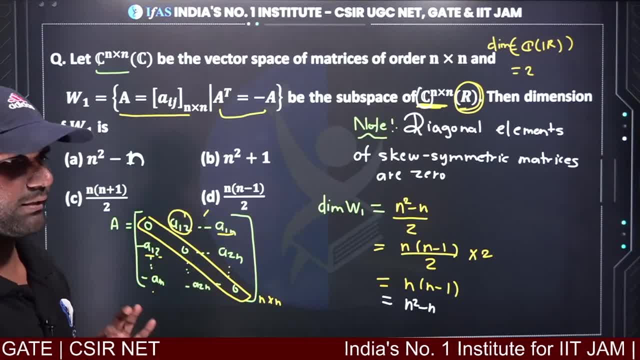 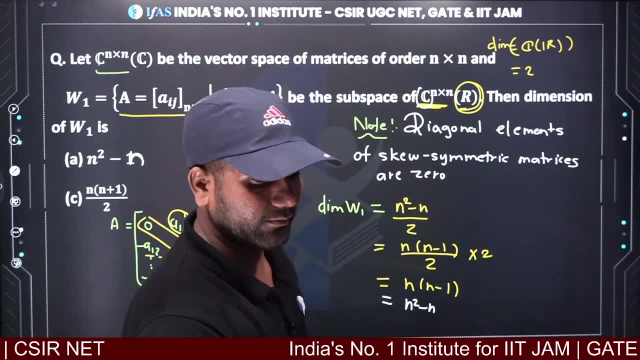 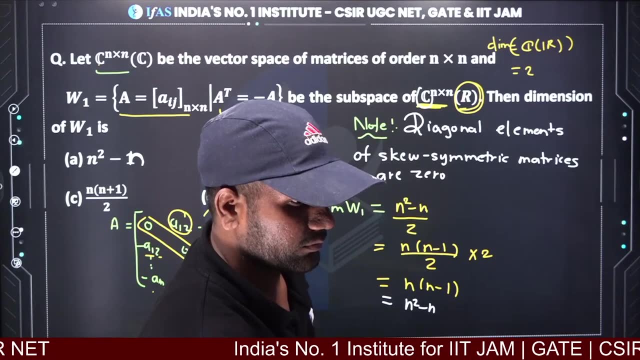 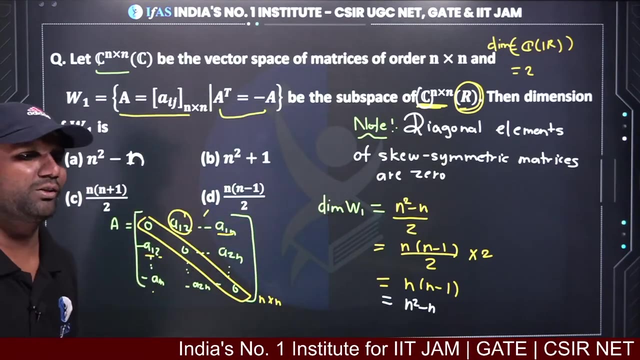 it is a complex number. that's why it happened. all the students: clear: move ahead, move ahead, move ahead. no, no, why are you getting serious? it happens actually. there must have been some typing mistake. no problem, move ahead, move ahead. let's move ahead to the next question. 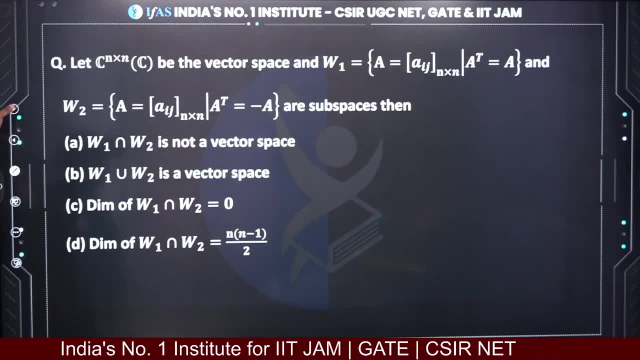 let's move ahead to the next question. this one is very easy. you guys can tell this one: I keep homework for you. this one: I keep homework for you. this one: I keep homework for you. this one is homework for you. you have to try this. please comment and tell me. 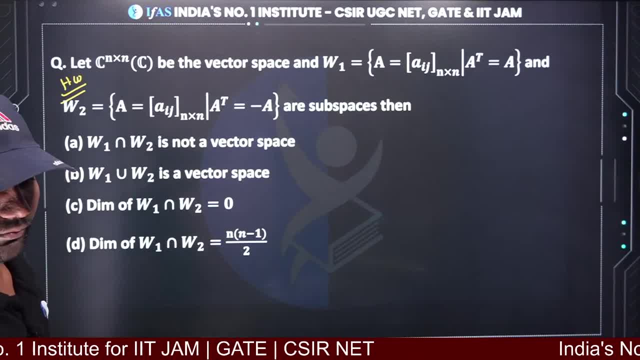 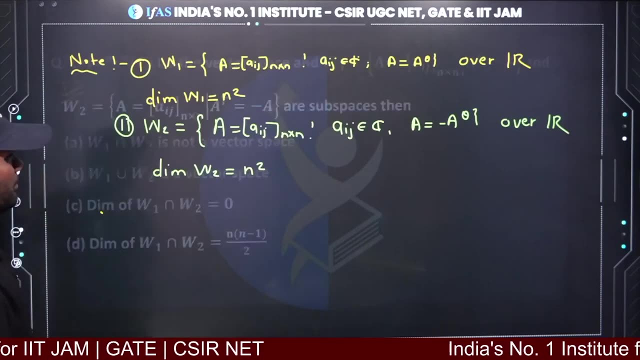 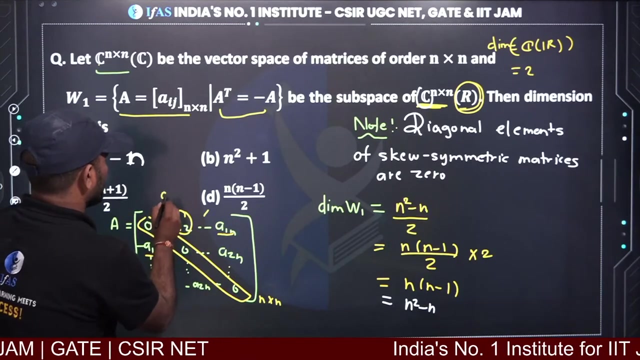 after doing this, please comment and tell me no alpha. please comment and tell me no alpha. N square minus 1 won't be there. N square minus N will come multiplied by 2. because, for this, because this matrix A 1: 2 like B 1: 2. 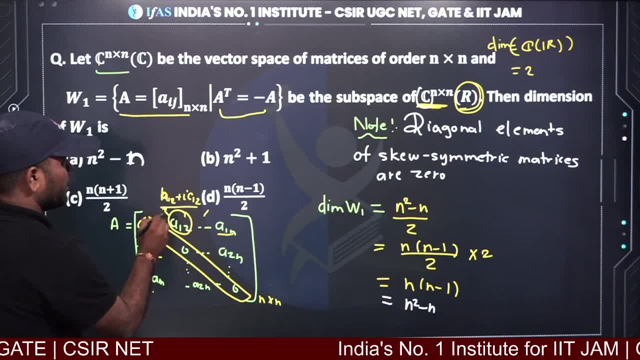 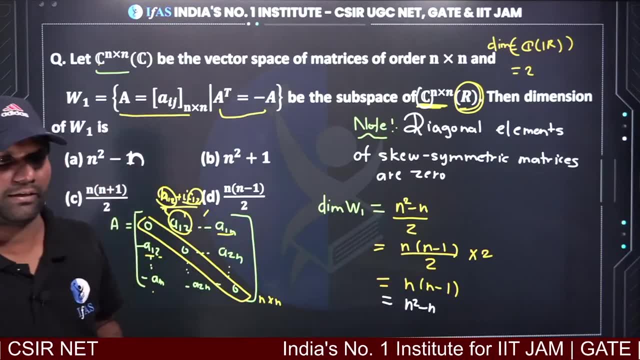 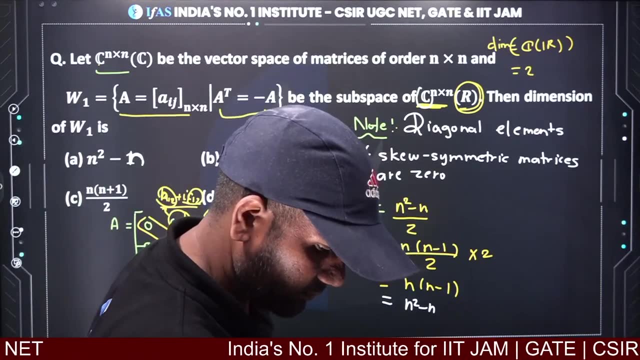 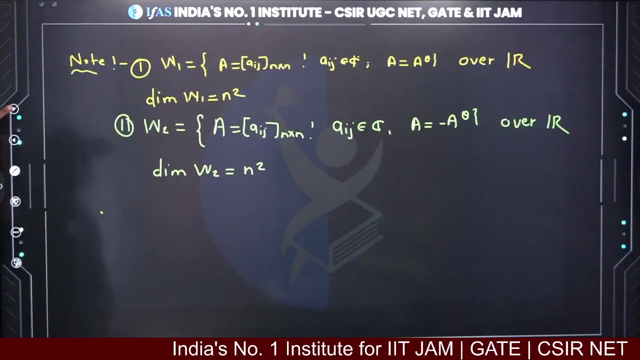 is in this form. it is a complex number to make over R. to generate every element over R, we will need two elements. that is why I had also multiplied after 2,. okay, let's move ahead. this is homework for you. you have to solve it. 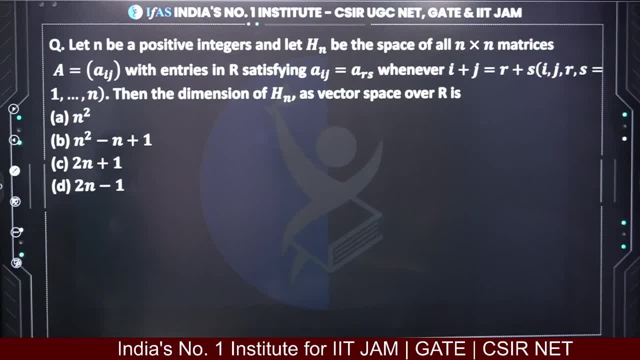 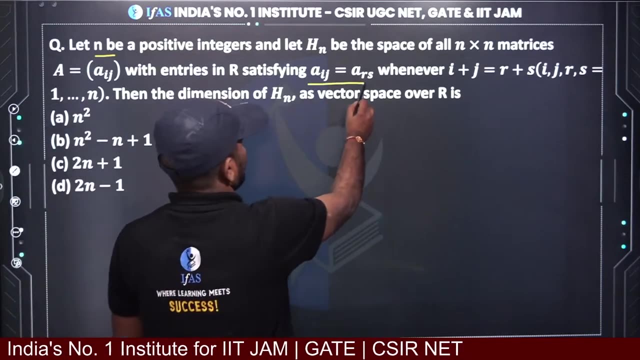 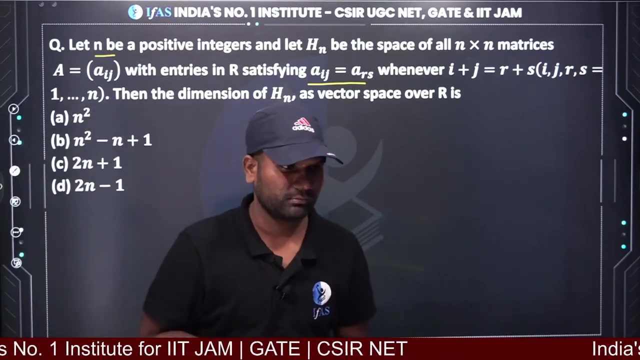 you can say something about this. look at this question. let n be a positive integer, hn be a space of all n cross n matrices with entries in R satisfying this condition. this condition is satisfied only when i plus j is same as R plus s. then dimension of hn as a vector space over R, what will happen? 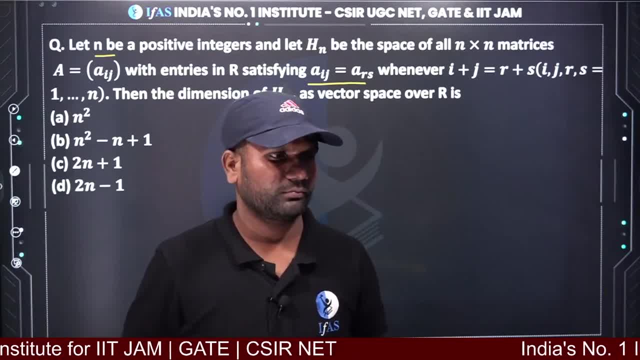 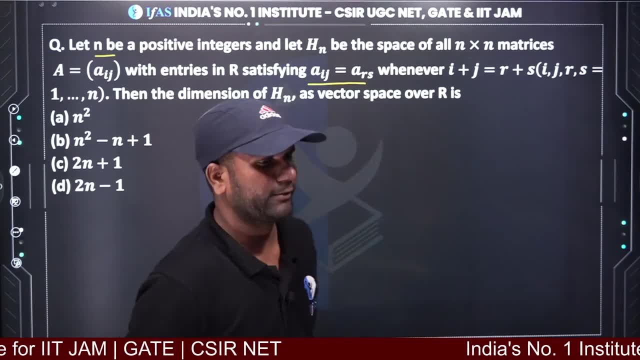 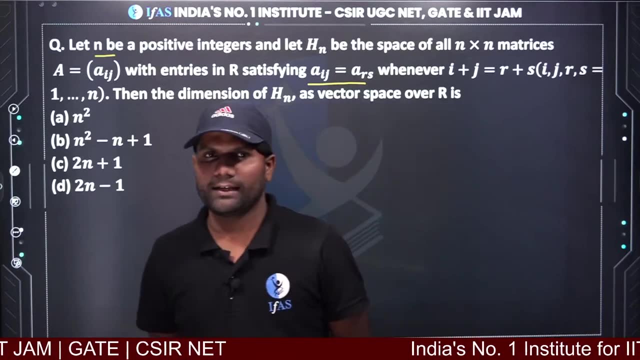 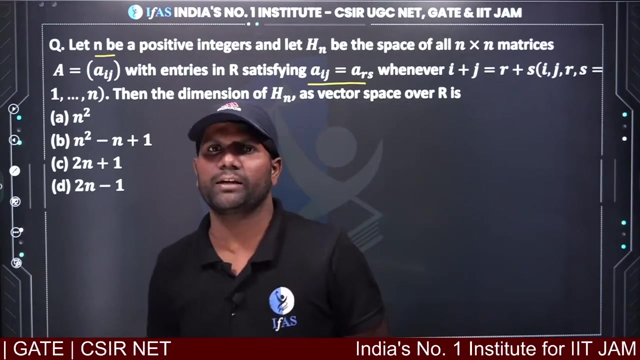 tell me what will happen. so come on the new people who are joining. if you have not liked it yet, then like the session. if you are new to the channel, then subscribe and turn on the notification bell. today's session is going on. tomorrow also, I will bring a session for you at 7 pm where we will study diagonalization, jc form, quadratic form and ips. okay, 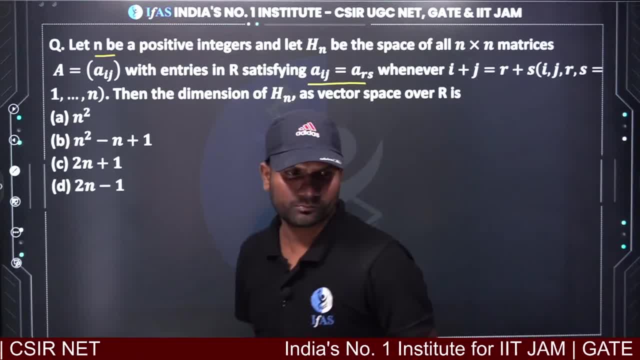 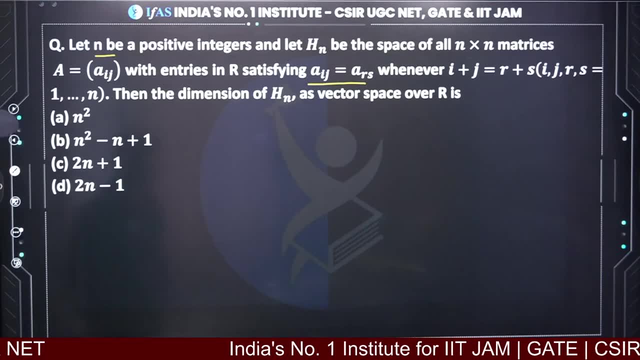 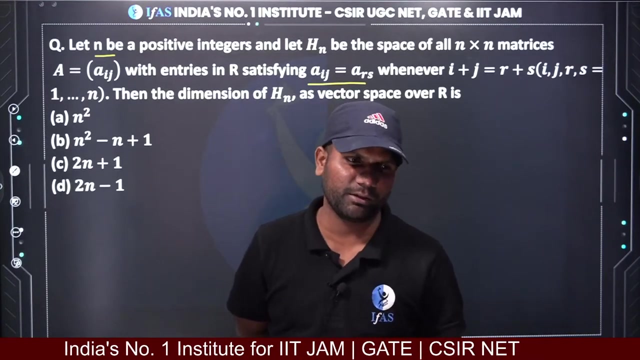 its d will be 2n minus 1,. other people tell the other people too. Ajay is saying this way. d will be okay. semi, almost everyone is saying d, so you must have done this with a particular example. 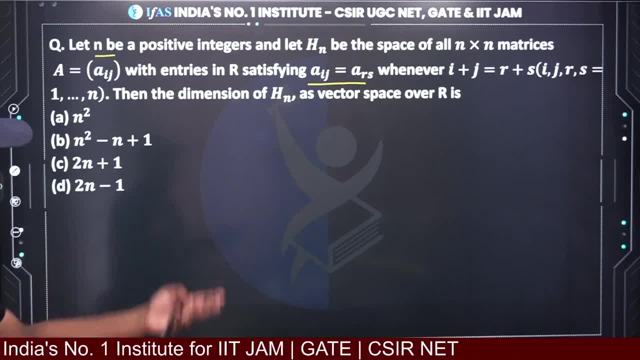 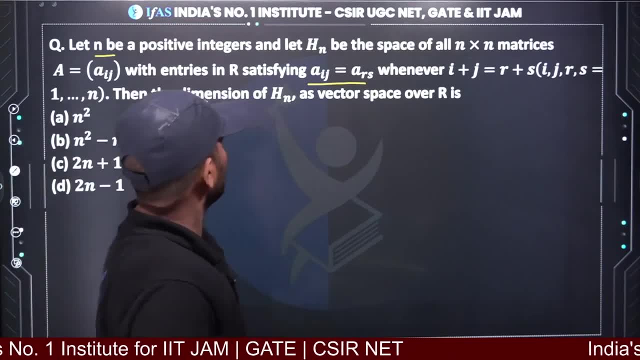 I think you did 4 cross 4, 5 cross 5, according to which you told: okay, do this, first, take some particular one, take 4, 5, 3, 2,, nothing in n, so you can try it on 4- 5,. 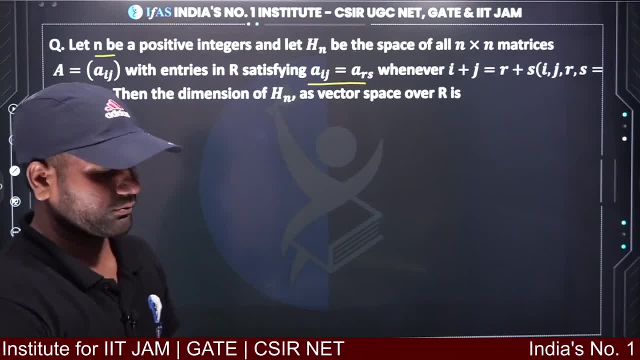 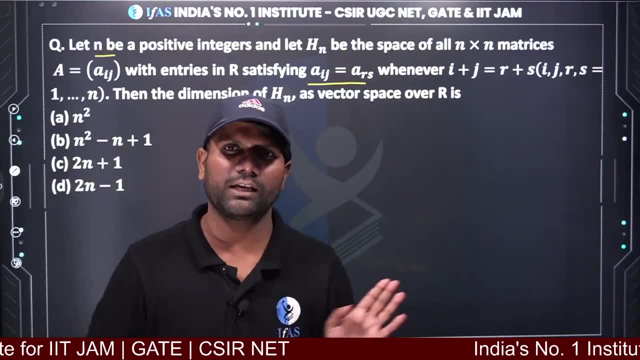 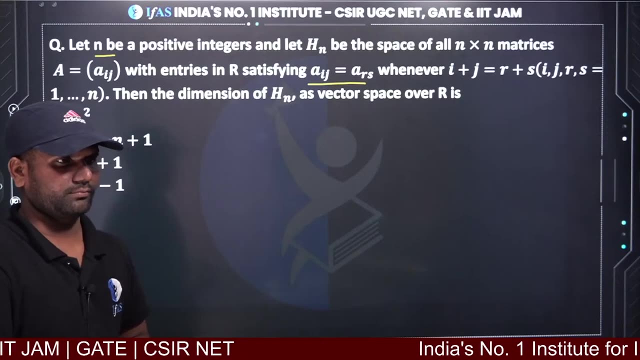 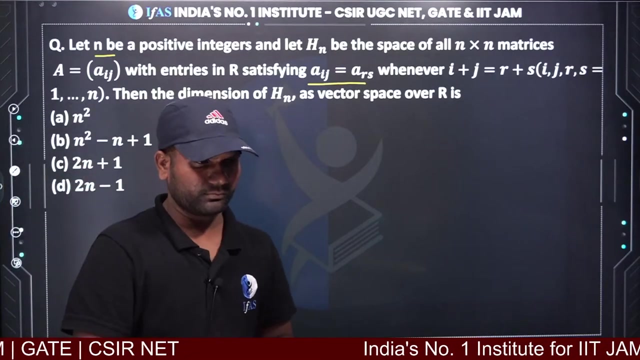 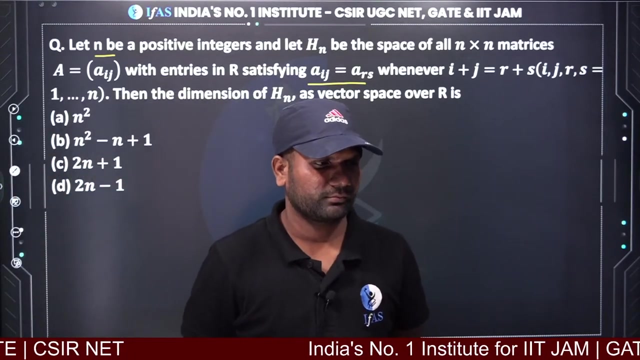 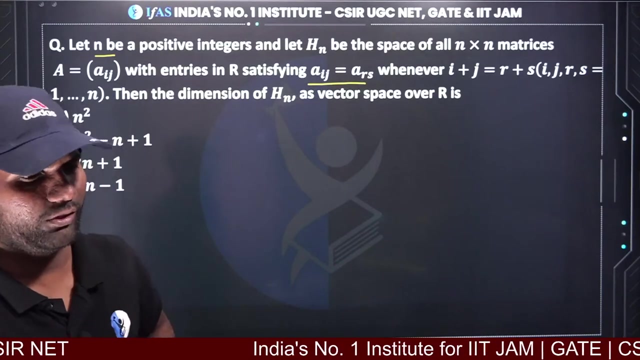 okay, you can try this. which order did you do it, ac? in fact, I had a question from the internet. I liked this question. that is why I brought it here. 2 x 2 is equal to 3 x 3. If you take 3x3,, the rest of the options will be discarded. This is the simplest way. 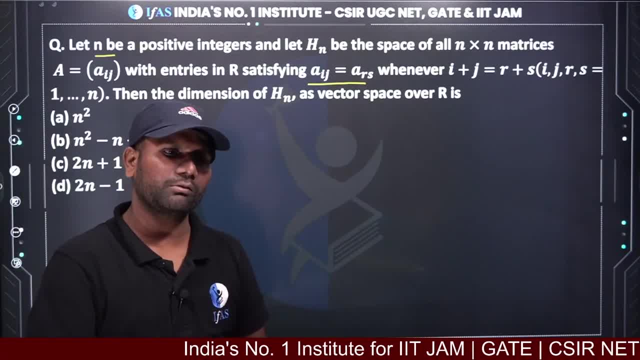 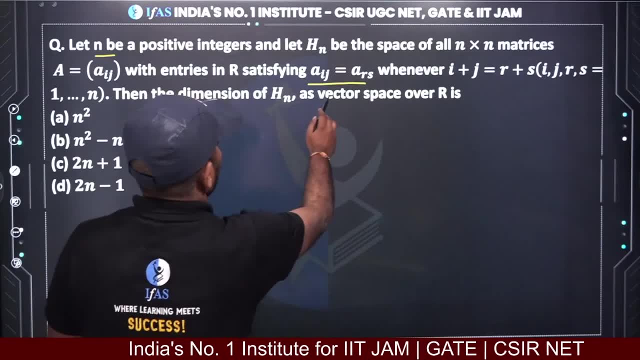 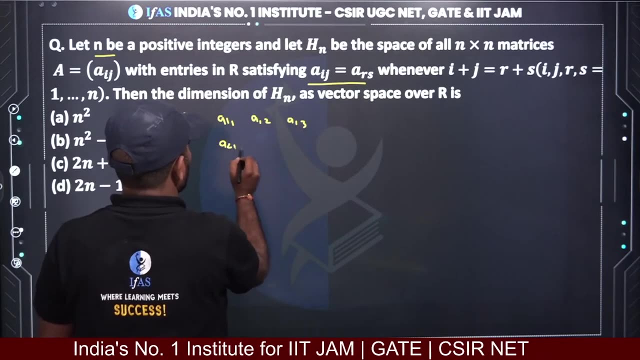 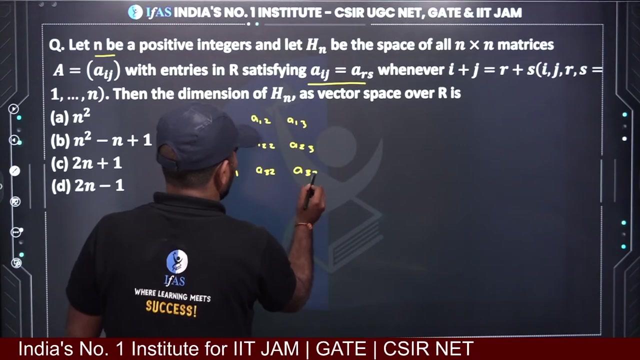 If you want to do it on nxn, it will take a little more time, but you will get it there too. Let's go to 3x3.. Let's take a matrix of A11, A12, A13, A21, A22, A23,, A31, A32, A33. 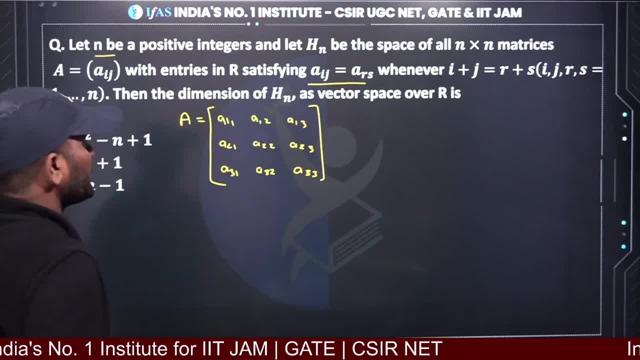 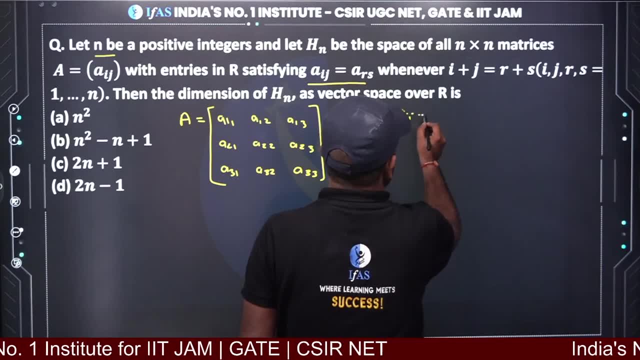 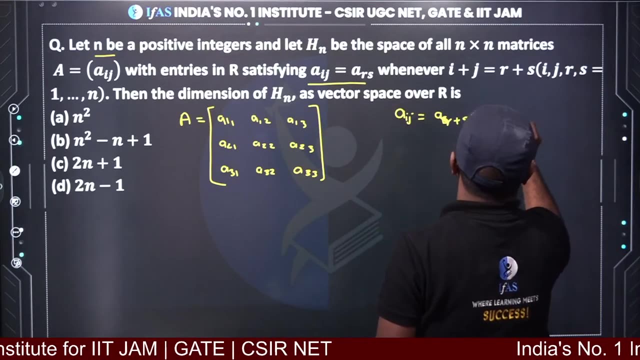 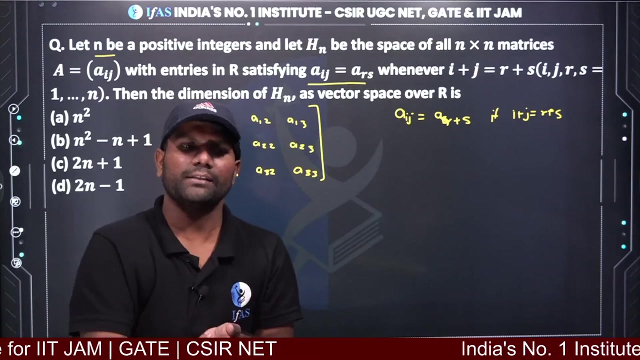 This matrix is given. If you see here, aij is same as ars, but it will be possible when aij is equal to ar r plus s. When is this If i plus j is equal to r plus s? So where the suffixes below are the same, their entries are being said to be the same. 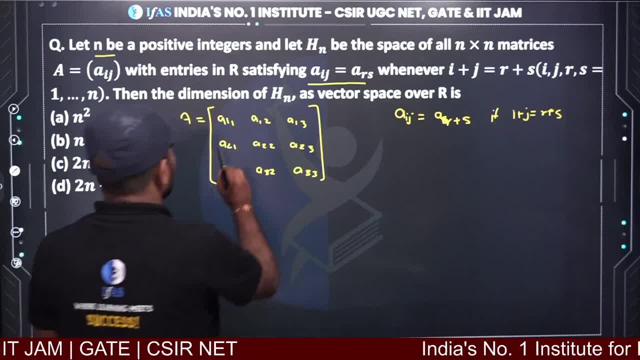 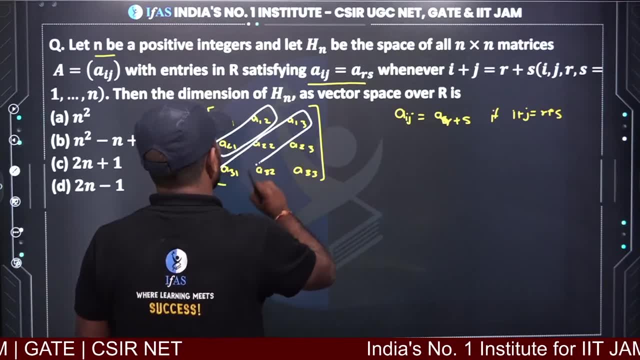 Let's see, They are saying that they will be equal. So see, one thing: if you add this, what will you get? if you add them, You will get 3.. If you add them, you will get 4.. And if you add them, what do you get? 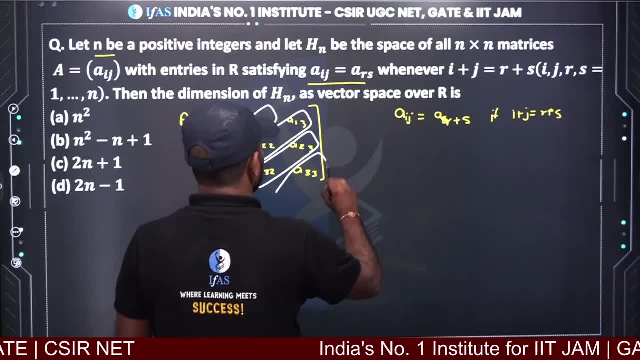 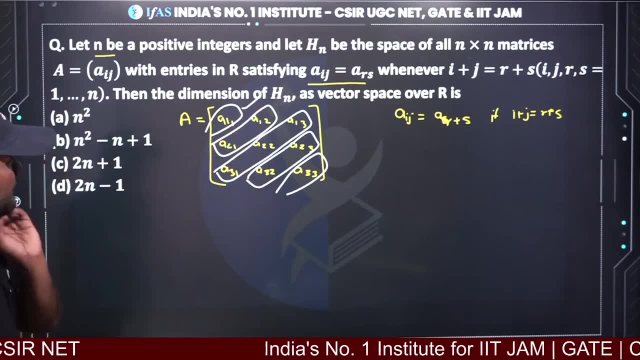 You get 5.. If you add them, they are 6.. And what are they? They are 1 and 1.. So see here, To generate this one element. Now, all these are becoming equal, So to generate this one element. 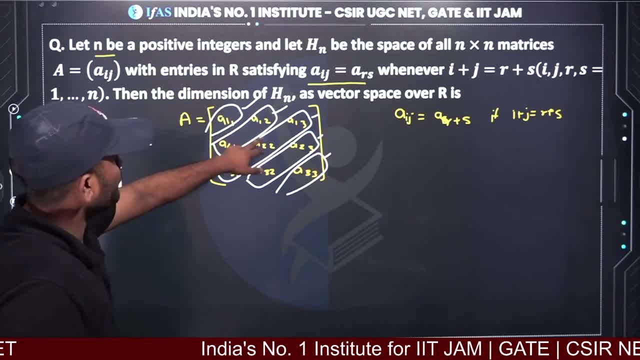 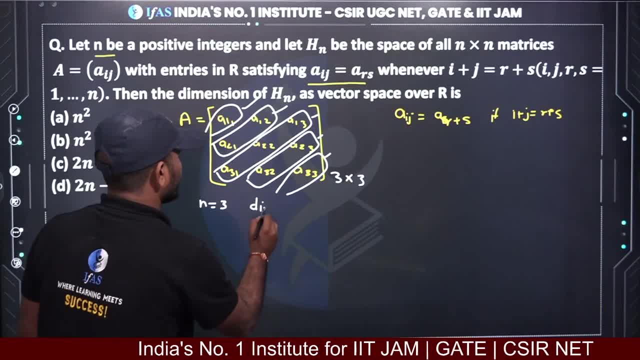 What is the value of n? It is 3.. So what is the dimension? you got The dimension. you got, whatever state you gave, w or hn, the dimension of x3, you are getting 5.. 1,, 2,, 3,, 4, 5.. 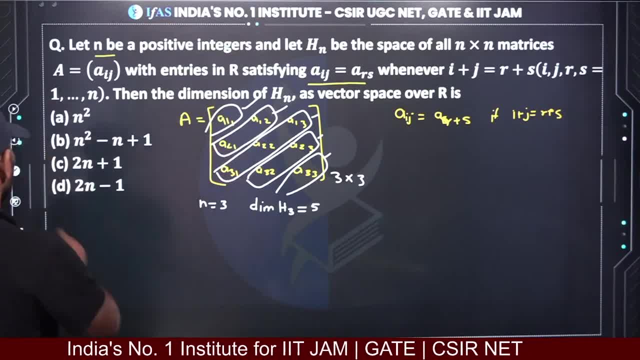 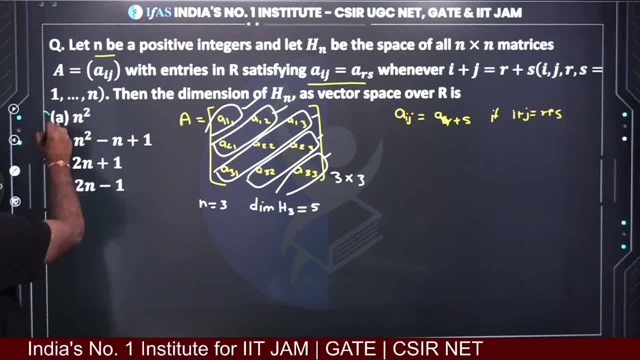 If you keep the value of n at 3, then what will happen? 9 will end. If you keep the value of n at 3, then 9 minus 3 will not be 6, plus 1, 7a will not happen either. 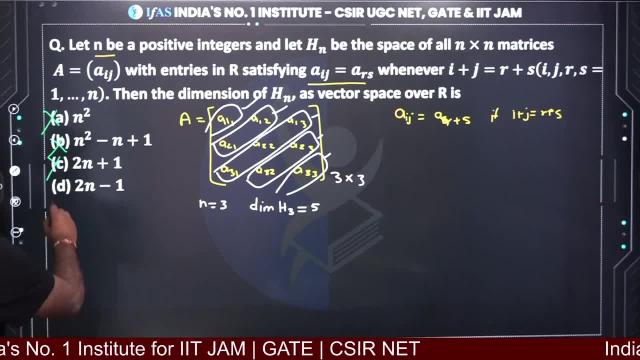 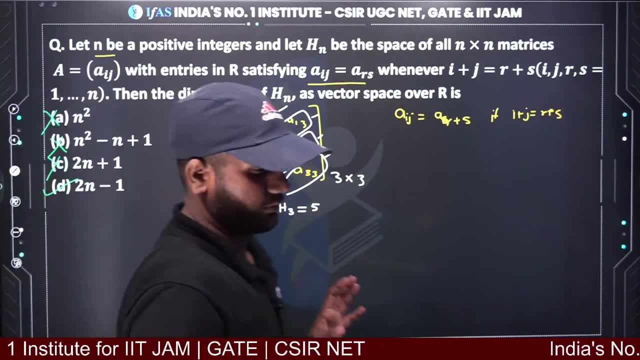 If you keep the value of n at 3,, then 6 plus 1, 7a will not happen either. So 5 is being created from here. So option d will be correct for you. So option d will be correct for this question here. 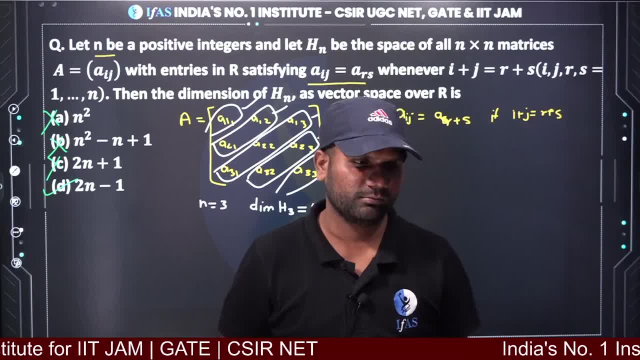 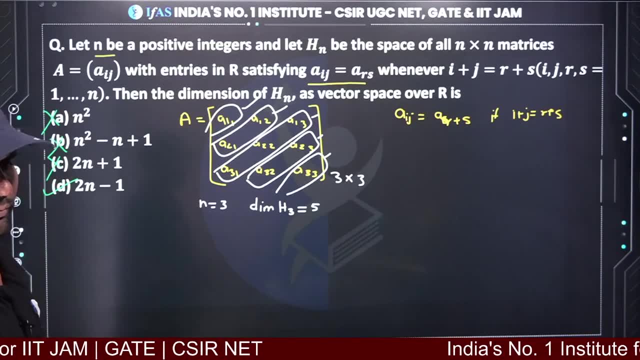 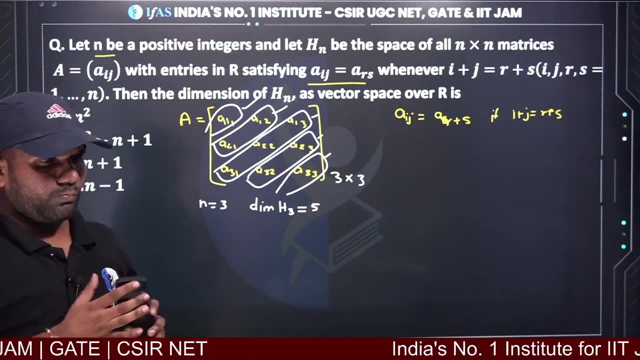 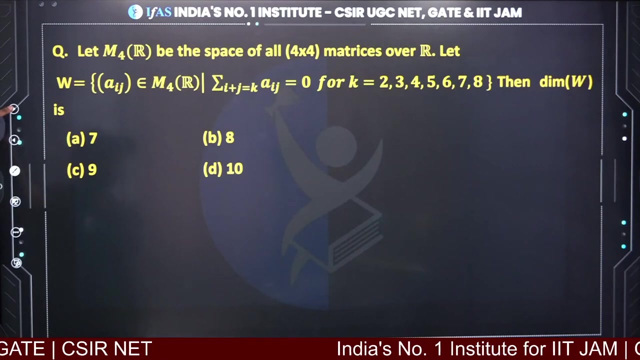 Go ahead. See you guys. So for this question, option d will be correct here. Go ahead, let's move on to the next slide. now this question. see this: can you solve it? if you can solve it, then I will give you the homework. 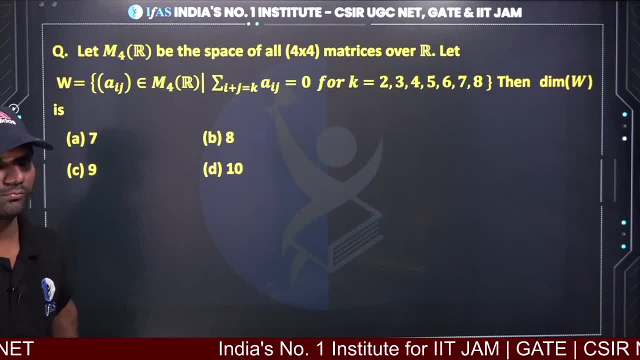 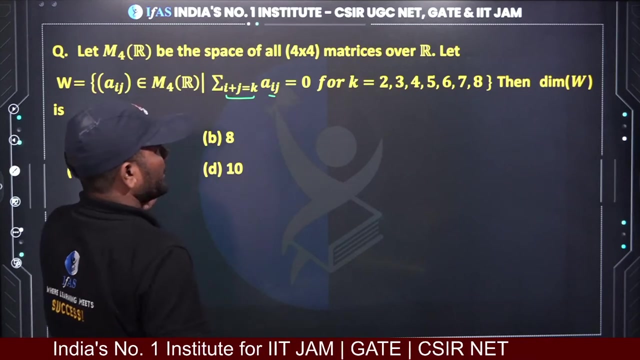 let's see it once. can you solve it? I think you can solve it. what is W? W has 4 cross, 4 matrices, but when we do i plus j, where k is there, the addition of all is 0. k's value is 2,3,4,5,6,7,8. 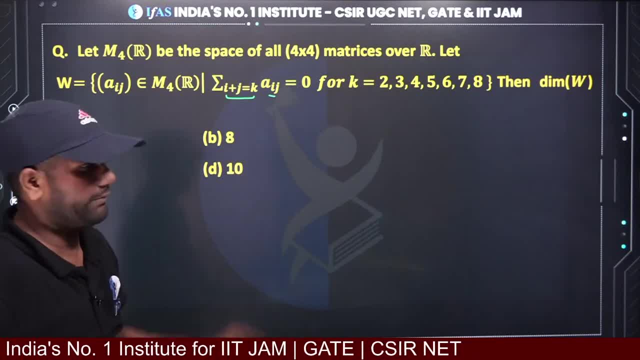 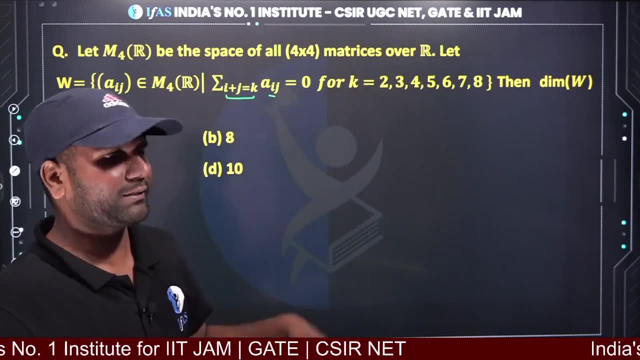 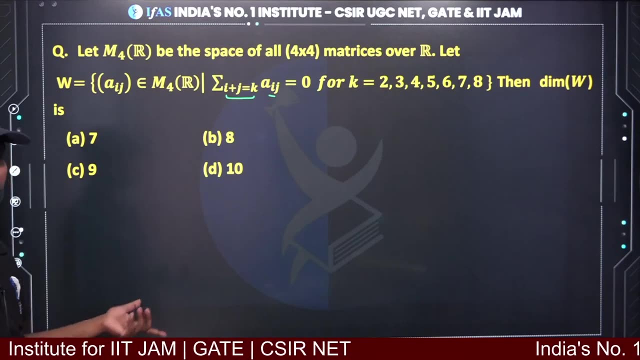 once k's value is 2, low,3, low,4, low,5, low, 6, low,7, low, every time you will get each element dependent, ok, so from there you can try it. ok, if you can solve it, then I will move on. otherwise, if you have any problem, then tell me, I will solve it. 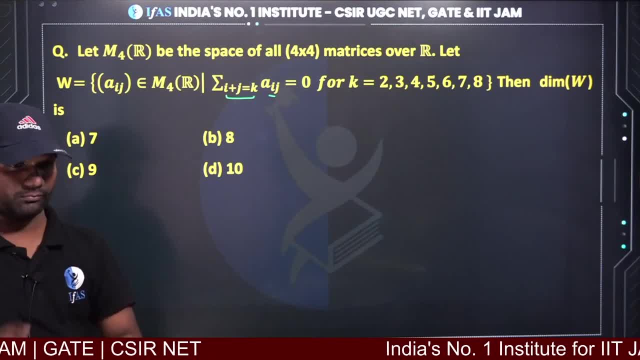 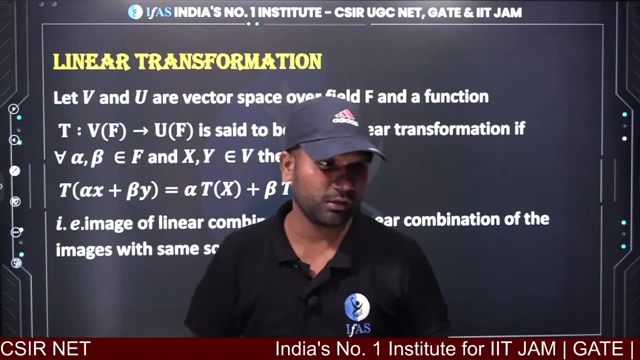 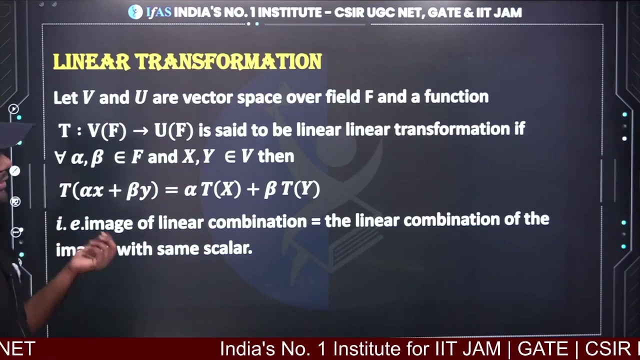 ok, so this is the homework for you. after solving it, you must comment and tell me: ok, let's go now, let's come to linear transformation. so I hope you must know something about linear transformation. ok, so, yes, ok, so any function, you will call linear transformation only when. 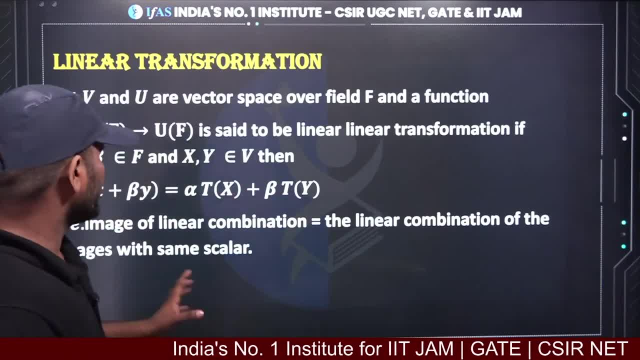 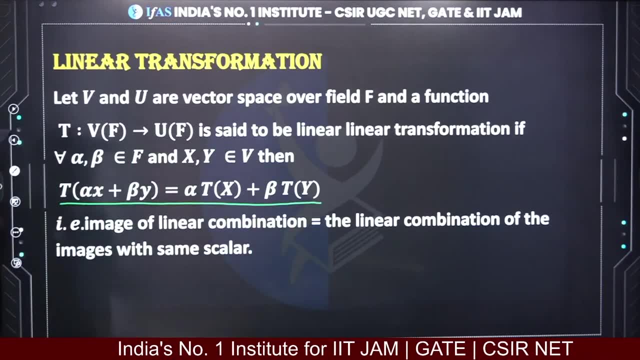 its domain and codomain. take any vector space over the same field which will satisfy this condition. t of alpha x plus beta y is same as alpha times t of x plus beta times ty. so if any function satisfies this, then we call it linear transformation. now let's come here. 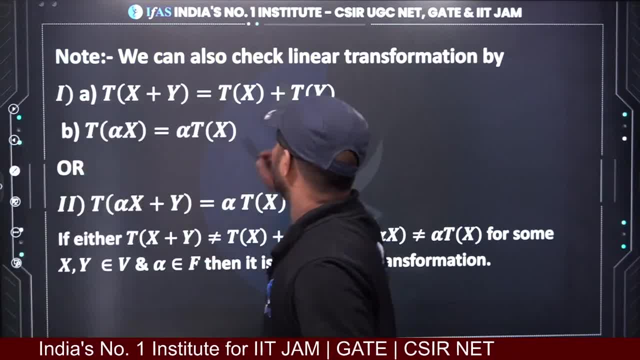 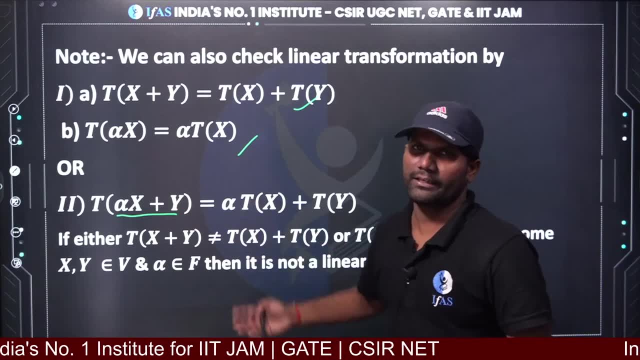 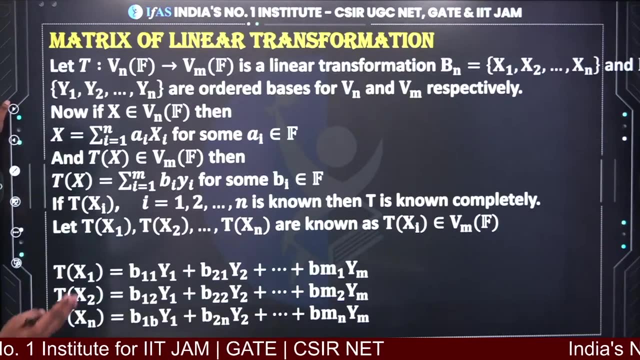 linear transformation is not necessary that you check like this once: check for addition separately, check for scalar multiplication, or your work can work with only one scalar. so these are three ways from where you can check linear transformation. ok, I hope you know all these things. and if every linear transformation is on finite dimension? 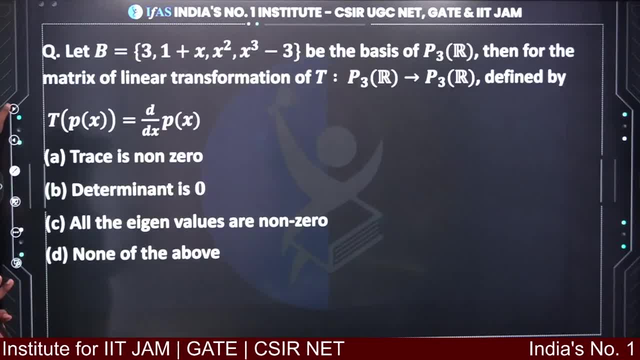 then you can convert it into matrix also. now let's come here to the question. see the question. what is the question given here? B, it has given a basis, basis of P3R. then it is asked: matrix of linear transformation, which is defined like this: so which one will be correct for this? 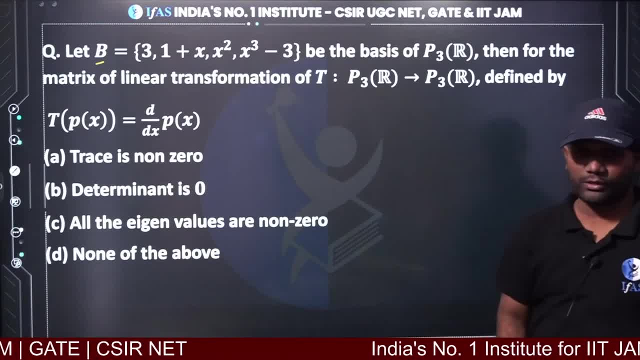 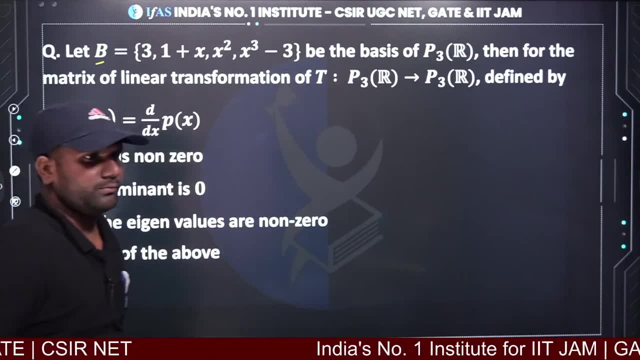 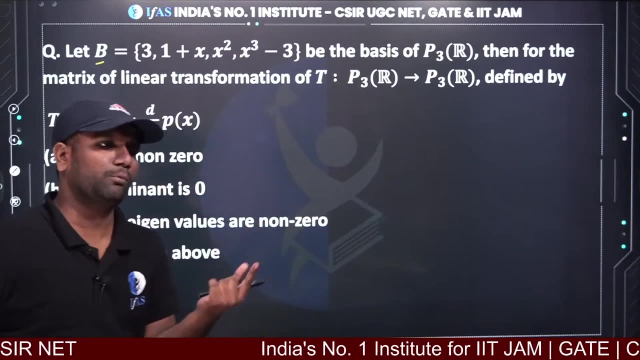 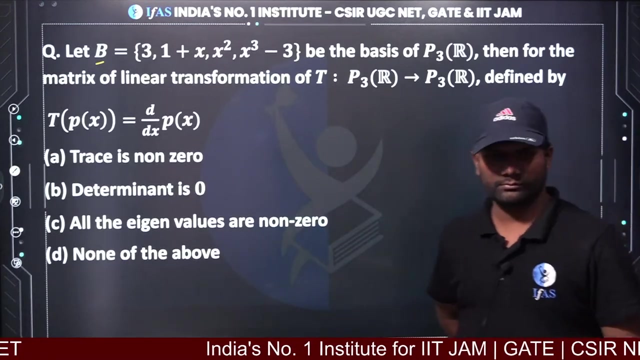 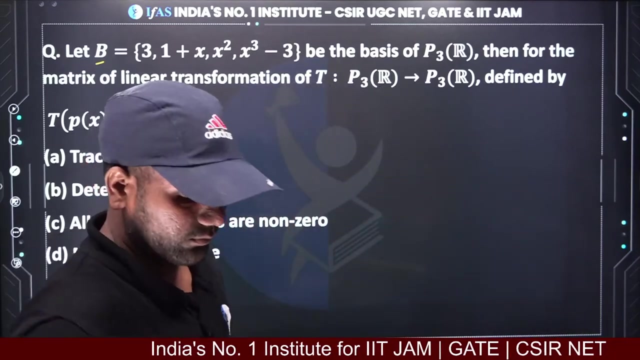 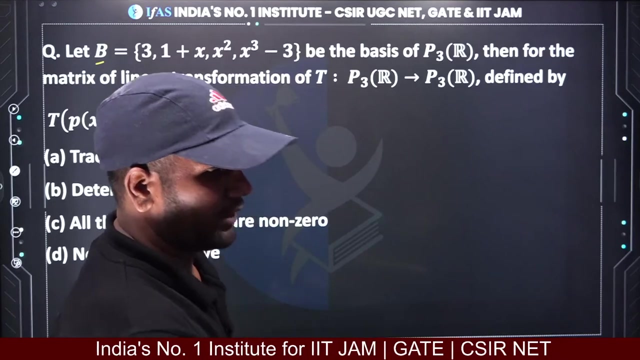 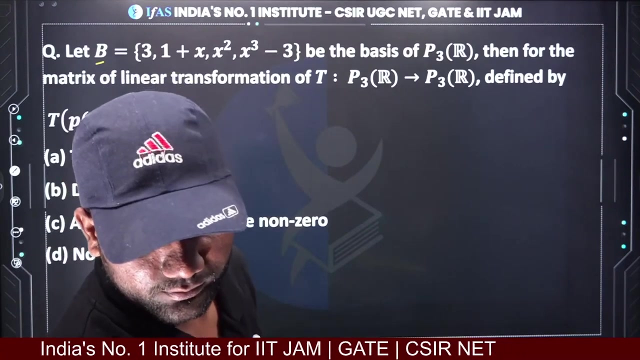 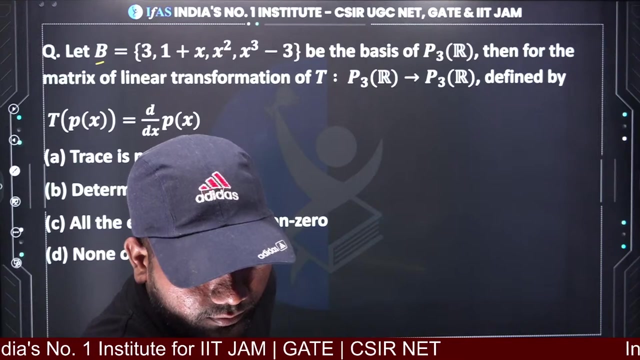 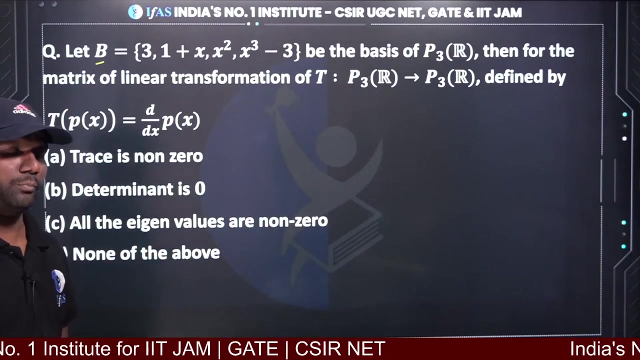 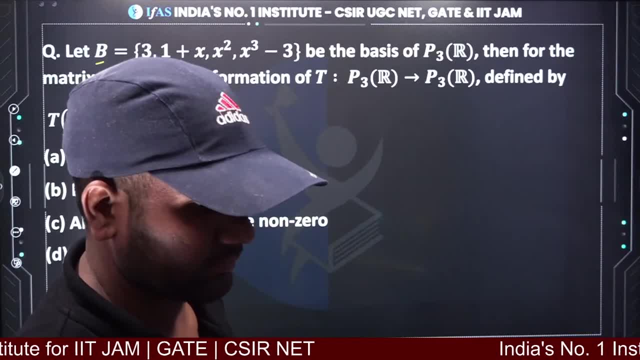 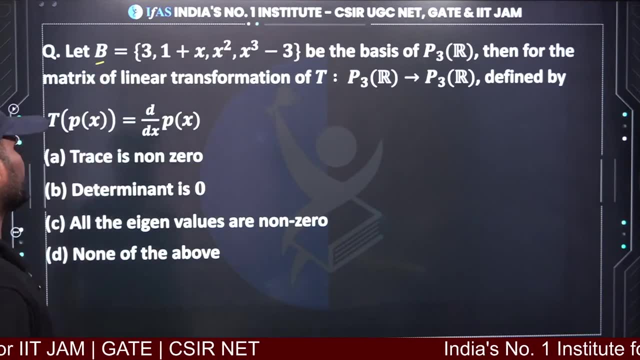 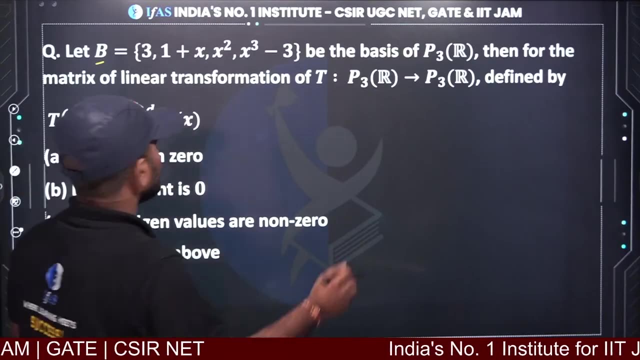 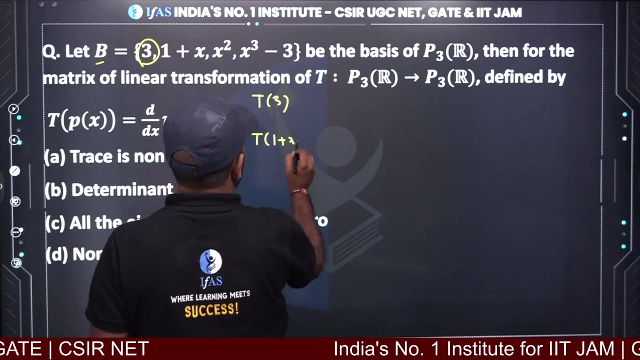 because I'm saying the same thing. okay, Then remember, aged in two B okay is still earned rice. okay, because the Audio B, okay, you can come here. I already gave you here as, because Audio, not M, is wooden, So here. 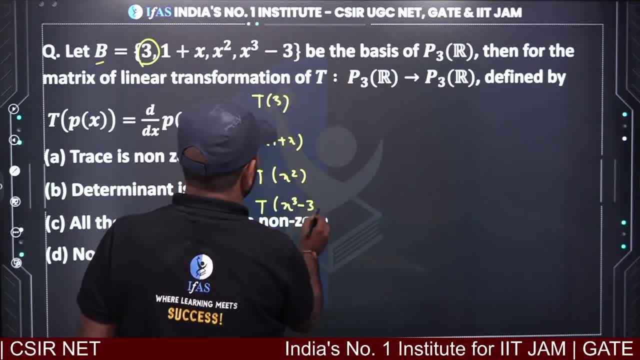 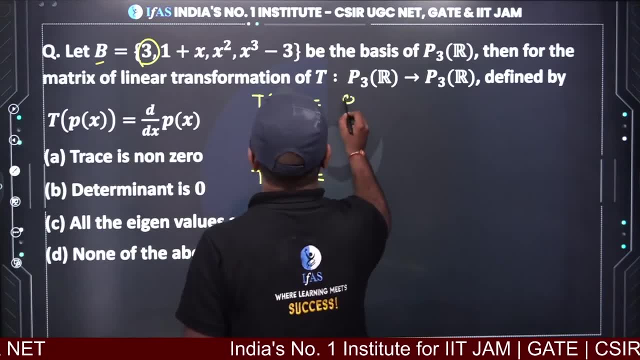 so here. So here, If you subscribe, you see, here we have to find minus 3. ok, see, any function. what we have given here, the polynomial is mapping on its derivative. so what will happen? 0 will happen, that your derivative of 1 plus x will be 1. 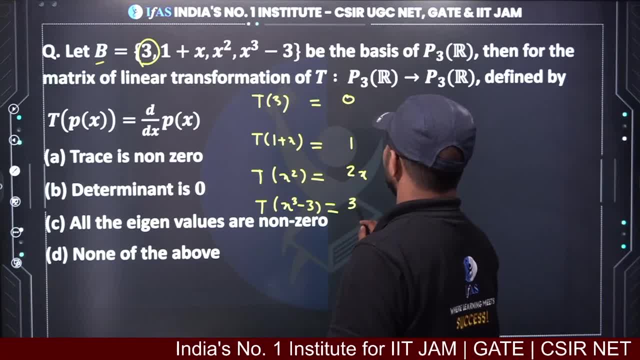 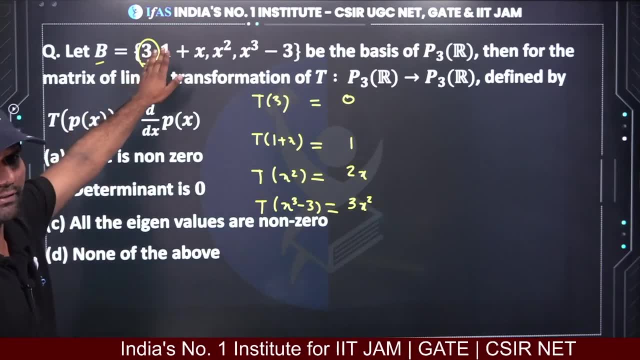 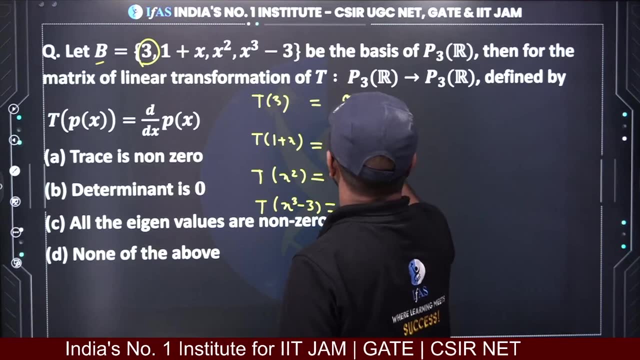 x square will be 2x. this will be 3x square. you got this ok. now, with respect to standard basis, you have to write in its linear combination, not the standard basis which has been given to you. ok, so the first one will be provided completely. how will you write the second one? 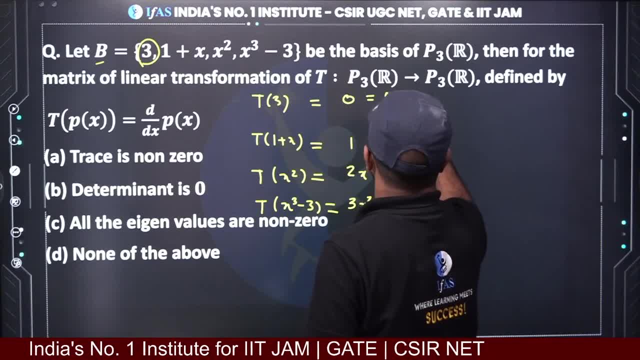 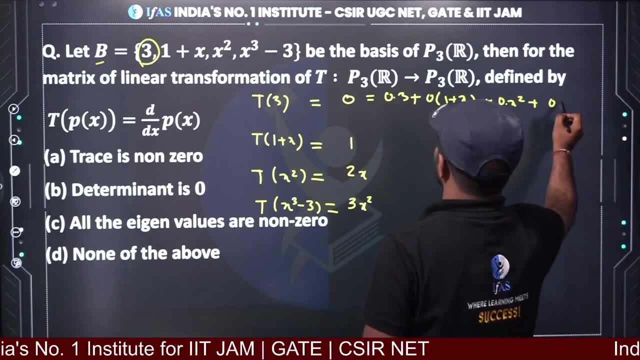 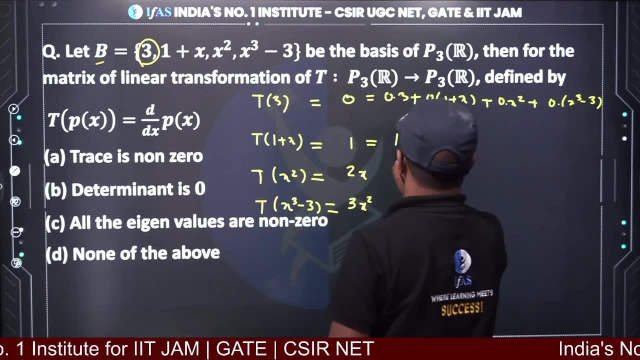 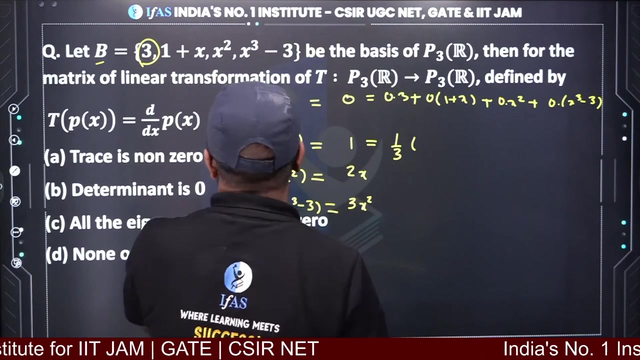 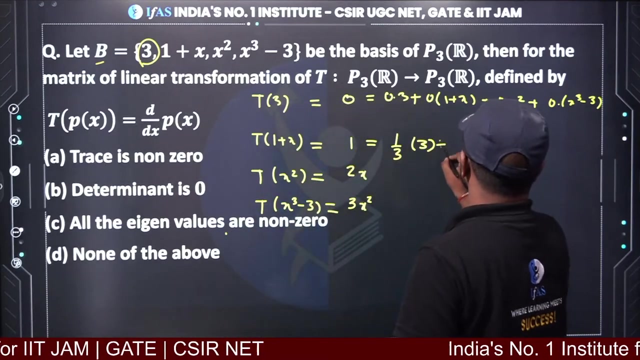 if you get the first one now, what will you write to this 1x3, 1x3. I have got one here. only write 1 by 3 times 3. write and plus 0 times 1 plus x plus 0 times x, square plus 0 times. 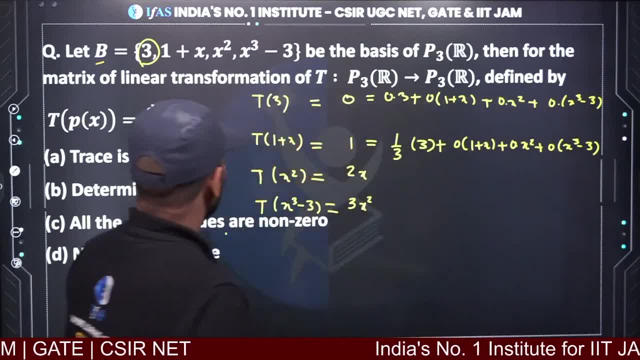 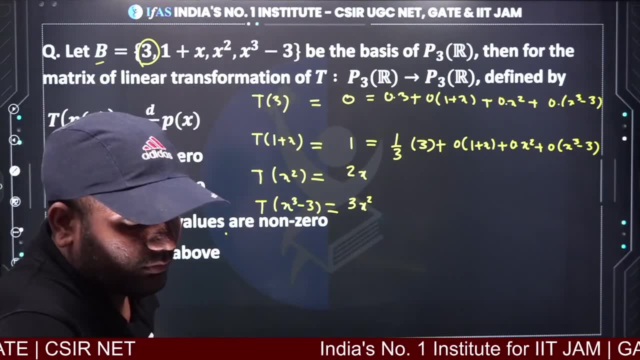 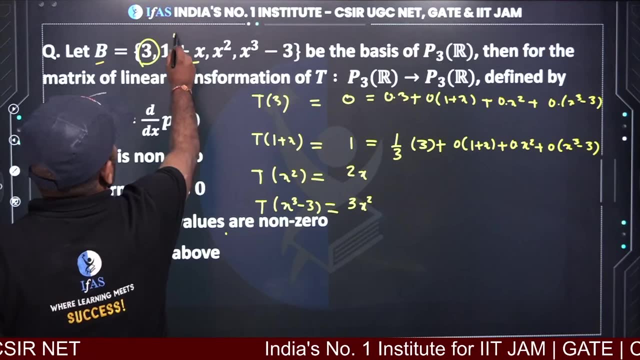 x cube minus 3, write. ok, now what you get: x square, you get 2x. so how will you write it? write it, how will you write it? and you want 2x. so here you can do 2, here you will get 2, but it will also be 2, but you have to remove it. so here what to do. 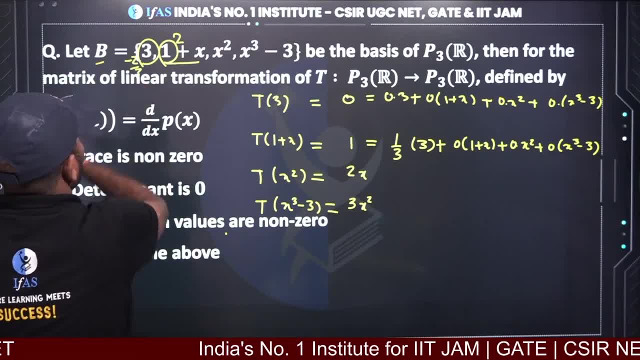 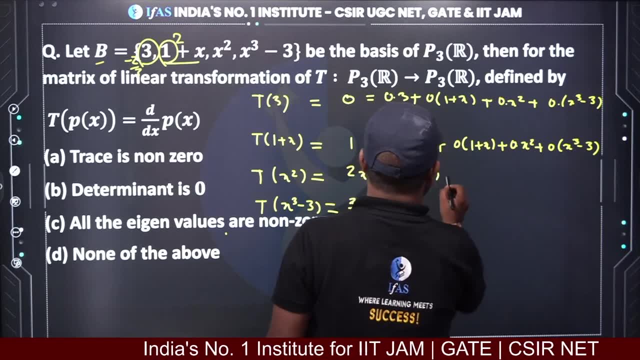 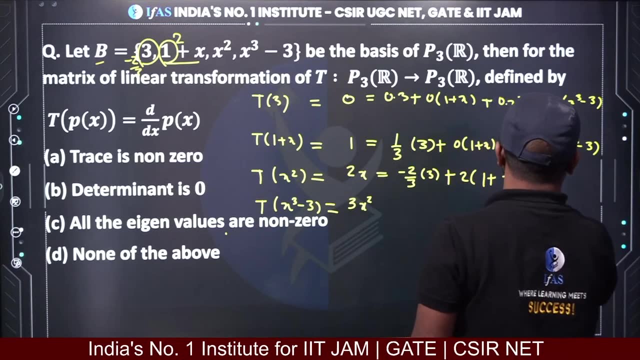 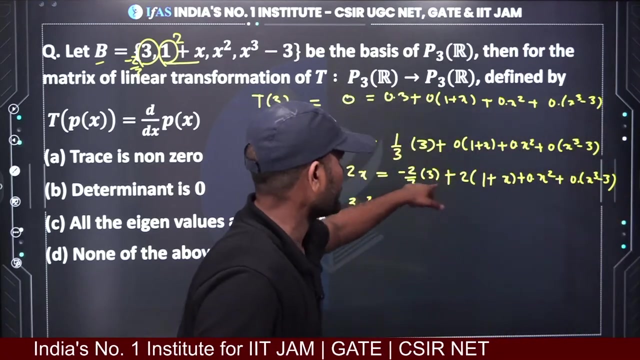 minus minus 2 by 3 here, see here: if I do minus 2 by 3 into 3 plus 2 times 1 plus x plus 0 into x square plus 0 into x cube minus 3, write like this: see what is happening: just 3, 3. cancel minus 2 minus 3. 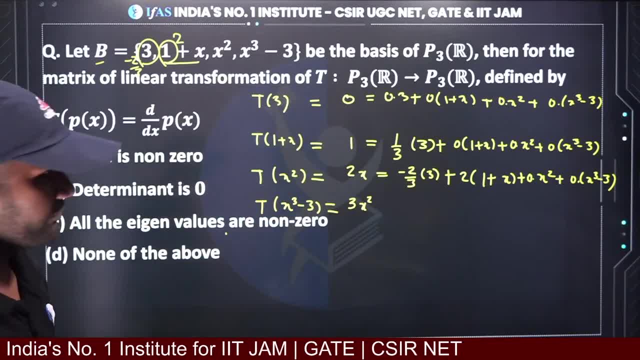 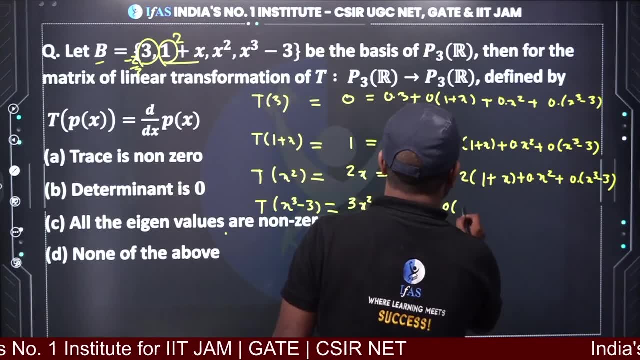 to cancel. yes, 2x will be done. Now here, 3x square is there, so I can simply write it. it will be 0 into 3 plus 0 into 1 plus x will be done. plus 3 into x square will be done. plus 0 into x cube minus 3 will be done. 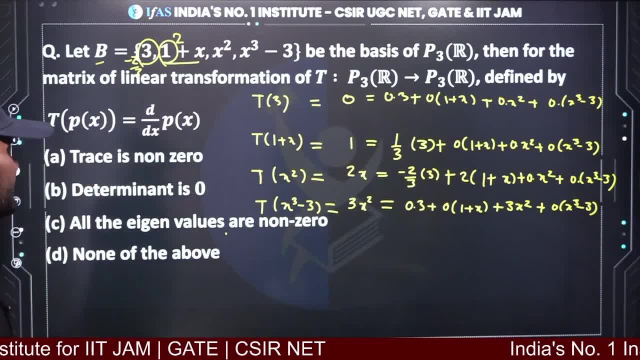 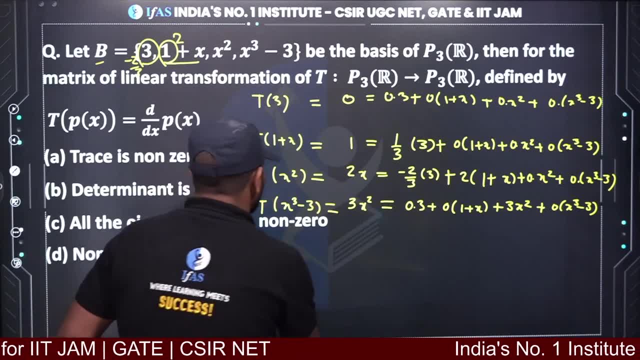 Now convert it in the matrix, write it in the column, you will get the matrix. So if you write in the column, then what will you see in the matrix? You will see something like this: t is equal to first. it is completely 0, 0, 0, 0,. 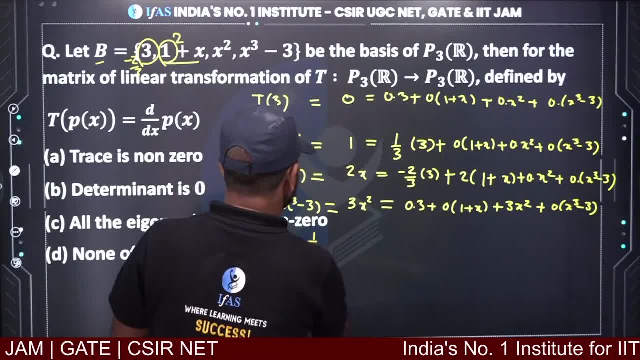 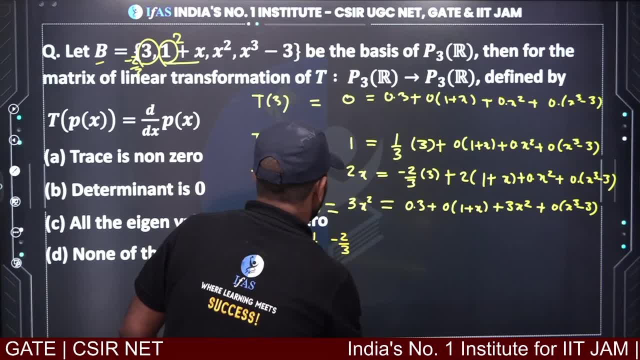 ok, and what will you get from the second 1 by 3, 0, 0, 0, and what will you get from here, Minus 2 by 3, add 2, 0, 0,? 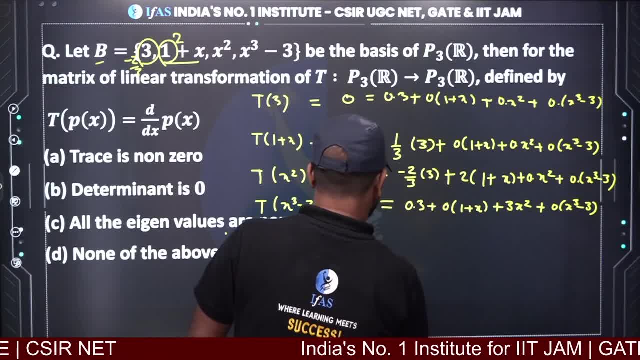 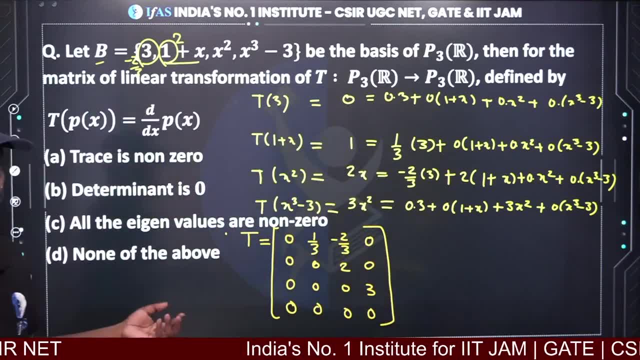 and in the last you will get 0, 0,, 3, 0.. If you see the all eigenvalues of this matrix, it is 0,. all of its eigenvalues are 0, it means that it is a nilpotent matrix. if all the eigenvalues of this matrix are 0,, 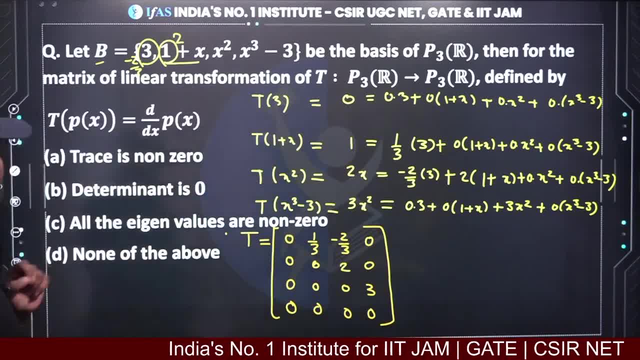 what will it mean? It will be a nilpotent matrix. if it is a nilpotent matrix, then the first option: trace is non-zero. incorrect. determinant is 0- correct. all the eigenvalues are non-zero. incorrect, none of the above. 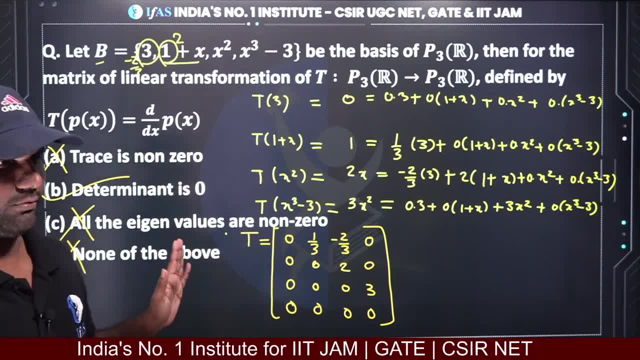 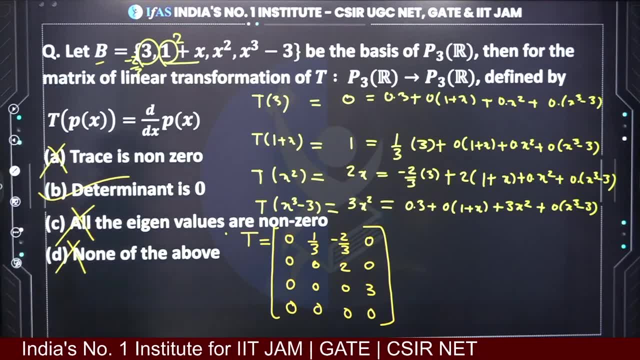 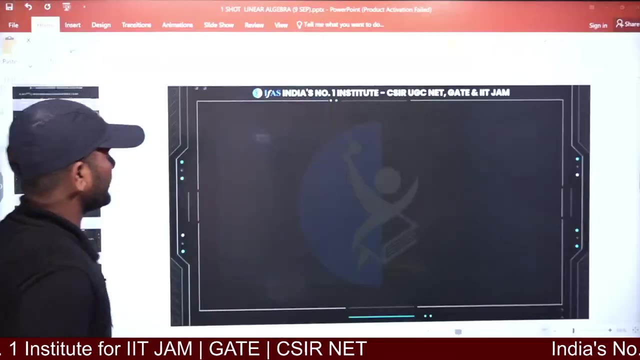 so here only one option will be correct, that is option B. ok, I hope you have cleared it up to here. yes, ok, now we move ahead. wait, I am giving a question first, solve it, then we will do it later. 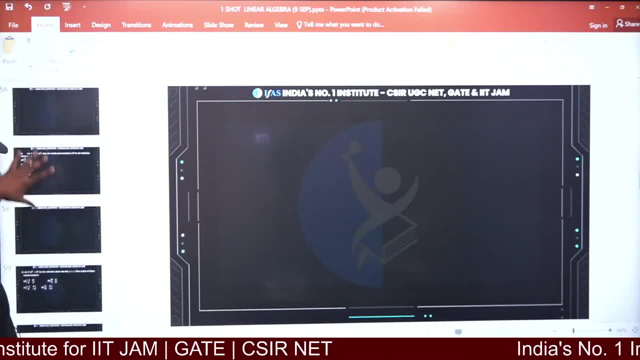 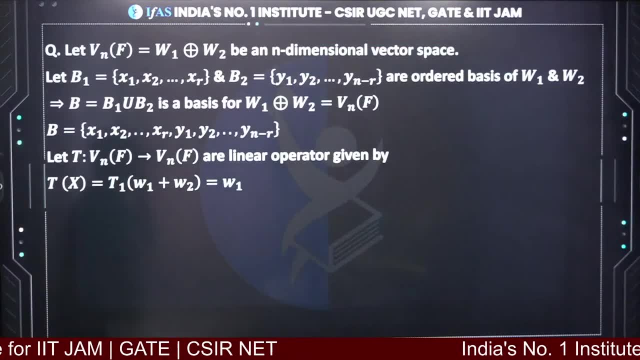 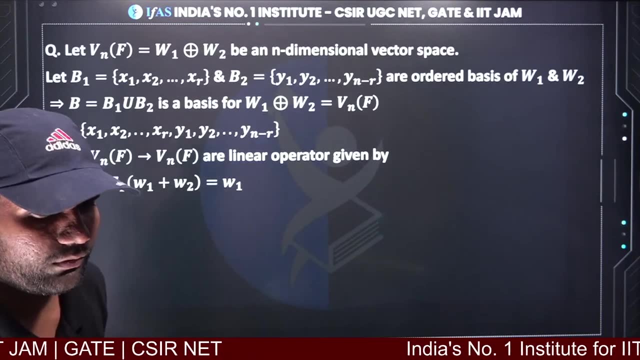 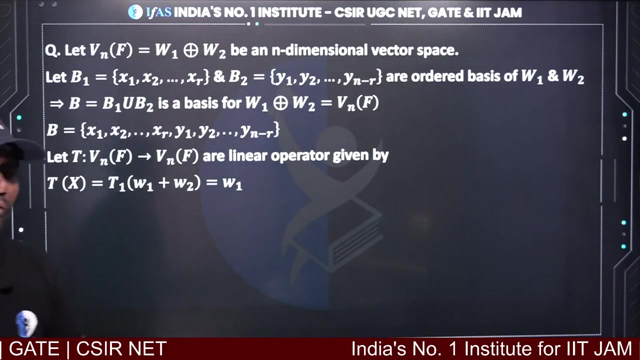 wait first. there is a question. first solve this question. if you come to the exam to convert in LTE, then it will not be so simple that it will ask you on derivative 2, yes, you can use it now. then there were some others. maybe there will be something different. 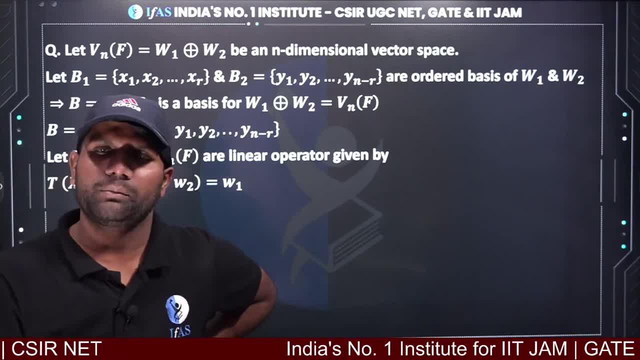 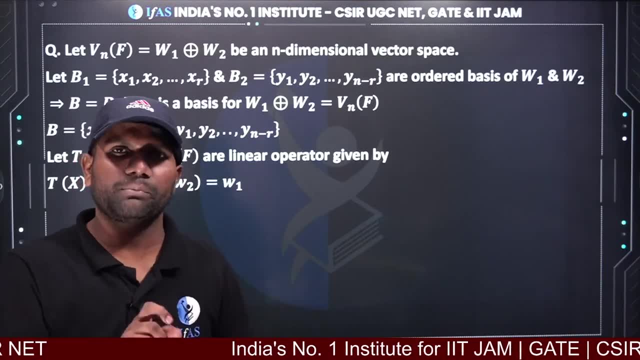 I multiplied it so that what we had to do we had to write in the linear combination of the basis. I had to adjust the linear combination because when you find the T of something, then write it in the linear combination of the basis. there was 2x. then you can write it in the linear combination of the basis, then you will find that the T of something, there was 2x. 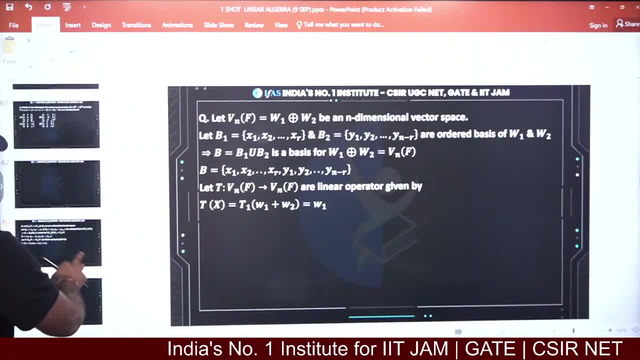 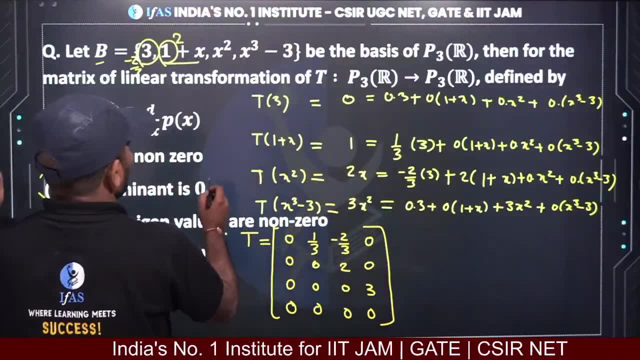 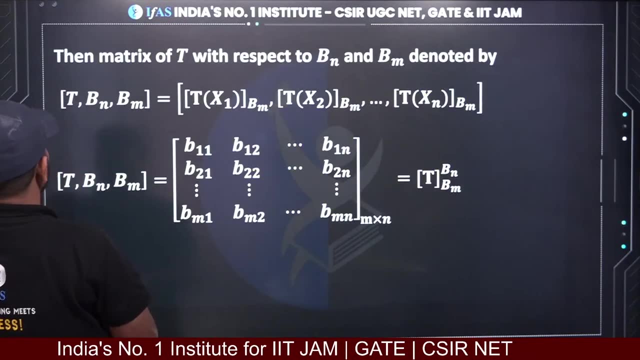 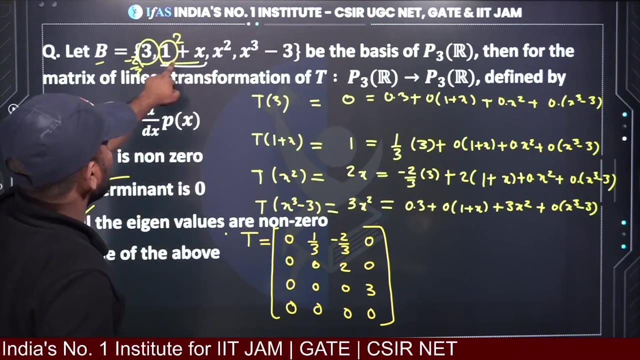 see here: 2x. here you got 2x. so if you look at the basis, then 2x. see, now it was 1 plus x. so if I multiply it by 2, then here I would have got 2. also, yes, to finish this 2, I used this. that's it. 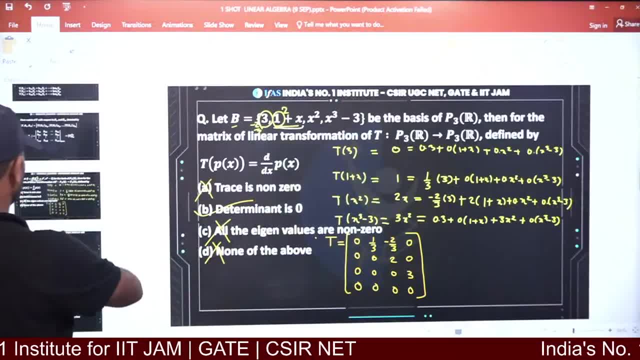 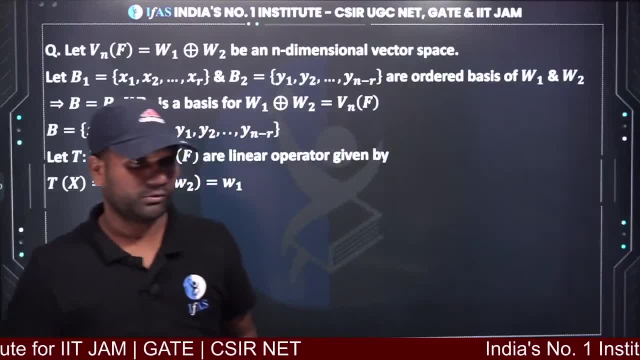 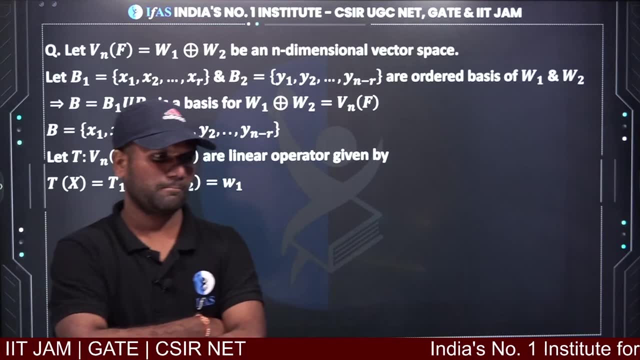 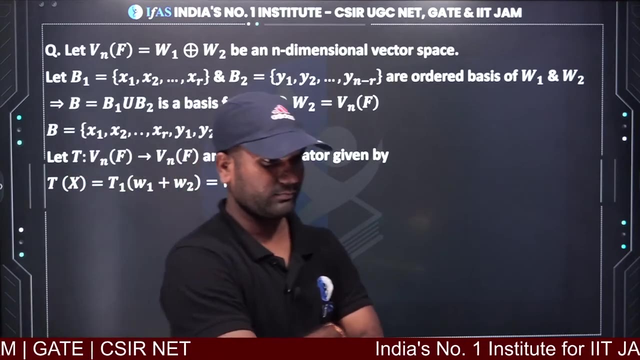 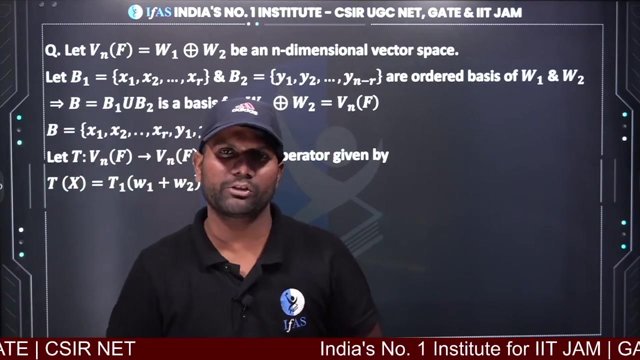 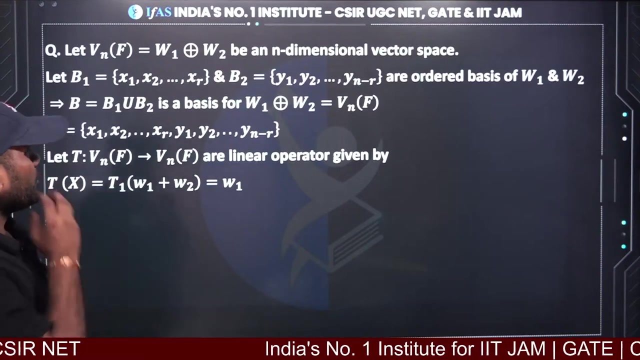 ok, yes, you guys, solve this question and tell me about it. you can say something about it. if you want a hint, then you can ask: what do you think? but if you will be snowing, to convert the question now a little paper pattern, But hasn't changed much questions, this type of chances are here. see what we have given. 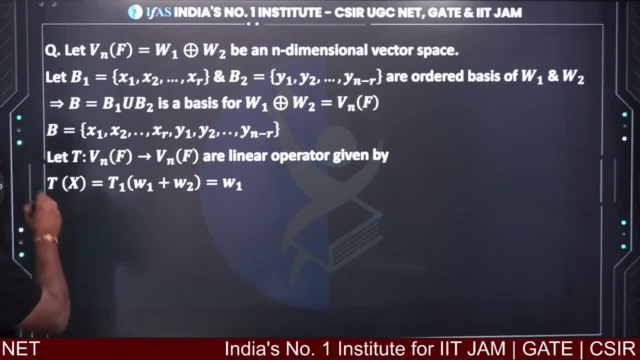 some information here so that you don't suffer. please see here what i have given. we have special vector which is direct sum of w1- w2, where the basis of w1 is same, but instead, if you can change something, then it will also help. 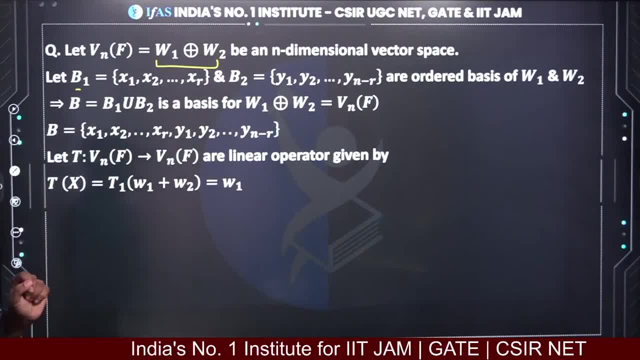 where w1 is the basis of a and w2 is the basis of a. if this is the basis of w1 and w2, then the basis of direct sum union of basis of w1 and basis of basis of w2 means, if I take, union of b1 and b2. 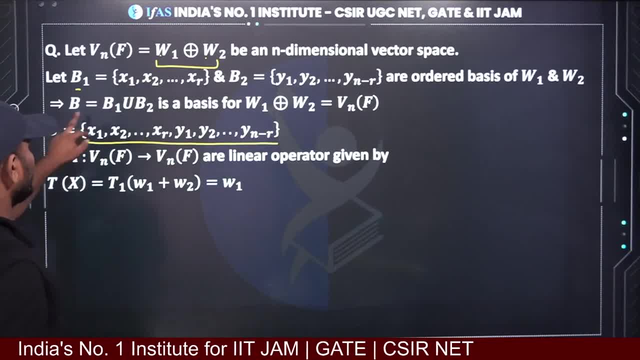 then, whose basis did you get? you got the basis of a and you got the basis of b. now I have defined a linear map, t from vnf to vnf, which is defined like this: here it is t, it is twt1, it is t. 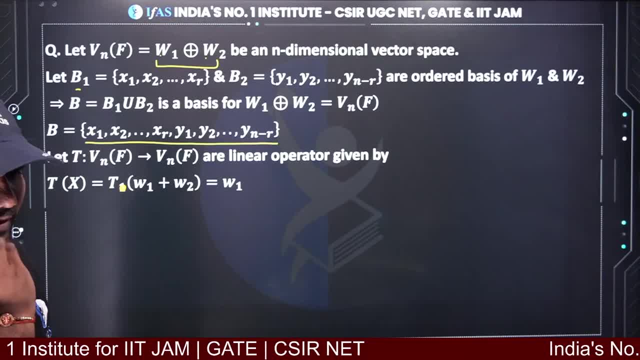 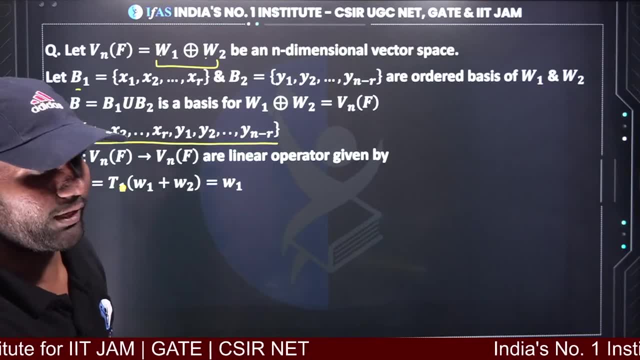 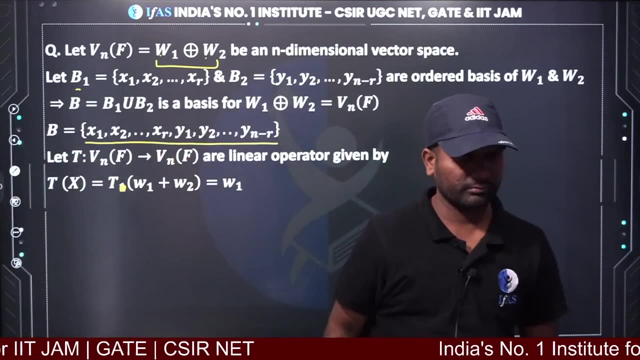 ok, it is defined like this: Ok, ok, we have to convert this in matrix. with respect to this basis, no, no, do not remove the project, so let the orthogonal projection be kept. just convert in the matrix. ok, now tell me a special thing about Direct sum. when I say: 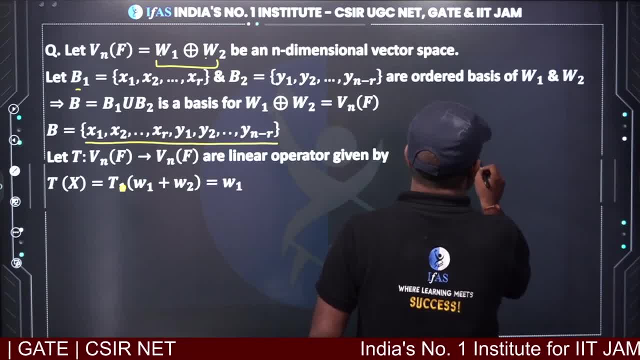 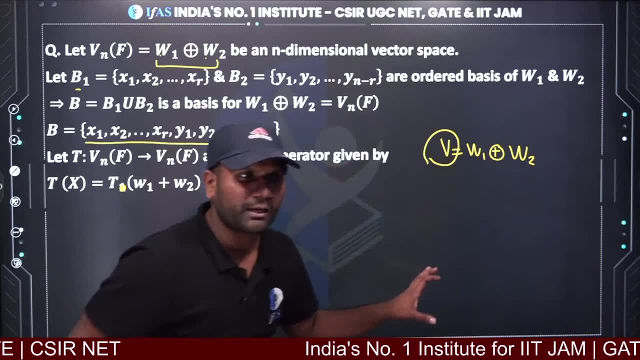 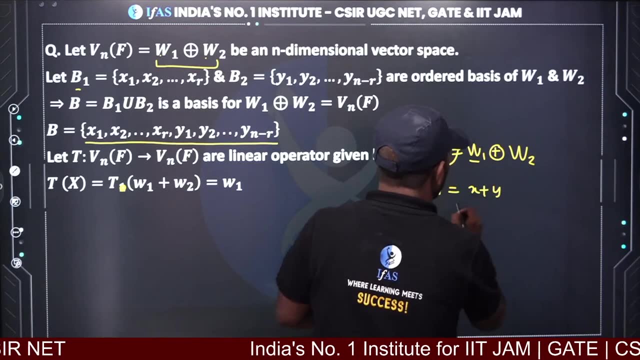 v, if I am saying that v is direct sum of its subspace, w1 and w2, which means listen, listen. if you take any element of V, then you will get one element in W and one element in W2. you can write like this: 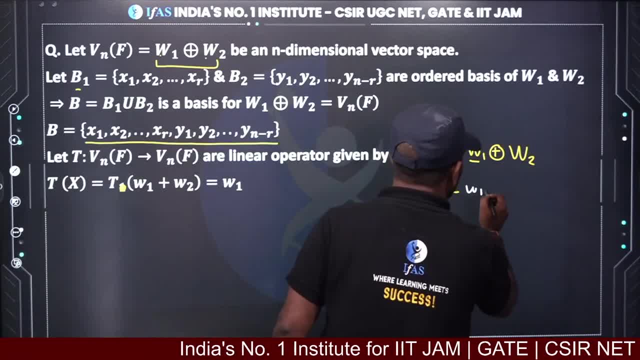 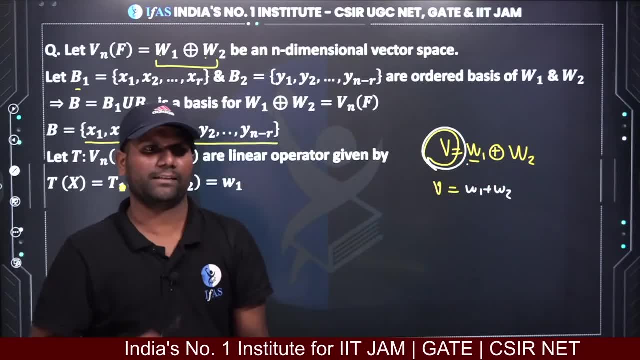 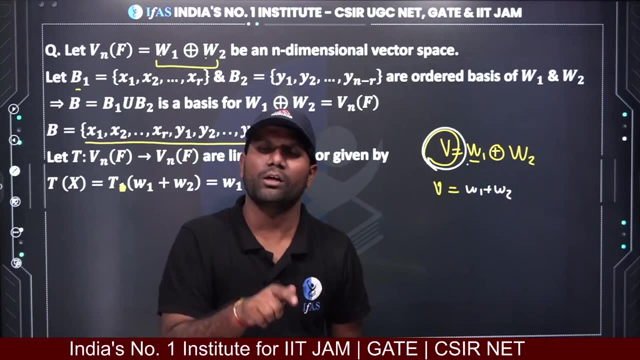 let me remove the notation. you can write all the elements of V in the form of W1 and W2. if I say V is a direct sum of W1 and W2, it means that every element of V can be written as a sum of W1 and W2. 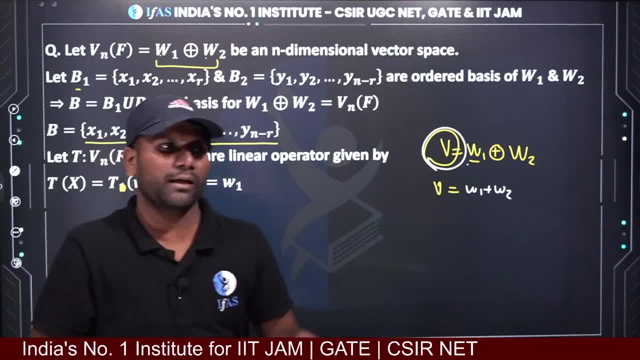 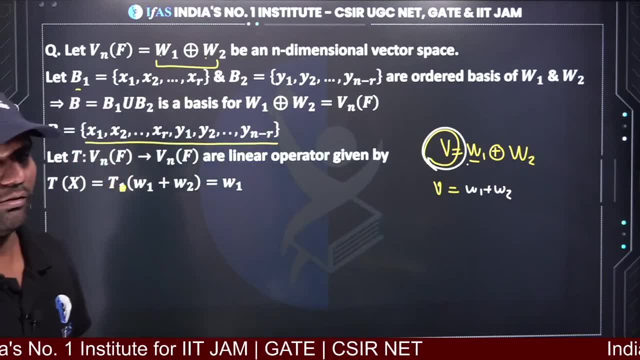 you will get one element from W1 and one element from W2, which you can write in the form of W1 and W2. can you convert this into a matrix? is it easy or difficult? it is easy in my opinion. I have told you the rest of the things. 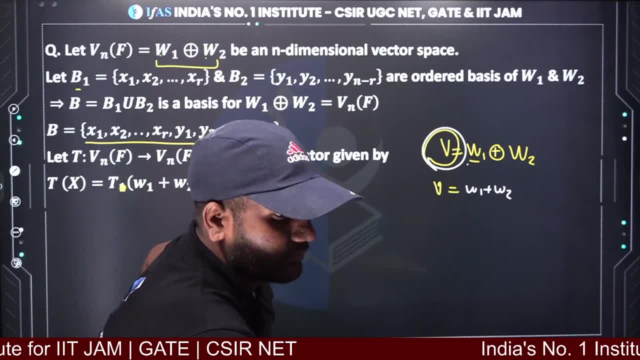 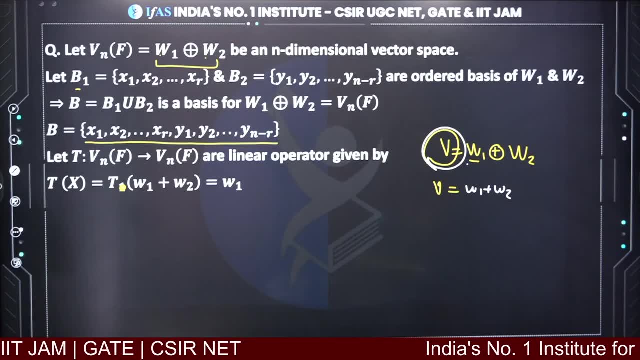 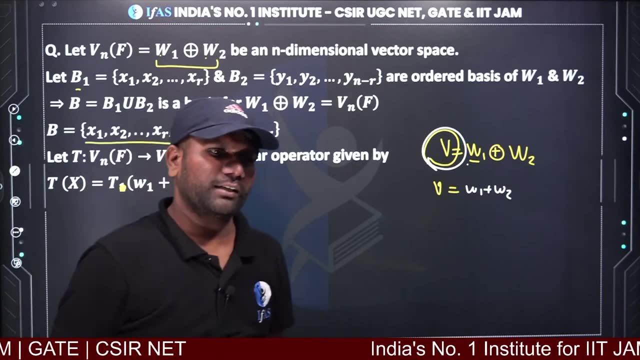 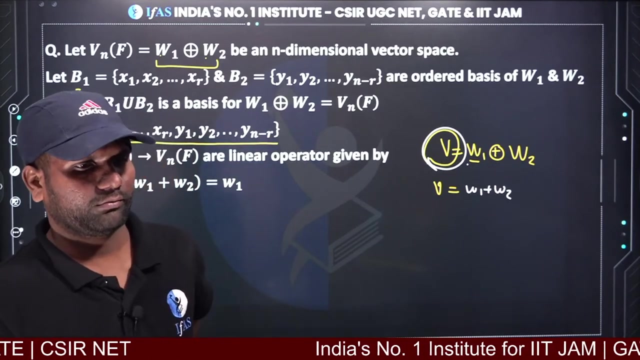 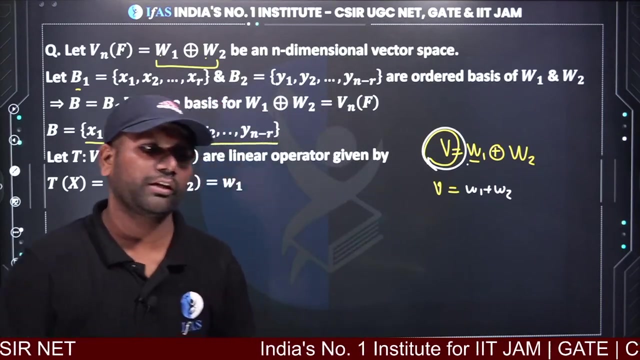 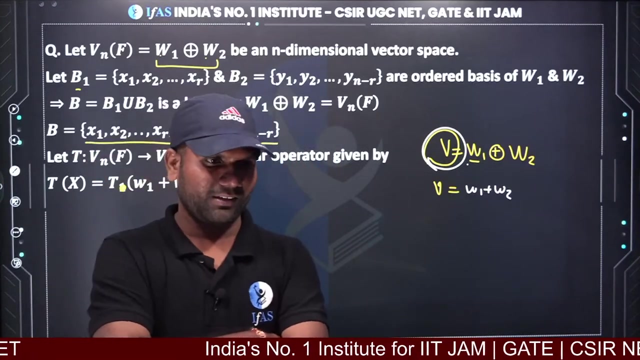 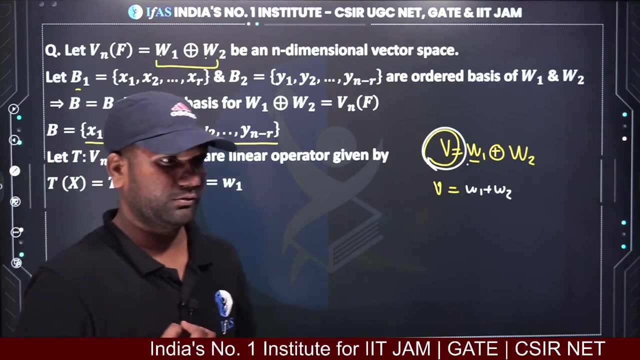 now you tell me. tell me quickly, yes, very good, Asha, very good, very good. other people: tell me: what do you think of the rest of the people? yes, if someone is having a problem, then I will try and tell you how to do it. see, you have already given you the element of the basis. 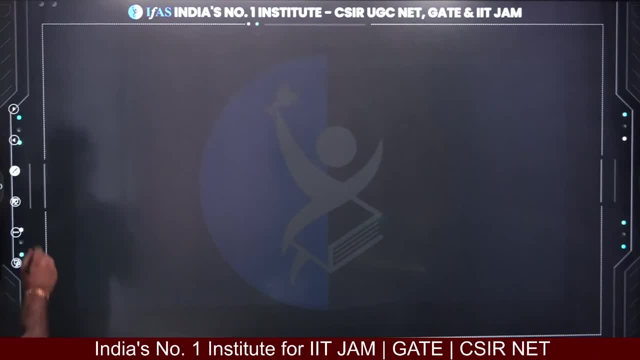 this is the basis element. given means what you have to find. the map you have given by defining T of X. what is T of X now? where does X belong in V? what do we know? V is the direct sum of W1 and W2. 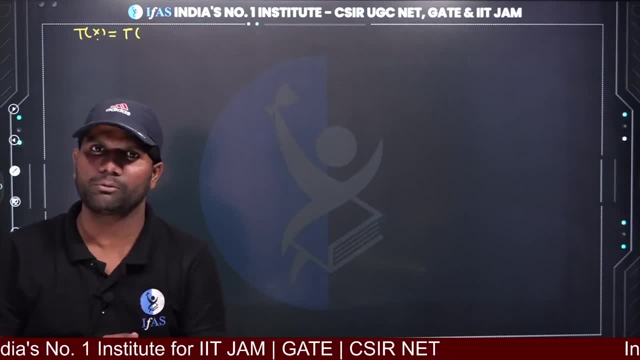 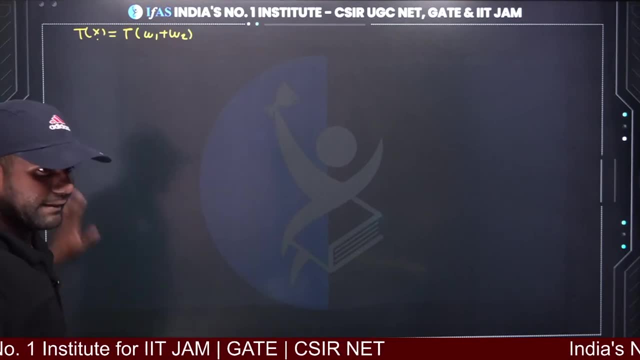 it means that every element of V can be written as a sum of W1 and W2 means you can take it from one element, W1. you can write it in the form of an addition of one element, W2. you can write it like this and after writing, it is saying that T of W1 plus W2 maps to W1. 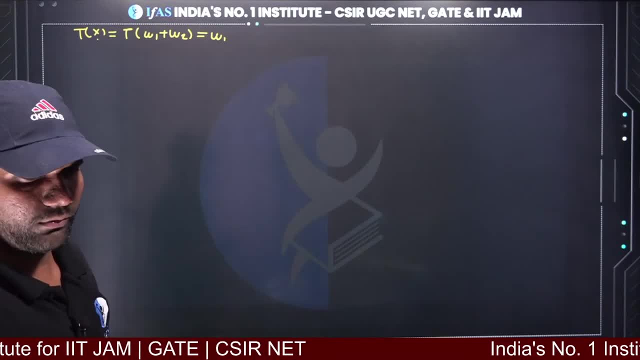 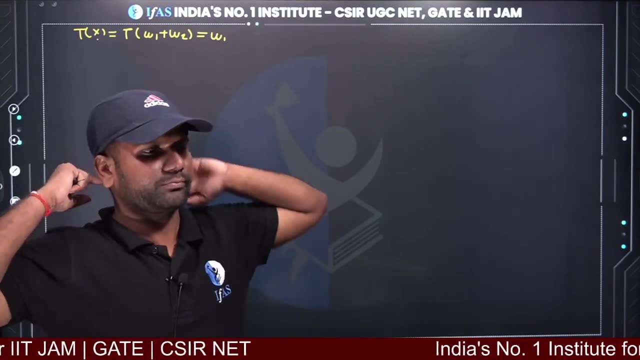 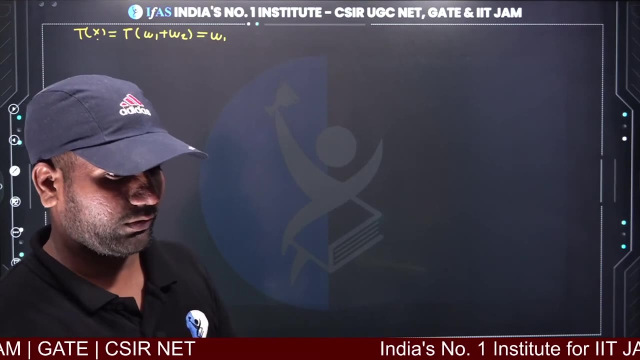 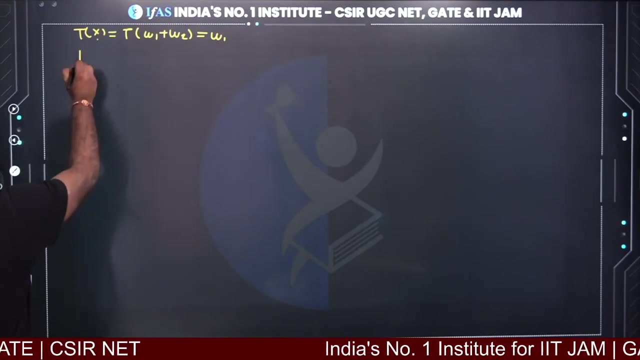 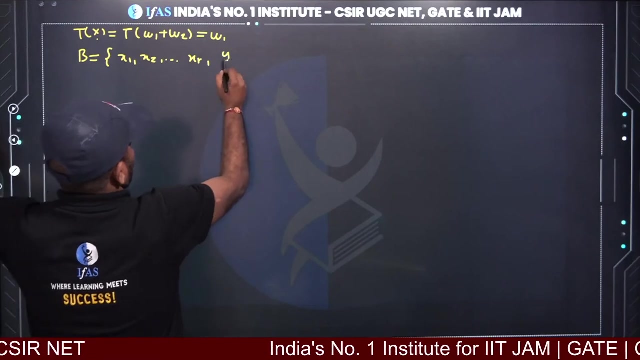 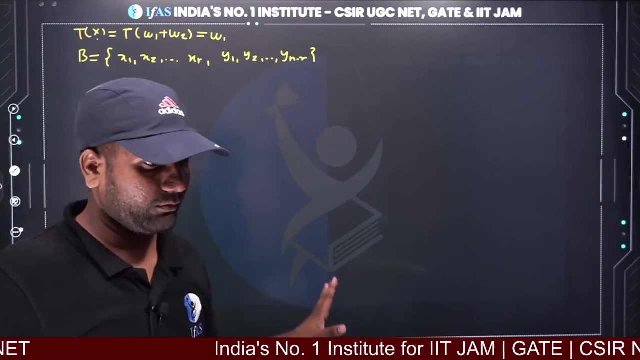 ok, this is given to us for DU. when is the exam for DU, Parul? once you tell me when is the exam, yes, ok, I will write it in the form of an addition of W1 plus W2. what is this? this is its basic element. 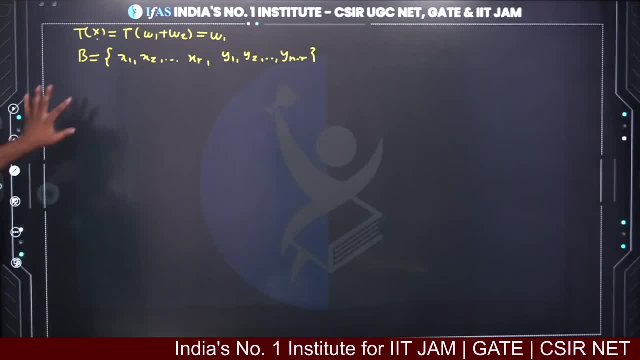 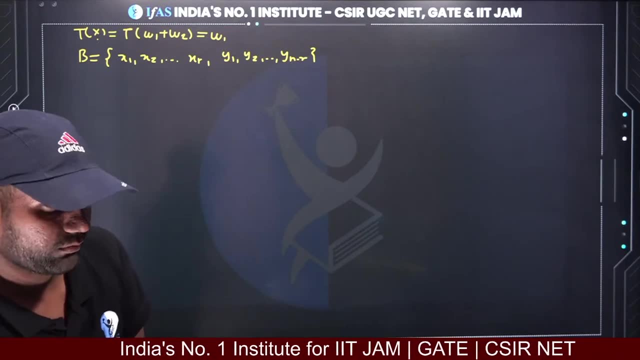 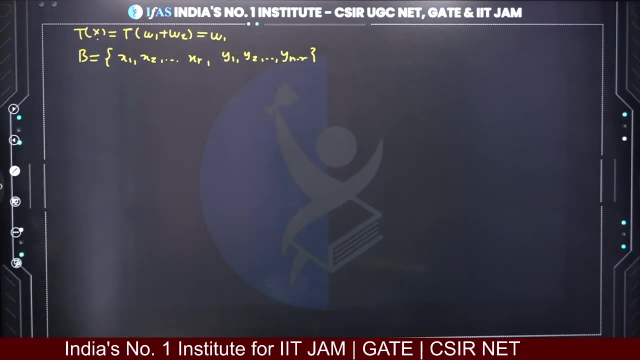 ok, this is its basic element. now let's come here. see you guys, see carefully, now what do we have to find? we have to find the T of the basic element. if we have to find the T of the basic element, one minute, ok, now it will come out. 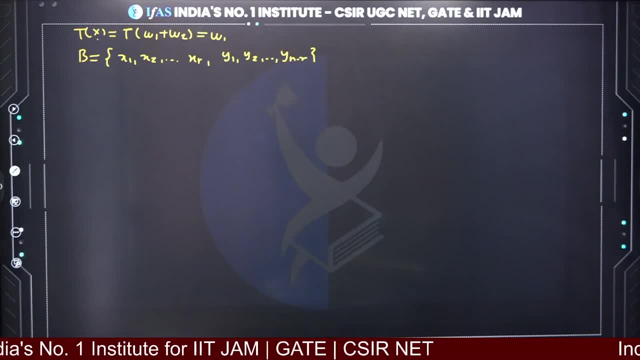 ok. 1, 2, 3, 4, 5, 6, 7, 8, 9, 10, 11, 12, 13, 14, 15, 16, 17, 18, 19, 20, 21, 22, 23, 24, 25. 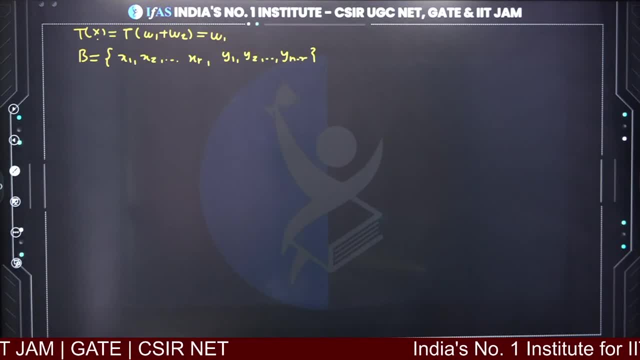 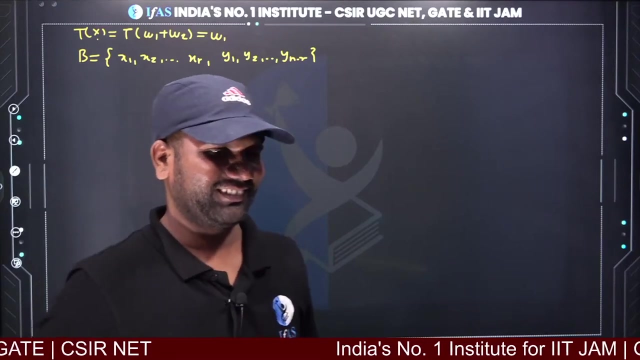 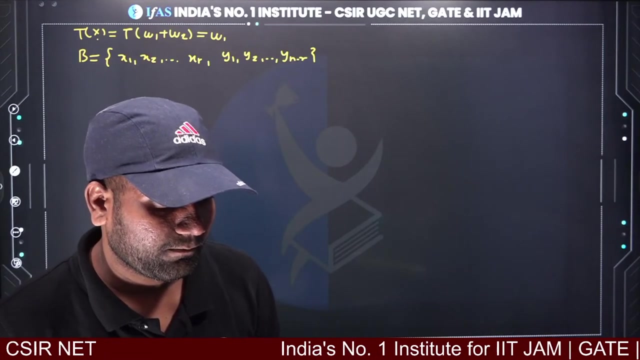 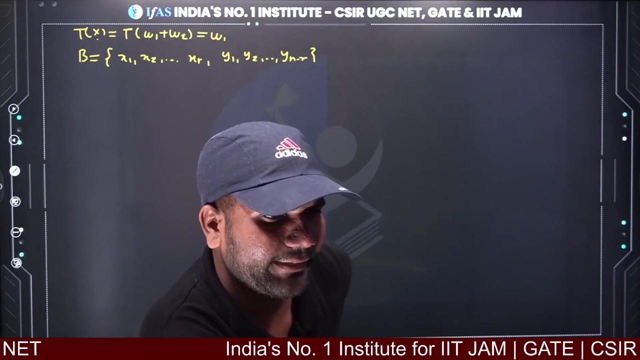 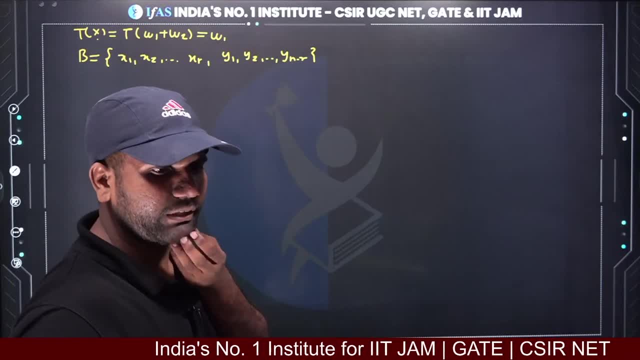 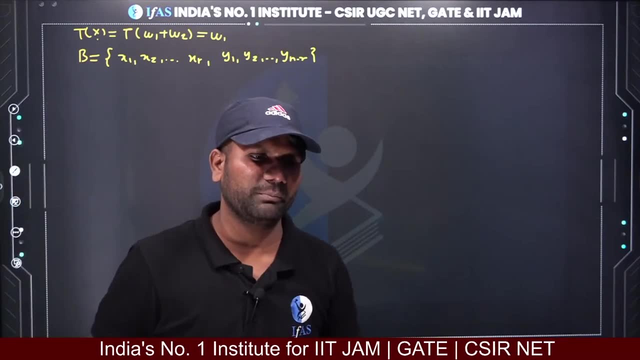 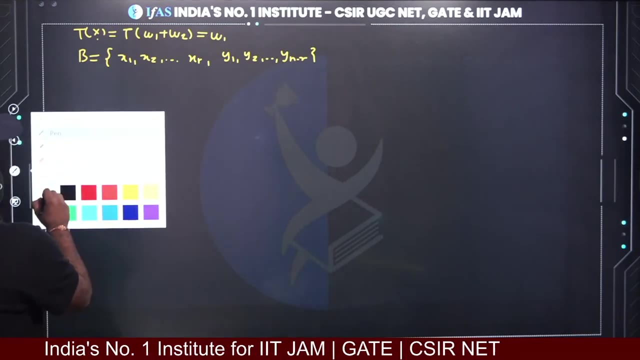 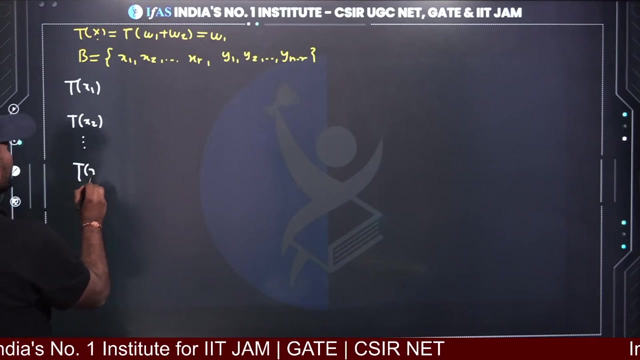 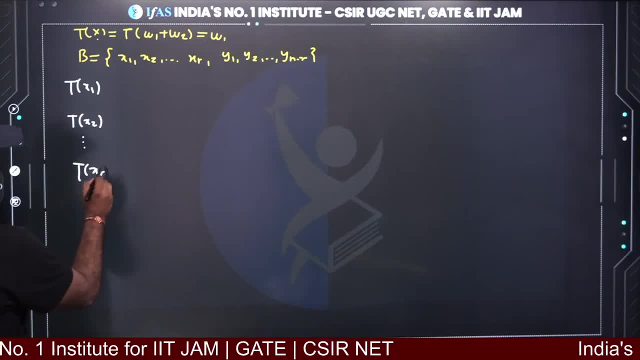 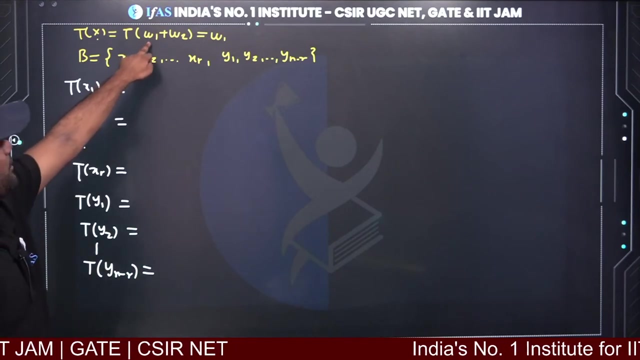 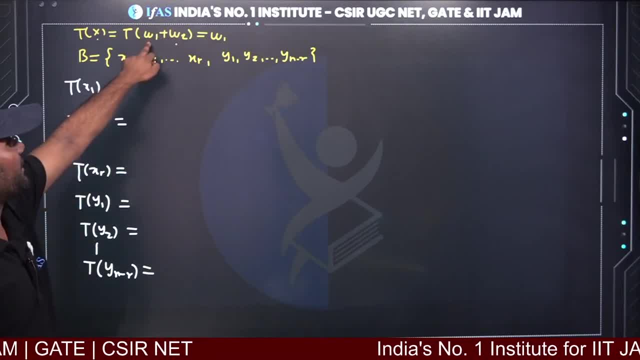 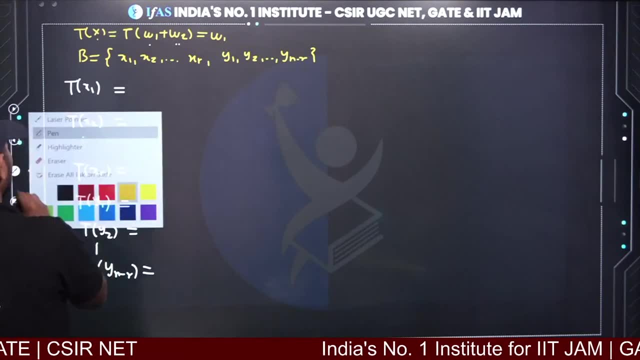 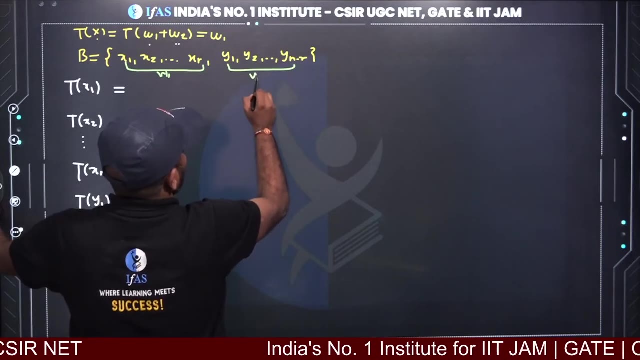 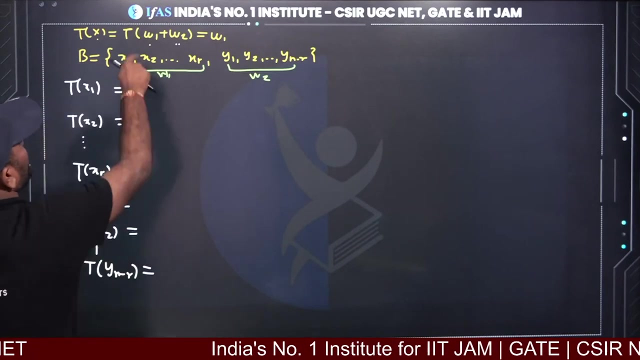 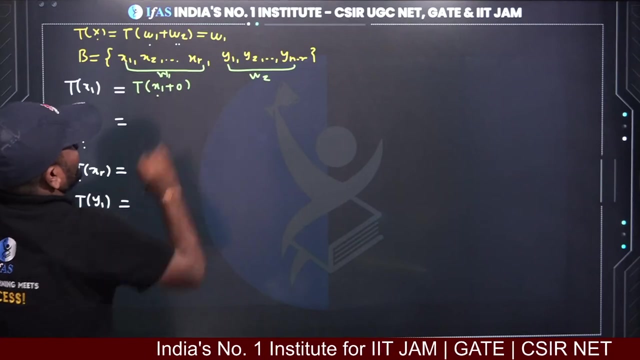 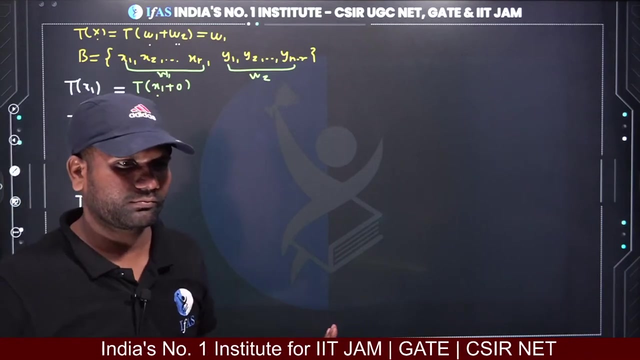 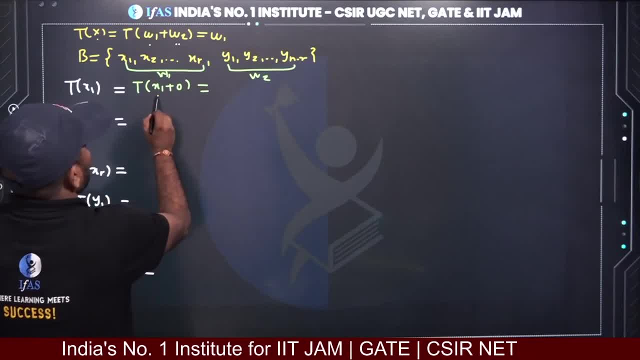 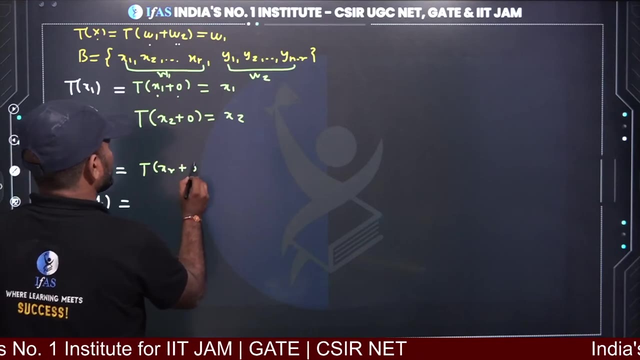 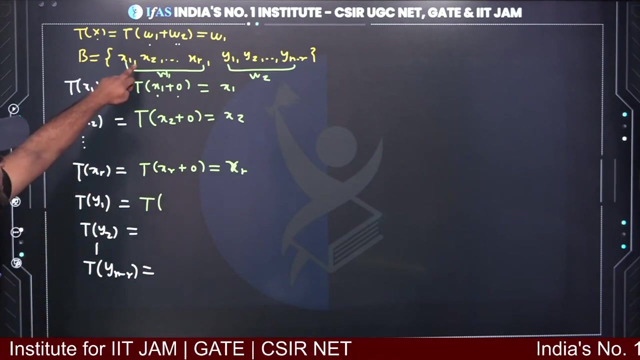 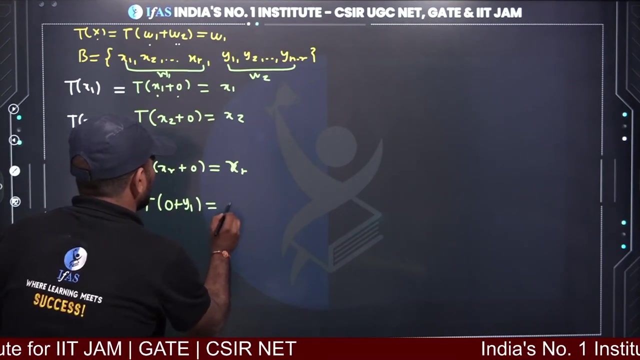 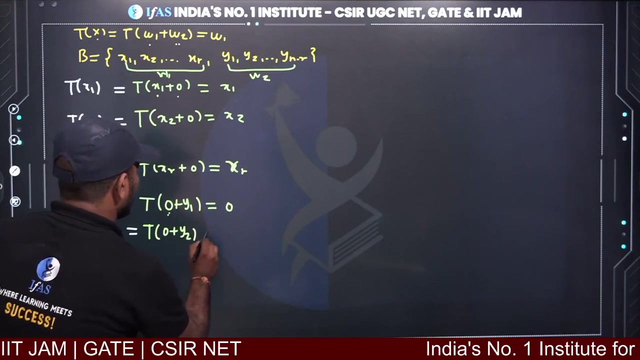 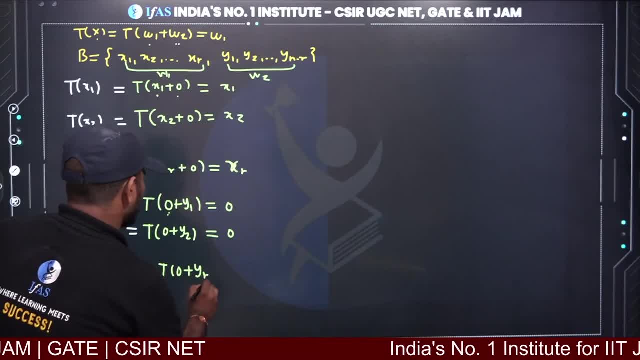 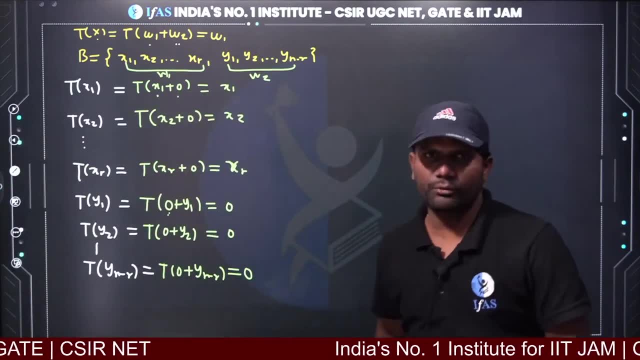 similarly, t of 0 plus y, n minus r. where will a go? it will go to 0. so if you can convert it easily in the matrix, I don't think it will be a problem to convert it in the matrix. do you think you have any problem? 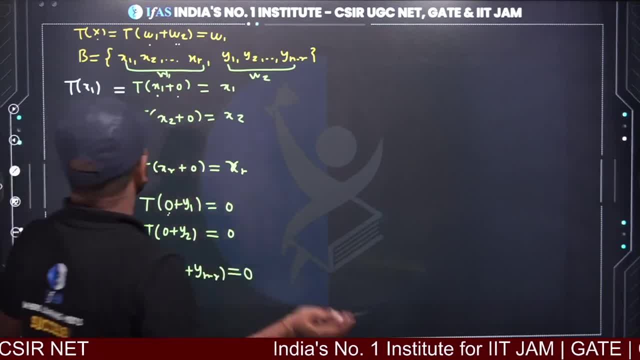 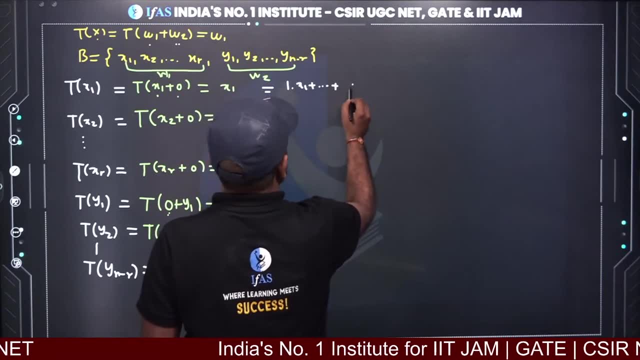 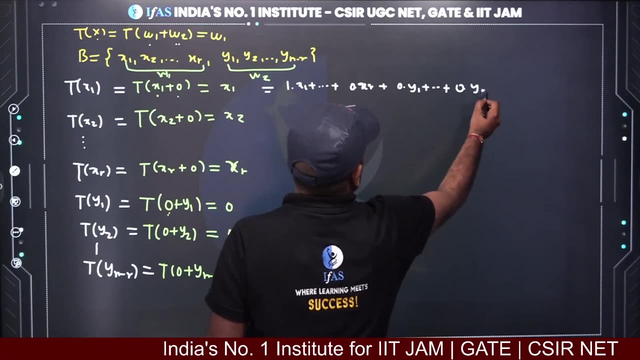 ok, now see here. I can write it like this: 1 times x1, plus, and so on: plus 0 times xr, plus 0 times y1, and so on: plus 0 times y, n, minus r. similarly, if you write it to all and convert it in the matrix: 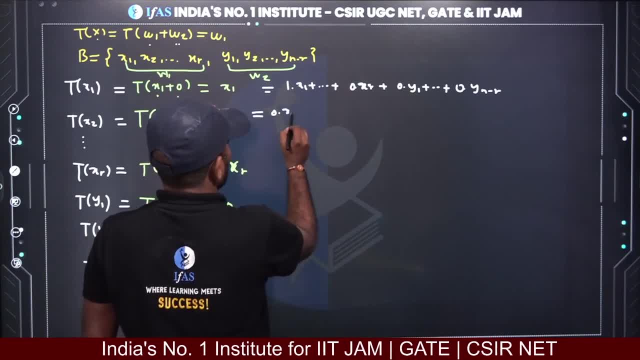 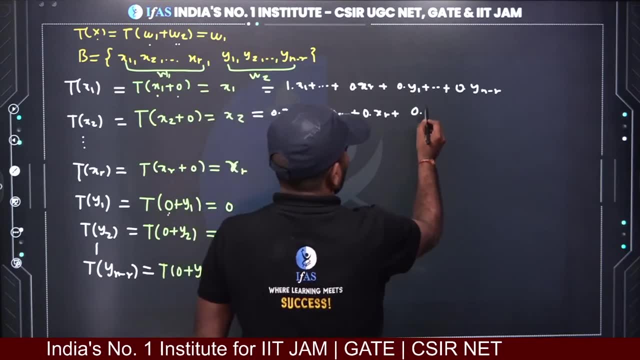 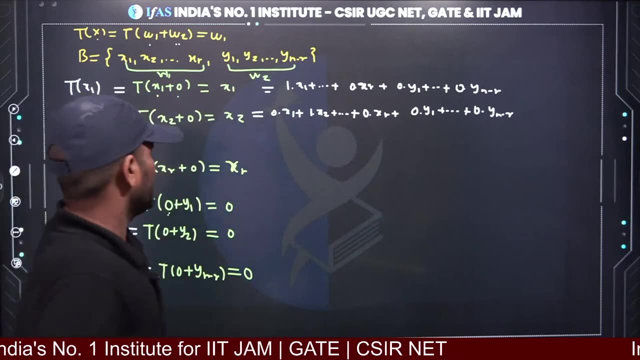 then what will happen? 0 into x1 plus 1 into x2, and so on, rest all 0 into xr, and this will be same 0 into y1, and so on. 0 into y n minus r, and this will be same 0 into x1, and so on. 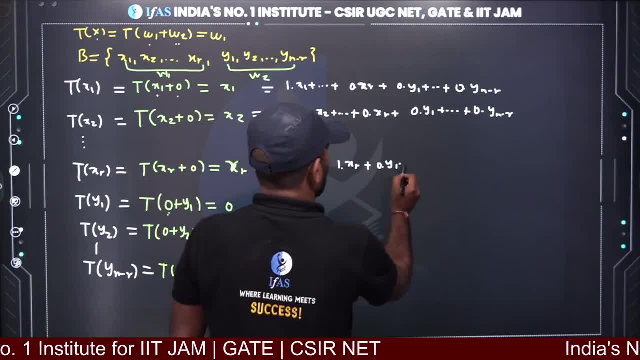 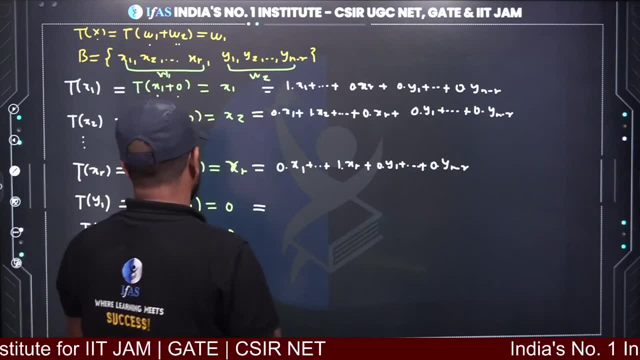 1 times xr plus 0 into y1, and so on. 0 times y? n minus r, and this is equal to what will you get in the end? all will be 0,, 0 times x1 plus 0 times x2, and so on. 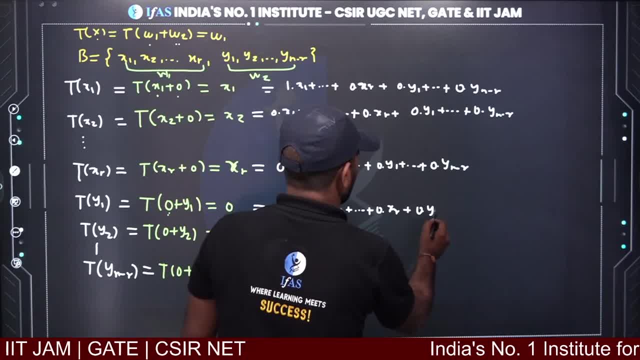 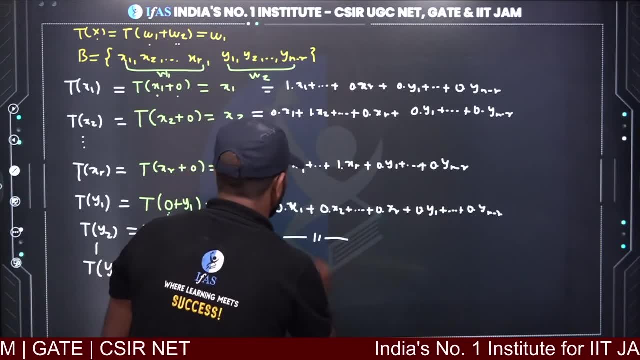 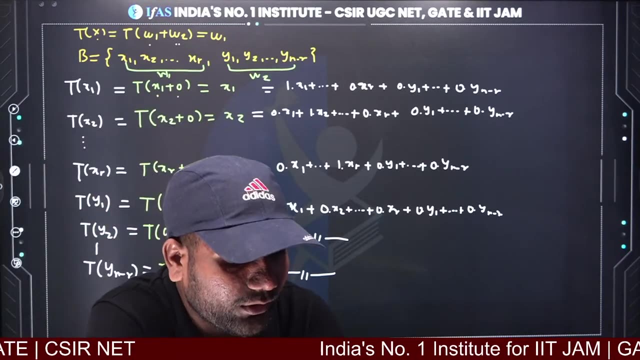 plus 0 times xr, plus 0 times y1 and so on. plus 0 times y n minus r. similarly, you will get the same thing in the end. you have written it like this. now you can convert it in the matrix. tomorrow is the date of the admit card. 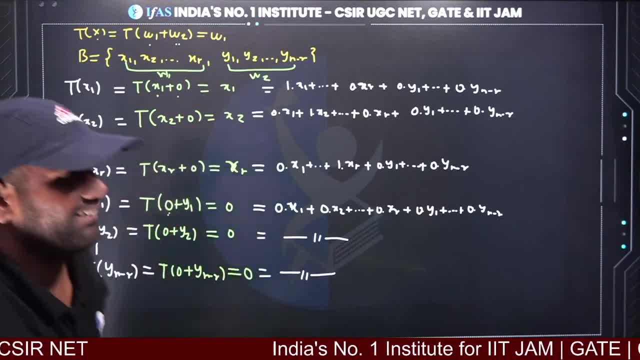 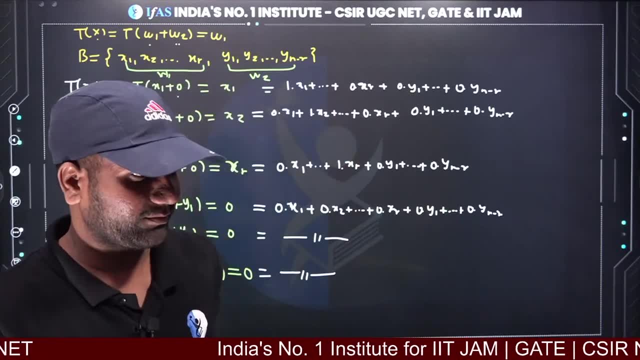 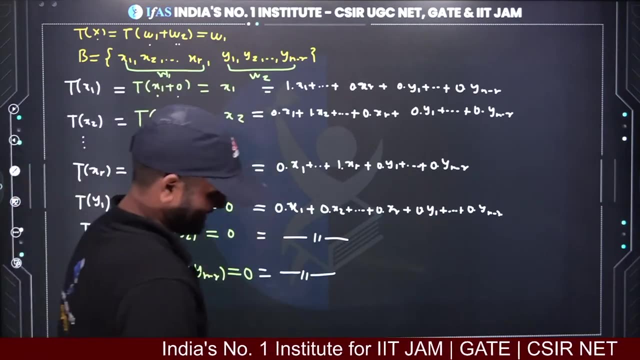 how do you know that tomorrow is the date of the admit card? how do you know that tomorrow is the date of the admit card? who told you? the MTA told you: it's good. if tomorrow is the date of the admit card, then it's good. 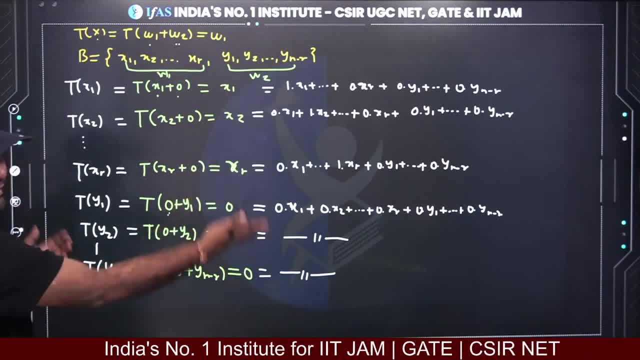 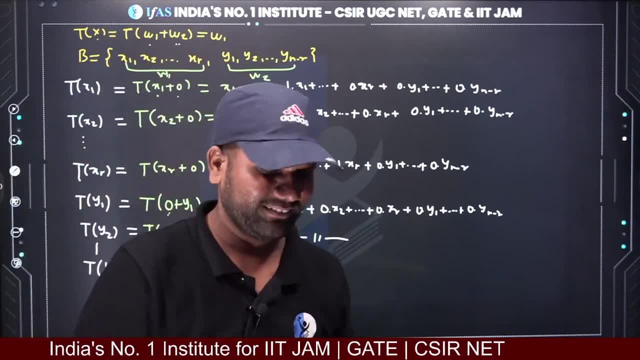 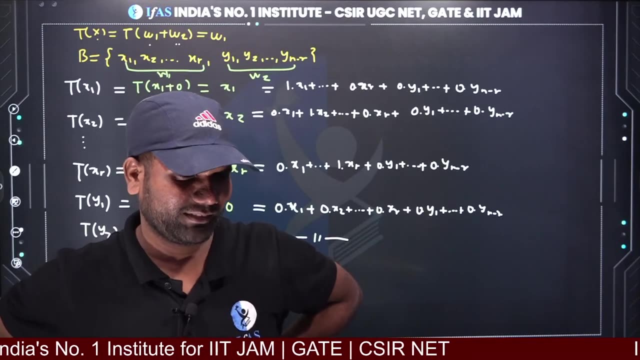 now you can convert it in the matrix. this is what I wanted to show you. if I give w1 plus w2 plus w1, then how will you write it? 33508 Pandit by Vinu Maharaj. if you write surjit r cross r. identity matrix by Vinu Maharaj. 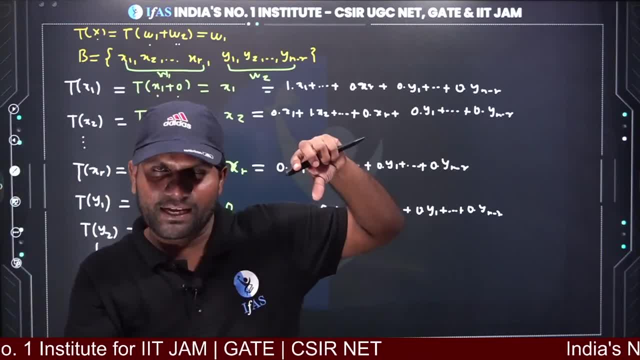 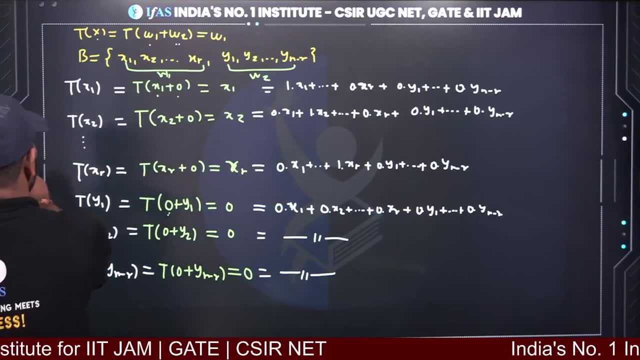 r cross r identity matrix by Vinu Maharaj. the matrix is matter buys er eliminated and after that the below 1 comes to 0 authorities 處34 b of x and by n minus r plus n minus r sulla. all the others will be set as zero entries. 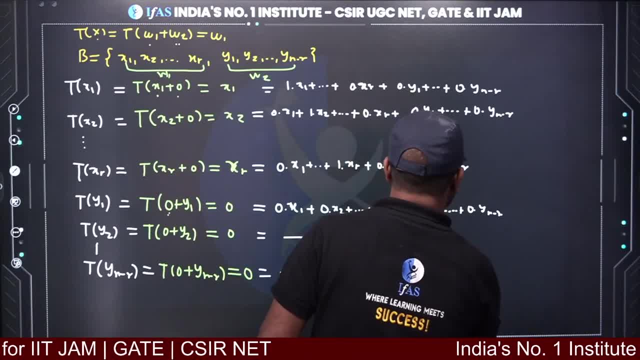 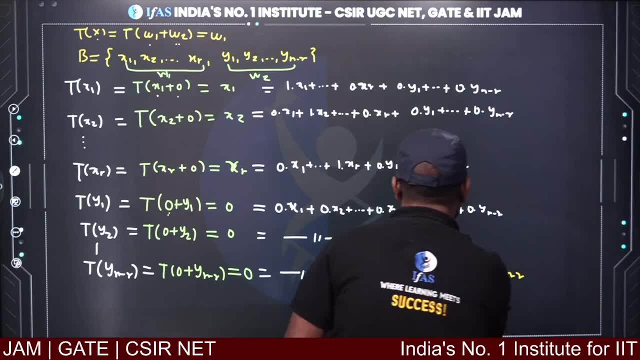 I will give you an hint here, Trدا, we will write it like this: ts. this will be its matrix representation. this will get identity matrix of order r across r and zero. matrix of order n minus r, cross n minus r and the rest of the entries are zero. 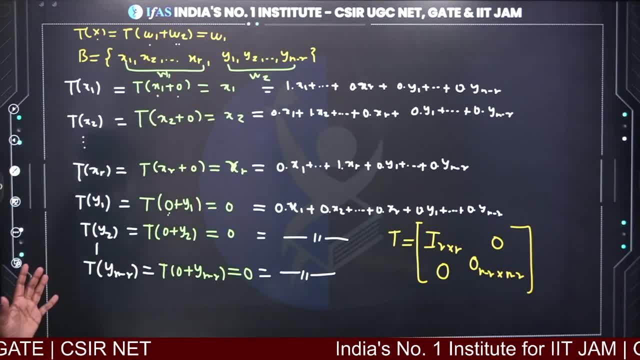 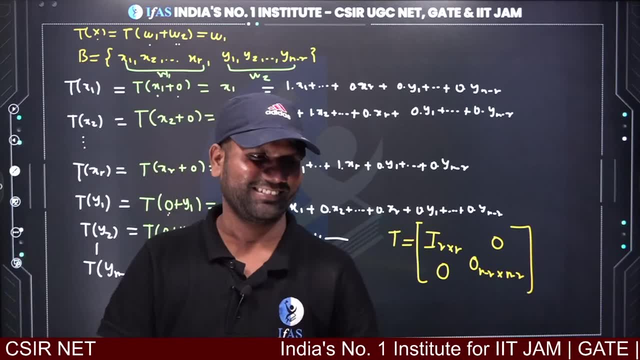 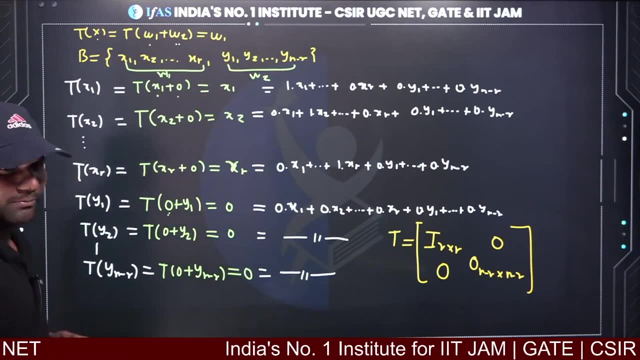 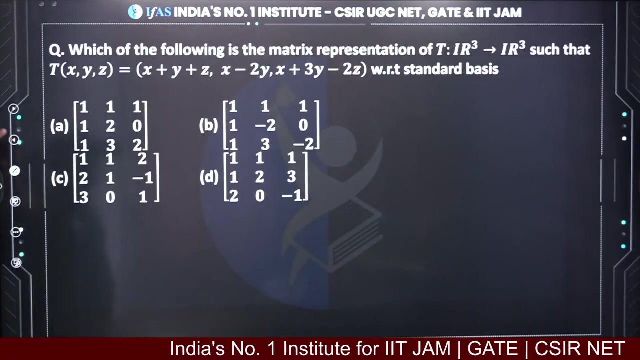 and all others will be zero. it will get to you problems. soon it will be n cross n ok, come on. it was fine till here. ok, you only get the wedding auspicious time. come on, very good, come on now. there are some questions here for you. 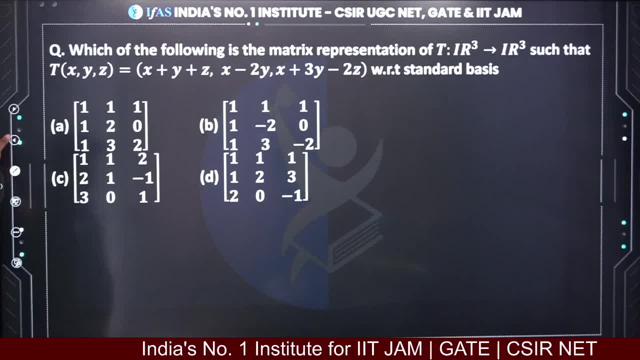 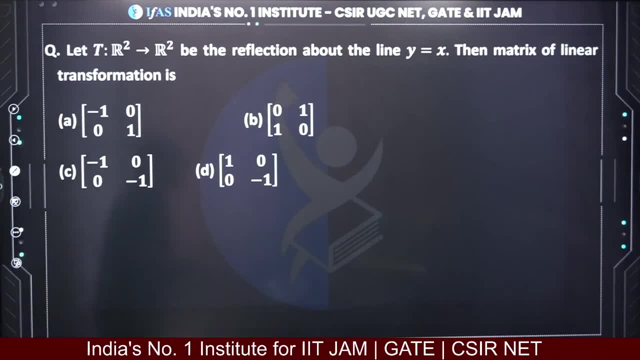 take a screenshot of it, solve it later and tell you. see, it is simple, see, there are chances of being asked such questions in the exam. ok, no, it will not happen. Ruchi will not be possible. ok, you guys prepare it. it will not be possible. such people who 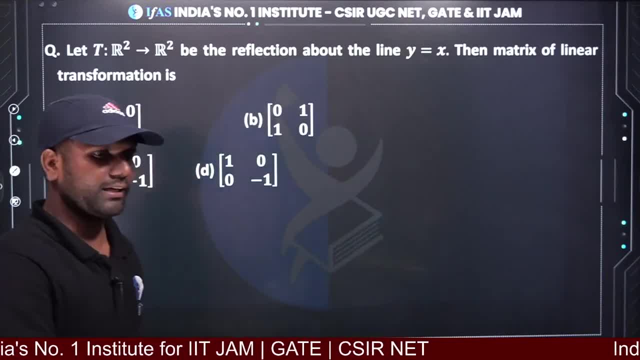 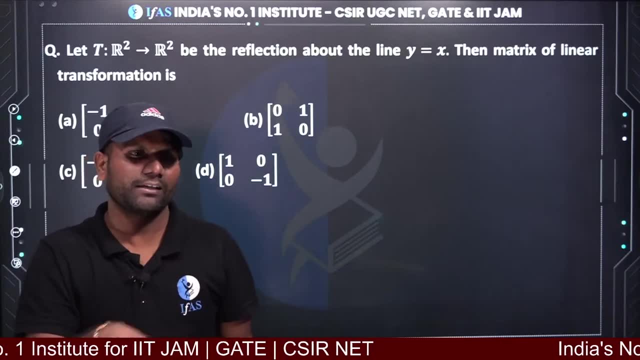 have not liked it yet, then you like it. ok, now I feel that now I will end the session. tomorrow we will do the final revision of the linear by doing the diagonalization, jc form, quadratic form and ips. ok, the one who will take me from the point of view of the exam. 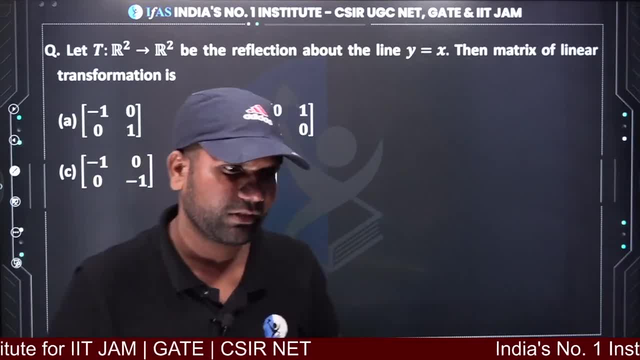 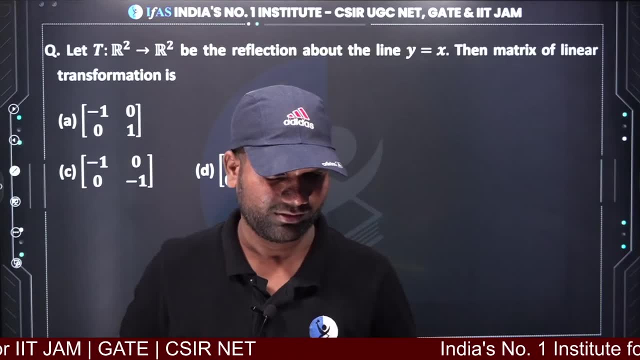 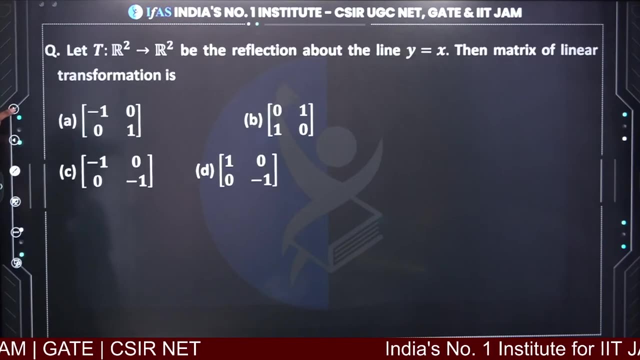 which is very important, can be asked in your exam. you should. ok, we will do it. it will not happen. the exam will be postponed. it will be postponed right now. you also have a question. take a screenshot of this. you guys solve all these questions. 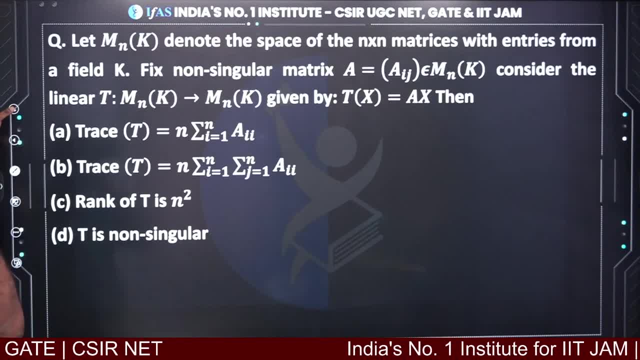 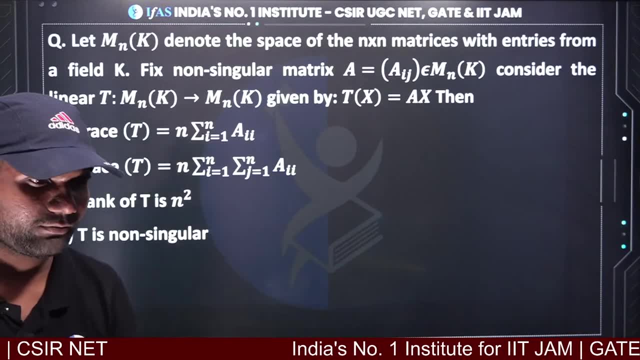 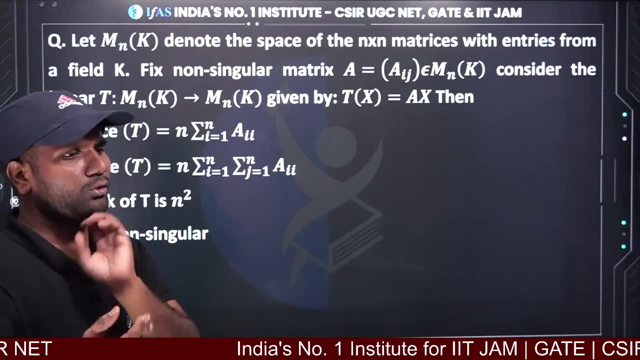 later comment on me and tell me: oh, I forgot this beautiful question. come on, I will tell you tomorrow about it. there is a story behind it. how to solve it. ok, we will take this. Okay, you guys try today. if the reflection one or this one does not come, then I will come again tomorrow. we will talk tomorrow. okay, you guys try today. 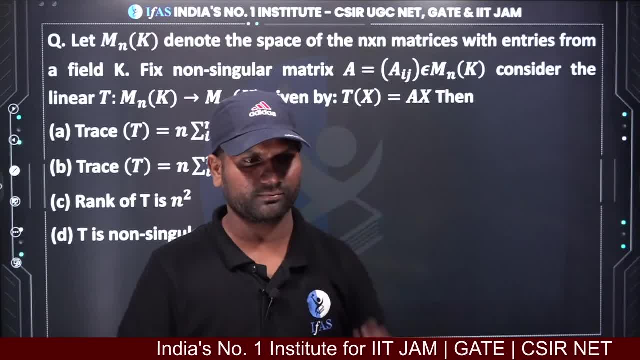 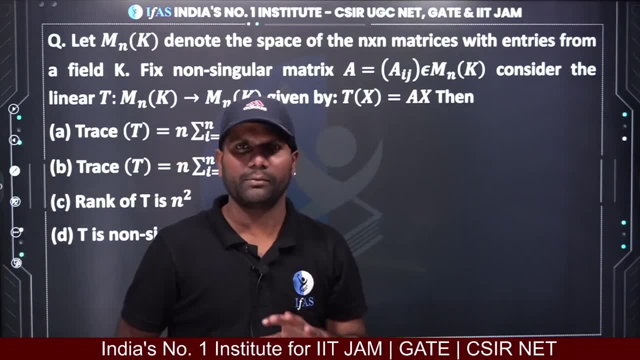 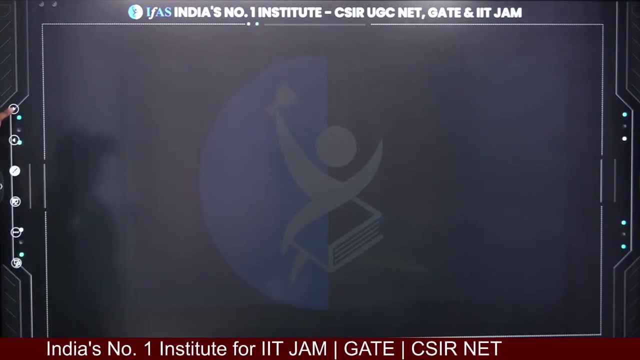 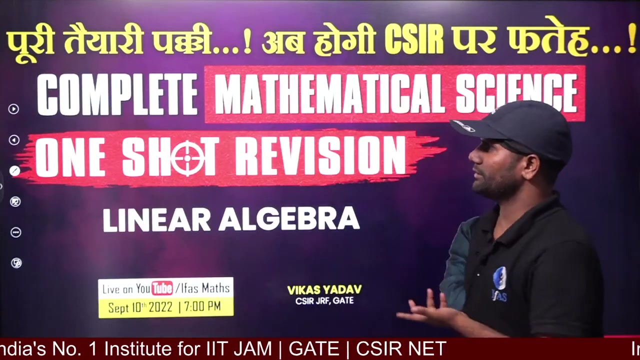 And, by the way, you must be thinking why I have not worn a cap. so I took out the hair and I have all the hair. there is no hair. okay, let's go Tomorrow. we will meet at the same time. this will be the channel. I will also be here. you guys will also come at 7 pm. then we will try to do all the remaining things tomorrow, okay. 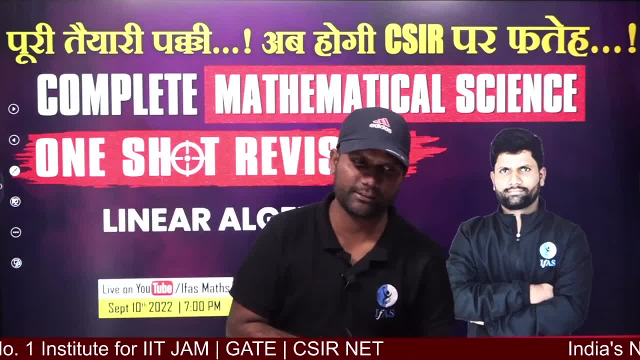 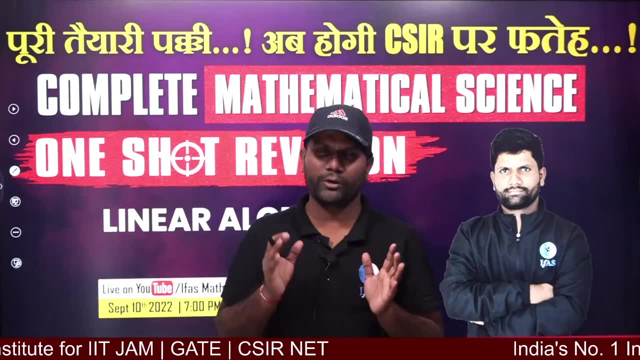 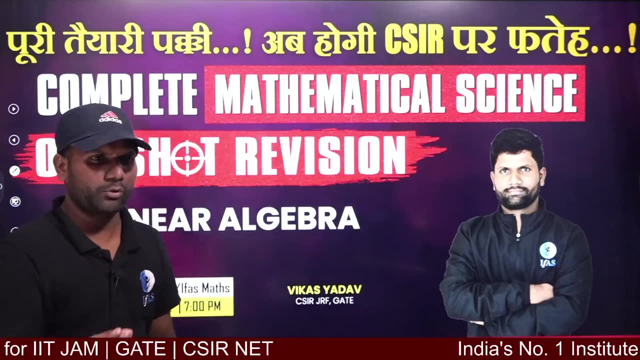 So whatever session you guys have, you can comment and tell once. okay, now you guys don't have much time. there is only one week. the exam is on Friday, right? So you guys read it well once, as much as possible. you will revise the maximum whatever notes you have made, wherever you have taken the result property. 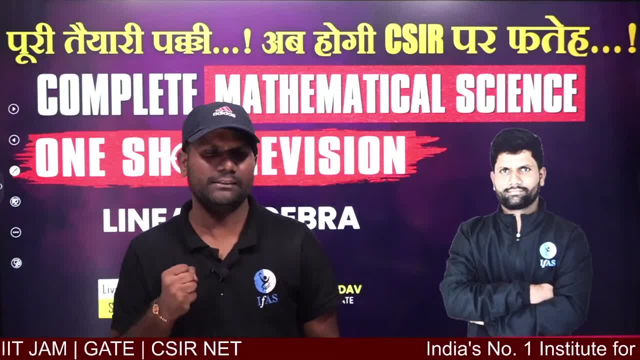 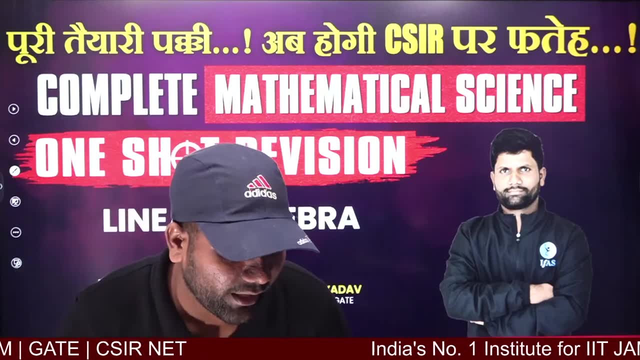 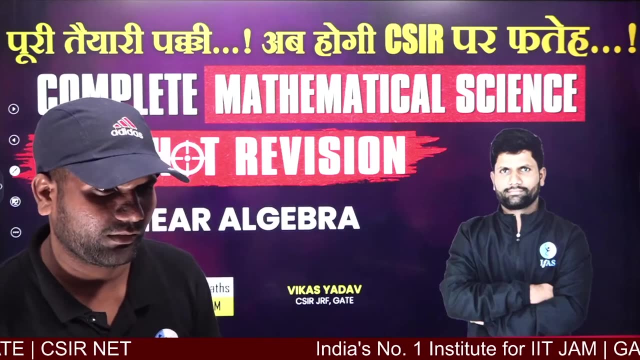 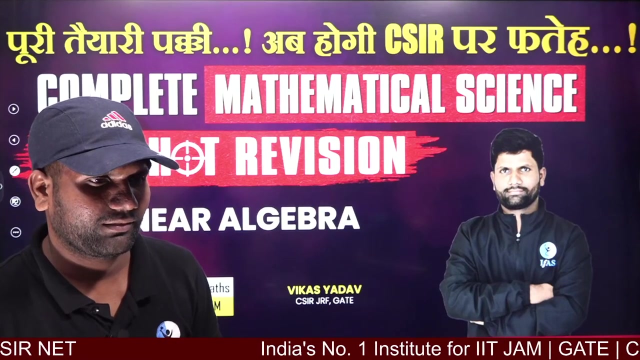 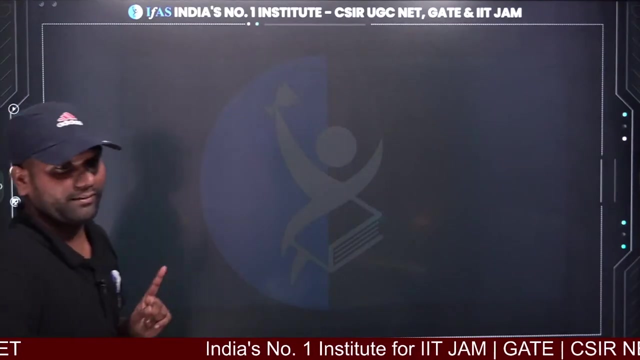 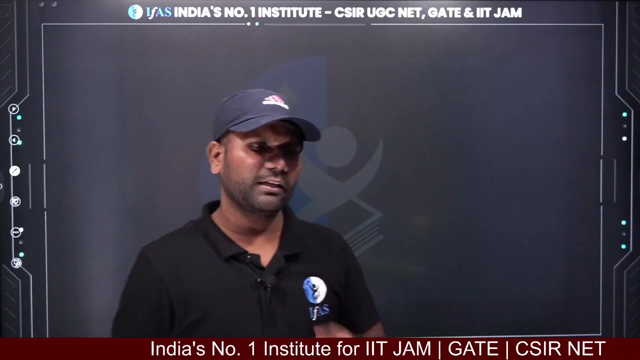 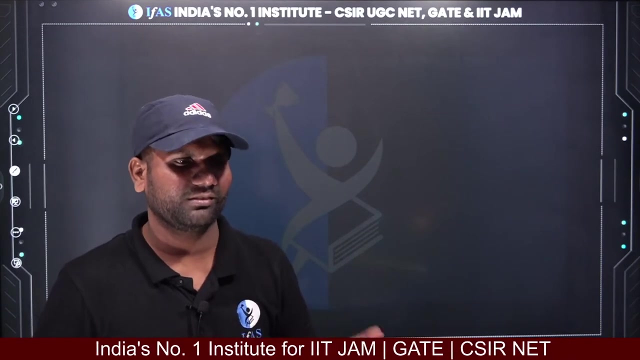 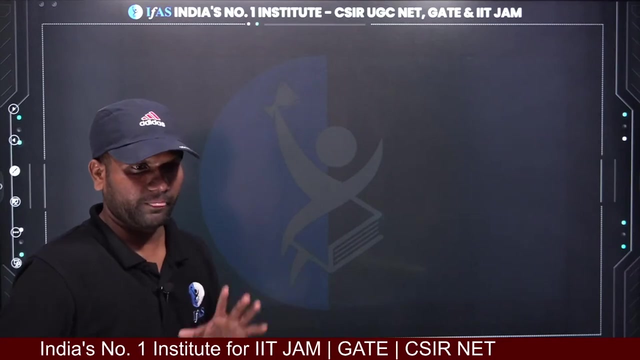 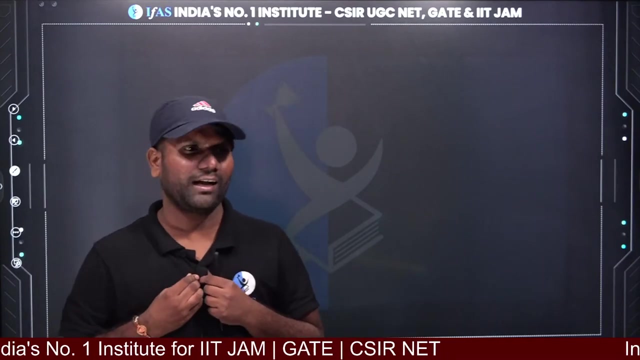 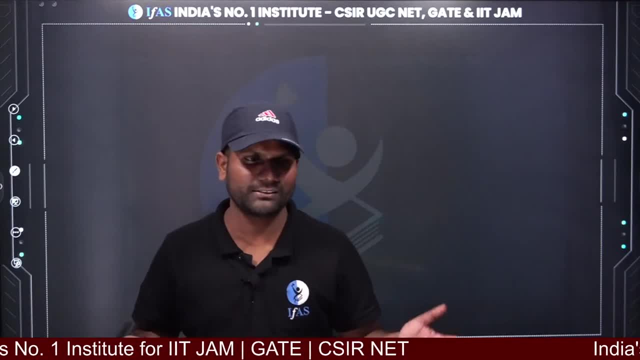 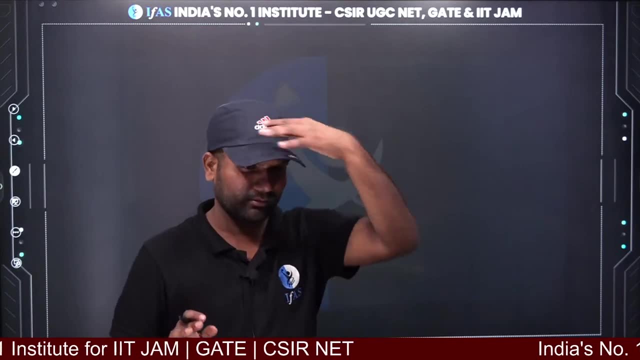 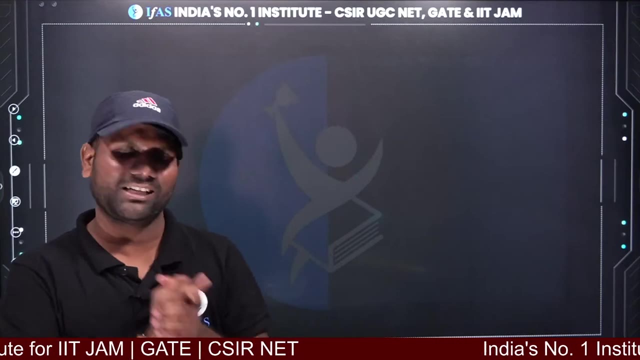 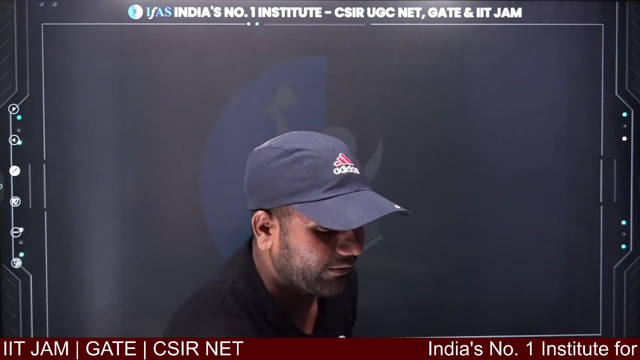 We will meet you here after talking to you for many days. it was very nice, ok? no, no, alpha, I have all. there is no such thing. people must have seen in the lecture in the classroom. ok, next class tomorrow evening at 7 o'clock. tomorrow evening at 7 o'clock, same YouTube channel, same person will be there and you will also be there. come on till then. thank you, bye, bye, see you tomorrow. 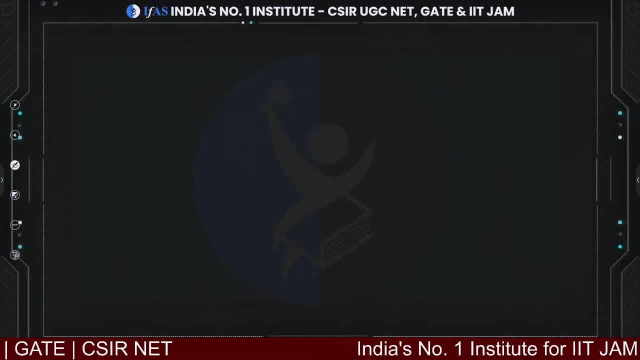 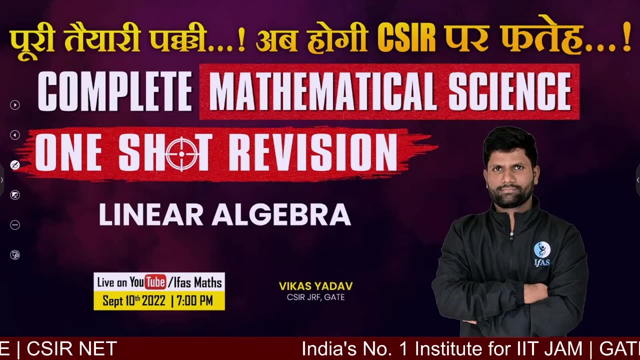 Thank you, Bye, Bye.